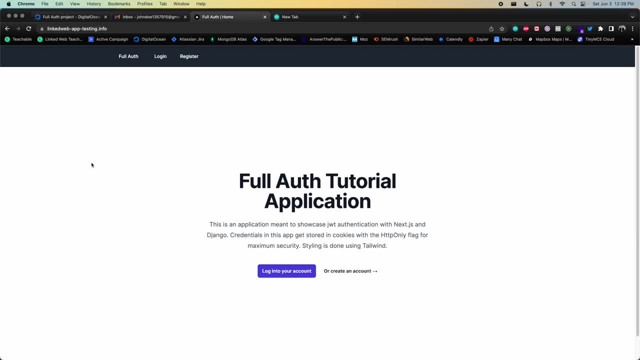 this differently in development and production. So during development we'll handle it more like the standard way you do with Django, And then in production we'll have our static files stored in the DigitalOcean Spaces Also- just something to note for this particular. 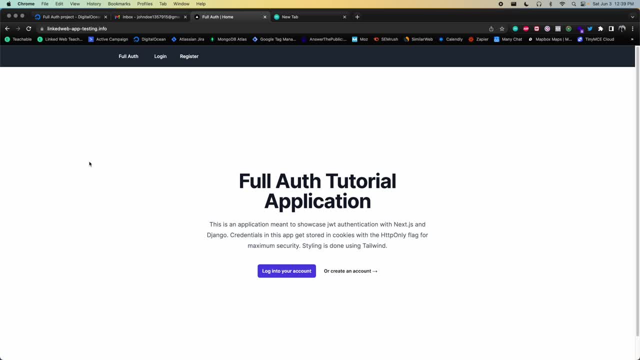 app. setting up the static file storage in this way is pretty overkill, since there will barely be any static files in this particular app. But the reason I implemented this way is just so that you can see how you can do the sort of setup, And then also because, realistically, you'll never have 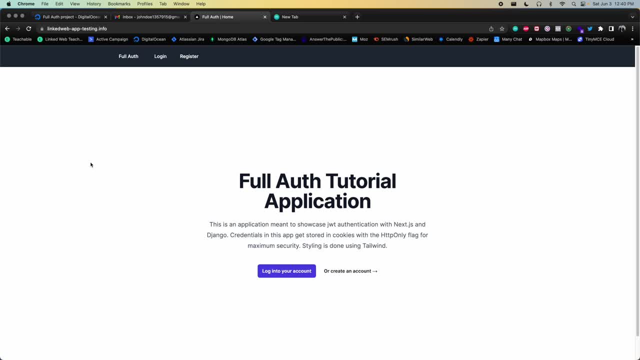 an app that does just authentication and that's it. Typically, an app that has authentication will have tons of other features built on top of it as well. For example, you might have a social media app, and then you can have users that store all kinds of posts and images. 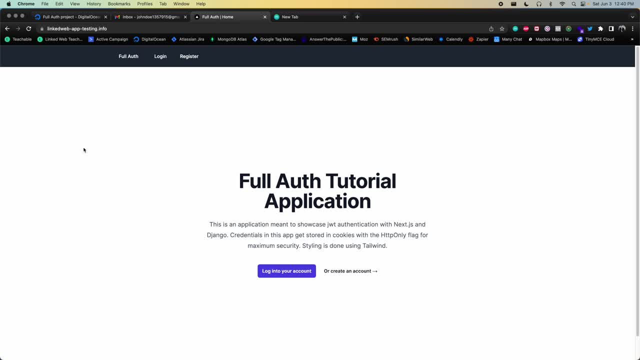 And then in that kind of case, a solution for static file storage, like I have implemented here, would be a lot more effective. So just wanted to put that out there, just so that it's clear why we're doing things the way that we do them in this app. And then other things to note with the 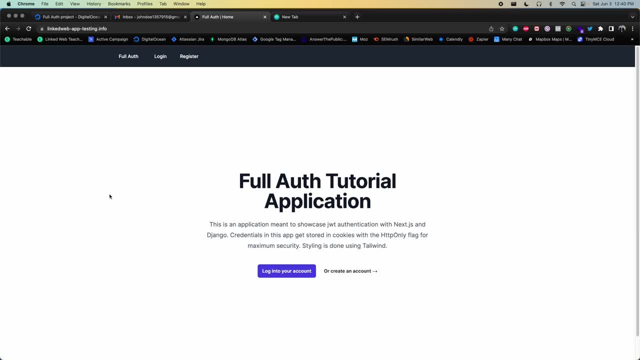 backend. we'll be setting up a custom user model And then that way, users can register and log in using an email and password. We'll be using the Joeser library to help us quickly put together a fully featured authentication backend API, And then you'll also see how to easily 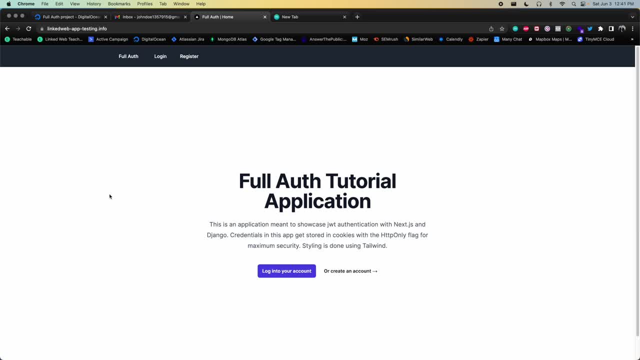 override certain behaviors in a library And then that way you can get it to do something specific to what you want in your particular use case in your app. And then what we're going to be overriding in particular in our app is how the JSON Web Token authentication endpoints behave. 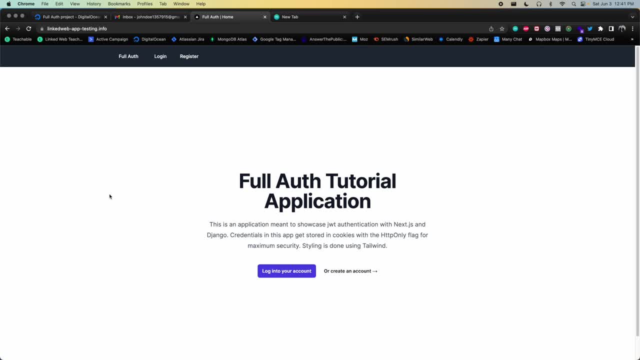 as well as how the authorization behaves. So, by default, the way that things will behave is that when you hit an endpoint to create your JSON Web Token credentials, you'll get back in the response data, your access and refresh tokens, And then you'll also need to. 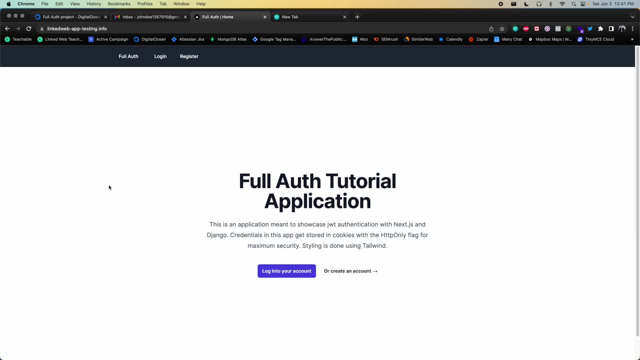 store them somewhere. Then to make authorized requests you'll have to pass an authorization header And then you're going to have your access token in there of the value in that header. We'll be changing this behavior so that instead the access and refresh tokens get stored in cookies. 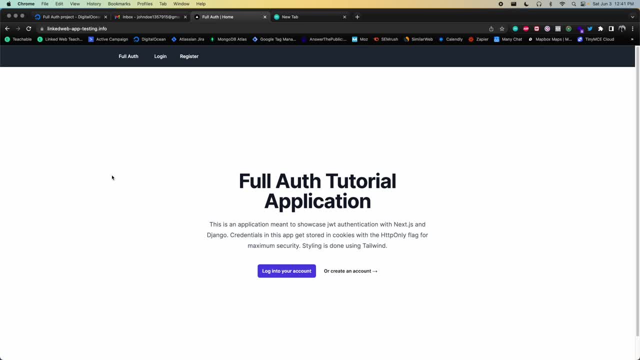 with the HTTP only flag set to true, So that way, client side JavaScript won't be able to read the values of these credentials and they're going to be stored in a very secure way as a result. And then we're also going to see how we can override the authorization so that you don't need to pass. 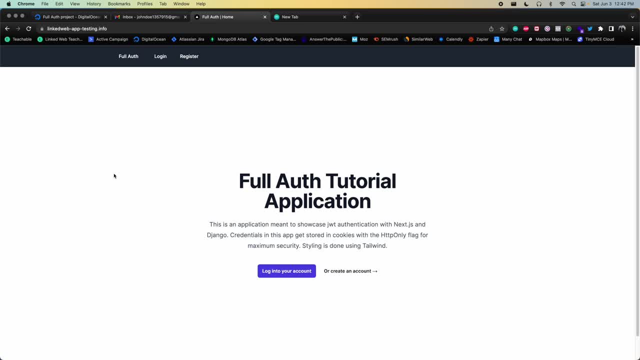 an authorization header, But instead you'll just have the access token which is in a cookie, and then you'll just extract that value and use that to make the authorized request. Then we're also going to see how to implement social authentication with this app. 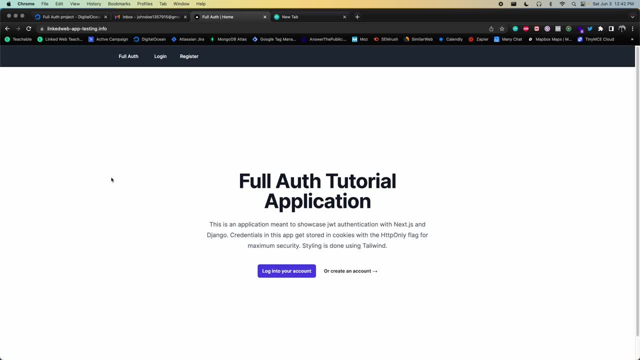 and we're going to be using Google and Facebook OAuth 2 in order to implement this. Now for the front end. to build out the front end, we'll be using Nextjs 13 with the app router. We'll be using Tailwind CSS for the styling, along with things like headless UI. We'll also be using 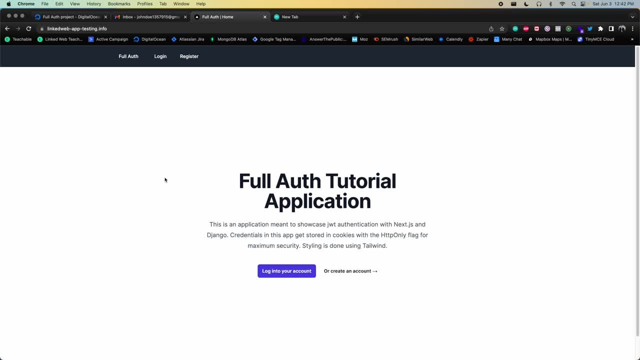 RtkToolkit for our global state management for the authentication and RtkQuery for our client side requests, And then these will be the authentication requests, because that's the only feature we really have in this app. So you'll see how to configure this setup with Nextjs 13's app router. 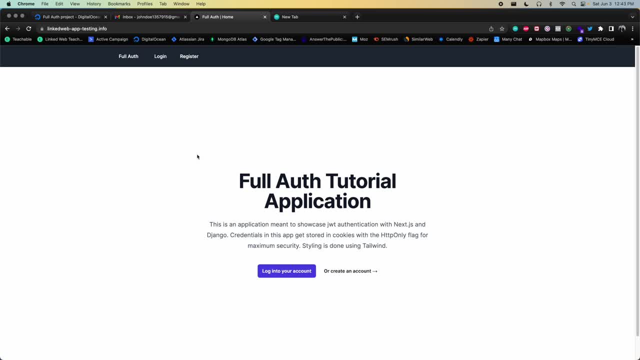 Then another thing that we'll set up with RtkQuery is automatic reauthorization. So this means that anytime we hit an API endpoint where we're unauthorized to make the request- which will frequently happen, because we'll have access tokens that expire after five minutes- what will happen in this case is that when we get this unauthorized, 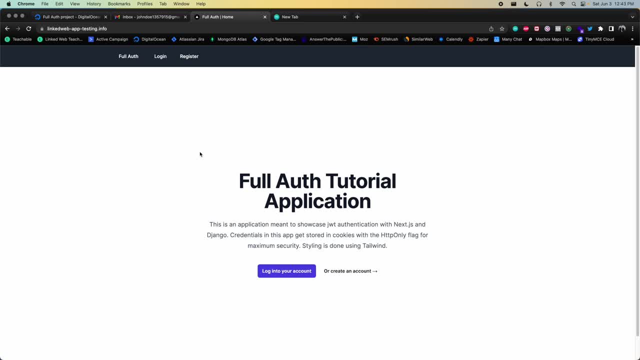 response. we'll automatically, in our app, hit a refresh endpoint using the refresh token that's stored in our cookies. We'll get back a new access token and then we'll retry the unauthorized request with the new access token, which will now be valid, And so the request will work during the. 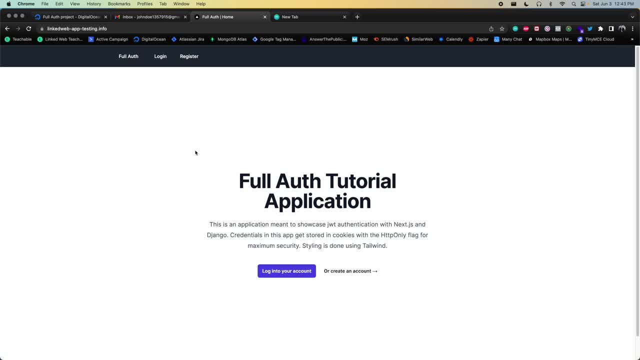 retry. Now I just want to point out that in this particular app, with this setup, we won't be taking advantage of certain things in Nextjs 13. 13,, such as the server-side data fetching, So our app will instead be doing client-side. 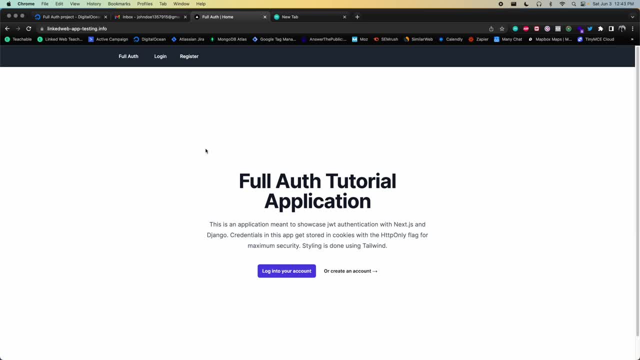 data fetching and caching with RtkQuery. So currently with RtkQuery, we can only make client-side requests with the server components, and that's why we're doing that in our particular app. However, in an app that builds on top of having authentication, you would technically 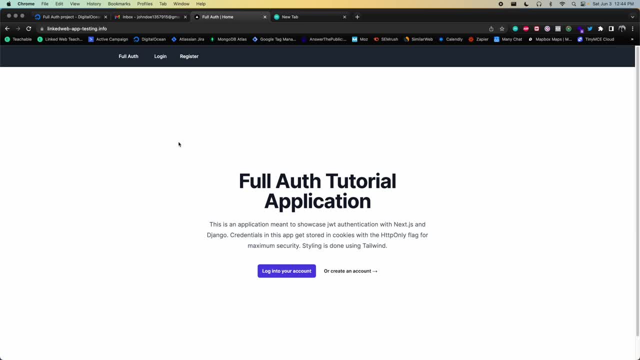 have many features that could take advantage of things like server-side data fetching. So, for example, an e-commerce app is something that you could build on top of this authentication system and that will have things like product data, which is a great use case for things like server-side data fetching. 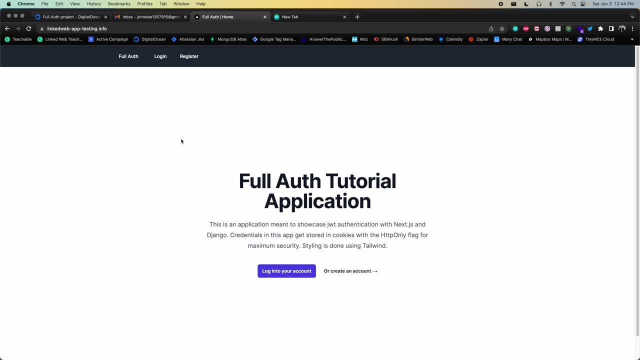 of the products And then when you're on, like a shop page or product detail page, in that case you could take advantage of these sorts of things. But in our app, since we're using RtkQuery with the automatic reauthorization setup for our authentication, 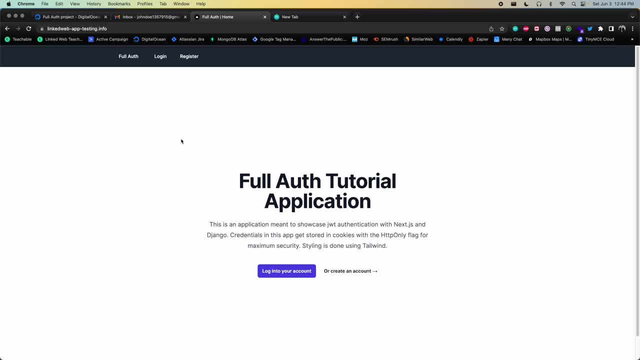 endpoints, we'll only be doing client-side data fetching, So that's just something I wanted to put out there. Anyway, that is an overview of what we'll be going over in this series, And next I'll go over the actual app itself. 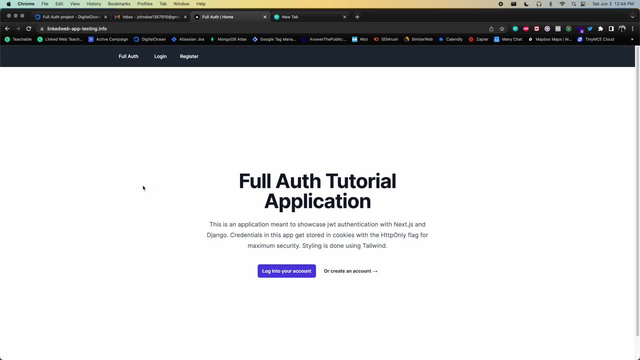 And, as you can see on the screen, this is an app that is running in a production environment on DigitalOcean with our DigitalOcean setup right over here. But before I get into the overview of the app, make sure to hit that like button on the video if you haven't done so already. 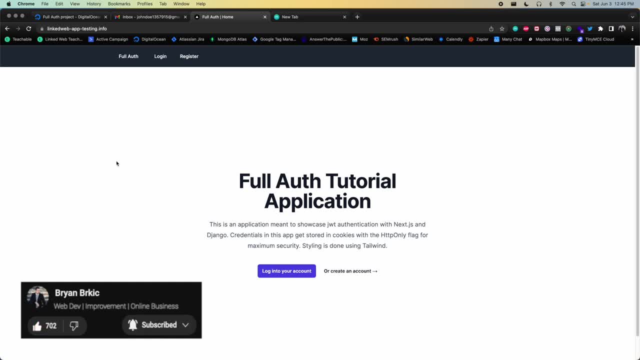 Helps the YouTube algorithm so that more people can find this kind of content. Also, hit that subscribe button if you want to see more content like this, and hit that notification bell if you want to be notified when I release new videos. And with that, let's get into the overview. 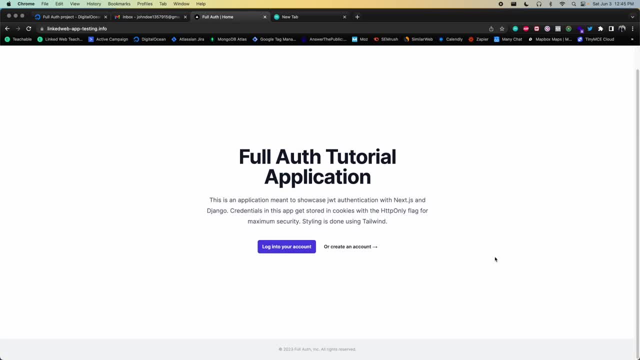 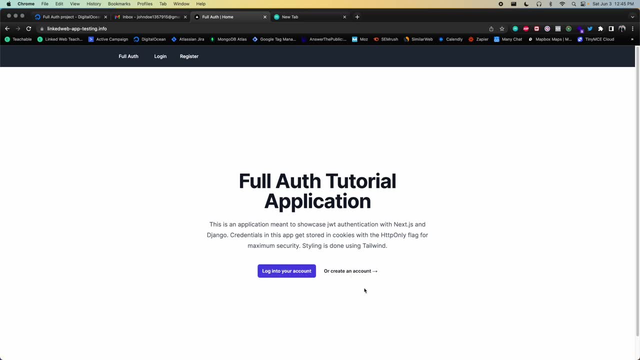 So here we go. We can see, this is the homepage, styled with Tailwind CSS. We have our navbar, we have our footer and then we have our login and create an account- buttons that we can click So I can go to create an account. That'll bring me to the signup page, So let's go ahead and sign up for an account. 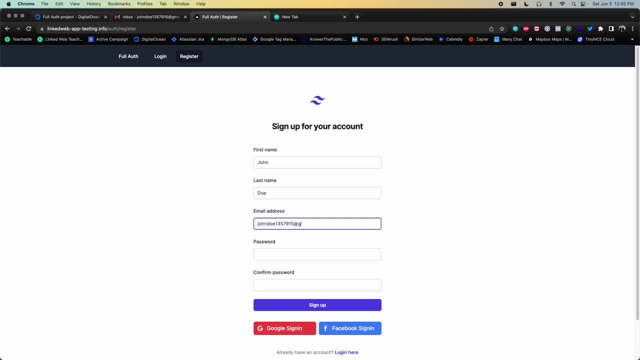 So I'll sign up with a John Doe account. So there we go. We put in the credentials, and then you can also sign up with Google and Facebook, but first I'll show this, So I'll click the signup button Now. we're also going to have alerts in. 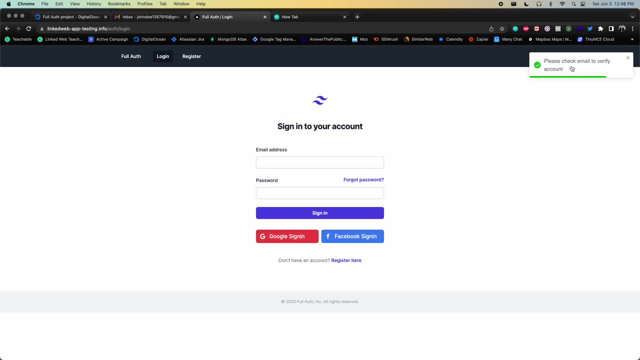 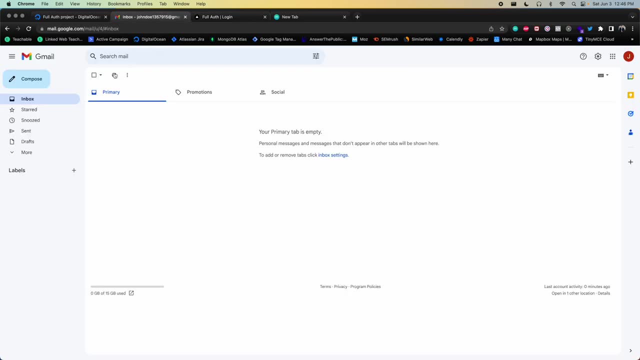 this app. So these will be handled with react toastify. So here we can see an alert for please check email to verify account. So I can now go into my email. Then if I refresh, I should receive an email. So this one ended up going in the promotions tab, So let's make sure it's over here. 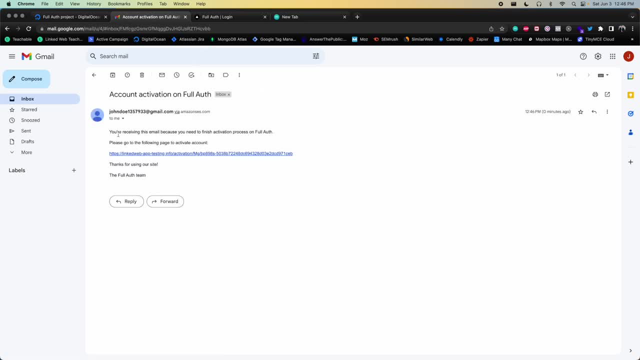 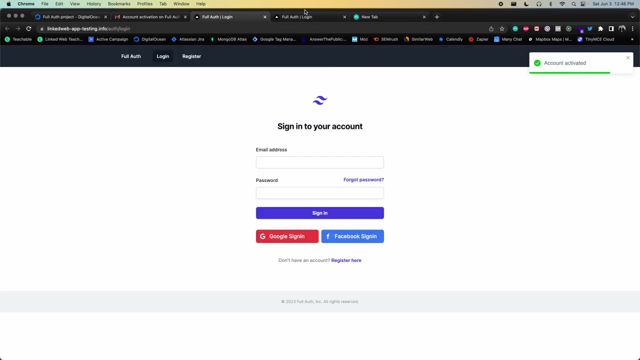 I'll click on this. and now I get a link. so i see you're receiving this email because you need to finish the activation process on full auth, which is the name of our app, and then please go to the following page to activate the account. so i can just click on this and there we go, account activated, just like that. so now. 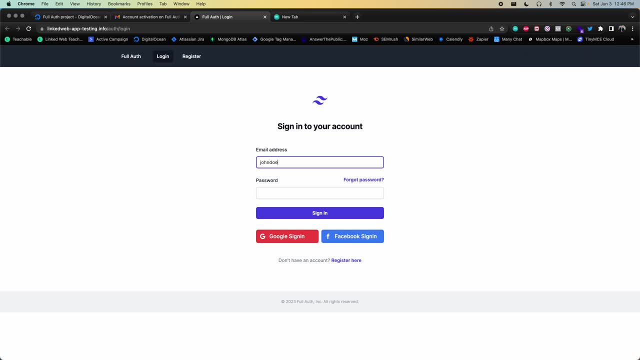 i can log in with this account. and there we go, we're logged in and now we see we're on a dashboard page. we also see our navbar was updated, so now we have dashboard and a logout button. so i can see happy- first name: john, last name: doe, email. so all of the things that i signed up with on this account. 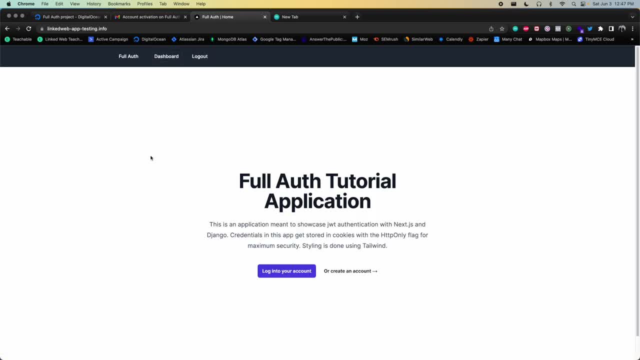 i can go back to the home page dashboard logout. i can refresh the page. i'm still logged in. so in this particular case, we use things like our verify route in order to make sure that we have a valid access token and if we end up being unauthorized because, let's say, more than five minutes passes, so our access token expires. 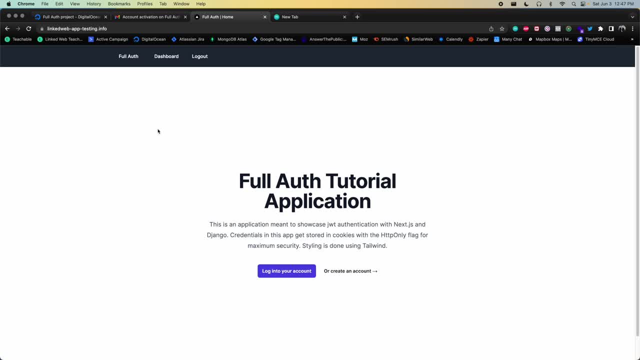 when we refresh the page, we're going to get a 401 response. so we're going to go, hit the refresh endpoint automatically, get back a new access token and retry the verify route, which will do a lot of work for us. so we're going to go ahead and hit the refresh endpoint automatically, get back a new access token and retry the verify route, which will do. 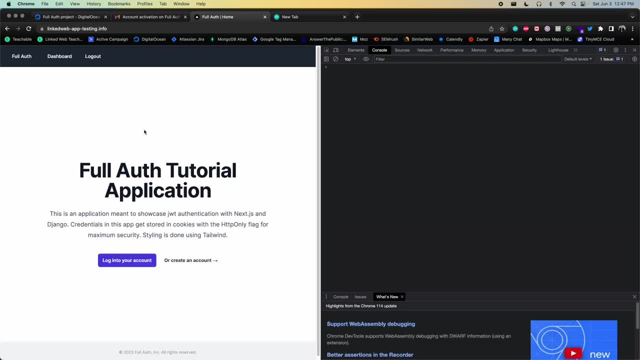 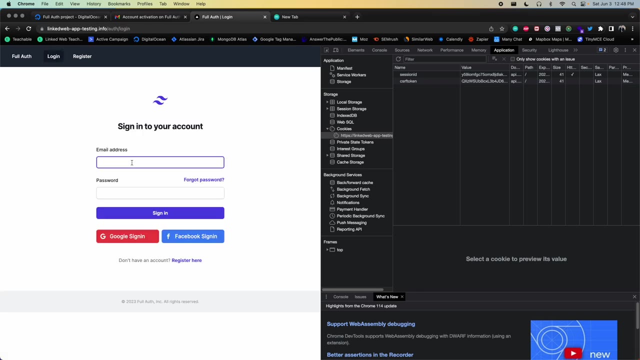 then succeed and keep us logged in. i can also open up the console along with the application and then here i'm going to have to log out and then re-log in, just so that we can see the access and refresh tokens here. so if i log out, go to login and then i log in. 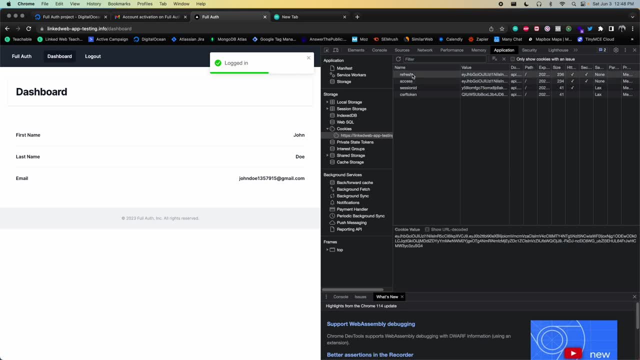 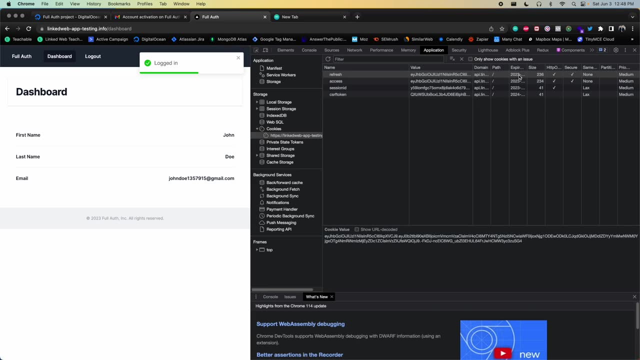 so i'm going to see that the access token is here along with the refresh token, and then we can see some other properties on this as well, so we can see that the domain is set up, the path when it expires, the http only flag, which is an important one. so these cookies here, they cannot be. 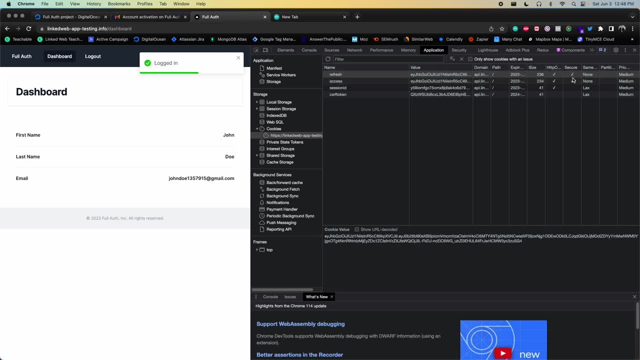 accessed with client-side javascript. because of this setting here, they also have to be secure, so they need an https connection, and then we also have same site as none, and this is because our front end and our back end are on different domains. our front end is on this domain and 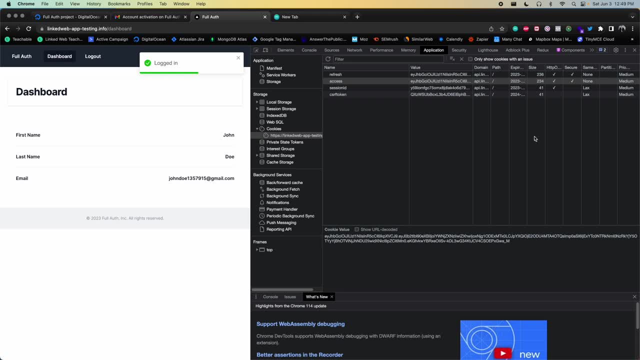 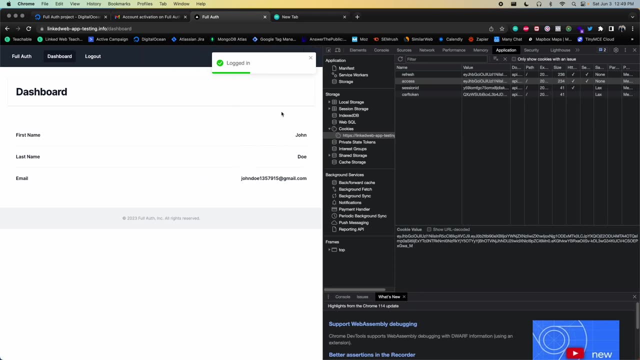 then the back end is on a sub domain, so we're also going to see how that works. so we're going to see how to do that setup so that this works properly and the cookies get sent in the requests and yeah. so now back in the app. if i'm on the dashboard page, i click log out, i'll get navigated. 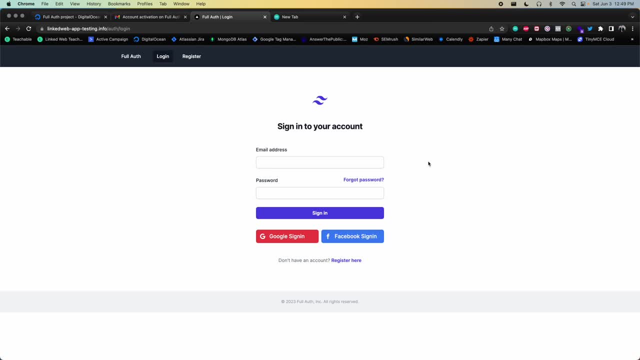 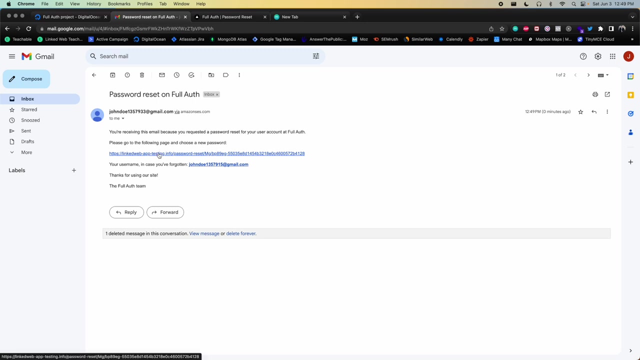 to the sign in page. so now the next thing i'm going to show is the forgot password. so if i click on this i can put in my email and then i'm going to request a password reset. so request sent. check your email for reset link so i can go back. i'll get a new email password reset on full auth. so now i can click. 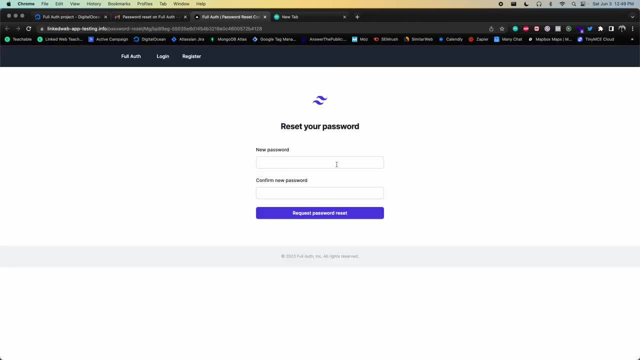 on this link and then here i'm prompted to put in a new password. so let's go ahead and do that. and then it seems that i didn't have these passwords match. this is also a great thing. it shows what happens if the passwords don't match. it won't end up working now if they do match. 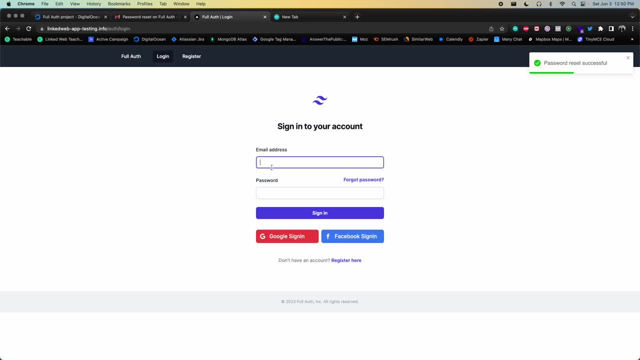 there we go. password reset successful. so now i'm going to try to log in with the old password. and if i try to log in with the old password, i should not be able to log in. so there we go. failed to log in, so now if i put in my new password and sign in with that, 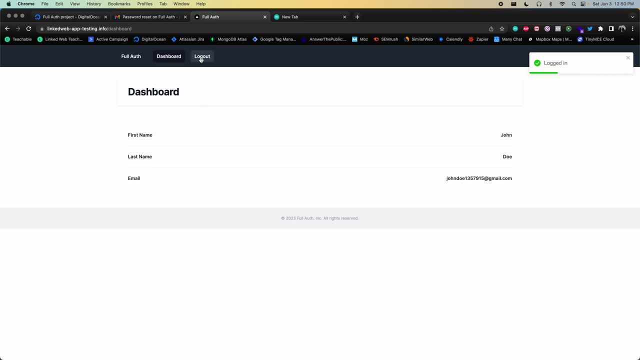 there we go, it works. so that is the password reset. and then only one more thing to showcase in this app, and that is the google sign-in and facebook sign-in. so if i click on the google sign, here's the google sign-in page. i can click on this account. 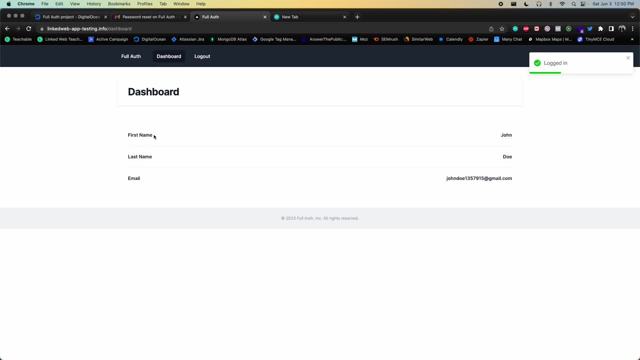 and there we go, i'm logged in with that account, and then the final thing to showcase will be the facebook oauth2. so if i click on this button instead, there we go, i'm logged in, and i can also see that the first name and last name is slightly different than the other account, because these are 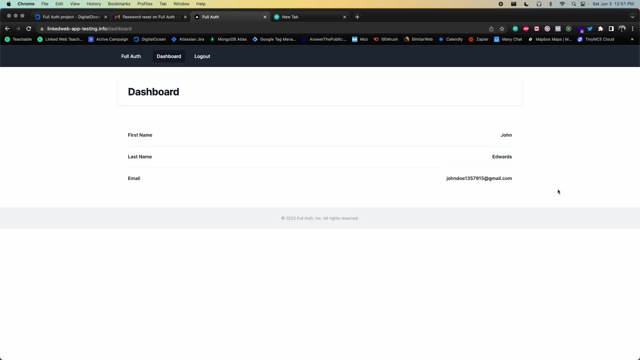 the details on the facebook account for this email. so we can see that now we have an email and a password login, we have account activation, we have password reset and we have social authentication with Google and Facebook OAuth 2.. So that is the complete overview for this. 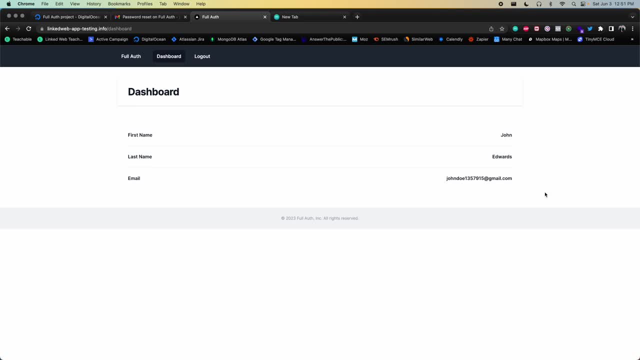 particular app. And now what I'm going to do is in the first video I'm just going to go over the whole setup for just the backend API. So that's going to be with Django, And then the second part in the series is going to be just the Nextjs setup. So that way, if you're interested in just 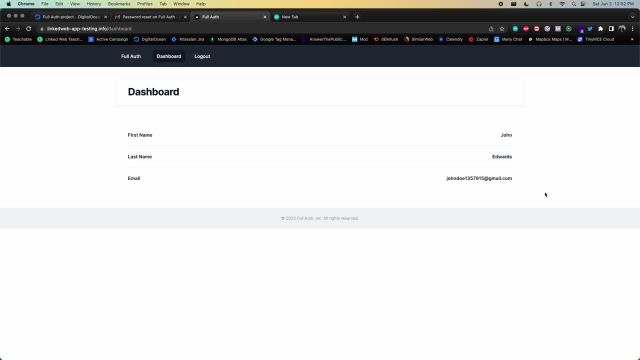 say Nextjs, then you can just go to the second part of the series And then you'll just have to configure the backend API so that it works on your local system And then from there you can just see how you can implement this sort of authentication system on the front end with. 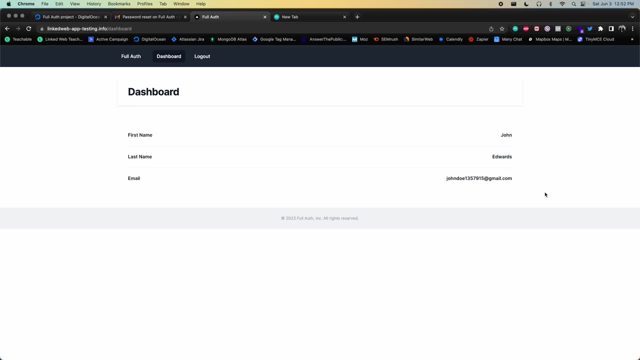 Nextjs app router. If you're interested in just the backend API, I'm going to cover that in this video, And if you're interested in both, then you can go through both parts of the series. So with that, let's now jump in and see how we can put together this Django backend. 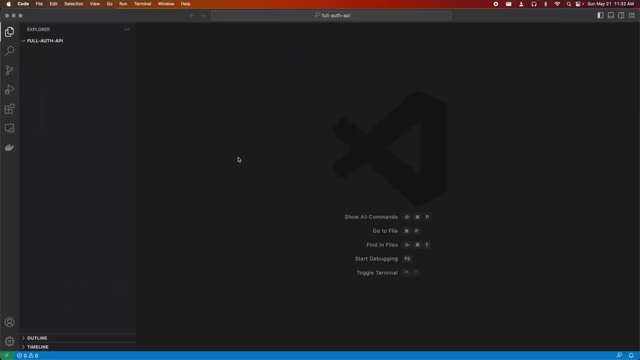 All, right now let's see How we can build out this Django backend API for this project. So right now I have VS Code open, which will be my text editor of choice, And then I have a folder open called full auth API. 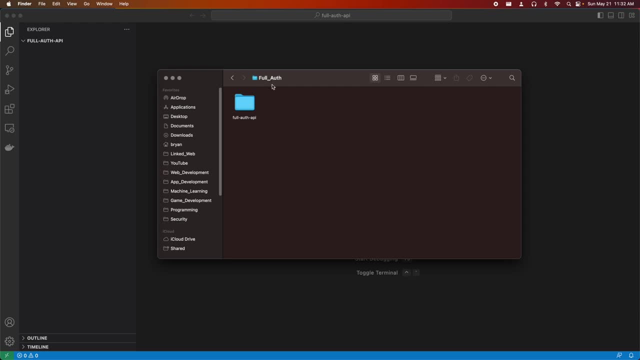 And then this right now is sitting inside of a full auth folder. So I'm going to have my backend API with Django And I'm also going to have my Nextjs project in here as well, just to organize things. So before I get started, I'm just going to show some of the VS Code extensions I'm using. 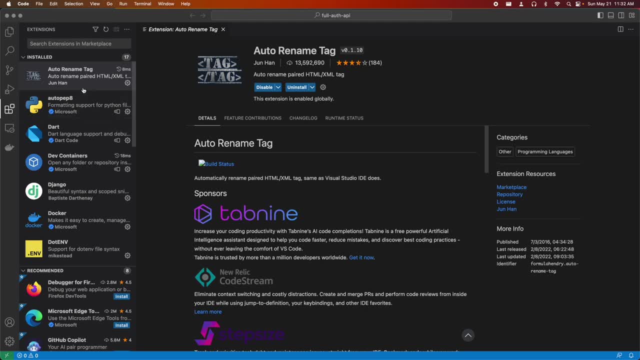 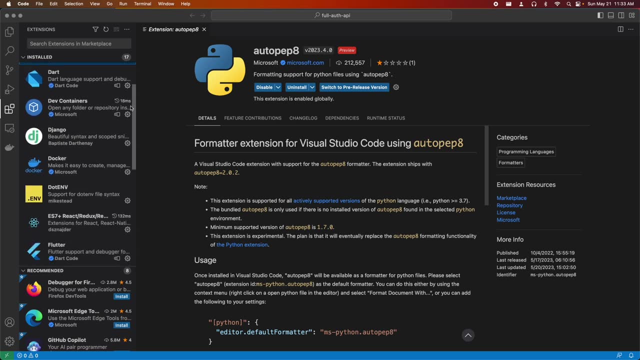 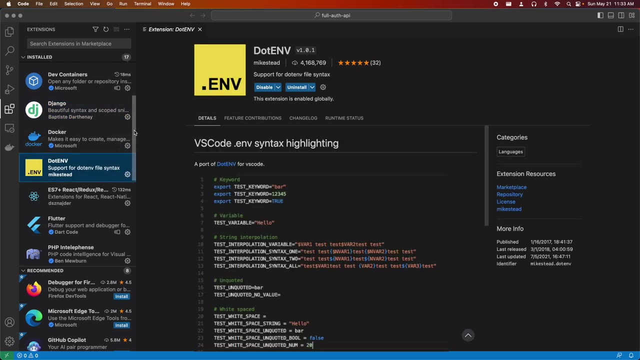 So I have this auto rename tag, Which is pretty handy. This one's more handy for when we get to the Nextjs stuff. Also, I have auto pep 8 as the Python formatter. And then there's this Django extension, which is more useful for when you're working with templates, env. just for some syntax highlighting with env. 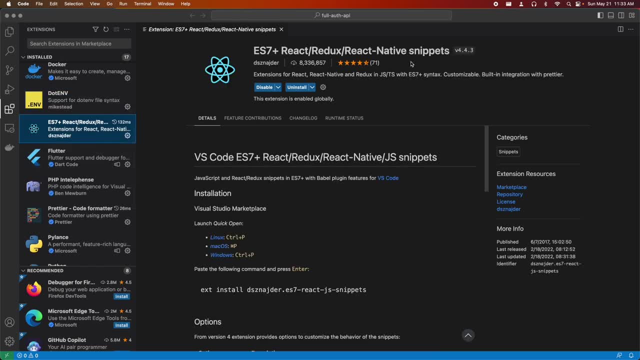 files. And then we also have this React Redux snippets extension. So this one, you get these little commands you can put in and then click tab and then it'll just auto generate some stuff. Now, personally I don't really use this one that much, but it is a useful one. I would just have to. 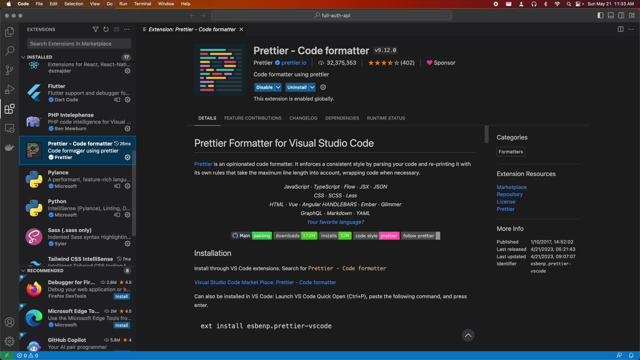 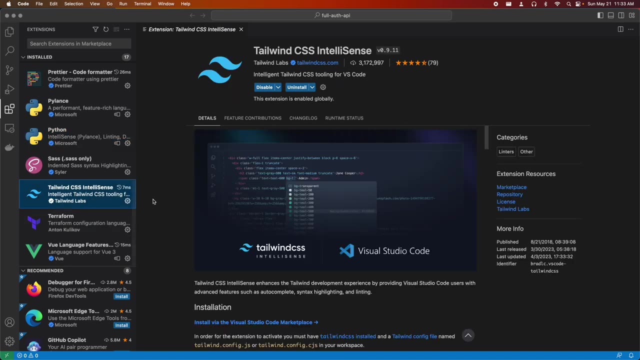 get used to some of the shortcuts. And then we also have prettier, which is the code formatter that I use, except with Python. I'll be using auto pep eight instead. Then we also have this py lance and Python extension, and then we also have tailwinds, So that's going to be something. 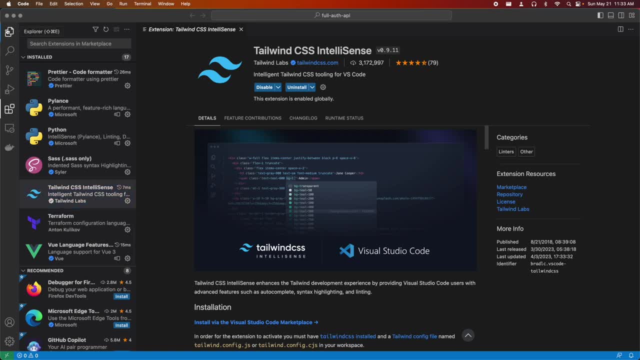 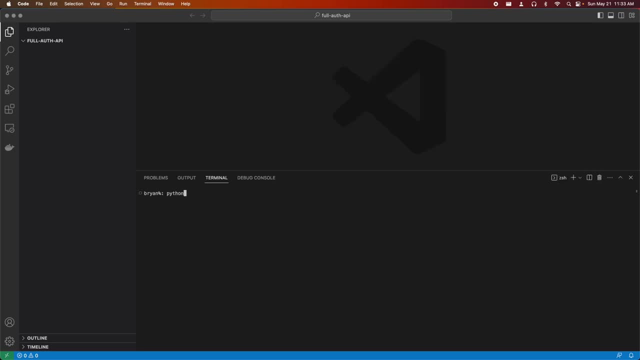 once we get to the Nextjs part. So those are my extensions. So the next one I'm going to do is open up a terminal, So the version of Python that I'm using right now is 3.11.3.. And then I'm going to set up a virtual environment So I can do that with Python 3. 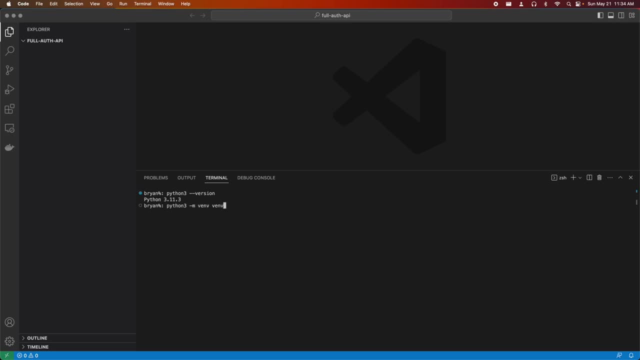 dash m, then venv and then venv. So this is the command. this is the name of the folder. I'm going to have the virtual environment And this way I can have my Python packages installed in a virtual environment instead of on my global system. 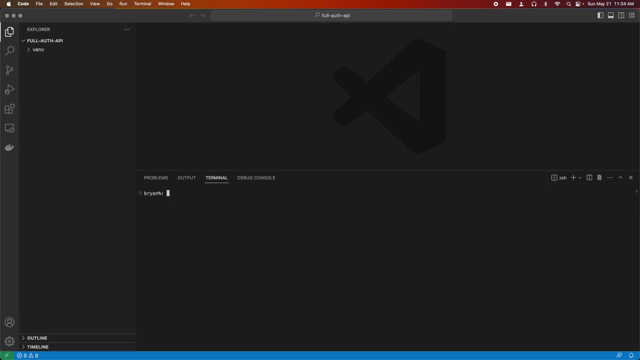 And then the next thing I'm going to do is activate this virtual environment with source venv, bin activate, And if you're on Windows, this will look something like dot, backslash venv, backslash scripts, backslash activate dot. that, Although one thing I do. 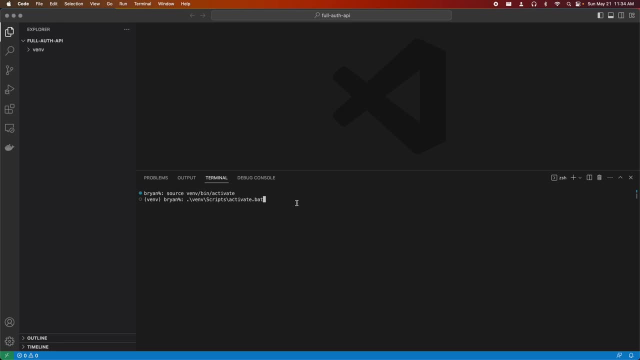 recommend, if you are on Windows, is you can also set up Windows subsystem for Linux, that we can have an Ubuntu environment on your Windows system. Then there's some extensions you can have in VS Code to work with that. So then I'm going to go ahead and activate this virtual environment. 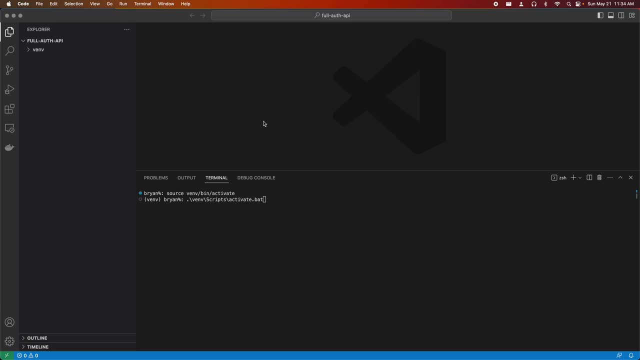 And then you would just go here and then you could connect to your WSL environment And then that way you can use the Ubuntu terminal, which you'd be using bash, instead of using the command line with Windows, And it's just a nicer way to develop when you're on Windows. So the next thing: 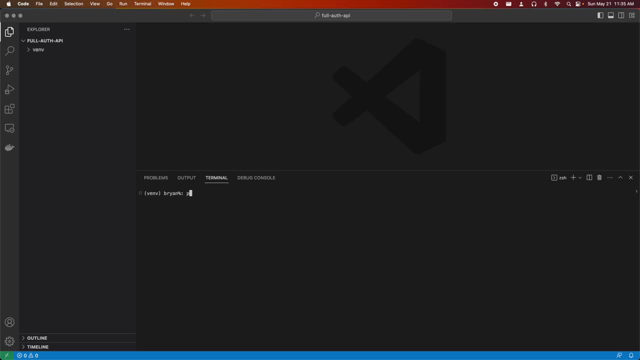 I'm going to do is install some packages I need. So I can do that using pip install And then also right now inside of my virtual environment. by the way, if I do Python dash dash version right now, I don't have to use. 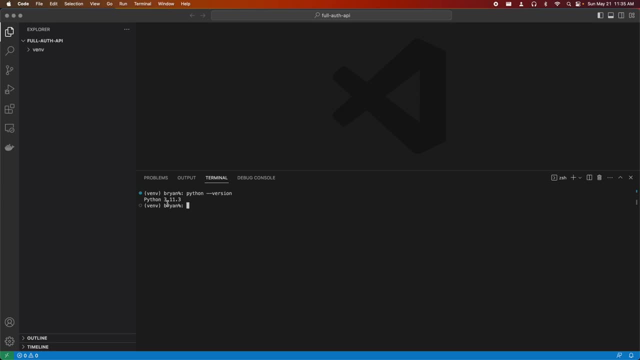 Python three, because the default version of Python in my virtual environment is already this same with pip, So I don't have to do things like pip three install, I can just use pip install. So one thing I'm going to need is Django REST framework, And Django REST framework has a 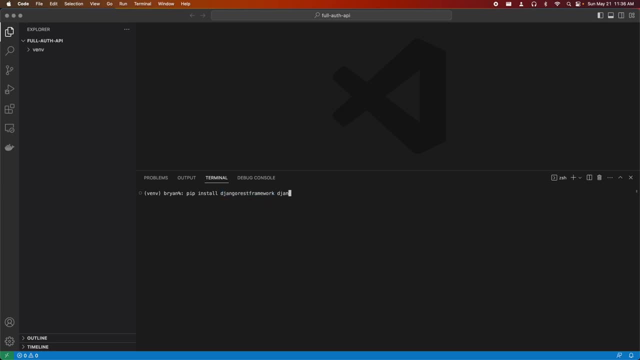 dependency of Django, So I don't have to specify Django here as well. I can just install Django REST framework And that will behind the scenes. So I'm going to go ahead and install Django REST as well. I'm also going to need JOSR. This is gonna be my library for managing authentication in. 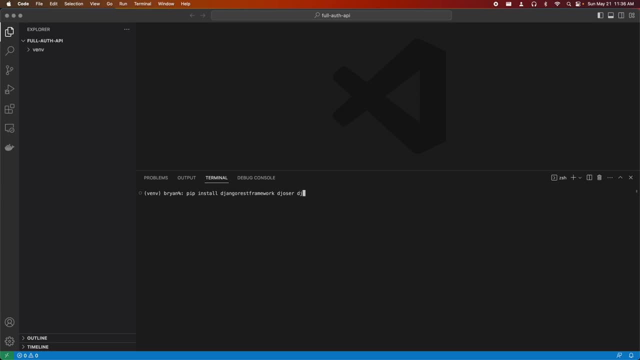 this project. And then another thing I'm going to need is Django course headers. So we're gonna need course headers in this project because our back end- API- and our front end is going to be on separate ports and also separate domains. So in particular when we're in a development 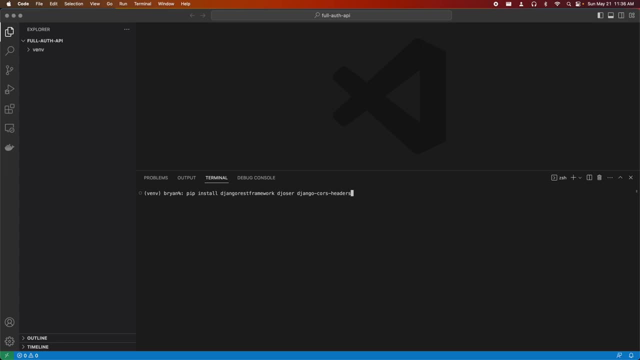 environment. it'll be separate ports, because the back end will be on localhost- 8000.. The front end will be low cost- 3000. and then, because we're going to have authentication and we're going to be using cookies, we're going to need course headers in order to allow cross origin requests to happen. 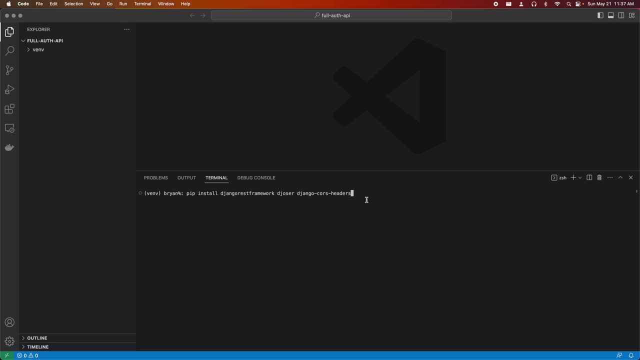 and then in a production environment, we're also going to have different domains, because our backend, api, is going to be on a sub domain. so it's going to be like api, dot, whatever the domain is, dot com, let's say, and then the front end will just be the domaincom. so it'll be different domains. so we're 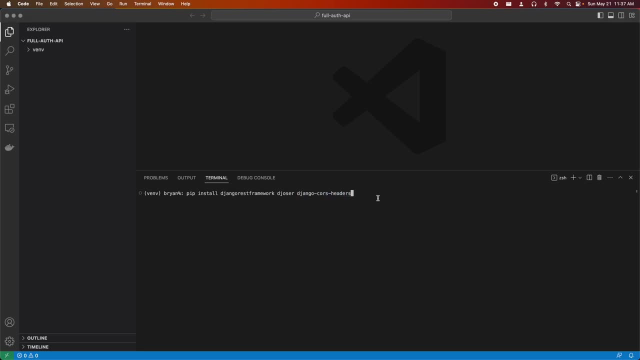 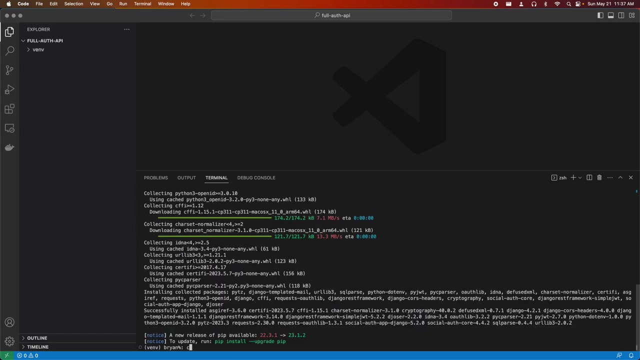 also going to need to set up course headers to allow those cross origin requests. and then the last thing i'm going to install for now is python dot env. this way we can have a dot env file where we can have environment variables. so all of those installed now. so i'm gonna clear. and now, if i do, a 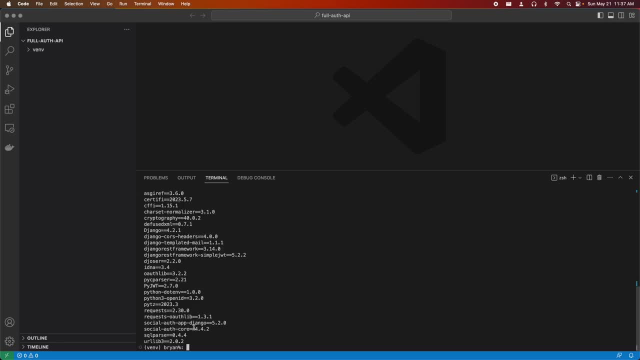 pip freeze. so these are now all the packages that we have, and this is in the virtual environment. so now what i'm going to do is i'm going to create a requirementstxt file which is going to have all of those dependencies. so i'm going to do pip freeze, then this greater than sign. 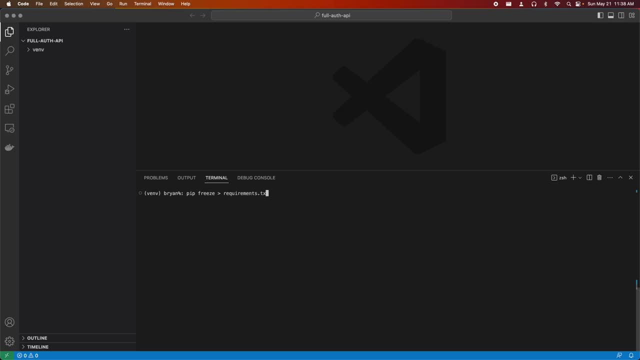 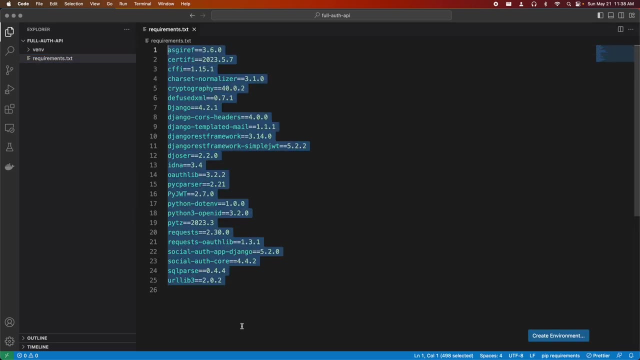 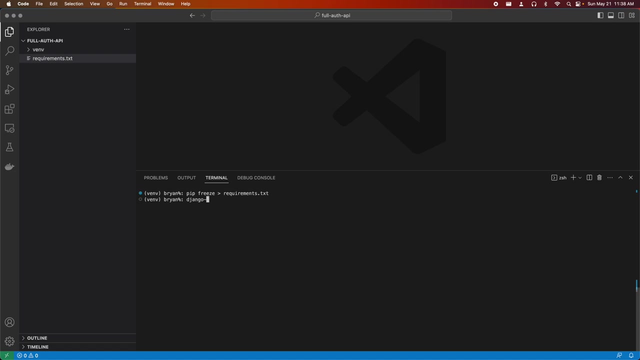 and requirements dot. txt. so now, inside of here, i have all of those dependencies right here. the next thing i'm going to do is generate the django project so i can do that with django dash admin start project project. i'm going to call this full underscore auth and i'm going to put a dot so that it gets. 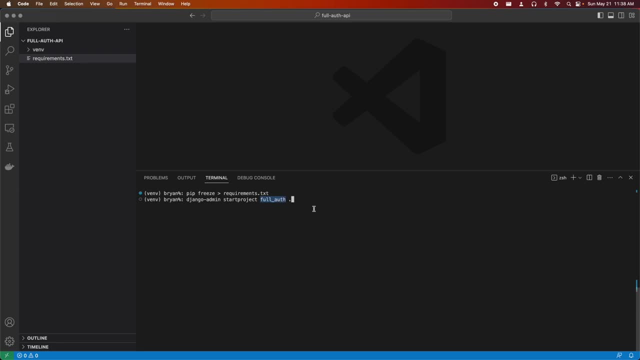 made in the current directory and then i don't have full auth and then another full auth folder. so i'll show you what i mean. so if i don't put that dot inside of here, i'd have another full auth folder and that would have all of this inside of there. so i didn't want that. so that's why we. 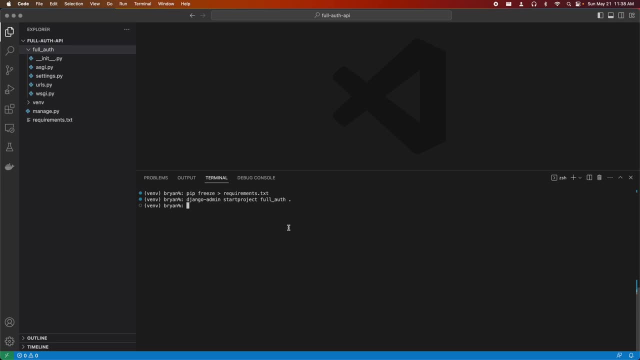 put this, for the current directory is where i want to have this project present. so the next thing i'm going to do is i'm going to create the app. so i'm going to have only one app and that's going to be a users app, which is going to be for managing users and authentication. so 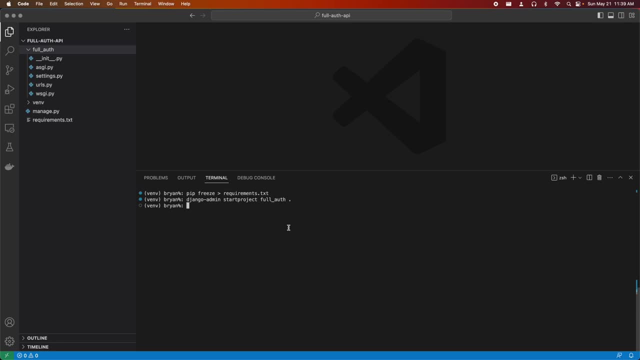 anything custom i need with authentication, which i will need in this project, so i can do that with python, managepi start app and i'm going to call it users. so here we used django admin, but once we created the project we got this managepi, so now instead we can run these. 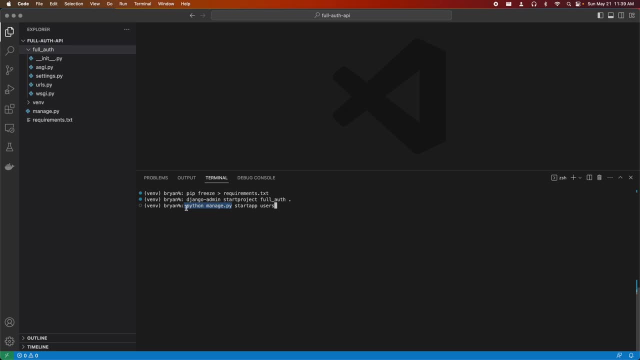 commands like start project and start app by using this. instead it'll be python managepi command and whatever options it has. so there we are. now we have our users app, and then the other thing i'm going to make is my dot env. so i'm going to do a dot env, dot local, and this is where i'm going to set up my environment. 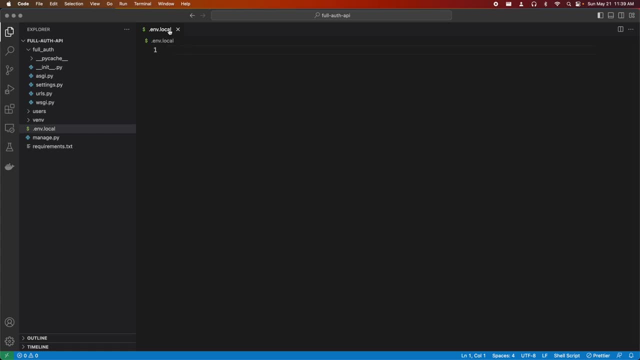 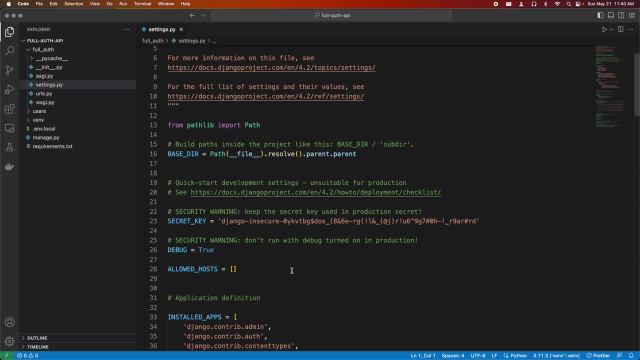 variables for my development environment. so i'm going to close this for now. i'm going to come back to this later. for now, i'm going to go to my settings, because this is where i'm going to start configuring some things. now, if i want to configure something, i'm going to do that by 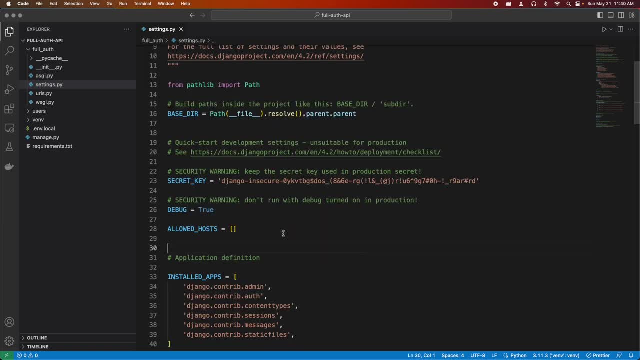 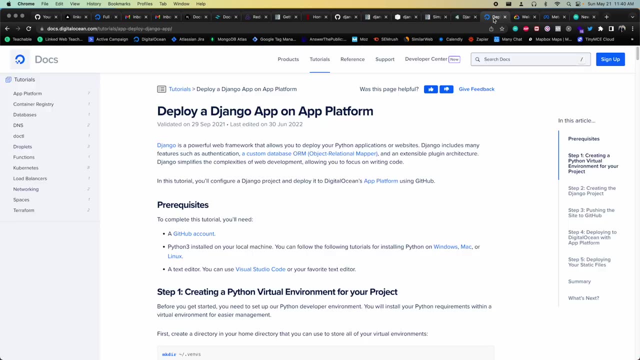 default. so i'm going to do that by default. so i'm going to do that by default. so in this particular project, we're going to end up deploying things to digital ocean, so i'm going to do that a little bit later. but one thing that i'm going to be using to kind of help out with that whole process is 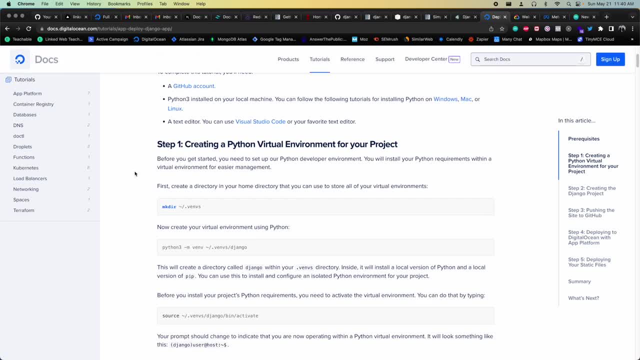 there's this link to deploying a django app on app platform with digital ocean, then a lot of these steps in here are going to be very similar to what we do in this project. i'm also going to have a link to this in the description below. so shows you creating your virtual environment. 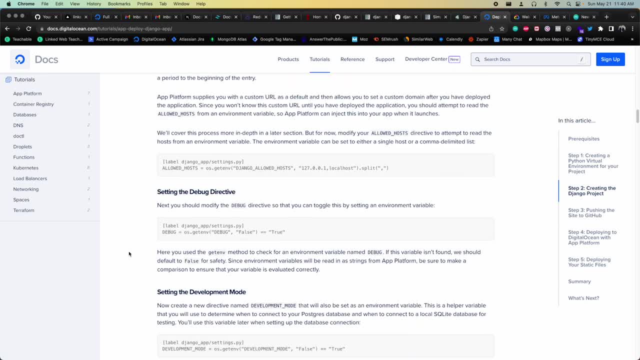 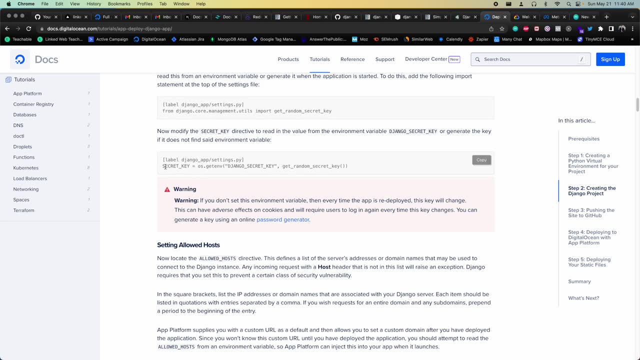 project. so we're kind of going through those steps and then later on there's some project setup things. they kind of start right here actually. so let's say, for setting your secret key you can use an environment variable of django secret key and then you can also use this utility. 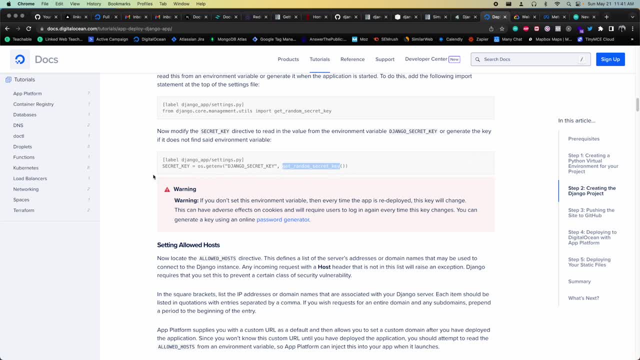 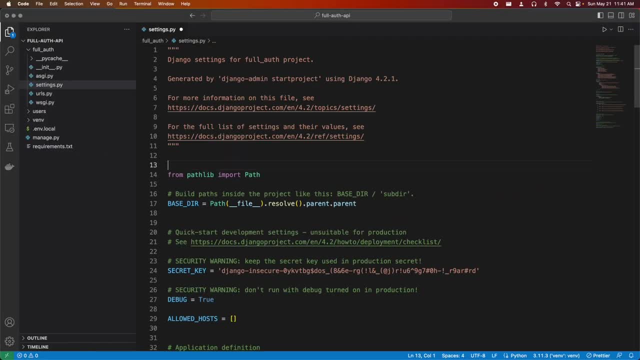 function to generate a random key. so we're going to be doing things similar to this. so i'm going to show that setup right now. so inside of here at the top, i'm going to do from os, i'm going to import, get env. so this is what we're going to use to get our environment variables. 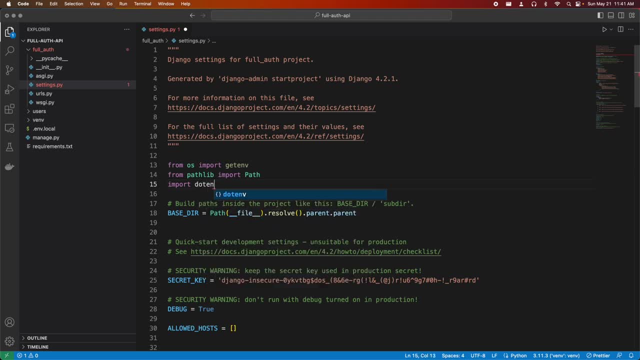 another thing i'm going to need is to import dot env. so that was that pythonenv package that gives me support for the dot env file right here and getting the environment variables from there, because by default i can't get those environment variables from this kind of file. instead, they 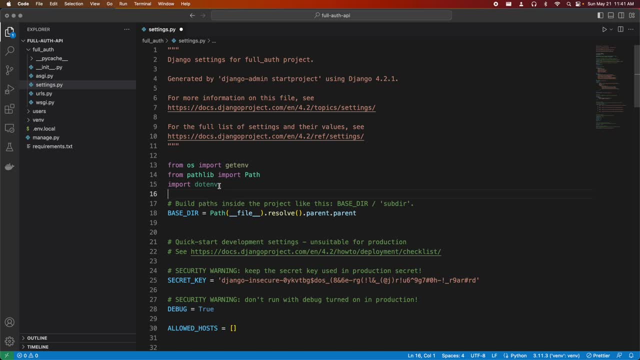 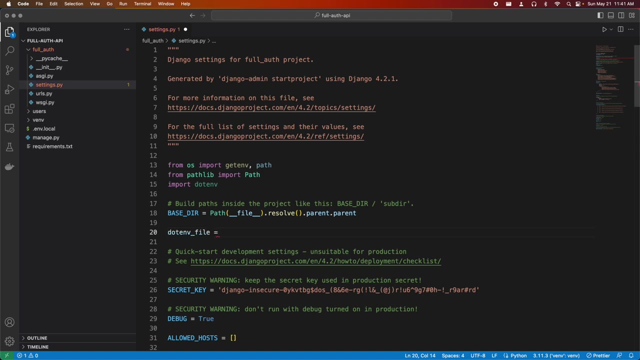 would have to be environment variables set up on my system itself. so this just makes development a little bit easier. and then below here, another import i'm actually going to need is going to come from os as well. it's called path. then what i'm going to do is set dot env file. this is going to be base directory. 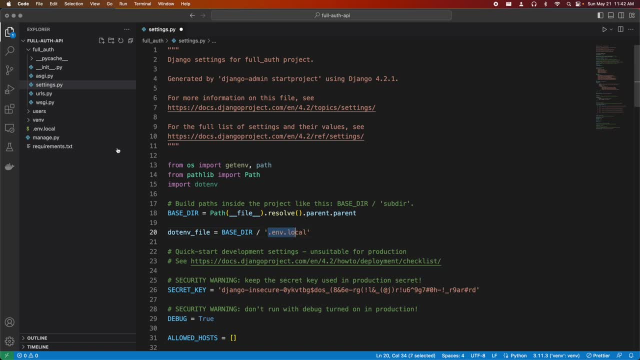 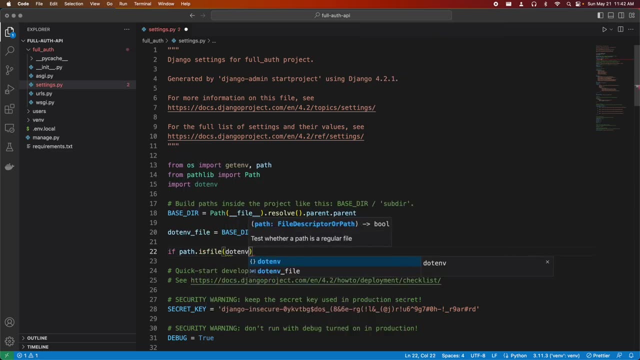 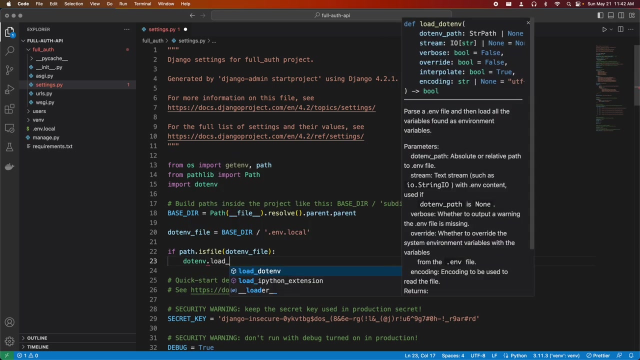 and then dot env, dot. local. so this is going to be this file i made here. then i'm going to check if path dot is file, dot env file. so if this is a file, then i'm going to do dot env, dot. load dot env- the dot env file. so i'm going to load the environment variables from this. 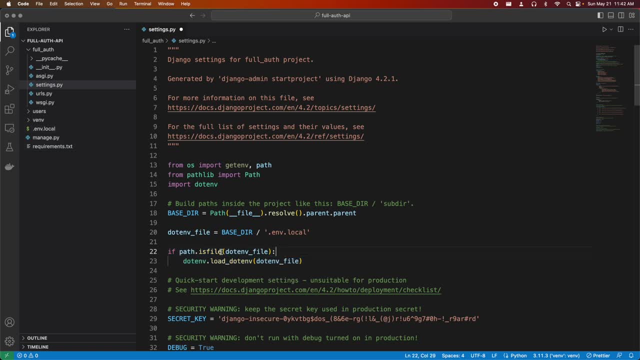 if this exists, so in our production environment this is not going to exist. so we're not going to be doing this loading of the dot env file. instead we're going to have more like global environment variables on there. but in our development environment this just makes things a lot more convenient. so i have to go into my terminal and set up global environment. 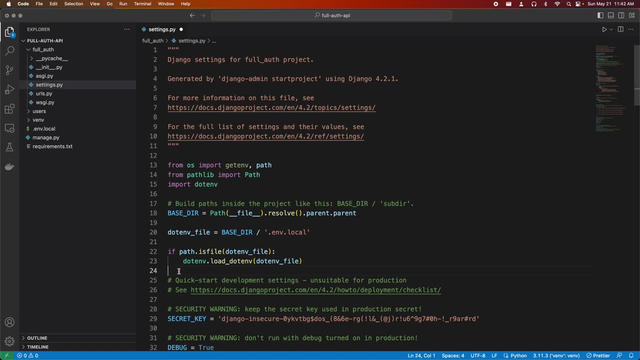 variables and it also complicates things if you're on a windows system and you want to set up these environment variables. so this is a much better development experience, so i'm going to save that also. when i save here, i get this little suggestion: you have the auto pep 8 formatter extension. 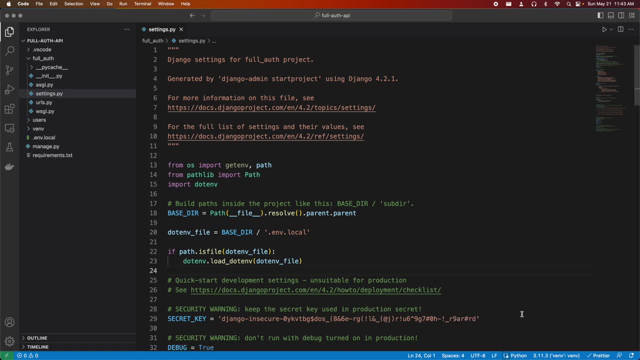 installed. would you like to use it as a default formatter? yes, i would, because my default formatter right now is prettier, but i'd rather use auto pep 8.. so then it'll just create this dot vs code folder, and then there there's this settings json, where it just sets this up. 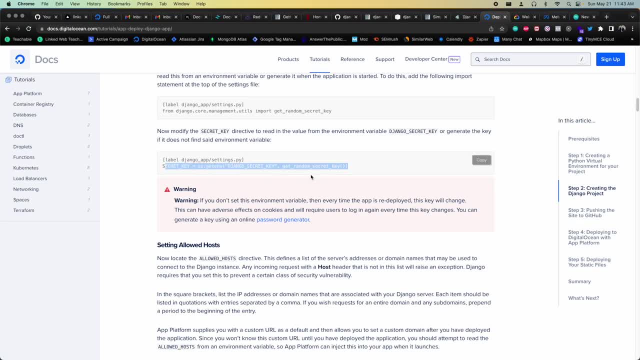 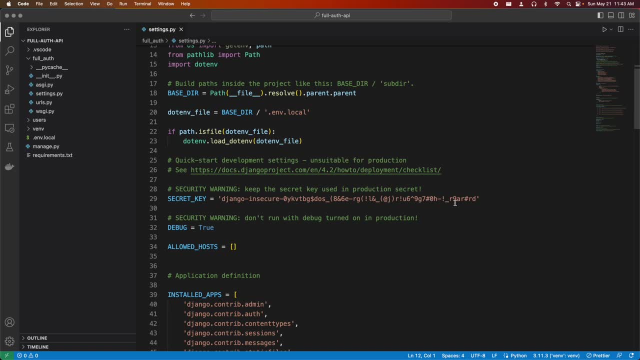 and then i'm going to go back. so right here i have this whole secret key set up, so i'm just going to copy this and then i'll go paste right over here. so right now i don't have to do os dot, get env, since i just imported this directly. so my secret 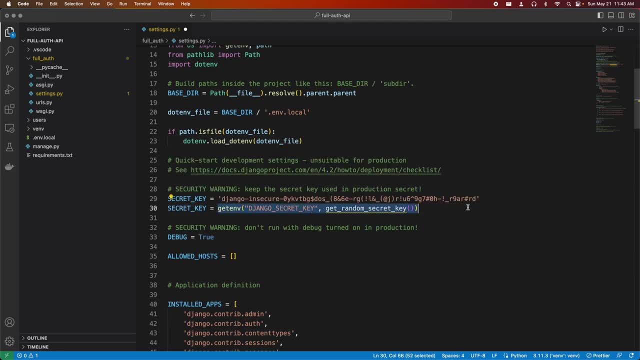 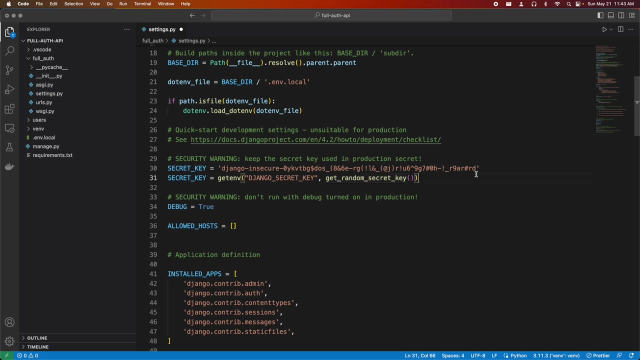 key that's going to be equal to this, and then i need this import as well. so that's right here. so this will just generate a random secret key, and then i can just cut this. so this is how i'm going to set the secret key up now, and then also i'd rather use 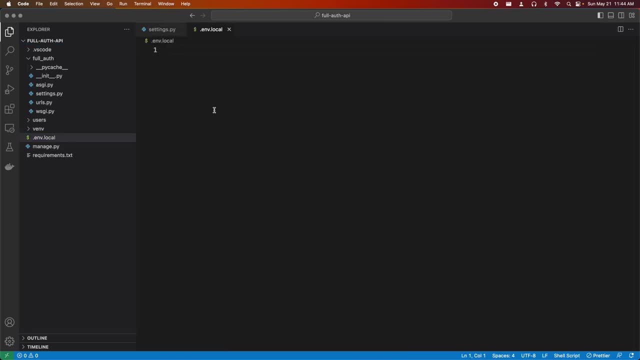 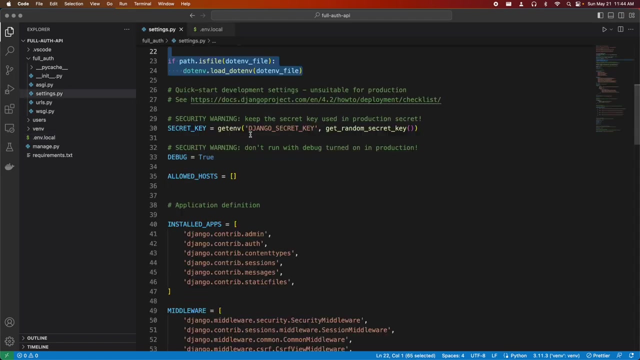 single quotes. so i'll do that, and then inside of here i can do django. secret key is equal to this, And actually I'll put an extra quote here. So there we go. So now we have this environment variable that's going to get loaded up by this, And then we'll be using it here. And if you don't, 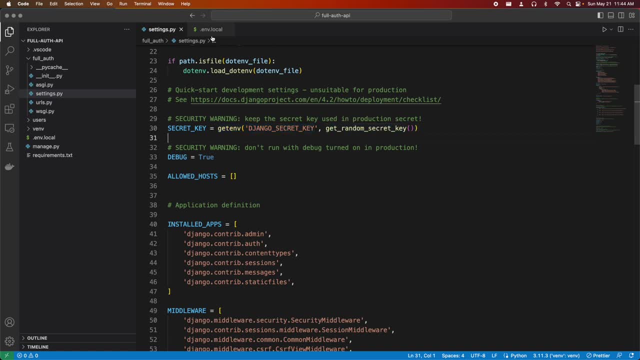 have this set, then you're just going to generate a random one, But I'd rather just have one set up in here, So that way, every time my server kind of reboots, I don't want to generate a brand new key. 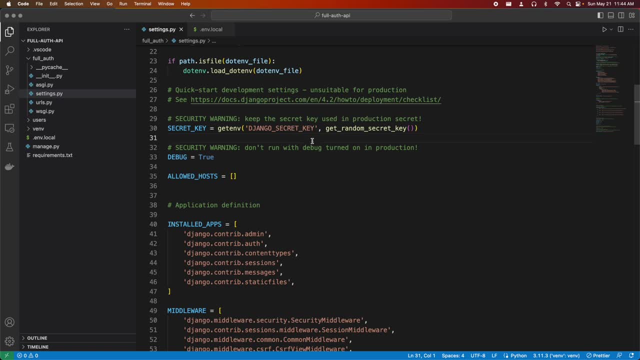 especially because we're going to be using JSON web token authentication And then we're going to have, like the cryptography it's going to be using this secret key so that every time it changes then your access tokens aren't going to work. So I'd rather just have one. that's kind of. 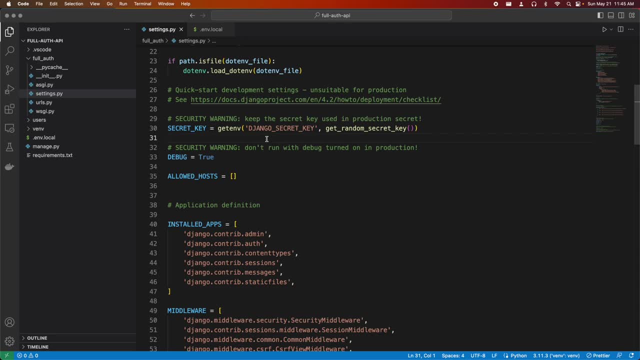 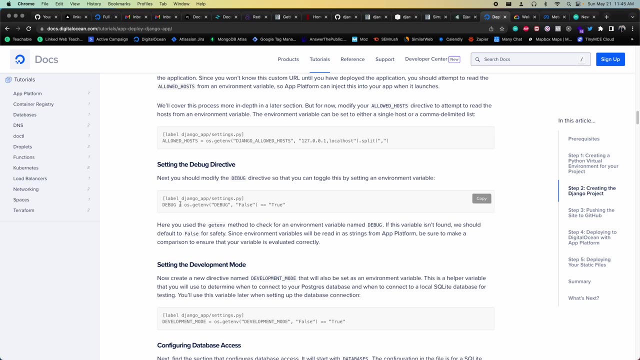 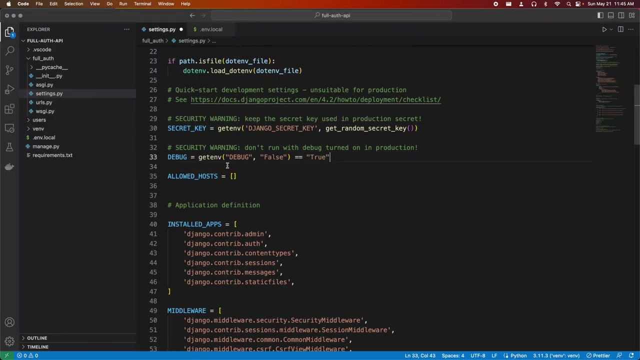 in place. So every time my server restarts I hold that value. Then the next thing I'm going to do is tackle this setting. So here we have: debug is equal to this right here. So we're going to get an environment variable of debug. 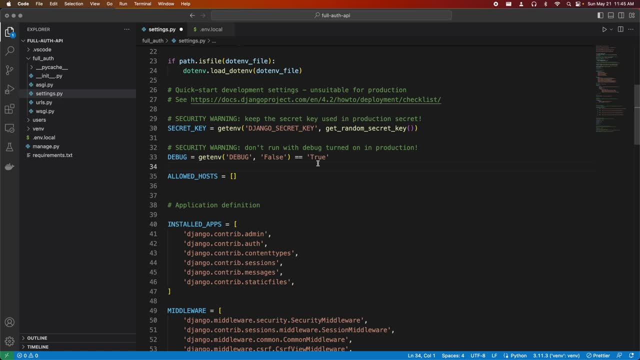 And by default it's going to be false. And then environment variables are always strings, So you have to do it like this. you can't just grab it and use like a value of true, otherwise going to be like the string true or the string false. So you have to do this kind of comparison. 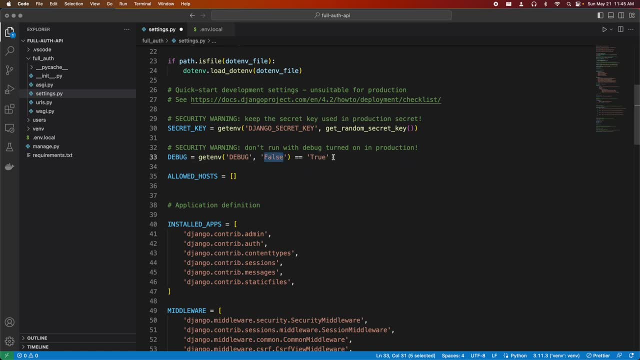 And then by default we're going to have this be. false equals true, which is going to evaluate to a Boolean of false. So that way in our production environment we don't have to set this thing, it'll just be false. And then in our development environment we will have to set it. So here: 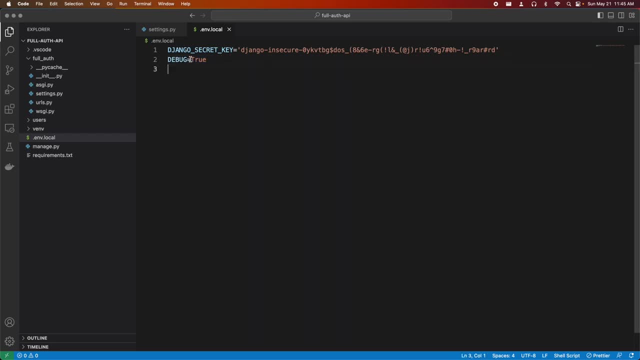 I'll do. debug is true, And again, this will be the string true. And now, if I put quotes around it or if I don't, it's the exact same thing. So you can use whatever syntax you want inside of here. 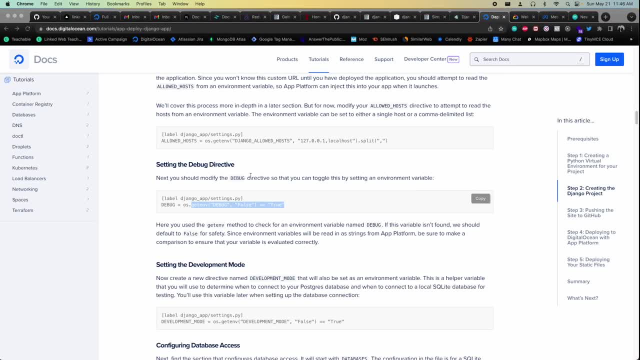 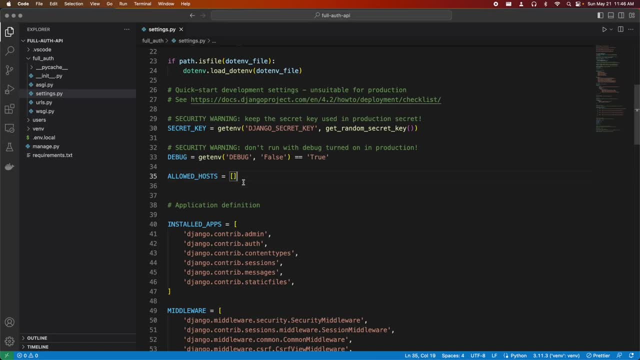 And then the next thing I'm going to do is tackle the allowed hosts. That's right here, And then I'll paste that right here. So we're going to get an environment variable of Django allowed hosts, which by default, is going to be our local host environment. we do this dot split. we're just going to split this into an. 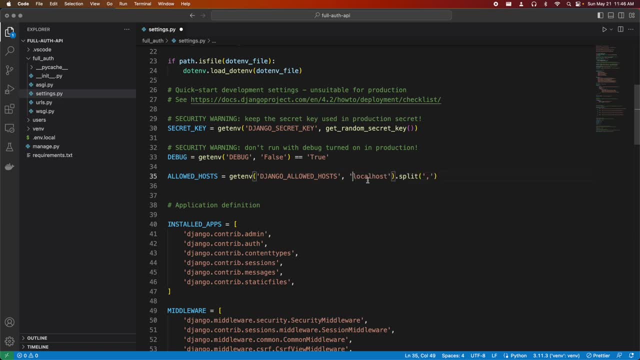 array. And also, by the way, if you, let's say, had only one item here and you did a dot split, it would be an array with just one item. So that would work. you don't need to have the comma there. 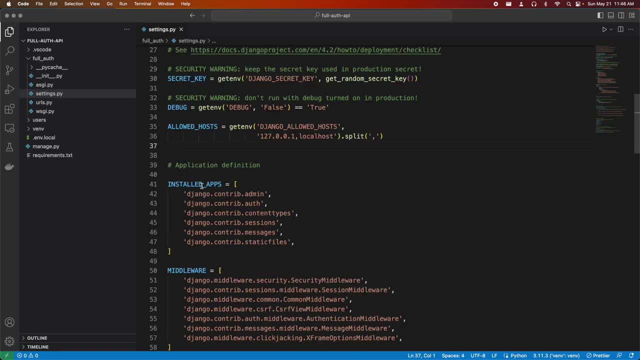 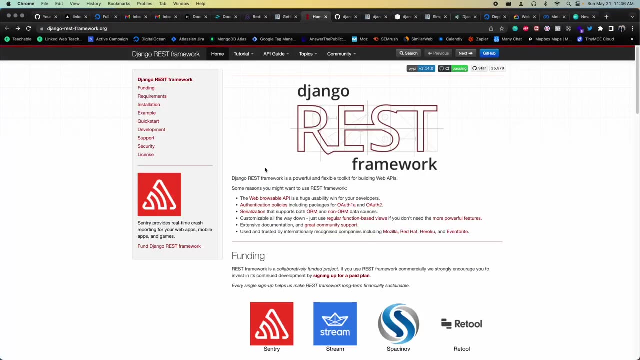 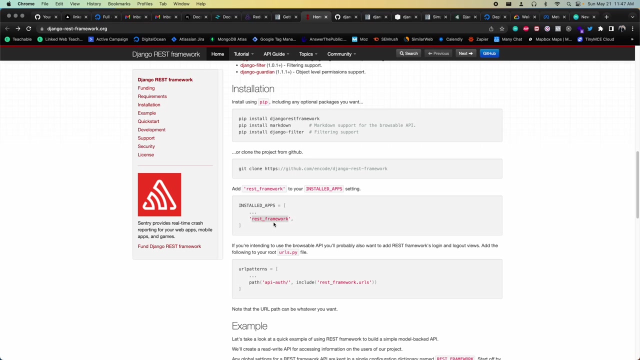 So I saved in that formatted things. I'm going to tackle my installed apps. So we have Django rest framework in this project. So after documentation open here, that'll be the first thing I set up. So we need to install it, which we did. you have to put it in your installed apps And also, if you want to use the browsable. 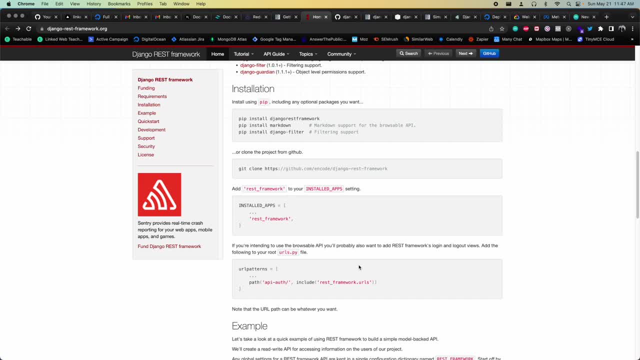 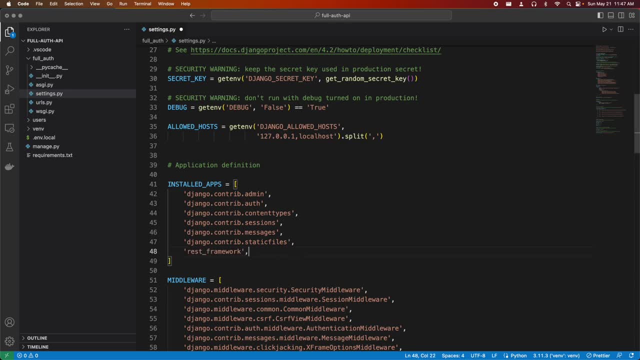 API. you can also set up this here, but I won't be using the browsable API. Instead, to test out my API, I'll be using postman, So let's put this in here. So we got rest framework. Next, we got to. 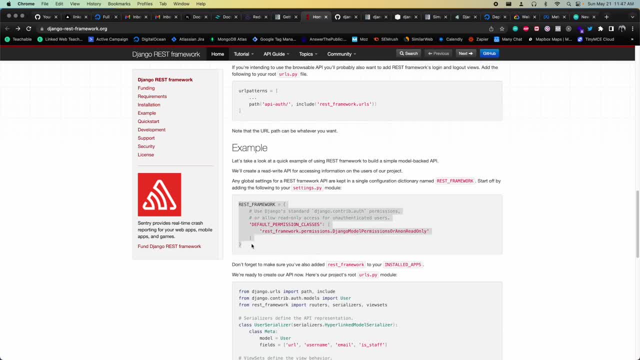 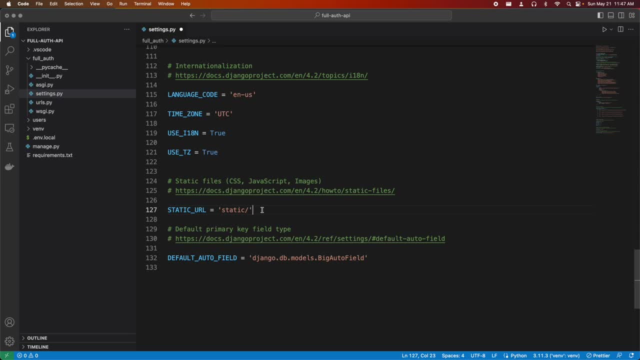 set up the settings. I'm just going to copy this example here And I'll scroll down And I can put that, say, below the static settings or remove these comments And then for my default permission classes, instead of having this here I'm going to have is authenticated. 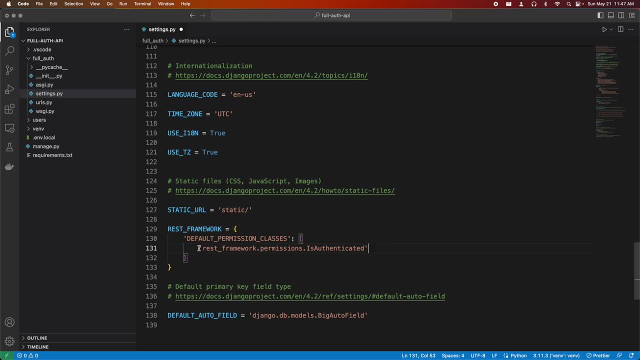 So what this is going to do is, on all of my views, by default we have to be authenticated And then, if we're not, we're going to get a 401 unauthorized. So if we want to overwrite this, then we can set a different permission. 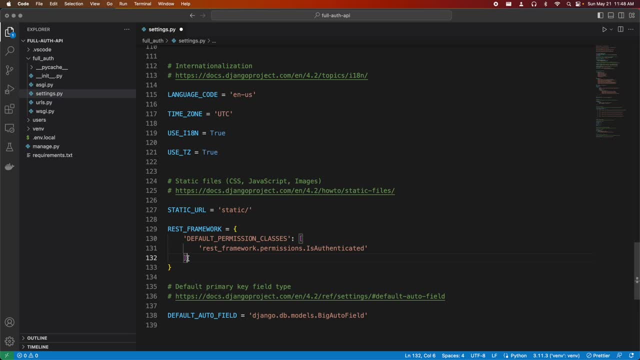 For example, we can have permissions of allow any and we have to specifically define it on the view, But I want by default, the behavior to be is authenticated. So that's going to be for the permission classes. we're also going to have authentication classes. In particular, we're 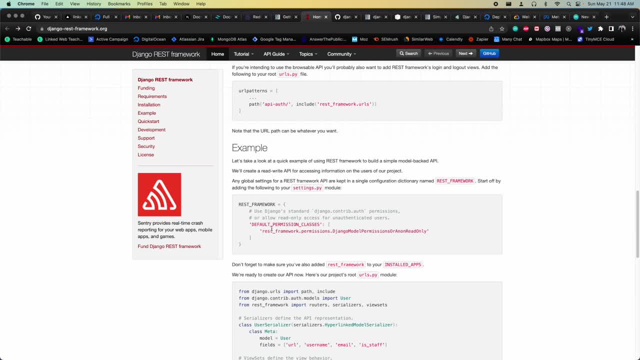 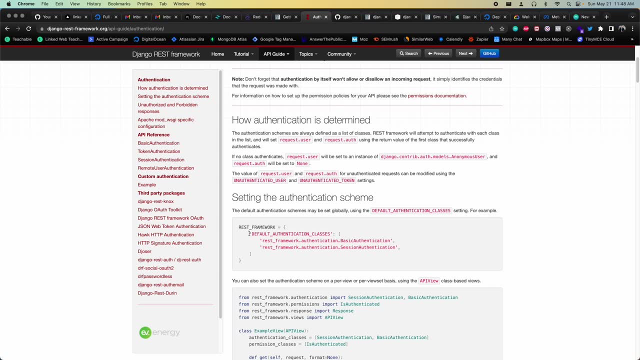 going to be using JSON Web Token authentication. Well, we can also go inside of Django rest framework, inside of authentication, And then here you can see the setting that we need to set for authentication classes. So that's this one here And that has some examples. 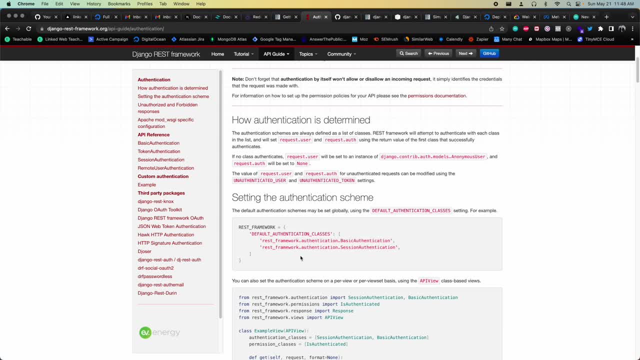 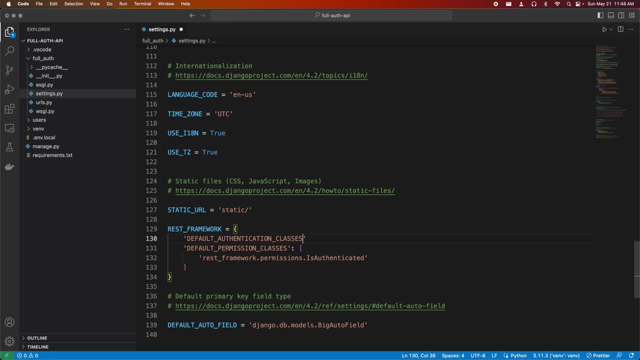 of, let's say, basic authentication, session authentication, But ours, of course, is going to be the JWT authentication. I'm going to set up that setting here And then that's going to be a list And then this is where we're going to set that. So right now we have the Joeser library. 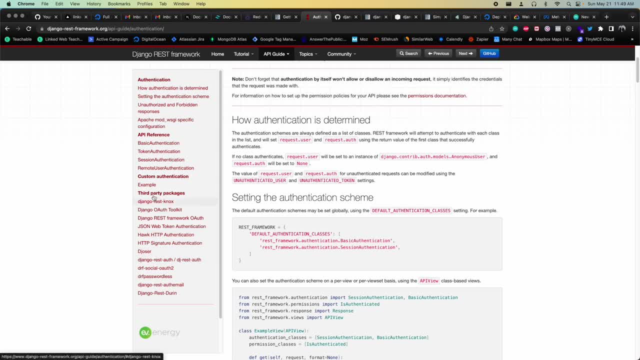 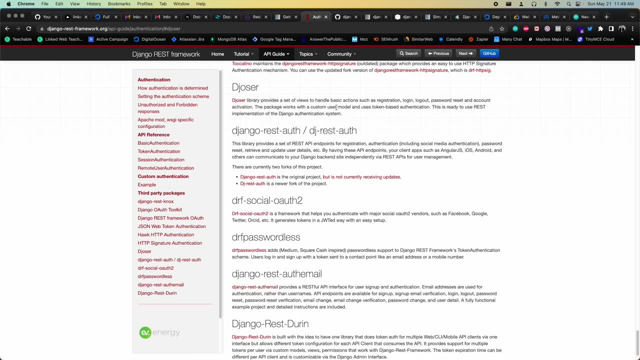 that we're using And that's also one of the suggested libraries in here. So third party is Joeser, And then here you can see that it's a library that provides views for handling basic actions like registration, login, logout, password reset, account activation. So all. 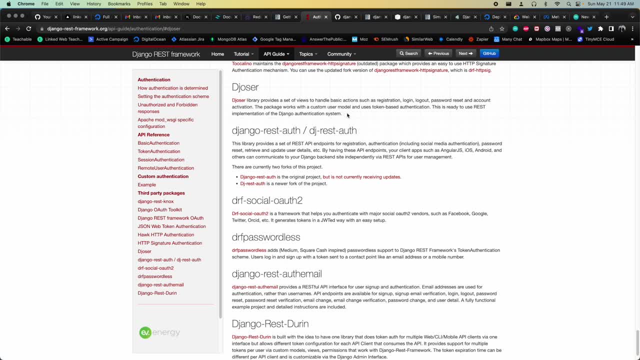 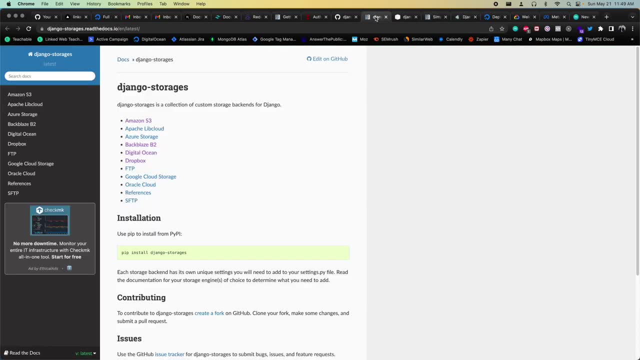 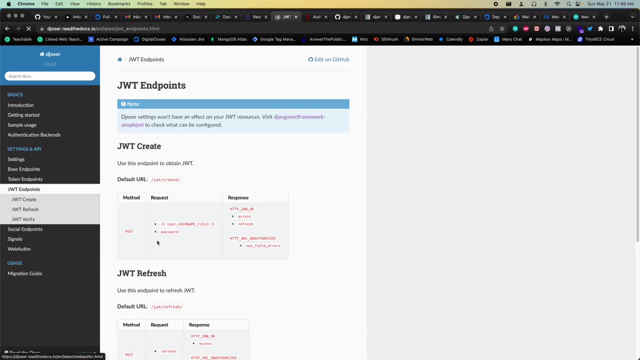 of that we get with this And then behind the scenes when we're doing the JWT authentication. so I have the documentation open for it. It's one of these- Let's see which one, This one. So here, if we also have this JWT endpoints and then we also have the JWT endpoints And 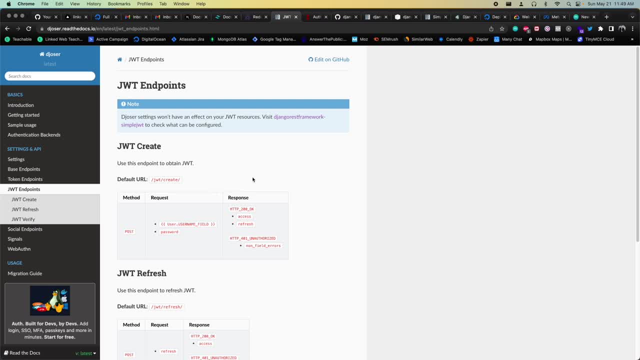 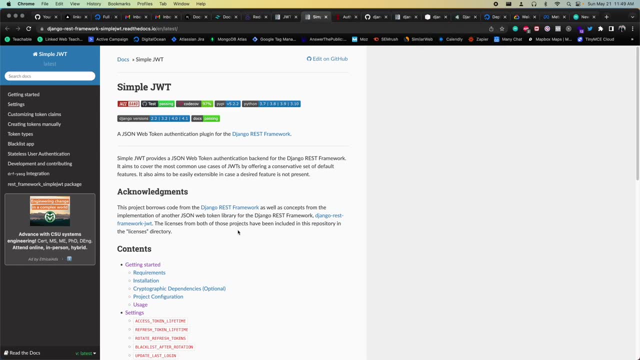 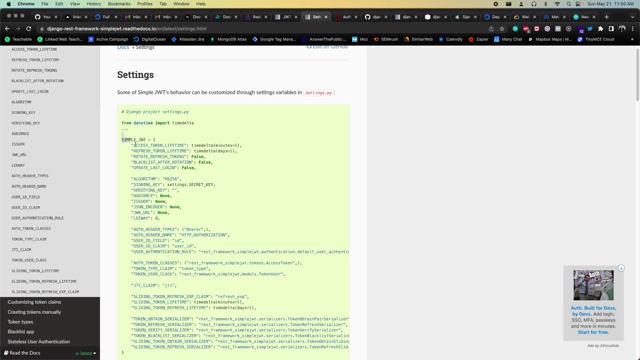 then these JWT endpoints, they're going to be using the simple JWT package, So then I also have the simple JWT documentation And then here we can take a look at some of the settings it has. you can go to the settings and then you can see the default settings, And then there's also how. 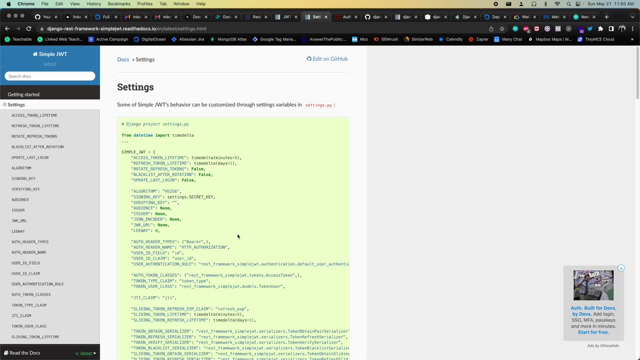 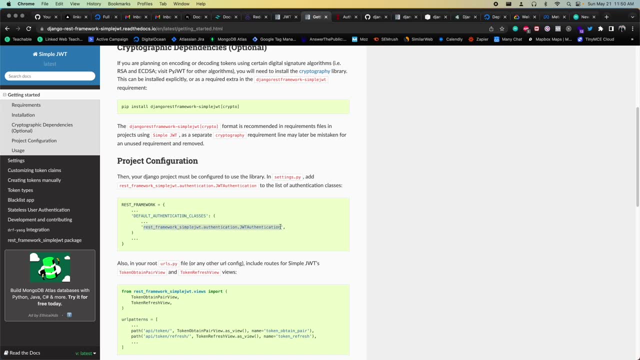 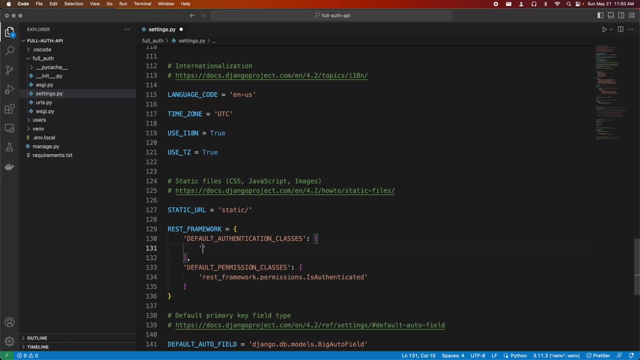 you can set this to be your default authentication class. So I think it shows it somewhere here. So if you want to use the JWT authentication classes, you will put this right here And that will use the JWT authentication then. So that is what I'm going to paste right here. 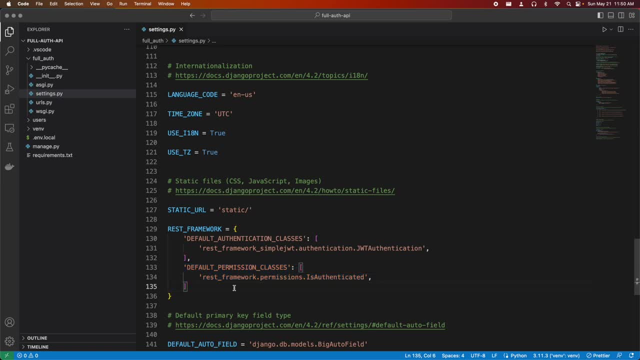 So now I have my authentication classes and my permission classes set up And then also just to show with Joeser that it's using the simple JWT package behind the scenes. you can also go in your virtual environment. you can look for Joeser And then here you have URLs. 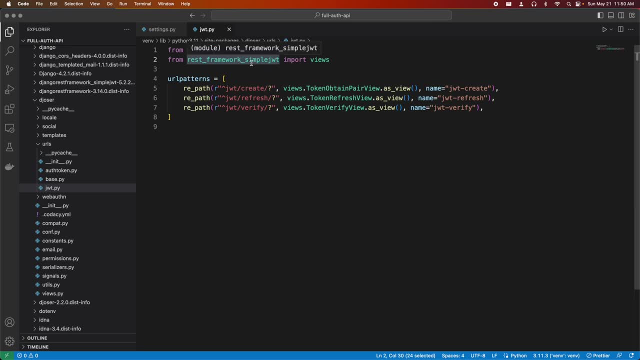 JWT And you can see it's using the simple JWT package And it's just setting up these endpoints and, behind the scenes, just using the views from there. So we have things like the token- obtain, pair view, refresh view, verify view and the endpoints for that. 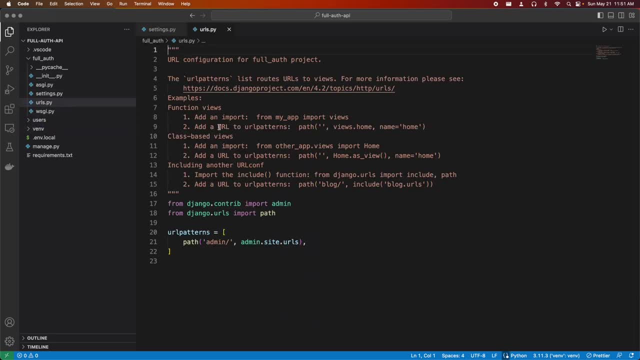 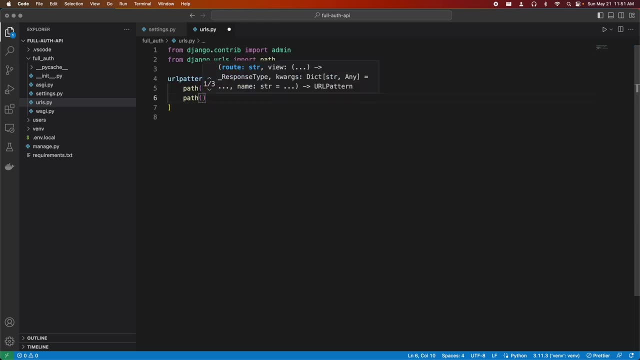 All right, so now with that, we can go into our URLspy. just going to remove the documentation comment. there I'm going to have a path which is going to be API slash, And there I need to bring in include, And then I'm going to include joeserurls. 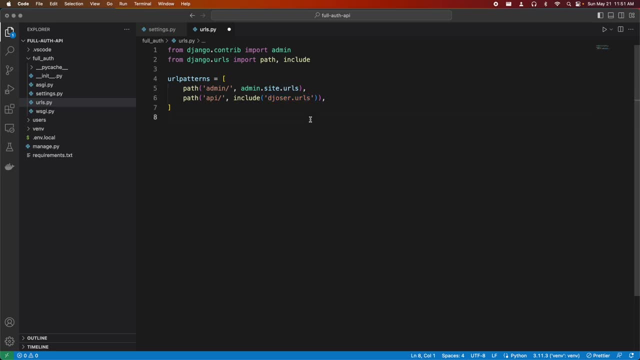 So joeserurls. this isn't going to give me the JWT URLs, it's only going to give me the other ones. If I want the JWT URLs, I have to do API slash and then include joeserurlsjwt. Then I think it shows that. 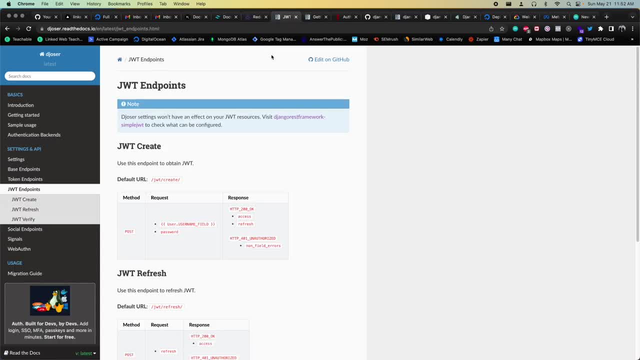 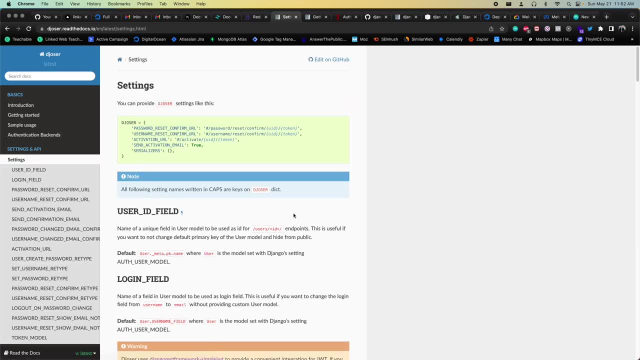 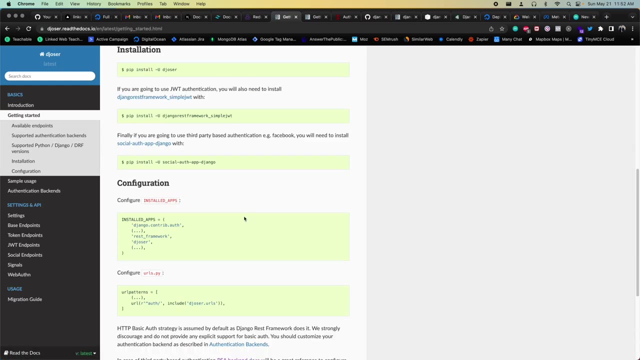 in the documentation for joeser. that's this one here, And then if we go to settings or not settings, that's going to be all of our settings. I'm not sure exactly where it is in the documentation. might be in the getting started, But anyway. 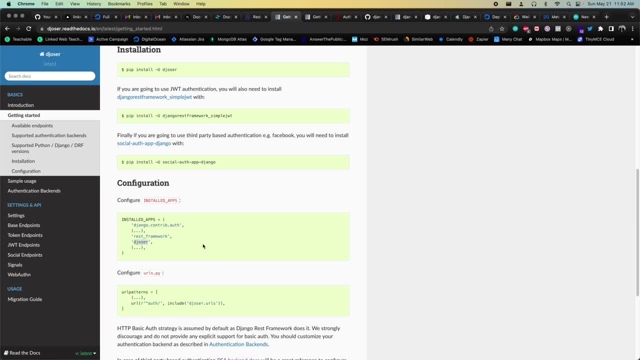 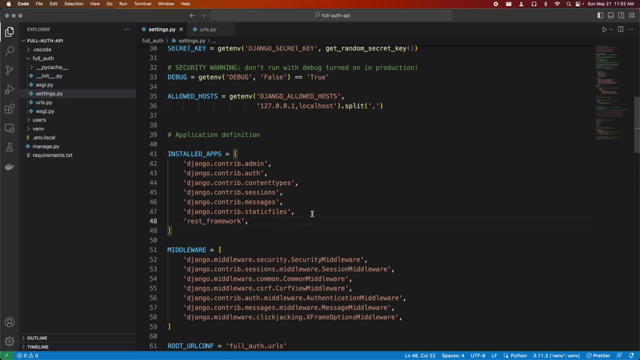 we will need this. So here we have joeser that we have to put in our installed apps. Let's just go ahead and do that. So, back in my settings, I'm going to scroll up And I'm going to put joeser right over here. 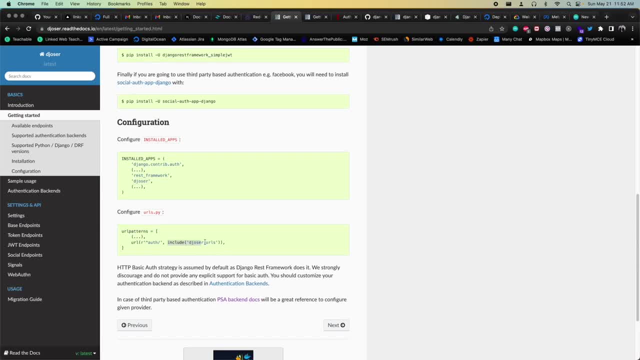 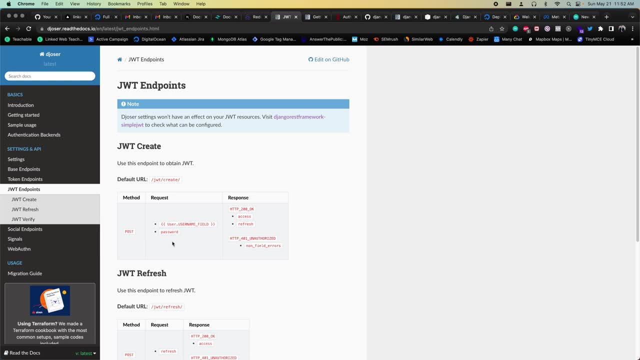 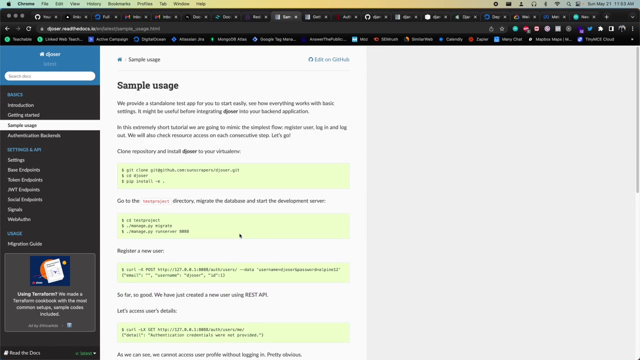 And then it shows you how to set up the URLs. So you just include joeserurls And then for JWT. I'm not sure exactly where it shows it. I would expect it to be in the JWT endpoints, or maybe somewhere else. Perhaps sample usage? No, it's not sample usage, But anyway. 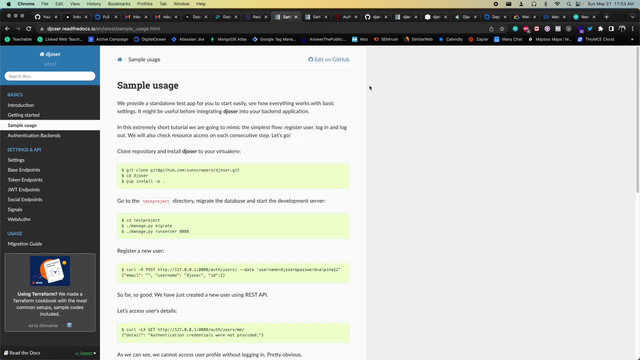 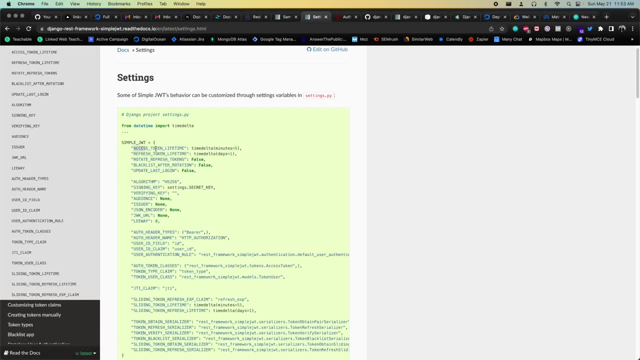 that's how you would set up the JWT endpoints. Now, once we have the simple JWT package set, we will go ahead and do the setup. And then it says: this is what we want to do And we're going to go ahead and do our setup. So here we have the default values, So we have, let's say, the 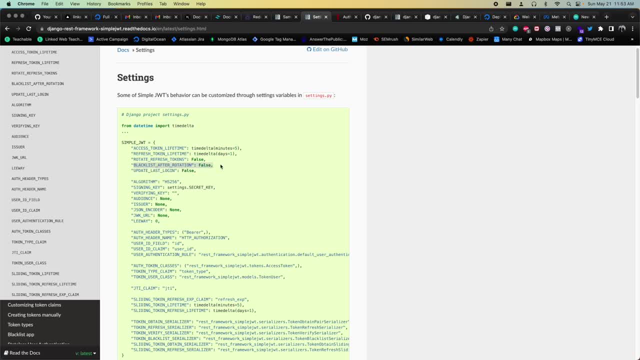 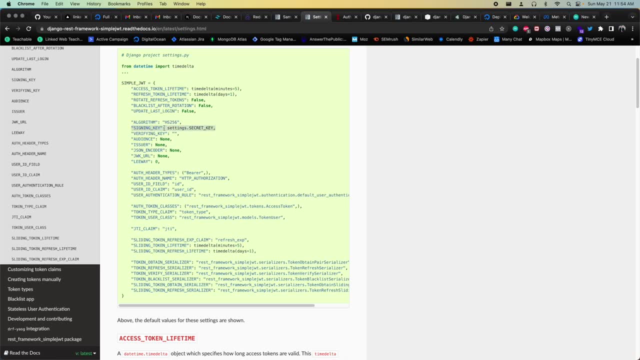 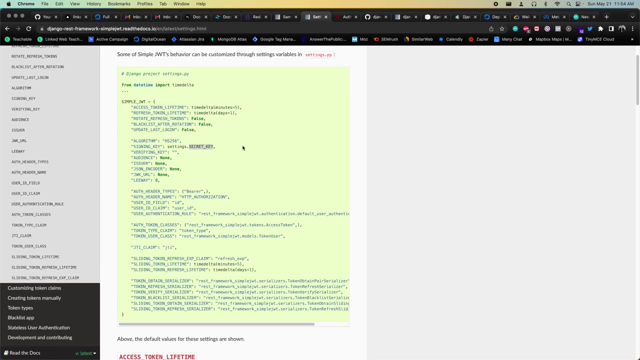 access token lifetime five minutes. refresh token lifetime one day, then rotate refresh tokens falls, blacklist after rotation falls, and so on, so forth. And then also, one thing that's in here is our signing key. So the signing key, that's the thing that uses our secret key. So this is the 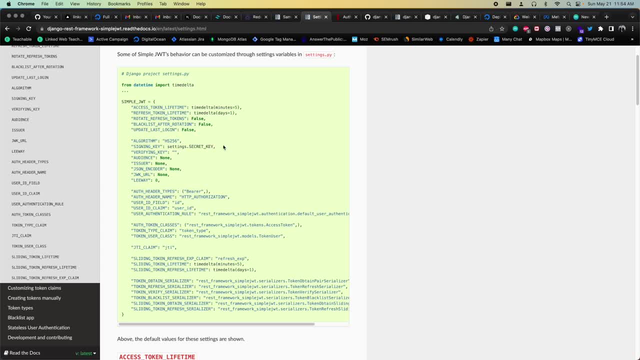 reason why I wanted to have in the environment variable the secret key, because every time it changes the signing key will be different, different, and then your jwt authentication won't work. you're gonna have to re-sign in, and then re-signing in when you're using json web tokens is just creating a new access token. 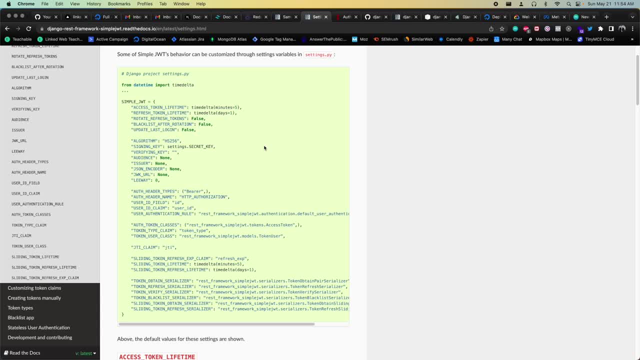 and that's because you use your access token for authorization. so if you wanted to overwrite any of the settings in here, you would just put a simple jwt setting, which will be your dictionary. you can overwrite any of these settings, but i will be sticking to the defaults. 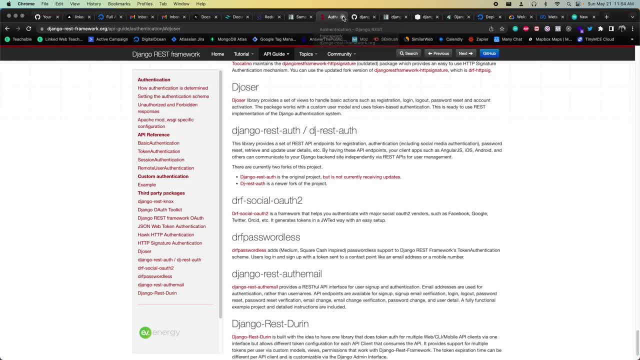 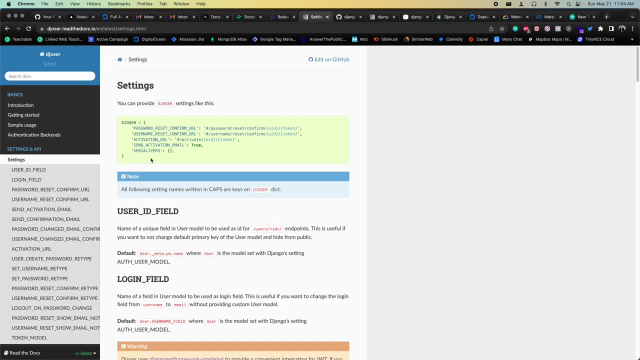 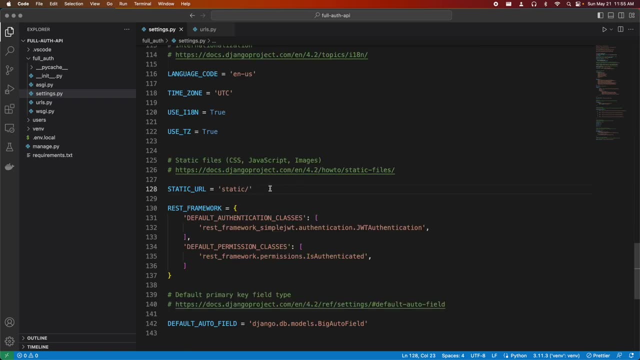 that you don't actually need or want to save to if you useрas. so i don't need this open anymore. i also don't need this open anymore. and then one thing i will need is the settings in joser, because we're going to be setting these up. so i'm going back to the code, i'm going to scroll down. 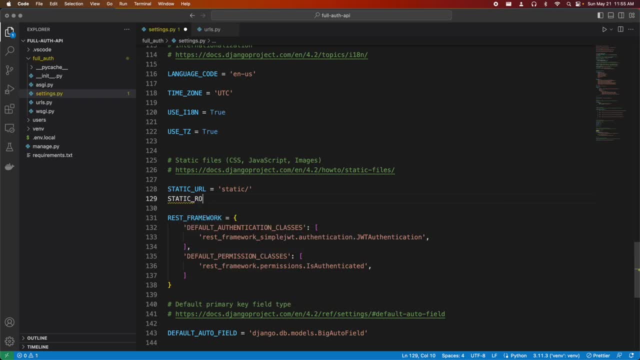 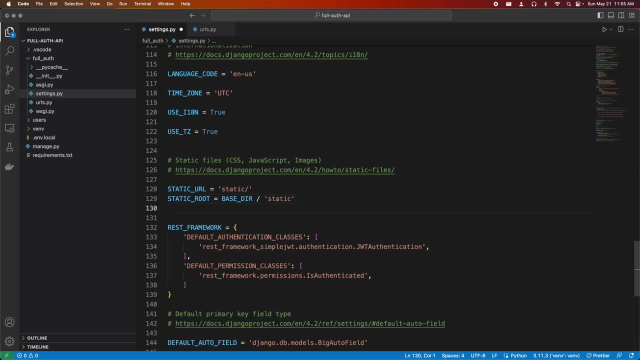 to the bottom here. and also, while i'm at it, i might as well set this up: i'm gonna have my static roots, which will be base directory static routes. So for the media, this is going to be where you have things like photos and videos and 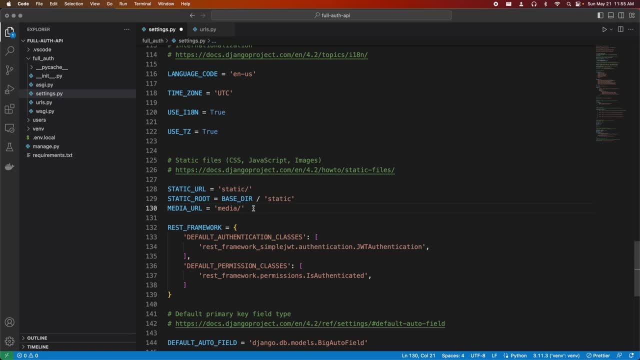 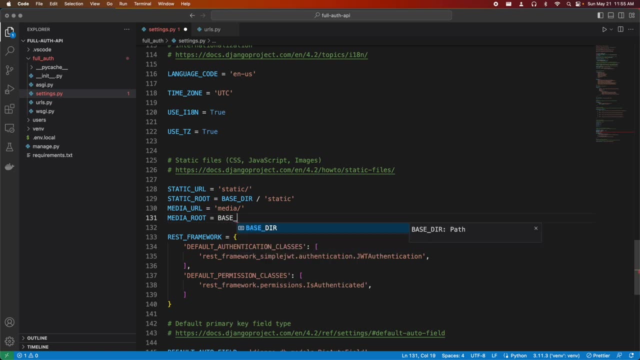 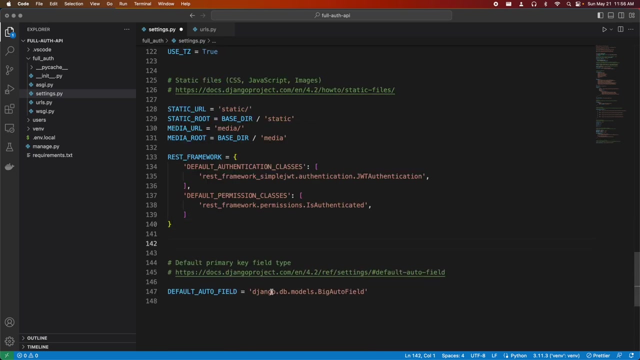 whatnot. Now, I'm not going to be using that in this project, but it is very common to have it in a project, So I'm just going to include it here And then, for media routes, it'll be base directory, media, And then, below my REST framework settings, this is where I'm going to have my 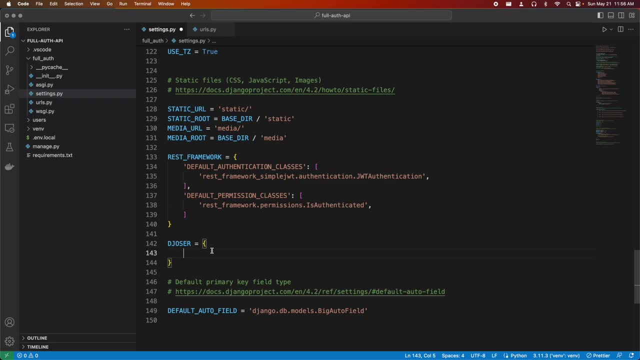 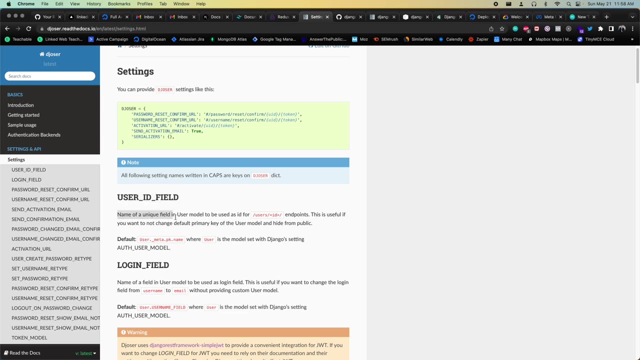 Joeser settings. This will be my dictionary And let's see what we need to set up. So the first setting we see here is the user ID field. So this will be the name of unique field in the user model. This is something we can just stick to, the default. We have the login field. 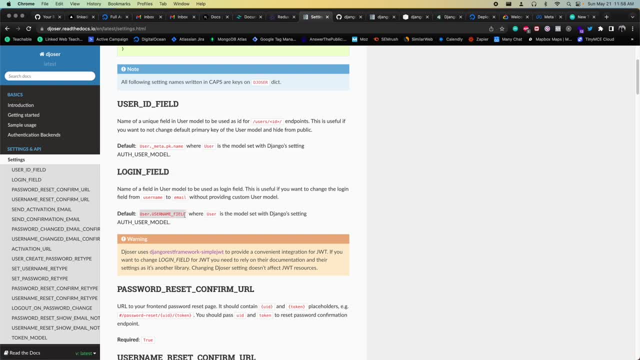 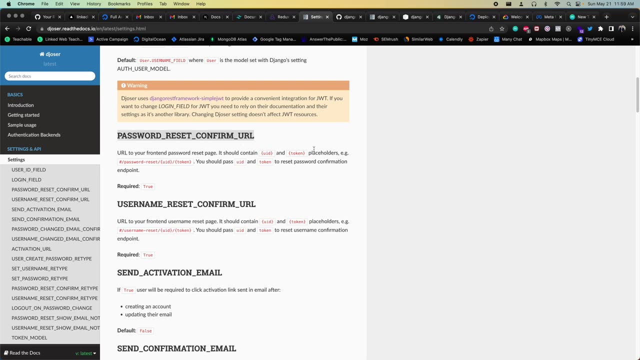 So login field, this is going to be set to userusername field. But this is something that will be overwritten once we create our custom user model, So we can just stick to the default on this. Then we have our password reset, confirm URL. So this is going to be a setting I'm going to set up. 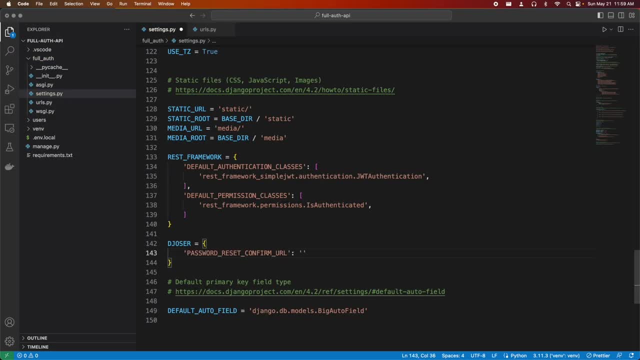 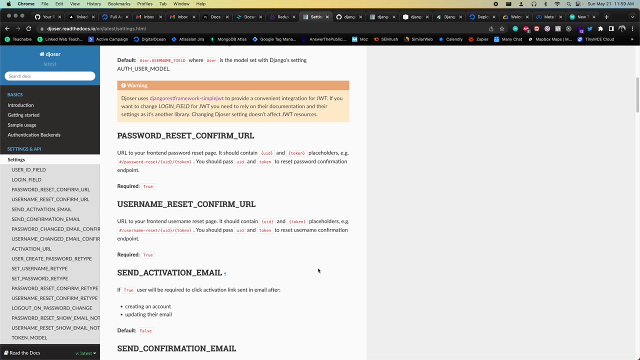 So back in here I'm going to paste this, I'm going to set this to password, dash reset, and then UID and token, And then we also have username reset, confirm URL. So this is going to be when you're resetting a username, which in our case would be an email. Now, I'm not going to include this one, just because 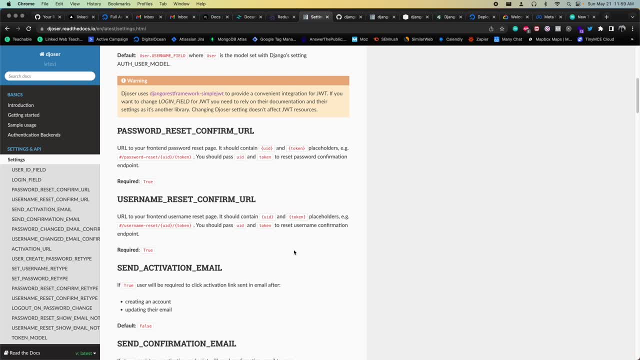 we're not going to be doing a username reset, which, in our case, is an email reset. Now, you can include this if you want, And it's very similar to how it works with the password reset. So once you know how to do this one, you'll know how to do this one as well, But I'll just skip that one. 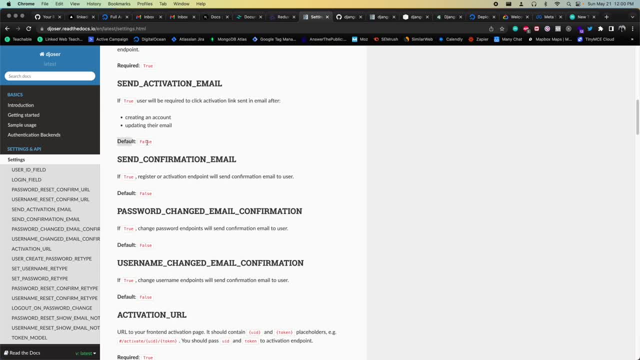 And then we have send activation email. So this, by default, is false, but I will want this to be true, just because when someone creates an account, I'm going to want them to get an activation email, where then they're going to have to click a link and activate their account. 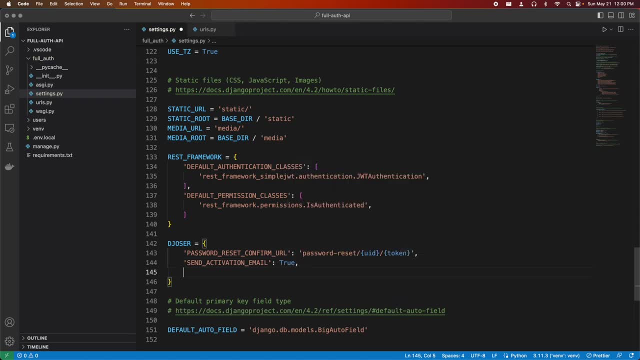 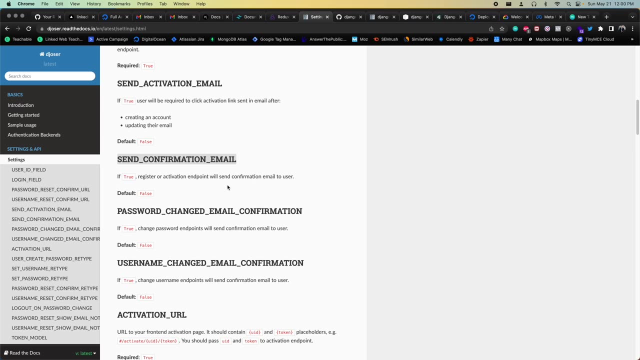 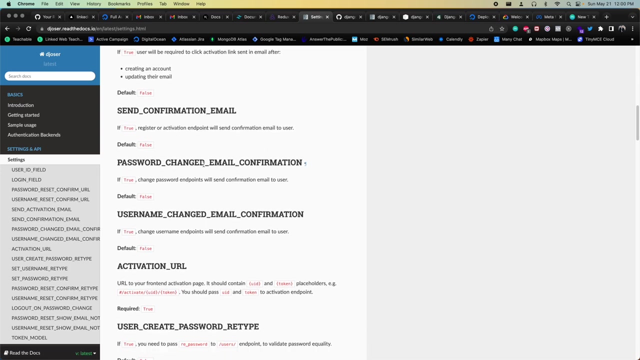 So I'm going to set this to true. And then we have send confirmation email. So once one registers or activates, then send a confirmation email. So I don't want to send a confirmation email, So I'll stick to the default of false. And then password changed, email confirmation. So when someone changes their 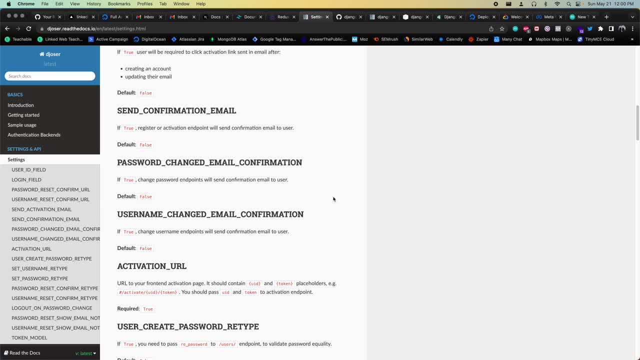 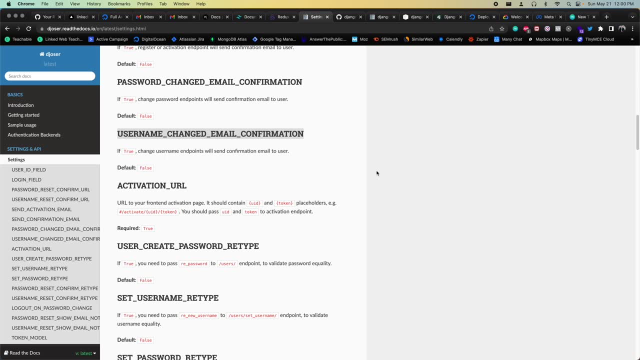 password. I don't really want to send a confirmation email, So I'll leave this at false And then username changed: email confirmation. We're not going to be doing that, So I'm going to set the username changing. So I'll just keep this as false. Then we got activation URL, So I'm going 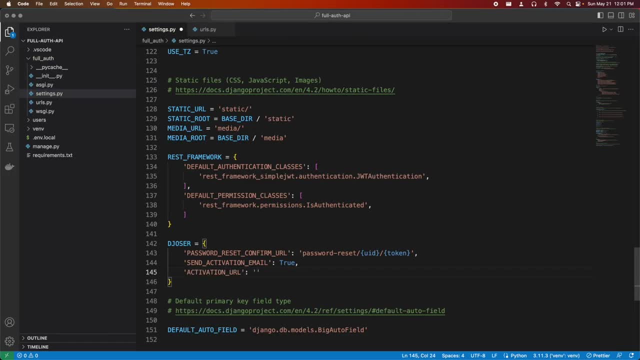 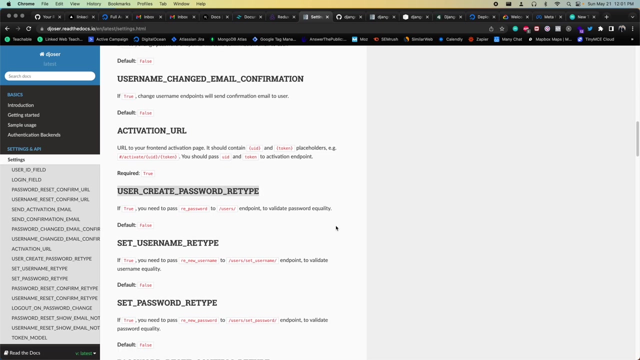 to copy this one. So this is going to be the URL for when someone needs to activate their account, which will be activation: slash the UID, slash the token. Then we got the user creates password retype. So this means: do we want to have a repass? 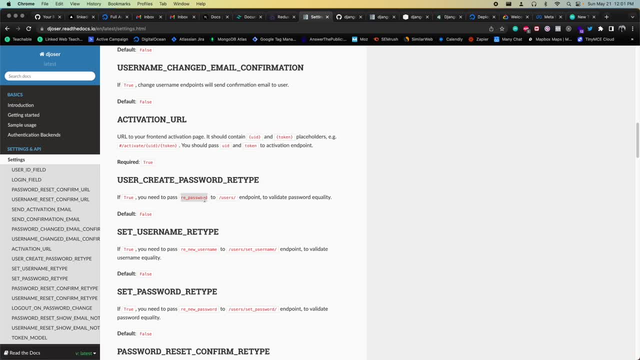 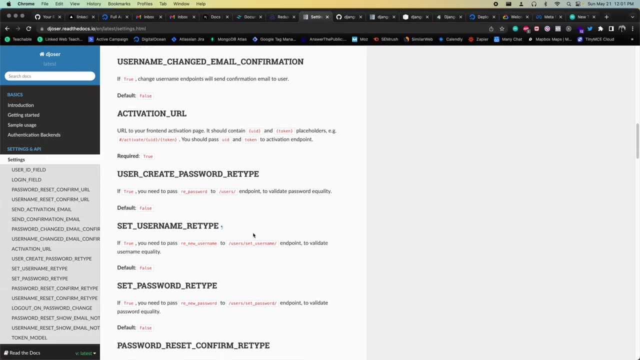 password field when someone hits the create user endpoint. So I do want someone to confirm their password. So I will set this one to true, because by default it's false. And then the next one set username retype. So this is, if you're setting a different username. 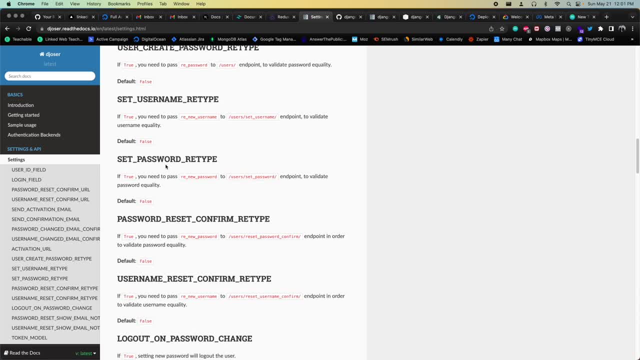 which in our case would be a different email. I'm not going to include this. We have set password retype. Now I'm also not going to have setting a password. We are going to have resetting a password, but setting a password. This is in particular if you're logged in and let's say you want to. 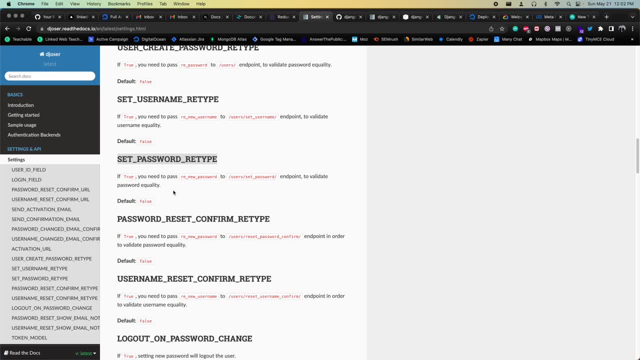 set a different password, then this is what you would use, And then this pretty much means: do you have to confirm the password that you're trying to set? So then you'd have to include this renew password field. I'm just going to set this to false, since I'm not going to have that. 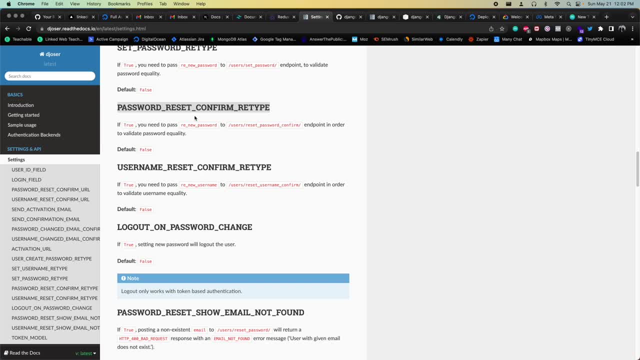 functionality in this app. And then I'm going to have password reset, confirm, retype, So this one I will have. so this will require the renew password And that's when I'm hitting this endpoint here And that's going to be when I'm resetting a password. So when we're resetting, 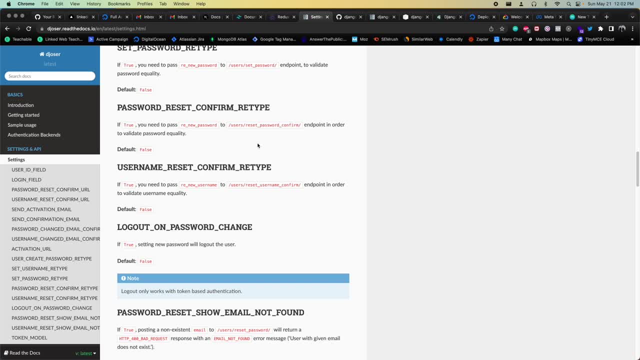 a password. what we do is we hit an endpoint which is going to send us a reset password link, And then we're going to go to that, And then we're going to have to put in our new password, And then I don't want to just have one field where I just set the new password. 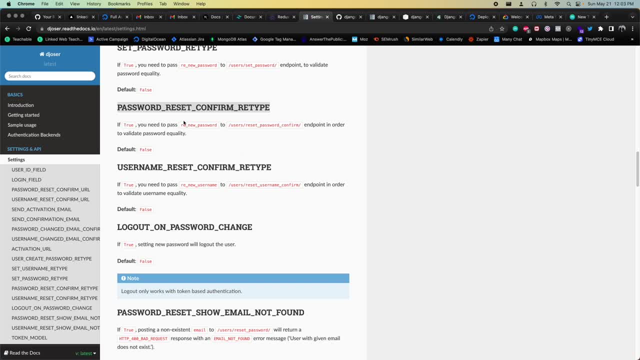 I also want to have a user have to confirm that new password. So I'm going to copy this And I'm going to set that to true And then, going back, we have username reset, confirm, retype. So I don't have username resetting. So 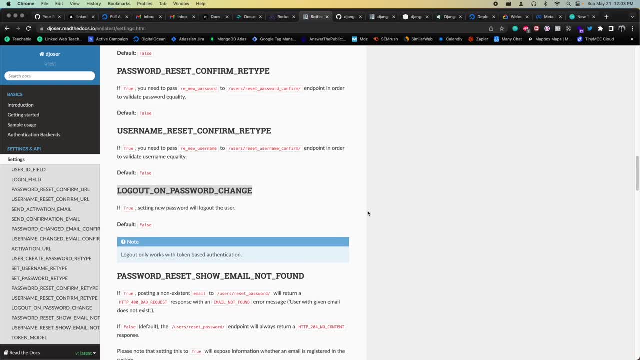 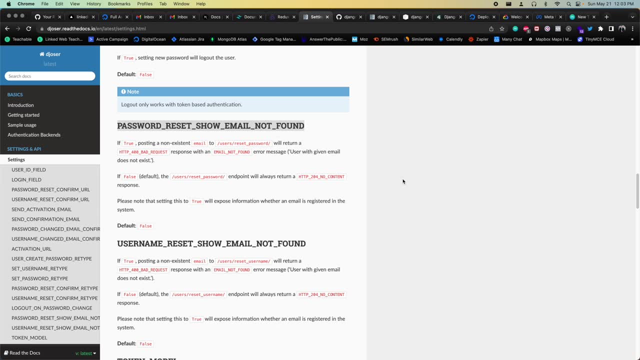 I'll leave that as false. Log out on password change. That will be false And then password reset. show email not found. So this is going to be when we're requesting to reset our password: We're going to put in our email and then we get the link. 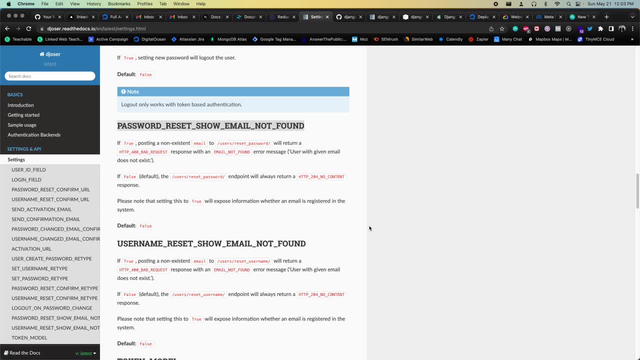 This will make it so that if your email it doesn't exist in the database, then we're going to get a 400 bad request. That's if you set this to true. But I'm going to leave this as false And in particular, it's because of what it explains. 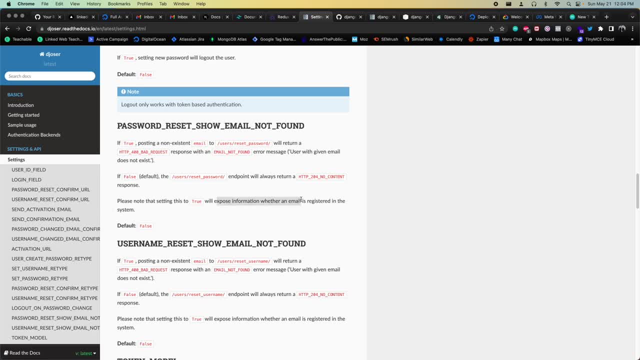 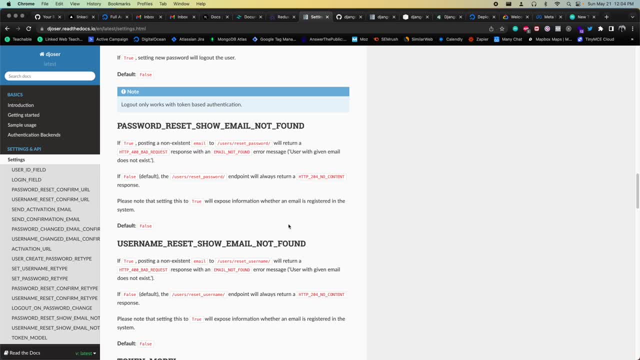 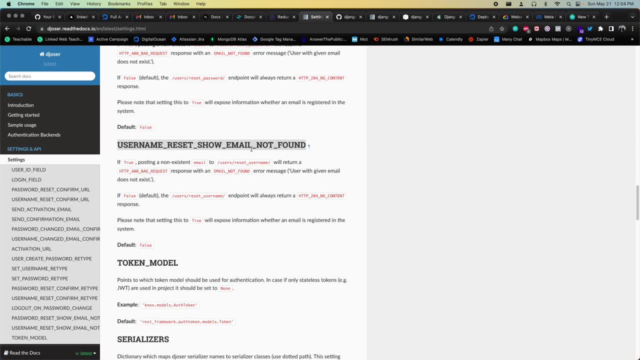 If it doesn't exist, then you don't receive that email, And I'm okay with that, just so that it doesn't reveal that this email exists in the system. Then we have username reset: show email not found- This also false, since we don't have username resetting. And then we got token model. 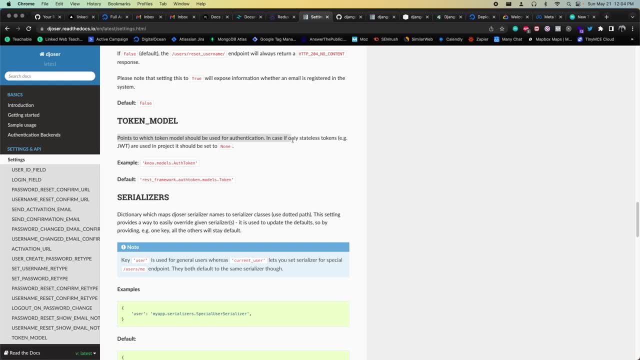 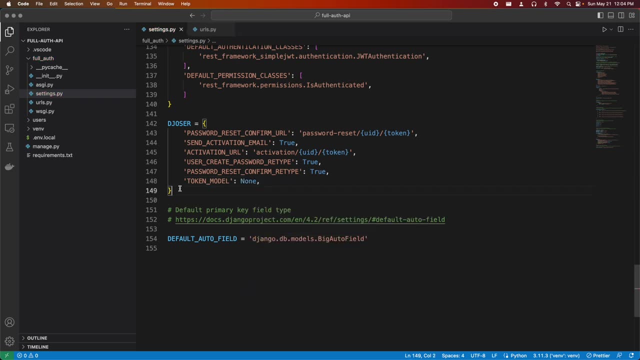 So points to which token model should be used for authentication in case, if only stateless tokens like JWTs are used in the project. this should be none, So I'm going to go ahead and do that, since we are using JWTs. So token model that will be none. So there we go. Those are the Joeser settings. The next thing: 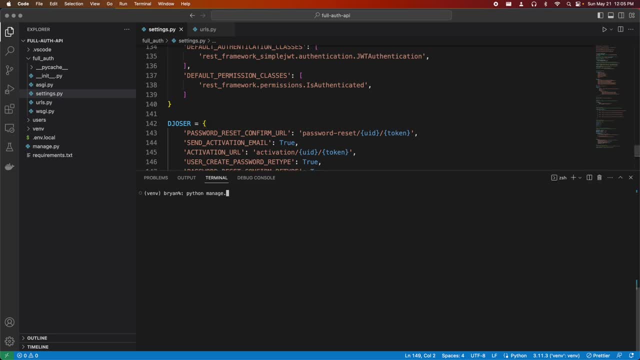 I'm going to do is: I'm just going to run this. I'm going to do python managepy run server localhost 8000.. And this way I can just see if I made any typos. So I didn't make any typos. 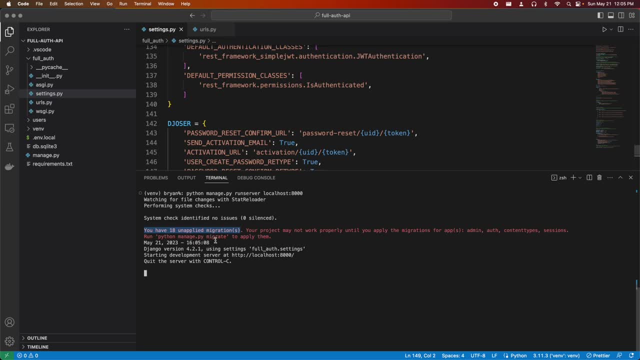 Now there's going to be these unapplied migrations. I'm not going to make these migrations yet, And that's because I want to set up the custom user model first, make those migrations and then I will migrate. So I'm going to stop running this. I just wanted to see if any typos are made. so far It. 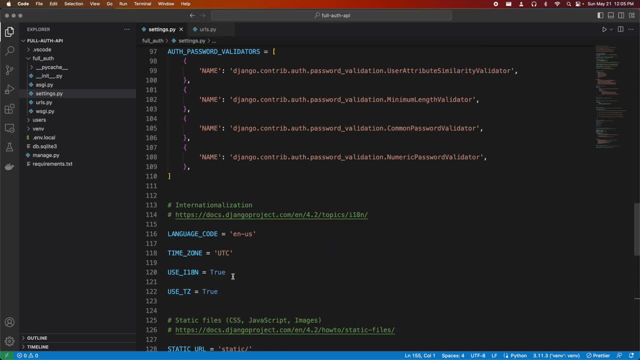 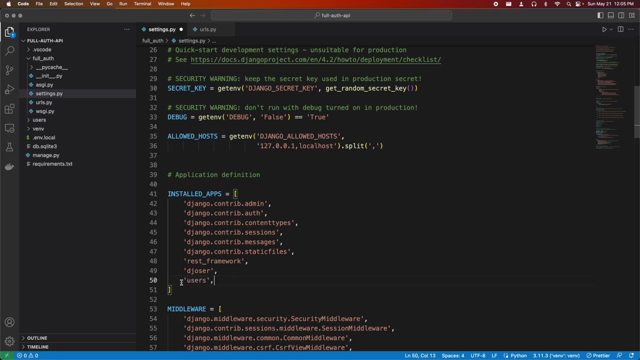 seems like there weren't. So the next thing I'm going to do is I'm going to scroll up, I'm going to go to my installed apps, I'm going to include my users app, because I will need this here, And then I'm going to start working on that custom user model. I'm going to open this up. 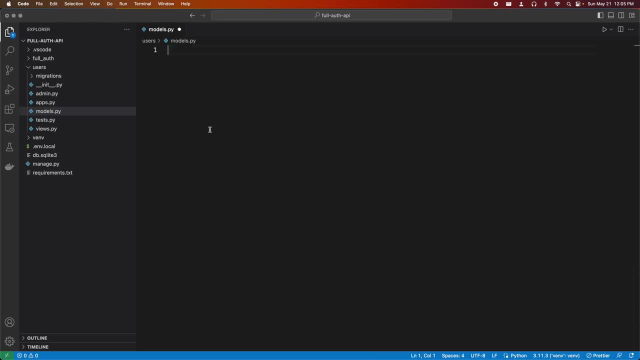 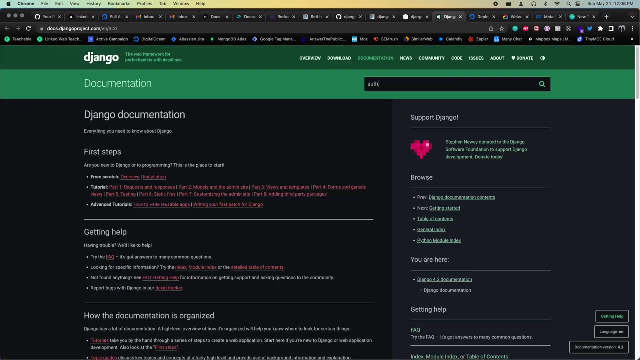 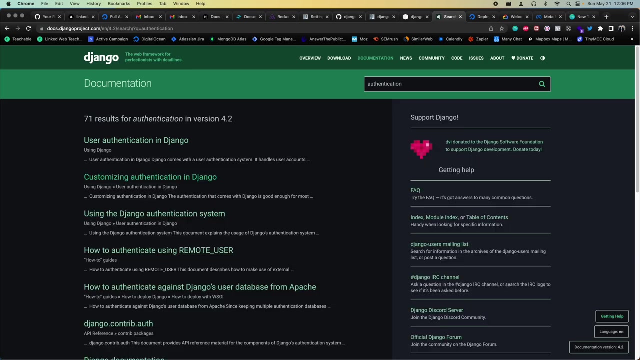 open up the models, and this is where I'm going to work from. So to help me out with this process, so I have the Django documentation open and I'm going to search for authentication, And then there's this right here, which is for customizing authentication in Django. 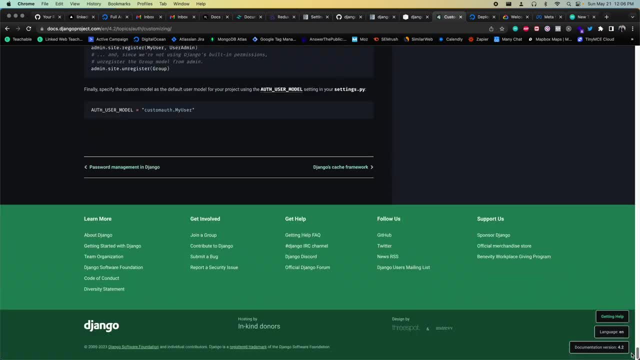 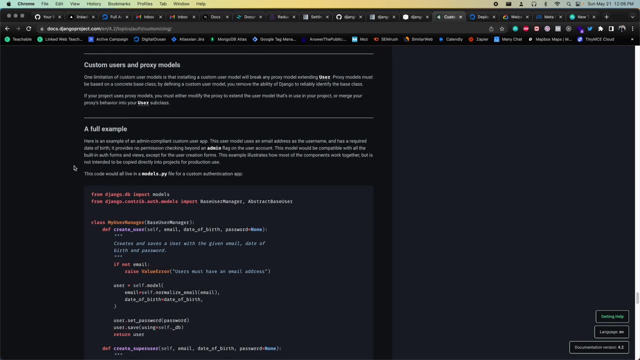 Then inside of here at the bottom, there's a full example of setting up a custom user model. So there's a section here. It says a full example. I'm going to do something very similar to what this shows here, So to help me out, I'm just going to copy this: 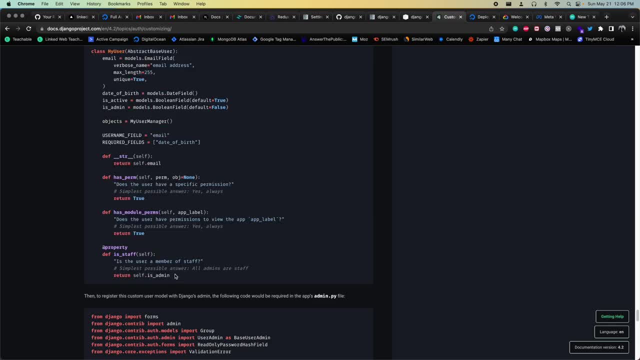 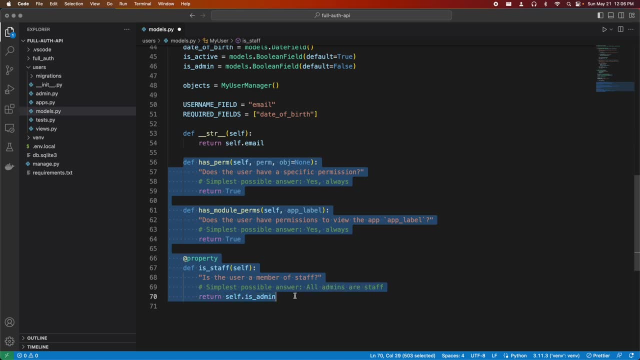 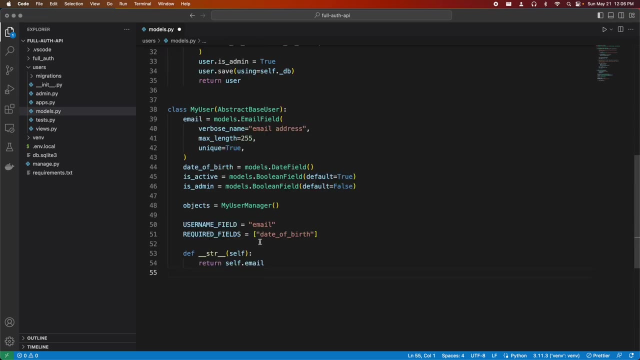 I'm going to copy everything here. I'm going to paste it inside of here. Now there are going to be things I don't need. So all of these things I don't need, So I'm just going to delete them And then string representation of this model. I'll keep it as email And then 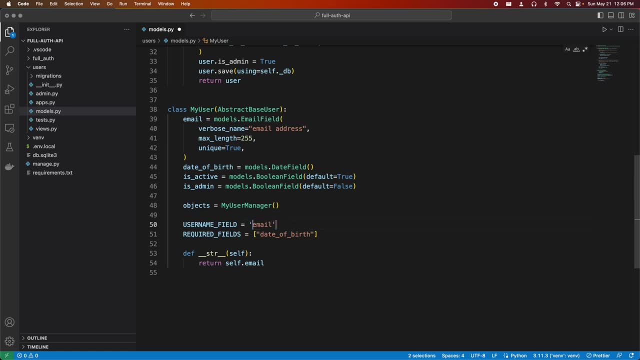 username field is going to be email. I'm going to be using single quotes And then I'm going to have required fields. So the username field is going to be email Is what I'm going to be logging in with by default, And then required fields are any. 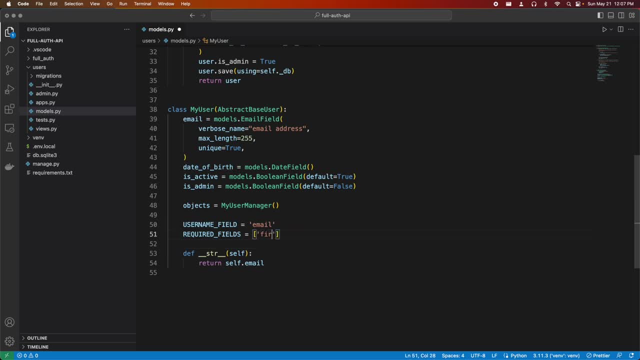 additional fields. I need to create my account, So I'm going to have here first name and last name, So when I'm registering I want these to be supplied as well. And then this date of birth field I don't want here, So I can have this email field. I'm just going to get rid of this. 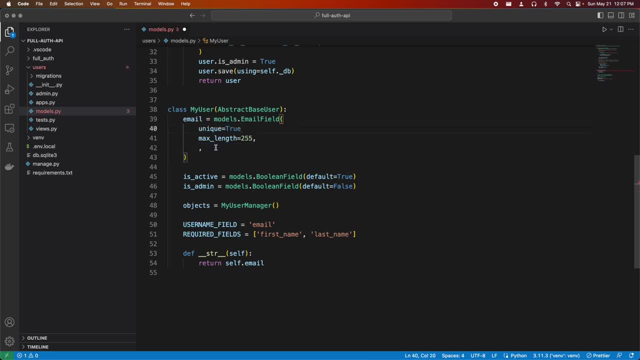 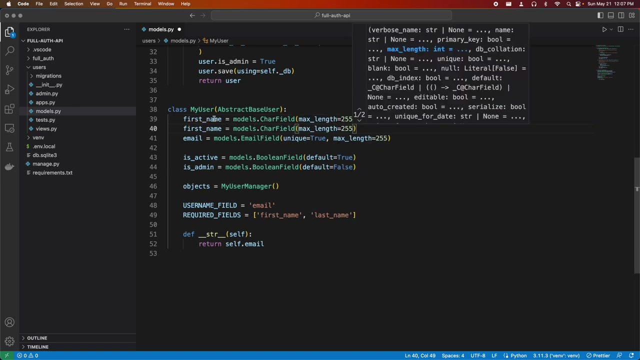 verbose name Unique. true, I'll have showing up first. I'm just going to reformat this a bit And then, because we have first name, last name, we have to define those. So I'm going to have first name, That'll be modelscharfield, And I'll have a max length of 255, let's say I'm going to 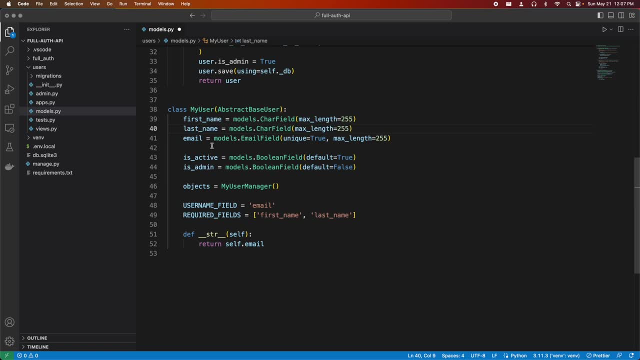 copy down a line and have the last name as well, And then I'm also going to rename this. So I'm going to call this user account And then I'm also going to have my objects. It's going to be user account manager. I'm going to. 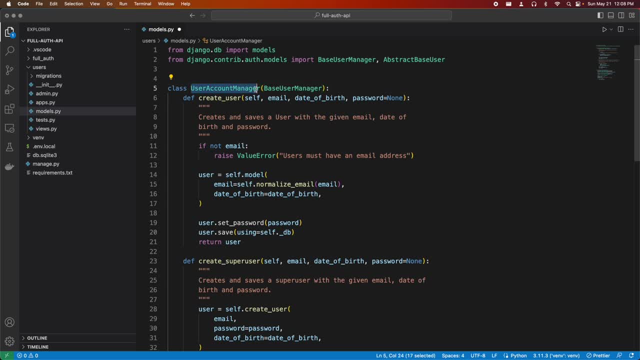 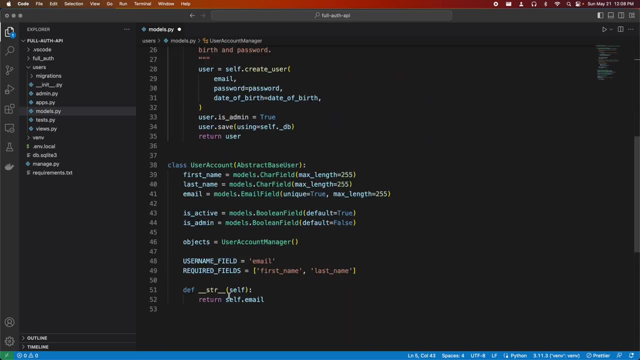 copy this and change the name of this, So it's going to be user account manager. So this thing is inheriting base user manager, And pretty much what this thing is is in Django. If, let's say, we have our user model, which is user, then we can do things like dot objects, dot create user. 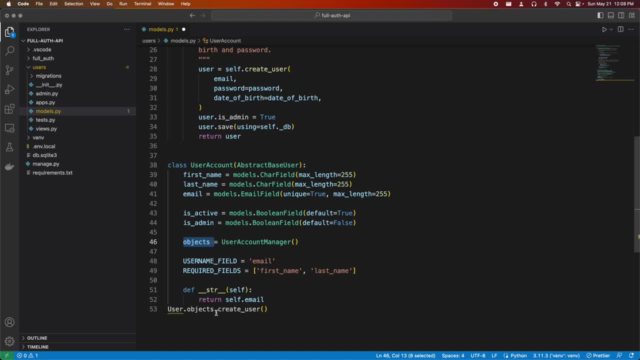 So that is what's going to happen, And then I'm going to have my objects. So I'm going to have this objects thing is It gives us access to things like create user and, let's say, filter and get, So all of those things are included inside of this manager. Now, in particular, we have this: 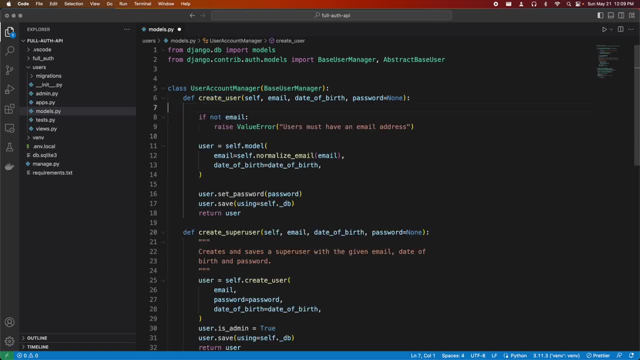 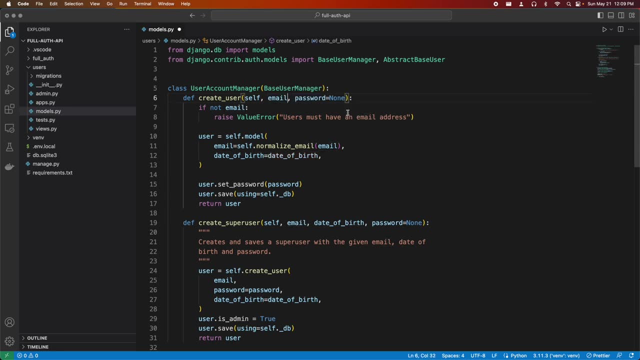 create user which I want to set up inside of here, And this is going to overwrite the behavior of creating a user, because now I'm going to be using an email And then we have this state of birth field, which I don't want. here We have the password. 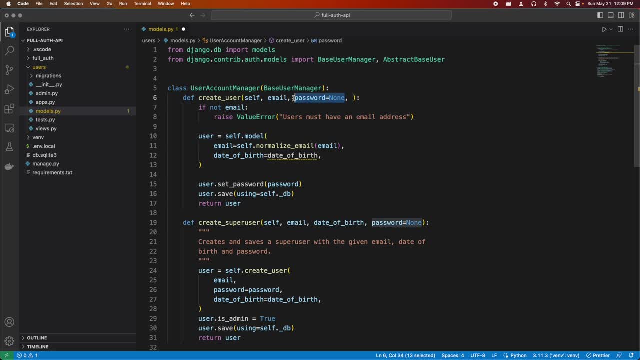 Which by default is none. So if this isn't supplied, then the creation isn't going to work, And then I'm also going to have keyword arguments here. So this is going to be a dictionary, and then it's going to include things like our first name and last name, So that's going to be our extra. 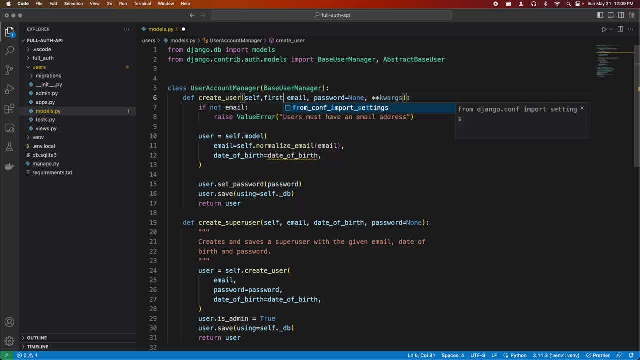 arguments. Now you can also, let's say, do first name and last name here, but I like doing it this way more, So I'm just going to keep it like this. And then, if we don't have an email, we're going to raise a value here, And then here's where we 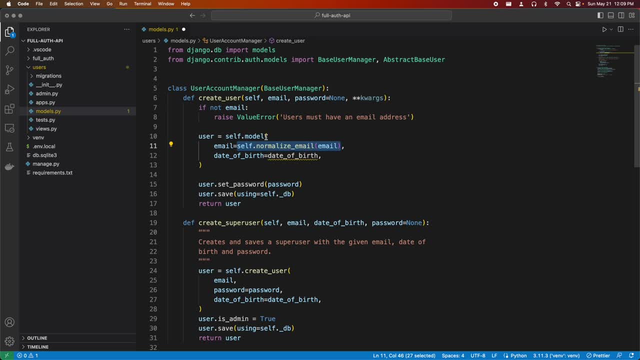 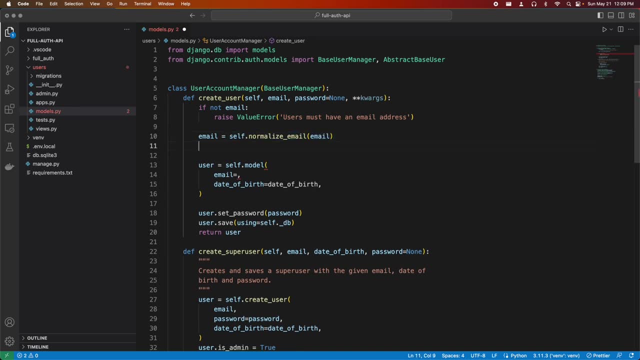 create our user model. So what I'm going to do is I'm going to do: email is equal to self dot normalized email. So what normalized email does is, if you have something like John Doe at example, dot com normalizing is going to set this part to be like lowercase. 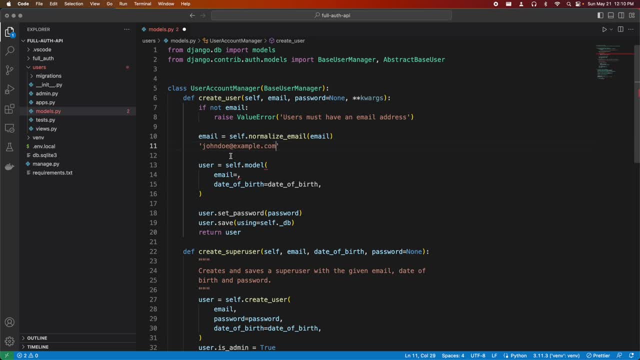 So I will end up with example dot com. Now one thing to note with normalizing an email: it only normalizes what's after the at, doesn't normalize what's to the left of it. So if I have John Doe and I put this through the normalized email, nothing will change. So what I want to do, 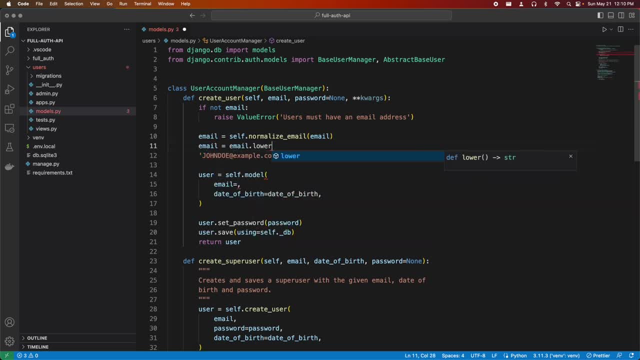 is email is equal to email. dot lower, And then that way it'll just set everything to lowercase And that way I would end up with something like John Doe at example, dot com, Because if someone, let's say, had their cap locks on or something and did John Doe at example, 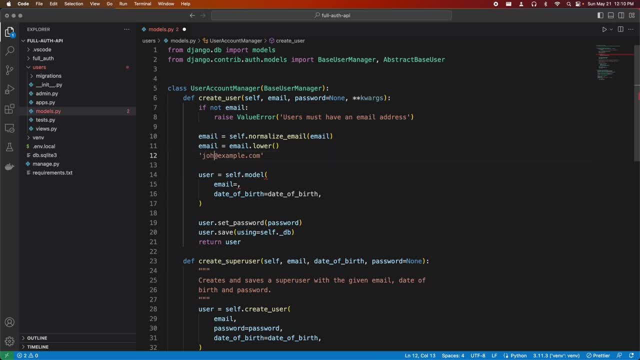 dot com the next time they go to sign in. if they use lowercase, they're not going to be able to log in. So that's where I'm going to have this email dot lower, And then here I'm going to have email. 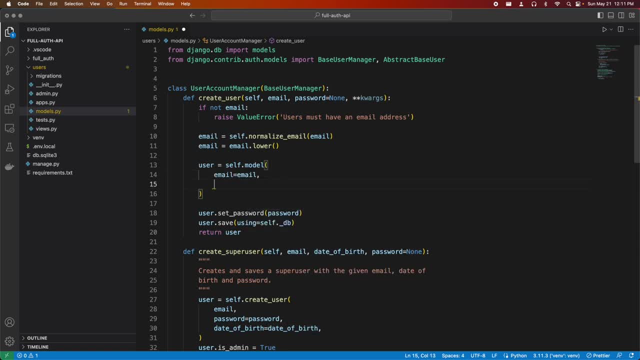 is equal to email, And then I'm going to have keyword arguments And then after that we're going to do user dot set password. So this is going to hash the password, Then we're going to save the user And we're going to return. 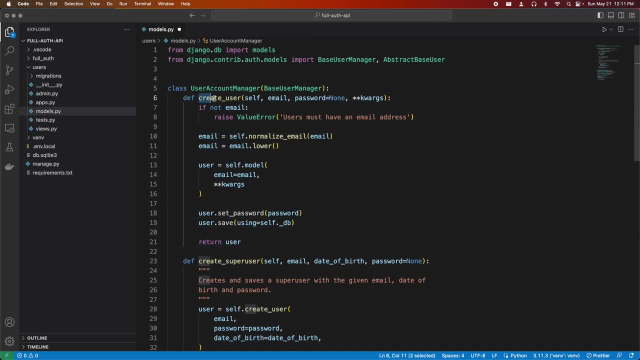 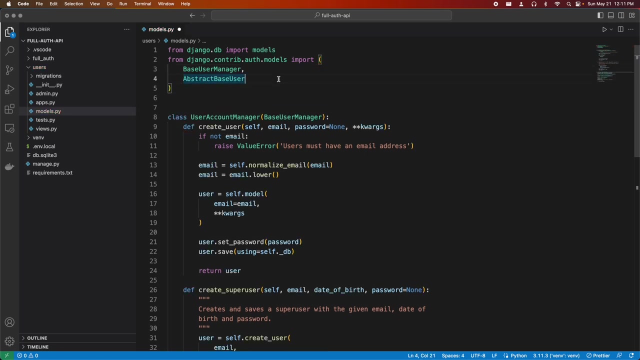 the user, And then Joseph behind the scenes is going to be using the create user of our custom user model now. Now I also want the ability to create a super user, And then I will want another import, And that one is going to be my permissions mixin, And this is something I'm going to have my 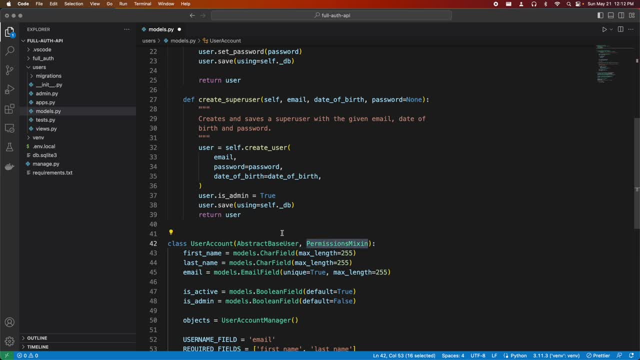 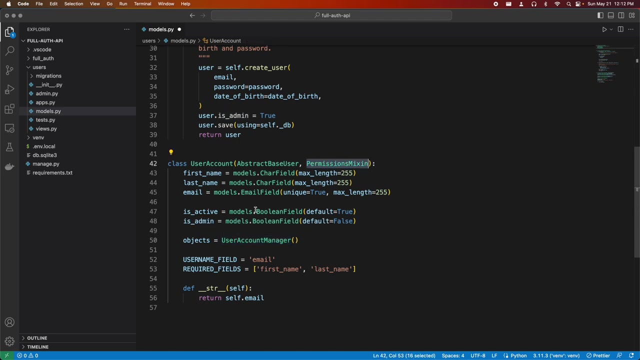 account inherit, So I'm going to place it in here And that's going to give me some additional fields like is staff and is super user and whatnot. So that will come with the permissions mixin And then, instead of using this is admin, I'll be using those fields that come with the permissions. 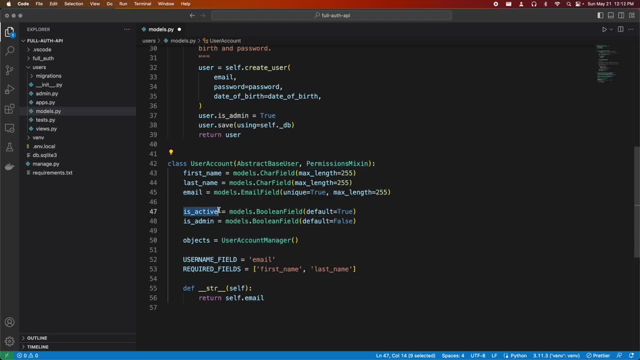 mixin. So right now we have this is active And this thing by default is set to true. Now this will be flipped to false with Joeser because of the settings that we have with needing to activate the account. So by default, even though this right now is true, 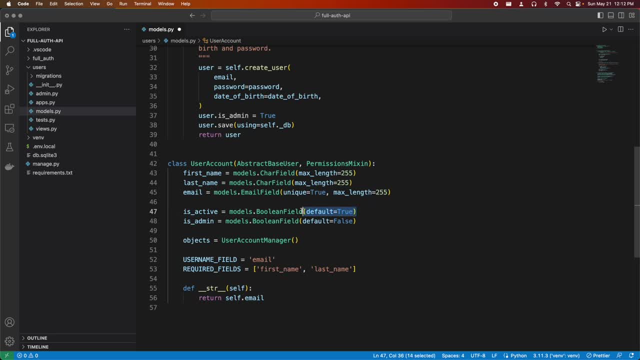 it will be false when we create users. Now I will keep this default as true here And in particular, this is going to be for when we're creating a super user. So if I have this default false when I do my like Python create or Python manage, dot pi create super user When I go to create that, if I 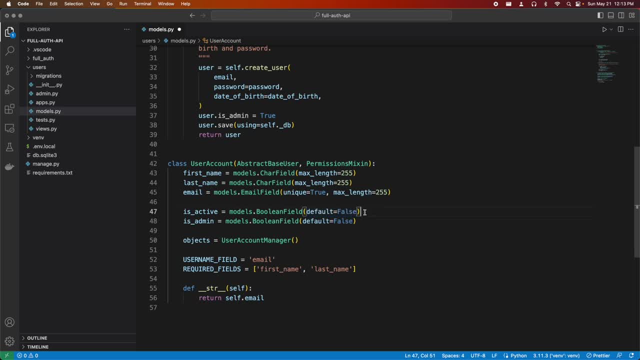 have this as false, my super user is going to have is active as false And then I won't be able to log in with my super user. I'd have to go into the database itself and adjust this to be true, just so I can log into my. 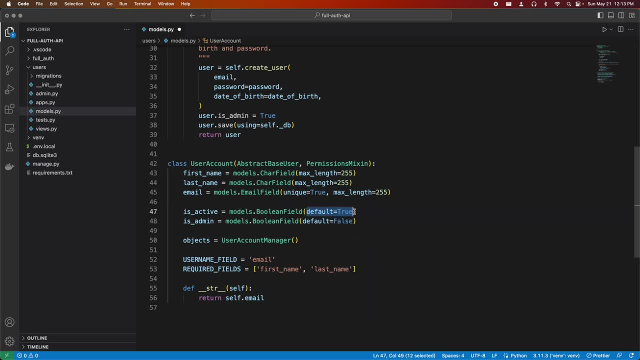 admin panel. So, because of that, I'm going to have this default be true. And then, instead of is admin, I'm going to have this staff. This, by default, is going to be false. Then I'm also going to have is super user. This will also by default be false. 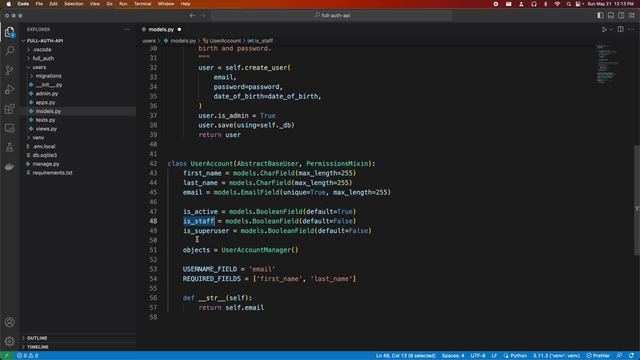 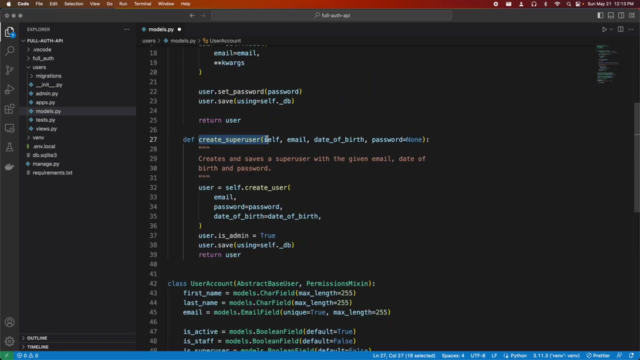 So is staff. This lets us log into the Django admin panel. And then is super user: just gives us a super user permission. So this right here is what actually gives us the ability to, let's say, go into the admin panel and edit things. So the next thing I'm going to do is go to this, create super. 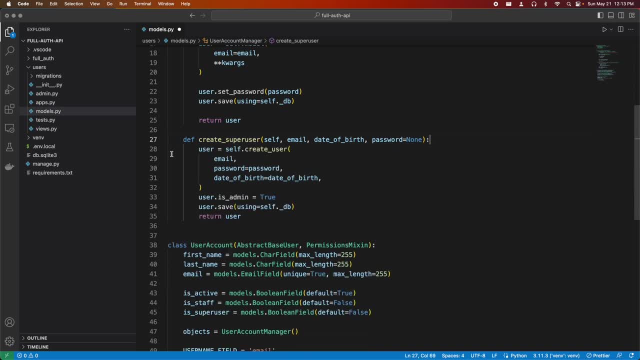 user. I'm just going to get rid of this doc string. And then this has date of birth inside of here. I don't want date of birth, I want keyword arguments. And then this behind the scenes is just going to do selfcreate user, which is literally this: 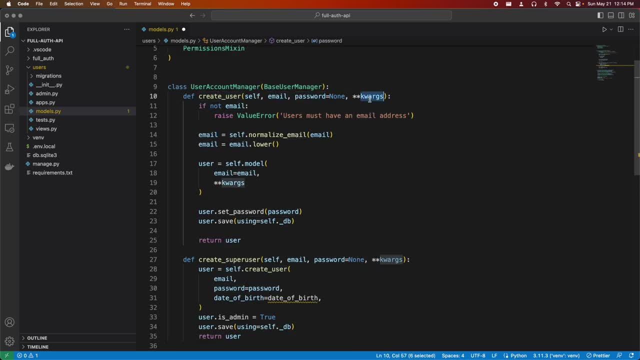 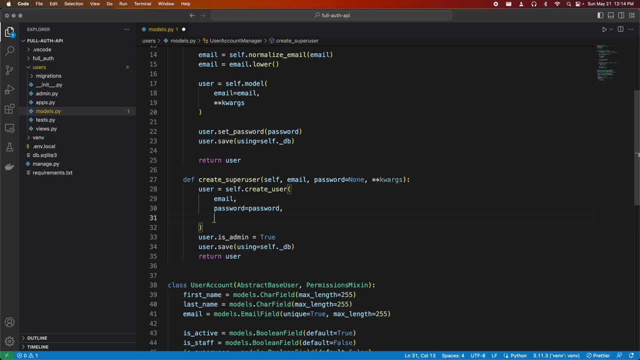 function here. So we're going to pass the email password and keyword arguments to this thing And it's going to create a user and it's going to return that user. So then here the main difference is I'm going to have keyword args, So we're going to get that user, which gets returned. So the next. 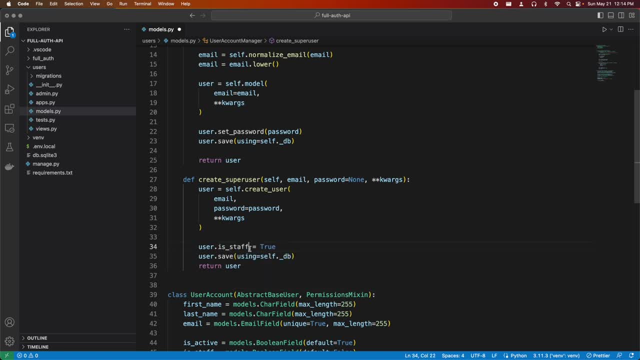 thing we want to do is we just want to set those properties. So is staff- we want to set the true, and also is super user- We want to set the true, and then we want to save that, And that's pretty much it. That is now going. 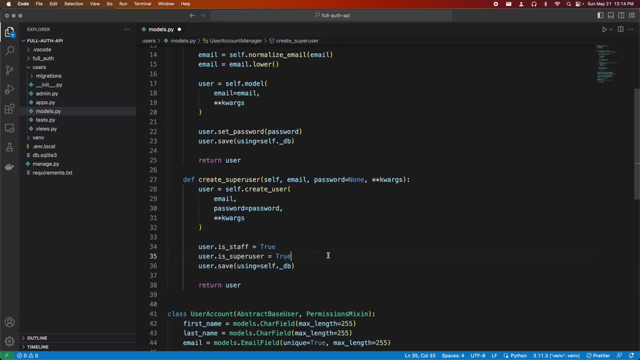 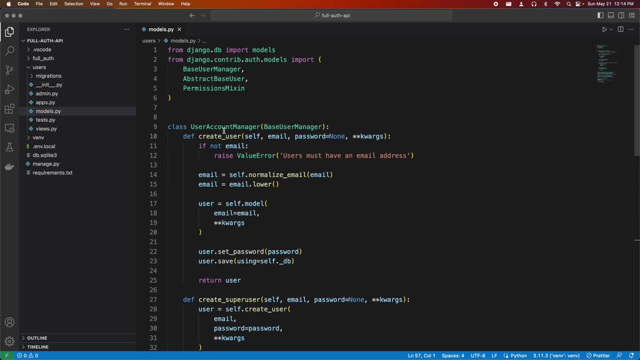 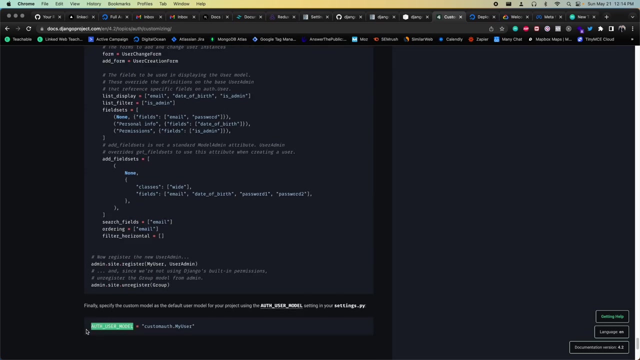 to be a super user because they have these two flags set to true. So there we go. That is our custom user model created, So it wasn't too bad. but now we have to set this to be used. So the way we do that is there's a setting inside of here. If you scroll down, you'll see this auth user model. 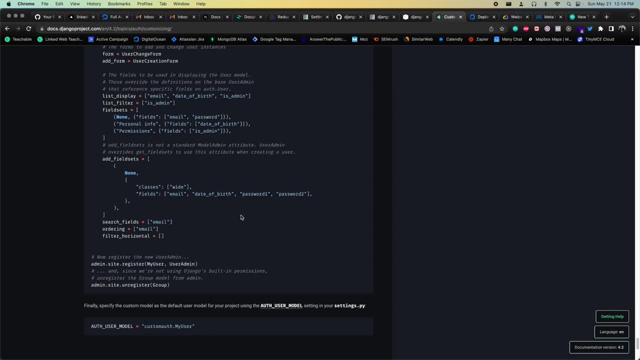 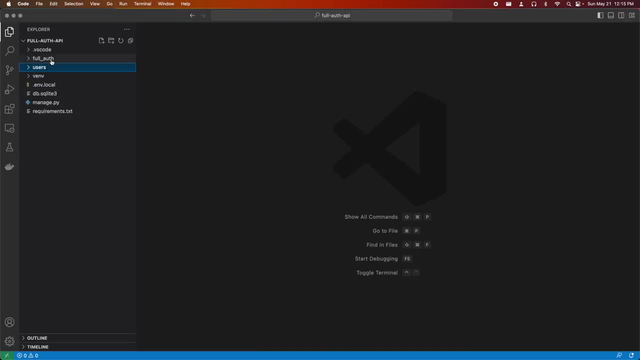 You just have to supply the path to it. So that's the last thing we have to do, and our custom user models in place, We can make our migrations. I'm going to go back to my project. open up my settingspy scroll to. 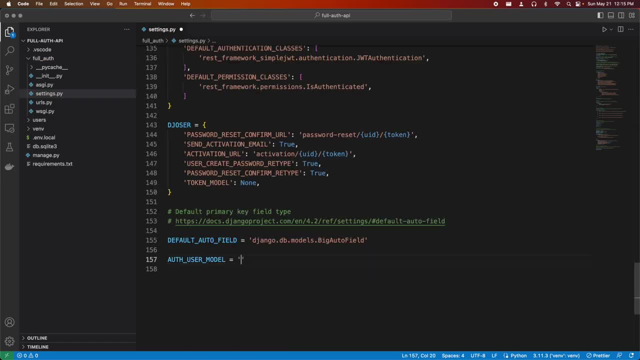 the bottom, and then this will just be equal to users. That's the name of our app and then user account. All right, So now we're in a pretty good spot. So the next thing I can do is Python manage dot pi make migrations. There we go And Python manage dot pi migrates, and that will migrate to my 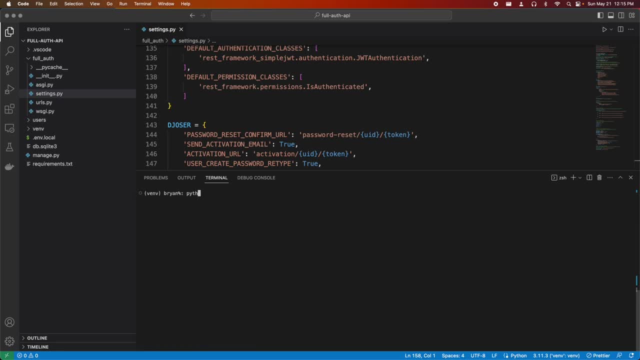 SQLite database. And now we can just have our server running. So I'll do manage dot pi, run server localhost 8000. And then I'm just going to have this running so that if I ever make a typo I can just very quickly catch it. So this is something I like to do. 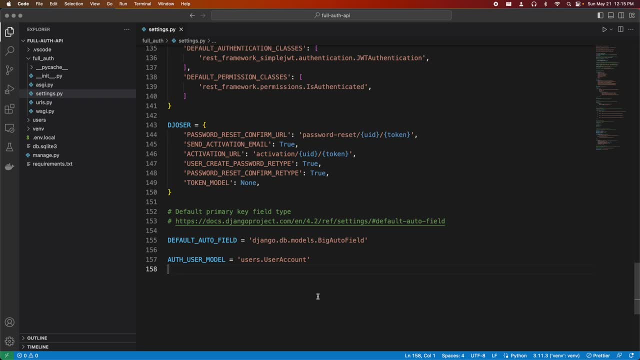 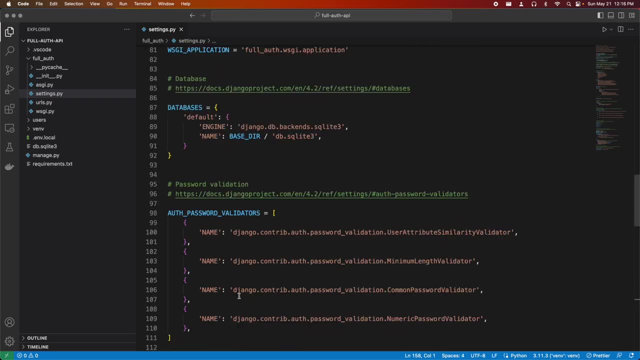 So I'll close that And then, with what we have here, we're actually already set to test things out. Now. we didn't set up course headers yet. I'm going to do that afterwards. It's not really important, The course headers are more important, But I'm going to do that now. So I'm going to do. 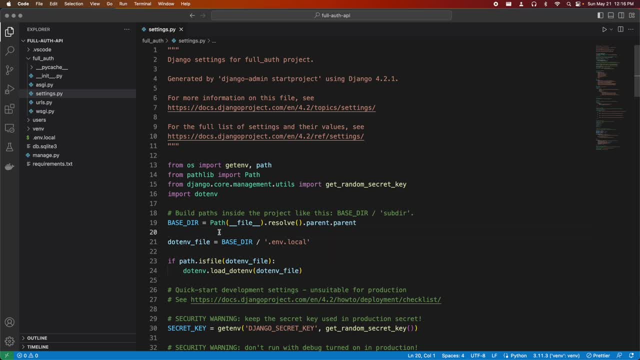 more for the client And that will set up some headers in the responses which then will allow for cross origin requests. Although if we're using something like Postman, we're not in a browser environment, So course doesn't really come into play. So course is more of a browser thing. So 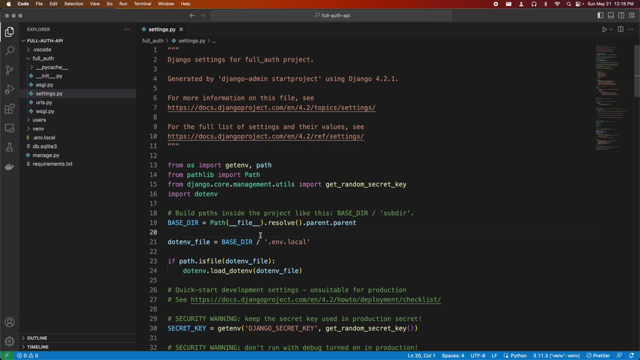 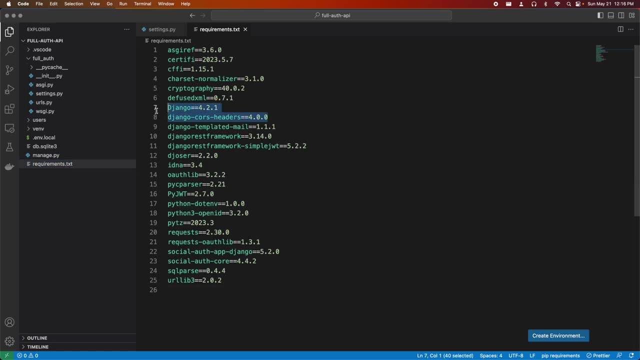 that's just something to note. Now we will have to have that set up, But to test that- what we have right now- we don't have to quite do that yet. Now that is something that we did install, But we're going to get to setting that up after just testing what we have. 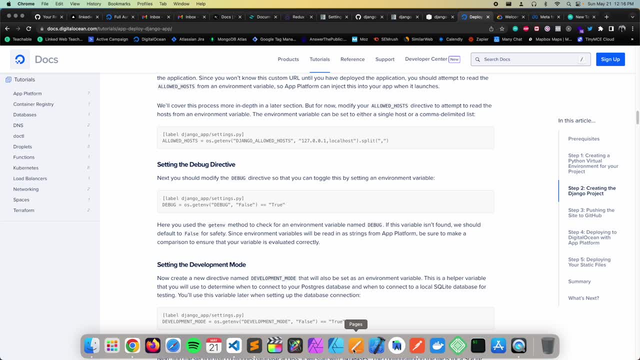 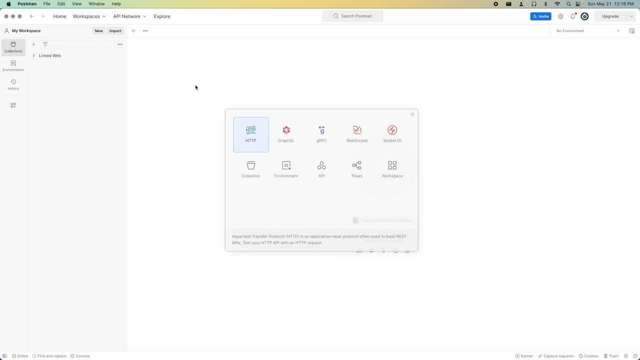 So let's go ahead and see what we got. I have Postman open, So you're going to want to do the same. If you want to test out the API. I'm going to create a new collection And then I'm going to call this full auth. 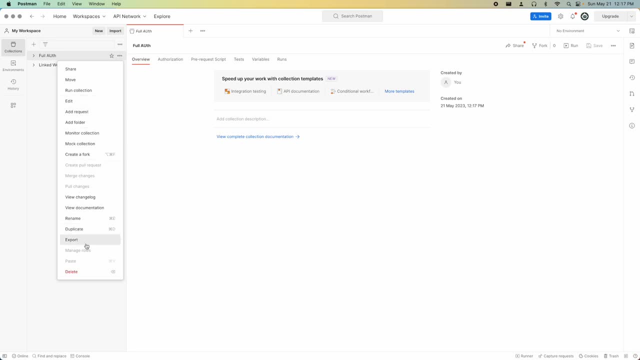 And, of course, I made a typo. Where's my renaming There? it is Okay. so this is where I'm going to put anything that I want to test out, And actually, something I have to do before I can even test this out is set up my email settings. 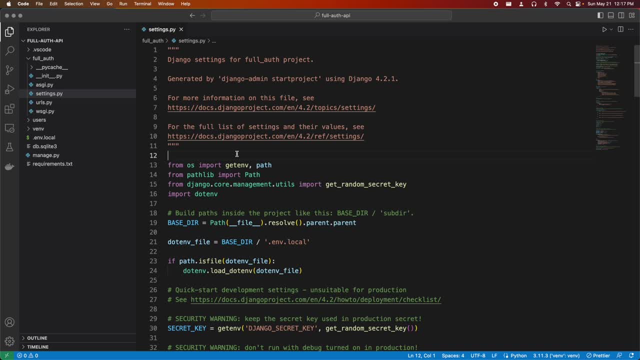 So that's something actually didn't do yet, So actually, so we can't test out quite yet. Now, when it comes to sending emails, there's different approaches that you could take, And the approach that I'm going to take in this app is by using an AWS service. So this service 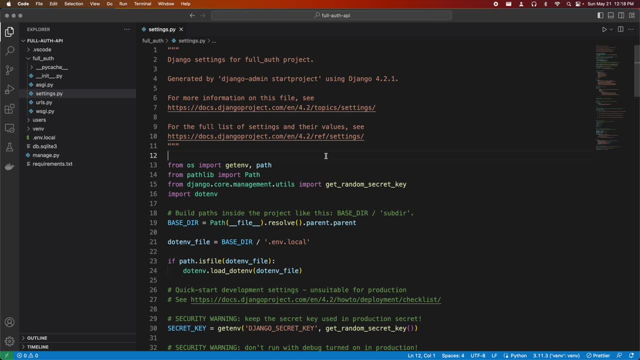 is going to be the AWS SES service, And that is a service made for sending emails. So that is what I'm going to be using in this project. Now there are other options. you can use things like SendGrid or other options as well, But in my case, this is the approach I'm going to take. 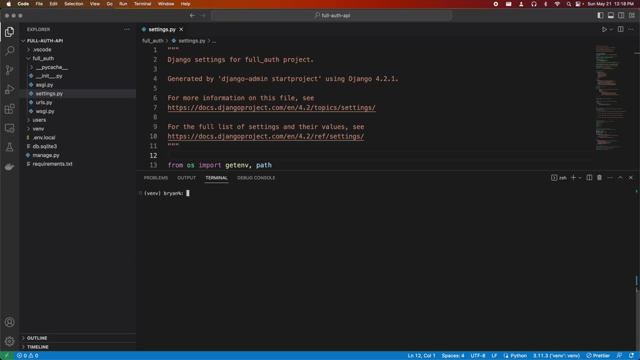 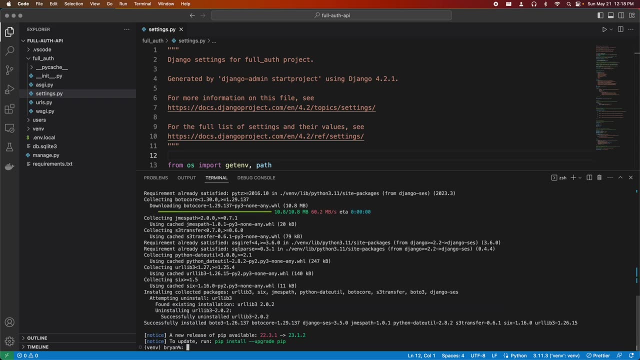 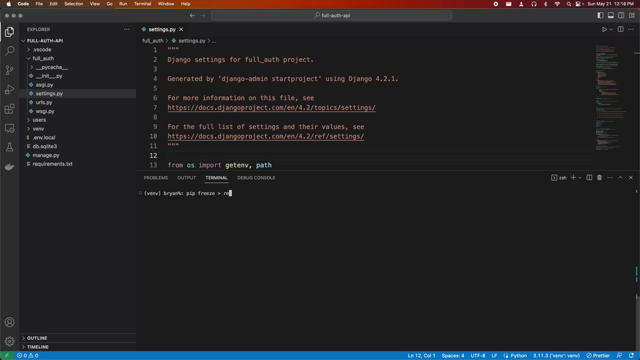 So I'm going to open things up. I'm going to stop running this And I'm going to do a pip install for Django dash SES. That's going to install that package for me. So I'm going to clear, I'm going to do a pip- freeze requirements TXT. So anytime I install new dependencies. 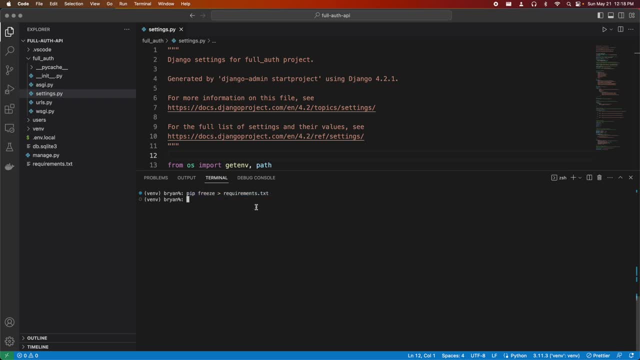 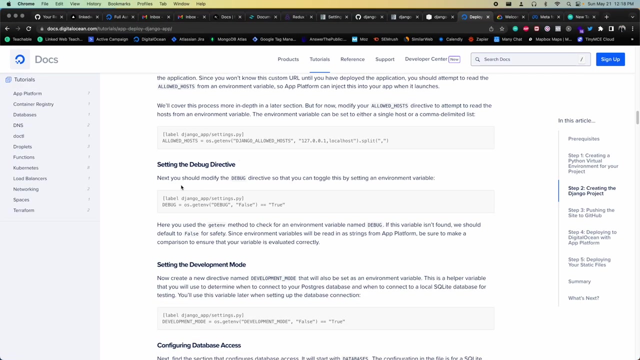 I want to do this just so I can put that inside of the requirements TXT and clear this up now, And I'm going to rerun my server, So set this up. So we're not going to test quite yet, but we're almost there. 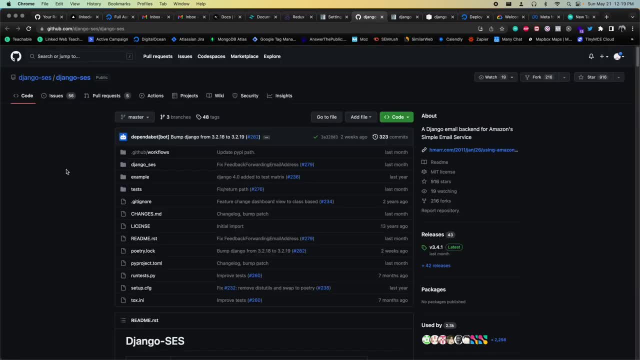 And this right here is the documentation for Django SES. So I'm going to have links to everything I'm using in the description so that we don't have to look at this URL and try to type it yourself. It'll all be in there. And then to set this up first, 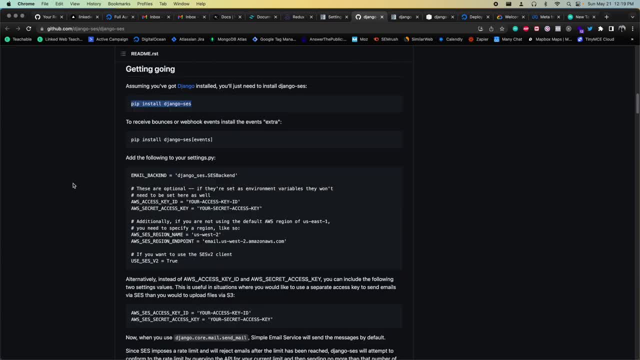 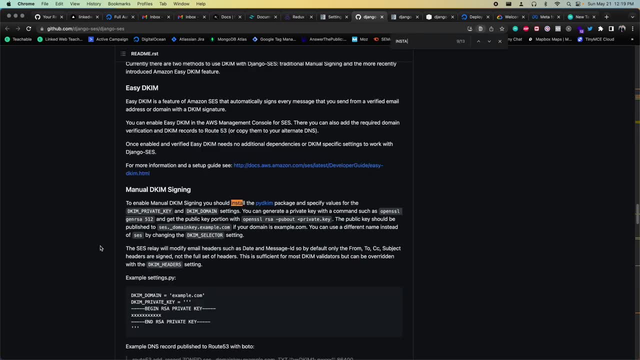 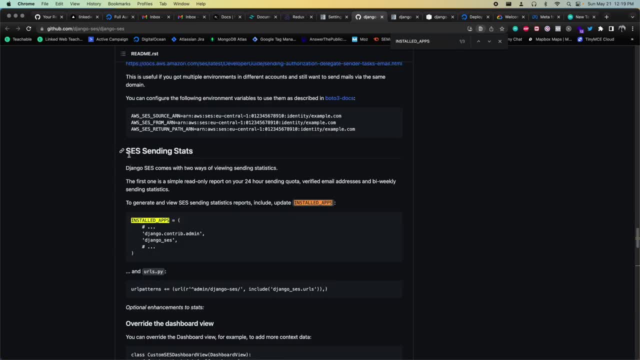 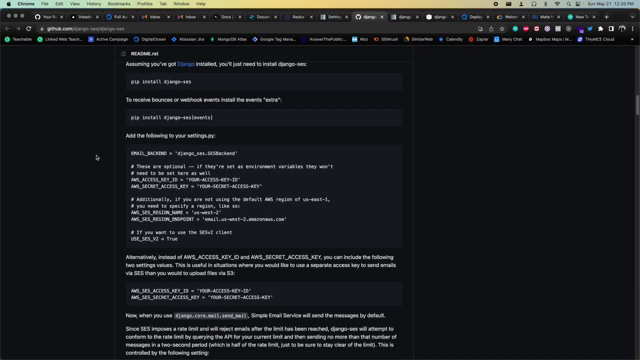 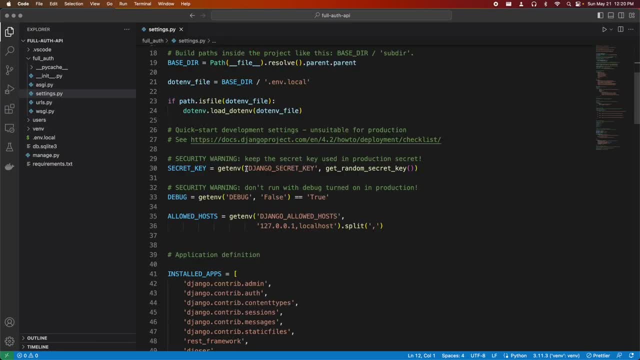 So I'm going to scroll up and find this stuff here. So first of all we want to set email backend to be this: So for my email settings I'm going to find a spot for that, Maybe below the databases. I guess we'll clunk that. 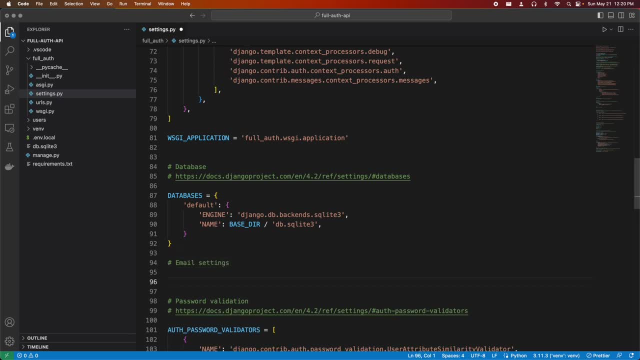 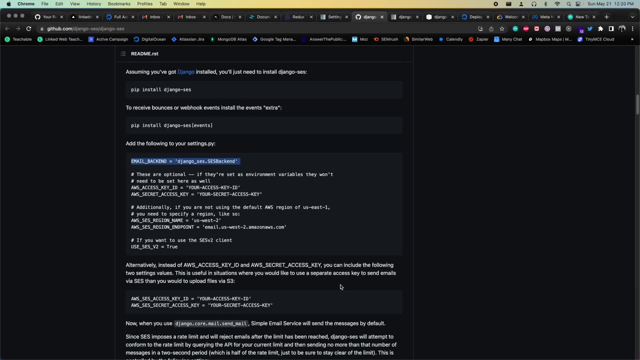 Okay, Let's see. I'll have my email settings, So email backend will be this right here, And then you're also going to have to set up your AWS access key ID and secret key. Now, one thing I'm going to be doing in this project is I'm going to be using digital ocean spaces. 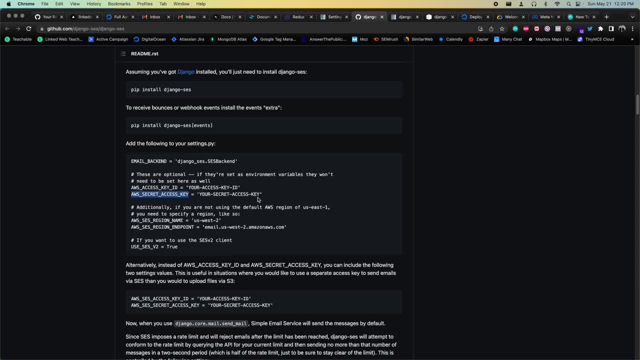 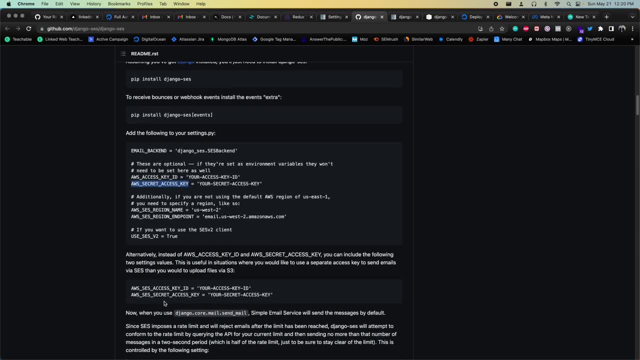 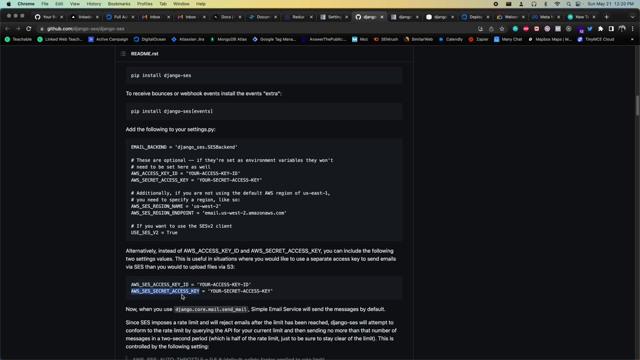 which is very similar to AWS S3 buckets, And then that is also going to have an access and secret key. So one thing that SES allows you to do is alternatively set up these settings- So AWS SES access key ID and also the secret key, And then that way I can have these credentials separated. 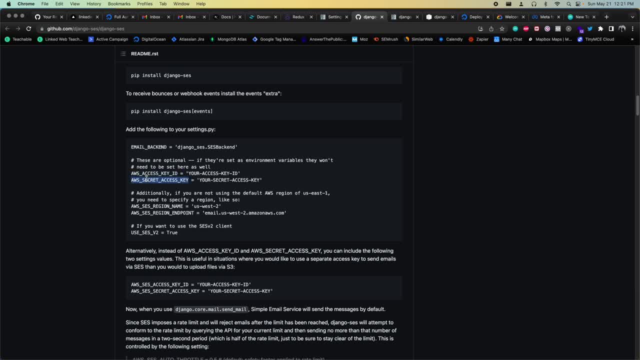 So the one for the digital ocean spaces, it's going to be these ones here, And the ones for SES will be these ones here, And then, behind the scenes, they're also using the Python Boto3 package to do this communication, So that's actually something you would see inside of. 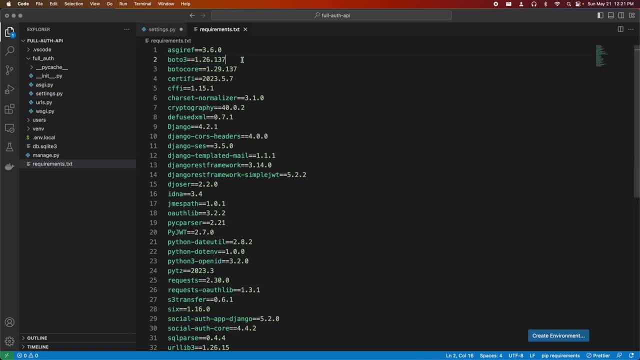 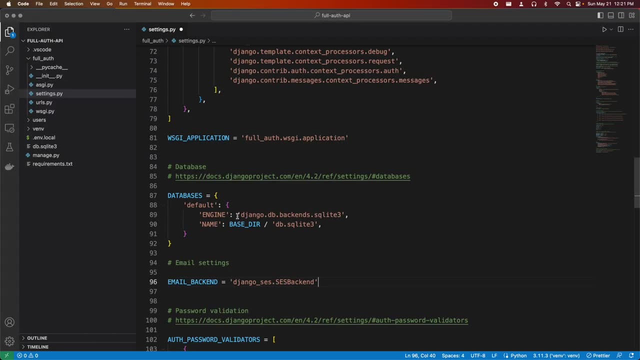 the requirements, TXT. So what I'm going to do is I'm going to copy this, Then I'm going to paste it here. I'm also going to grab this, paste it here, just so that I have these values. And then also I'm going to do: 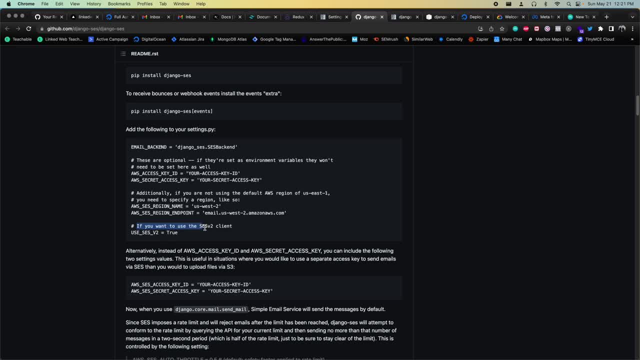 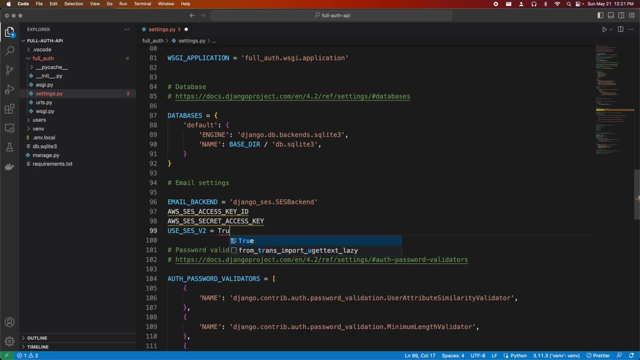 this use SES v2.. So that's, if you want to use the SES version 2 client, So might as well do that. So I'll also put that as well. I'm going to set that to true. So these we're going to set up in a bit, I'm just going to 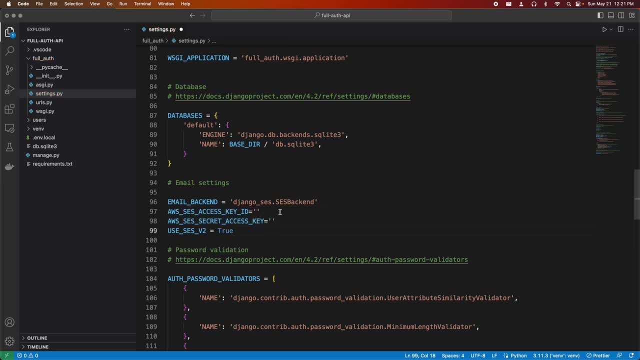 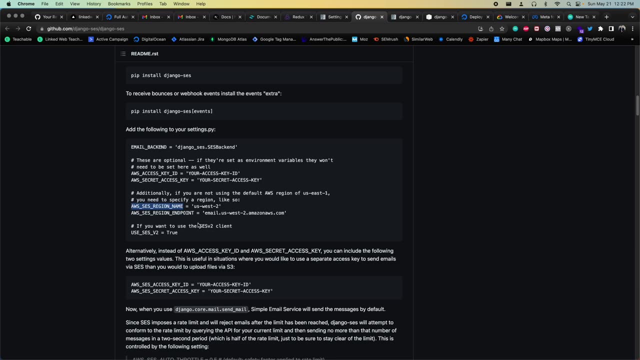 leave them like- actually I'll just put empty string for now, So it doesn't complain- And then we're going to have AWS SES region name. That's something we're going to need, So I'll put that here, And we're also going to need the SES region endpoint. 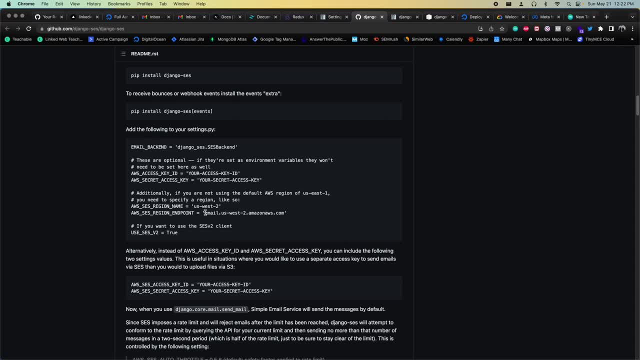 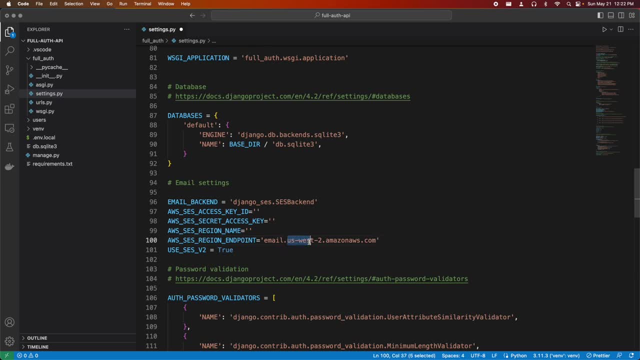 And then for the region endpoint, what we're going to do is we're just going to grab this right here and then paste it in here, And then this is going to be using the region name. So what I can do is, inside of here, I can just have the region name and I can make this an F string, So that way, 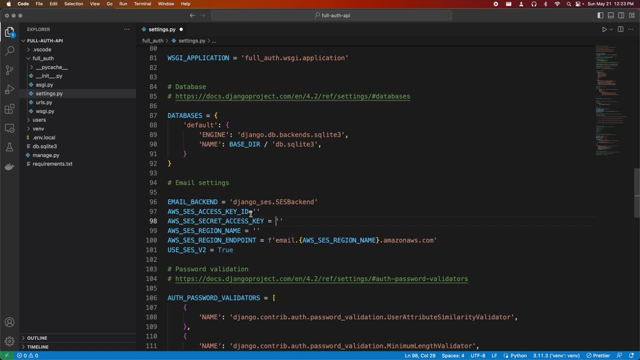 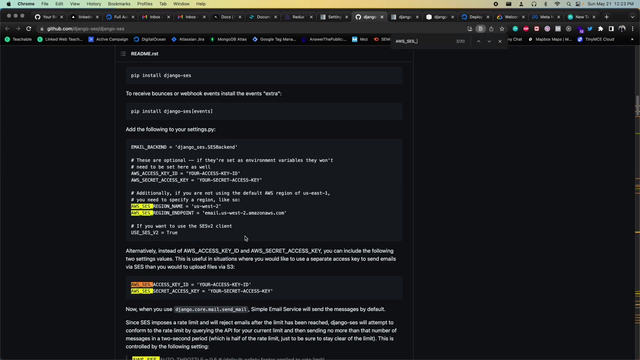 I can get plugged in there. So we're going to have email dot whatever our region is, dot Amazon, AWS dot com. It's going to set that up. And then another thing we're going to need. So if we search in here, there's AWS SES from email. So this is an optional option, So the email address can. 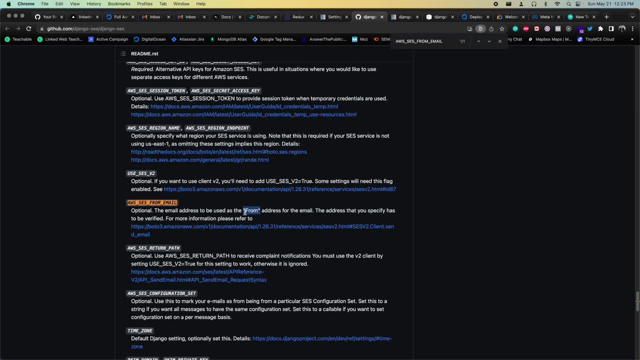 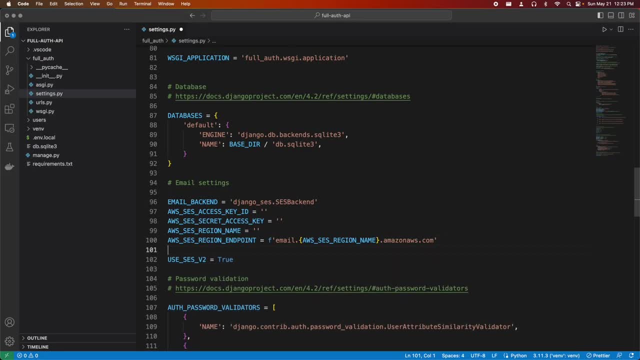 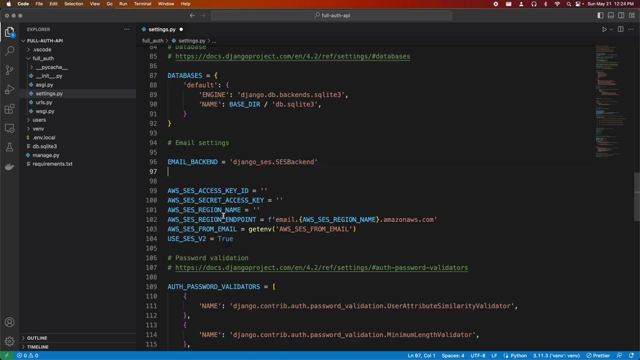 be used as the from address for the email, And that will be this setting here. So I'll put that say over here. And now I'm going to start making use of the environment variables. So I'm going to do this, I'm going to set this to be this, And there is actually one more setting we're going to need. 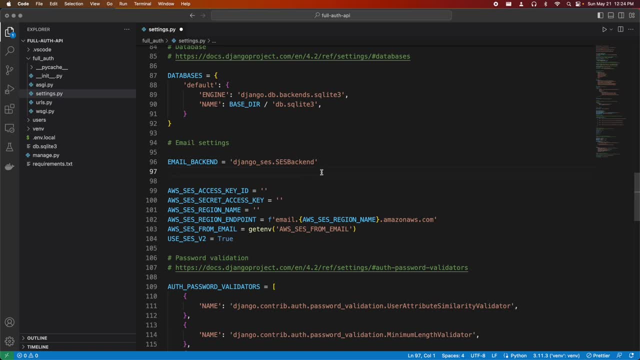 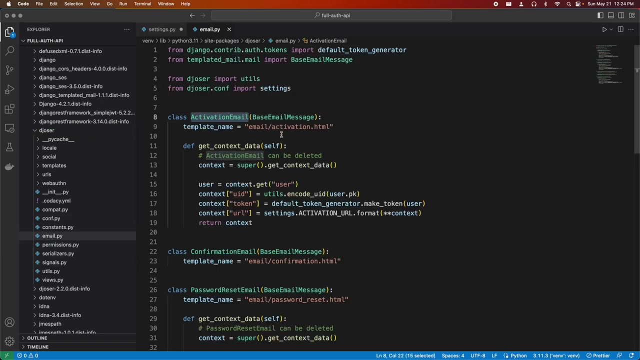 And it doesn't show it in that documentation. but it's also more particular with Joeser. So if we go into Joeser and then we take a look at email, So let's say, if we're sending an activation email Behind the scenes, this is: 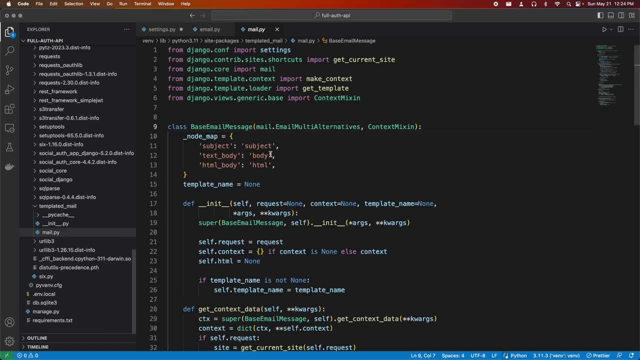 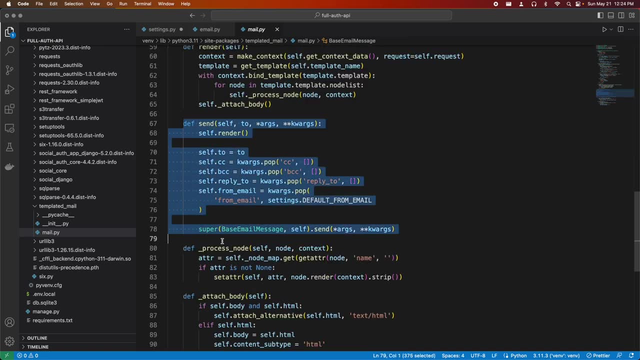 I'm going to set up the from email And then, if we go through this, we have contacts getting set up, but we also have the send. Now, this send it's going to set up the from email And it's going to do it using settings dot default from email. So it's going to be looking for the setting. 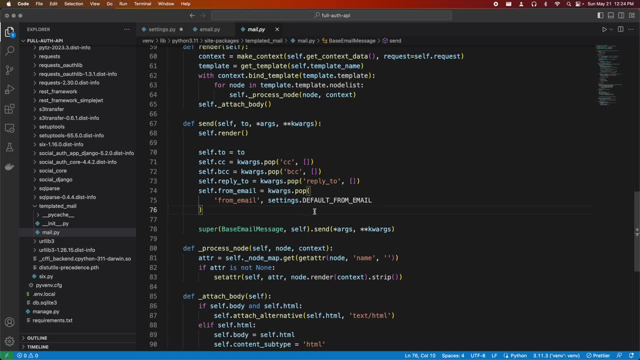 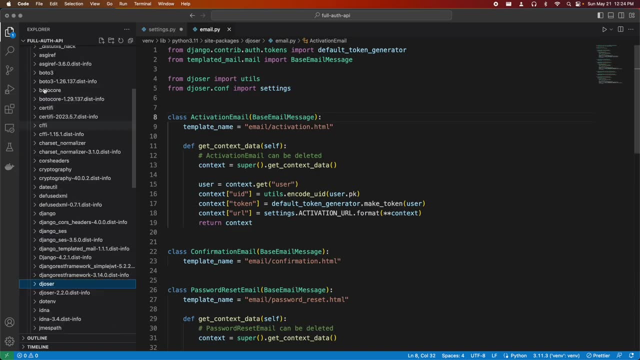 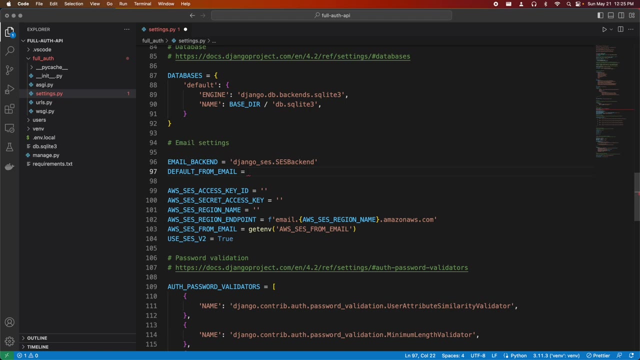 And that's going to be the from email when Joeser is sending emails. So we actually have to set this up, So I just copied that setting. I'm going to go back into here. I'm just going to paste that And I'm going to use an environment variable for this, And it's going to be the exact same as this. 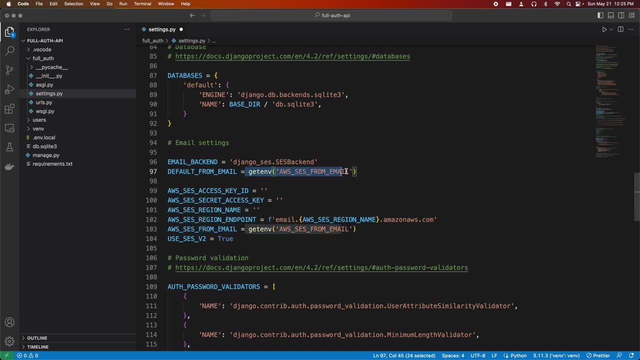 AWS SCS from email. So we're going to use the exact same value. Then for the access key, I'm going to have get env. I'm just going to copy this and paste it here and here as well. So for this, 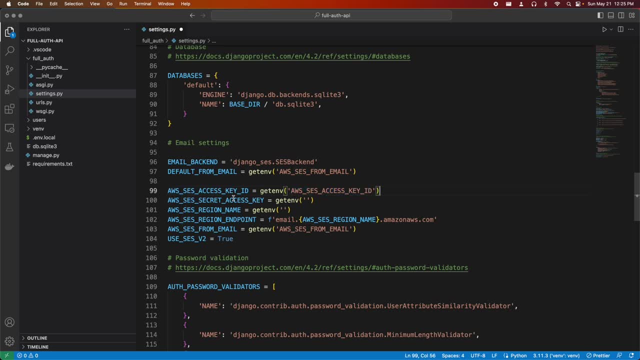 it's going to be AWS SCS access key ID. This environment variable is going to be the secret key. Then I'm going to have region name, And there we go. These are all the email settings. So now I'm going to open up my env file. I'm just going to start pasting these in there. 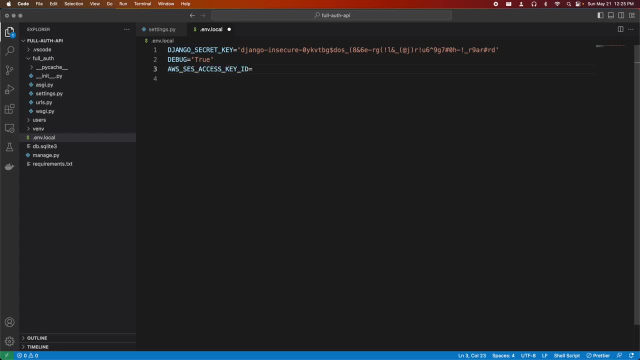 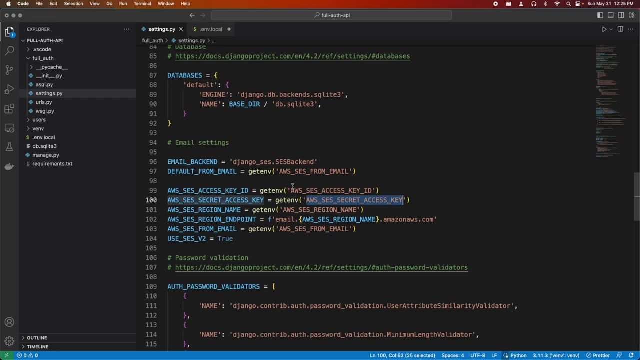 I'm going to have the access key, I'm going to have the secret access key, I'm going to have the region name And then region endpoint. we don't need to do. And then, finally, we have this AWS SCS from email. 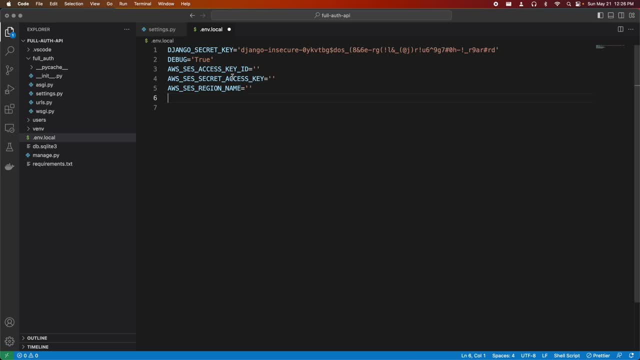 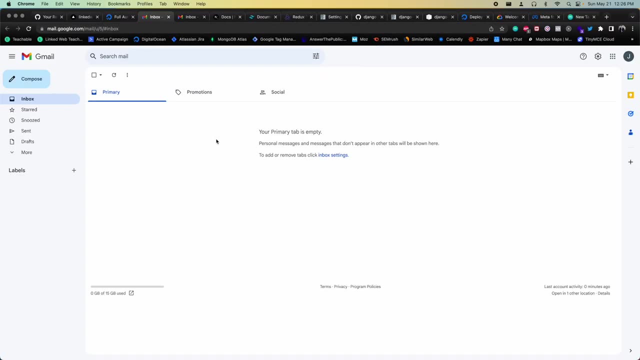 which both this setting and this setting will use. I'm going to copy that and paste it in here. All right, So now we have to set this up. So right now, I have two emails set up so that I can test things out in this project. So I have this general email, I have this regional email, I have this: 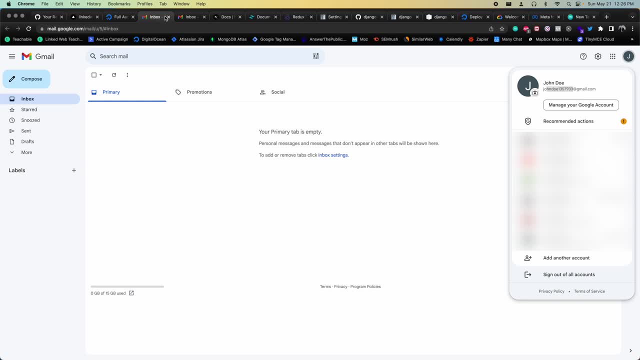 John Doe 1357933 email address. So this is going to be my sender email. Then I also have a receiver address And that's going to be this: John Doe 1357915 at gmailcom. So this is going to be using to register and log in with an account on my application. So the next thing I'm going to do, 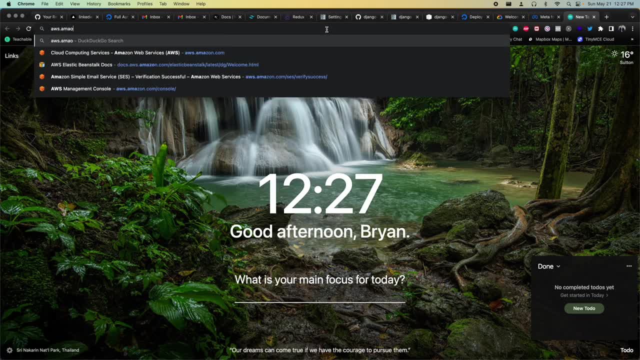 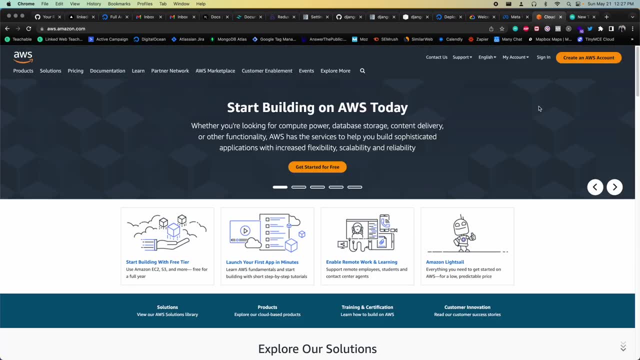 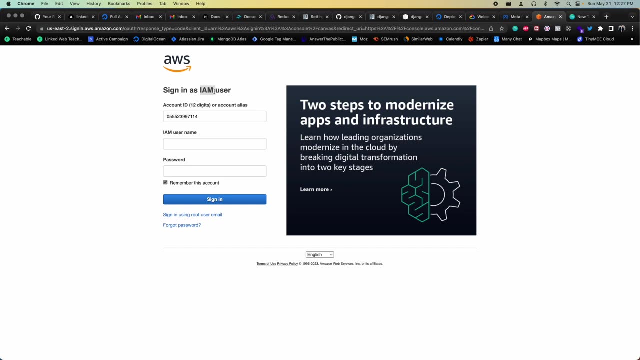 is, I'm going to go into awsamazoncom, So you will have to create an AWS account. if you don't have one, Then after that you can sign in. Now, in my particular case, I set up an IAM user and that's what I'm logging in with, So then I can put in the account ID. This is my account ID. 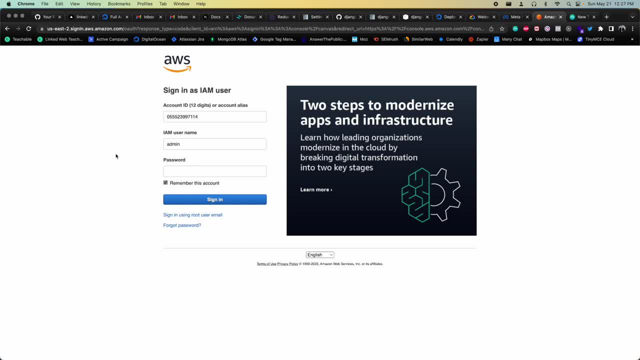 the IAM user I set up and the password. Now you can also log in with a root account. That's also perfectly fine And by default that's going to be your login screen And then, once you have your root user, you can set up an admin user. I'll also show that setup that I have. 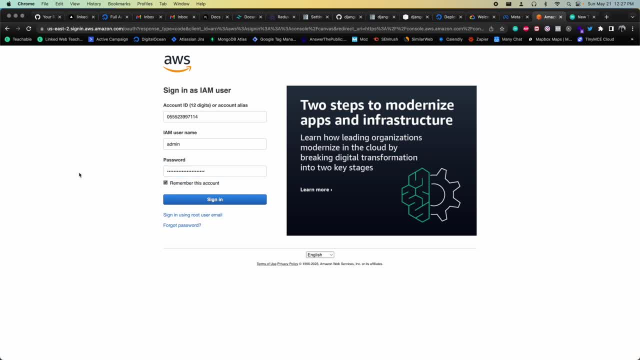 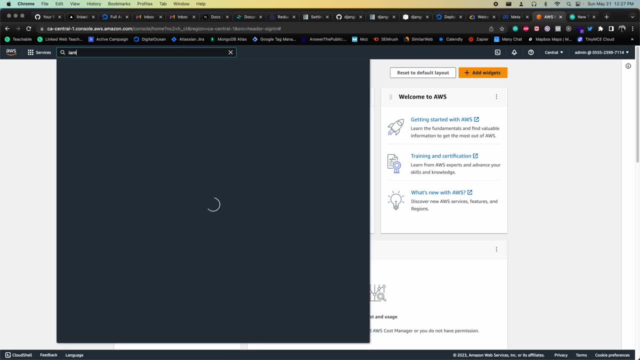 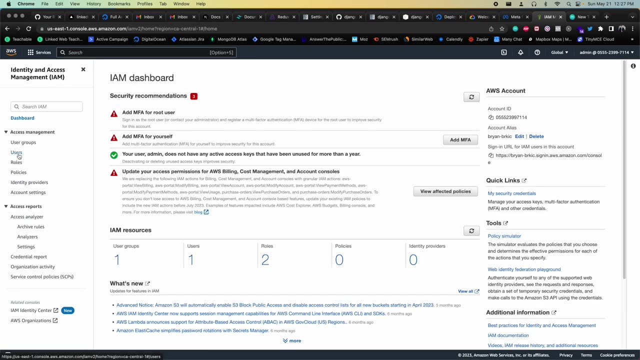 So for now, just because I have this IAM user, I'm going to log in with it instead of with the root, And then if you go into IAM, which you can also search for, so that's this service, So the setup that I have. so if you're logging in with a root user, 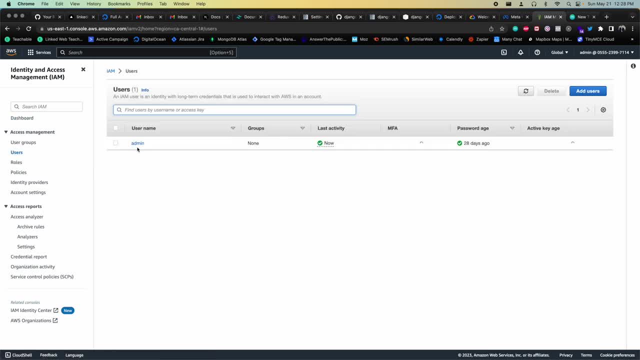 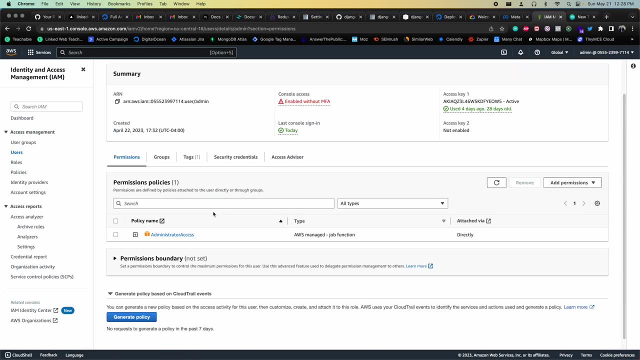 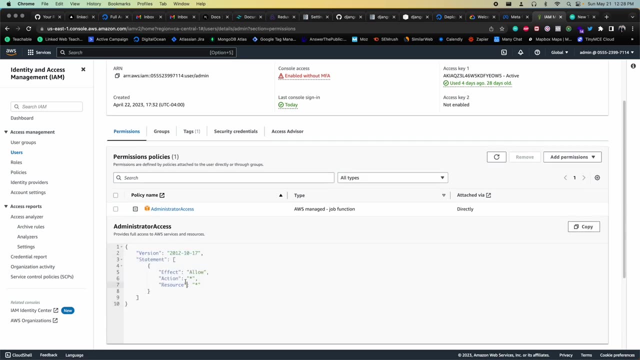 the way that you can do this is you just go under this users and then you can just add a user- and in my case I made a user with the username of admin- And then this thing has a policy of administrator access and this thing just gives me administrative access for this particular user. 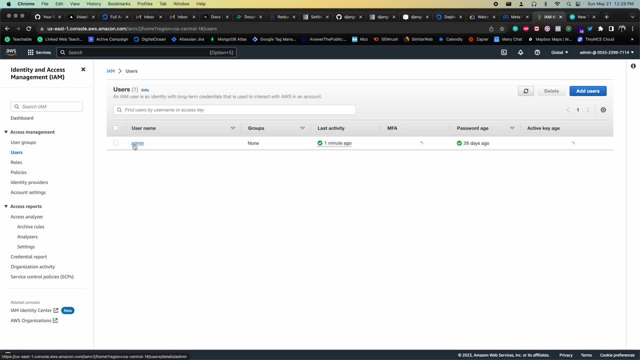 Now, in the case of this particular admin user, I attach permissions directly of the administrative access. Another thing you can do is you can also make user groups. So let's say I can have an admin's user group and then this thing here can have permissions of administrator access. 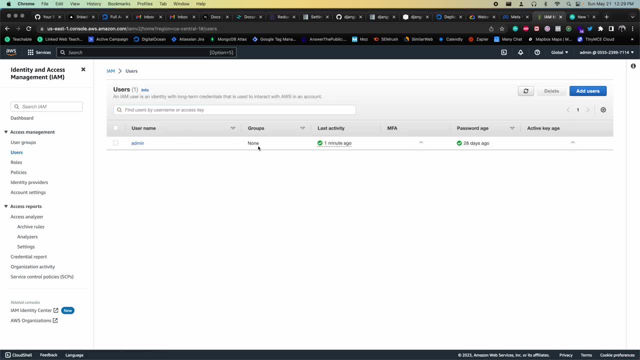 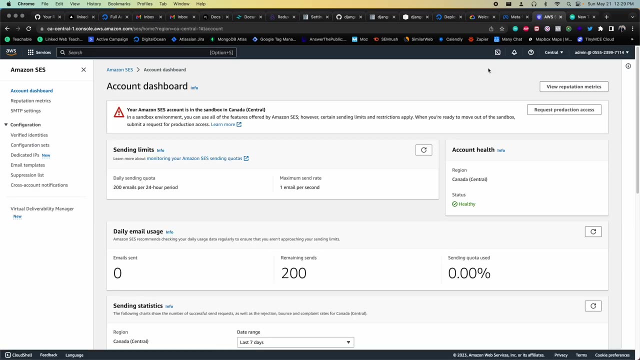 and then you can just have your user be part of the group. in this case, i just have them as none and he just has the permissions of administrative access. so that's that part. the next thing you have to do is go into ses, which is amazon simple email service, and then also you want to note the 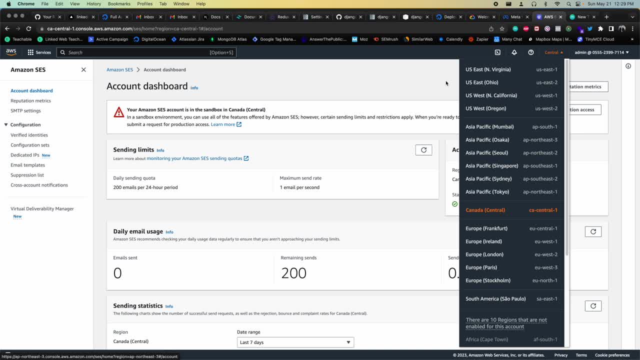 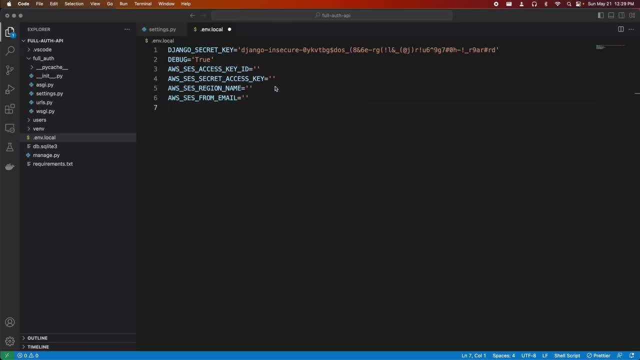 region. so right now i'm in ca central one, so that's my region. so what i'm going to do is i'm just going to copy that from the url, just so i don't make a typo. then, inside of the region name, i'm going to paste that in here: so ca central one, and then for the from email, that's going to be my. 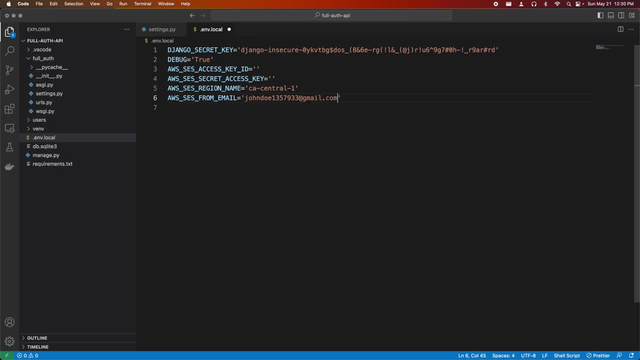 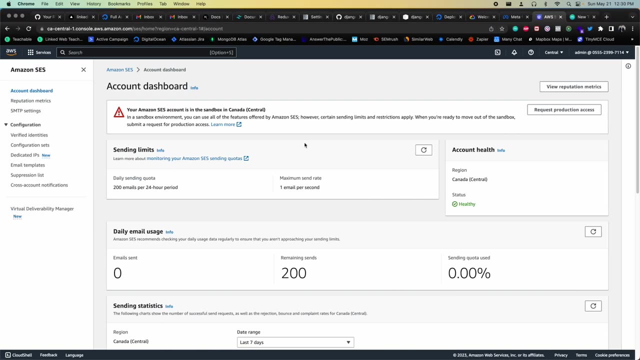 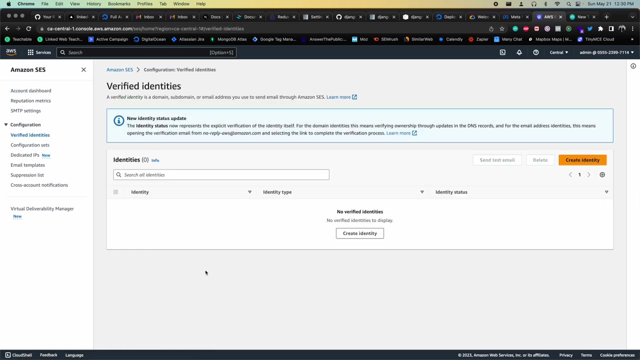 john doe: one, three, five, seven, nine three, three at gmailcom. so that's my sender email. now i need to set up these two things. so, inside of here, what you need to do is you need to go into verified identities and you need to verify both the sender and the receiver email. you can't just have the sender. you. 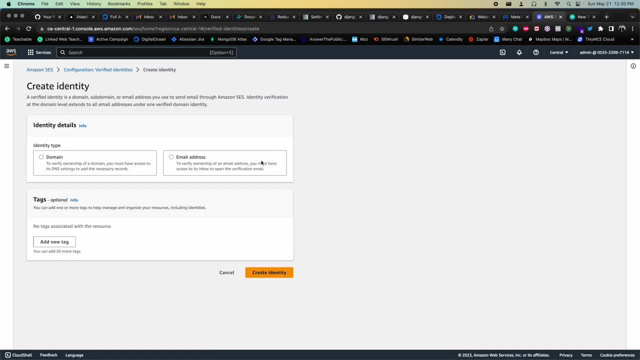 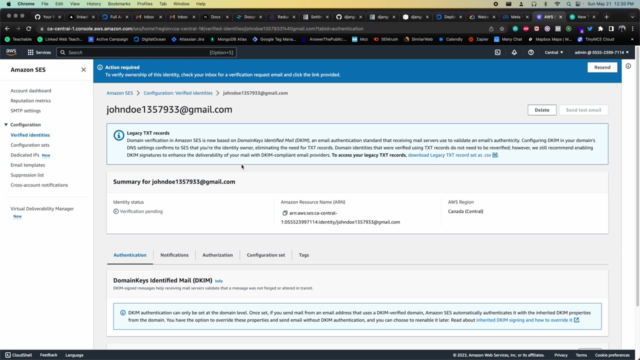 need both. so i'm just going to go to create identity email address. i'm going to put in john doe one, three, five, seven, nine, three, three at gmailcom and i can create that identity and i'm going to do that one more time. so back in here. so this right now. 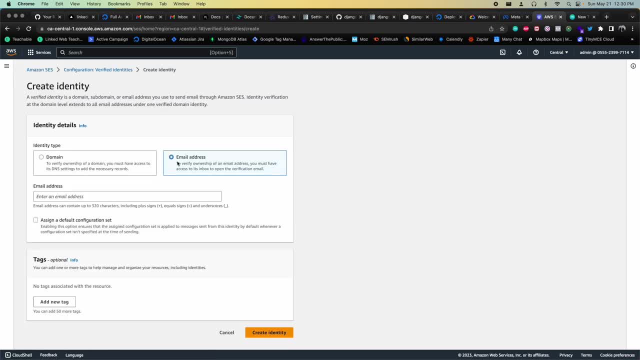 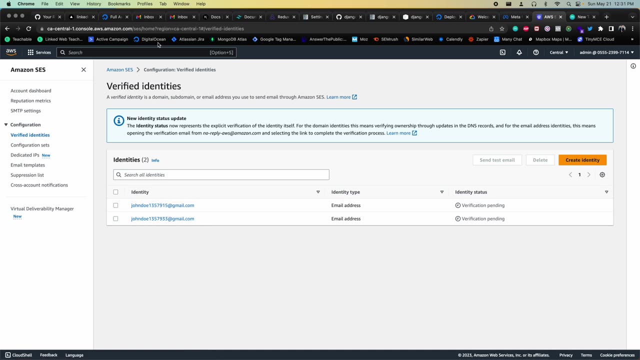 has verification pending. we're going to get to that. i'm going to create another email address and this is going to be my receiver email, so you need to include both, or this is not going to work. so right now, both of these are pending verification. so if i go into here, 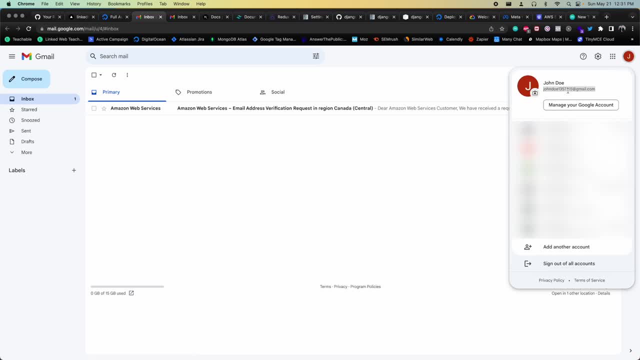 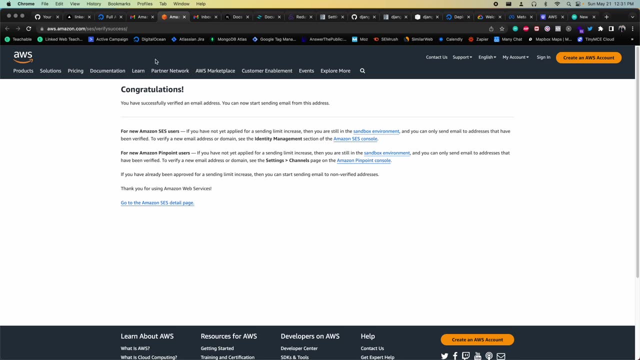 so this is my john doe one three, five seven nine one five email. so this got an email and that has a link which i can now click and there you go, verified, and i have to do the same thing with my other email address of john doe one, three five seven. 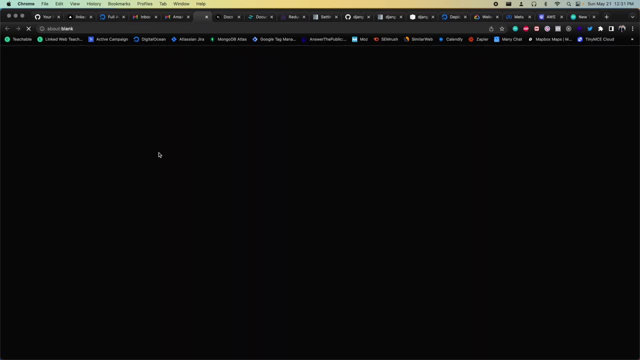 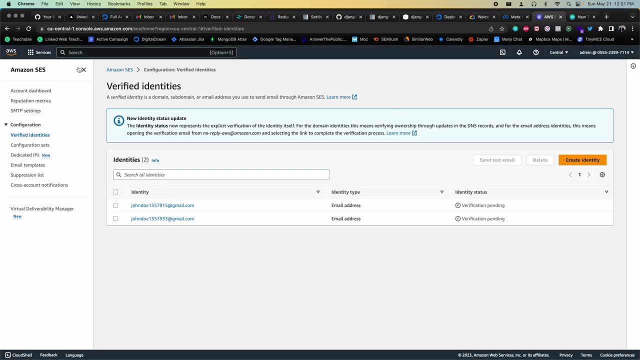 nine, three, three at gmailcom. so here's that link, click it to verify and there we go. that's all you got to do to verify. so back in my aws console. if i refresh, they should now both be verified. beautiful. so the next thing you have to do is go into my smtp settings and create smtp. 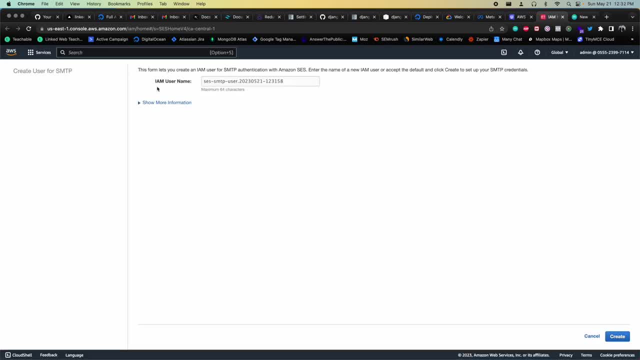 credentials. so i'm going to go ahead and do that. so we have iam username. we can show more information if we want. so this is some stuff it has configured so i can just create this user and this user it's going to have credentials which i'm going to be using and it's going to be responsible for sending. 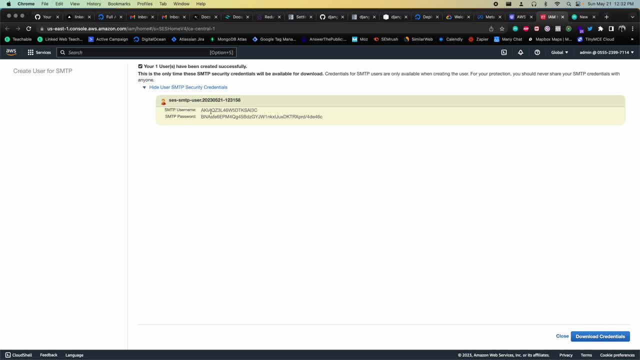 these emails. so now i can show these credentials. now. one thing that i found is, whenever you create this for some reason, the credentials it gives you off the top of your email is going to be a lot more than the credentials it gives you off the back. don't work and have to recreate them. 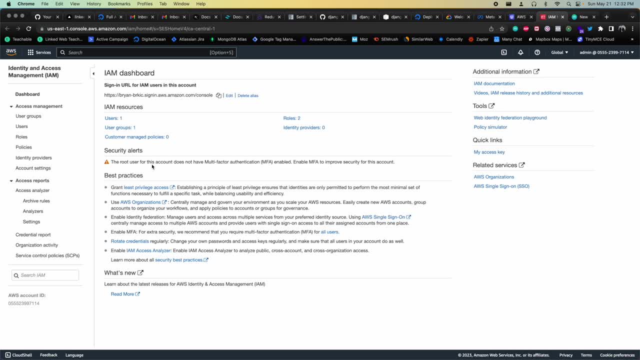 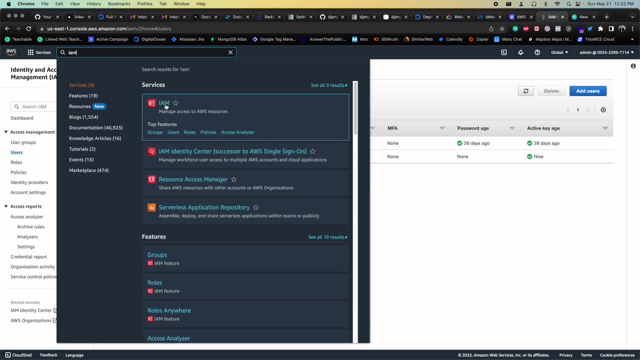 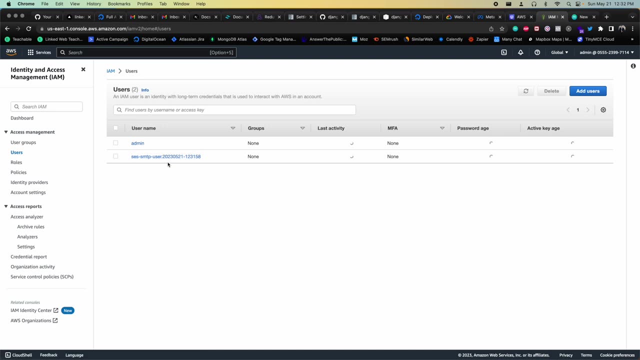 so i'm just going to close and i'm going to go through that process just to make sure that it works. so under now i am users, so we are now in i am. so right now we have this user created, so i'm going to click on this user. go to security credentials. 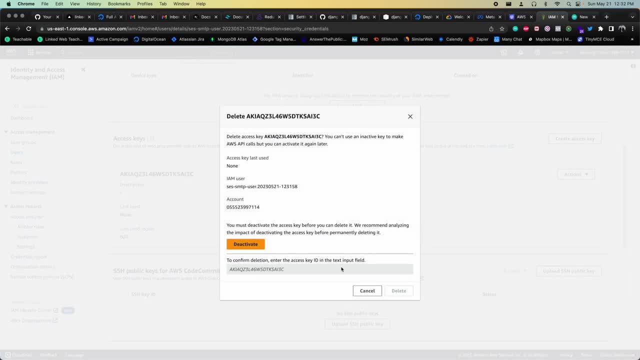 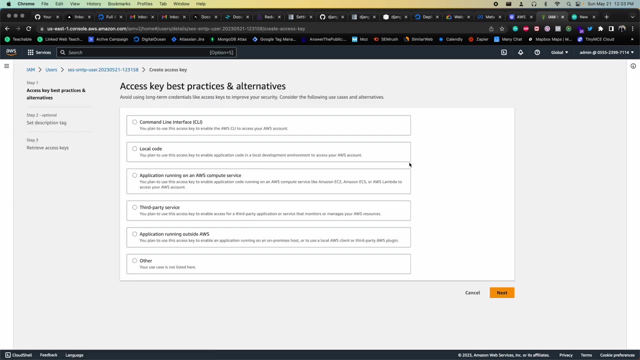 and i'm just going to remove the credentials it has right now, and then you have to deactivate the key before you can delete it. so i'll deactivate, paste this in and delete, and i'm going to create a new access key. so it's going to be for local code and you have to check this thing. 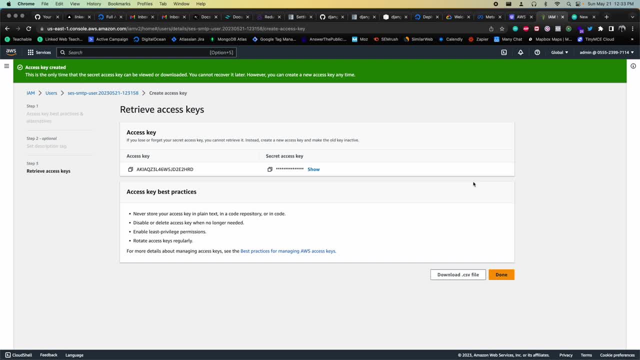 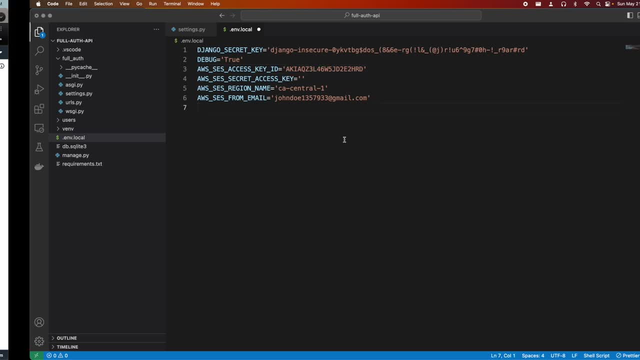 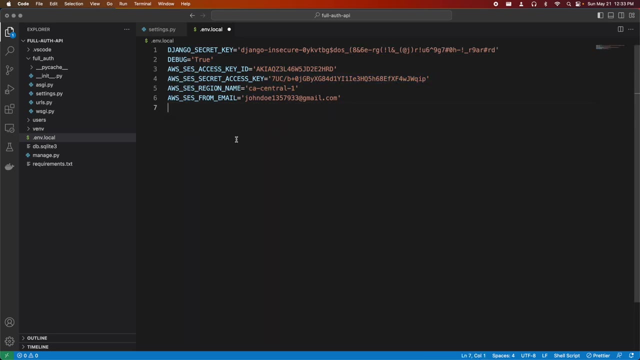 and then you can set up tags. i'm not going to do that, i'm just going to create the access key and i can grab these values so i can put the access key here, go back here, copy this and paste in my secret key. so i have both of these set up. so now i have all of my settings so that emails work. 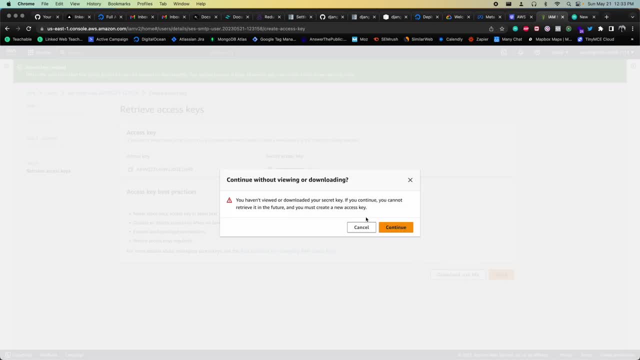 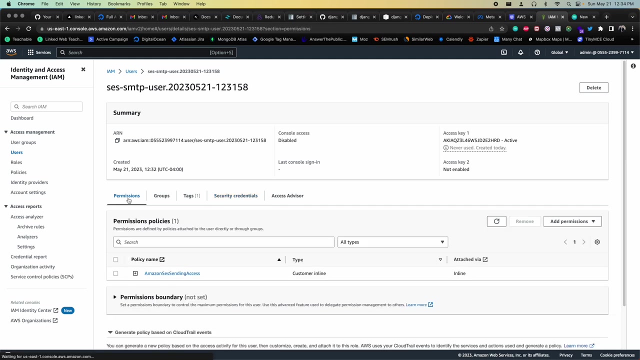 and now i'm just going to click on done and continue. so i already have the secret key copied. so if you click continue, you won't be able to see this anymore. so make sure that you set up those environment variables, otherwise you have to recreate these. so there we are, and then the next thing i'm going to have to do: 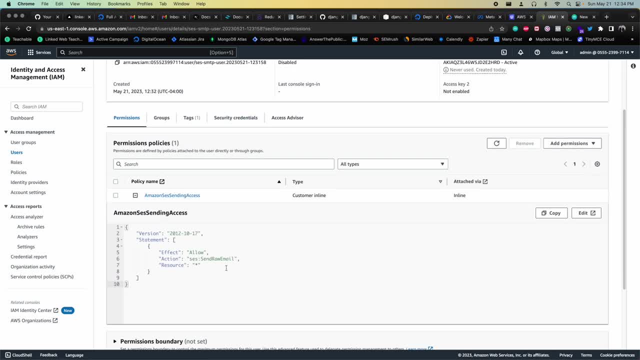 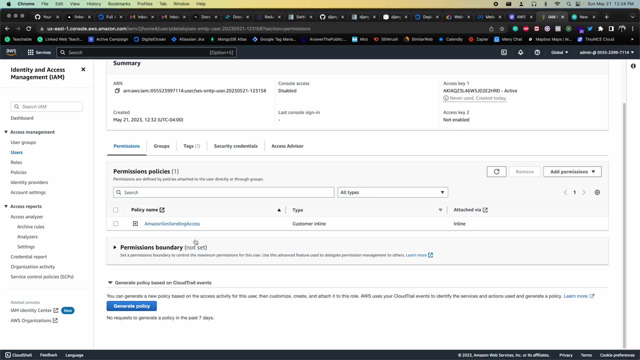 as well is going to permissions. so right now we have this permission of amazon ses sending access, which just gives you an allow action of ses send raw email. but i will need another permission to have sending emails work. so i'm just going to do that. now i'm going to go add permissions and then i'm going to use attach. policies directly. i'm just going to sort them out among the free classics. you can just drop all of them into one place and then go to policies, and you can also set them directly to accessories. so i'm just going to sort them into expresses and i'm 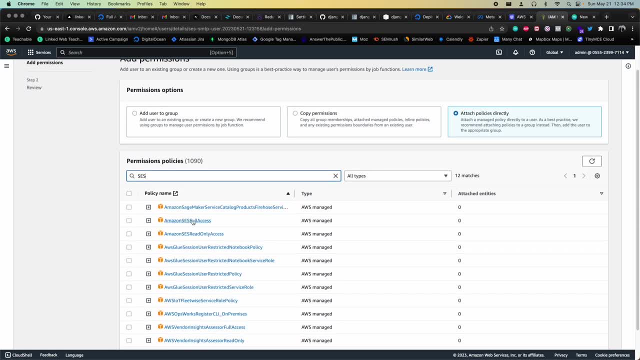 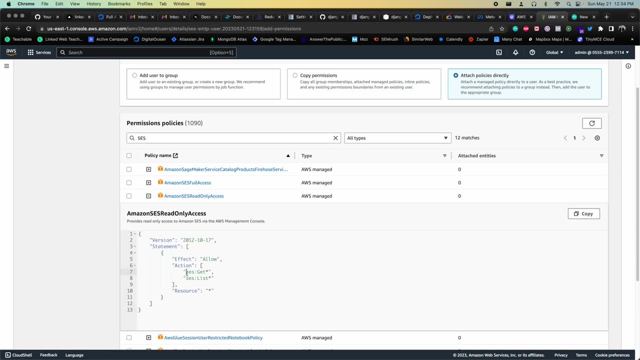 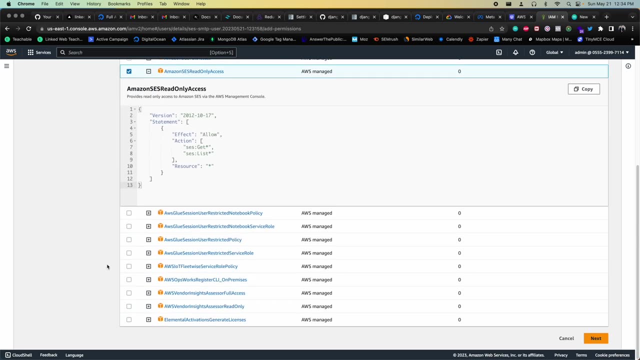 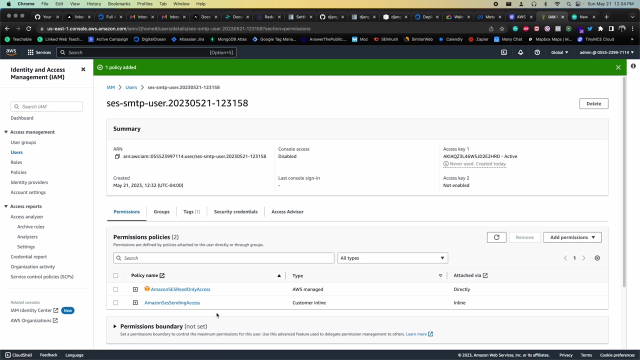 search for SES. Now, I don't need SES full access. What I do need is- I think it's yeah, read only access, because I do need this get access, and that I get with this policy. So I'm just going to attach that one, So click next add permissions, And now we have this as well. So with that, 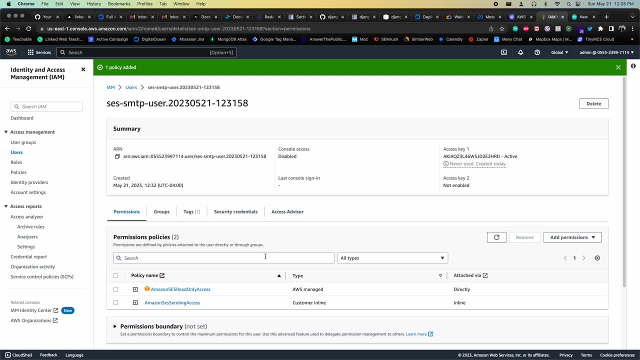 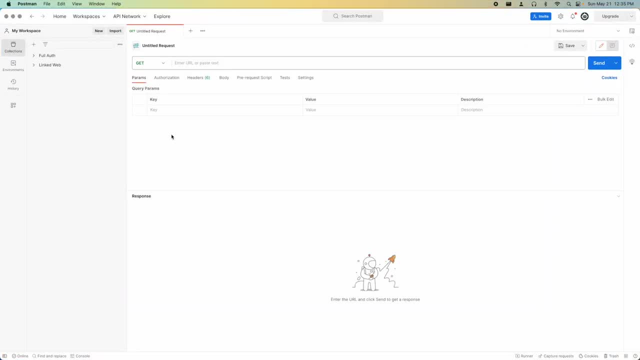 we are now all set up with SES, So now we can test out our backend API. So I'm going to now open up Postman once again and let's test these endpoints out. So the first thing I would want to do is create a user. So let's actually also make sure that our server is running So it is, And 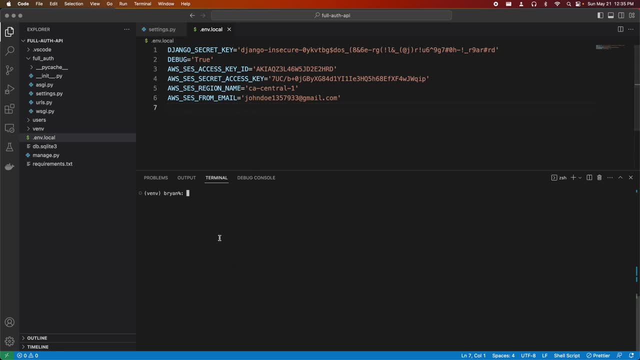 actually I'm going to restart the server just because I added these environment variables. So I want to make sure it picks that up. So I'm going to rerun And then I can also just close this stuff up. And now let's take a look at the endpoints that. 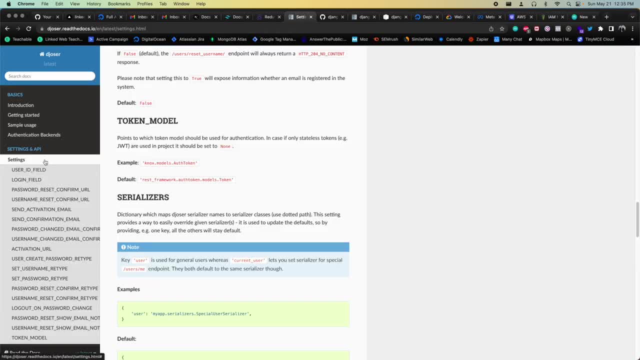 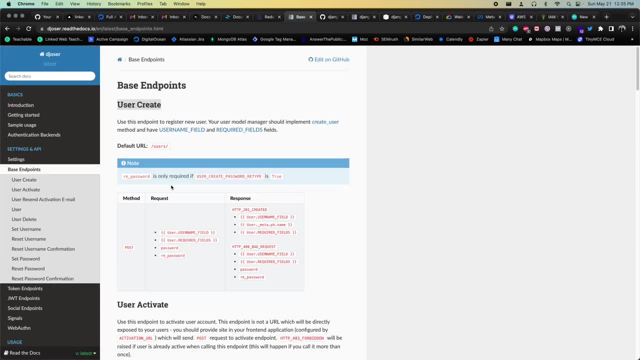 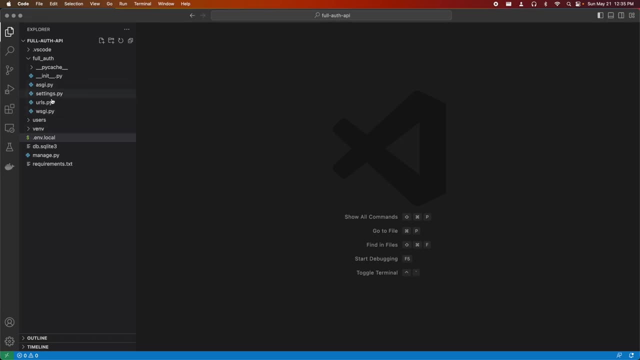 we have. So back inside of my Joeser settings- or I guess inside of the documentation, can go to base endpoints, And here is our user create endpoint. So we're going to be hitting this endpoint here Now. in particular, when we set up our URLs, we prefix this with APIs. 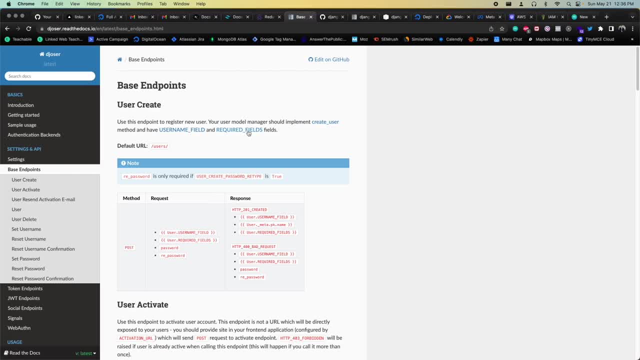 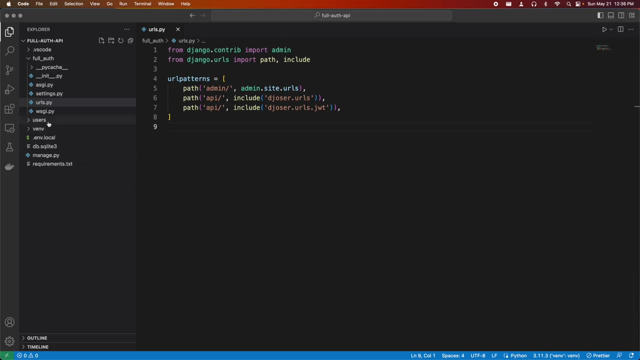 slash. So our endpoint we're going to be hitting is lochost 8000, slash API, slash users and then slash. So make sure to have that trailing slash there. That is important. Then these are the things we have to put in here: the username field, required fields. So we define those in our custom. 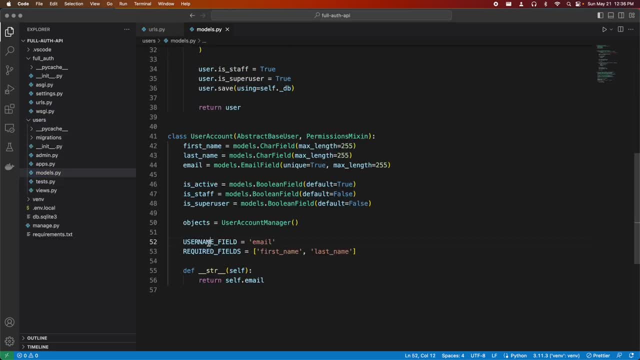 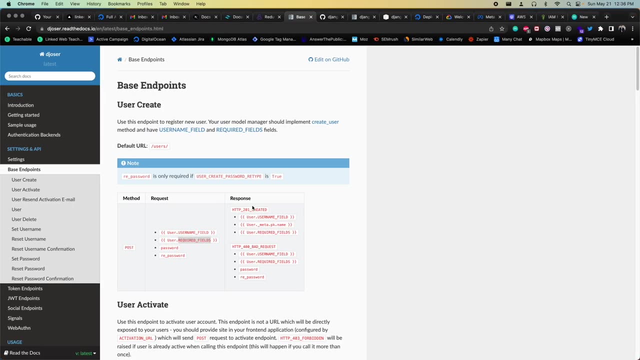 user model. So we have username field, that's email required fields- first name, last name And then, if we get 8201, created, this worked or 100 bad request means this didn't work, So let's try this out. 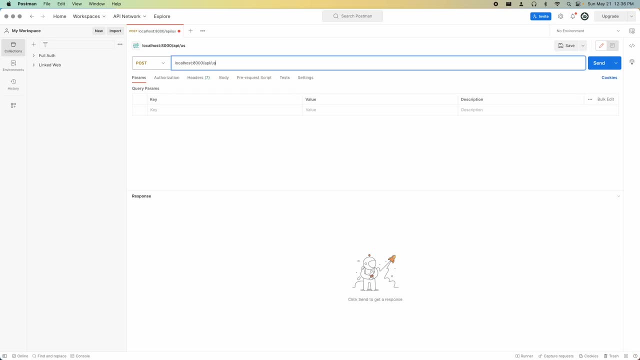 So lochost 8000, slash API, slash users, slash. So again, make sure to have that trailing slash there. We're going to have content, type of application: slash JSON, And then I'm going to send some raw data, So I'm going to have first name. 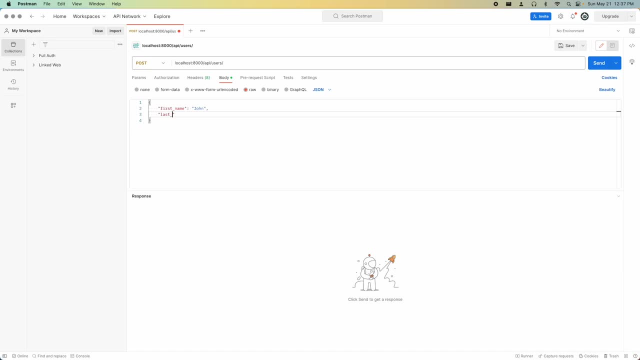 which will be John last name. This will be Doe the email. This will be my John Doe 1357915 email. So this is my receiver email. I'm going to have password and I'll do my secure password, And then I also need the repassword. 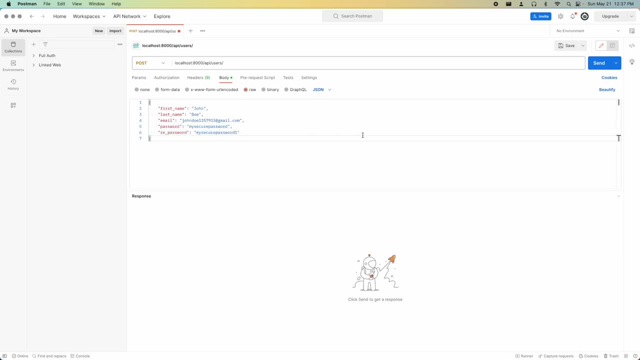 So let's test out what happens if these don't match real quick. Two password fields didn't match, So that means we set things up correctly to have these two get compared. I'm going to get rid of that. I'm going to click on send. 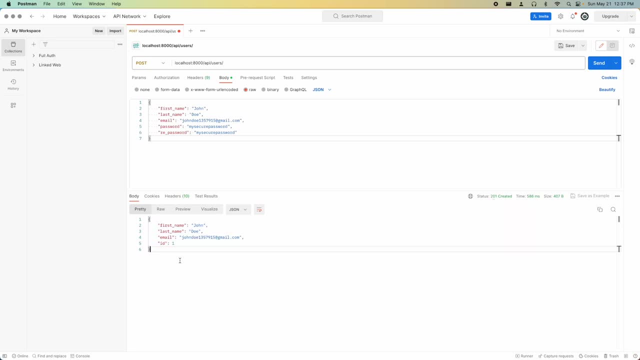 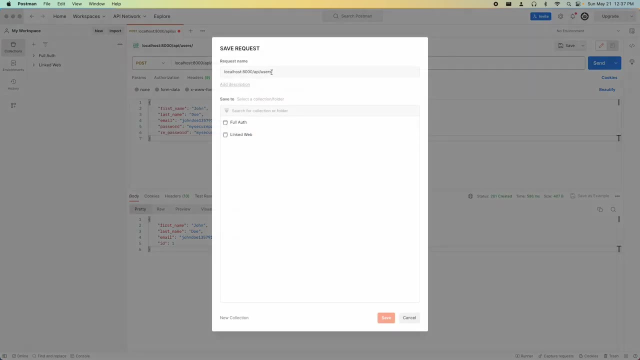 And there we go. We got a 201 created and we get back our data, So first name, last name, email and the ID of the user. So perfect, I'm going to save this now. This will be my create. 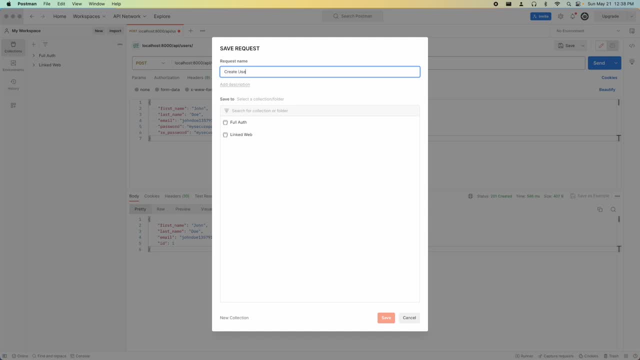 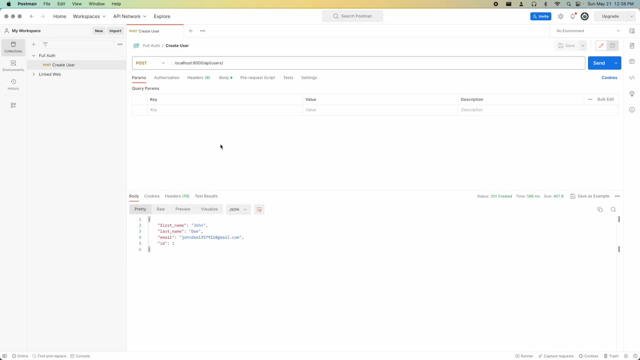 user, And I'm going to save that in full auth. So now the next thing I'm going to do is test out logging in, which should fail right now because our account isn't activated. So I want to test that behavior. So that endpoint is going. 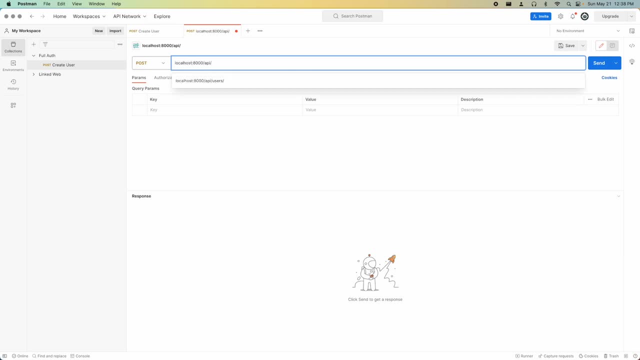 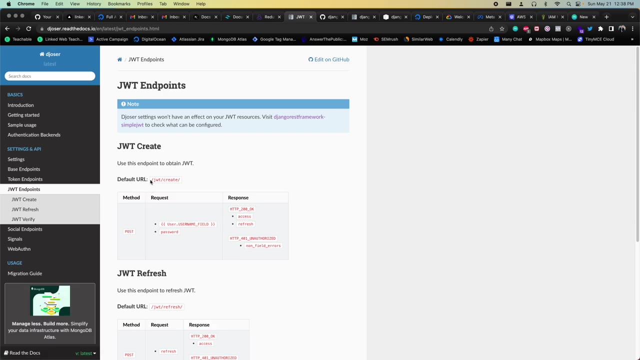 to be localhost8000,. slash, API, slash, JWT, slash, create slash. Now you can also go into the JWT endpoints and you can also go into the JWT endpoints. and you can also go into the JWT endpoints and you will see these endpoints here. So we need to pass the username field, which is our email. 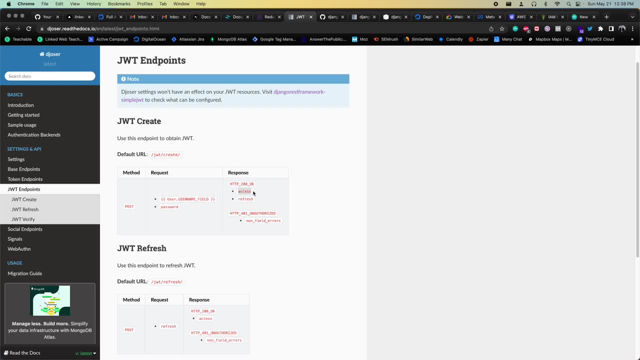 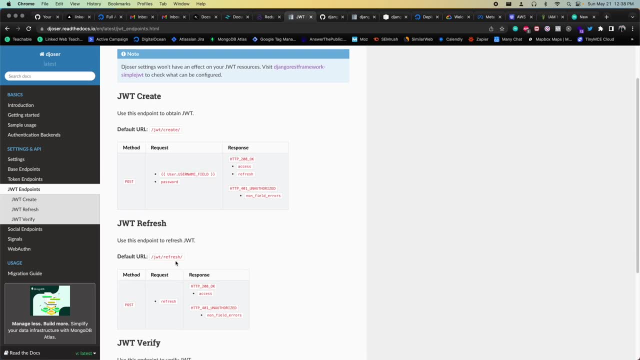 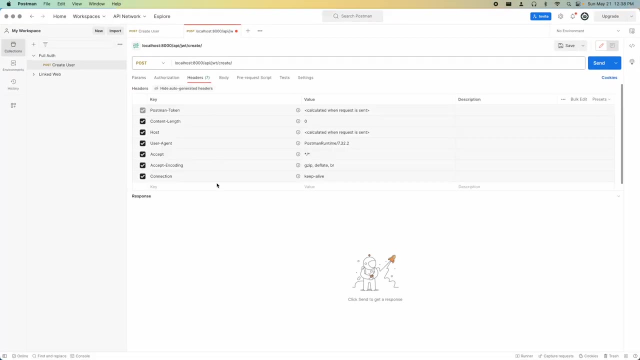 and the password and a 200 OK with an access refresh token means things worked. A 401- unauthorized means things did not work. And then we're also going to be testing out this refresh endpoint and this verify endpoint as well, So let's go ahead and put in our content type. 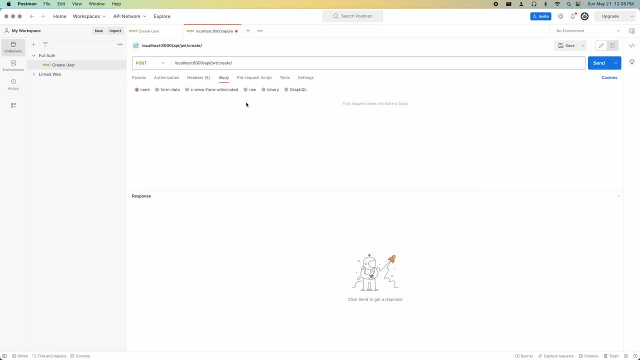 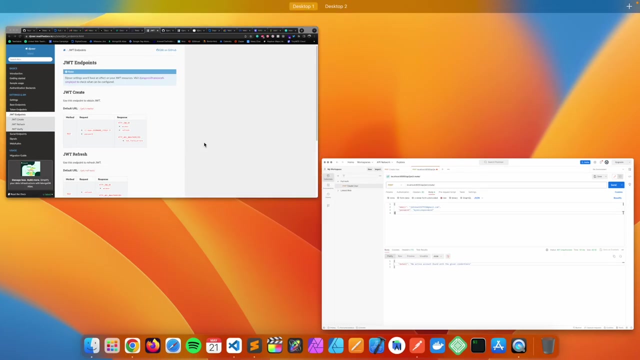 of application JSON and my body, And then we'll have the email and the password, which is my secure password. So let's send this. So no active account found with the given credentials. So that's what I expected. So now we have to go through the 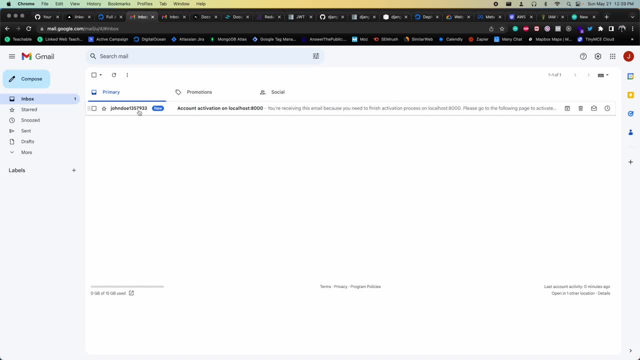 activation process. So back in here. we received that email successfully, So that's really good. Now another thing that we're going to notice is here we have the localhost8000 team and we also have this domain being used here. Now, these are things we're going to want to customize, So, in particular, 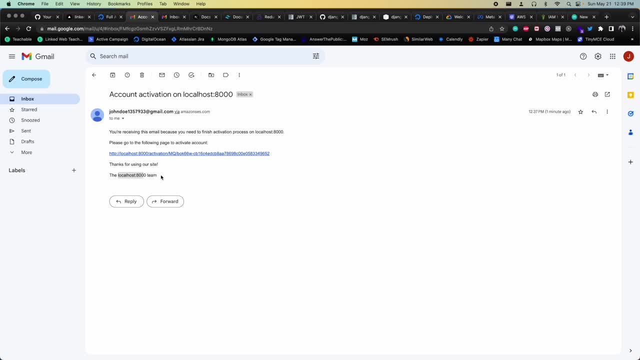 here I want to have something like the my full auth team or something like that. And then here I'm going to want localhost 3000 instead of 8000, because my front end application is going to end up running on localhost 3000.. And also, when we're in production, we're going 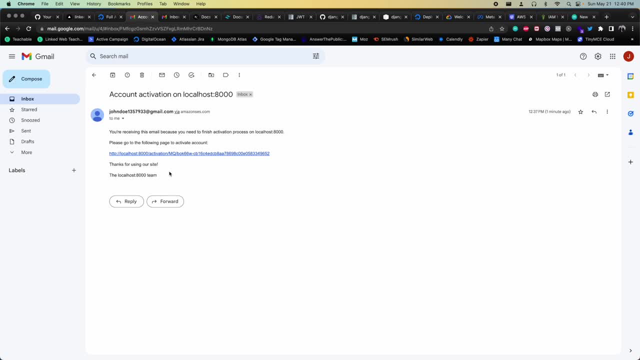 to have our API on a subdomain of apithedomaincom And then the front end Nextjs project is going to just be on the domaincom. So when I get this link in production, I also don't want it to be like apimydomaincom. 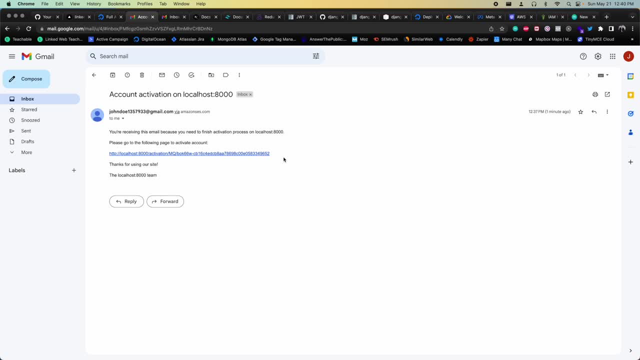 slash this activation link. So that's something we're going to edit, But before we do that, I'm just going to copy this. Actually, I'm going to copy this part here because we have the UID and the token. I'm going to want those values in order to activate the account And 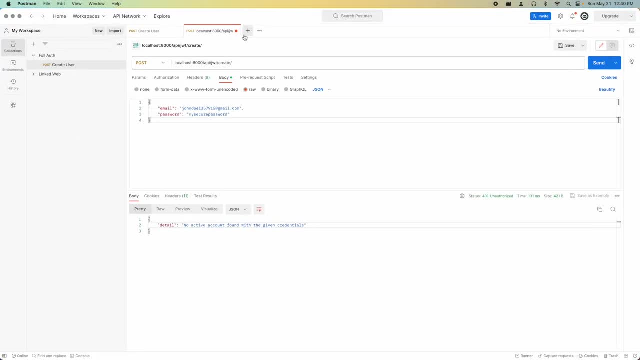 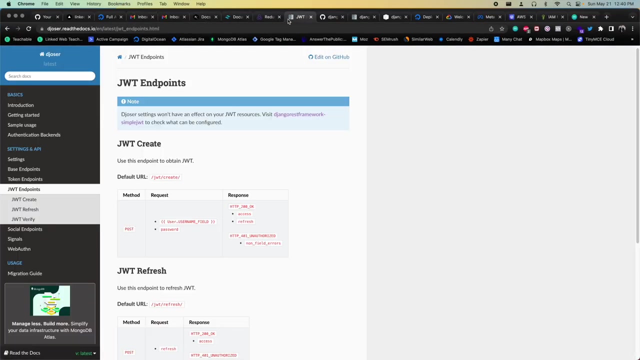 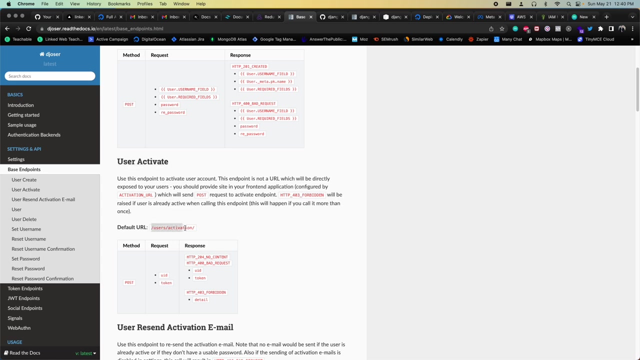 count. So back inside here we're going to do localhost 8000 slash, API slash. It's also going to be a post request And let's take a look at the endpoint we have to hit. So back in the jostr settings I'm going to go to base endpoints And here we have user activate, So this will be. 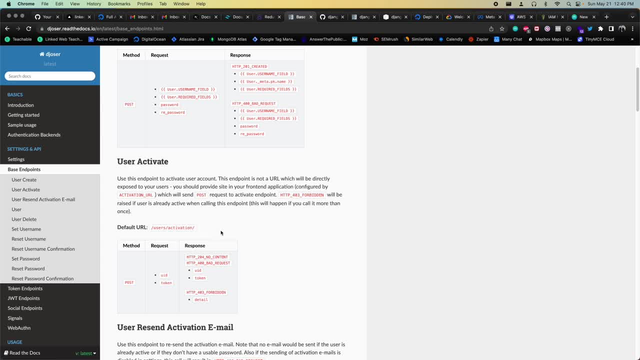 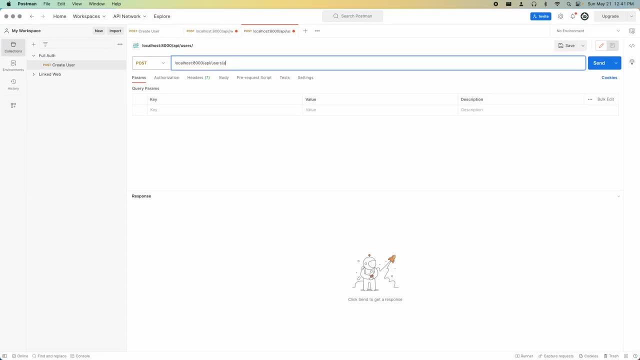 users slash, activation slash with the trailing slash And we're going to put in the UID and the token in a post request. So 204. no content means this worked. Anything else means it failed. So users slash activation slash. So content type will be application JSON And in the body we're going to have 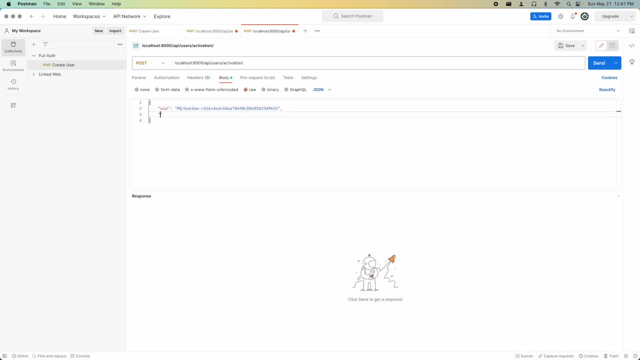 the UID. So I'm just going to paste this whole thing and the token. So the token is this part after the slash. So we're going to cut this and delete that slash put in the token, and this should be good. So now what I'm going to do is I'm just going to add an extra character just to test. 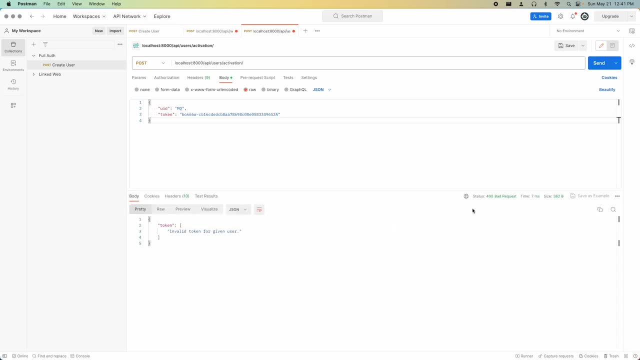 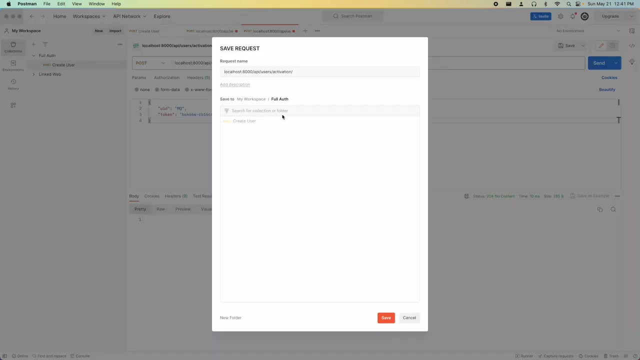 out that this works. So there we go. We got the 400 bad request because the token was incorrect, So now, if I get rid of that additional character, this should not work. I'm going to send this. There we go. 204- no content. So the activation succeeded, So I'm going to save this. This will. 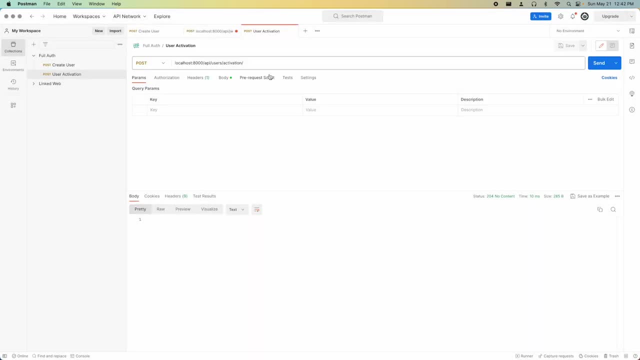 be user activation And now this should work. So I'm going to try the JWT create once again. And now we get the access and the refresh token in the response body. It's perfect. So we tested out those endpoints. Now let's test out the other JWT endpoints. 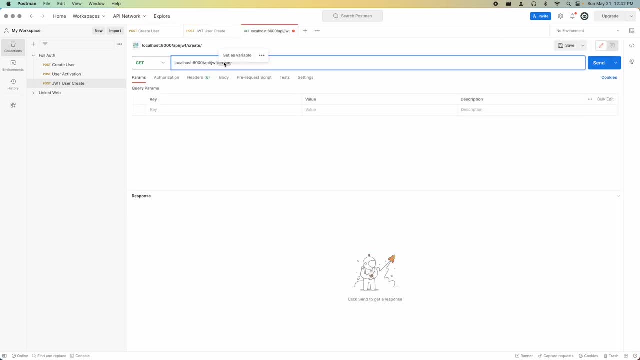 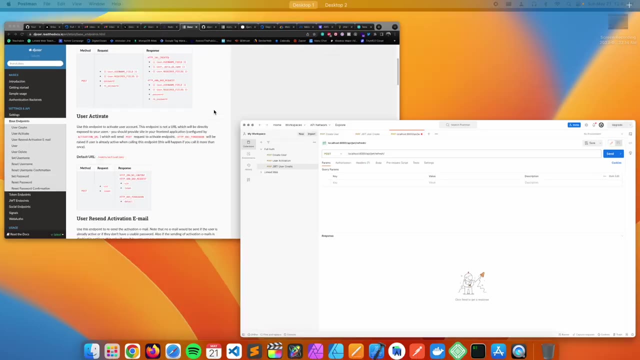 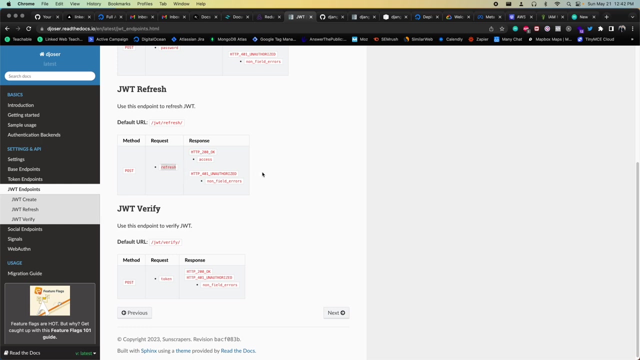 I'm going to copy this paste. So we're going to have our refresh endpoint- That would be a post request, And if we go into our JWT endpoints, the refresh will just expect in the request the refresh token and the response will be a 200. okay with the access token. 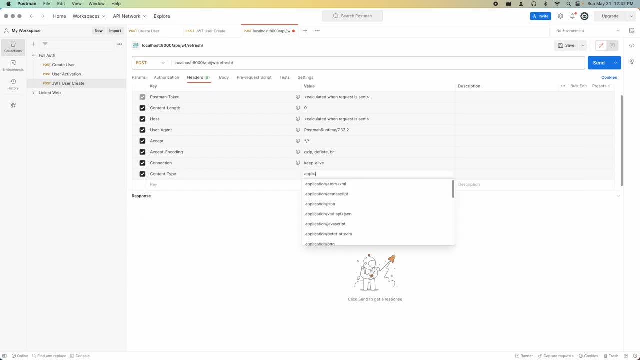 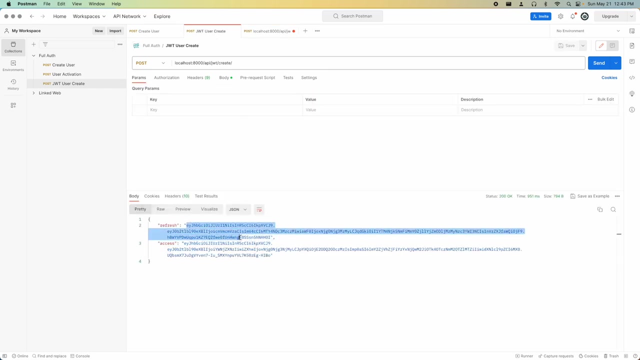 So let's put in the content type of application: json. I'm gonna pass raw data with refresh And that will be the refresh token. So here in the response we've got that refresh token. We're going to copy that. Go back here. 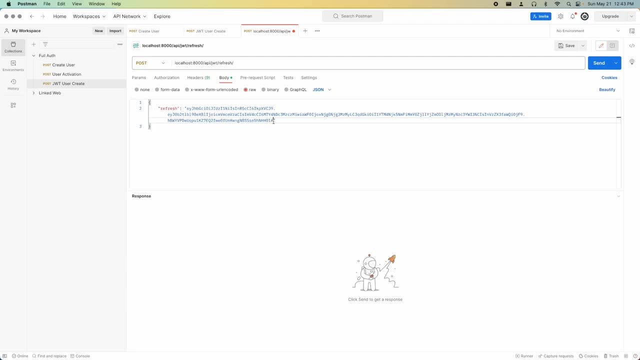 I'm gonna paste it. I'm going to add an extra character just to test the non-working behavior. 204. So that would be 100 accept訂. there we go. token is invalid or expired. now, if I get rid of that, it should now. 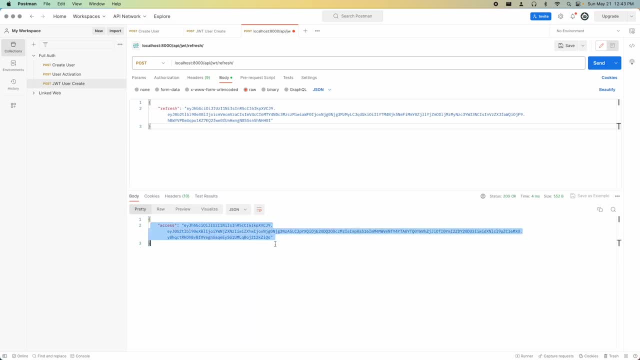 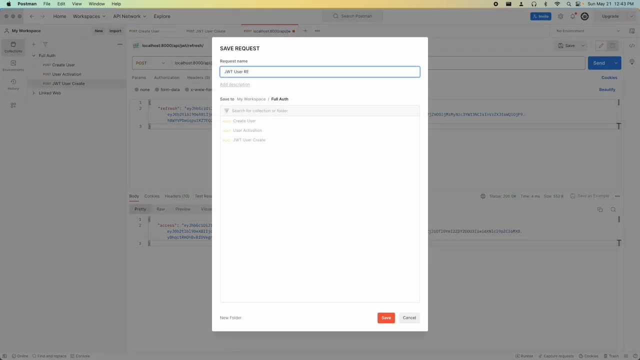 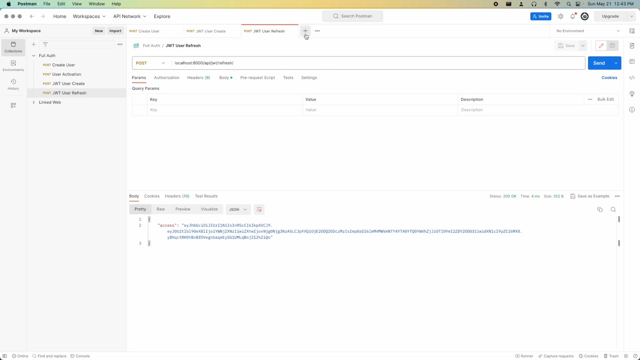 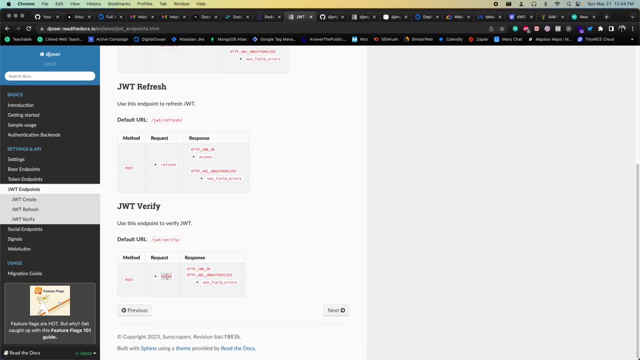 work. there we go 200. okay, with the access token, I'm gonna save this. there we are. and the last JWT endpoint I will test is the verify endpoint. this will be a post request to API, JWT verify and then here and have content type, application JSON, then ask for the data. what we have to pass is token and this token will be the access token. 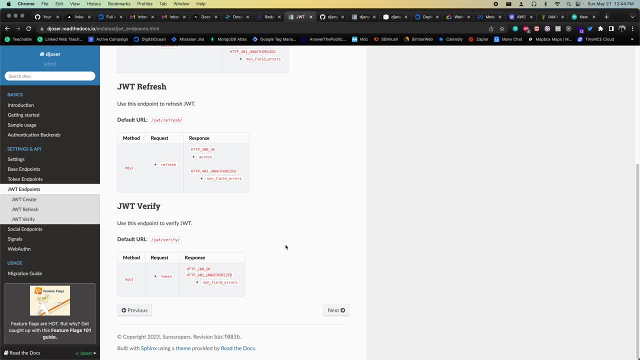 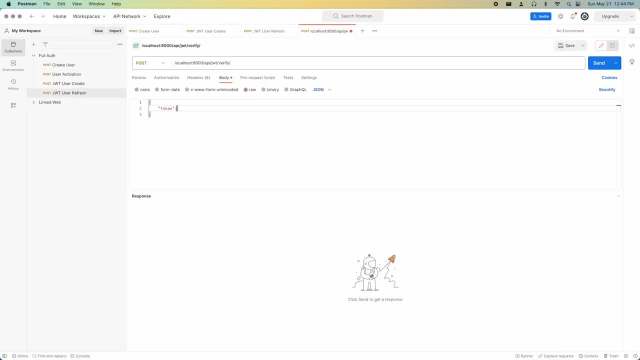 everything works: 200, okay. otherwise, 401, unauthorized. so let's try this out. so we're going to have token, so this will be the access token. so I'm going to copy my access token, go back here and paste it. I'm going to put an extra character just to test out the non-functioning. 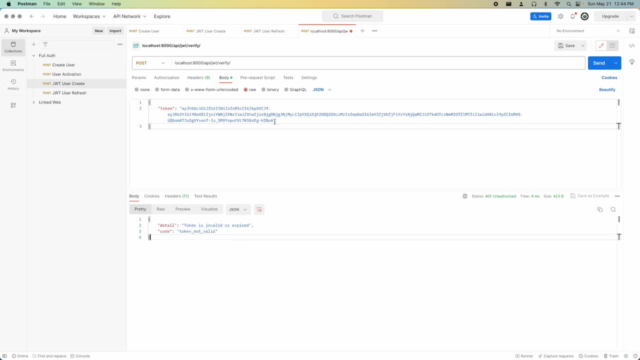 behavior. there we go. token invalid or expired, if I get rid of the extra character send. there we go now. if it's been over five minutes, then yours might have just gotten as invalid, so so, if that's the case, just hit this endpoint one more time, grab a new access token and then. 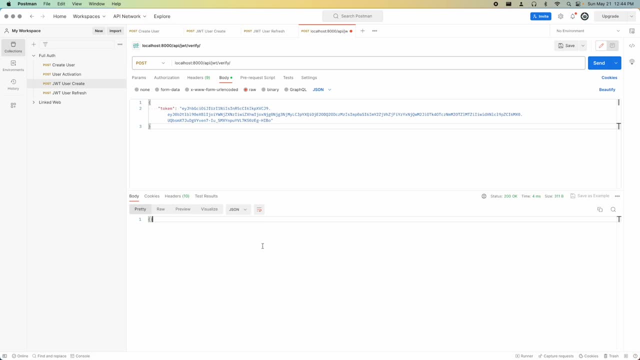 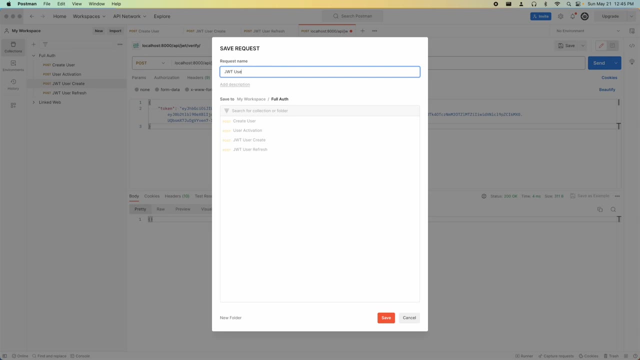 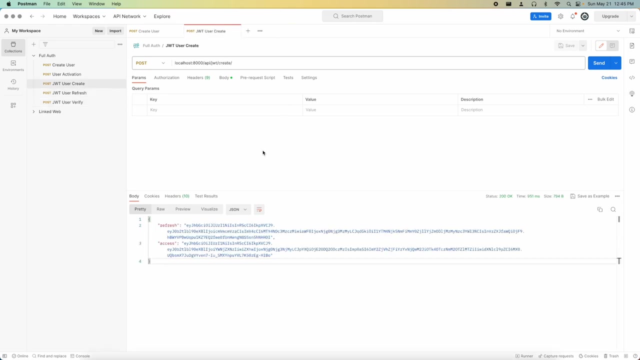 you can test out the verify endpoint because, remember, by default access tokens expire after five minutes. I'm going to save that JWT user verify so I'm going to close these up. so now, going back the other base endpoints we want to test. so we did user activate. 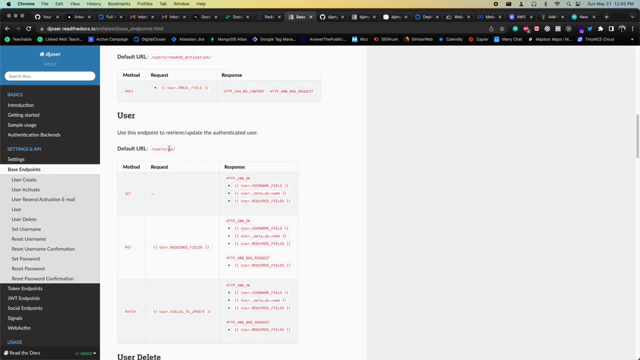 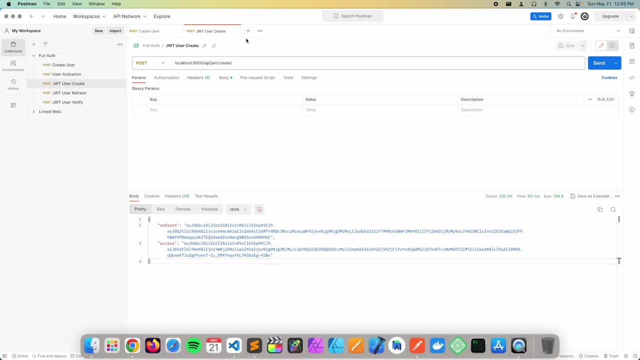 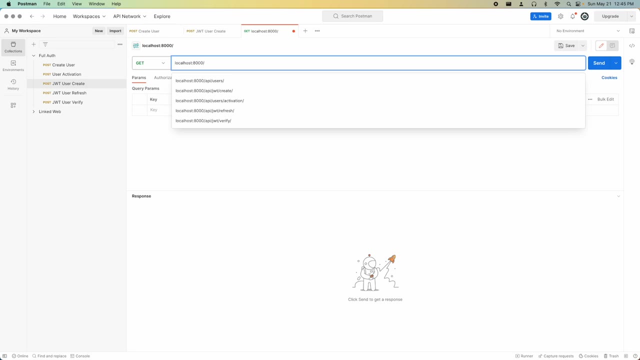 now we also have retrieving a user, so it's going to be users slash me slash. so localhost 8000 slash API slash- user slash me slash. this will get the current user and this is an authorized route. so if I were to send this as is, it's not going to work. 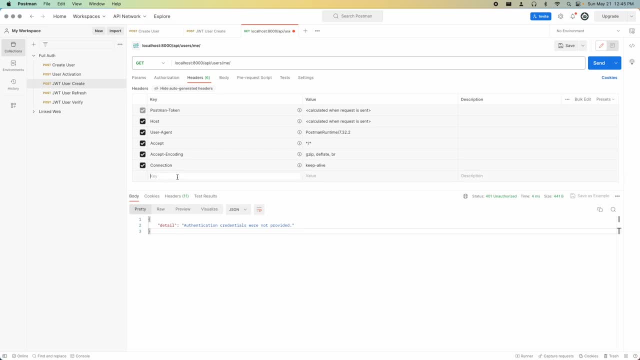 I need the authorization header. that's by default how this works. you're going to have authorization, then you're going to have bear. so that's the auth header type and then the access token. so I can copy the access token and I can paste it after bear. so bear space access token. 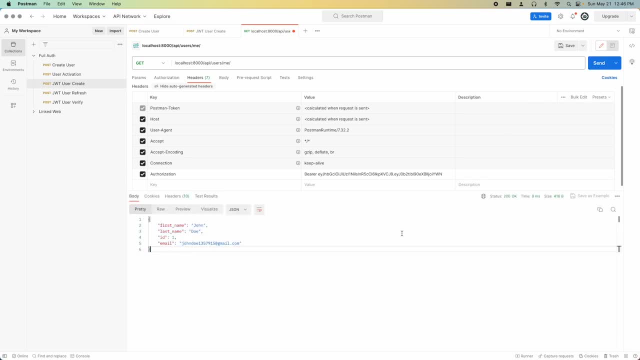 send this. you should now get back the user with the 200. okay, now this behavior with passing the authorization header. this is something I'm going to overwrite for now, just testing out the default behavior, but we will come back to this that we're not going to need. 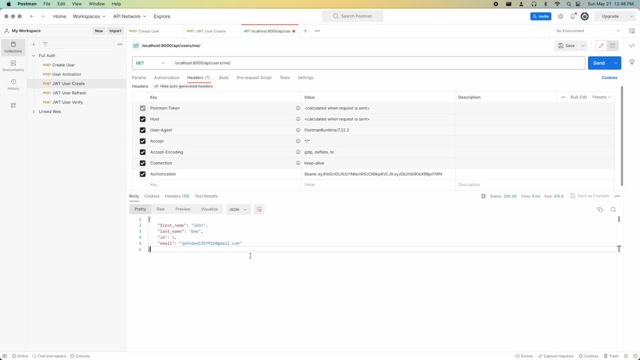 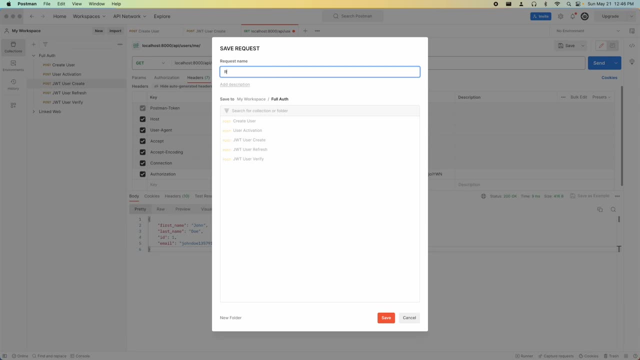 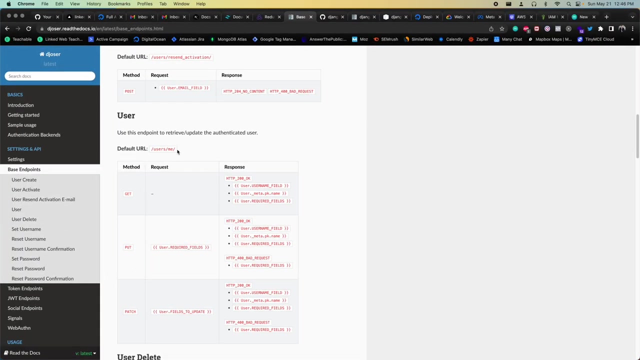 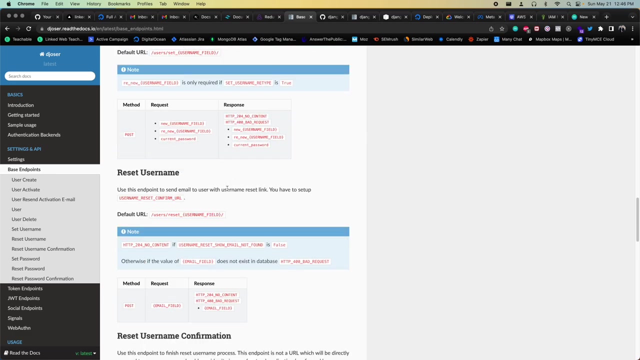 an authorization header. instead we're going to have HTTP only cookies which are going to have our access and refresh tokens. so we'll get to that a little bit later. I'm going to save this as retrieve user and then next I've got to use root delete. I'm not going to test that one. we have set username. set reset username. 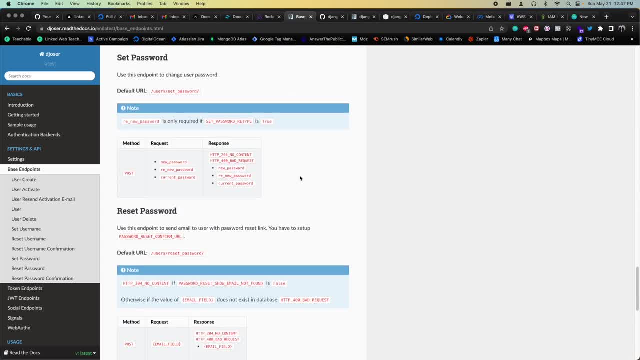 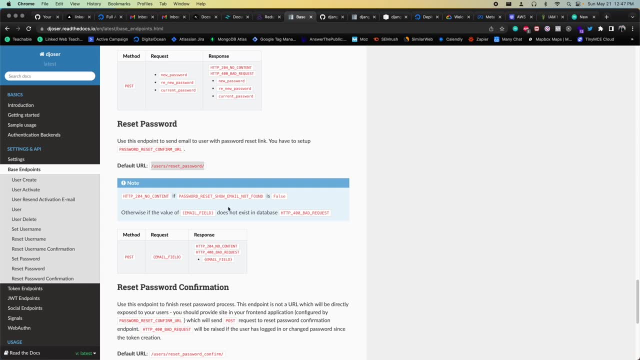 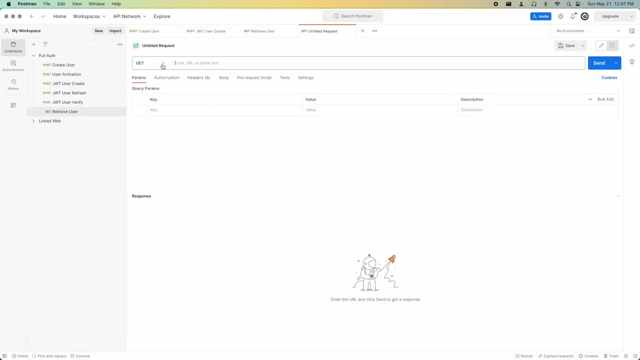 so all these I'm going to skip. same with set password. so I want to test out reset password. so this one's going to be this endpoint. it's going to be a post request where we pass in the email field: so post request, localhost8000. I'm going to have content type: application JSON. then in the body, I'm just going to. 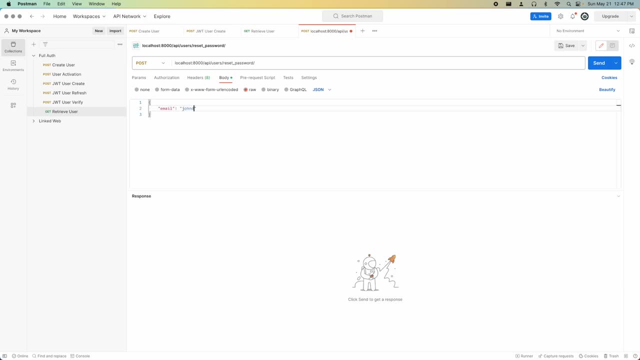 have email and I'm going to have John Doe 1-3-5-7-9-1-5 at gmailcom. And actually, before I do this, what I'm going to do is I'm going to edit the template settings. 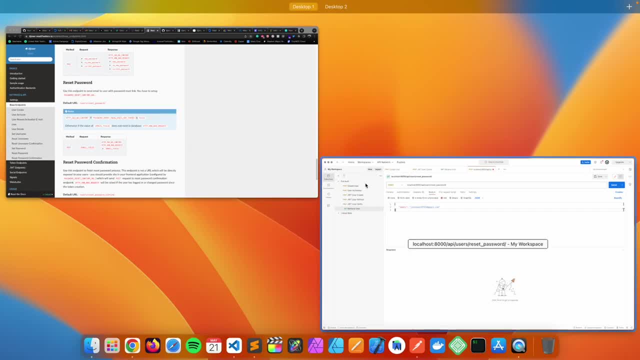 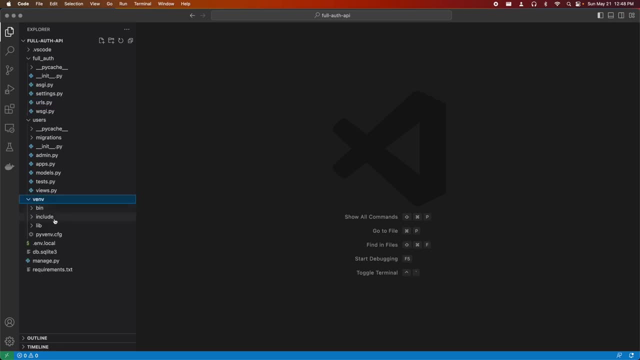 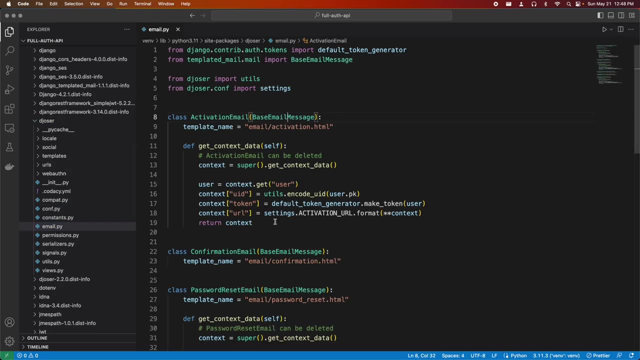 just because that was the one thing I was mentioning before. So I'm going to have to go back to my code And then, in particular, if let's say we go into Joeser. So previously we were looking at this email and we had things like activation email. 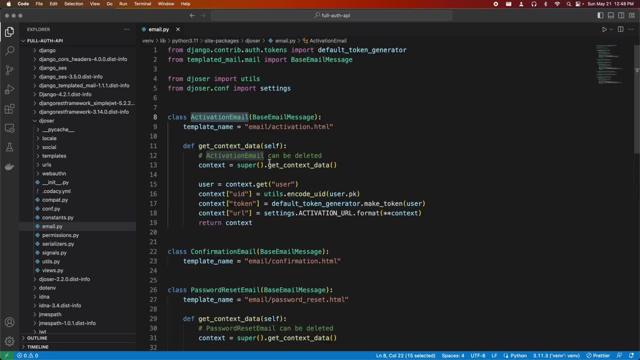 Then we also have other things like password. We set email And these things use these templates. So these templates we can find here. We have templates, email, and all of these. I open up, let's say the activation one. 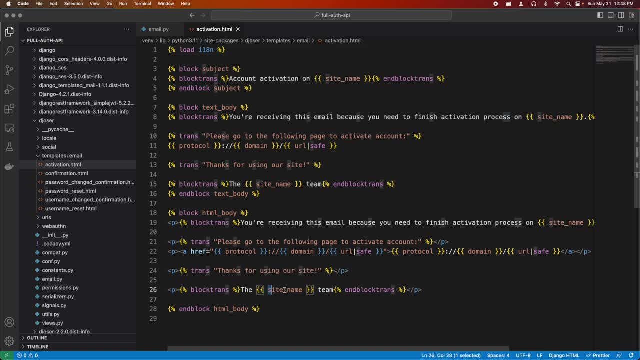 What we're going to notice is in the context. we have things like site name, We have things like domain, So somewhere this context is getting passed. So here we'd have the protocol like, let's say, HTTP localhost 8000, and whatever. 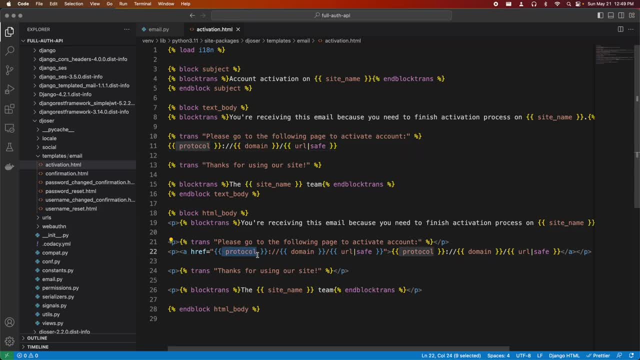 And same thing here. So HTTP the domain- which might be localhost 8000, and then slash whatever you have here. So that would be your href And then also you'd have what you display And then also site name. 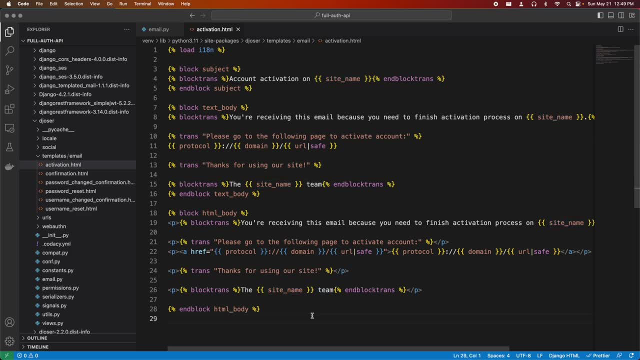 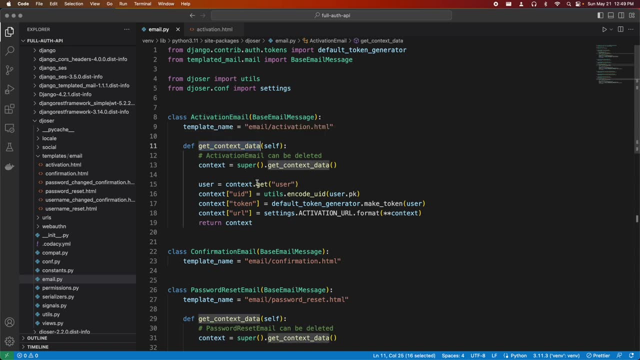 So let's say, the full auth team. So how can we edit these? Well, let's take a look Right here. what we have is this: get context data, And this get context data is calling: get context data- Okay, From the parent class. 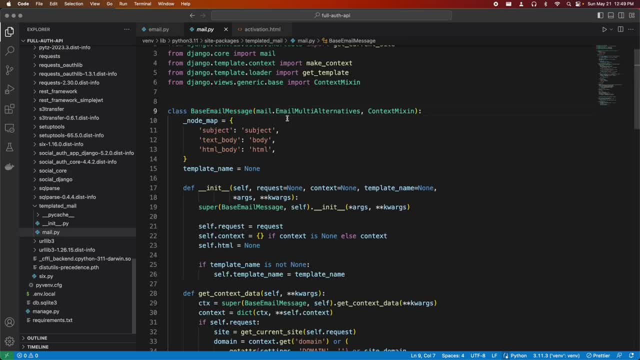 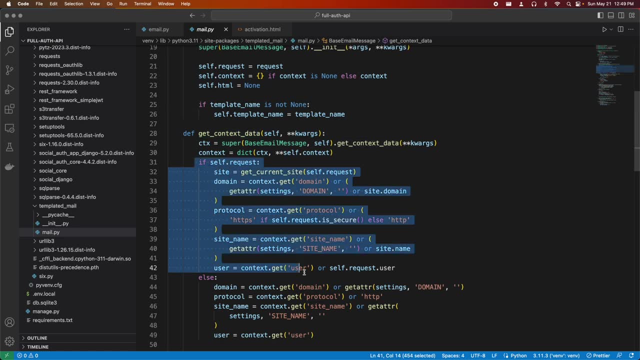 So that is this right here, what we're inheriting. So if I visit this, we have get context data And then, if we take a look, we can see some things getting set up here. So in particular, we have this domain. 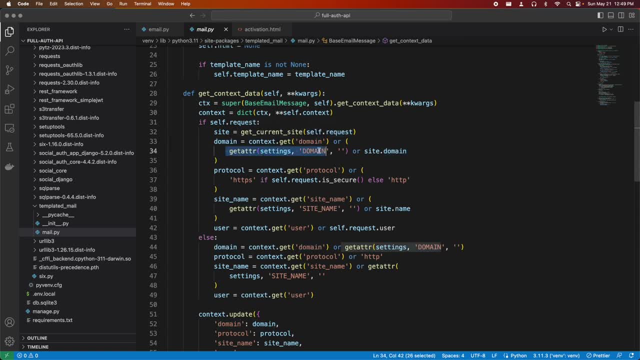 It's equal to contextget domain. or you get this domain from your settings And then protocol, we have it doing it like so And then we have site name grabbing it from the settings Site name, And then we have users equal to contextget user. 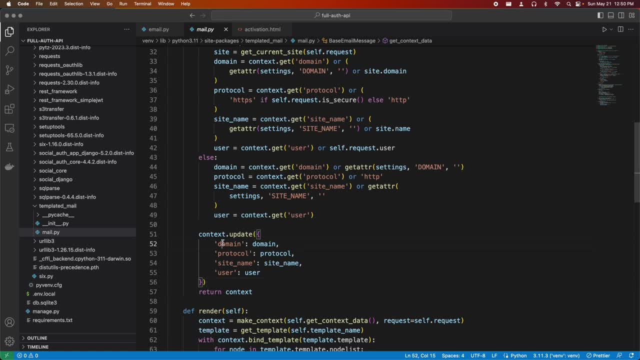 And then, finally, we have context update, where then we update domain and site name protocol user to what we have here. So then in the context itself, this domain that we get from the settings and the site name that we can get from the settings will be inside of the context. 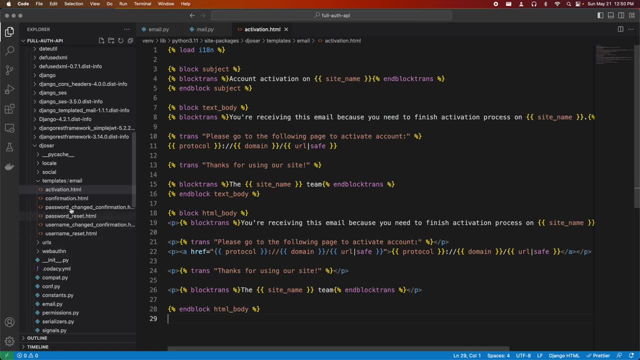 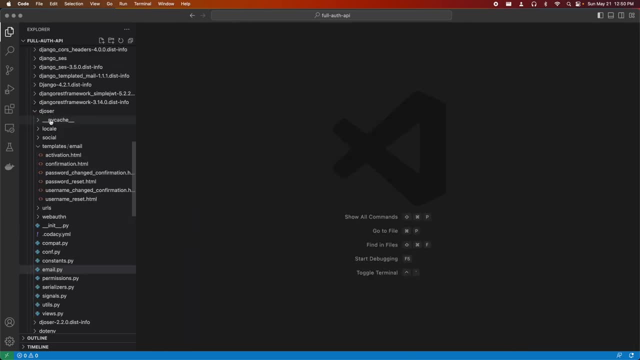 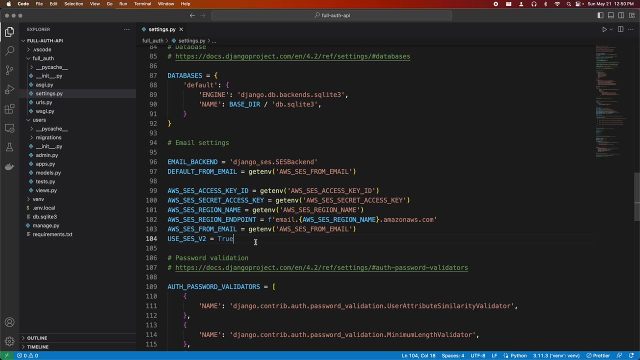 And they'll be plugged into this template, And same thing for the other templates as well. So, knowing that, what we can do? so I'm just going to close up all this now, So we can now go into our settings and we can set these settings up. 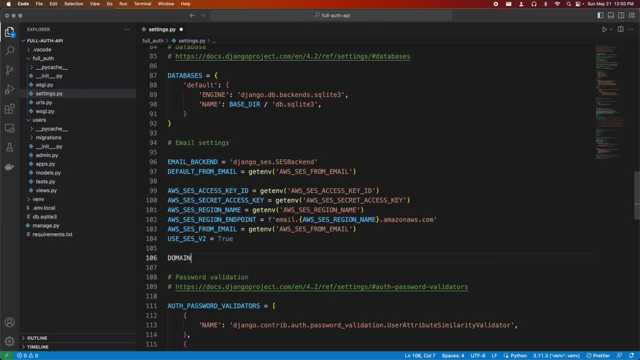 So I'm going to set those up right below here. So I'm going to have my domain And this I'm just going to get from an environment variable called domain, And then I'm also going to have site name And this I'm just going to set to like full auth, because this will be the same in both. 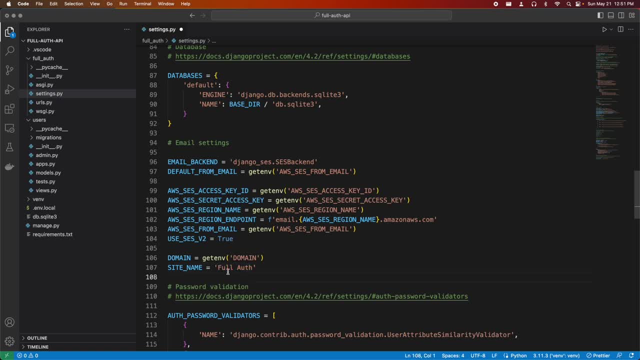 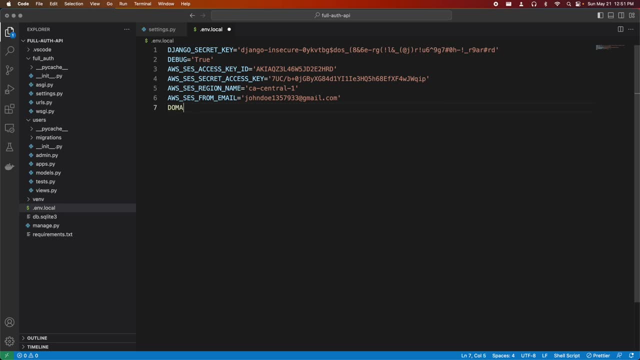 development and production. I'll just have this And this will be whatever your site name is, And the next thing I will do is go into my env. local And then set up the domain And then the domain. in this case it's just going to be localhost 3000.. 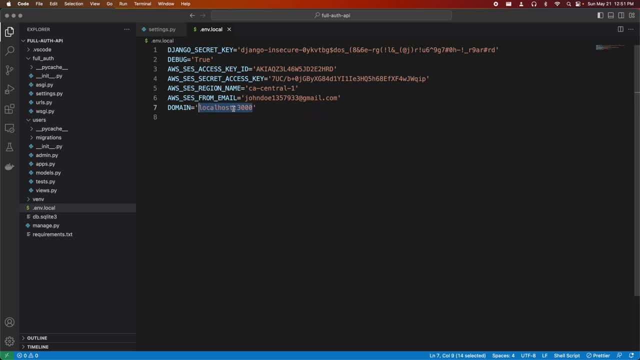 Because later on that's where our Nextjs application is going to be running. So now that we have that, I'm going to restart the server, I'm going to clear and do Python And then I'm going to go back here and I'm going to run server with localhost 8000.. 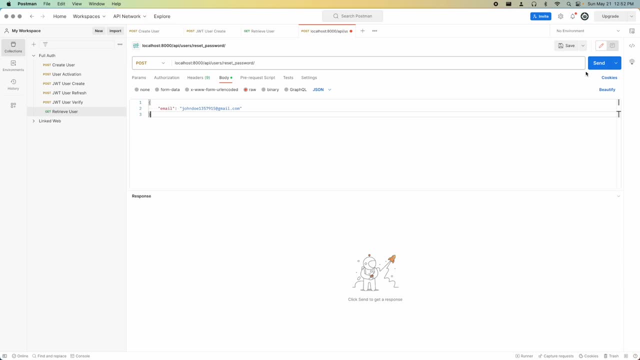 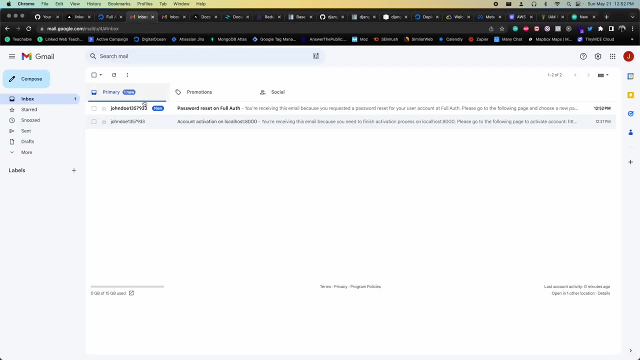 And then back here. now I can send this request off. So tool for no content, let's see if it works. There we go, We got the email And now what we're going to notice is here, instead of localhost 8000, we have localhost 3000. 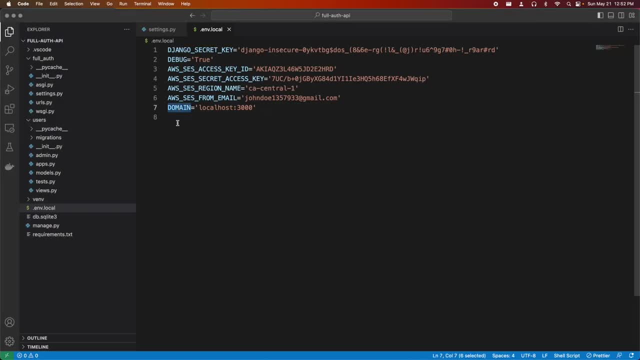 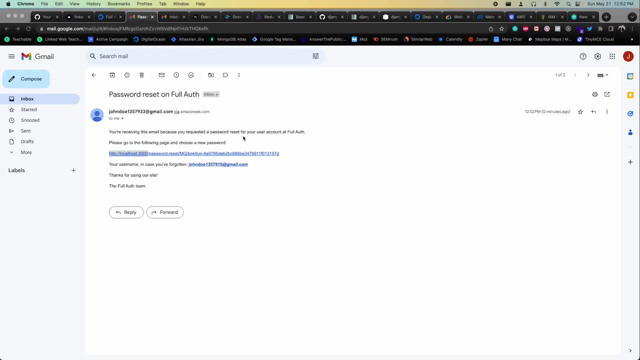 And then further, once we're in our production environment, we can also set up this domain environment variable And set this up to our domain. So that way this will work in production too, And then we just have the URL, and then here we have the full auth team. 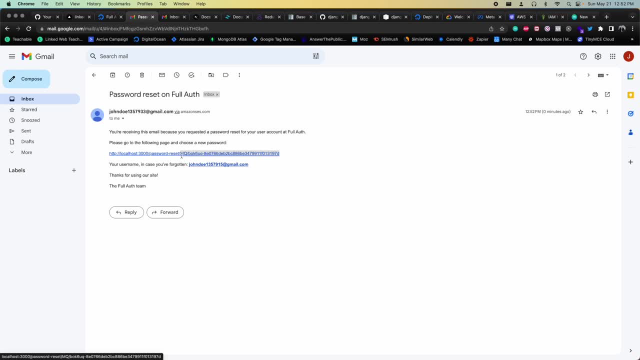 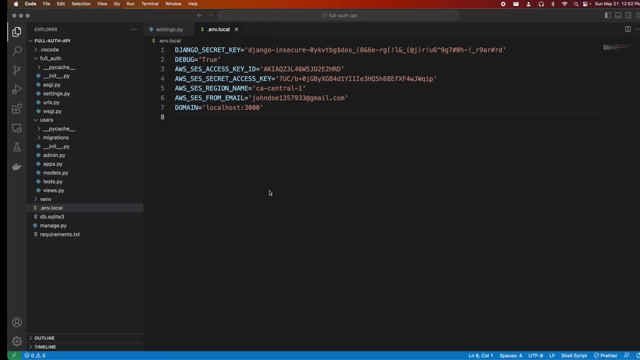 So it looks a lot better. So now what I'm going to do is I'm going to copy this part That's our UID and our token, And then also this right here: by the way, it's following what we set up in our settings. 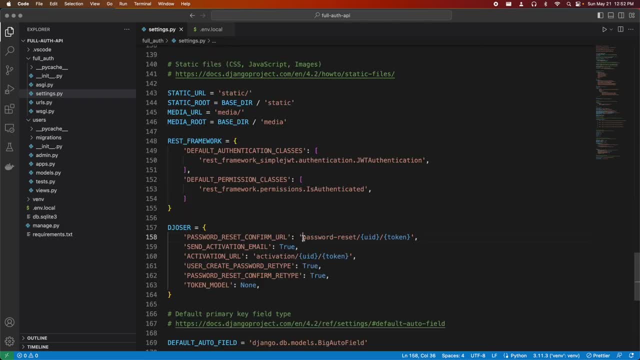 So that was for the Joeser settings. So right over here We have password dash reset, slash UID slash token, So it's following that scheme for the password reset confirm URL. Now you can also set this to whatever, but this is what I have in my case. 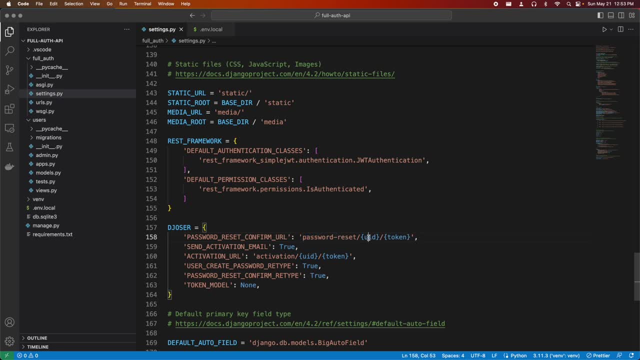 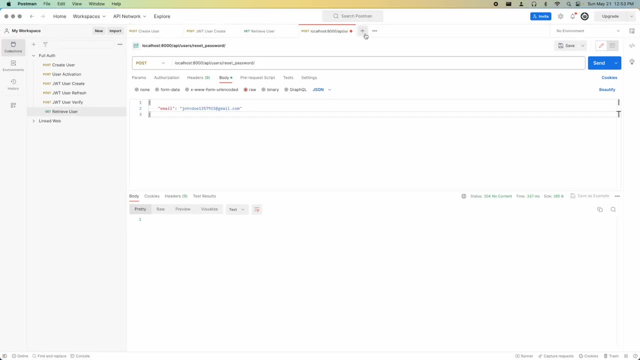 You can even have it as like, let's say, reset UID token, but you do need the UID and the token in here. So, going back now into Postman, we can send off a new request And let's see what the endpoint here. 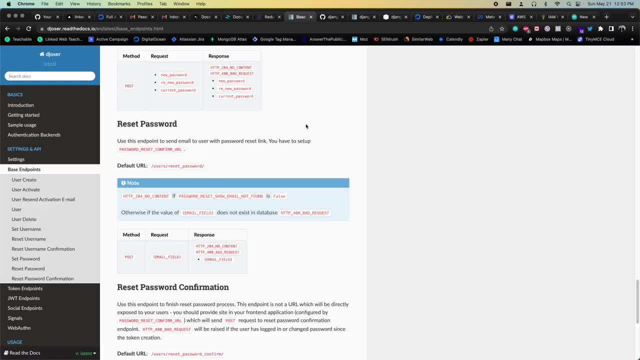 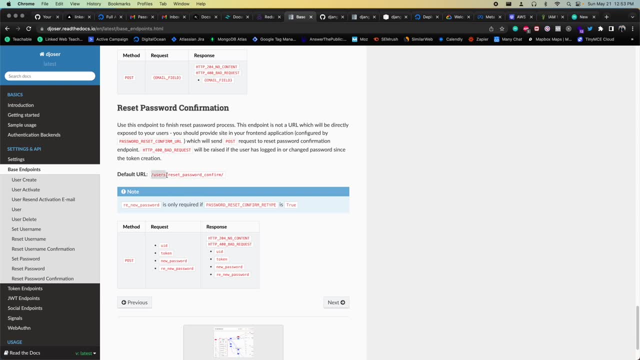 Will be so back inside of Joeser. this was reset password. Here we have reset password confirmation. So this is going to be slash users. slash reset password. Confirm slash. you have to pass UID token, new password and renew password. If it works to a four, no content. otherwise 400 bad requests. 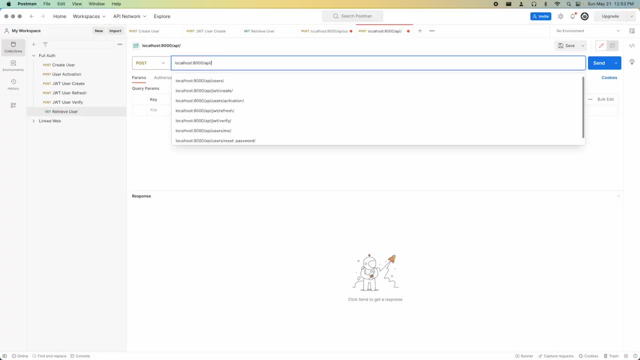 So let's test that out. So slash users. slash. reset Underscore password: Underscore- confirm slash. double check that: reset password: Confirm slash- good. And then we're going to have our headers of content type: application: Jason going to pass in raw data and have UID. 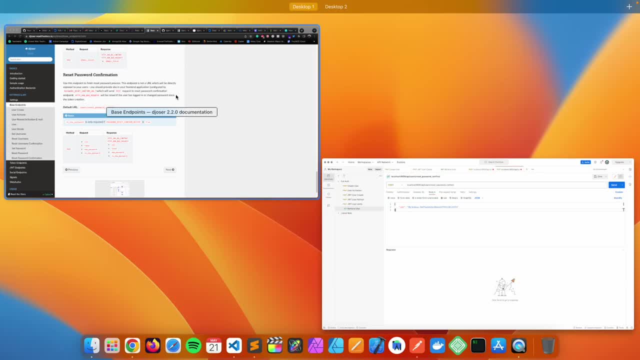 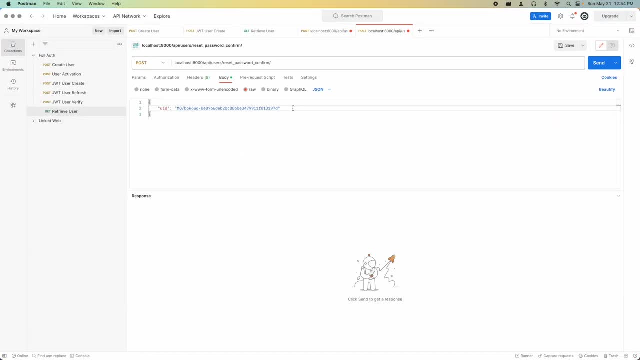 I'm just going to paste in that which I copied, So that was just inside of that email, This part right here. So I'm going to have UID, I'm going to have token and then token It's going to once again, like in the activation email, be this part after the slash. 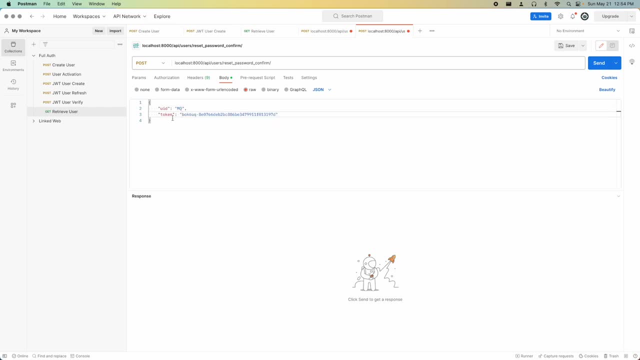 I'm going to cut that, I'm going to delete the slash, I'm going to paste this in the token parts And then I'm going to have new underscore password. I'm going to have my secure password one And then I'm going to have re new password, which will be my secure password two. 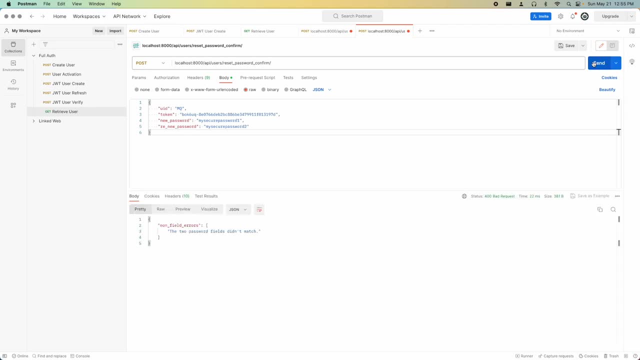 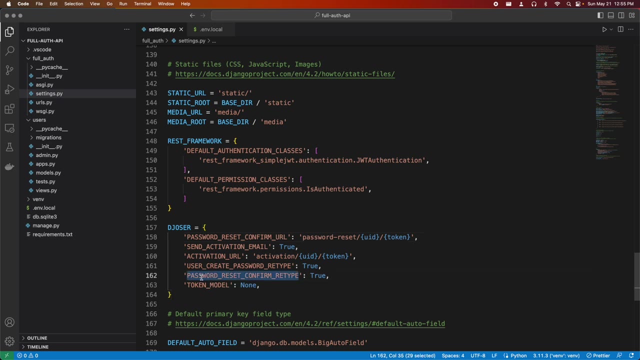 So I'm going to test when they don't match and see what happens. Two password fields didn't match, Perfect. So that is because of this setting right here: password reset, confirm, retype. So that means that we have to have that confirmed field, which is this field right here. 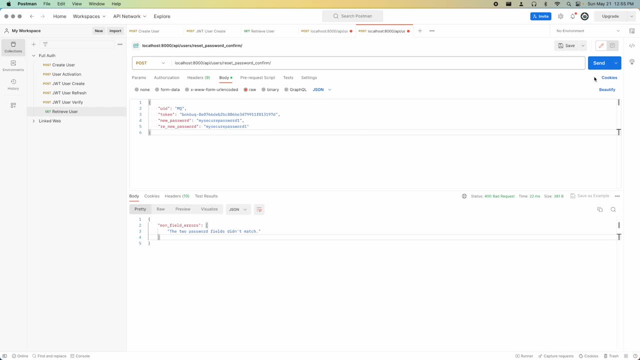 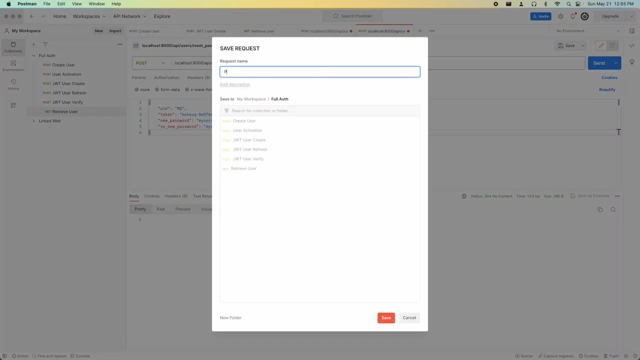 And they both have to match. I'm going to set this to not match. I'm going to click send and we get a tool for no content, which means that this worked. So I'm going to do password reset, confirm, save that. 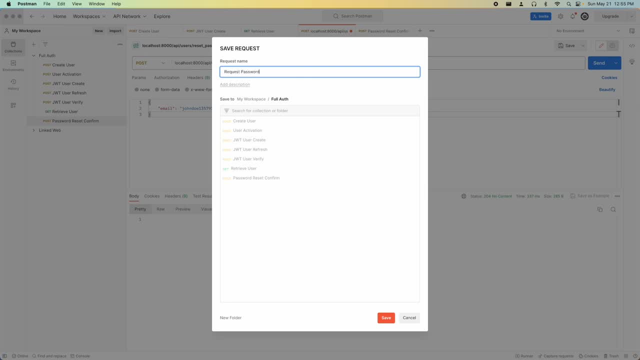 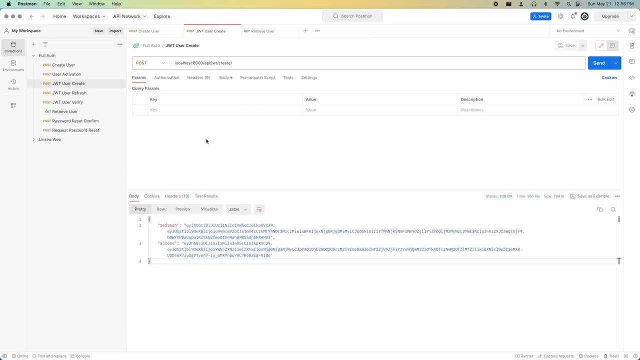 I'm also going to save this one as request password reset. and there we are. So we have all of these. And now, if I try to log into this right here using my secure password now, I get a 401.. It's unauthorized because we successfully reset the password to now be my secure password one. 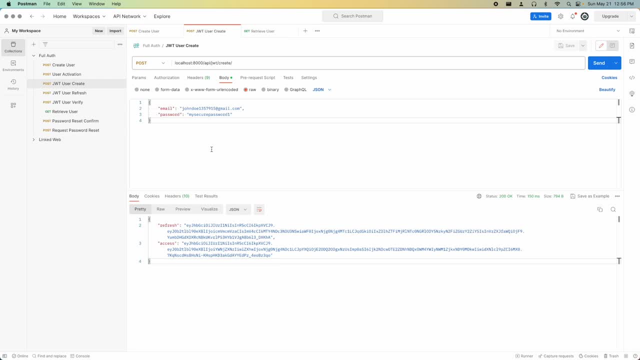 So there we go. Now I get the access and the refresh token. So now we tested out all of these endpoints. Now the next step I'm going to do is I'm just going to quickly set up these course headers. It's not going to change anything for us, but it is something we're not to set up. 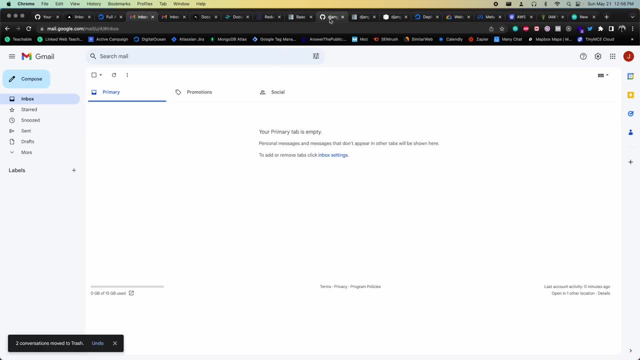 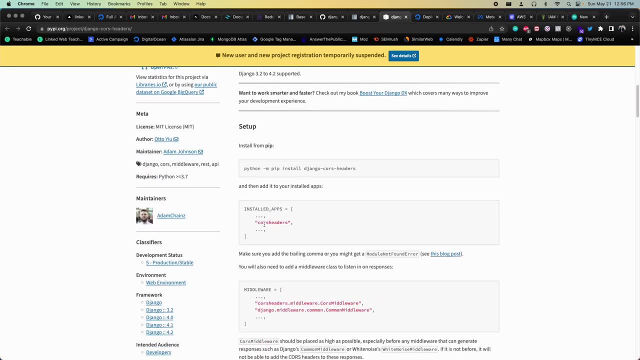 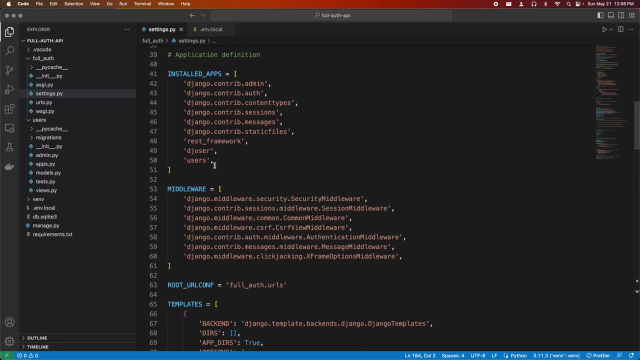 So I'm just going to delete these two And then, inside of Django, course headers. So there it is. These are the things you have to set up. So in our installed apps I want to have course headers. I'm going to go to my installed apps and I'll put course headers here. 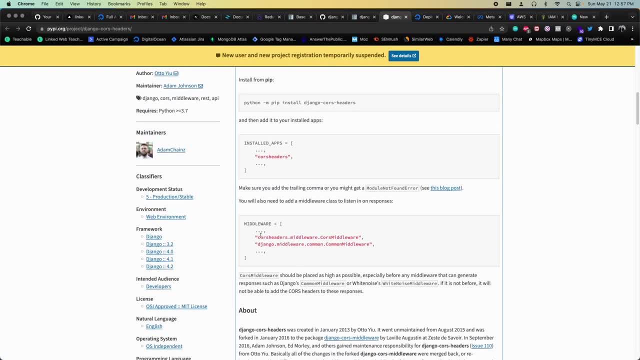 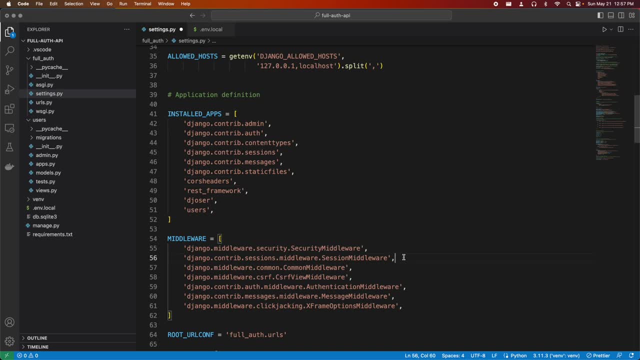 You also have to set up middleware for this. I'm going to copy this, I'm going to place this middleware above the common middleware, And then all of this is going to do Is it's going to set up some headers that I need to set up when I send responses from my server. 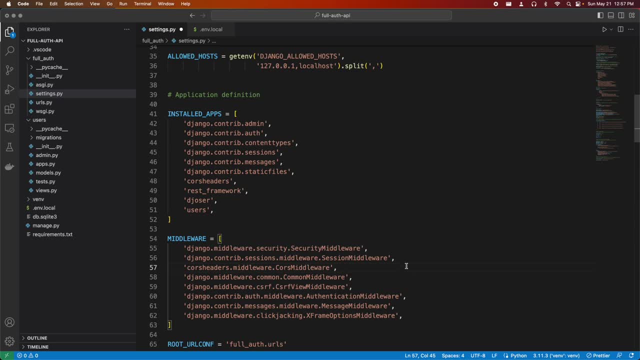 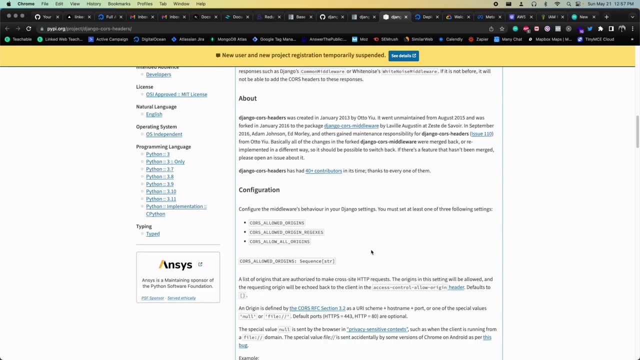 And then that way on the browser I can have these cross origin requests not get blocked by the browser. Then I also have to set up which origins are allowed, So you can do that with cores allowed origins. So I'm going to copy this: 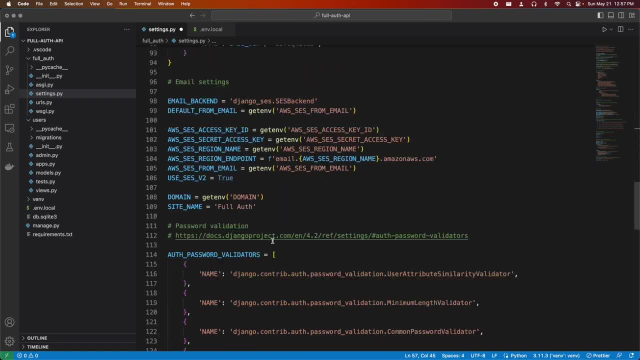 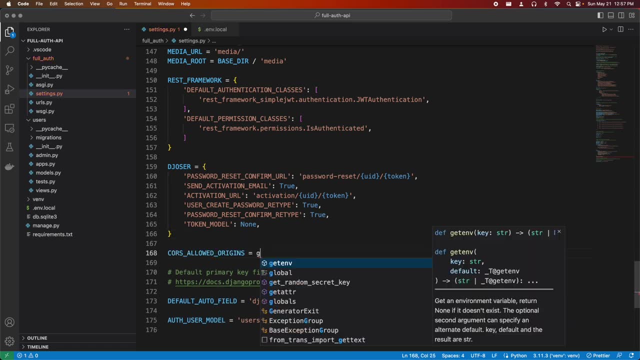 I'm going to go back here And I'll scroll down and put that somewhere at the bottom, Maybe below my Joster settings, And then I'm going to have get ENV And it's going to be the same as this here. 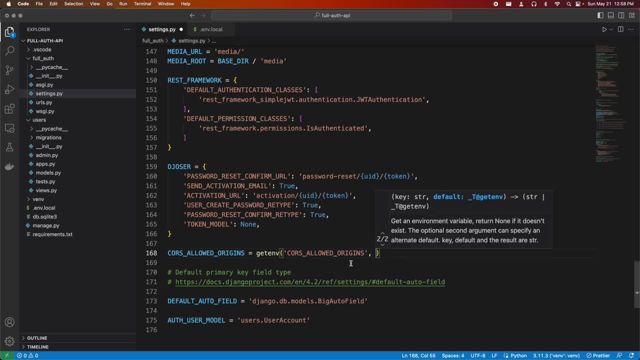 And then that way in production I'm going to set up whatever my cores allowed origins are. That'll be my production URL And I'm also going to have a default which is just going to be HTTP local host 3000 and also HTTP local hosts. 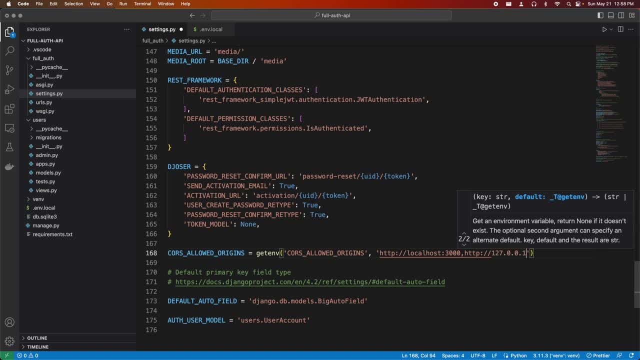 Or sorry, not local host, but 127.0.0.1, colon 3000.. And then I can do a dot split on the comma So that way when I'm running my next JS front end, I can allow cross origin requests to this right here, which is where next JS is running. 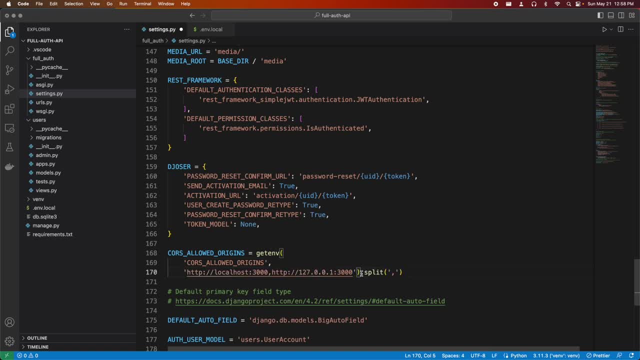 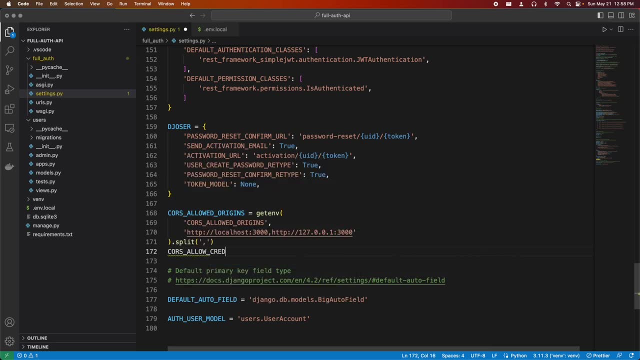 And I'm also going to format this a bit So it looks better. And then the next thing I'm going to do is I'm also going to have a core Cores allow credentials, which is going to be true. So this right here in my responses is going to set up a cross origin allow credentials heading. 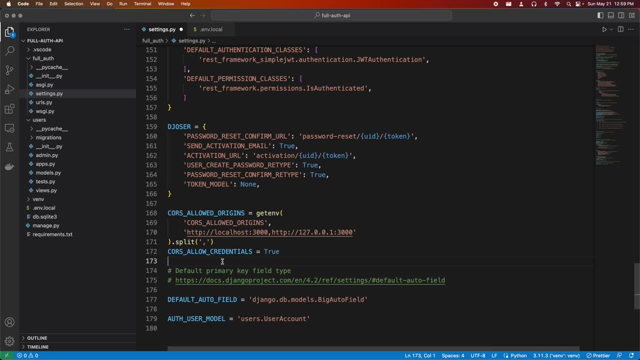 And then what this is going to do is it's going to allow cookies to be getting sent cross domain. So we're going to need that because when we have different ports, that counts as cross domain. So in our development environment we have local host 3000 and 8000 for the next JS front end and for the Django backend API. 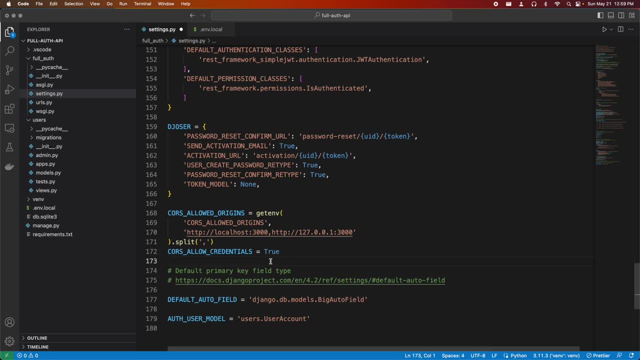 In production. we're also going to have different domains, or cross origins, because we're going to have, let's say, our domaincom for our next JS front end And we're going to have apimydomaincom for the backend. So this is something we have to include. 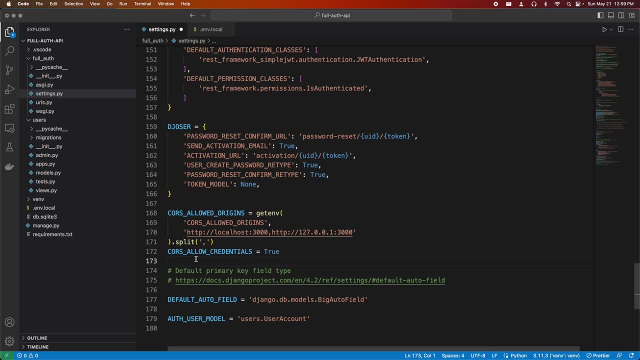 And then from the front end, when we make AJAX requests, we're going to include an option called credentials include And that's going to allow the cookies to get included in the request, And we're going to need this so that the browser doesn't block the cookies when they're coming back. 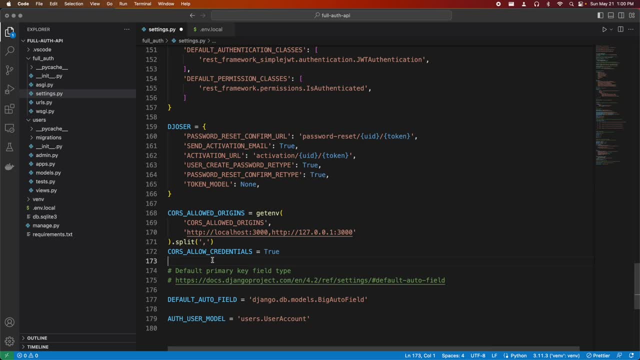 And so those are things that we have to do in order to manage the cookies. Now we're also going to have to adjust some other things, because there are settings in a cookie that will prevent it from being cross domain even when we have these things. 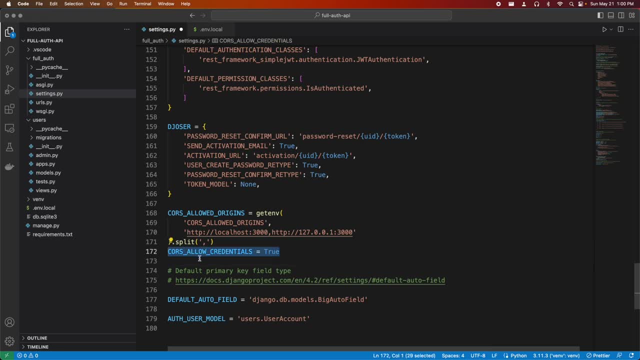 So we're going to get into that, But this is what we need for now with our course setup. I'm going to save that. So the next thing I'm going to do is I'm going to start to override the behavior of Joesser and simple JWT. 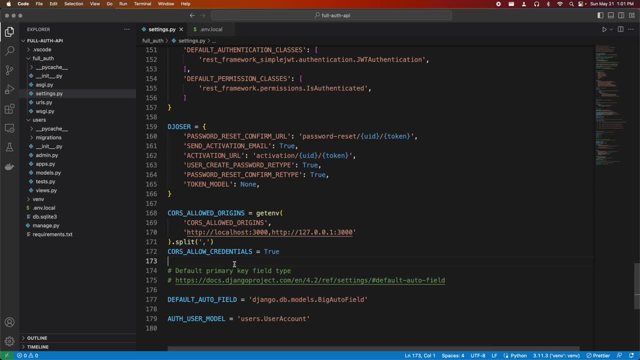 So that way I can get the behavior I want, Instead of having to put that authorization header inside of my requests whenever I want to make an authorized request. I just want this to be managed by HTTP only cookies, So that pretty much just means cookies that have the HTTP only flag set to true, which just prevents JavaScript on the front end from reading the values of our access and refresh tokens when they're stored in the cookies. 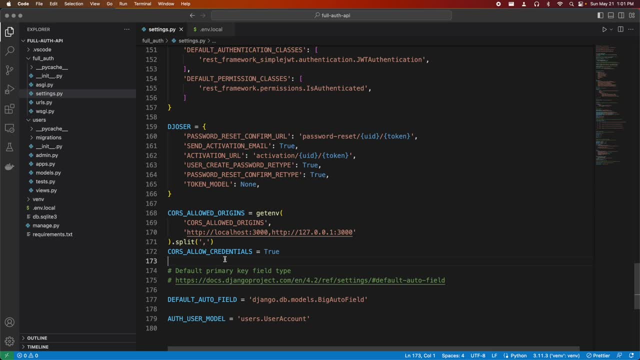 So it's just a very secure way to store these cookies, But we also need a way to have our authorization process. Let's actually read these values. So to do that, what I'm going to do is I'm going to create a new file inside of my users app. 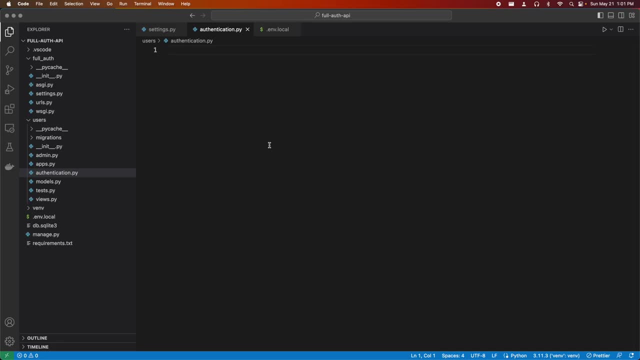 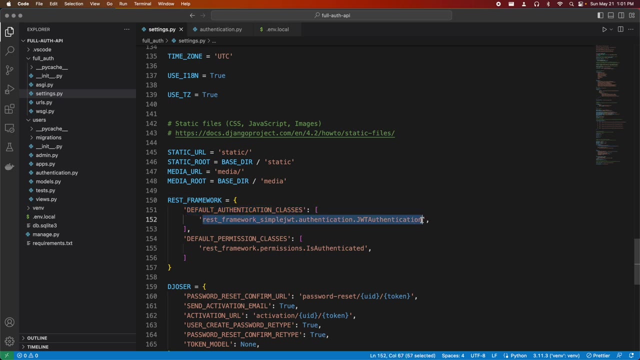 I'm going to call it authenticationpy And then right now in my settings, my default authentication classes is this, right here. So right now it's going to be a little bit different. I'm going to copy this, I'm just going to paste it here. 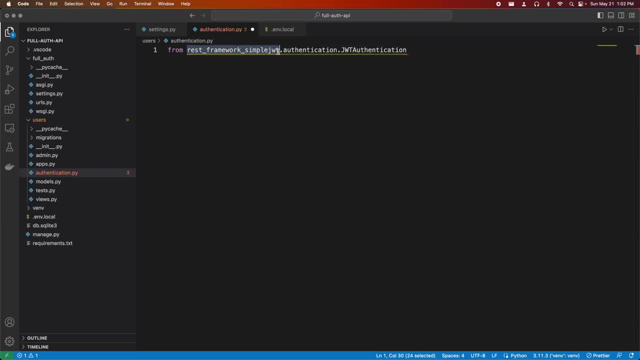 So what we're going to want to do is, from rest framework, simple JWT Authentication. I'm going to want to import JWT authentication and I'm going to want to override this. So what I'm going to do is I'm going to make a class called custom JWT authentication and that's going to inherit JWT authentication. 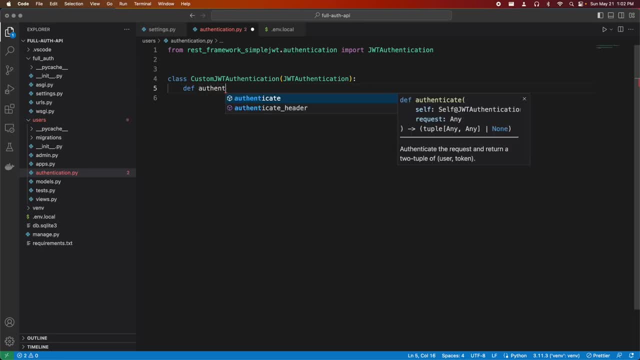 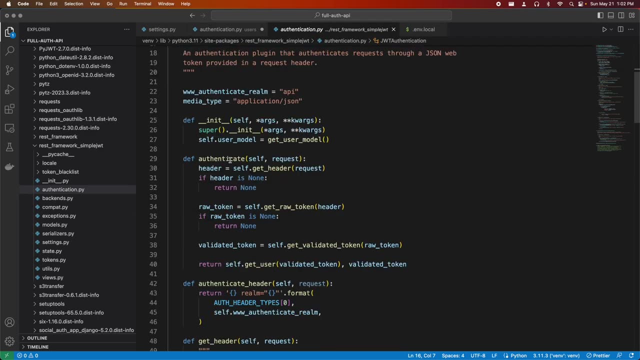 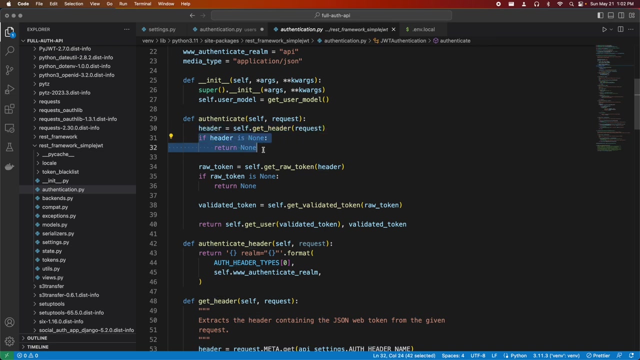 And we're going to override its authenticate method. So we've got some auto filling here. So if I click into this And look at authentication, this right now is how it works. It gets the header. If the header is none, we return none. 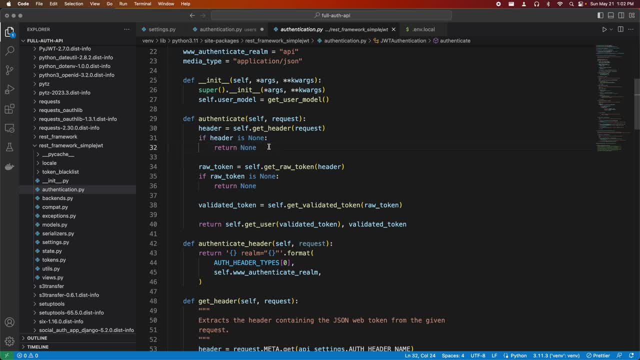 So this, in particular, something we're going to want override, because we're not going to have a header, but we're still going to want this to work, because we're going to want to get the values from the cookies instead, And then we get the raw token. 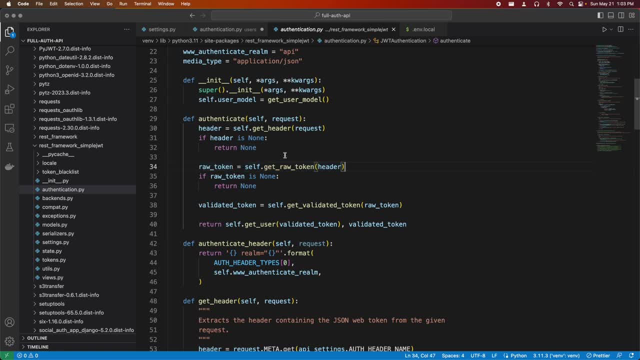 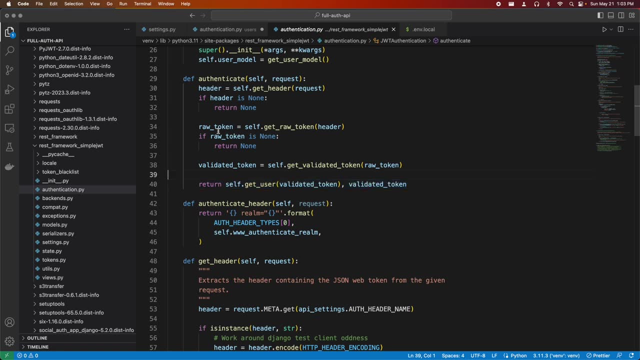 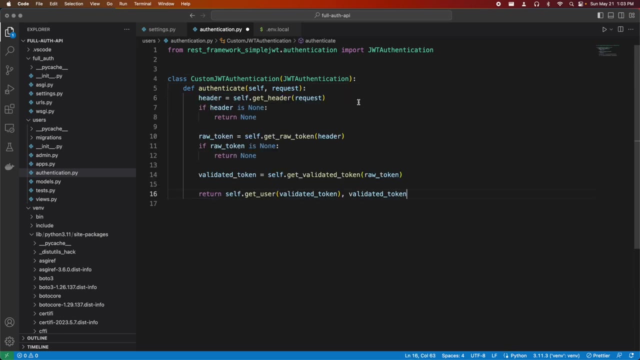 So because inside of the headers they have things like bearer token, So this will just get the raw token. It'll make sure it's there, It's going to validate it and it's going to return. So I'm just going to copy what's in here, go back into my authenticates and I'm just going to paste in here. 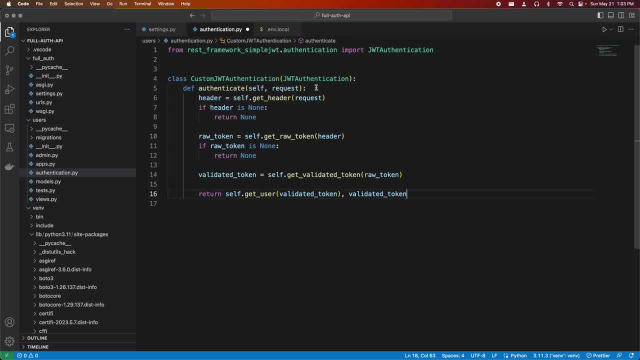 So we're going to have self and request, and then I'm just going to wrap all of this in a try, except just to make sure things work, And if they don't, I'm going to return none. So first thing I'm going to do is I'm going to try to get the header. 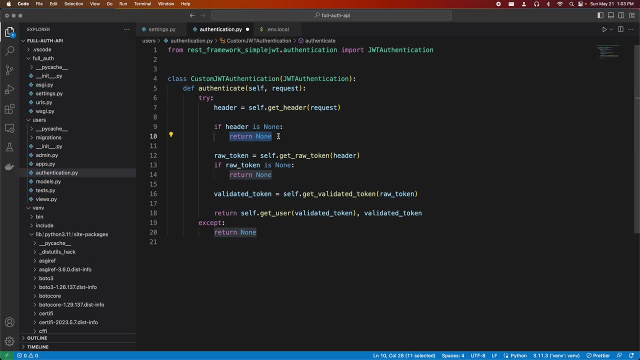 Now, if the header is none, instead of returning none, I'm just going to get the raw token from the cookies. So the way I can do that is raw token is requestcookiesget, and I'm going to get an access cookie. 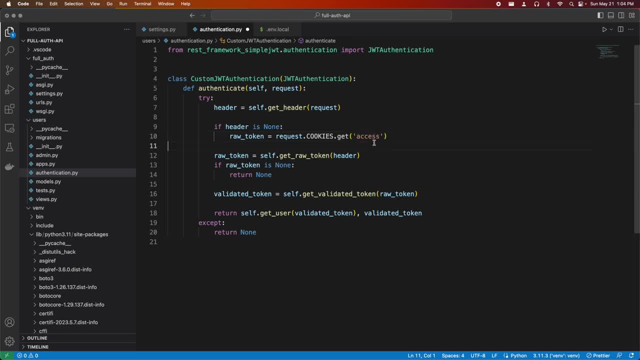 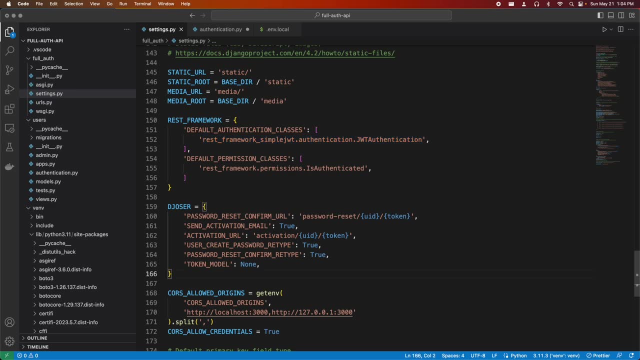 So I'm going to expect there to be a cookie called access and I'm going to retrieve it, And another thing I'm going to do is I'm going to go into my settings and maybe right over here I'm going to set up. 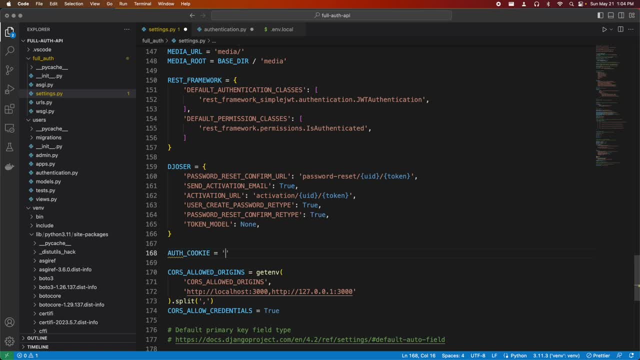 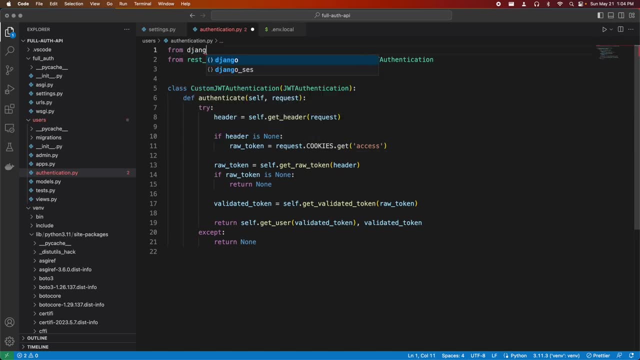 A setting which will be auth cookie. I'm going to set that to be access And then what I can do is from Django comp import settings And then, instead of doing access hard coded like this, I can do settings dot auth cookie. 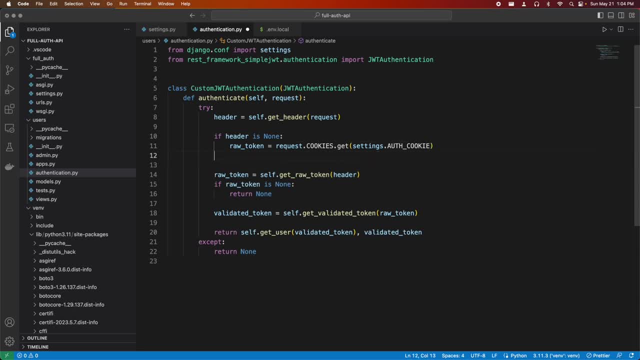 There's just a nicer way to do this part, And then I'm going to have an else. So if header is none, we're going to get the raw token From the cookies. Otherwise, we're going to do it like it was doing before, using the header. 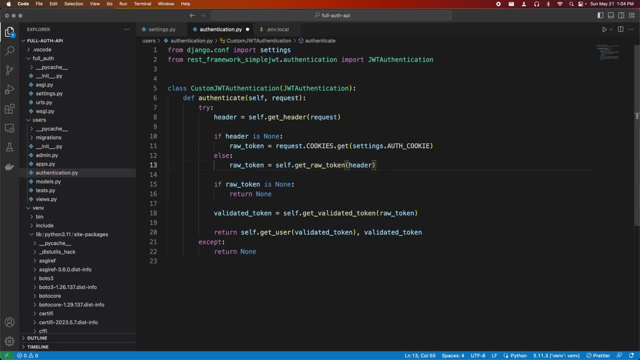 So I'm going to paste this in the else block. So there we go, Pretty easy to override this. And then we're going to see: is raw token none. If it is return none, I'm going to validate it just like before and we're going to return. 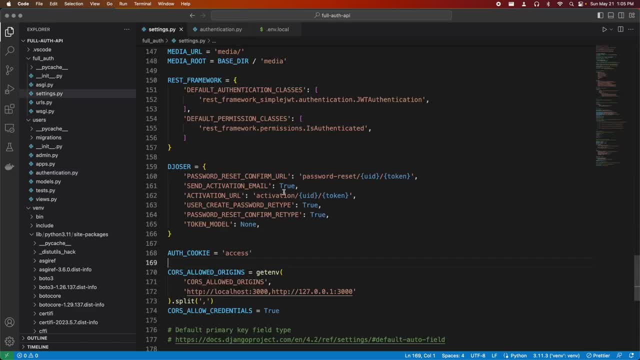 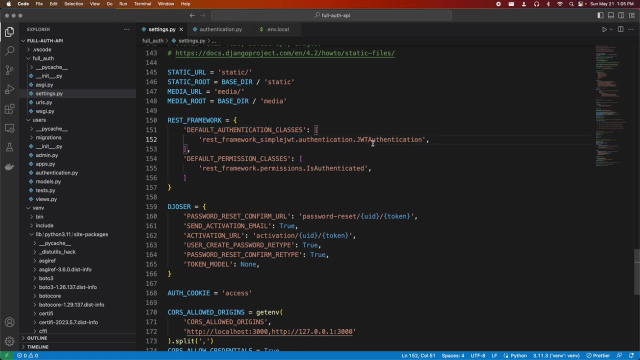 Now the only other thing we have to do is go back to our settings and then go to our authentication classes. We're no longer using this. We're going to be using our custom one. So Custom JWT authentication, which is going to come from our users app dot authentication. dot. custom JWT authentication. 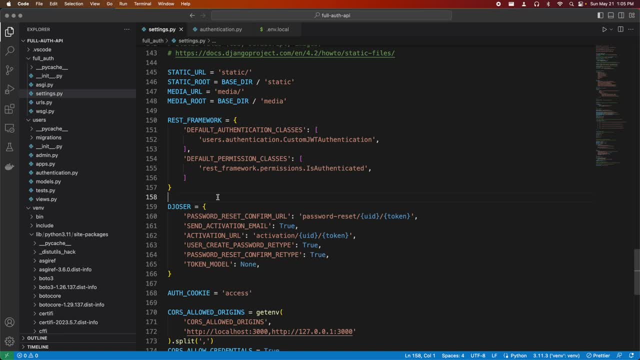 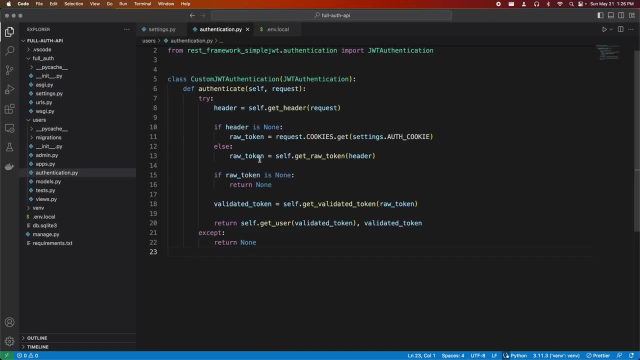 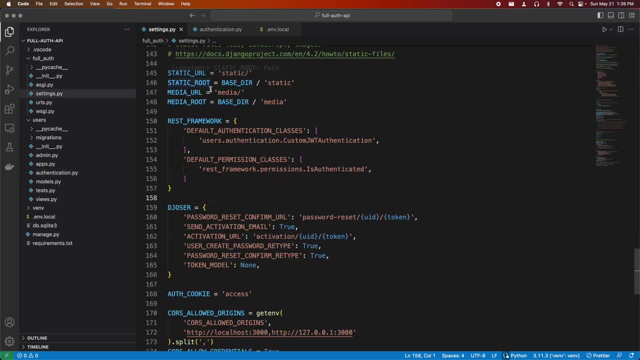 So now, any time you make an authorized request, we're going to use the cookies. right now are authorized requests. They are going to work because in our authentication file we are expecting to grab from the cookies the access token cookie. However, we still will have to override something. 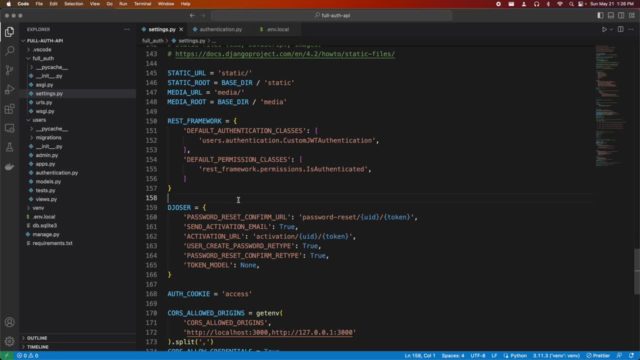 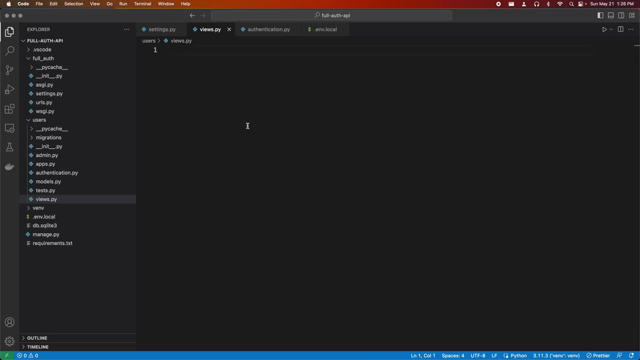 Some things for the views in order to have these cookies get set, and have them set with the appropriate options, And then that way this whole thing is going to work. So let's go ahead and get started on that. So, inside of my users app and the views dot pie, this is where I'm going to get started with overriding some of these views. 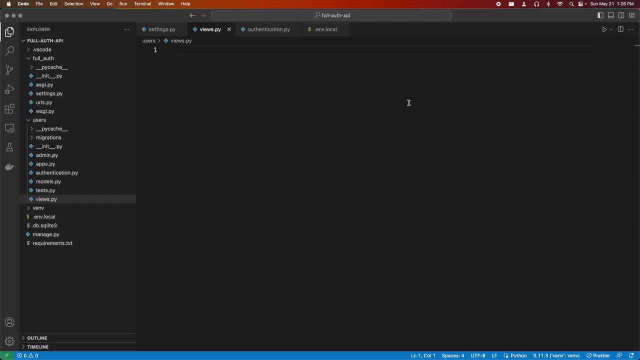 In particular, the views that I need to override are going to be the ones related to JWT authentication. So the create view, refresh view and verify view. So One thing I'm going to Do is I'm going to import my settings from Django comp- import settings- and then in my settings I'm going to define more settings than just this off cookie. 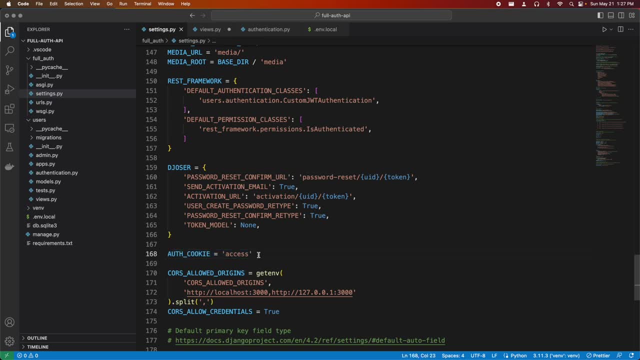 And then I'm going to be using those for some settings related to these cookies. So I'm just going to grab them from here to have them in one place and have these settings just be correct. So that way I'm not like hard coding things across my different views. 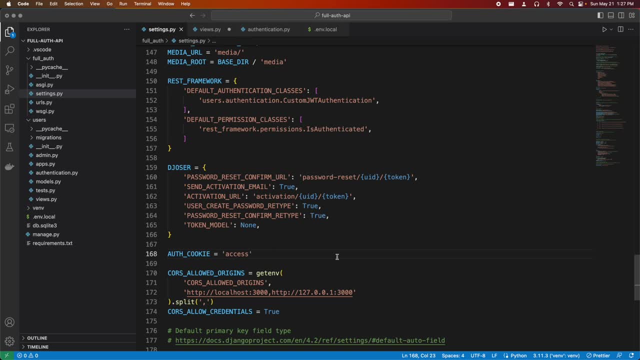 So it's just a nice way to kind of organize things. So while I'm here I'm just going to set these up So I have my off cookie already going to have off cookie access max age, and then this I'm going to set to 60 times five. 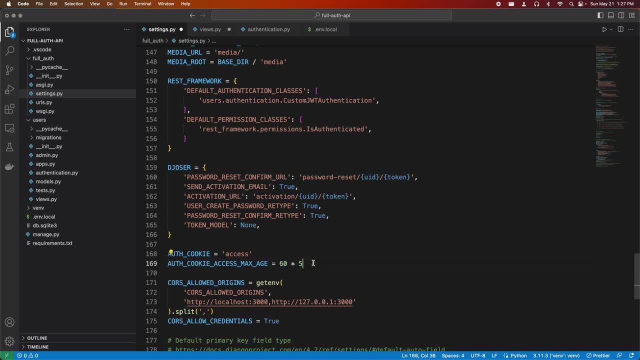 So that's going to be 60 seconds times five, which is five minutes. So by default, my Jason web tokens for the access token they expire after five minutes. So I'm just going to have this match that. So the cookie is going to expire after five minutes, as well as the access token. 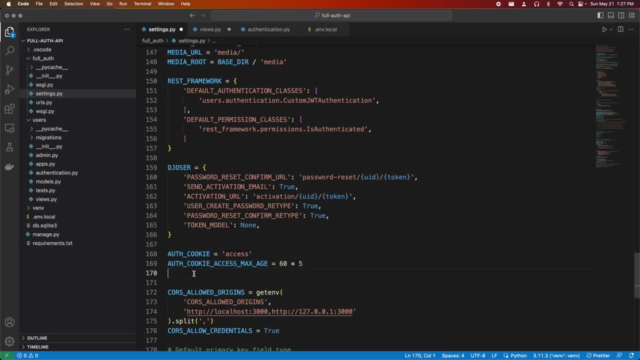 It's going to Have the synchronization be proper, And then I'm also going to have a max age for my refresh token. Now, this one's going to be longer. This one's going to be 24 hours by default, So I'm just going to match that by doing 60 times 60, which gives me an hour times. 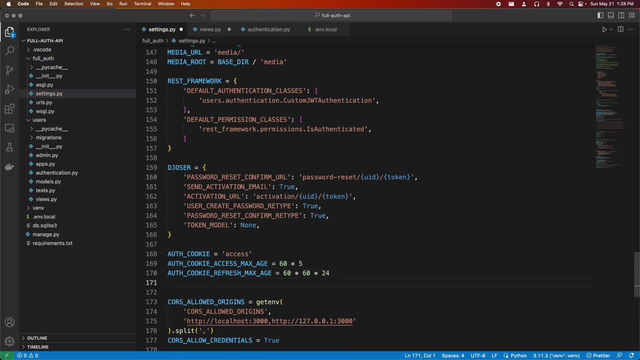 24 gives me a day, And then I'm going to have off cookie secure. So this is going to set whether we need an SSL certificate or, I guess, an HTTPS Connection in order for these cookies to get sent in the requests and their responses. 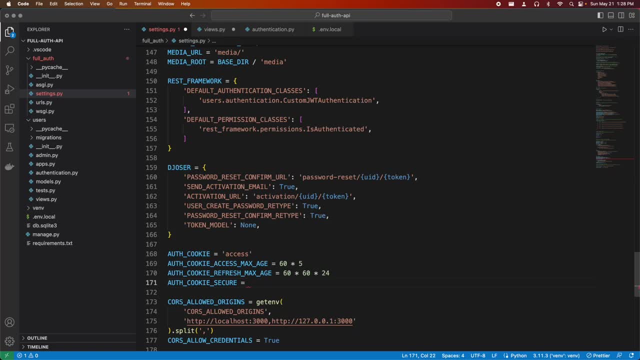 So in my development environment I'm going to want these to be false, but in production I'm going to want it to be true that we do need to have a secure connection in order to have these cookies get sent. in the requests and the responses. 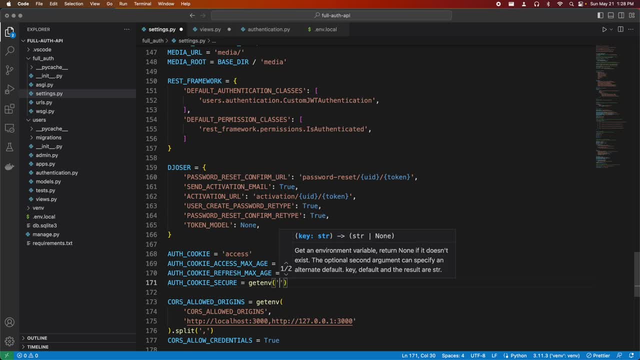 So I'm going to do is I'm going to put in get ENB, and I'm going to get an auth cookie, secure environment variable, which we're going to set up by default. I'm going to have this Be true and then equals true. 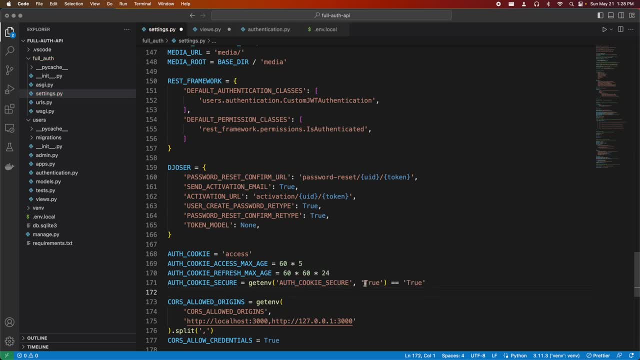 So that way in the production environment we don't have to set this thing up. It's just going to be true by default And true equals true is just going to give us the Boolean of true. but in my development environment I'm going to want to have this thing set up. 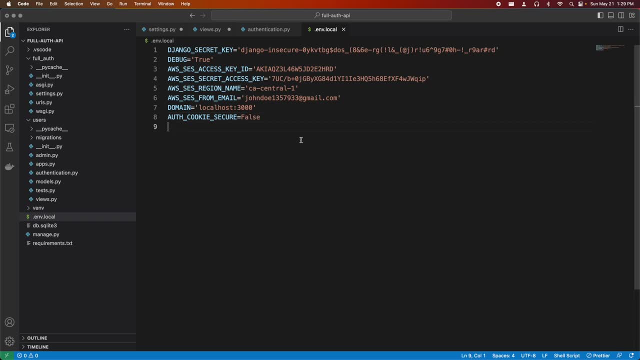 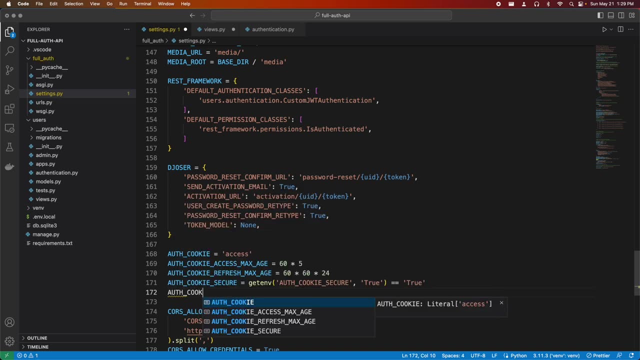 So I'm just going to put it here and it's going to be false. Now, another thing we're going to need after this is auth cookie: HTTP only. So This Is going to set the HTTP only flag on that cookie. 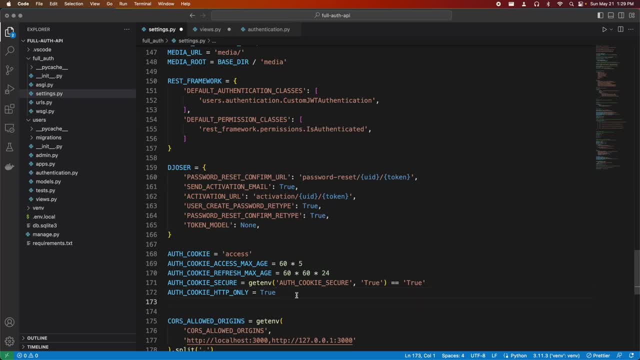 So that way, JavaScript can't access the values in the browser. I'm going to have the auth cookie path, which is just going to be slash in our case, And then I'm also going to have auth cookie, same site, which I'm going to set to none. 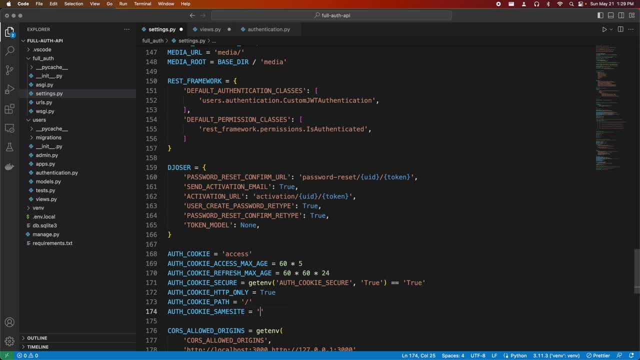 So for same site you can either have strict, you can have lax or you can have none. So strict means that in order for These cookies to get sent, the domains they have to match. So this will restrict where you can't have these cookies get sent. cross origin. 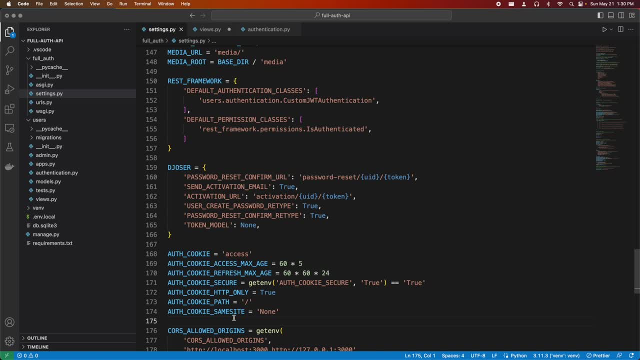 That's what we have strict, which means that my front end would have to be on, let's say, my domaincom, And my backend would also have to be on my domaincom. They'd have to be on the exact same domain, the exact same ports. 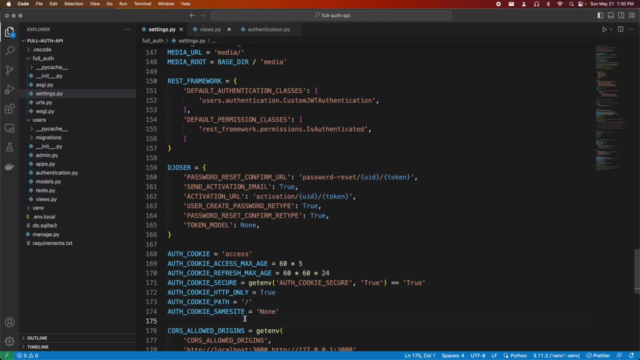 So that's, if you have strict Now, in our case, we're going to have these be cross origin and I'm going to want these cookies to get sent cross origin In order for that to happen. I can't have the same site property as strict. 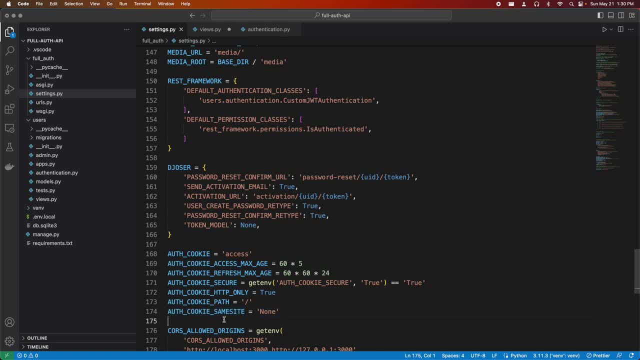 Now I can have lax, but what lax would do is it's going to allow these cookies to get sent cross origin, but only on safe methods. So safe methods are things like your get method, your options method, your head method. So these are your safe methods. but if we have things like post and put and patch and delete and so forth, these cookies won't get sent with lax. 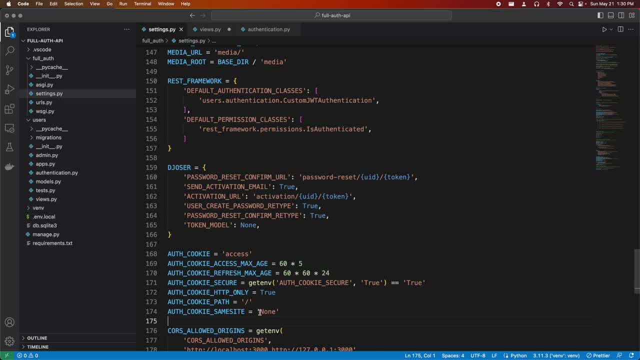 So in order for that to happen- To have cross origin cookies getting sent, I need to have none here so that it also works with those other methods. because, in particular, I will need that to work because even for these views I'm about to override, like my create view, the refresh view, verify view- these views are all post requests and I'm going to want these cookies to get sent with those post requests, so I need same site to be set to none. 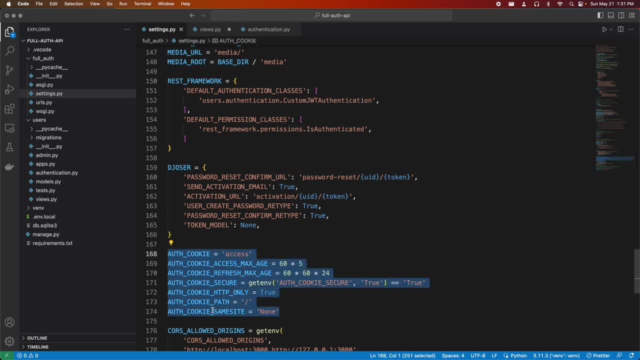 So that's going to be all the settings I need. Hopefully all of these make sense. And then there's also going to be a domain setting that gets set by default and that's going to be the current domain in our development environment. It's going to be localhost and our production environment is going to be apithedomaincom. 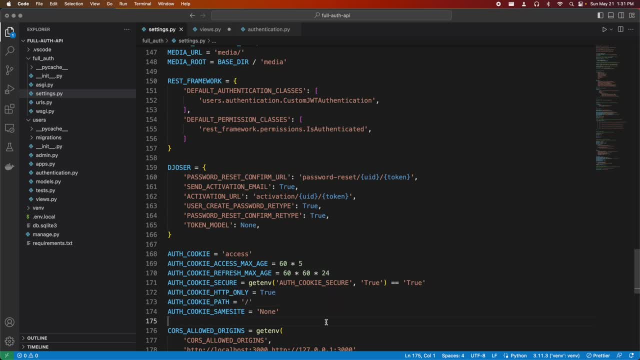 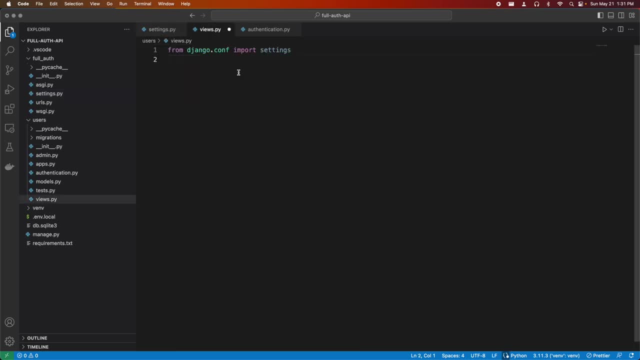 So that domain property. it's going to make these cookies only valid when they're getting read from here and here being our API server. So now let's go ahead and go back here, And what I'm going to do next is I'm going to import those views we need to override. 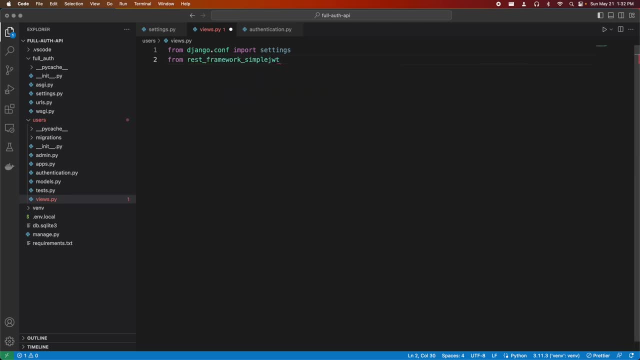 So those are coming from rest Framework, simple JWT views. and then we have our token obtain pair view. This is for the create. We have the token refresh view. This is for the refresh endpoint, and then we have token verify view. 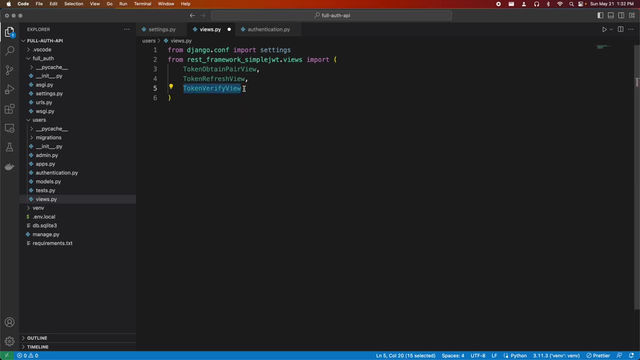 And the verify view. I don't think I explained it, but the verify view just verifies whether our access token is still valid. So the next thing I'm going to do is I'm going to set up a class which is going to be my custom token. 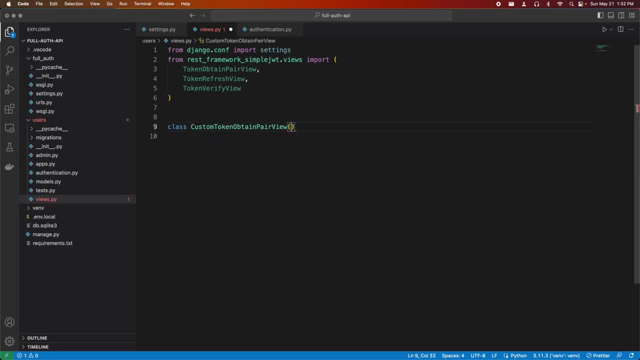 I'm going to say token obtain pair view and this thing's going to inherit token obtain pair view, And then we're going to want to override its post method. So, by default, the way that this is going to work is it's going to generate the access and refresh token and it's just going to send them in the body of the response. 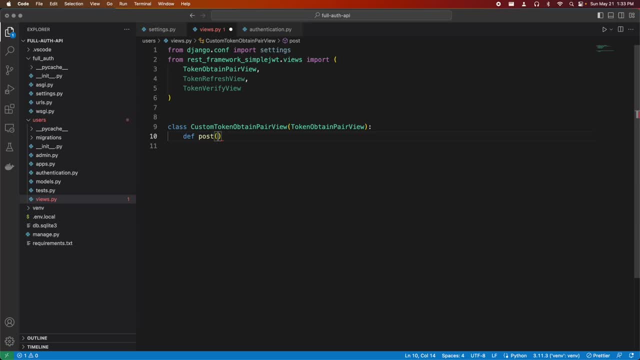 But I don't want to just do that. I also want to set the access and refresh token in the cookies. So I'm going to put in request, args and keyword arguments here, and then the way that I can do this is I can just call the super method post passing in requests, args and keyword. 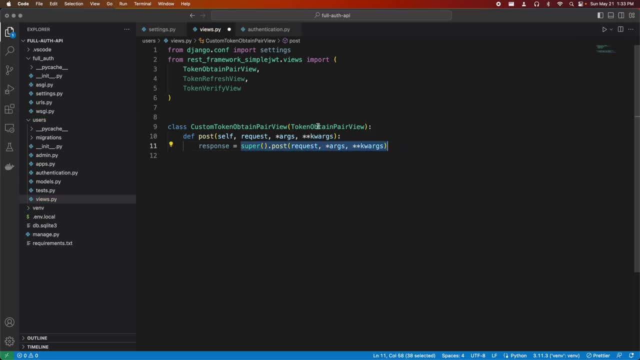 args. so this super class is just the token obtained pair of you. just like before, I'm gonna capture that response and then I'm gonna check was this successful. I can do that with response dot. status code equals 200, because 200 means this was successful and if that was, I'm gonna get the access and refresh. 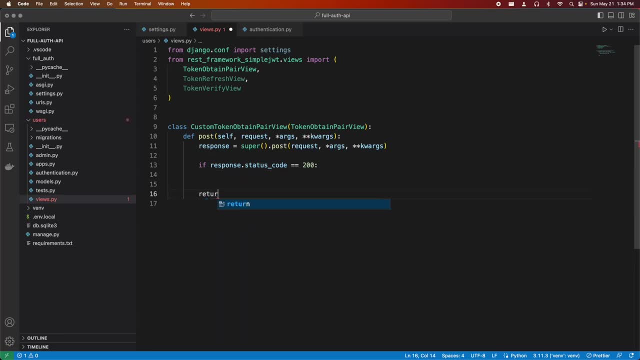 tokens, I'm gonna set the cookies and then after that I'm just gonna return that response. so before I return the response, I want to set those cookies because by default this token obtained pair of you will not do that so I can get the access token response data. get access is where I get that from. 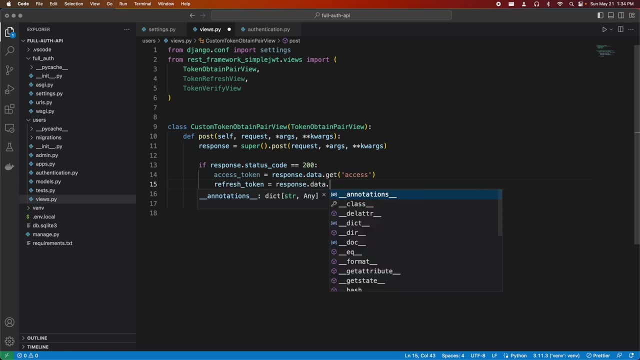 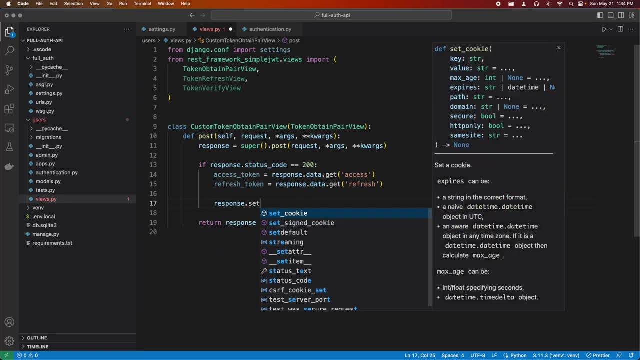 distance data get access is where I get that from. response data get access is where I get that from. and then we have refresh token, which is response data get refresh, and the next step is just to set these cookies. so i can easily do that with just response dot set cookie. and then here i'm going. 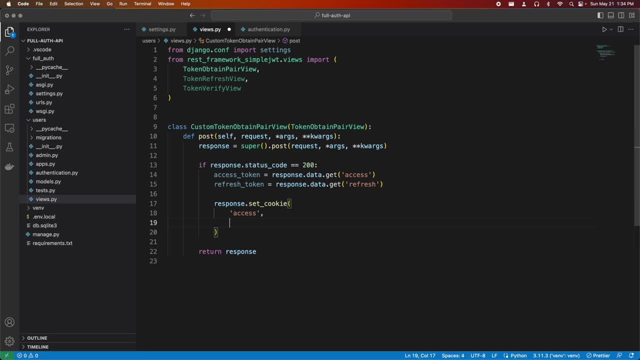 to have access. that's going to be the name of my cookie and then i'm going to have the value. this is going to be access token. so that's the access token i got. from the response of this token obtained pair view, and then i'm going to have a couple of those settings. so i'm going to. 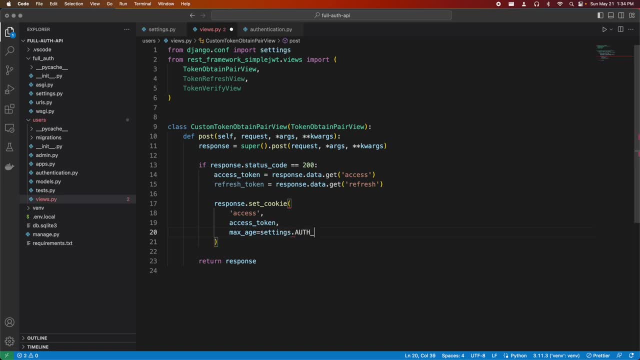 have max age, which will be settings dot auth cookie access max age. then, after max age, i'm going to have my path, which will be settings dot auth cookie path. so this is that slash path. i'm going to have secure, which will be settings dot auth cookie secure. 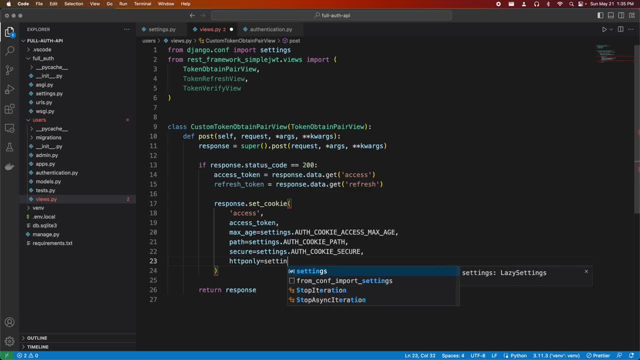 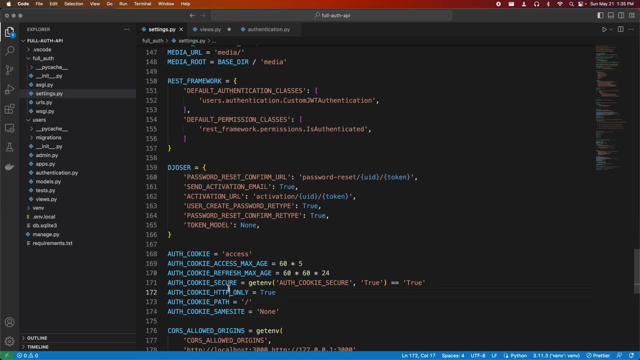 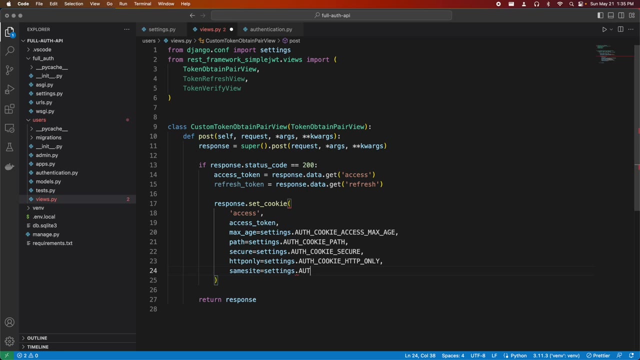 i'm going to have the http only flag, which will be settings dot auth cookie- http only. i think i named it like that- yep, http only. and then, finally, i have the same site which is going to be settings dot auth cookie- same site. so these are all the settings i need in order for this cross origin. 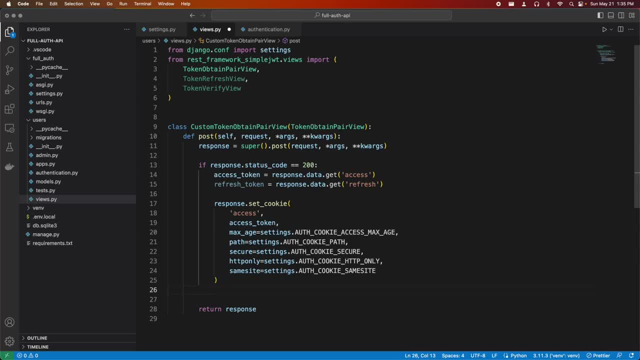 sending of these cookies to work with the access token and then i'm also going to have response dot set cookie and then i'm going to have the access token, which will be the same site which is going set cookie for my refresh, which will be my refresh token, and then the settings will all be very 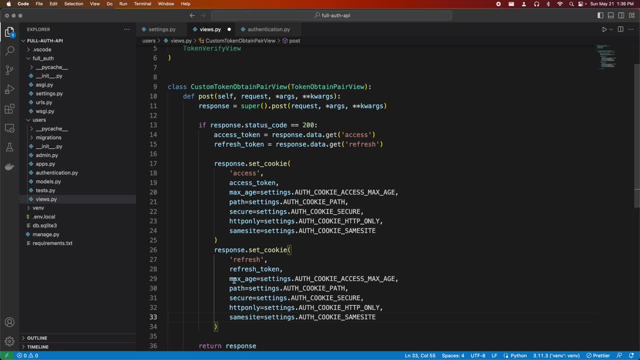 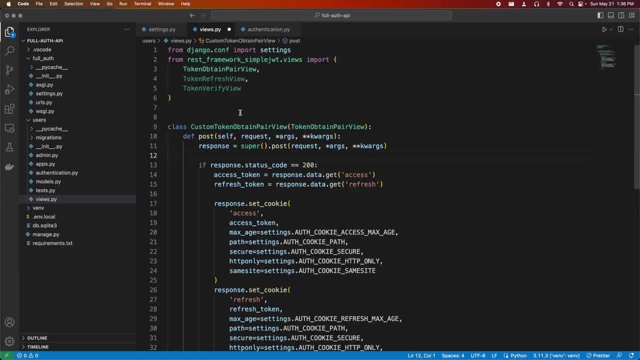 similar, so i'm just going to copy this and paste it. the only setting that's different is the max age, so that one is going to be auth cookie refresh max age, so that's going to be that 24 hours instead of the five minutes for the access, and with that we overwrote this one. so now we just have to do. 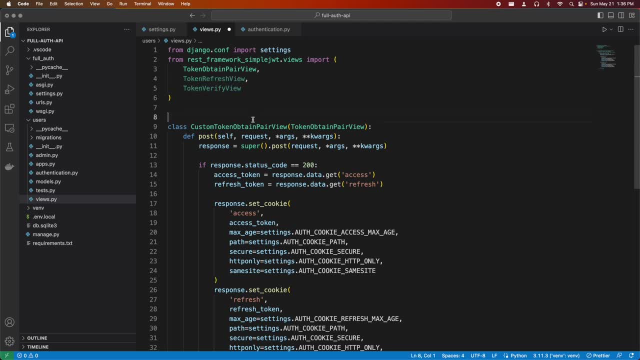 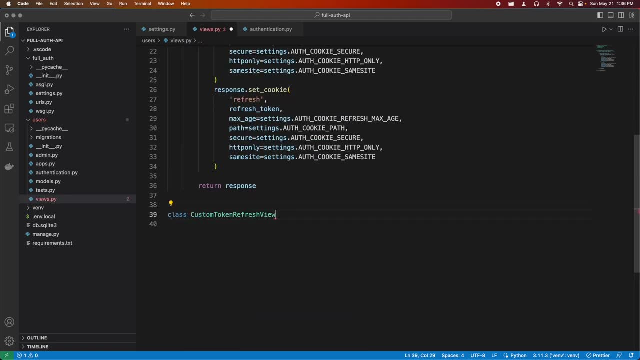 the rest for the refresh and the token verify. so let's go ahead and do that. i'm going to copy this, i'm going to scroll down and i'm going to create another class which will be my custom refresh view or, i guess, token refresh view. i'm just going to override the token refresh view, so 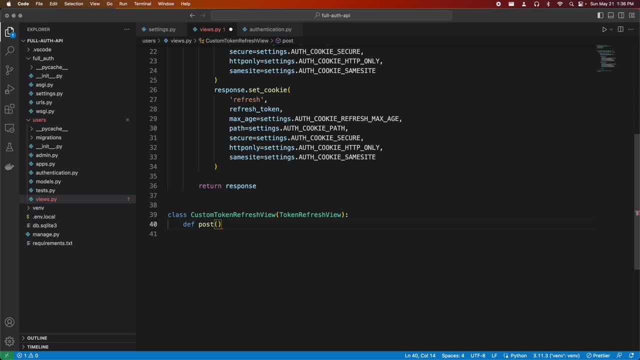 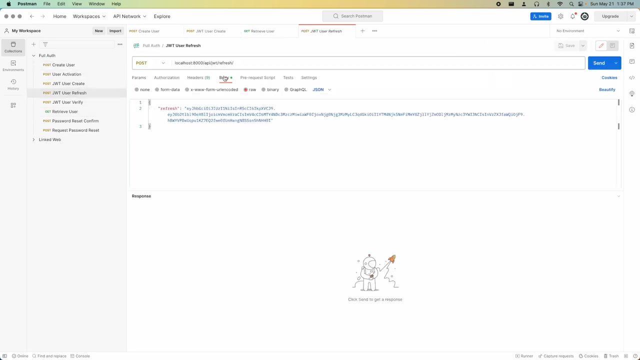 we're just going to inherit that and then we're going to override the post and then for the refresh view- so remember, inside of postman for our refresh, so we receive the refresh in the body, and then it's going to send us back in the response and access token and it's going to be 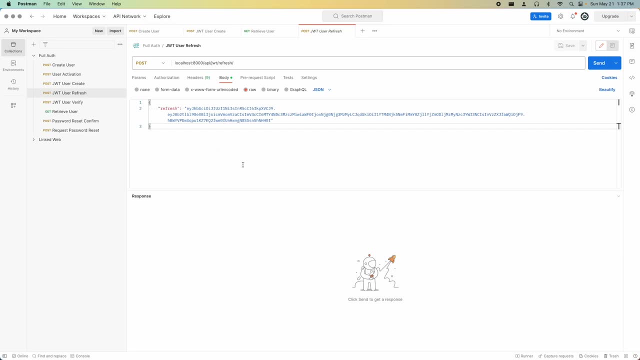 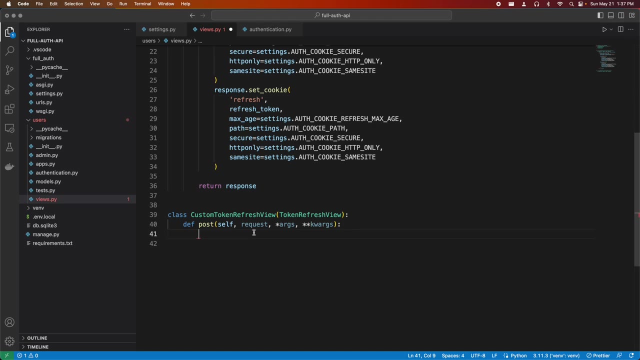 inside of like json data in the response, but instead i want to have that access token get set inside of the cookies. so, going back to the code, what i can do is i can grab the refresh token from the request and in this case we're going to have this refresh token be present in our cookies. 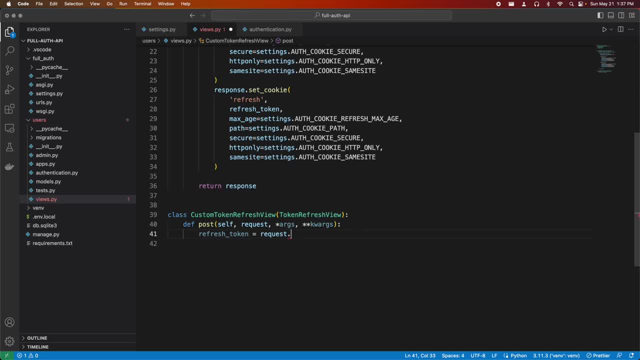 so what i can do: instead of grabbing it from, like the body data, i can grab it from cookies. i can do cookies dot get refresh and then if we have a refresh token, then we're going to set request dot data refresh to be the refresh token and then we're going to call the token refresh. 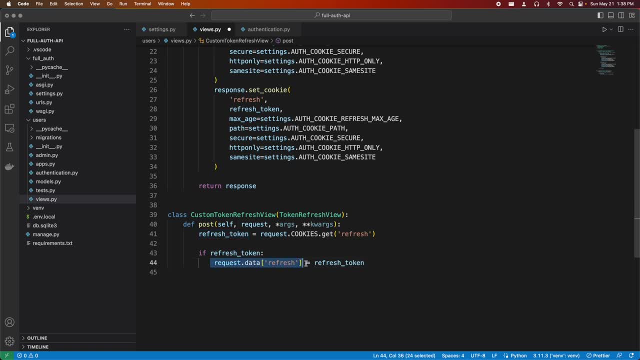 views post request and then we're going to have this inside of the data. so we're going to grab it from our cookies, put it in the data and then send the request off. so response will be the super class post request args and keyword args, and we'll do that. 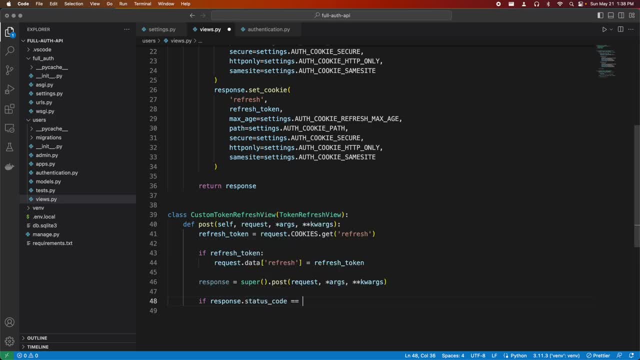 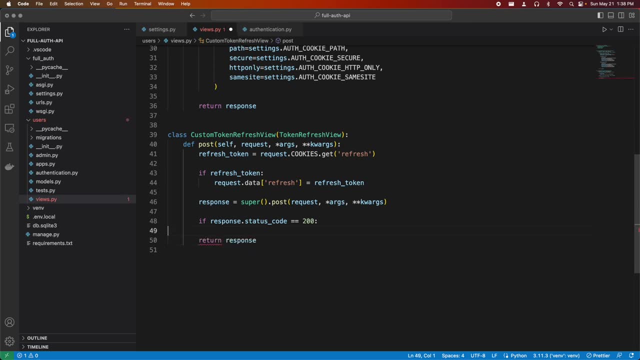 once we have that we're going to check, is the response status code 200? that means it was successful and eventually we're going to return the response. but before we do we want to set our access token. so we're going to get the access token value, so the new value, after hitting this. 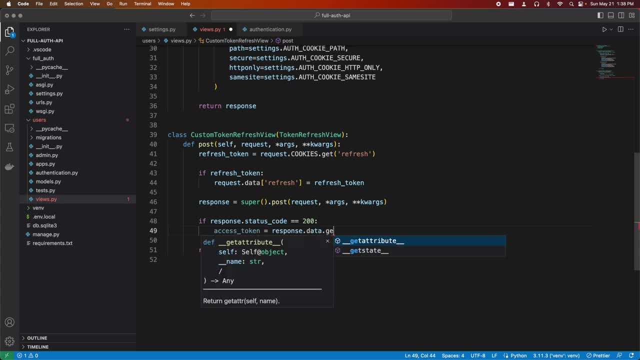 and that's going to come from response: data get access and then from there we can just do our response: set cookie, and then we're going to go ahead and set our access token value, and then we're going to go ahead and set our access token value, and that'll look pretty much the exact same as this. 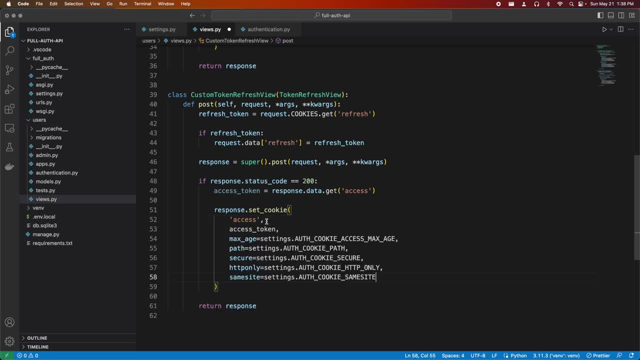 right here. i'm just going to copy this and paste it here, and there we go. now we don't have to do anything with the refresh token. now there are settings you can set in simple jwt. so when you hit your refresh endpoint, you get back a new access token and a refresh token. so this in 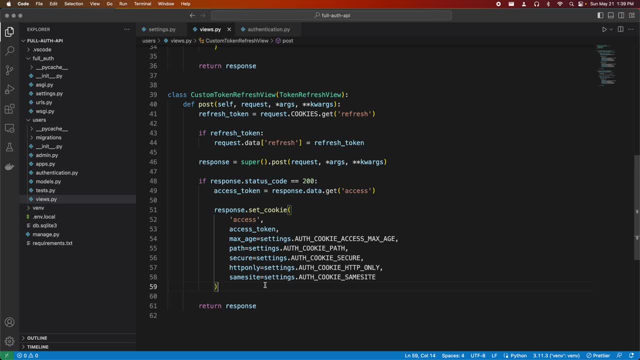 particular has to do with rotating tokens. so that's one of those settings there and then, if you do that, then you could also get back a new access token and a refresh token. so that's one of those settings there and then, if you do that, then you could also get back a new refresh token and set. 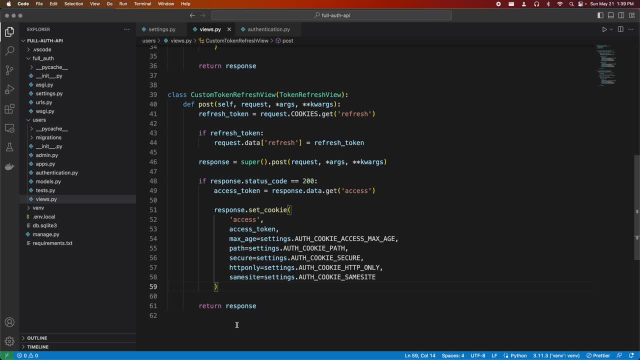 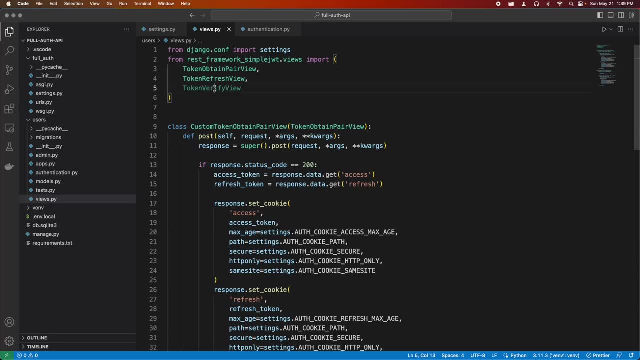 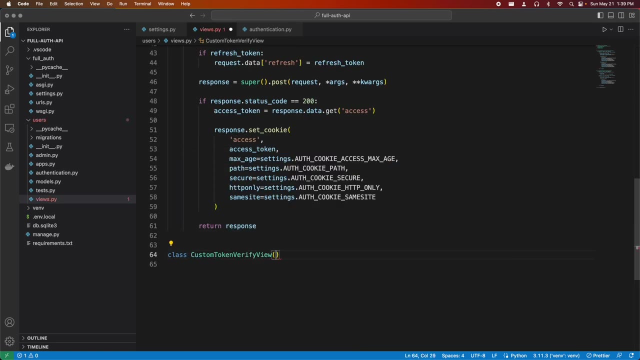 a new refresh token, but i didn't set that setting, so this is the way i'm handling it, and then the last thing i have to do is the verify view. so i'm going to grab this verify view. i'm going to have a class for custom verify view or token verify view. it's going to inherit the. 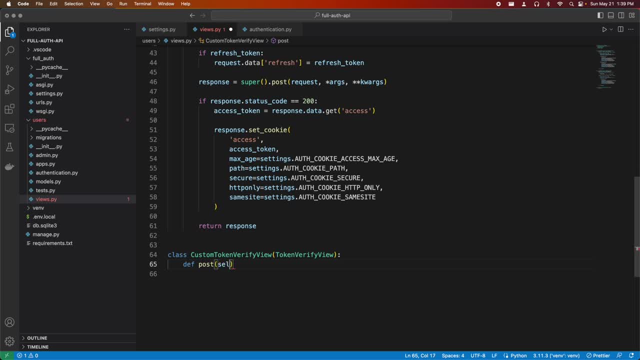 token verify view. it's going to be a post request with self request args and keyword args, and then this: right here, we are going to send this request to the token verify view with that token piece of data in the request, and then we're going to get the response, which is just going to be like: 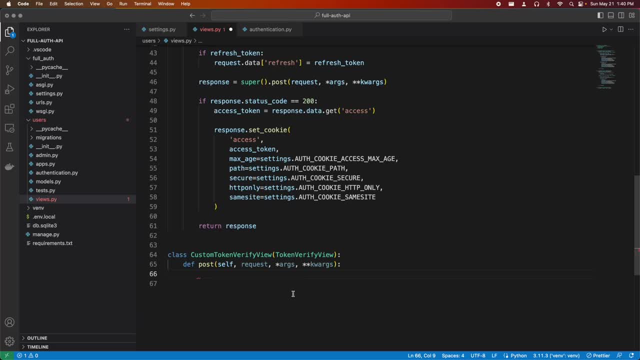 a 204- no content, if it was successful. so that's going to be what checks whether the access token is verified or not, which means that we are still logged in. so what i can do is i can grab access token from my request cookies access. then if i have an access token, then inside of the request data token. 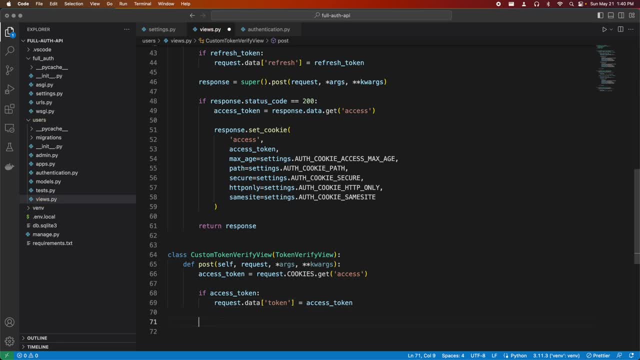 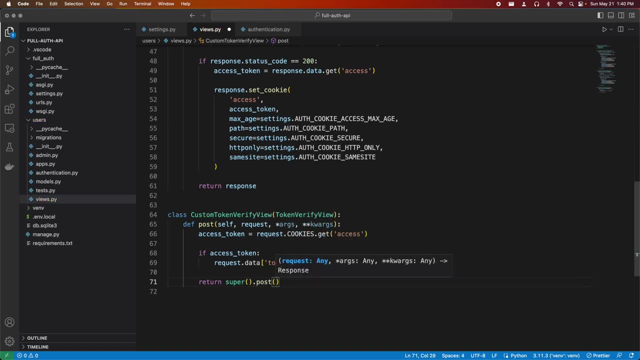 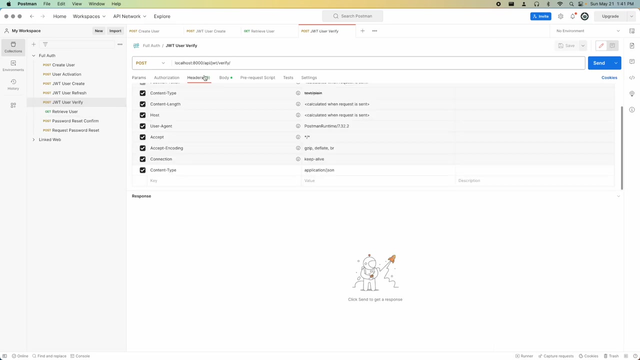 i'm going to place that access token and then all we have to do is return, calling the super classes post passing in request args and keyword args. so if we have this, we're going to put the access token inside of token, just like we did when we were testing this out in the body. we had this token. 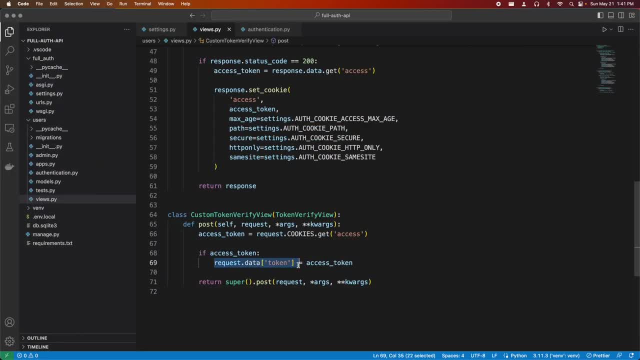 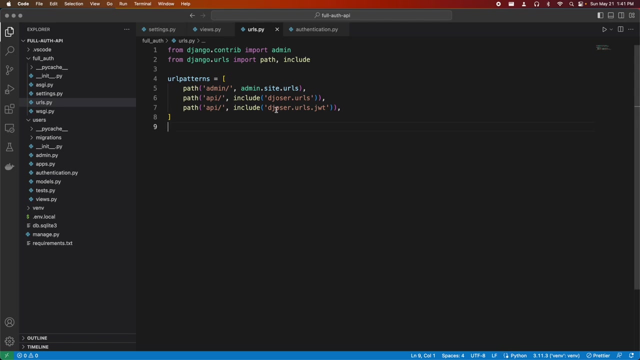 so now we're just grabbing the value from the cookies, placing it in the request body and we're just sending the request off to the token verify view, and that's how we deal with having these cookies. so now we have these, we're also going to set up urls and instead of using the joser urls, 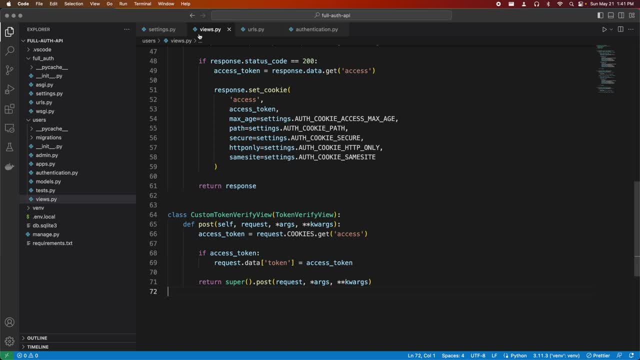 jwt. we're going to use our custom ones. but there is one more thing we have to do is we're going to do is create a log out view. so when you deal with json, with token authentication, the notion of logging out is more just like you get rid of your access token, your access token is what you. 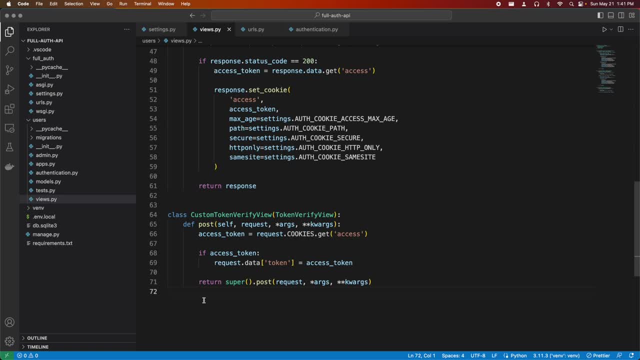 use to make authorized requests, and then, if you store it somewhere and you just delete it, now you no longer have that token, so you can't, let's say, make authorized requests. you're not logged in. so that's kind of the way that this works now. right now we're dealing with cookies. 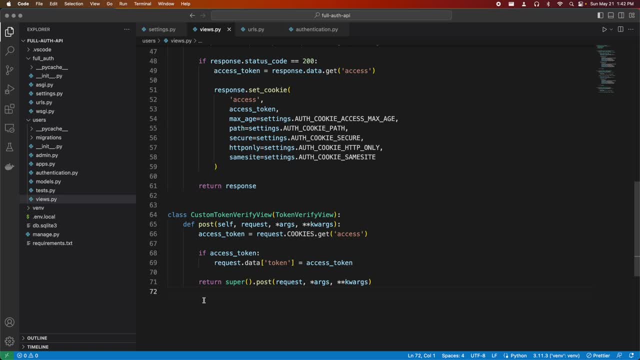 so one good way that we can deal with logging out is that our storage mechanism is that we have an access refresh token in our cookies and we just have to delete these cookies. so what i'm going to do to do that is i'm going to create a logout view. this is going to inherit api view. 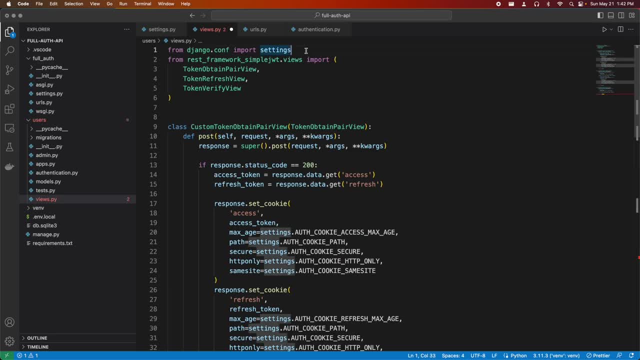 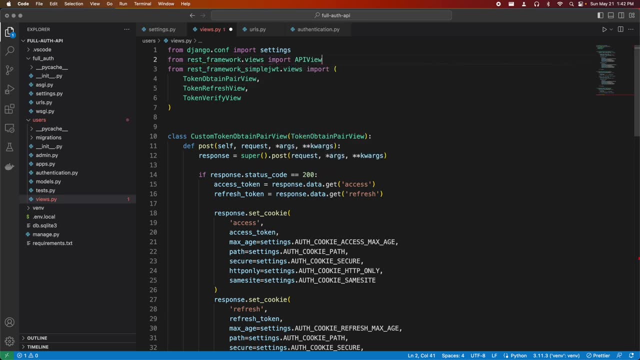 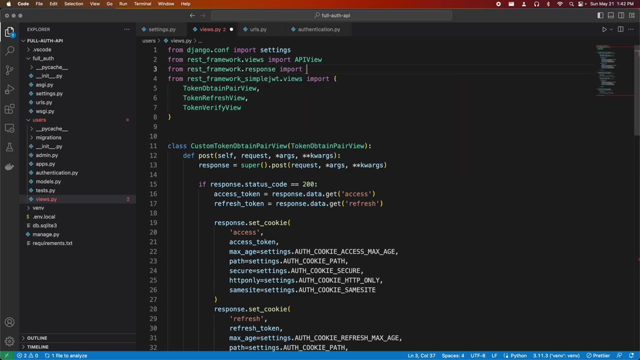 which i need to import. so i'll do that same here. so from rest framework dot views i'm going to import the api view. i'm also going to need a couple other imports. so from rest framework dot response i'm going to need response, and also from rest framework. 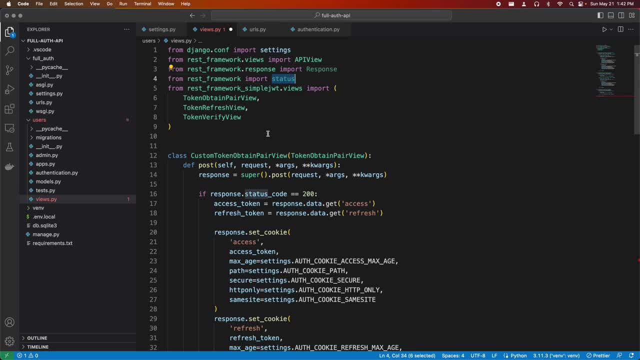 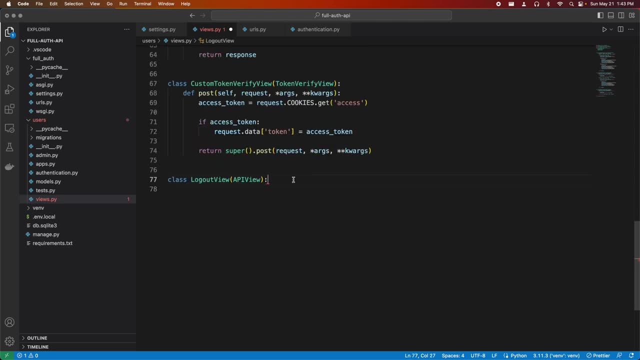 i'm going to need status. it's going to be for setting status codes in the response, so i'm going to scroll down and then this is going to be a post request. we're going to have to be authorized in order to hit this route and it's just going to delete our access and refresh token. 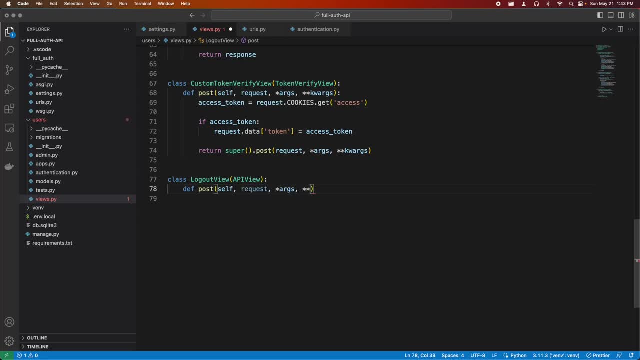 i'm going to pass in self request args and keyword args and then response. it's just going to be a response. we're going to have a status of status: dot http 204. no content. then we're just going to do response. dot. delete cookie. i'm going to delete access. we're also going to delete the refresh. 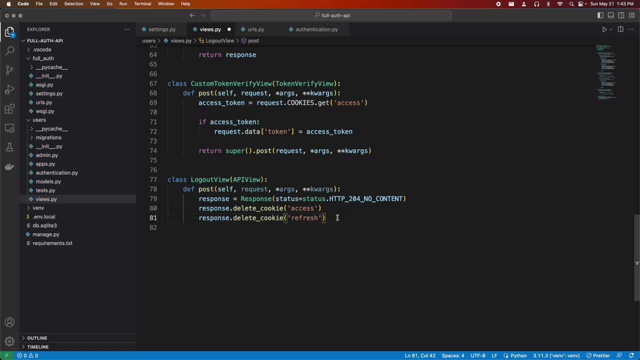 cookie. so this is how we do this in python with django, and then we're just going to return that response with our cookies being deleted, and there we go. so now the next step is going to be inside of users to create our urlspy file and create the urls for these custom views we created. 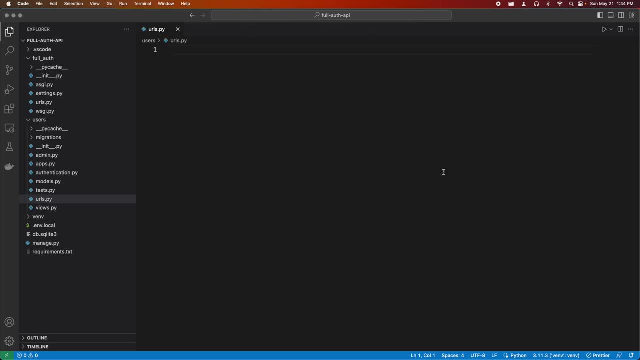 i'm just going to close up some of these other files i'm not using right now, so first i'm going to do is: from my views, i'm going to import these views. i made so my custom token: obtain pair view. custom token: refresh view. custom token: verify view. 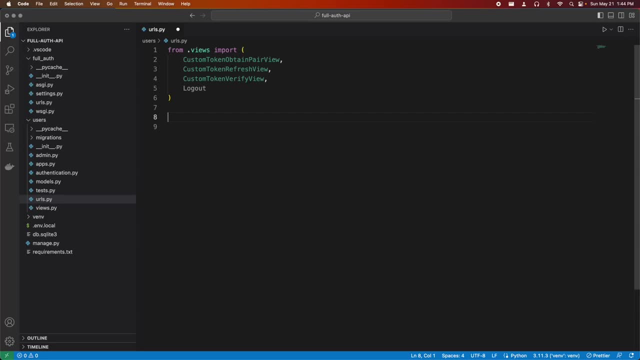 and my logout view. i'm going to make my url patterns- just going to be my list, and then here i'm going to have my different paths. so in the root i'm going to have api slash, and then i'm going to have here jwt slash, create slash. so it's going to be the exact same endpoints only. 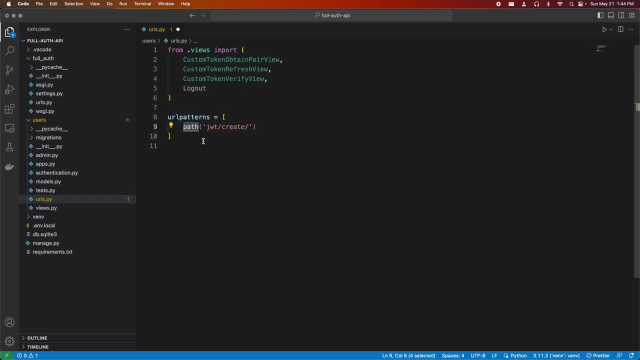 differences. we're going to use our custom views and then another thing i have to do is import path. so from django urls, that's where i'm going to import that- and then i can grab this view, paste it and do dot as view, because this is a class-based view, so i 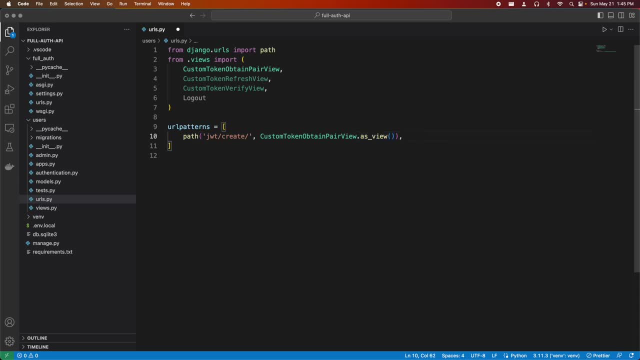 have to chain on dot as view. i'm just going to copy down a couple times, because i'm also going to have jwt refresh, which is going to use the custom refresh view, and i'm also going to have verify, that's going to use the token verify view, and then this has to have it, or where is this? 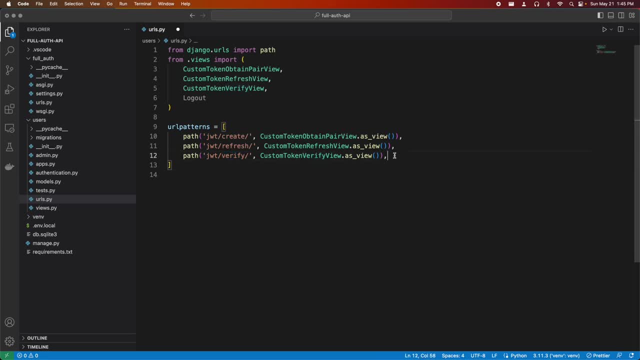 if i there, we go make sure that's spelt right. the last thing i'm going to need is my logout, so i'm just going to do logout slash. it's going to be with the trailing slash and this should be: log out view and then log out view dot as view. 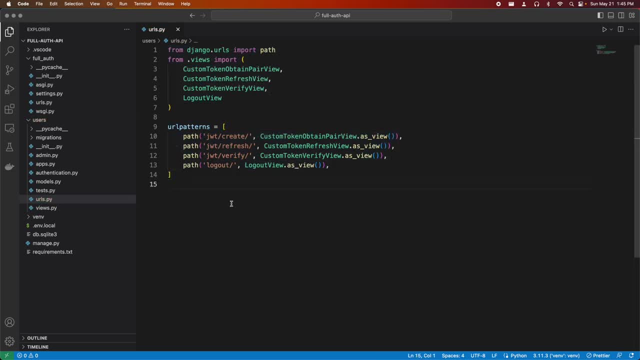 so there we are. we have our urls. the only thing we have to do now is go into our project urls and, instead of using joser urls, jwt now for our jwt endpoints, we're instead going to use our users urls. so this is our users app: the urls we just defined. 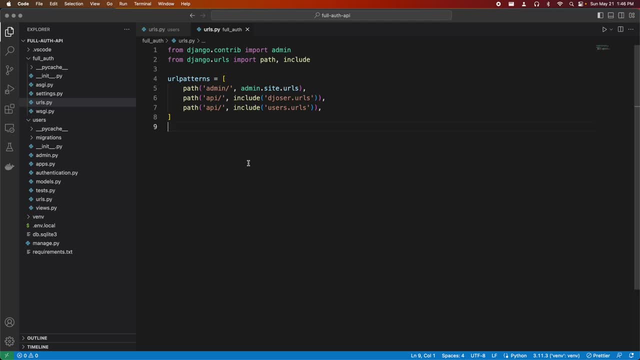 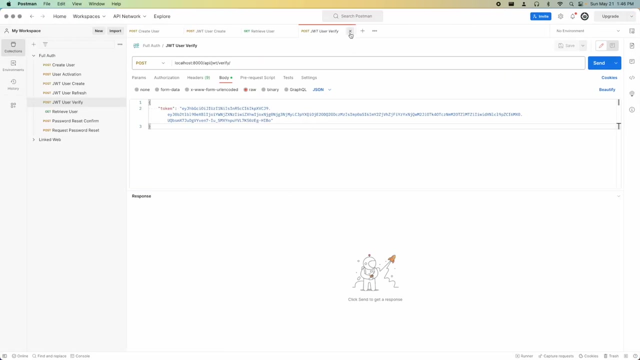 and there we go. so the last thing to do now is test out that this works. so just to be sure, since i added some settings, i'm just going to rerun my backend server, then i'm going to go to postman and i'm going to test this out. so first of all, i'm going to hit. 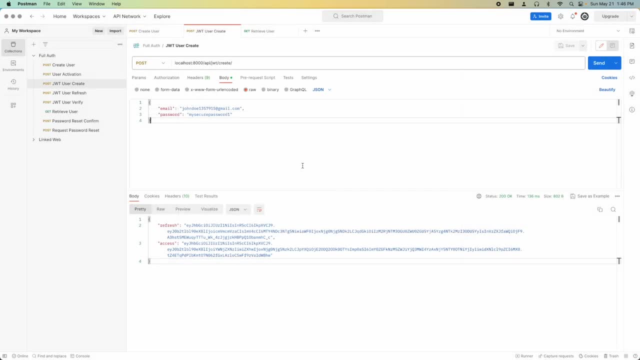 this create. so currently we don't have any cookies. now, if i send this off, we should have two cookies. so in our response we got the two cookies and then we have all the settings that we set. we have the domain default to localhost, so that's good. and then in here we also now have an access and a. 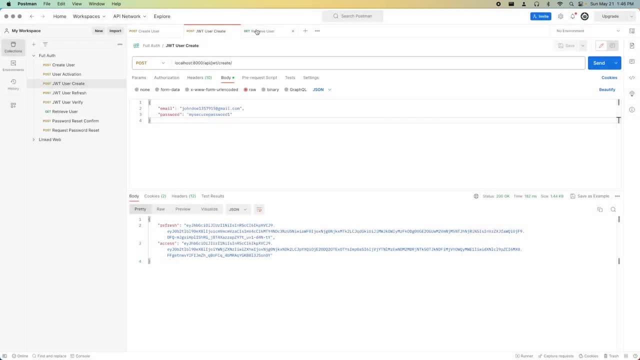 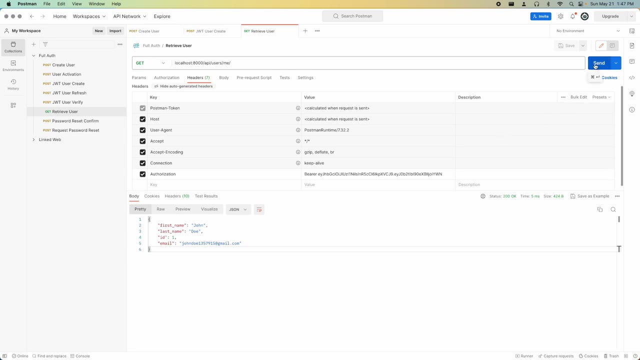 refresh token. so now with the retrieve user view, previously we were using the authorization header and we can still use the authorization header, although i can also not have it. send this request, and there we go, we get back our user. so this still works even without the authorization header. now. 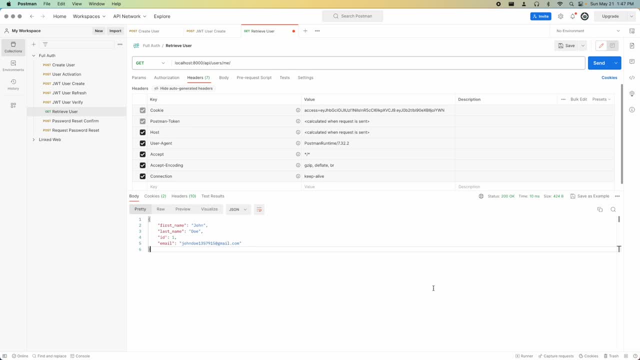 and this is going to make things much easier for us, because now we can have these credentials be secured in an http only cookie where the front end it cannot read the values of those values with javascript. but we're also going to have these automatically be getting sent in our requests from the front end and we're going to be able. 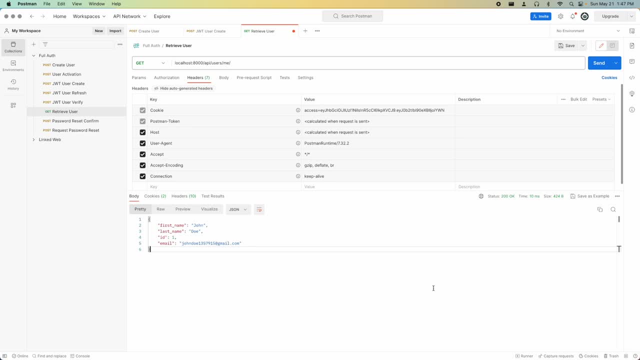 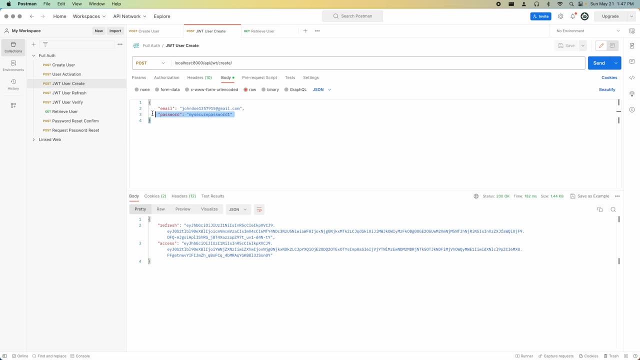 to use them to authorize any endpoint that requires authorization. so now in particular, the way this is going to change some things is here. we're still going to get back this data. now we can override this to not do that, but might as well also have the default behavior working as well. 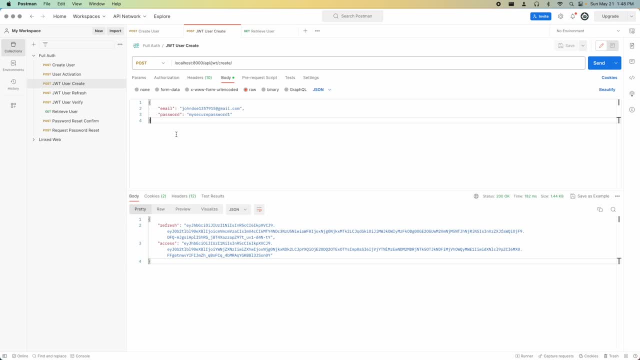 so you can use things just like you used before with simple jwt, but you also have this added functionality of the http only cookies storing the credentials. then in refresh how this is going to change some things. previously we needed to do this. we needed to have content type: application json. 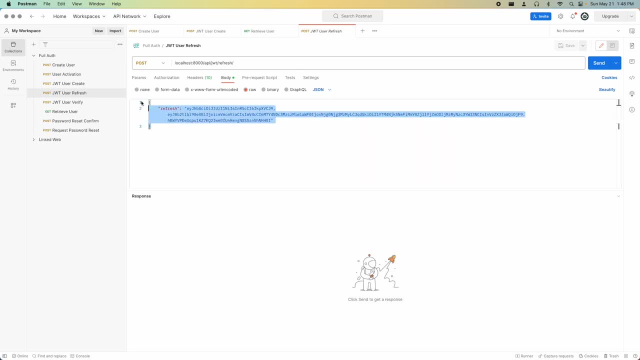 with the refresh, but now we no longer need this. i can just delete this and i can delete the content. type: application json. save that and i can save that, and now we're going to be able to use this. so i'm going to select this and i can send this, and it'll still work. i'll have the access token. 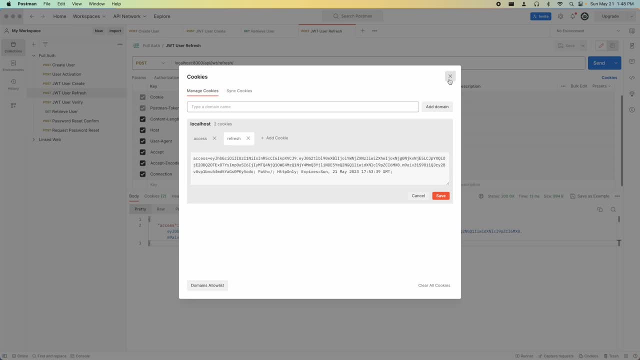 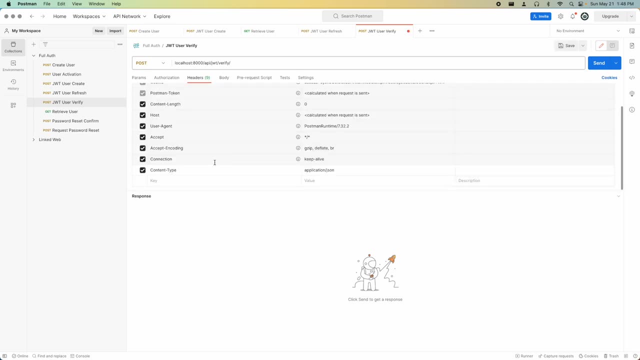 then in my cookies i'm going to get the brand new access token and it's going to get set here and same with verify. previously i needed this in the body and i needed the content type application json. i no longer need that. i can just send this off and there we go, 200. okay, this was verified, so our 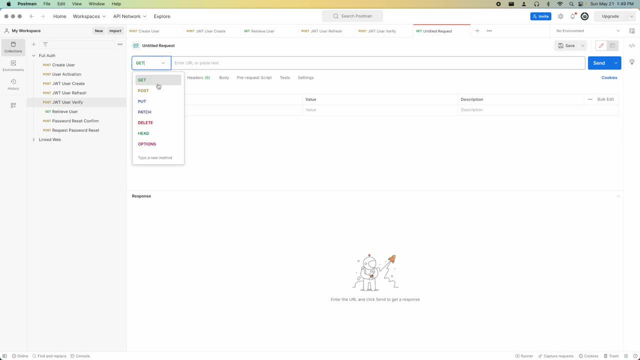 endpoints work, then the other thing we can now test out is also our login and login out. so you know, a post request: localhost 8000, slash, api slash, logout slash. it's gonna have the trailing slash. this will be my logout, or maybe user logout, and i can send this off. 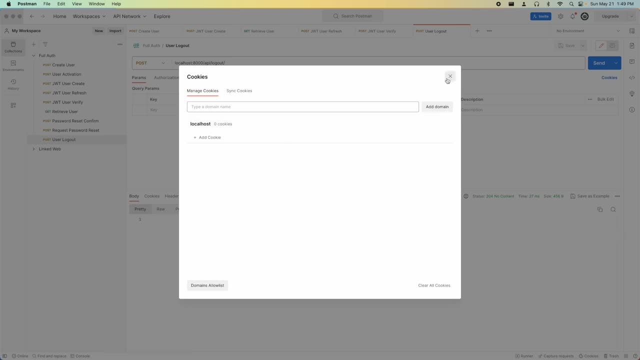 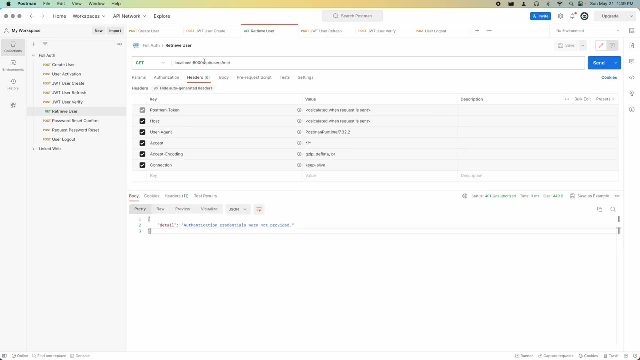 so i get a 204, no content, and my cookies are now gone, which means that if i go to retrieve my user, i'm now unauthorized, and then of course, we can go create our user again. there we go. access refresh token are here again, and now retrieving the user will work. so there we are. 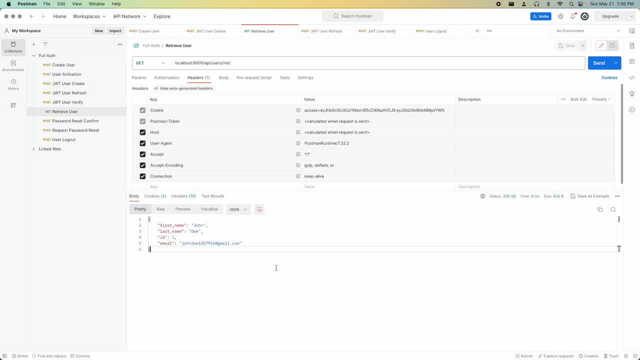 we've now successfully overwritten the behavior so that we can have these credentials stored in http, only cookies. now just one final thing to do for this back end and we're going to be all wrapped up. well, actually, not just one thing, because one thing we will have to do is set up 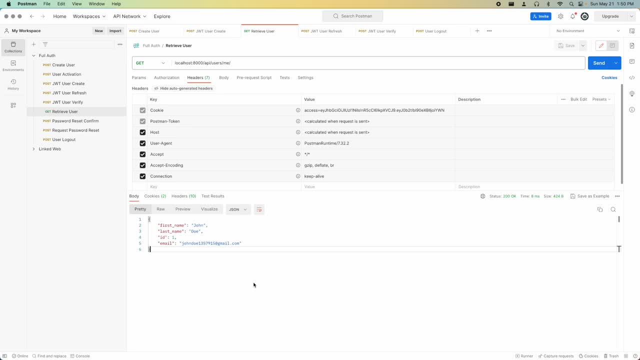 the user-referenced user-referenced user-referenced user-referenced user-referenced user-referenced- aloft with google and facebook. but we're also gonna have to go back and set up our static settings to use digital ocean spaces and we're gonna have to deploy this back. and so a couple. 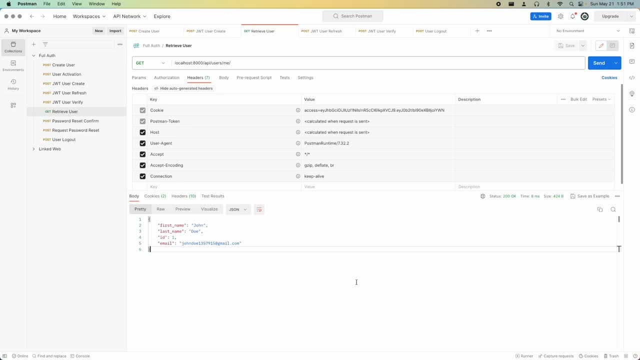 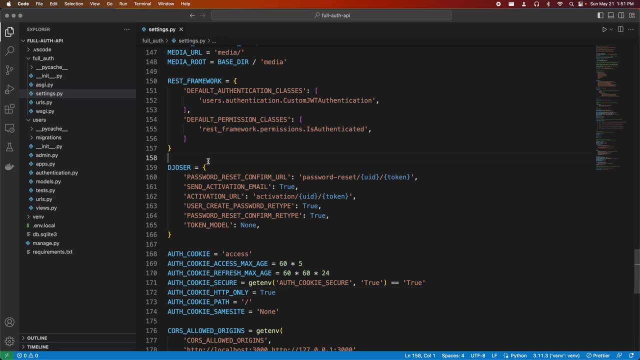 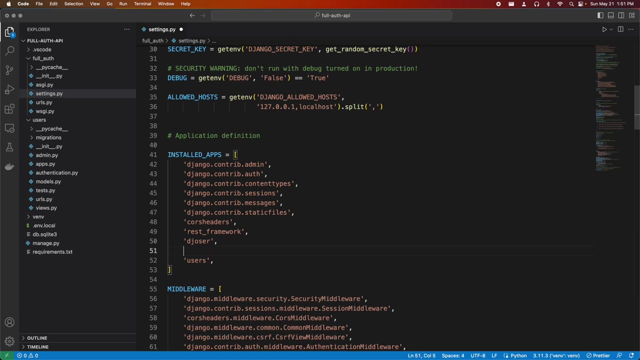 more things, but we're almost there, okay, so let's get started with setting up allot in this project. so first thing i'll have to do is go into my settings and then, inside of my installed apps, there is something else i will need, which is going to be social django. 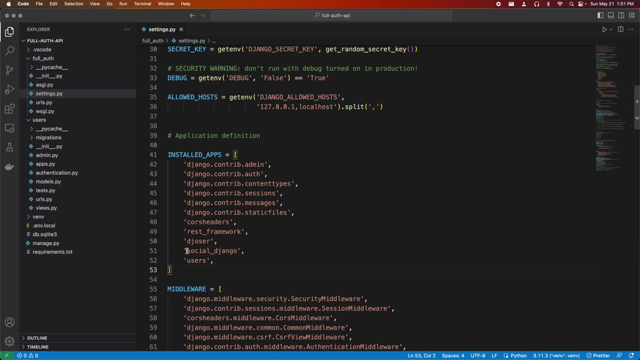 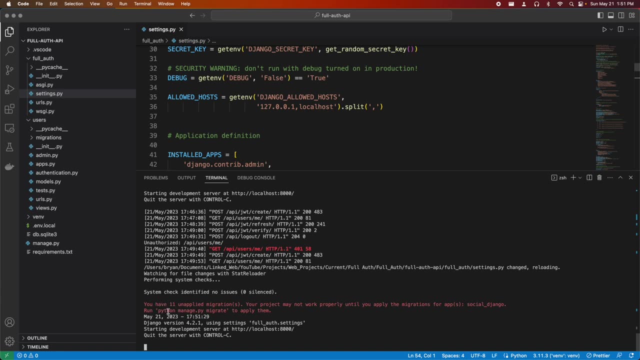 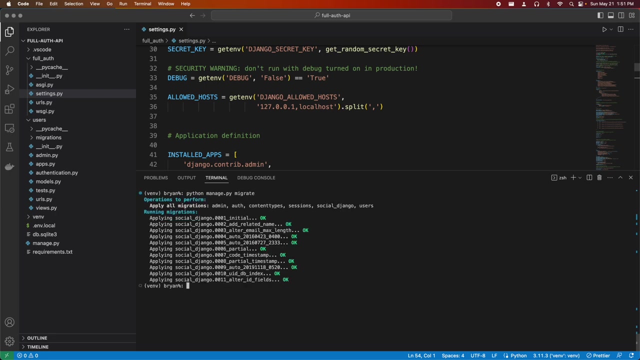 I'm going to save that now when I put this here. there are going to be additional migrations I'll have to make and I guess, in particular, I'm going to have to migrate. I'm going to stop running this. I'm going to do a python, managepy, migrate, and that will migrate things from social django. 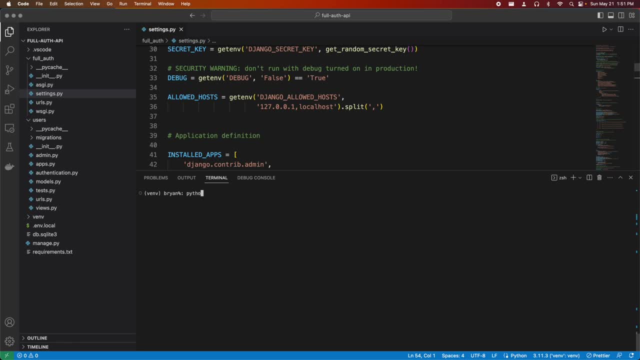 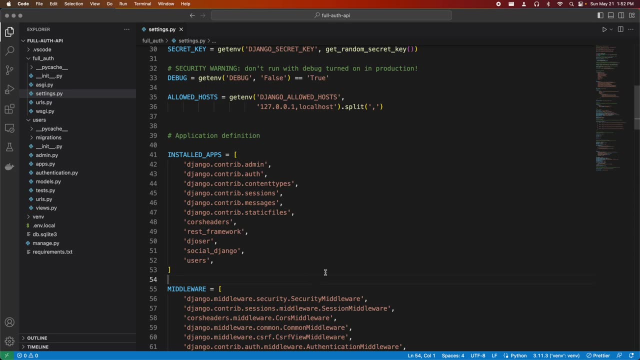 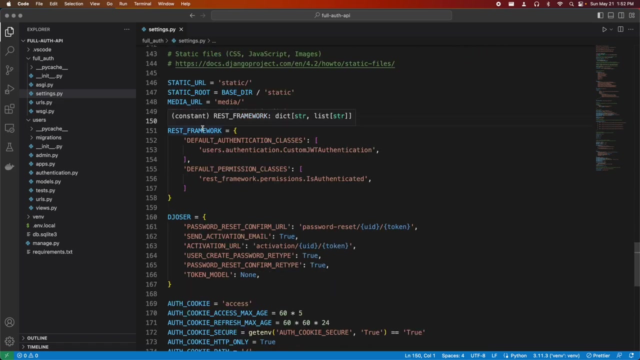 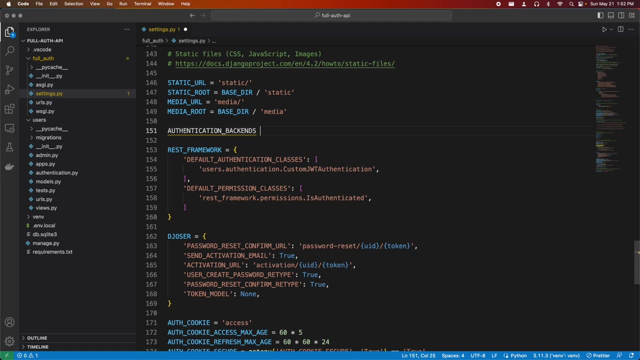 to my sqlite database and after that I can rerun and then after that we're going to have some settings we're going to have to set. so I'm going to scroll down and say, right above rest framework, I'll put authentication backends, which will be a list, and this is where I'm going to set up the backends. 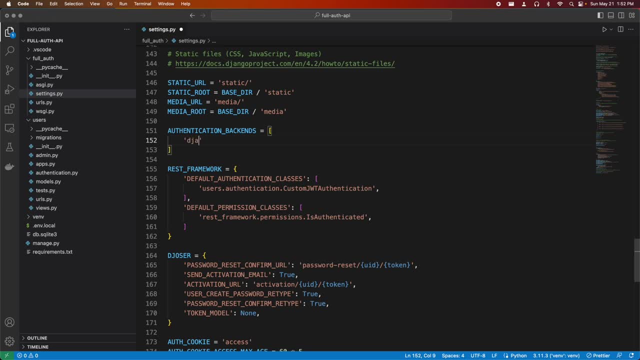 now we're going to have one in here which is going to be django contrib authentication auth backends, model backend. so this one here is going to make sure that our default behavior we have right now works. that's going to be one of our backends, but we're going to have additional. 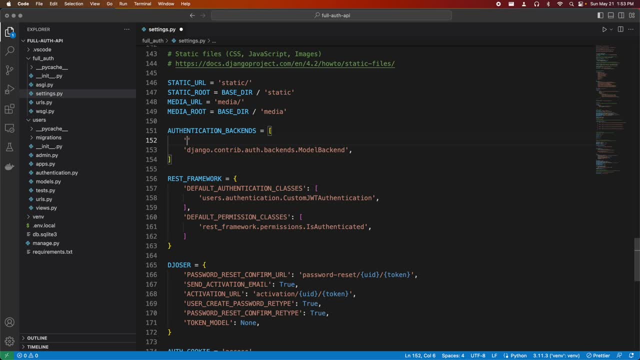 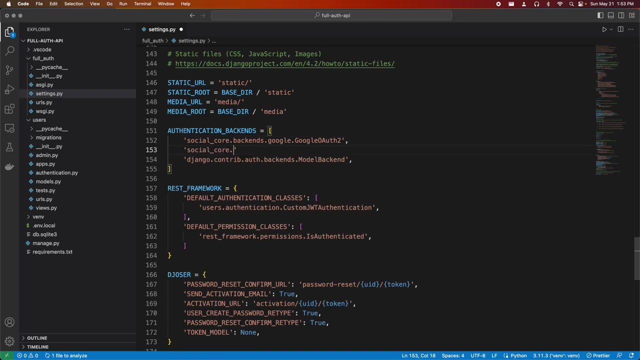 ones as well for the oauth. so the oauth ones are going to go above here. I'm going to have social core dot backends- dot, google, dot, google, oauth 2, and then we're also going to have social core backends, facebook, and then facebook, oauth 2. so that's going to set up these two as well, and then 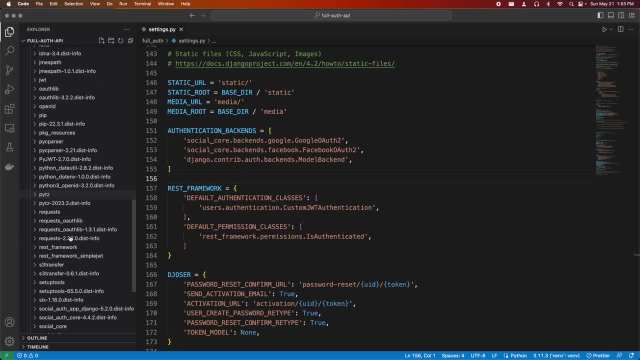 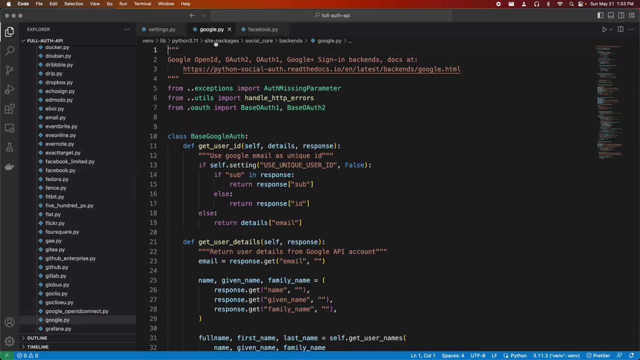 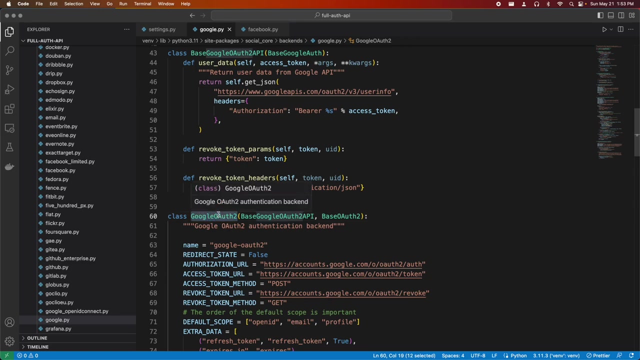 those you can even find inside of your virtual environment, because we have social core in here, and then we have backends, and then we have things like google, which is right here, and facebook, which is right here. so the base- google oauth 2, which is this one here- that's the one that we set up as one of our 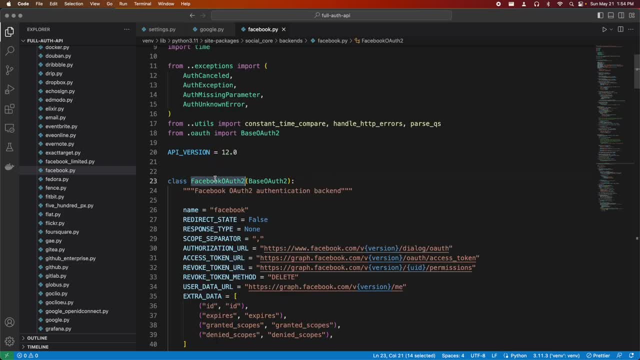 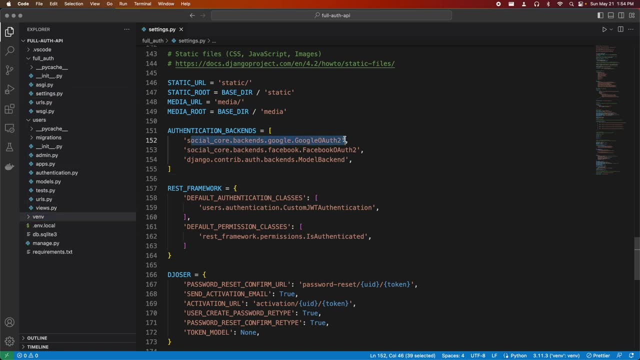 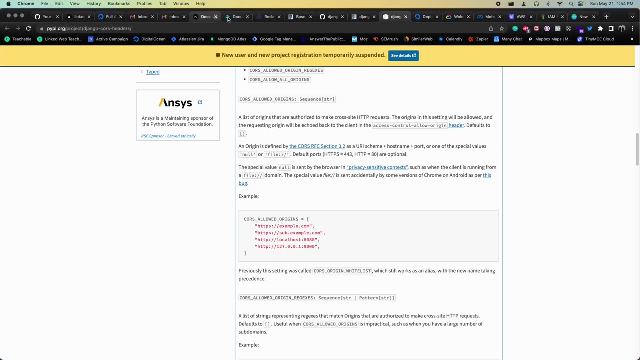 authentication backends, and then facebook, oauth 2 was the other one. so that's where these are coming from, just so that you understand how these paths work. and then the other thing we have to set up is with joser. so if I go back to the documentation for joser, just right here we have social endpoints. 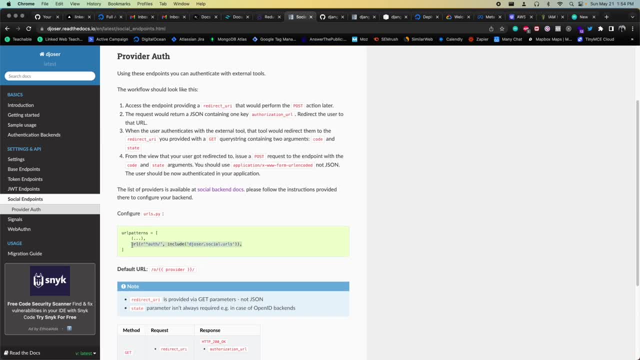 and then to set these up, you're going to go into your url patterns and then you're going to include joser's social urls. but the thing is, with these social urls it's kind of similar to what we had with the jwt, where when we get a response, we're going to get back the access and refresh tokens. 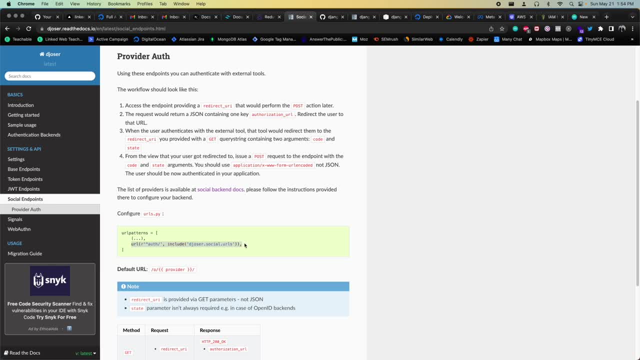 except those are going to be in the response data. I also want these to be stored in the cookies, so I actually will have to override the view that handles this social authentication and then part of my users urls. I'm going to have an endpoint which is going to do this like o slash provider. 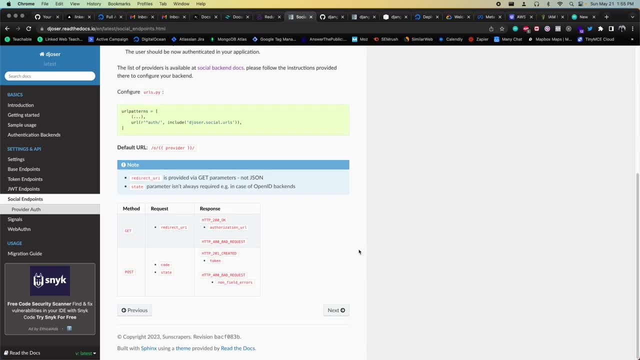 stuff. and then, if we look here, we're going to have two different kinds of requests that we make to have the social authentication working. we're going to have a get request which is going to give us a redirect uri which we can visit, and then, once we visit it, we're going to do things like 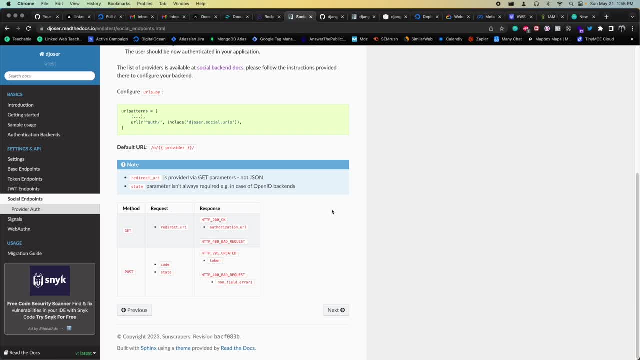 log into our google account or log into our facebook account and then we're going to get redirected somewhere. and then, for where we get redirected, we're going to set that up. that's going to be one of our joser settings we set up, we're going to get a code and a state and then we're going to pass those in. 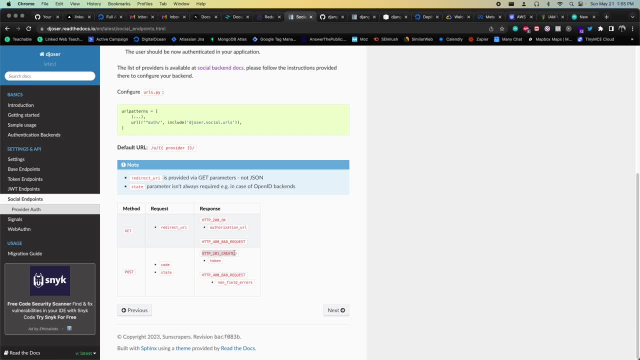 a post request and that is what's going to actually do our user creation and get us our access and refresh tokens. and then these also aren't going to be application json. right here it actually specifies we're going to have a json, and then we're going to have a json, and then we're going to. 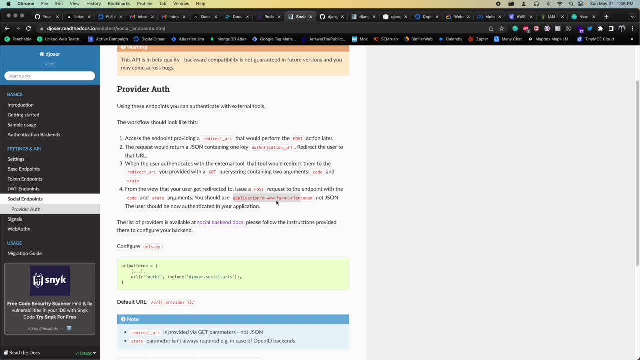 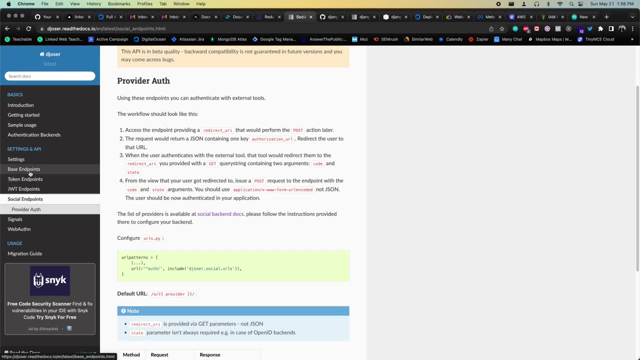 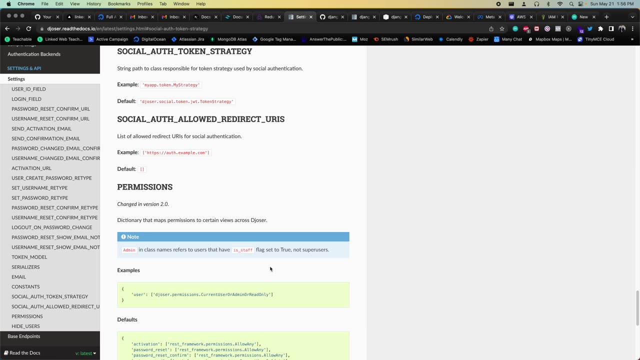 have application and then this x www form, url encoded format. so they're going to be inside of the url itself. so we're going to get to that, but before that i'm going to go to my settings and then here we have the auth token strategy. so that is right here. by default it's using this. 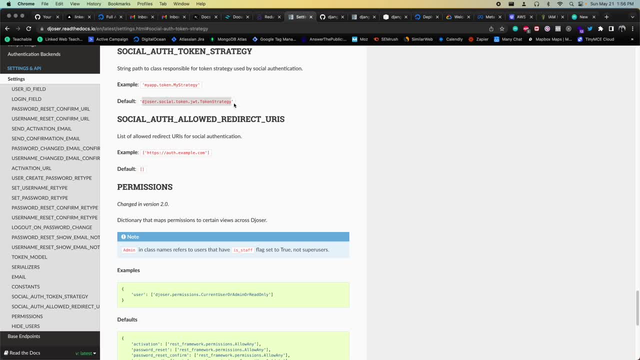 right here, which is the jwt token strategy. so that's actually what i want. so i'm not going to touch that setting, i'm just going to use the default. the other thing we need is social auth allowed redirect to our eyes. so by default it's empty. this is where we set where we're allowed. 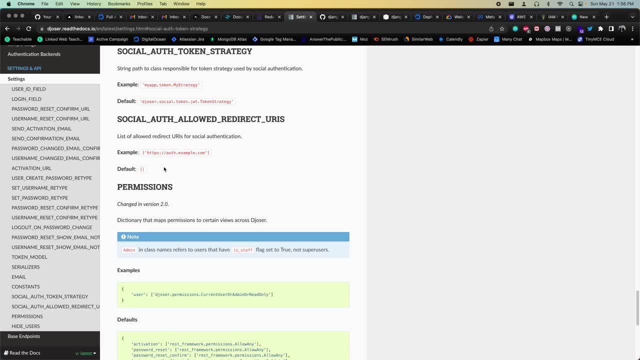 to redirect to which is going to be our front end app. so in development it's going to be low cost 3000 slash some endpoint that we're going to expect to hit which is going to make that post request, and then in production it's going to be our domaincom slash whatever that endpoint is. 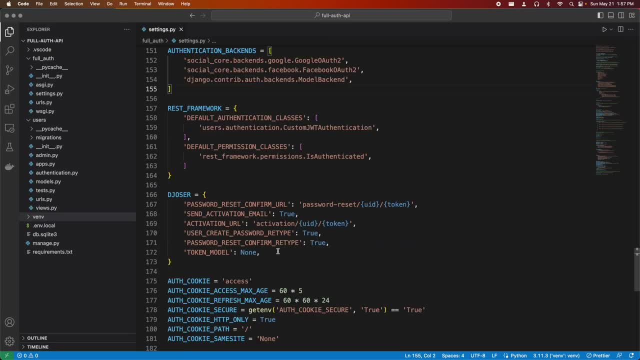 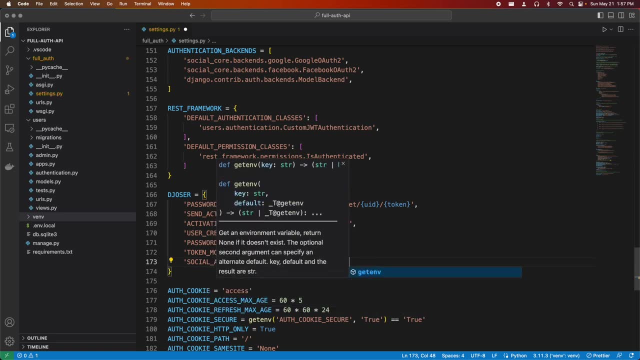 so i'm going to go back to my joster settings. i'm going to add this setting in here and then this setting. the way i'm going to handle it is: i'm going to get an environment variable called redirect urls and then i'm just going to do a split with comma- similar strategy to what we were doing before, because the setting 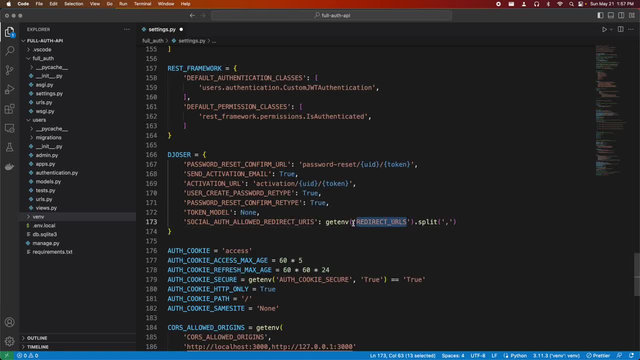 will be an array and this will just be a comma separated list. and then also just so that in my- actually maybe i will just have this in my development environment- yeah, that's how i'm going to do it. i'm going to have redirect urls. that's going to be my environment variable. 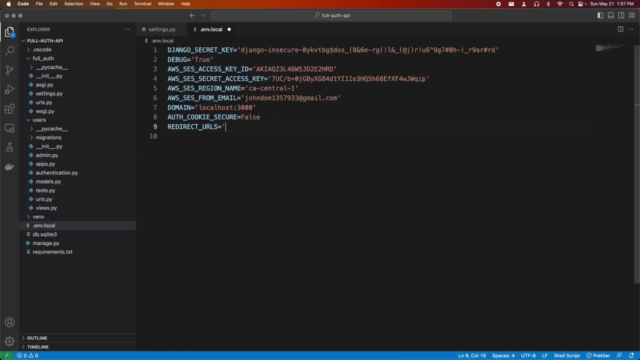 then inside of here it's going to be my comma separated list. i'm going to have http, local host, colon 3000, because that's where next gs will be running, and i'm going to have slash auth, slash google and then comma. i'm just going to copy this and paste it here and have facebook. 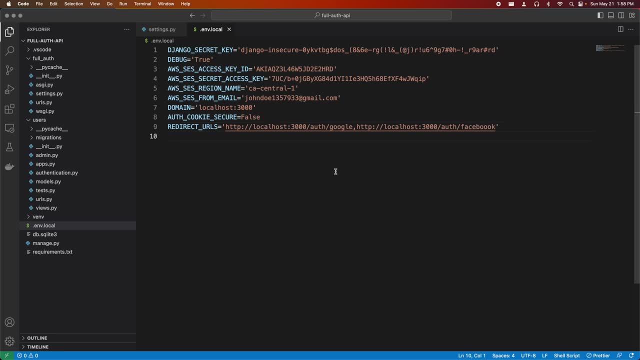 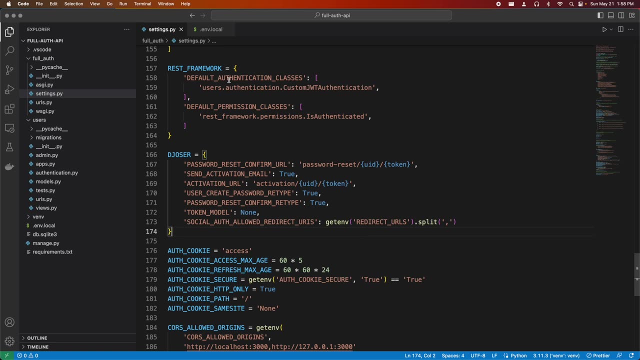 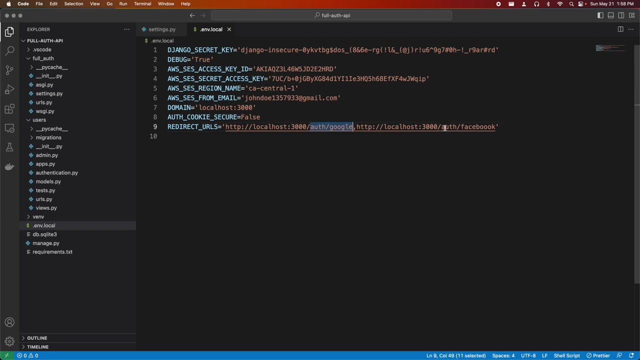 so then we're going to grab these values, we're going to split them into an array and that's going to be our redirect urls that we're allowed to redirect to. so i'm going to expect next js to have this route and this route and then this route. it's going to handle the post request for. 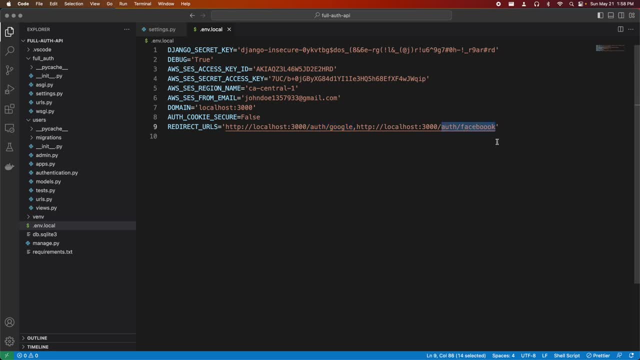 google oauth, and this one's going to be the post request for google oauth and this one's going to handle the post request for facebook oauth. and also here i noticed i put an extra o. let's try not to do that. so facebook. there we go. so this is all set up now and then because i set up some. 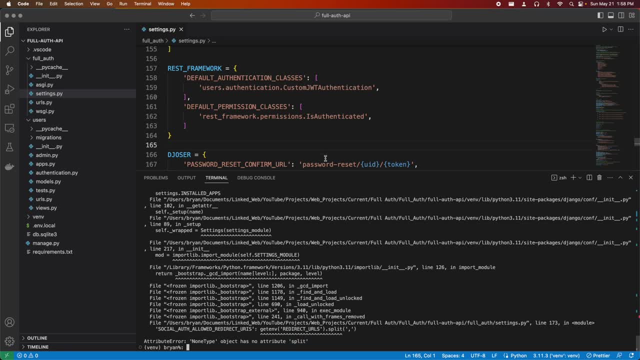 environment variables. i'm just going to rerun. also seems that we have an error on split and in particular that's because we got a none type that we're trying to split on, so that's not going to work. so once i rerun, we're actually going to have a string. 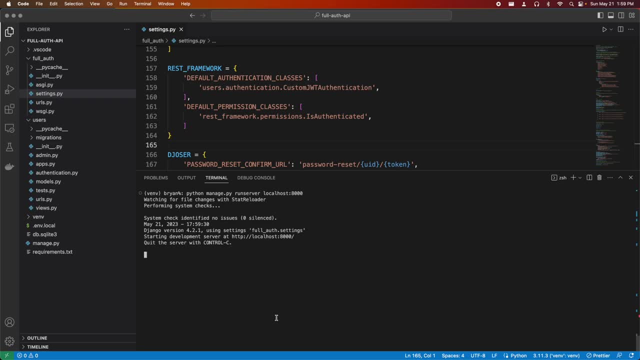 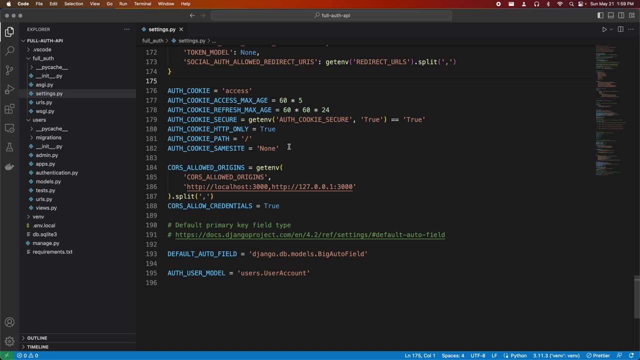 value and we're going to be able to do that split. so that's all going to work now and close that up, and then, after this, we're going to have some other settings we're going to have to set. so i'm going to set those, maybe right here. so one we're going to have is social auth google. 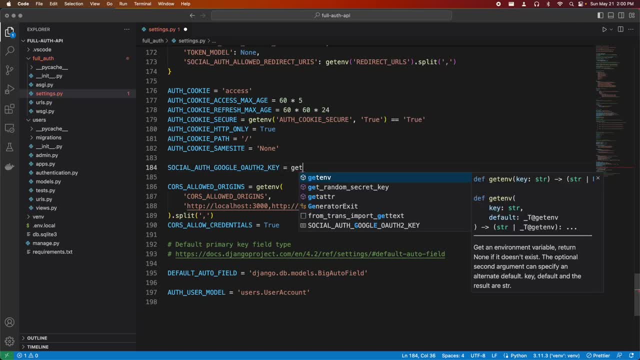 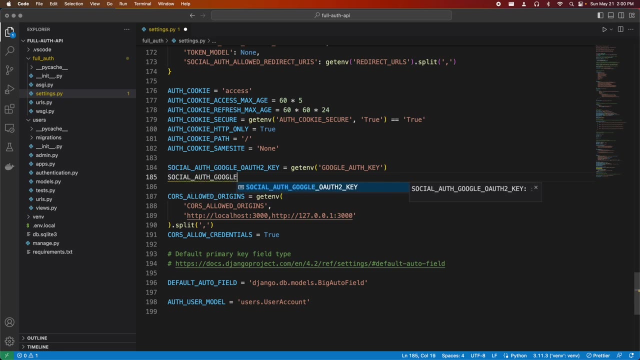 oauth2 key. we're going to get this from an environment variable which is just going to be, say, google oauth2 key. it's actually going to interact with google iw, or rather detect. so i'm going to give it, a'm going to tell you how to introduce it first. so i'm going to create it and i'm going to怎麼辦 it with. 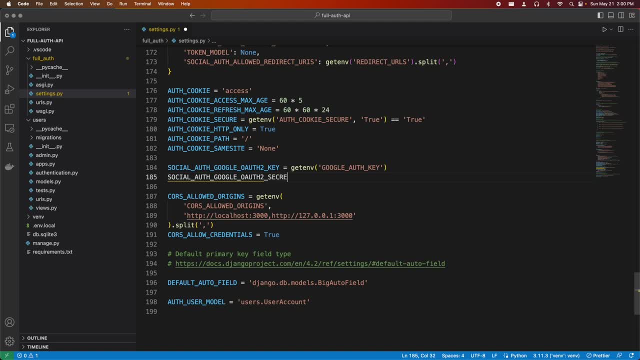 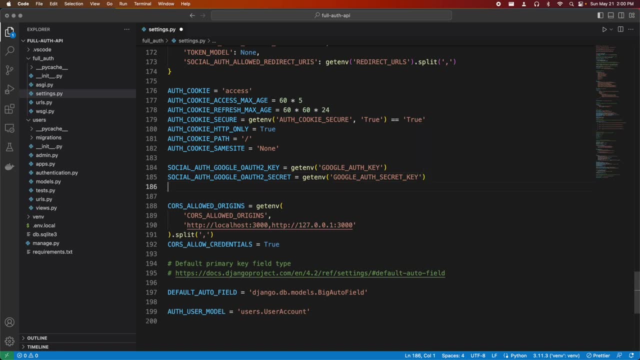 my local key. so if i find public key, then i want to select that key. so i plug this in and i'm going to enable the public key to activate. so i'm going to activate this and then i'm going to give it the public key. so, no, not. 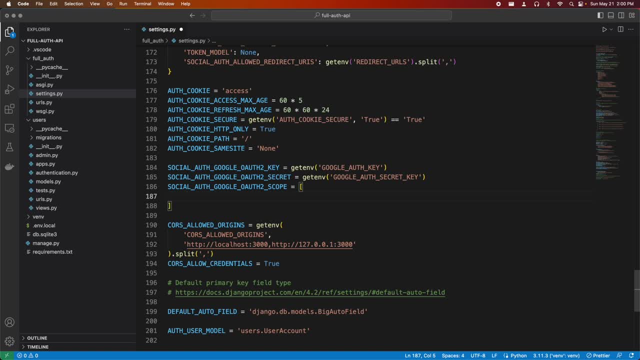 so i'm going to banish this in from then i'm going to press nt or tab on settings, gonna run the layout of the language that it supports. i'm not going to connect to the browser는데 brukbeker, google大家 dot. google apis dot com. slash, auth slash. user info dot email. i'm going to copy this down a line. 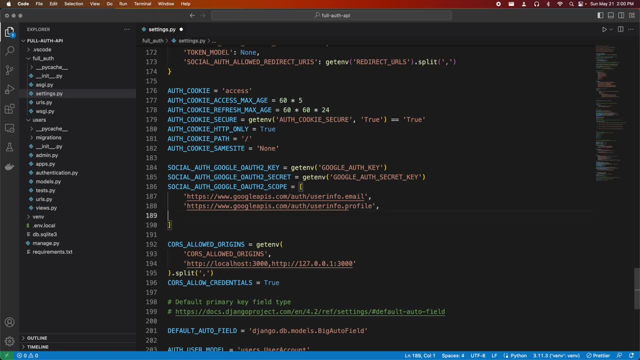 because i'm also going to have profile and then i'm also going to have open id. so these additional scopes are just going to let me get some additional values that i wouldn't get by default. so getting the email, first name, last name, things like that. i need to set up these scopes for. 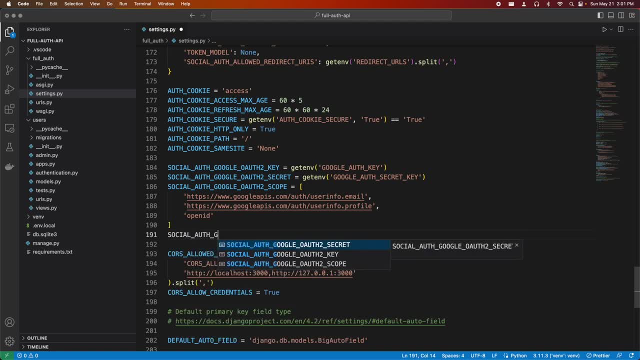 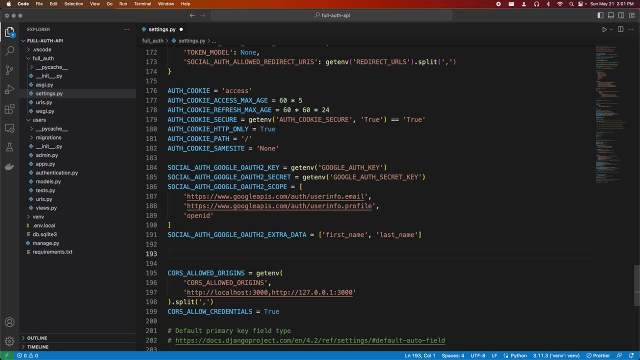 and then i'm going to have social auth, google oauth to extra data, which is going to be my first name and my last name, and then, after that, i'm going to have to set up the facebook settings. so i'm going to have social auth, facebook key. that's going to be an environment variable. 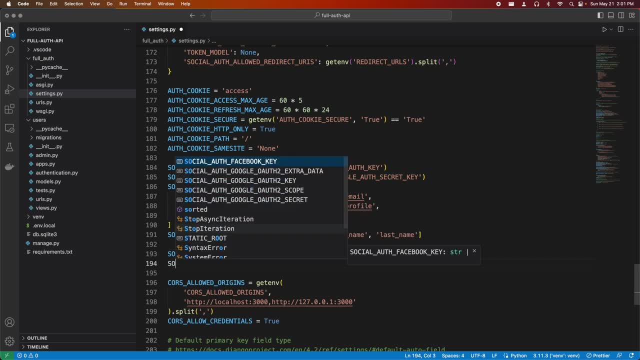 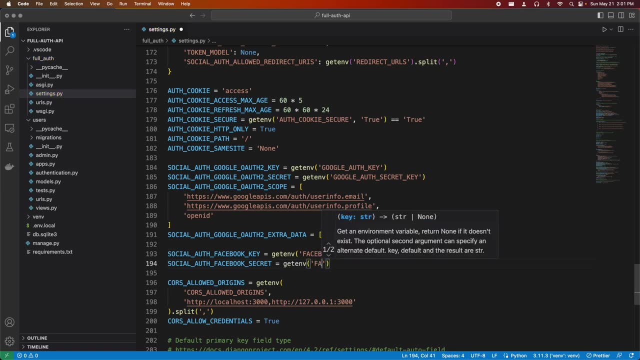 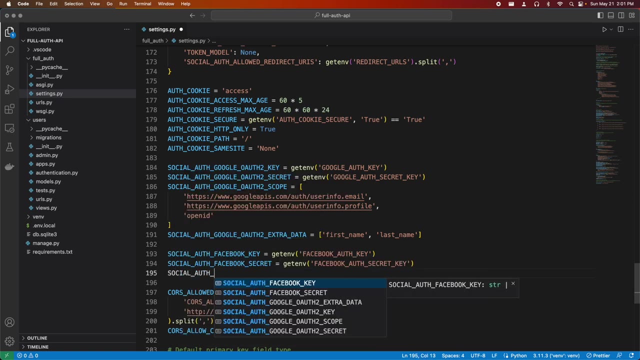 facebook auth key. so i'm going to have social auth facebook key. i'm going to have social auth facebook secret. so that's going to be facebook auth secret key and then social auth facebook scope. or i'm going to have email and then social auth facebook profile extra params. it's going to be a. 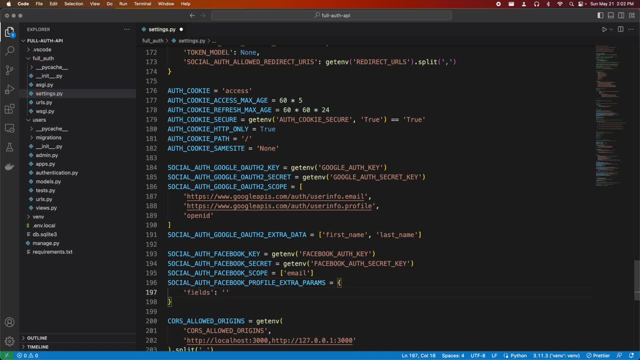 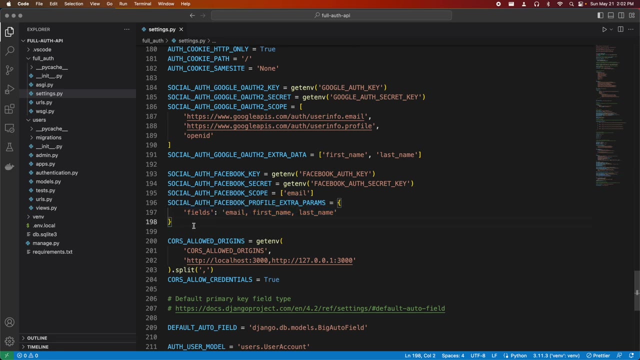 dictionary with fields which are going to be comma separated, which will be email, first name and last name. so there we are, and then that way i can also retrieve the email first name, last name when i log in with facebook. oauth 2. so these are going to be all the settings. we need the next. 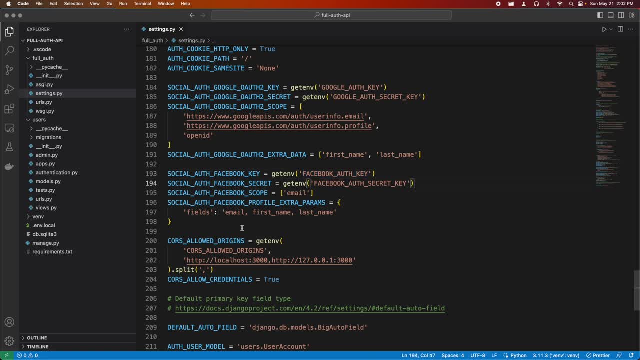 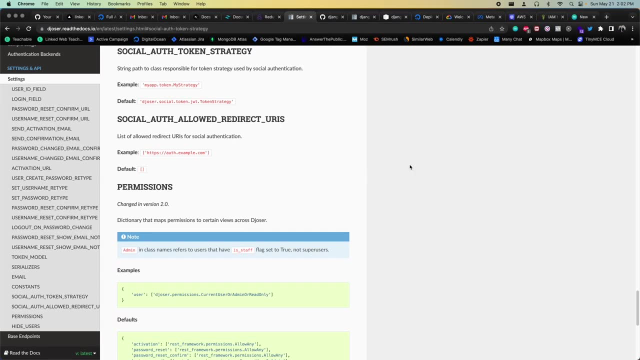 thing is going to be to actually get these keys so that i can actually do the oauth. so that's going to be our final step, and then we're going to have ourACE key, and then we're going to have our. we can test this out. so to do this, i won't need the joser documentation anymore, i believe, or maybe. 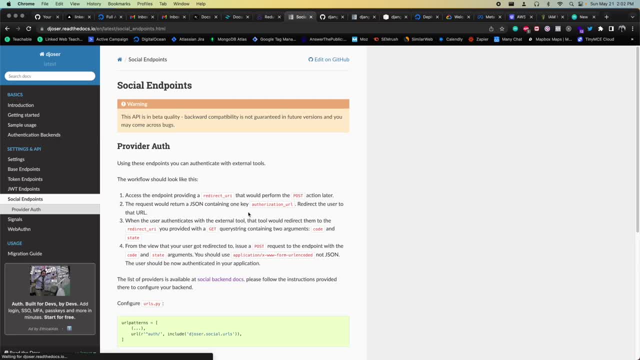 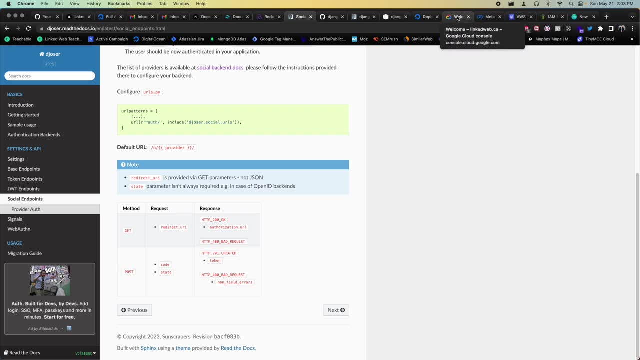 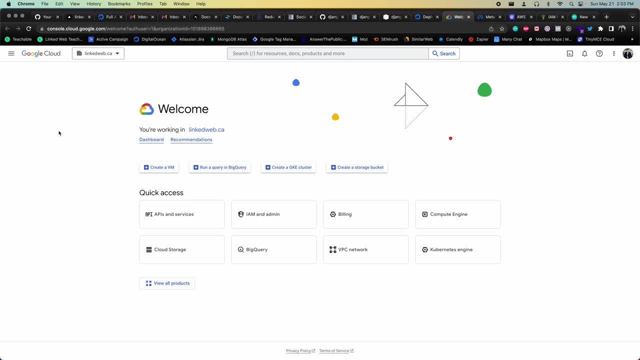 i'll leave it open just so that i can go back here and show this, and then what you're going to want to do is you're going to go to consolecloudgooglecom, you're going to log in with your google account and then you're going to create a project. 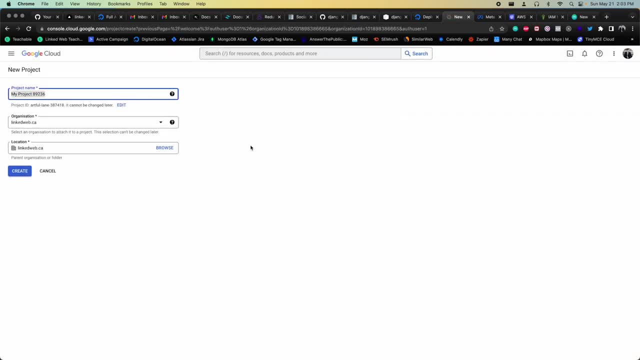 so you can do that by just clicking here, clicking new project. i'm going to call this full auth and create. you don't need an organization, you can do no organization. i just tab this here and that's going to go create the project. so we're going to wait for that to finish. 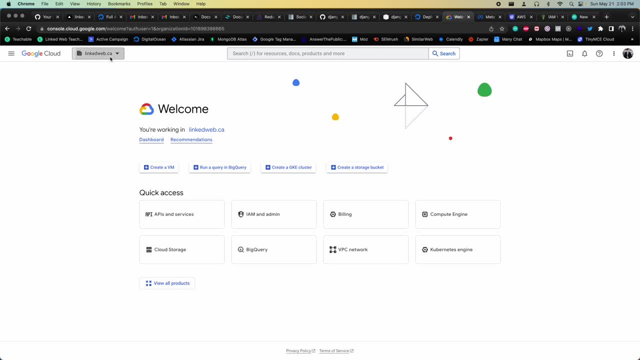 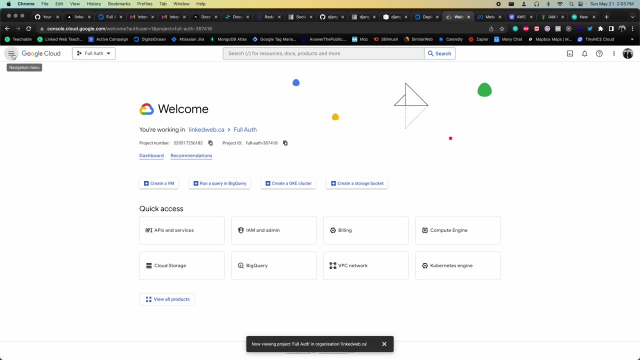 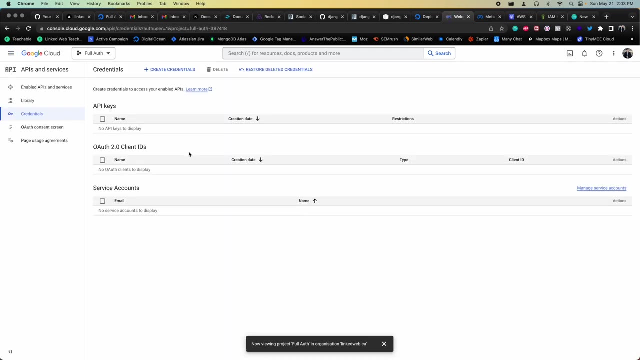 there we are. so after that you can navigate into the project. so once we see full auth here, we know we're in the project and then we're going to go to apis and services and credentials and this is where you set up your oauth login credentials. so that's going to be right over here now. before we do that, i'm going 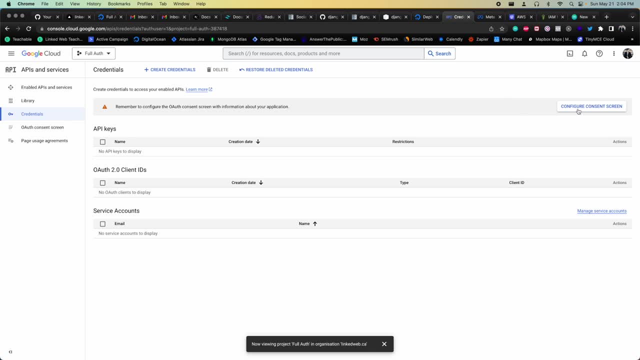 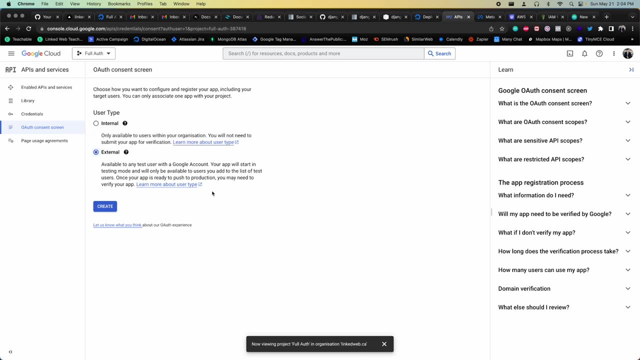 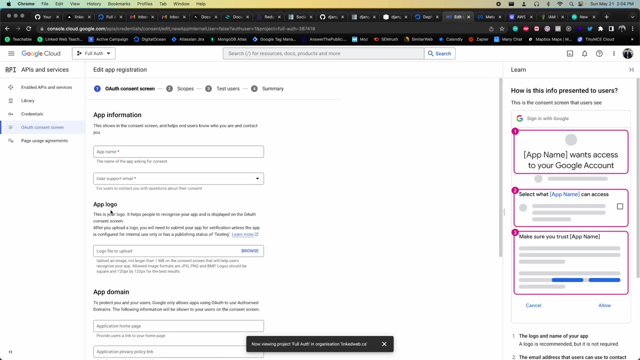 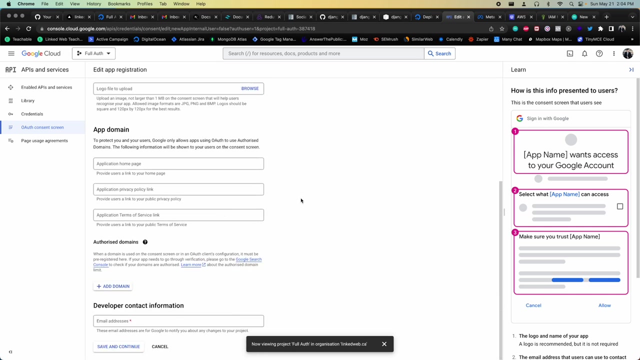 to do this consent screen, since i'm getting this popping up. so configure consent screen and here, for user type, it's going to be external. i want users outside of my app to log into my app using their google account, so that's going to be this. my app name will be full auth. i'm going to have my support email and then these settings. 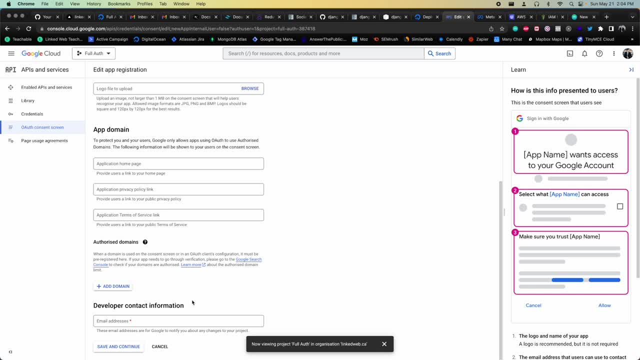 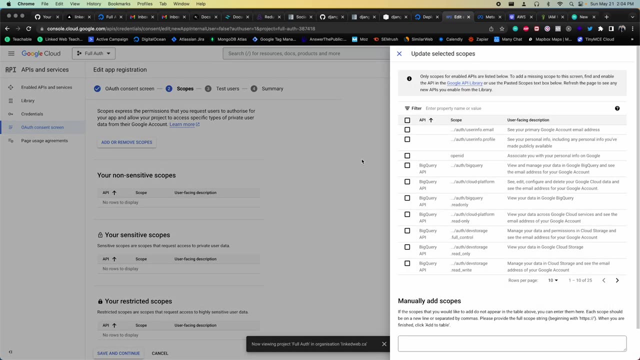 you don't have to set up. you can have authorized domains which we can get back to later, and then developer contact email. i'm going to save and continue and after that i'm going to add some scopes. so that's going to be these three scopes here. 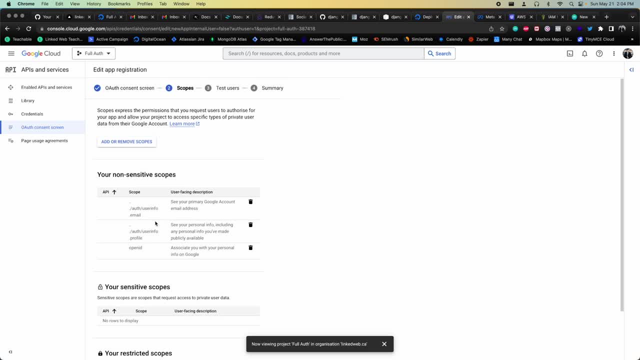 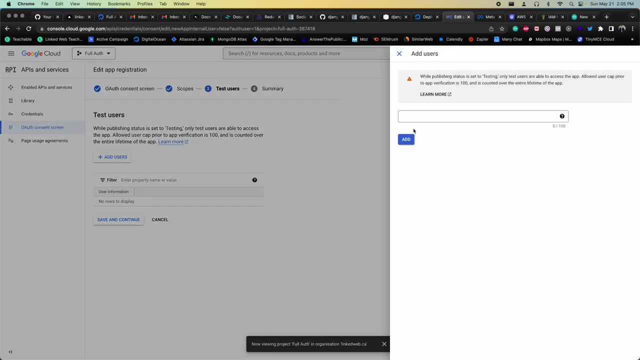 and i'm going to update so that they're present, and then save and continue and then you can add test users if you want. so i'm going to add a test user. in my case i'm going to have john doe. one, three, five, seven nine one five at gmailcom be. 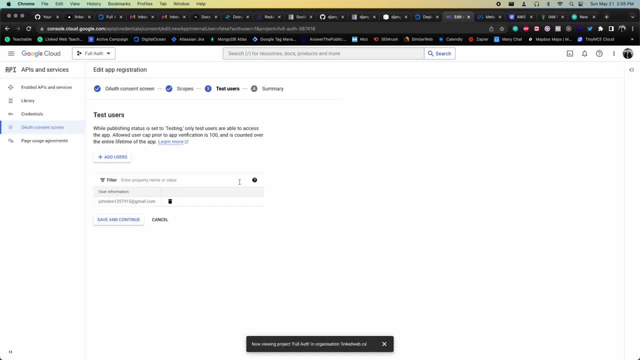 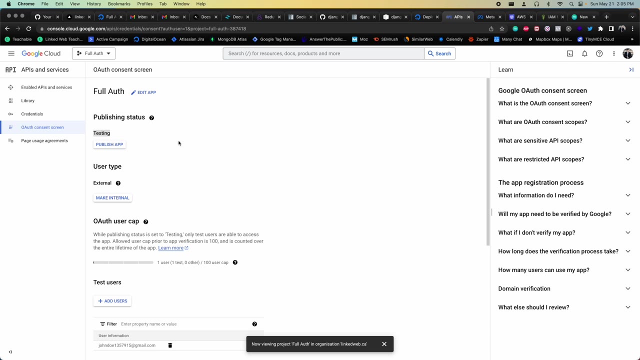 my test user. i'm gonna add that. so there we are, and then save and continue, and here's my summary. i can just go back to the dashboard now and then, when you're ready to deploy, you would just go publish the app. so i'm going to go back to the credentials now. 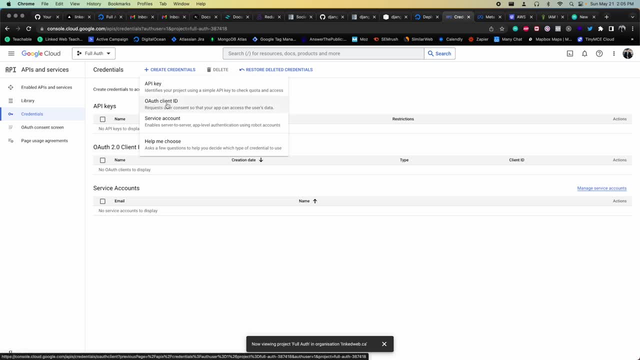 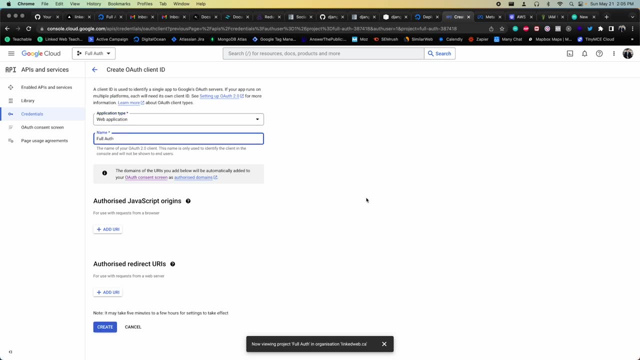 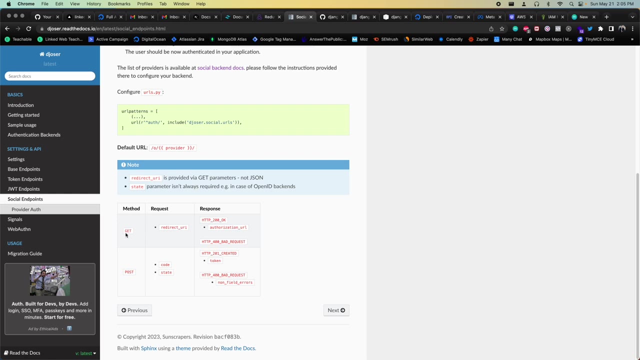 i'm going to create credentials and i want oauth client id. the application type will just be a web application called full off, and this is where i have authorized origins in javascript. just make sure that your application is with full off and then i'm going to just get that back to the devon application. 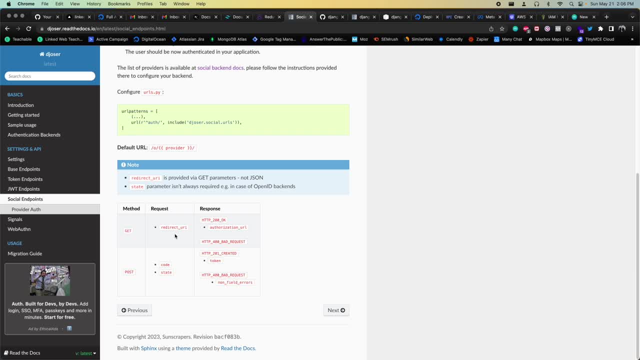 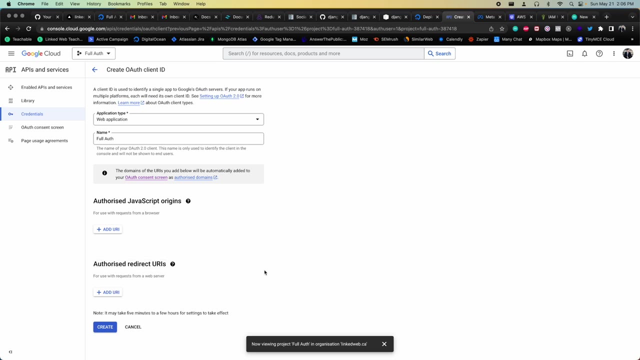 and i'm going to need to just use this test user as my default user, and that is here in java script origin. so in joseph, when we're doing this get request, we're passing in a redirect uri. now, this redirect uri, someone can go make a request. a slash o slash. 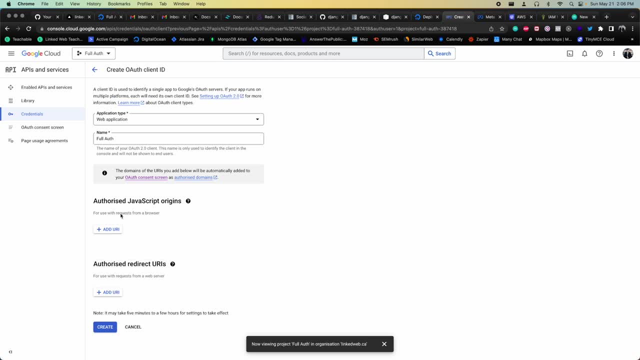 your provider pass in some redirect uri that goes to maybe their website specify here. so this is a security related thing around oauth. so here i'm going to put in my authorized javascript origins. so here i'm going to have http colon slash, localhost 3000, because it's going to be our nextjs app that we're redirecting to and then for authorized 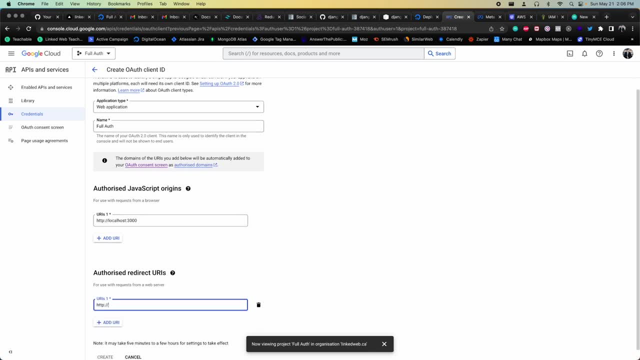 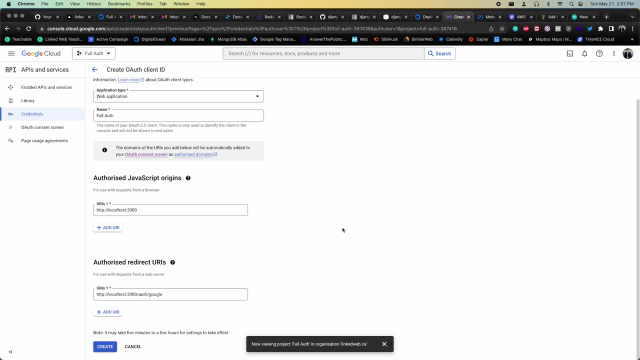 redirect uris and i have http, localhost, 3000 slash, auth, slash, google, and then later we're going to come back here once we have our domain. we're also going to add that in as one of the uris and also have the redirect uri for the domain. i'm going to create that and just click on. 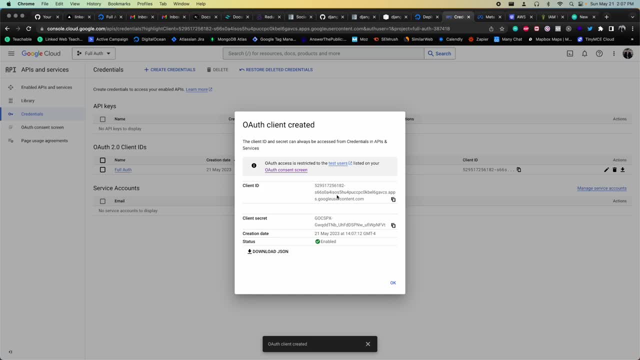 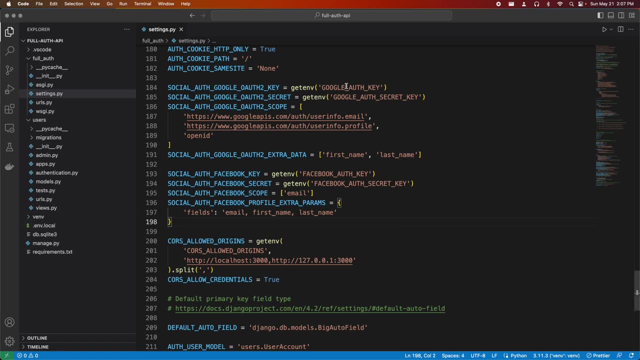 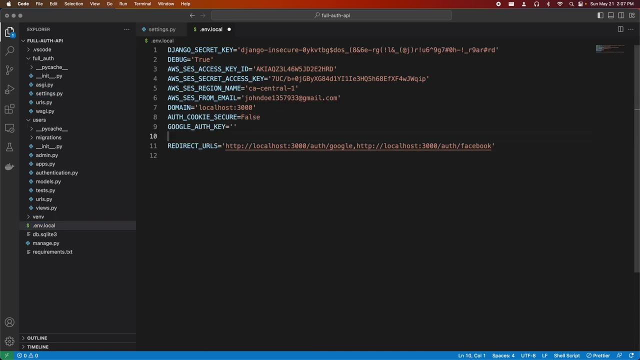 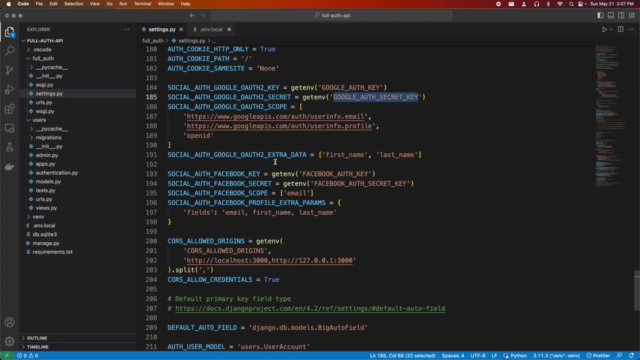 actually i need to copy these. so i'm going to copy the client id and then, inside of my env, local. actually, first i'm just going to copy these into that env, so i'll do that above the redirect. i'm going to copy the secrets, then i'm going to copy the facebook auth key. 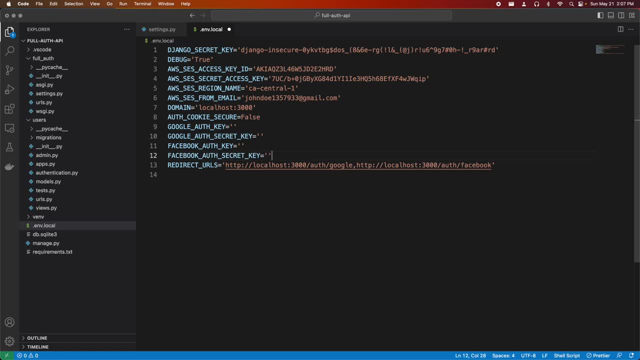 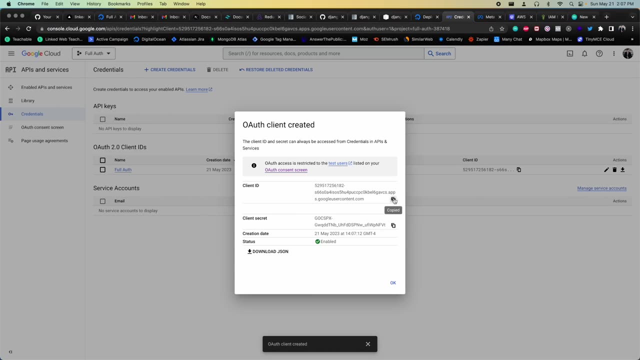 and then the facebook auth secrets. so now i just have to fill in all of these. so back here, i'm going to recopy that client id, i'm going to paste it in the google auth key, i'm going to copy the client secrets and i'm going to paste that here and save. 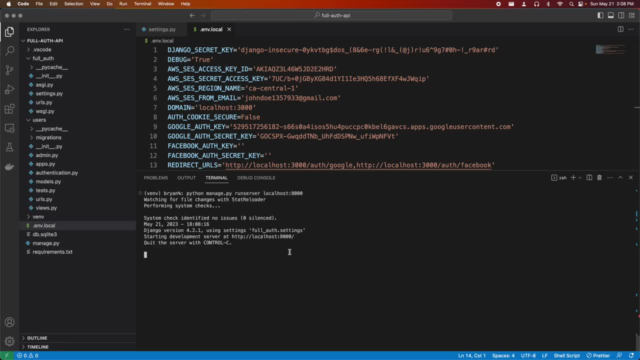 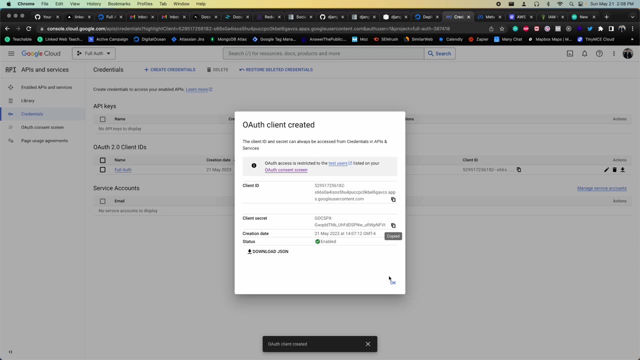 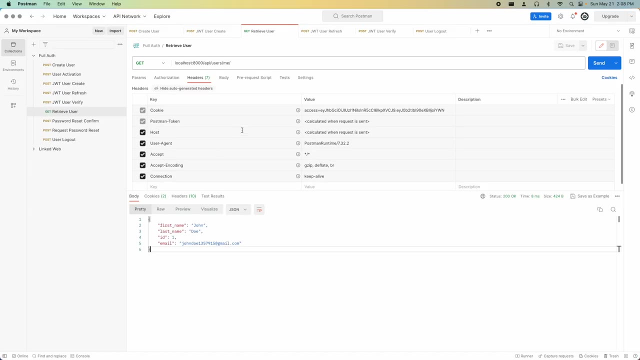 i'm just going to rerun my server just to make sure that we have those, because now we're ready to test our google oauth, so i'm going to click: ok, that's going to close that up. and now let's test this out. so i'm going to open up postman, then i'm going to close up some of these other things. 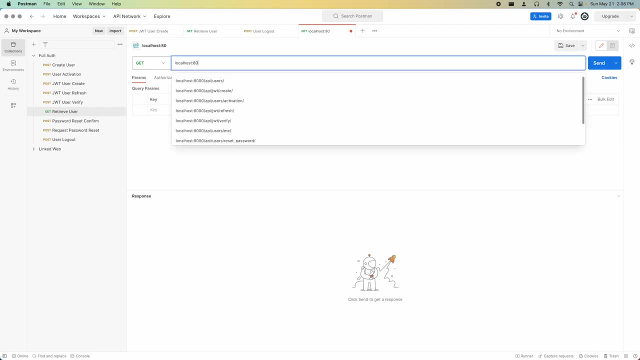 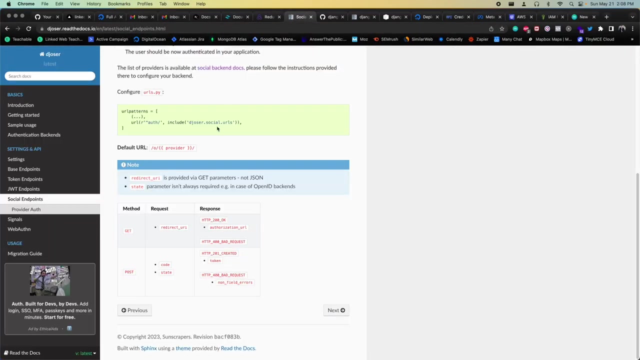 so, first of all, we're going to have our get request. this will be localhost 8000, slash, api, slash o slash- the provider, which in our case will be google dash oauth2, and then i believe there's a trailing slash. let's just double check: yep, there will be a trailing slash. 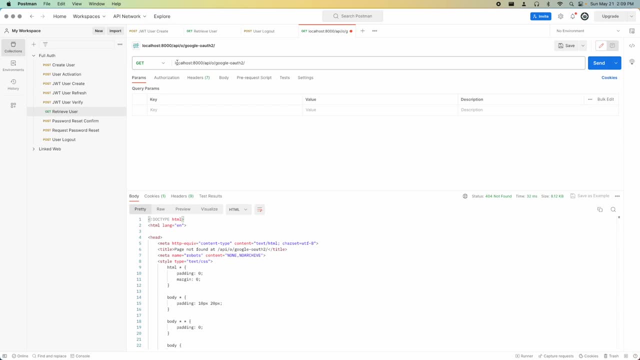 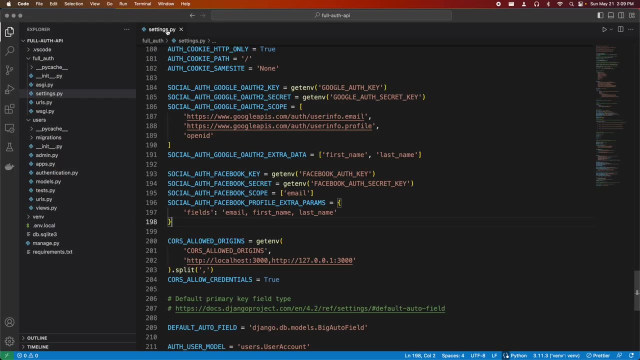 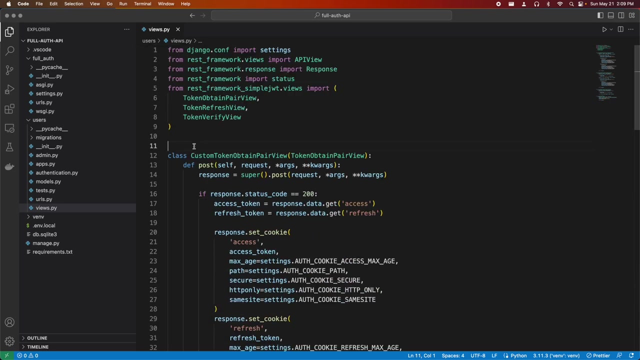 so i'm going to send that off. and, of course, we did not yet set up the urls, so let's go ahead and set up the url so that this actually works. and before we set up the urls, we do have to go into our views and override the default view that's used for this oauth, so the view that's 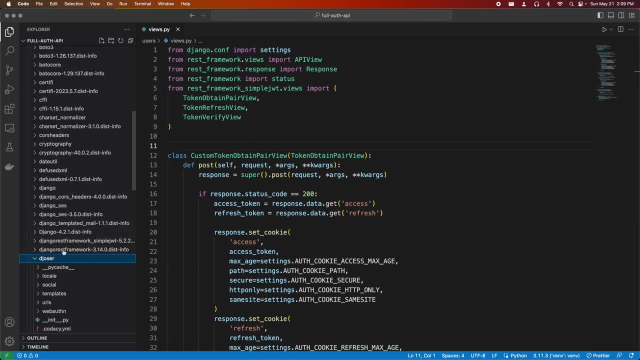 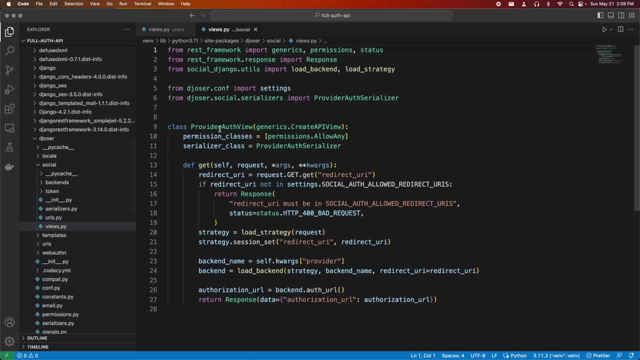 used for this. we can actually take a look. we can go inside of joser and then social and then views, and we have this provider auth view. this is going to be the thing that we override now. the only thing that we see in here is a get, but this also does handle a post. 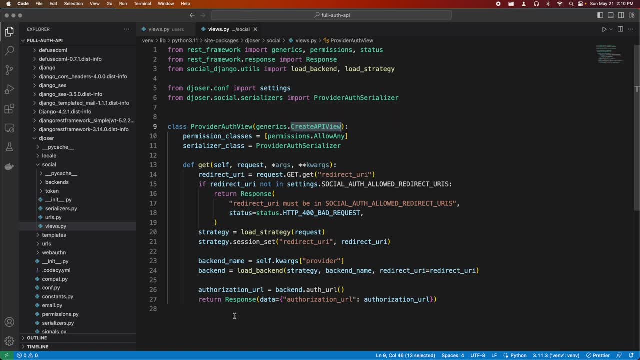 through the create api view, which is one of the generic views, and then we are going to want a url for this. now we can either set up, like we saw in the settings where we use the joser social urls to set up those urls, but we're going to want our own custom one. 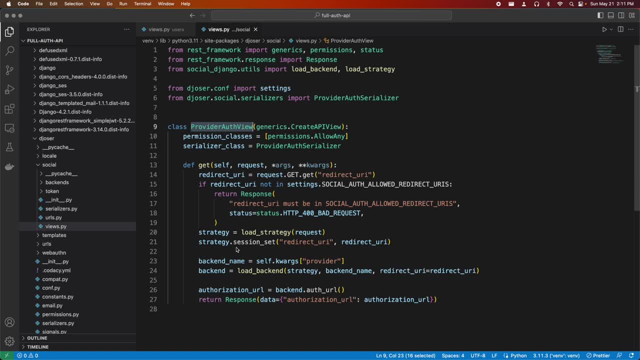 because we're going to override this in particular, we're going to be overriding the post, so we're going to send the post request to the parent class, which is just this provider auth view. i'm going to get the access refresh token. then we're going to set those in our cookies and send back the response. 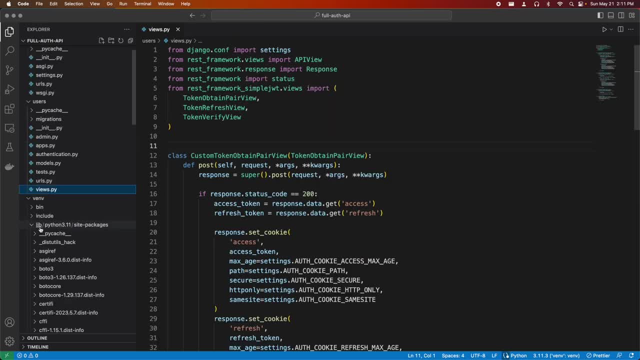 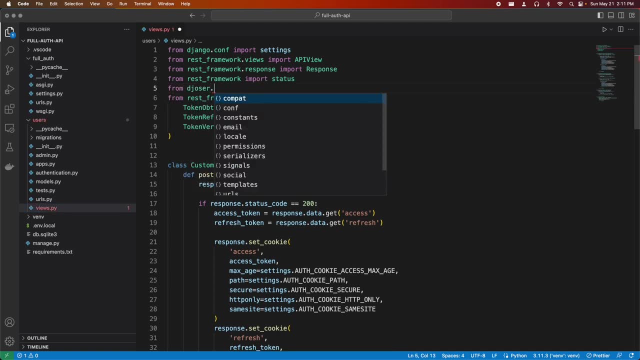 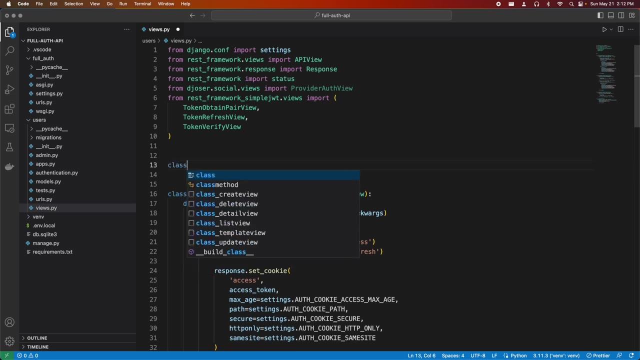 that's how this is going to work, so we're going to close this up and then back in our views. i'm going to import from josersocialviews. we're going to import that provider auth view and we're going to create a custom provider auth view. 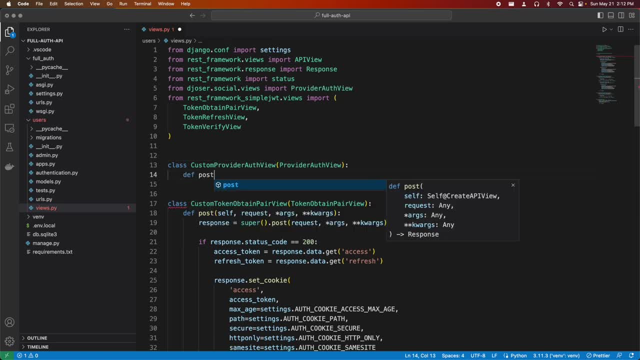 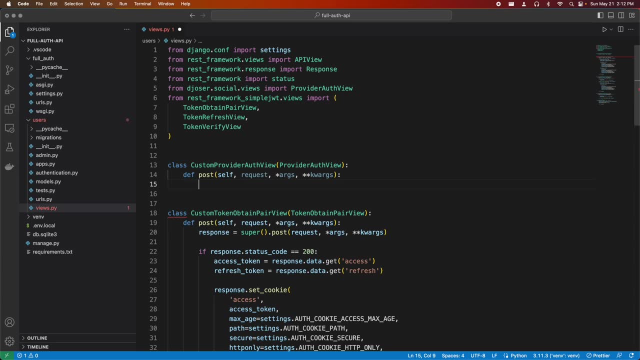 which is going to inherit this one. we're going to define a post with self request args and our keyword args of het month, and then we're just going to get a response by calling supr dot post. So this is just going to do whatever the provider auth view. 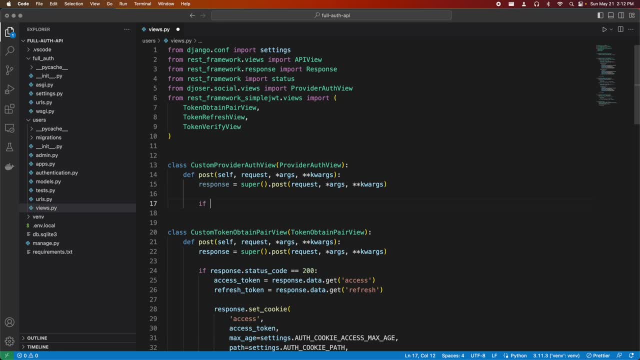 did. we're going to get that response and then we're going to check if the response dot um. So this is just for the post. we're not overriding the, we're just overriding the, and then we're going to eventually return this response. But first we want to set the access and refresh tokens. 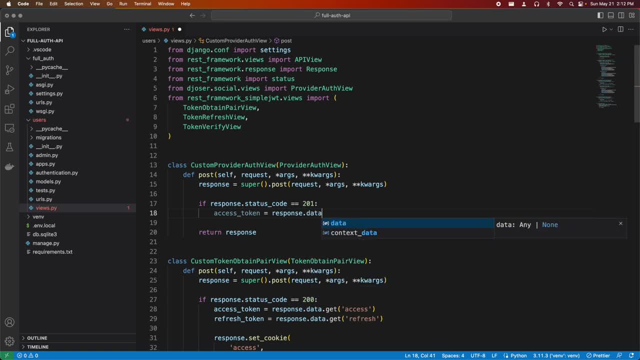 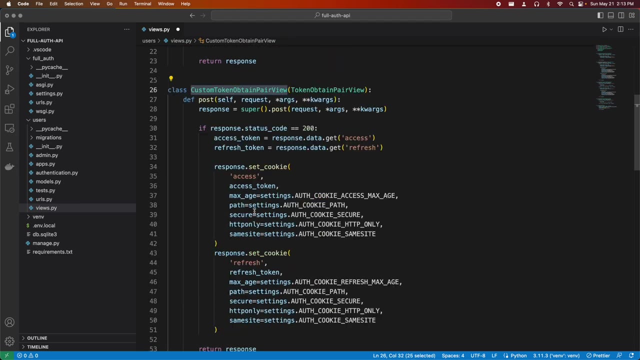 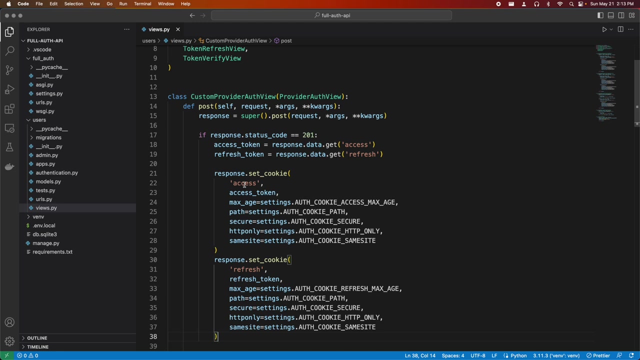 So access token will be coming from response data- get access- And then refresh token will be coming from response data- get refresh, And then we're going to set the cookies. So we've already done this inside of our custom token: obtain pair view. I'm just going to copy this part, go back up and paste it here. 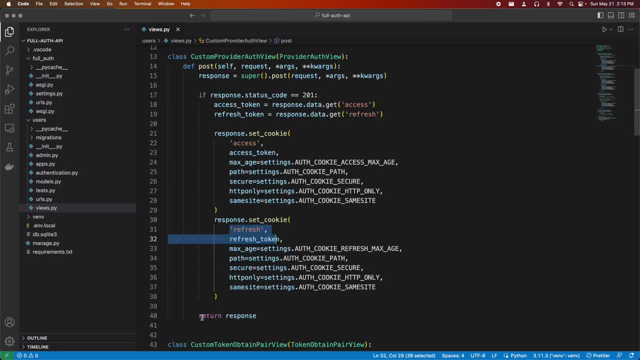 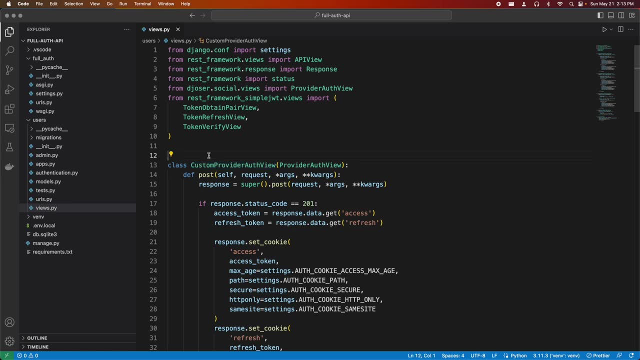 So we're going to set the access refresh token in our cookies, send back the response, and then we're going to have access to them in our cookies. So it's as easy as that, And the last thing we have to do is just go into our URLs. 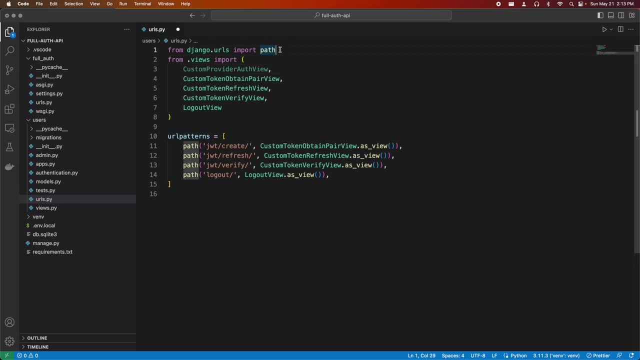 And then from there I'm going to import this custom provider auth view. I'm also going to import a regular expression path And then this path is going to be set up like this: So I'm going to have a regular expression, Which is going to be a hat, and then O slash and then I'm going to have in brackets question. 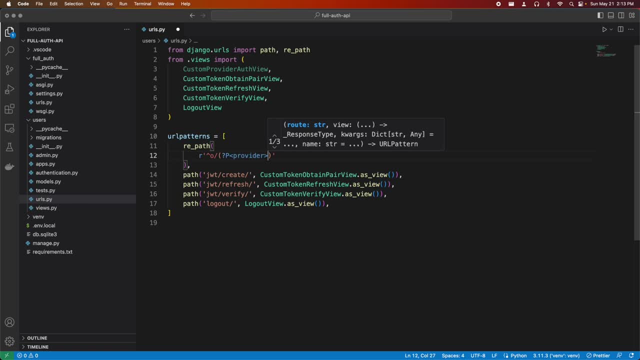 mark P provider and then backslash capital S plus and then slash dollar sign. So this is going to be O slash, a provider slash, and then this provider will be things like Google, OAuth 2, Facebook and so on and so forth. 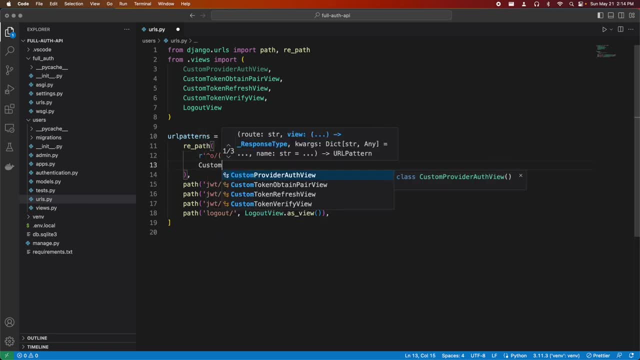 So I'm just going to have that, Okay. So we're going to handle all of those. We're going to use our custom provider auth view, do a dot as view And then we're going to have our name of provider auth. 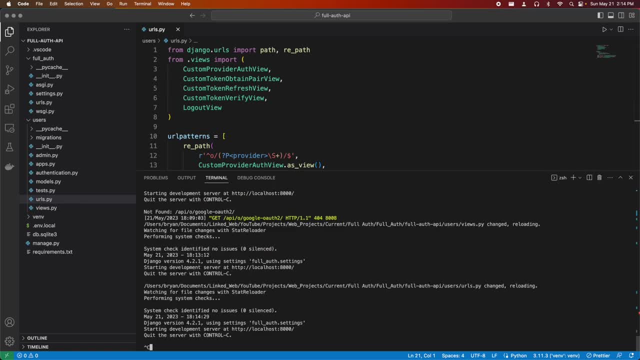 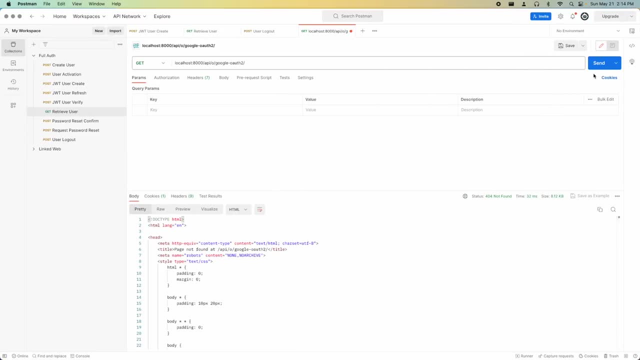 And there we go. We now have that URL set up. So now I'm just going to rerun the server and test this out. So back inside of here, let's retry this again. Redirect URI must be set. So let's set up the redirect URI. 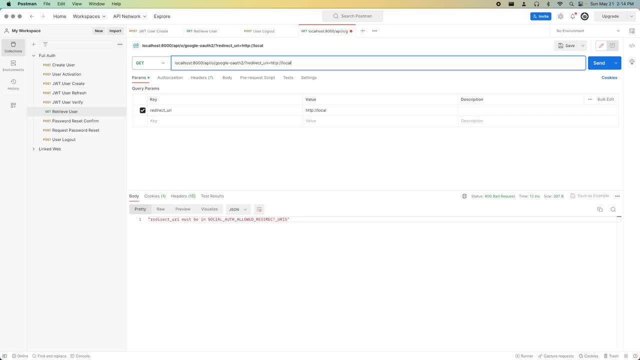 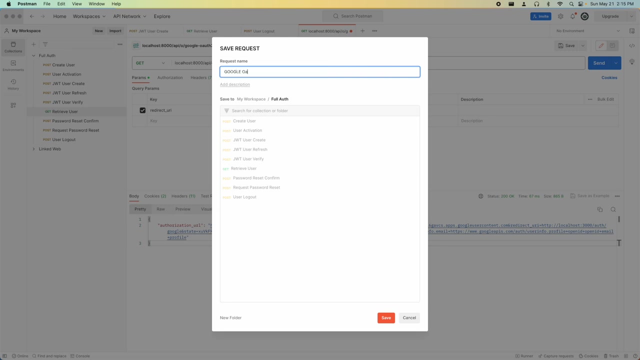 That's going to be HTTP local host 3000 slash- auth slash- Google. So let's send this And there we go, We get the authorization URL. This is going to be the Google OAuth 2 get, or maybe I'll do get authorization URL. 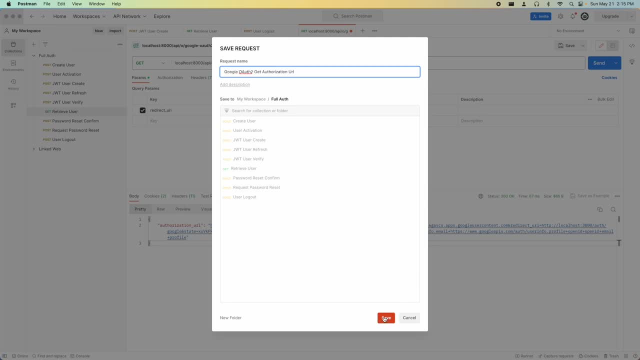 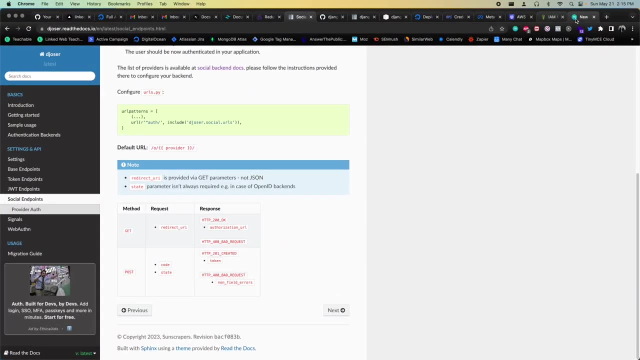 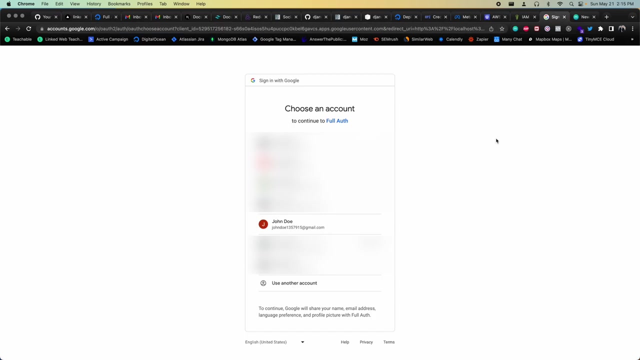 Okay, And I'll save that, And then I'm going to copy this URL and then back inside of my browser I'm going to paste, And then the account that I'm going to log in with is my. John. do one, three, five, seven. 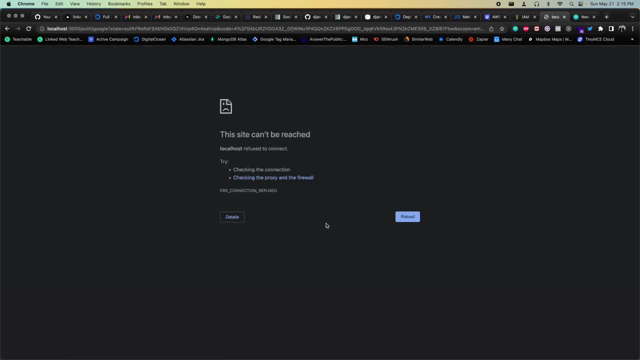 nine one five account. So I'm going to click that and I'm going to get redirected back. Now we're going to end up seeing this because we don't have an XGS app running right now, but we did successfully get redirected. We got redirected to local host 3000, where that's going to be running. 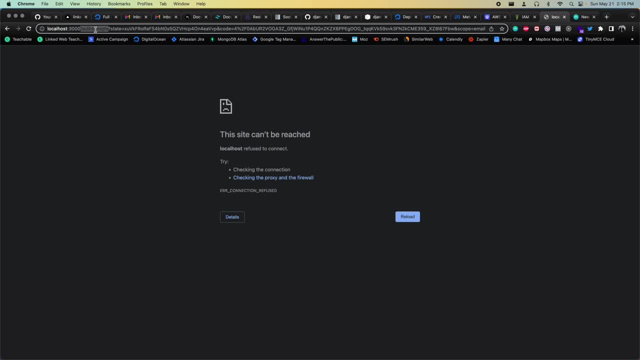 We got redirected to this path: auth Google, which our next year's Apple eventually handle, And then it's going to have this state and code inside of the URL parameters, So we're going to grab those and then make the post request. That's how that's going to work. 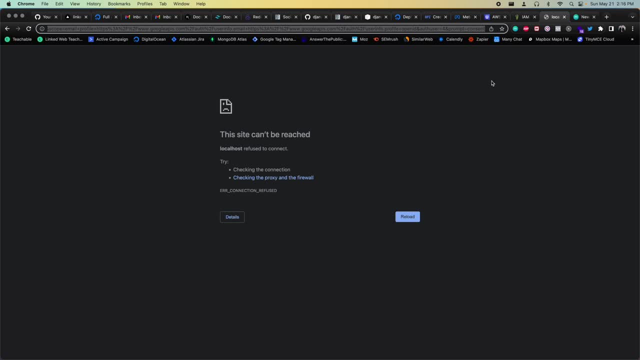 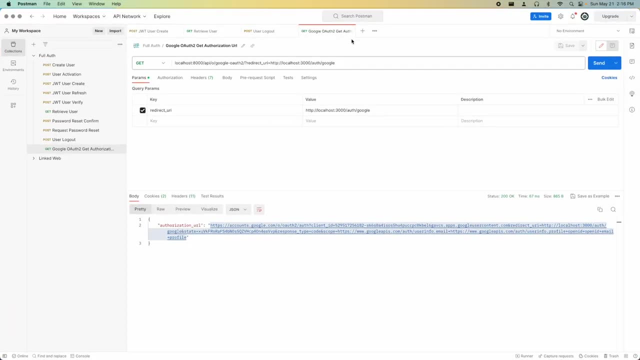 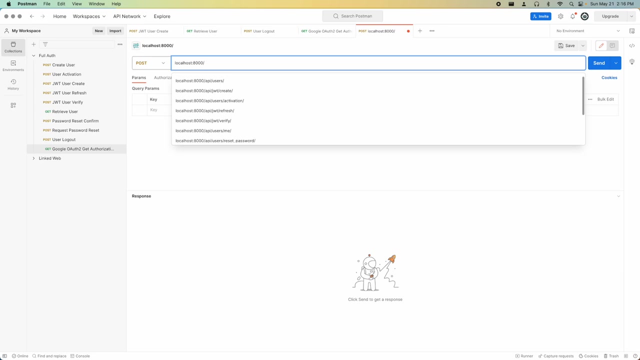 I'm just going to copy everything here inside of these query prams and then I can close this up- I don't need it anymore- And then we can test out that poster. Okay, So the post request is going to go to local host. 8,000 slash API, slash O slash the provider. 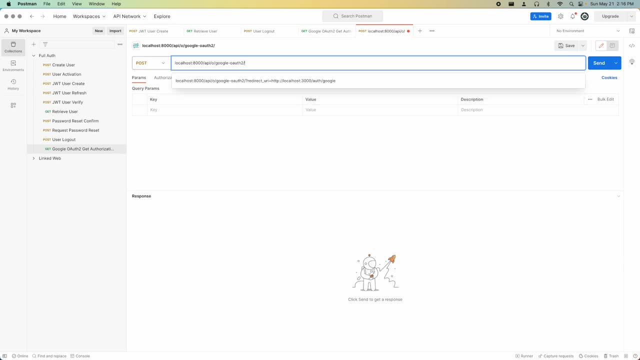 of Google OAuth two, slash. And now, remember, we're going to have the content type, not of application, Jason. instead we're going to have content type of application: slash X, WWW form URL and coded. So then inside of here I can have question mark and then this: and we have some extra. 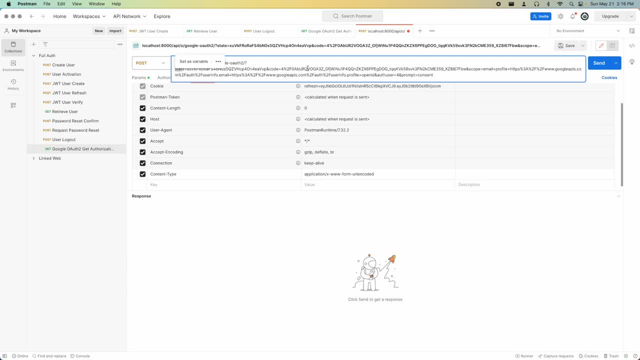 stuff here. So we have the state as a query parameter and we have the code, which is right here and its value ends right here, And we have all this extra stuff that we don't need. So I'm just going to delete that. 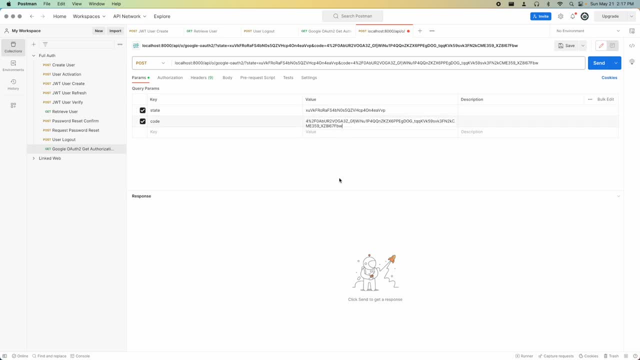 And then inside of our prams, we can see both our state and code here, And then one thing that we need in order for this to work is we need the states to be present in a cookie, because it's going to take that value and compare it. 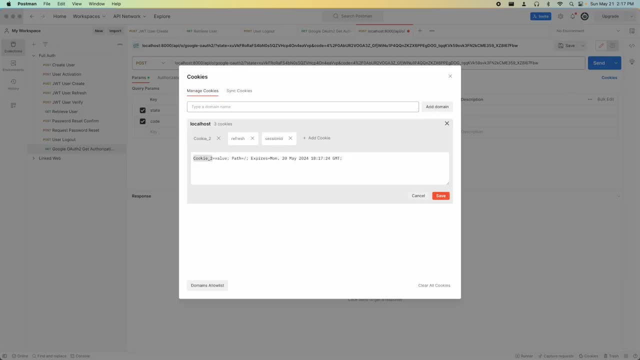 So I'm going to go open up my cookies, I'm going to add a cookie for state and paste it here And I'm just going to save. And there we are. So it is not enough to just have this state inside of your query prams. 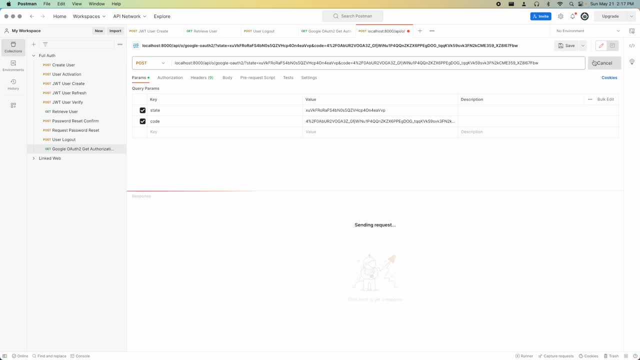 You also need to have it in a cookie And then with that we can send this request and there we go. It worked. We got 201 created, We got an access and a refresh token and user, So now I can even go retrieve the user, and this should all work. 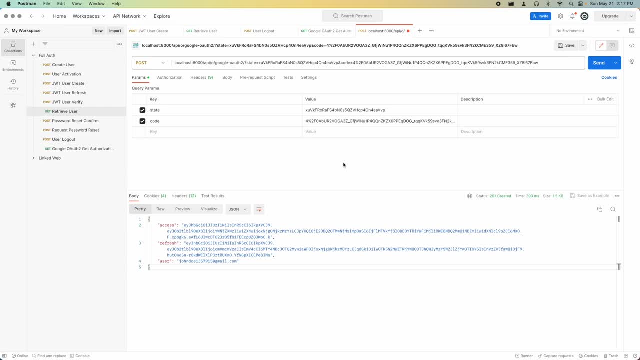 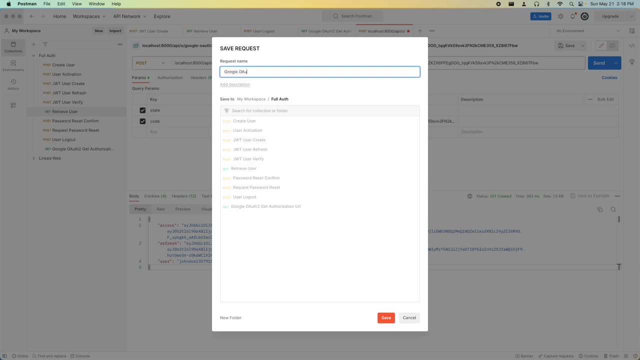 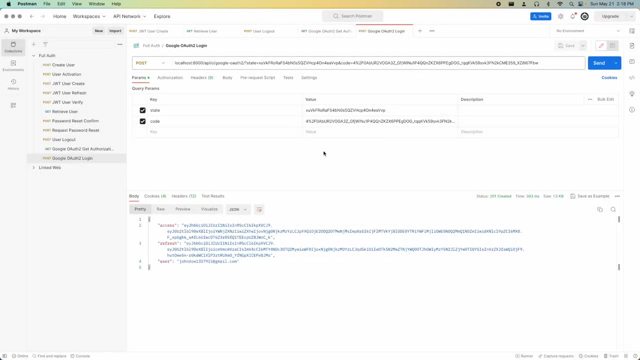 There we go. We successfully logged in using Google OAuth 2.. I'm going to save this. This will be Google OAuth 2 login, So now the only other thing that we have to do is also set this up for Facebook OAuth. Okay. 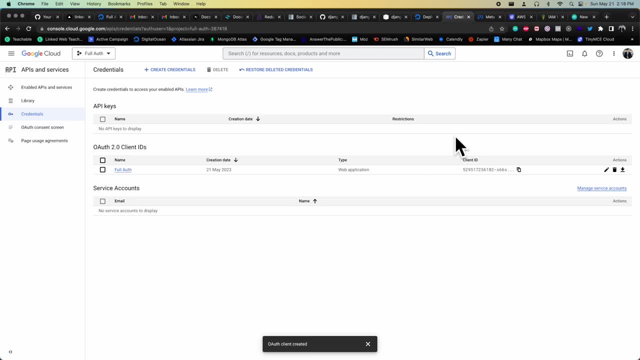 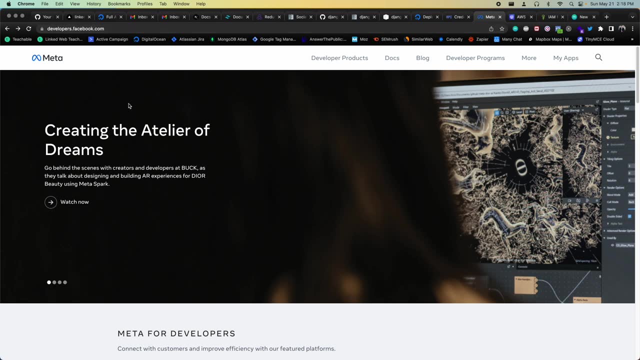 So for Facebook OAuth. now I don't need this open anymore. Actually, I will come back to this. I will leave it open. So where you're going to want to go is developersfacebookcom. So you're going to want a Facebook account. 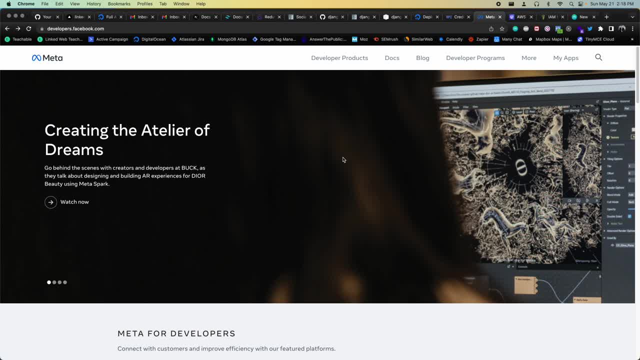 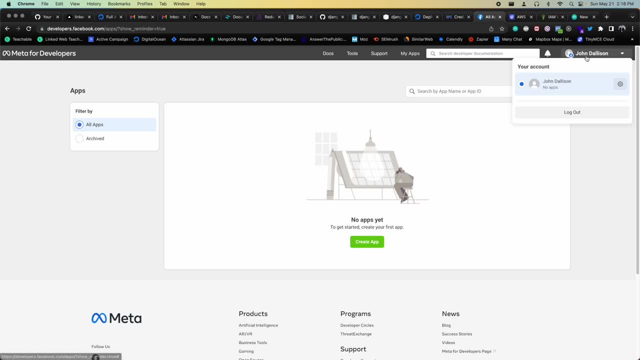 And then, when you go here, you're going to sign up to this developer's Facebook and then you're going to be able to log in Once you log in. so I'm already logged in right now And, in particular, I'm logged in with my John Doe 1357933 at gmailcom email. 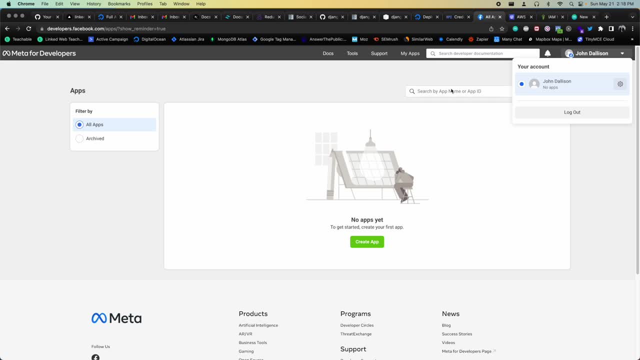 So I'm going to log in, I'm going to log in, I'm going to log in, I'm going to set up the email So that one is John Dallison, And then, under my apps, you can create an app. 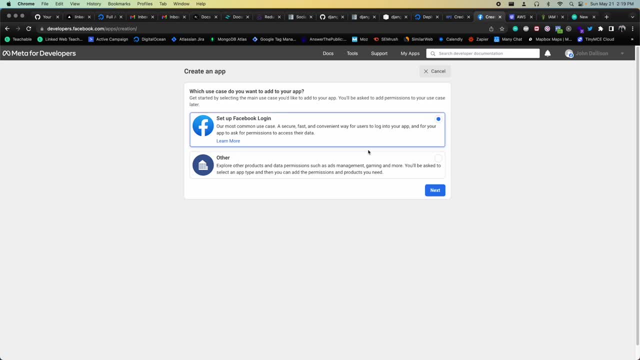 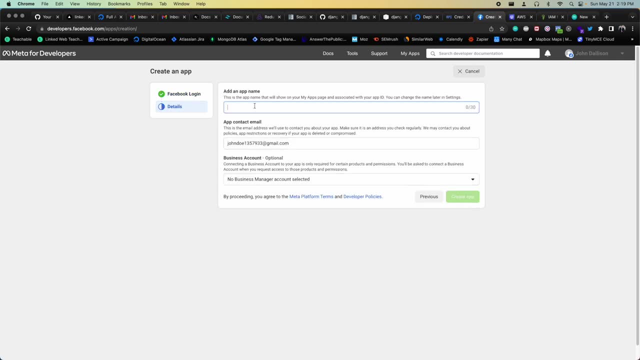 So I'm going to do that. I'm going to set up Facebook login, Click next. it's going to be a website, I'm not building a game- And then you can add your app name, which, in my case, will be Full Auth. 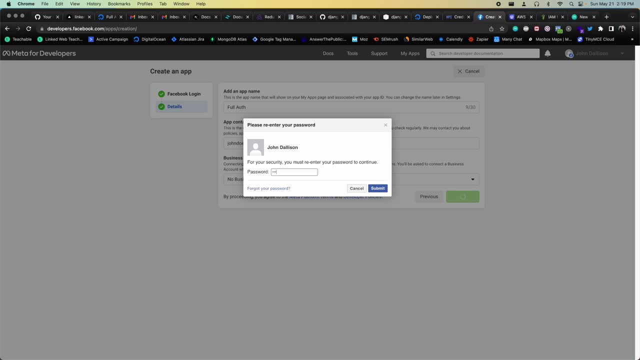 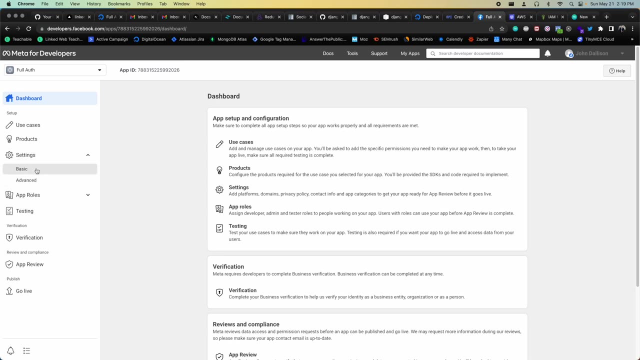 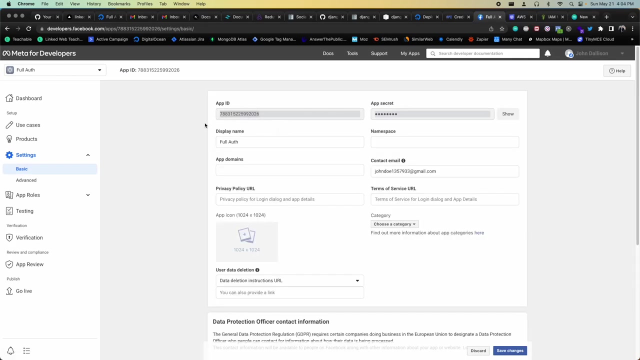 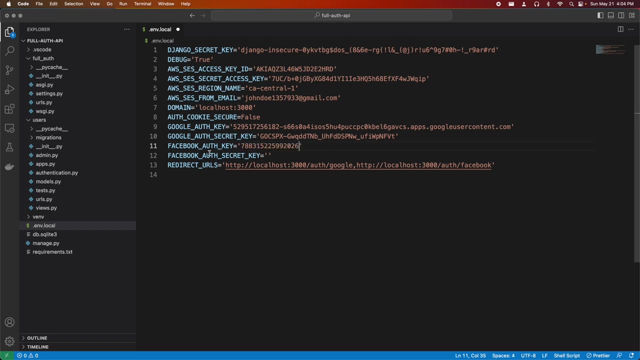 And then this is my email. Okay, so now we've hit the dashboard, so we're gonna now grab those keys that we need. so under settings, basic, next I'm gonna grab these two keys. so I'm gonna grab the app ID. I'm gonna flip back to my app, open up my ENV local, paste in inside of: 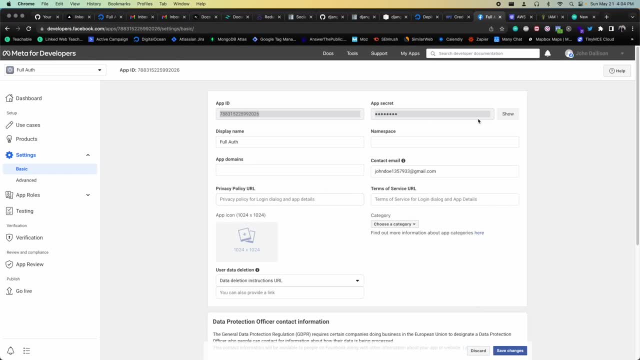 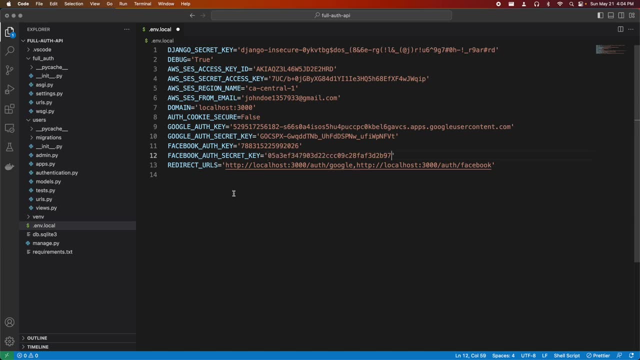 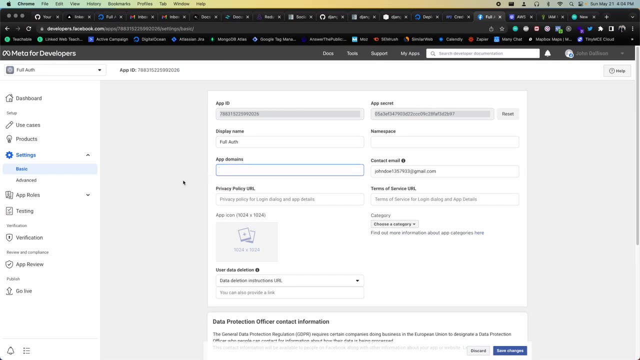 the Facebook auth key, this key, and then I'm gonna show the app secret. I'm gonna copy that, go back and paste that in here for the Facebook auth secret key. so with that now I can go back for app domains. I'm just gonna add in localhost here. I'm. 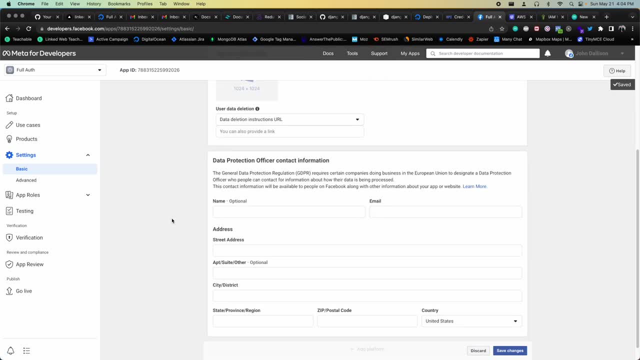 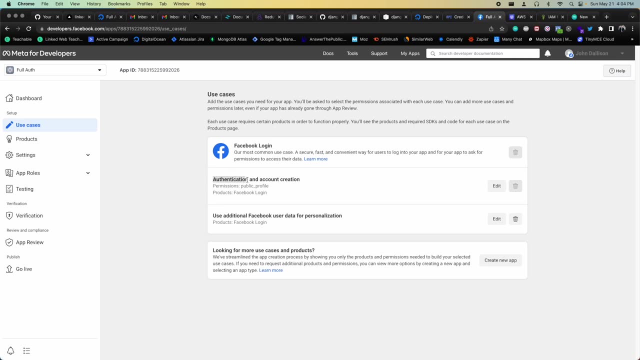 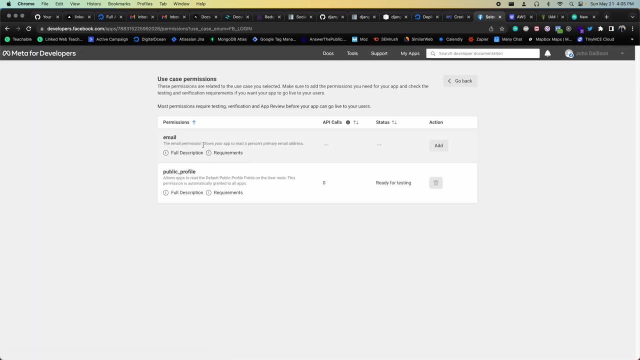 gonna save that. and then the other thing I have to do is go into use cases and then here for authentication and account creation, one thing I have to do is go edit this. then by default we don't have permission to grab the email, so we have to add that. so there we go. so now that's ready for testing, so I can go back and 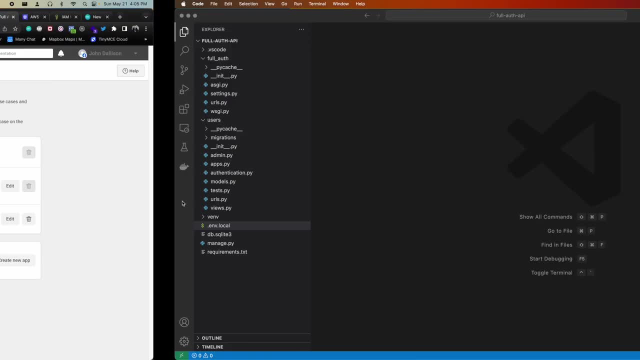 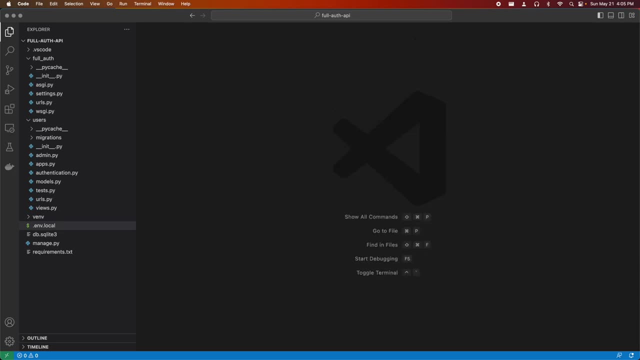 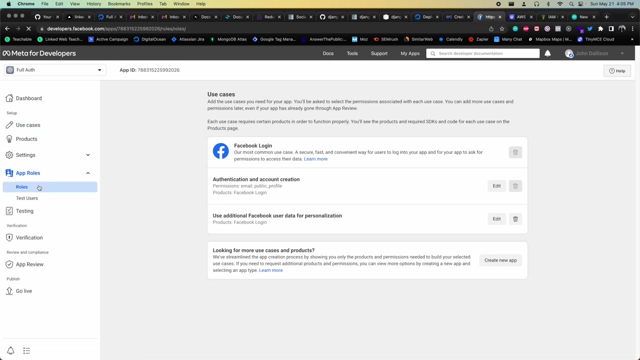 then we can try things out. so I'm gonna do is: since I added those environment variables in here, I'm just gonna restart the server, I'm gonna flip on back, and then we also have to create a test user. so I'm going to go under App roles and this is where we can add testers. so I'm 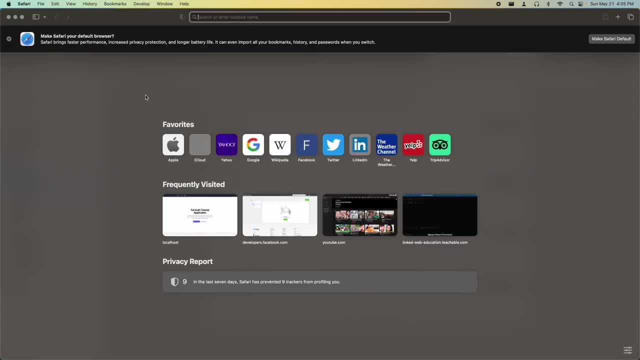 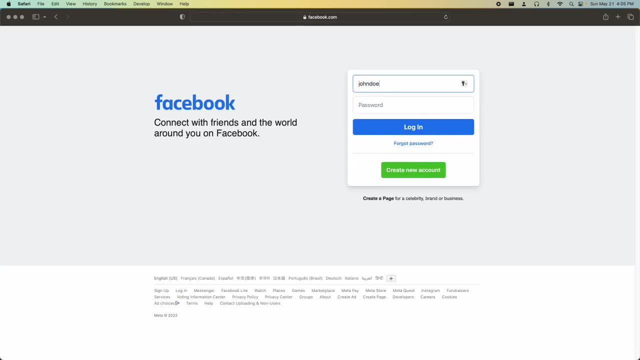 going to open up a Safari window, or you can open a Firefox girl on Windows, doesn't matter, I'm just going to navigate to Facebook, so facebookcom. I'm going to log in with my John doe one, two, three, five, seven, nine one five at gmailcom email. 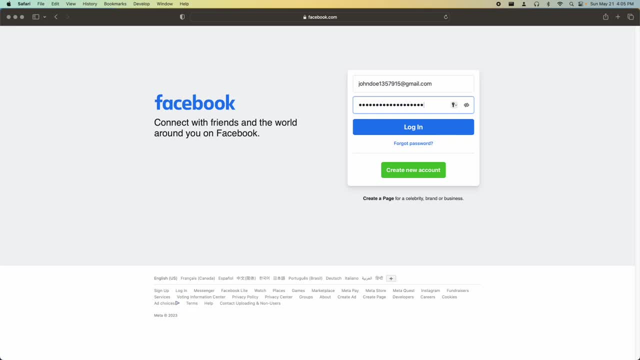 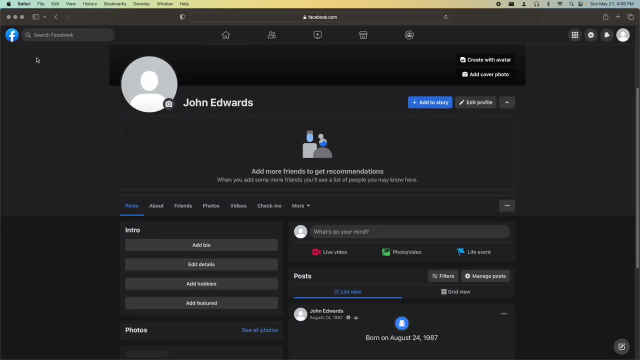 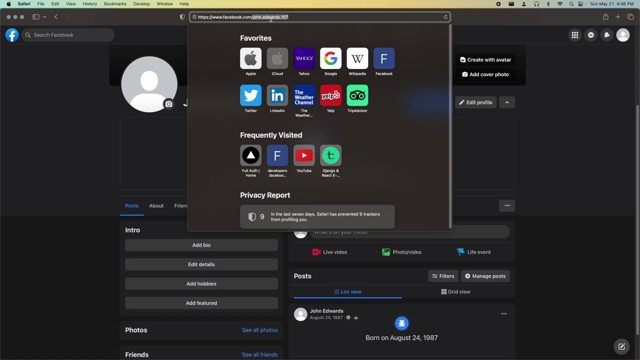 and then I'm gonna go to the case experience tab here and data security head formed through the test, and then I'm going to go to the profile. I'm just going to grab the Facebook ID. So that's this part right here. So in my case, for my account, it's going to be John Edwards 107.. 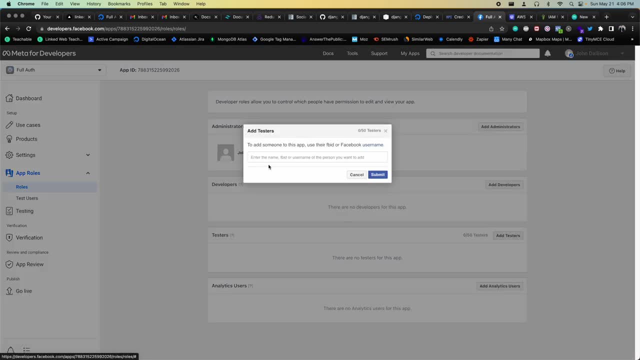 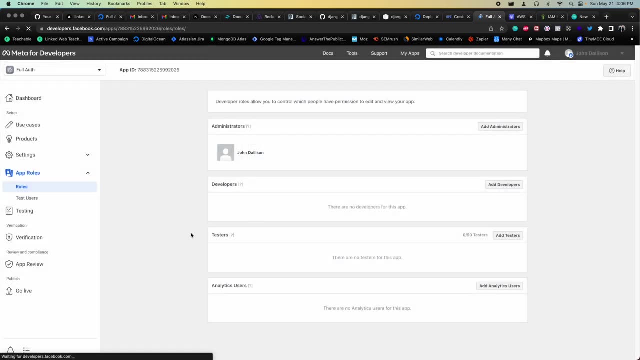 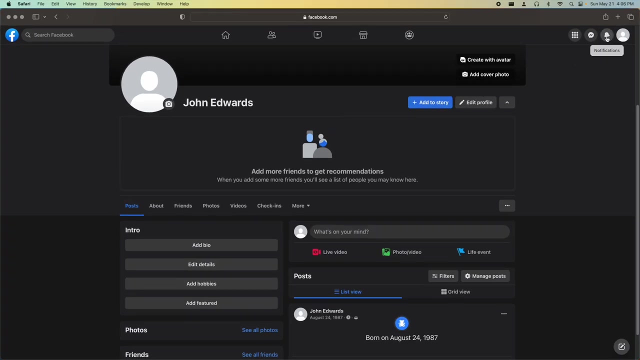 So I'm going to flip on back here, I'm going to add a tester. I'm just going to put in that Facebook ID here And then submit. So now it's going to be pending, So if I go back, so inside of my notifications nothing's going to show up. So the place where this actually shows up, 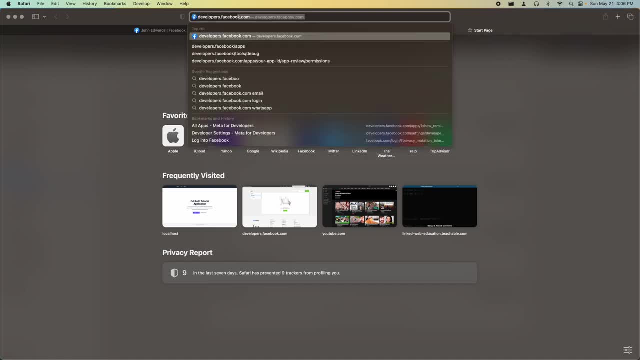 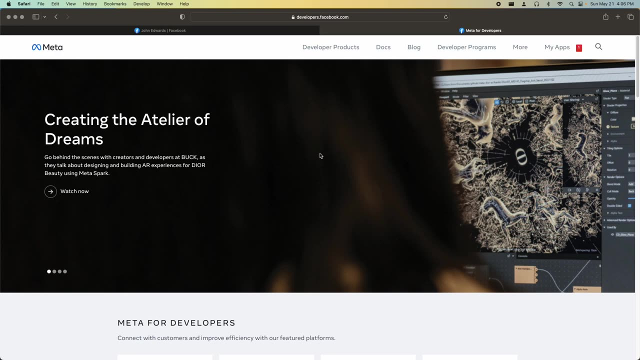 is if you go to developersfacebookcom. So this is now with my other email. So this is John Doe 1357915 at gmailcom. This is the one that I'm requesting so that I can be a tester, And then we're going to see. 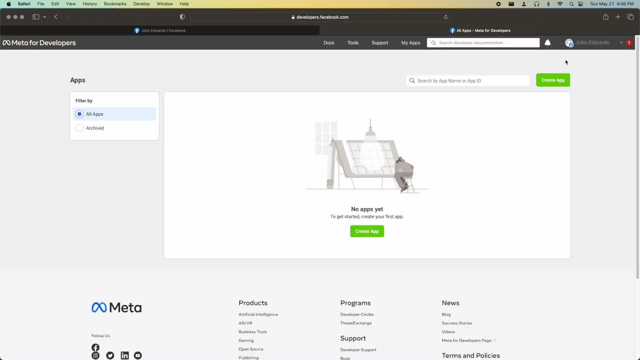 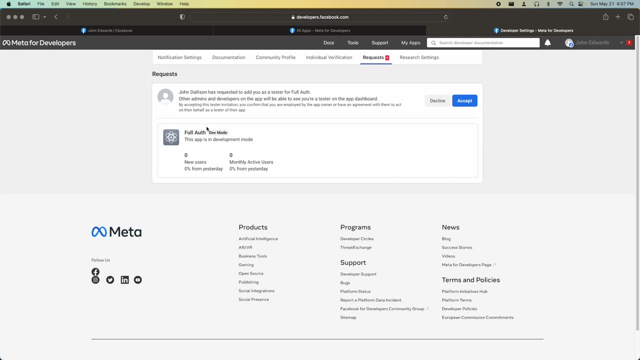 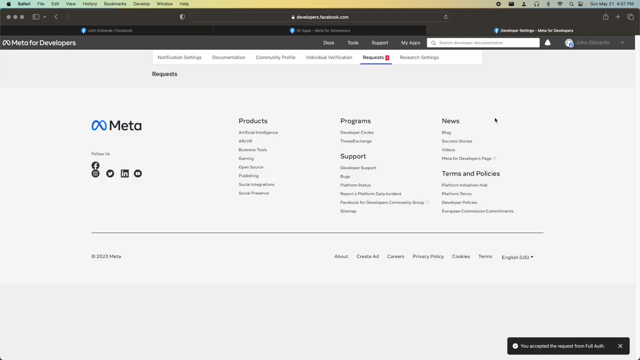 under my apps we have a notification So I can click on that and click on this drop down. Then we have pending app request And this is where this request is. So full auth dev mode I'm going to accept And that's how you can be a tester. So now, if I were to refresh that notification's. 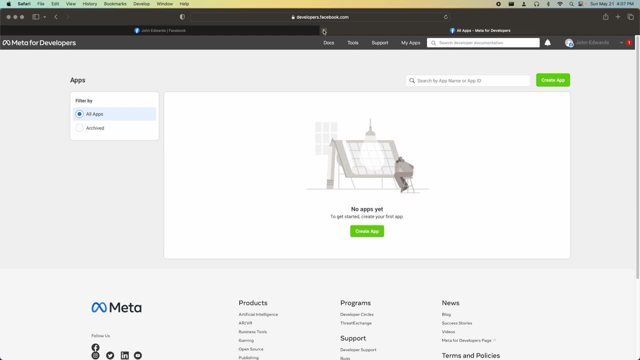 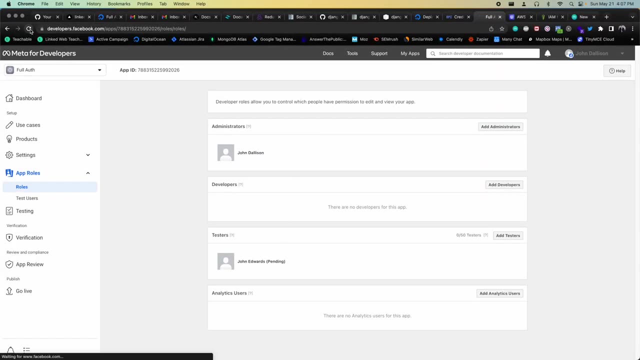 now gone, So I can close out of here And I can close out of here, So now the next thing I can do is I can come back here. I can do a refresh. I'll see that pending gone, There we go. So now this is a tester for this app, And the next step is going to be to 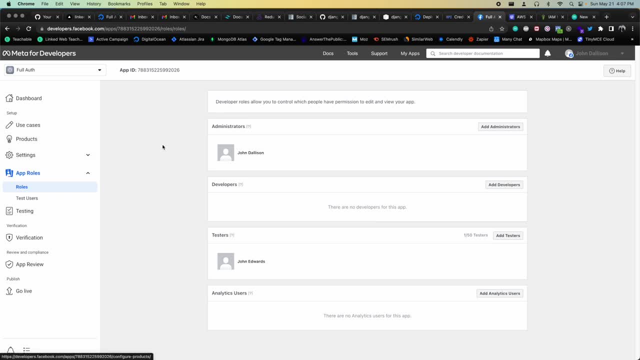 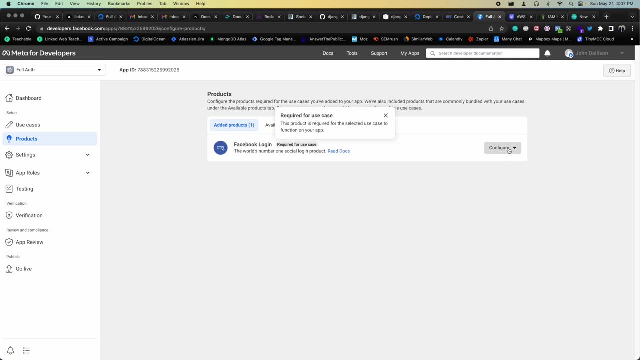 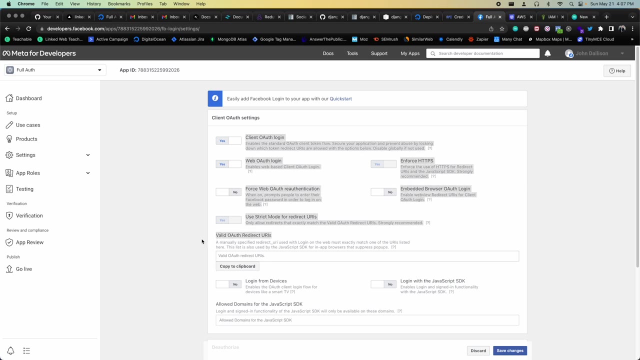 send the request. So I believe everything is in order. to test this out now. And then also another thing to note: inside of products, Facebook login settings: right here we have valid OAuth redirect URIs. Now, when we were setting things up for Google. 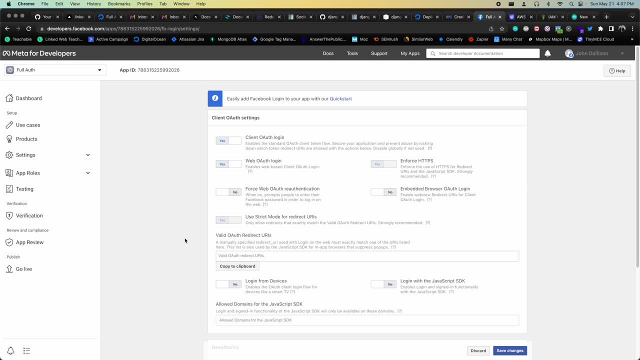 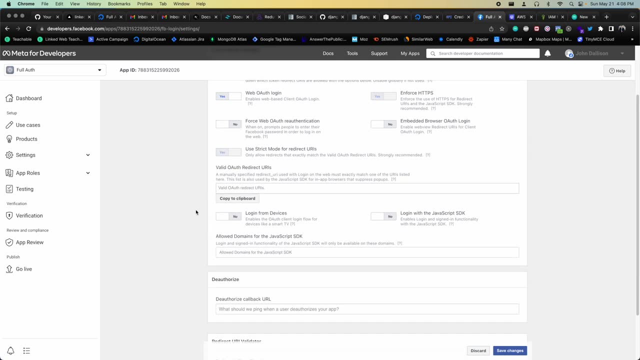 OAuth 2, we put in those valid redirect URIs for Locos 3000, slash auth, slash Google. Now we don't have to do that here And in fact it's going to complain if we do this sort of thing here. 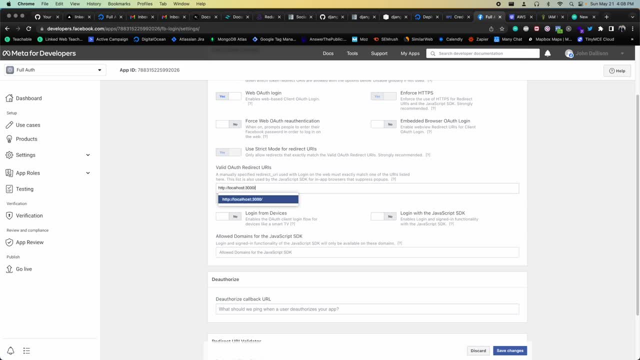 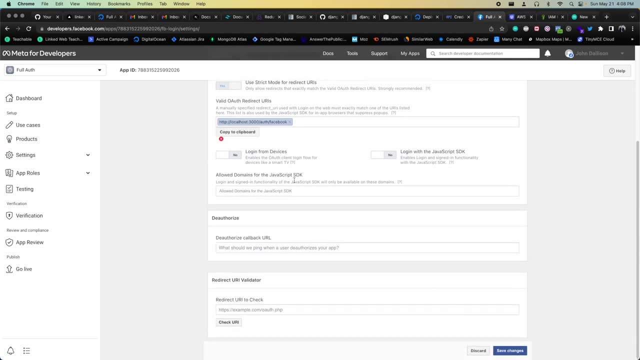 And I'll show you exactly why. So this is our redirect URI. I can put that here, I can click save And then I'm going to get this little prompt. So localhost redirects are automatically allowed while in development mode only, And you don't need to add them here. So that's pretty much. 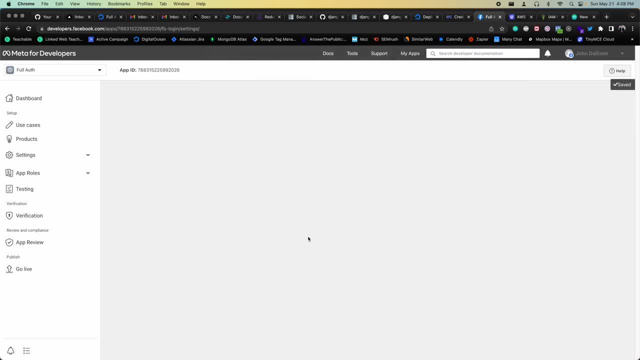 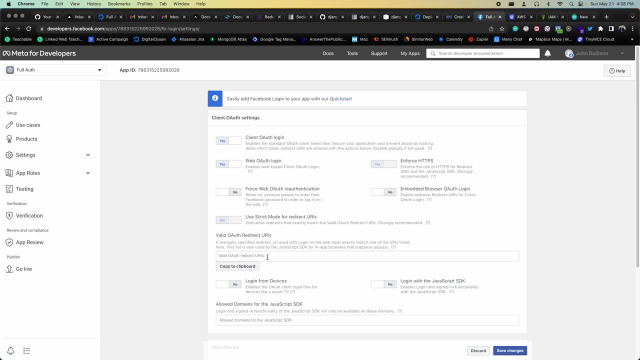 what it's warning me about. So I can just remove it, save and that'll get rid of that. So by default localhost is already valid And any endpoint for localhost is good, So we don't actually have to configure anything there. Now, in production we will, We'll have to put like: 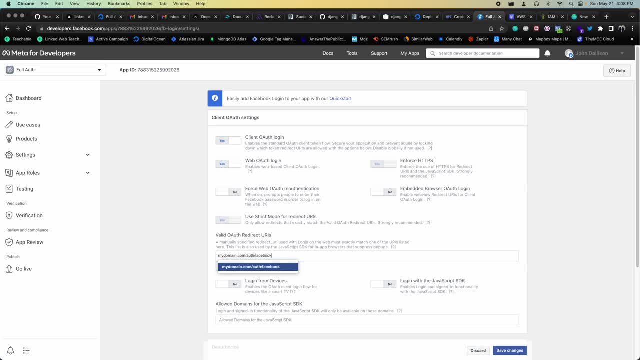 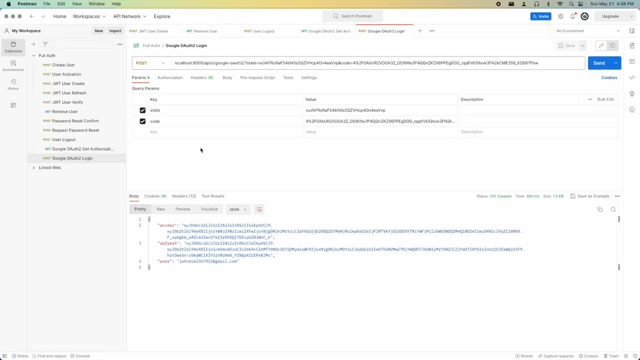 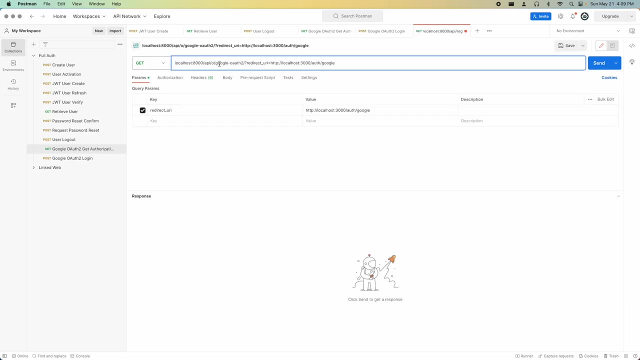 mydomaincom. slash auth, slash Google. So that's pretty much what it's warning me about. But for development, when we're using localhost, we don't have to. So with that I can now go into Postman. I'm going to copy this: open up a new tab, paste And this one's going. 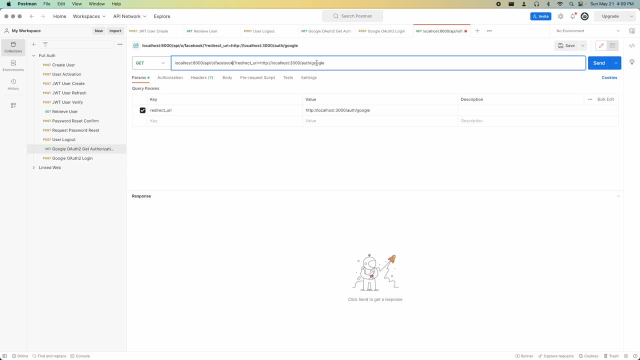 to be for Facebook. So I'm going to put Facebook here And the redirect URI is going to be like: so So, localhost 8000 API- auth Facebook, with the redirect URI of localhost 3000, auth- Facebook. So I'm going to send this So we get back a response, So I can copy this authorized URL. 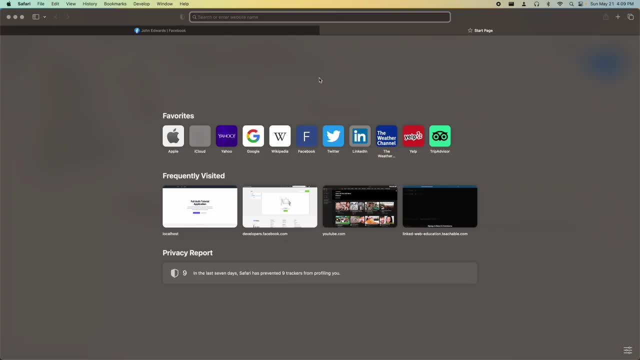 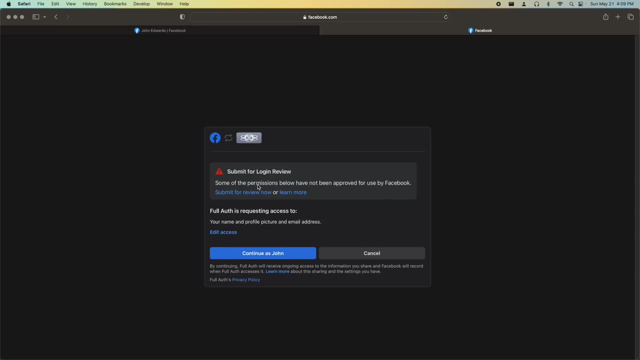 I'm going to flip back into my Safari window, open up a new tab and paste this in. And there we go. We get the submit for log interview. Some of the permissions below have not been approved for use, So I'm just going to continue as John. And there we go. So now. 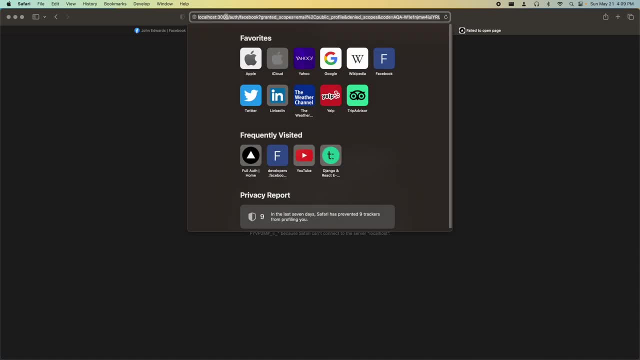 of course we get. So far, I can't connect to the server because we're on localhost 3000, and we don't have our Nextjs app running yet, But we did get redirected to the correct place. This is where Nextjs is going to be running And this is where we're going to handle that post request. 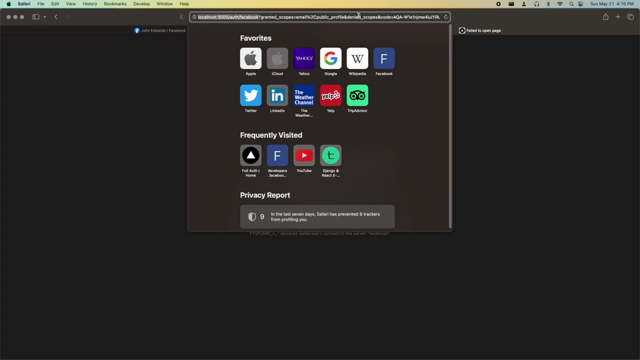 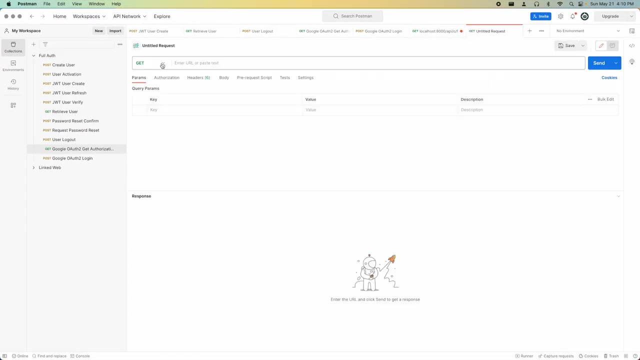 But what we're interested in is right over here in the query params we have this code. I'm going to grab this code and copy everything onwards. I'm going to copy. I'm going to flip back into Postman. Okay, I'm going to open up a new tab. This is going to be a post request. It's going to be localhost. 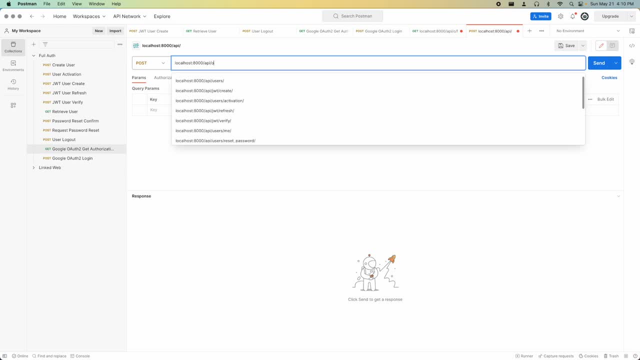 8000 slash, API slash O slash, Facebook slash. And then I'm going to put a question mark and paste. So here I have two query params, a code and a state that I can see here on the params tab. So now we're good, except again we need to set that state, So the state's cookie just. 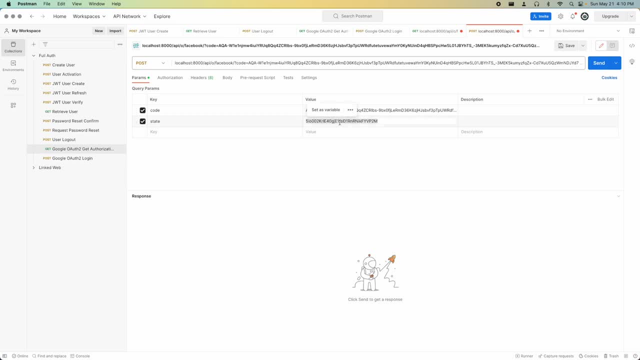 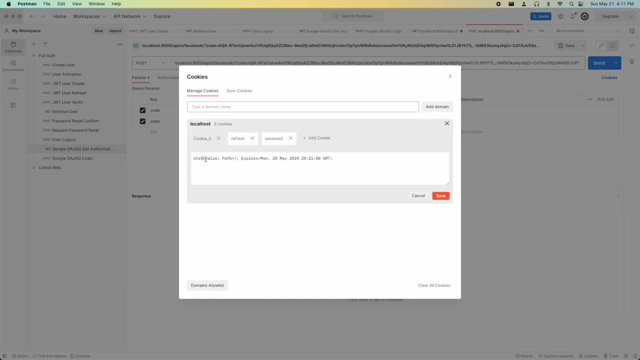 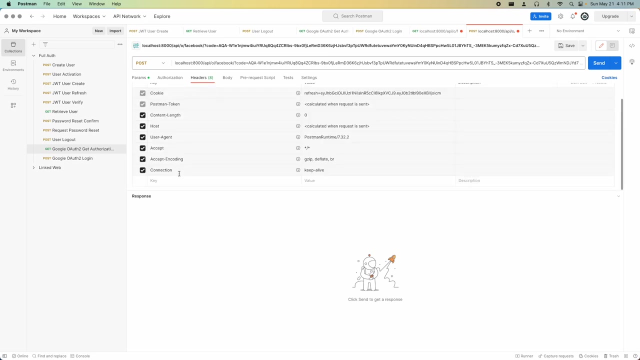 like how we did. We were doing things with Google OAuth, So we're going to copy the state value and go into my cookies. We're going to remove the one that's there at a new one, put in state, put in the value and save. And then the last thing I have to do is go into the headers and put in the correct. 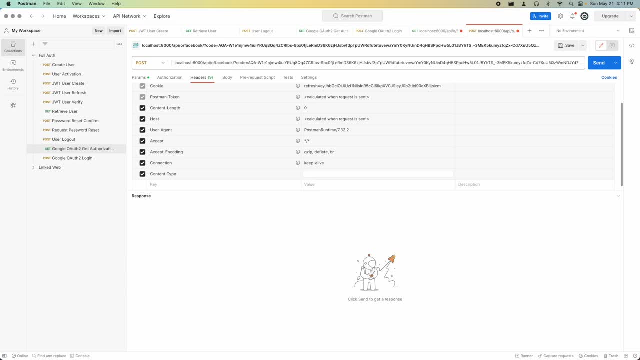 content type. So content type of application: X www form URL encoded And with that we should be good to make this request now. so I'm going to send it and there we are. we got back a response with a 201 created, so Facebook. 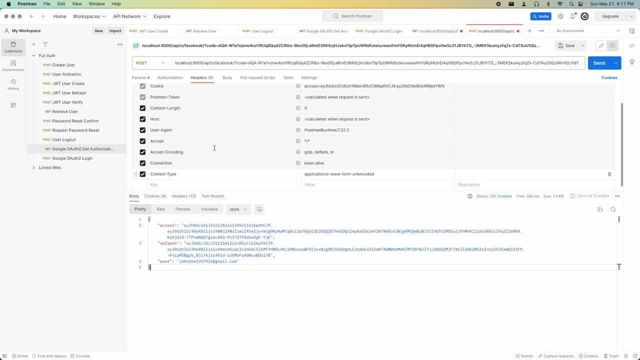 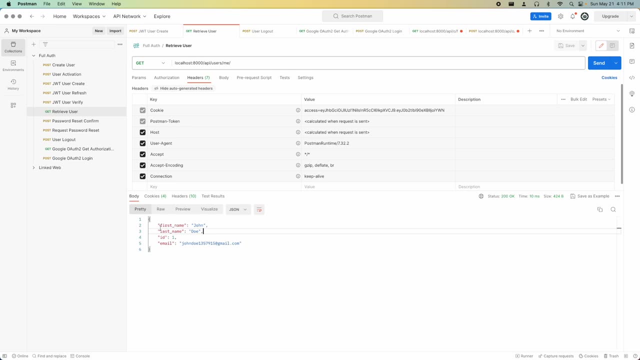 OAuth 2 has worked and on top of that now I can go to retrieve user and I can retrieve and we're going to have different details here because this user actually has a different last name. so we're going to see that if I send this now, we see the last name of Edwards, so it overwrote what was in. 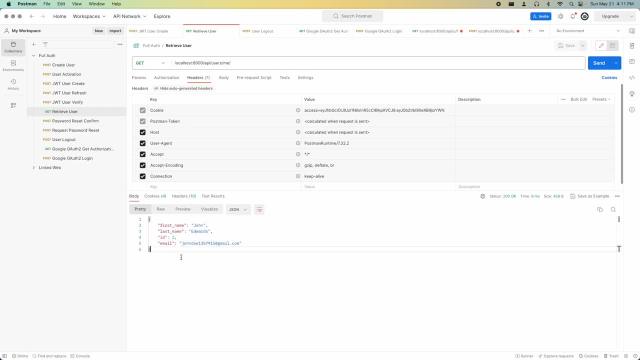 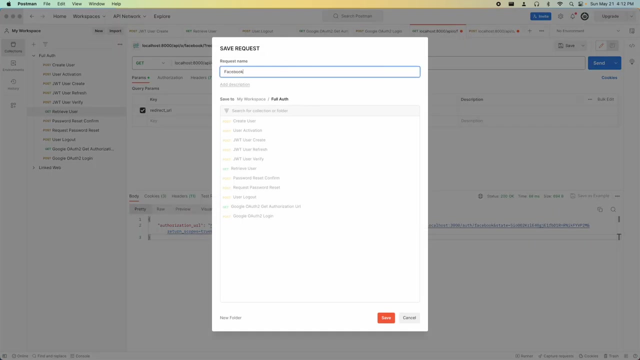 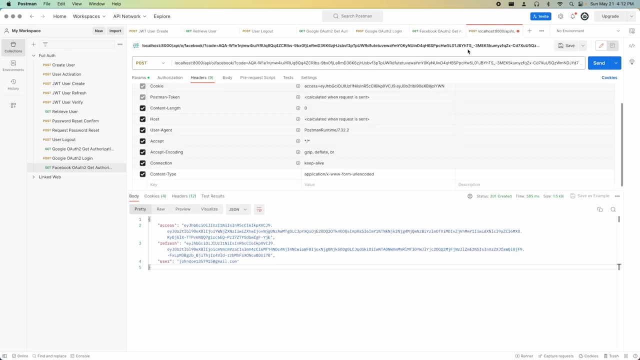 there now we still the same ID, so that didn't change, but the details are slightly different. so there we go. now we have Facebook and Google OAuth 2 working, so I'm just gonna save these now. so this one's gonna be Facebook OAuth to get authorization URL, and this one's gonna be. 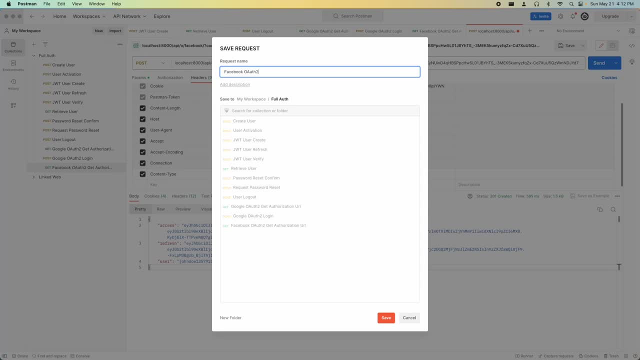 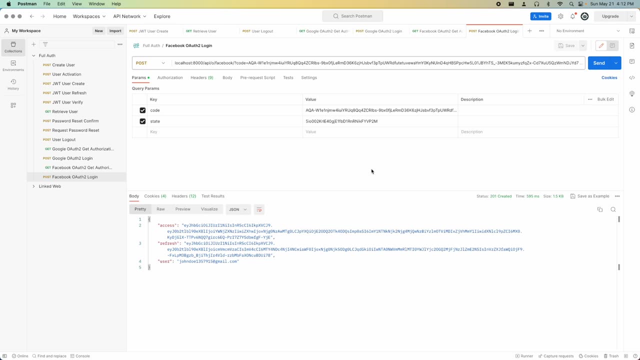 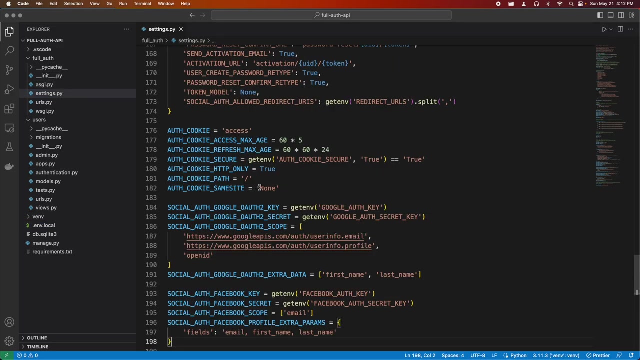 Facebook OAuth to login. all right, so only one thing left for us to do, and that is to deploy this back-end API, and then, after we deploy it, we have to test it now. before we do that, there are some things that we need to set up first. so, in particular, one thing we're gonna have to set up is right up here. where is it right here? 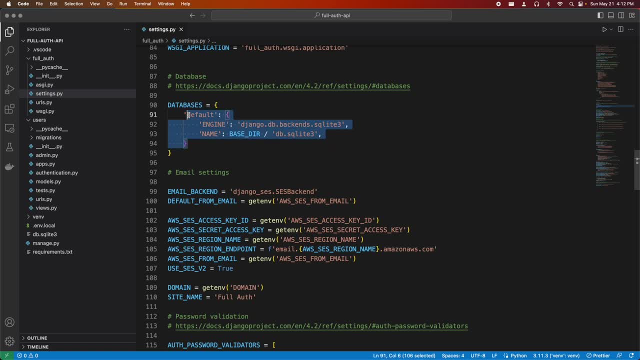 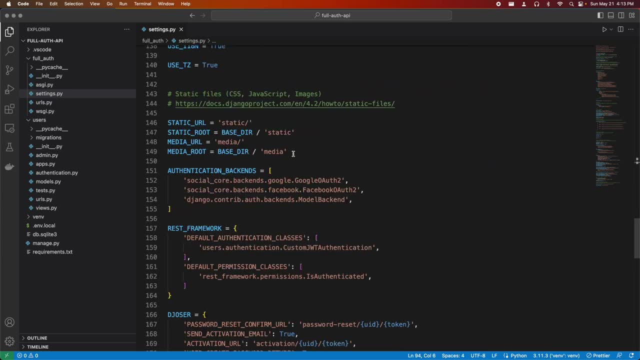 our databases. now we're using Sqlite, but in production we're gonna be using postsgres, and then another thing we have to do is the static URLs and the media URLs. so this is what we're using during development, but during production we're going to use digital ocean spaces. 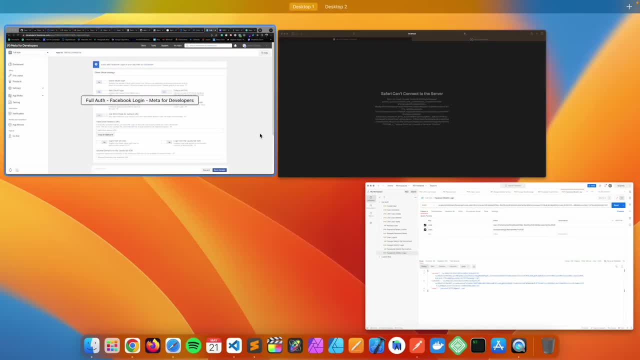 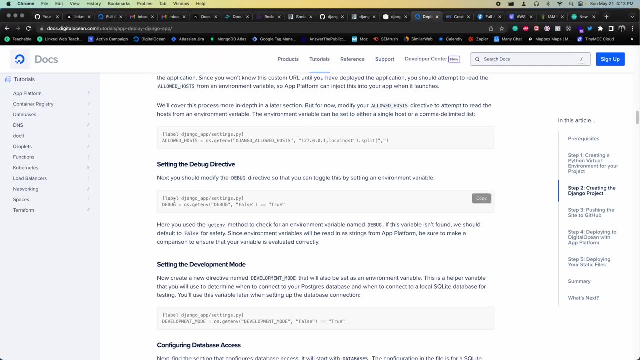 so let's see how we can configure that also. I can close out of this now, so I'm gonna open up this here. so this is that guide for digital ocean and just open up the project that's already in 달�os at the moment, but really essentially it's just 800 files with a document at the moment that has the digital. 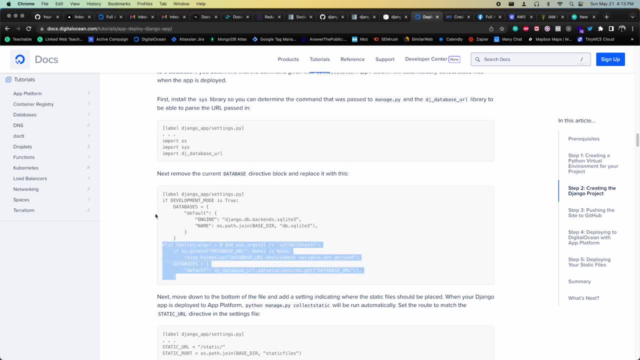 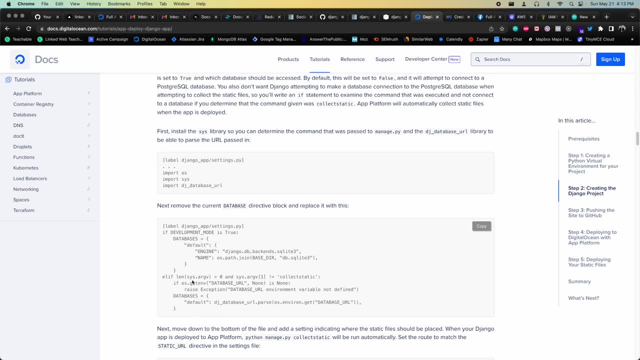 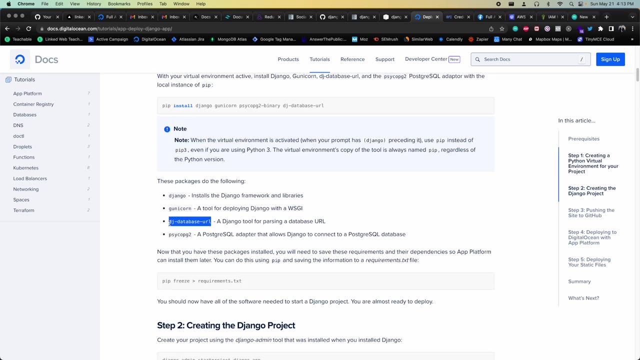 dango. So there is a section here and this is for setting up the database in production. So in particular, we're going to need a package, and it does mention it further up. So right over here we have dj database URL. So this is something we're going to have to install. 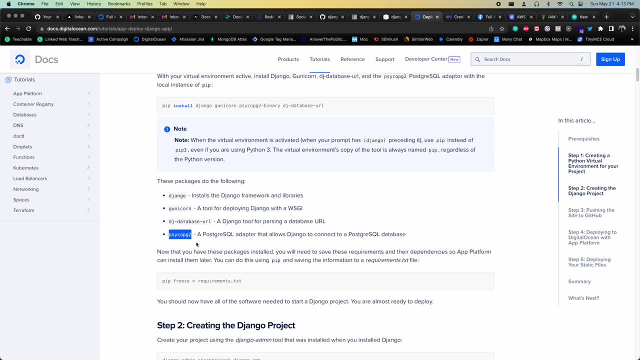 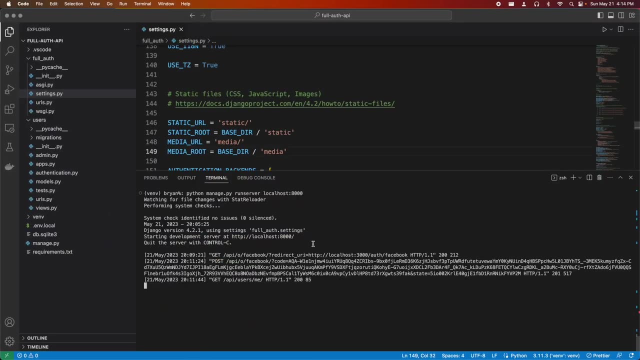 We're also going to need this PSY-COPG2 package. So this is a PostgreSQL adapter, And then we also need Gunicorn, And that's going to be for our web server. So let's go ahead and install these three packages. It's going to open this up. stop running. 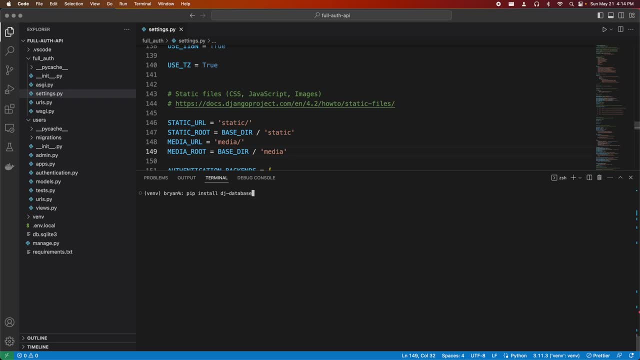 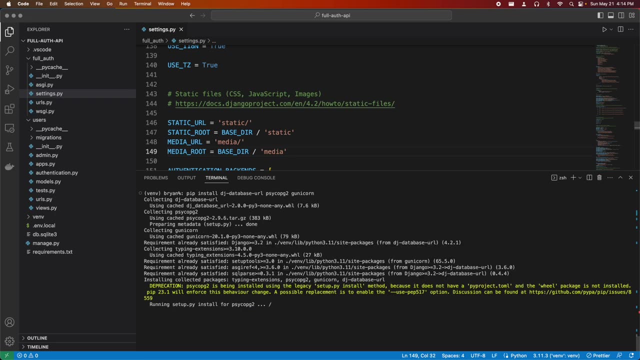 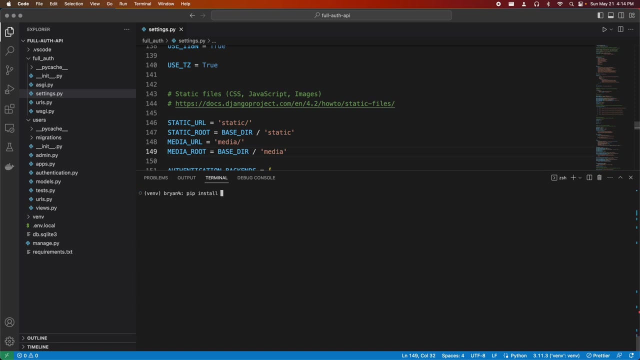 and then pip install, dj database URL, PSY-COPG2, and also Gunicorn. And then there's also going to be one additional thing we need to install. So I'm going to add another pip install and that's going to be for django-storages. 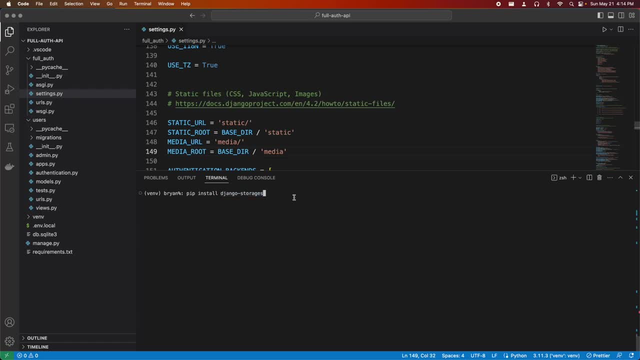 So this is what's going to allow us to set up using DigitalOcean Spaces in order to have our static files. So our static files are going to be stored in there, And with Django storages, you can also very easily configure this to work with AWS S3 as well. But in our case, 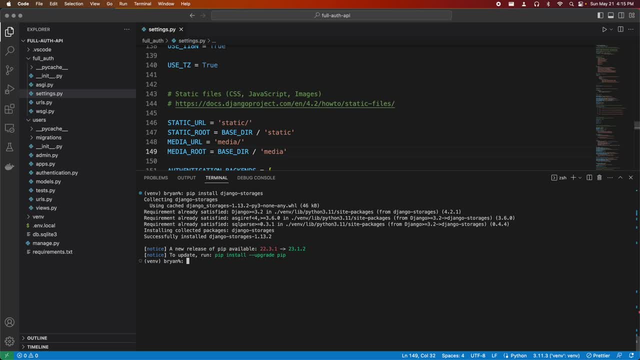 we're going to use DigitalOcean Spaces, So with that we have all the packages we need. So I'm just going to do a pip freeze requirements txt. So that's going to update our requirements txt to have everything it needs. And we need to make sure that this has everything we need because in production, 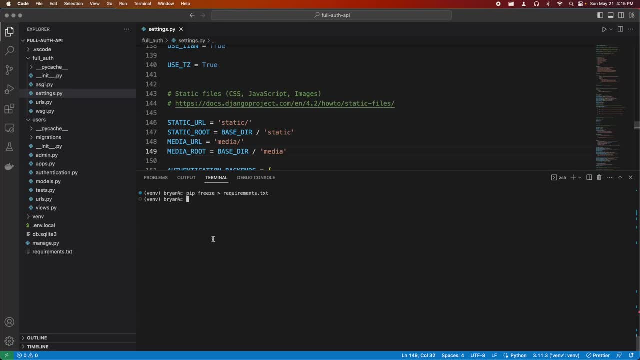 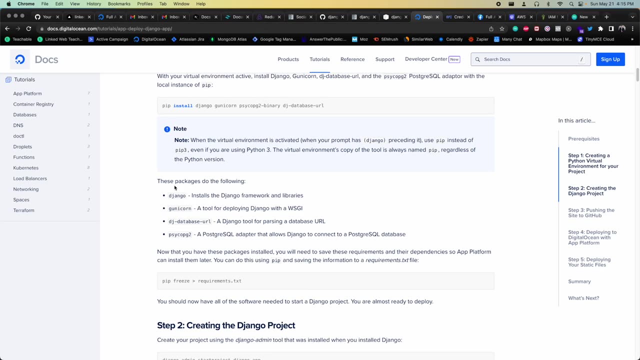 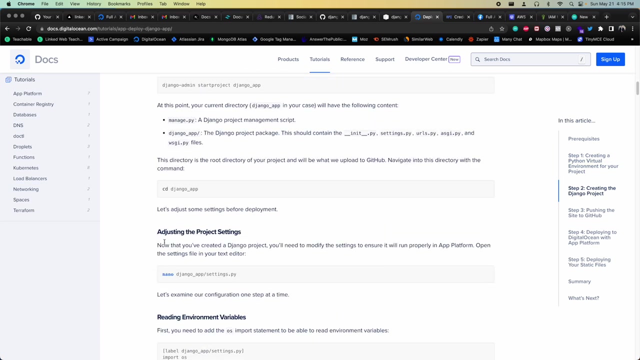 DigitalOcean app platform is going to read from that and install our dependencies, And if we're missing one, things are not going to work. I'm going to clear, I'm going to go back And then something that we also need to do. it was somewhere in here. it has to do with a 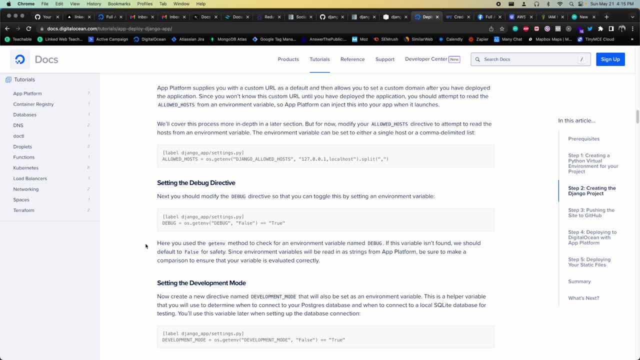 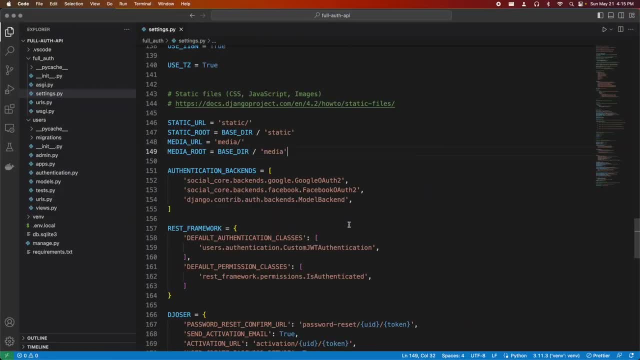 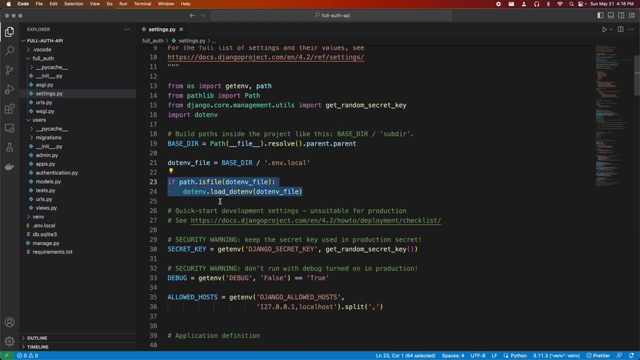 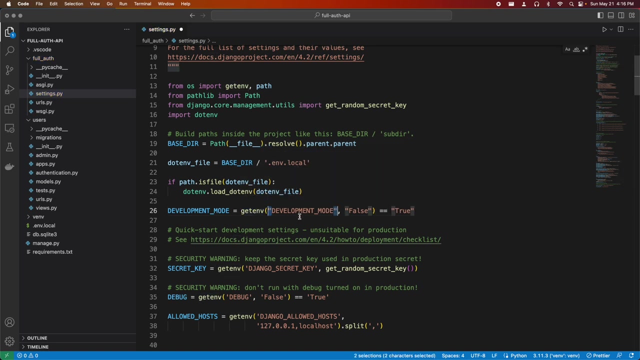 I'm going to copy this line And then I'm going to scroll up And then right below where I have this dot env stuff, This is where I'm going to paste this in and remove this OS part. So we're going to get an env called development mode And then by default it's going to be false. So in production, 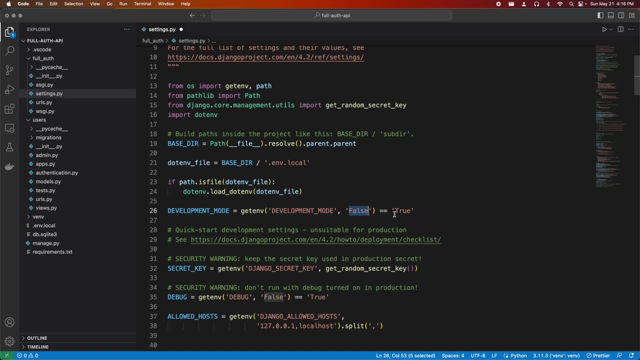 we don't have to set this thing. it's just going to be false. We're going to have false equals true, which is going to be a Boolean of false, But in our development environment we're going to have this thing be true. So true equals true is going to give. 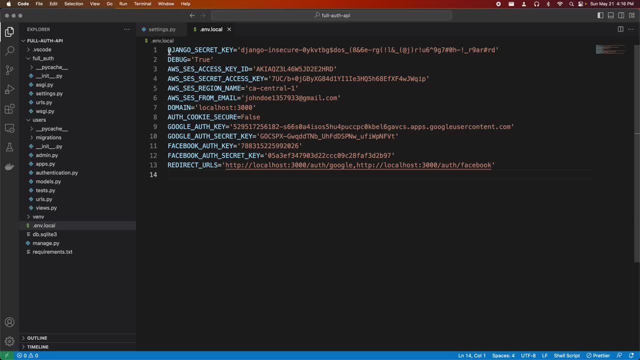 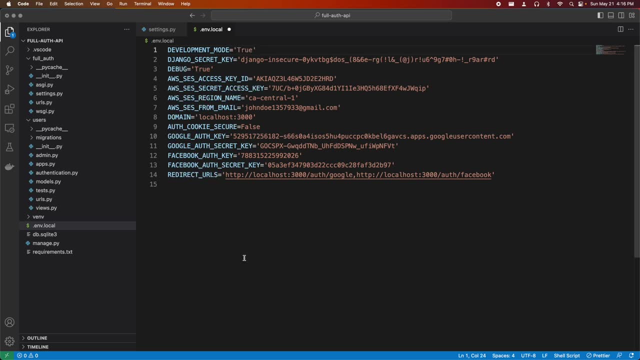 us a Boolean of true. So now I can open up my env local And at the top I'm going to set this equal to true And I guess I'll put quotes around it, since I've been doing that for the other environment variables- although you don't have to Also I can do that for this one. It's just more to make. 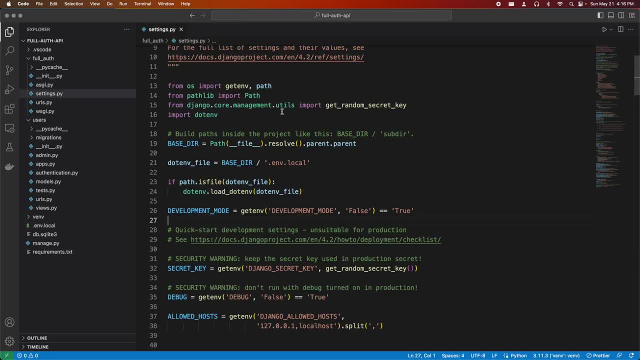 it clear that these variables are true. So I'm going to set this equal to true And I guess I'll put quotes around it, since I've been doing that for this one. So true equals, true is going to give us, are going to be strings, And then with that I can now scroll down. First thing I'm going to do: 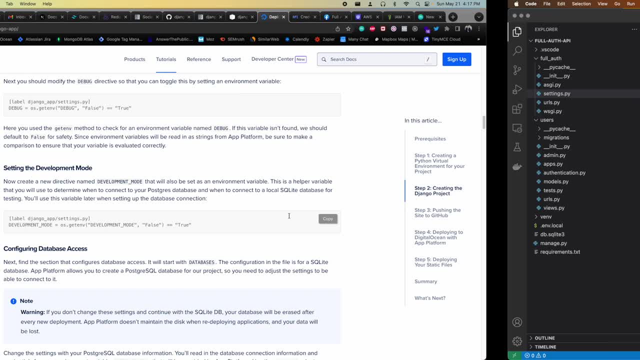 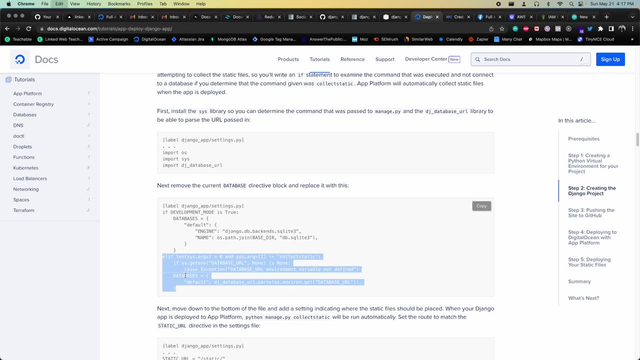 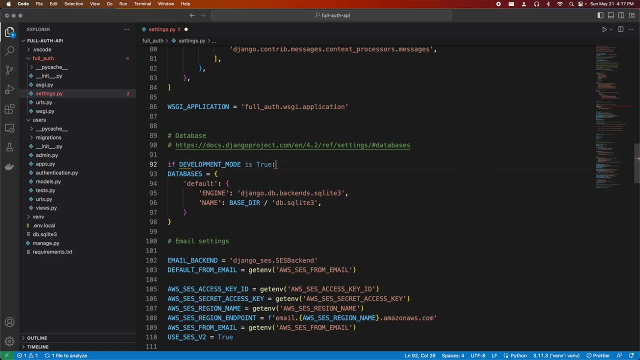 is the database configuration. So if I go back there's going to be that section on setting that up. So I'm just going to copy this line here And then I'm going to check if development mode is true. If it is, we're going to do this And then l if 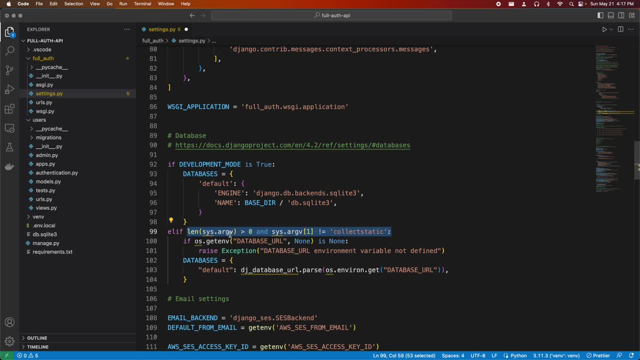 So if we're not doing collect static, then we're going to do this here, which is grabbing the database URL from our environment variables. If that doesn't exist, we're going to raise an exception. Otherwise, we're going to set databases equal to this right here, And that's going to. 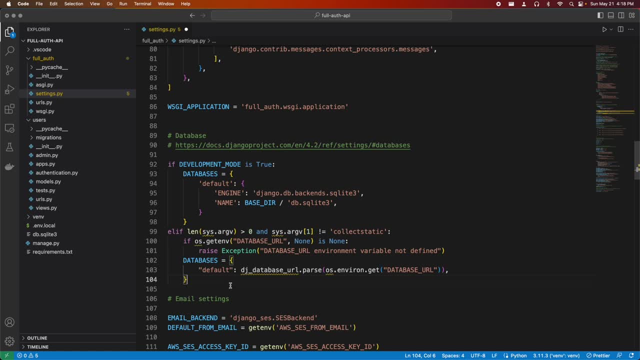 configure our default database to be set up in production with the default database, And then we're going to do that with Postgres. So this is an easy way to do it. Now you can also do it the same way as you have right here. You don't have to use this package, So I can just set up the 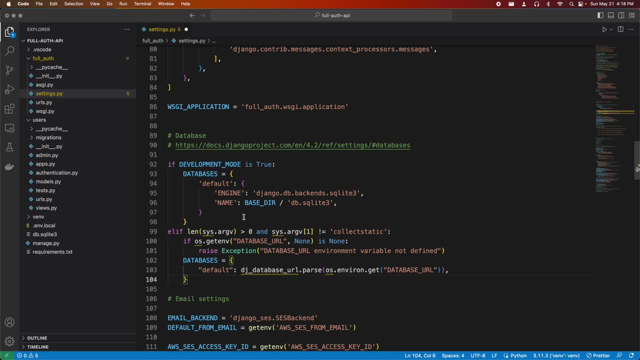 engine name, then the user host and all that stuff, And then I can have a longer configuration here, Or I can just use this, which makes it a little bit easier. So now I'm going to have to switch some things up here, So I'm just going to have get env, I'm going to use single quotes. 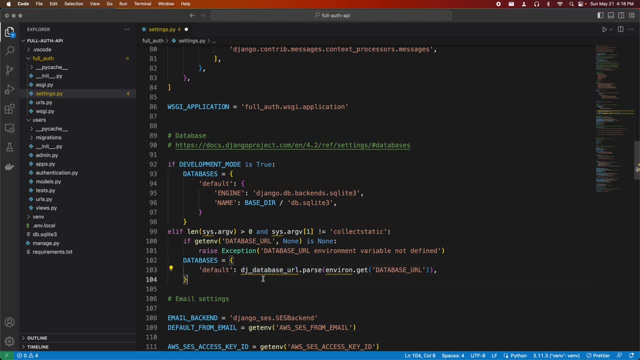 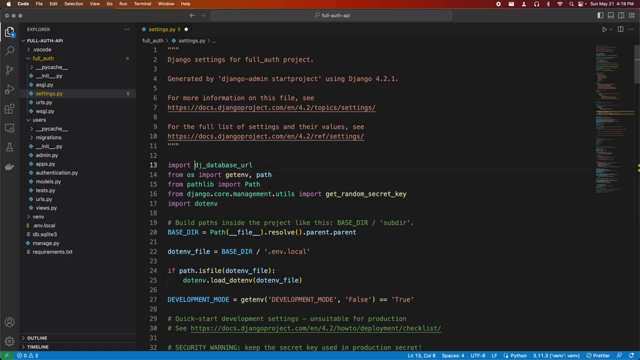 And then here I'm also going to get rid of the OS. Then I have to import this. So at the top I'm going to go right here And I'm going to import dj database URL And I'm also going to. 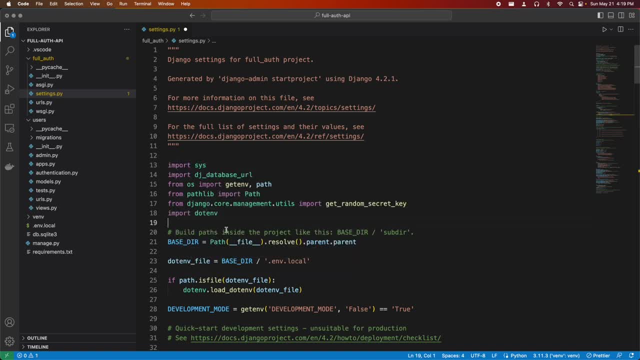 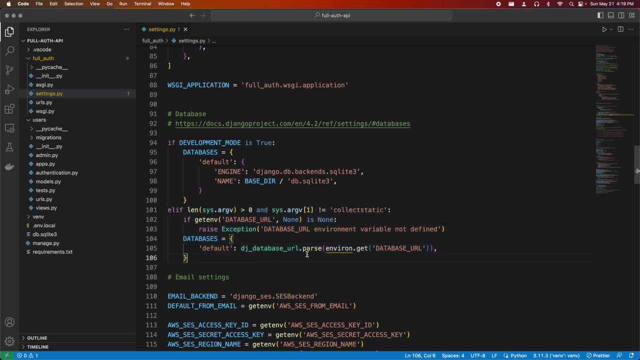 import sys, since that's something that I need in order to access the arguments. So if I scroll back down, we shouldn't have any other issues here, Although we do, since this has to actually be get env And now we shouldn't have any other issues. 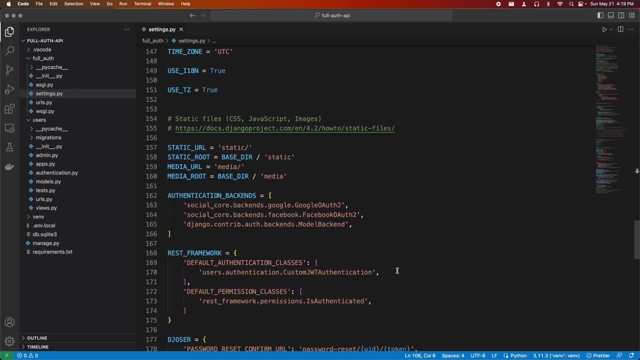 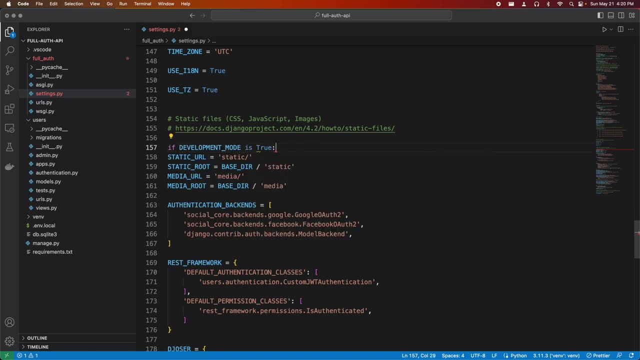 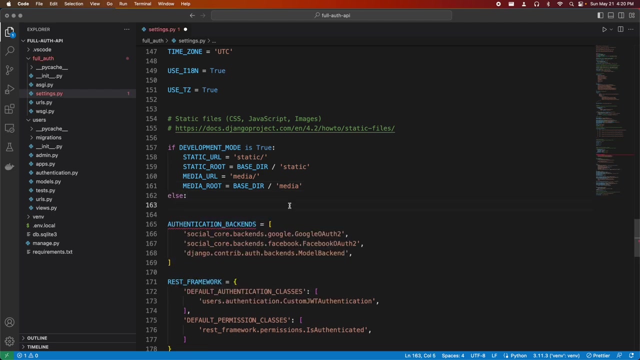 So with that, our next step is going to be now the static settings. So we're going to want to do something pretty similar. So if development mode is true, then we're going to do this. Otherwise, we're going to use our production settings. So one thing we're going to have to do is go into 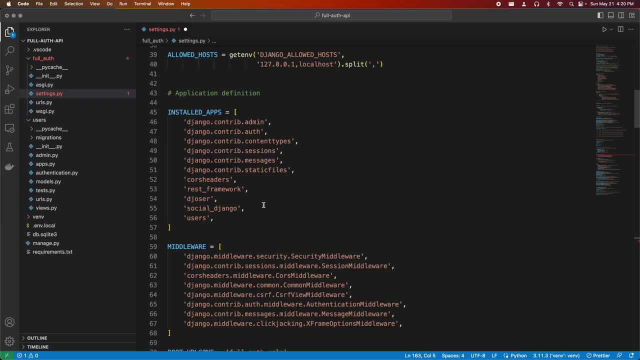 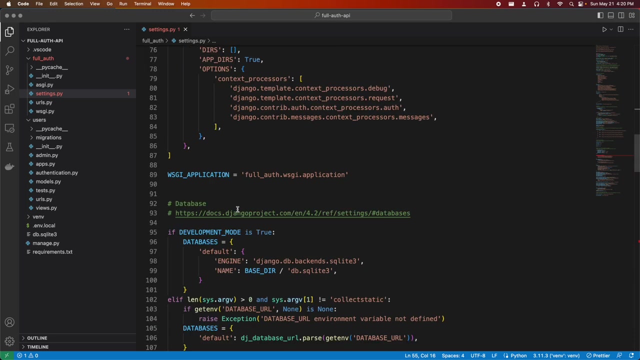 our installed apps And then we installed that Django storages package. So then right below, say, here I'll put in storages, So that's going to be the app name for Django storages. Then I can go back down And then this is where I'm going to have all of those settings for Django. 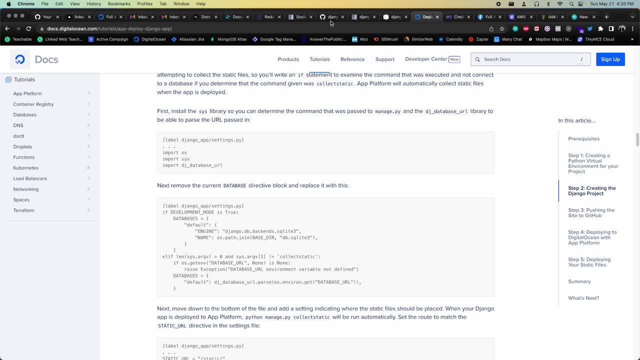 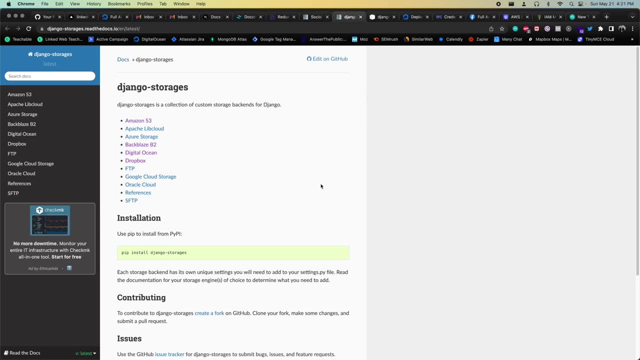 storages. So let's see what things we have to set up. So one of these is for Django storages, So this one here and I don't need this anymore. So here we have what we have to do, So we have. 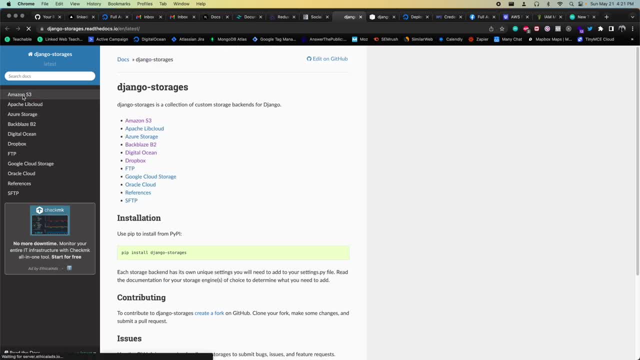 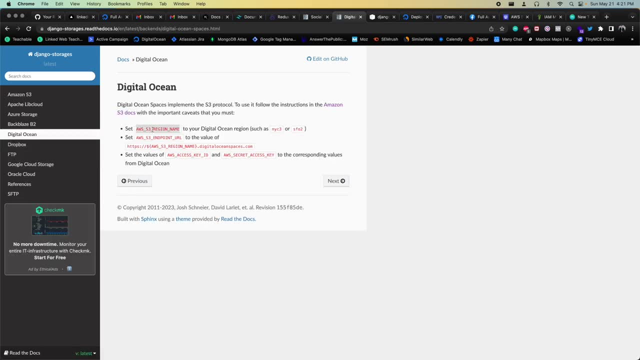 to install. And then you have Amazon sd S3.. This is where the majority of these settings you're going to find. We also have digital ocean. This is going to show you the ones you need to set up for digital ocean. So the 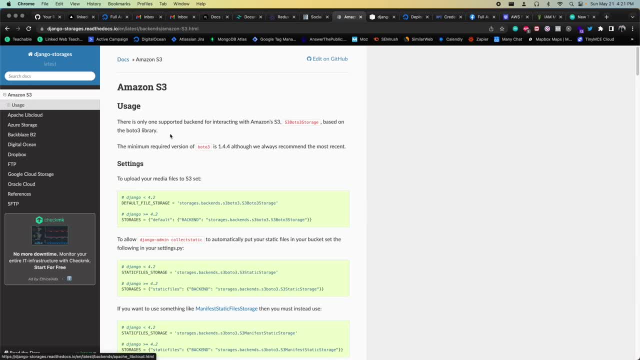 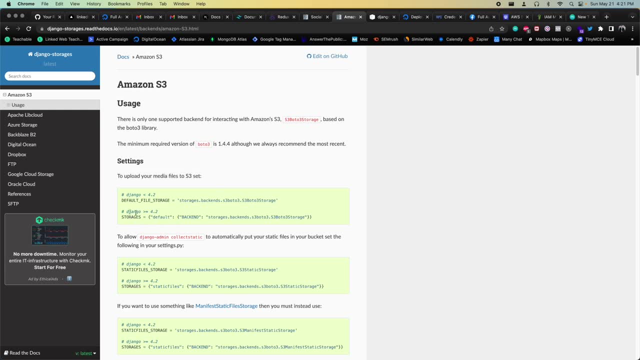 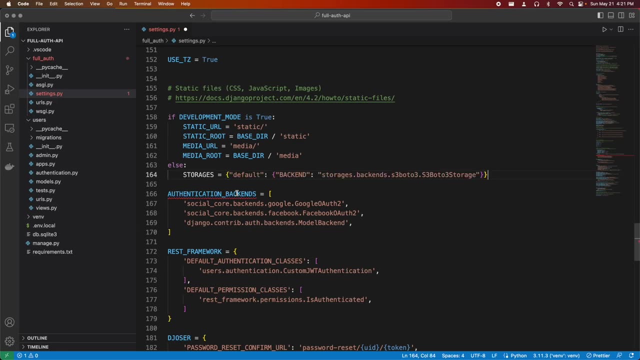 region name as well as the endpoint, But most of the settings we're going to grab from here. So first of all, this is going to be for media files. So if we're using Django version that's greater than 4.2, we want this in our case- we are going to grab that and paste that here. 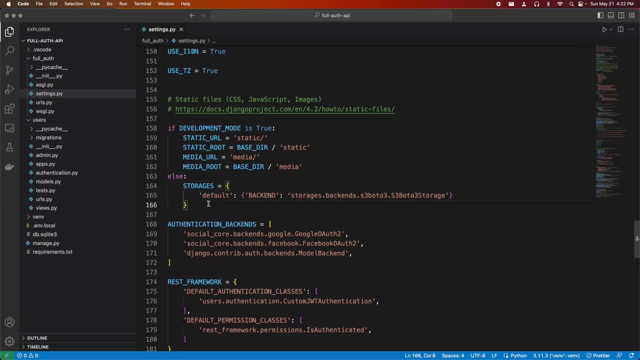 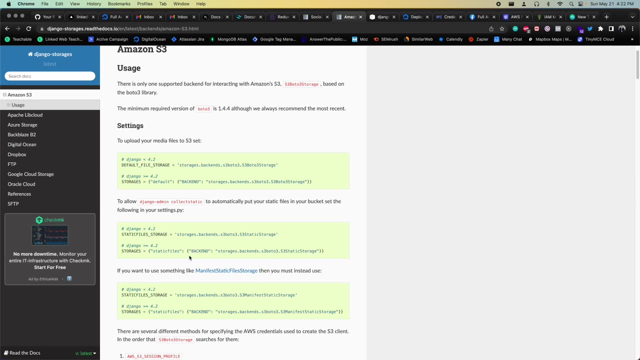 So there we go, I'm going to go back And then this one's going to be for static files. Now, this particular project, this setup, of course, is a little bit overkill, since our only static files we have in our entire project are just the ones for, like, the admin, because we do have that admin. 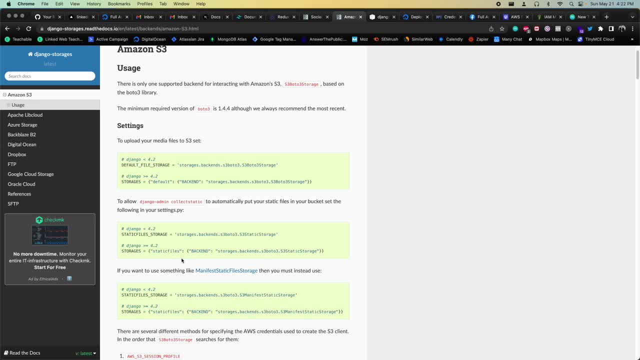 panel, But in maybe a more production app where you have a lot of features, then this could be useful. This is more just to show you how to do that, So I'm going to go back to my project And I'm going to show you how to do this, more so than it being something that makes sense to have in. 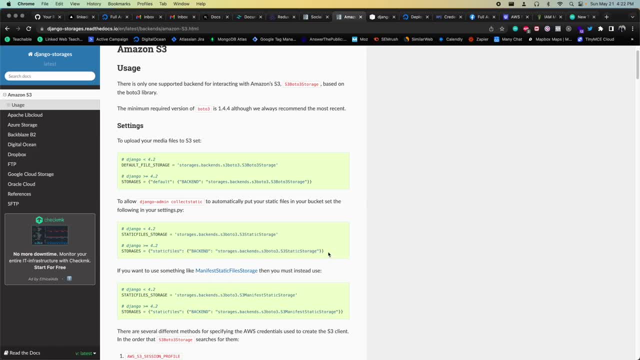 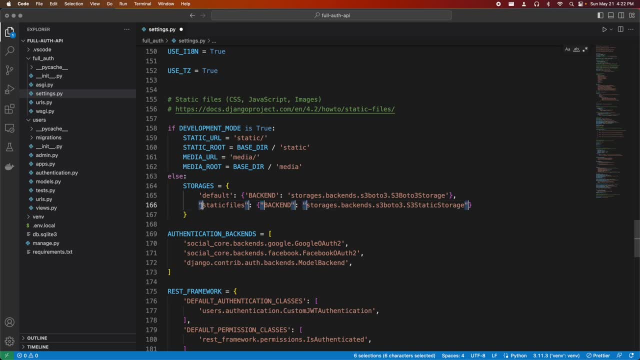 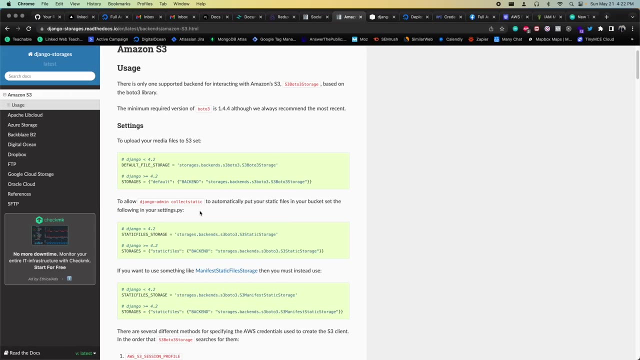 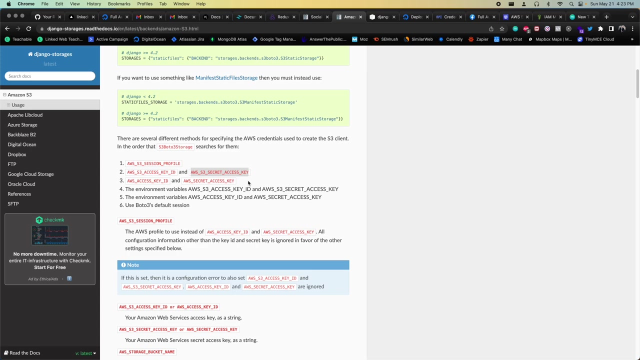 this project. I'm going to copy this now And then below here I'm going to paste that. Use my single quotes. That's going to set up my storages, And then I need a couple more settings. So if I scroll down, we have AWS S3 access key ID as well as the secret access key. So I'm going to need 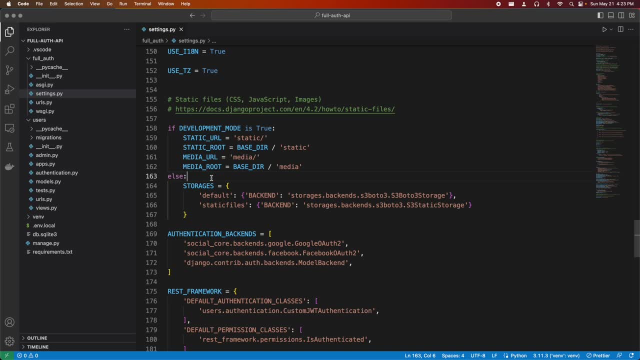 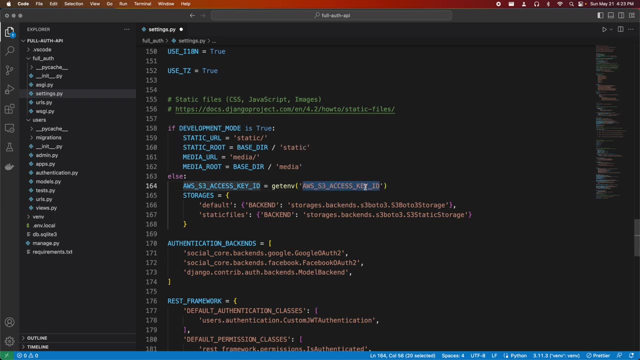 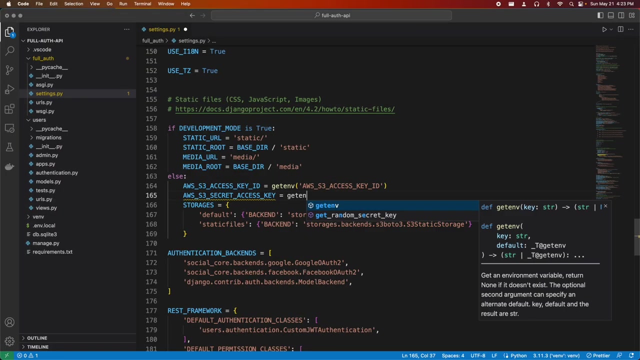 that, And then this one's going to be equal to get EMV, And I'm just going to have the exact same name for the environment variable. I'm also going to want the secret key And I'm going to paste that: get EMV, And it's going to have the same name. And then, if we go into the digital ocean, 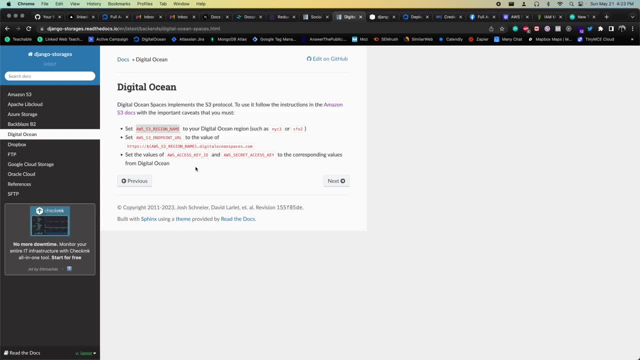 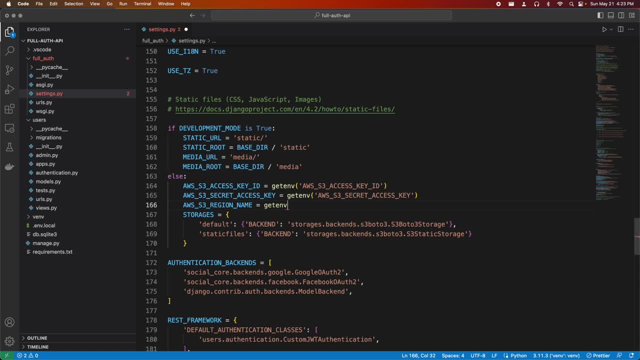 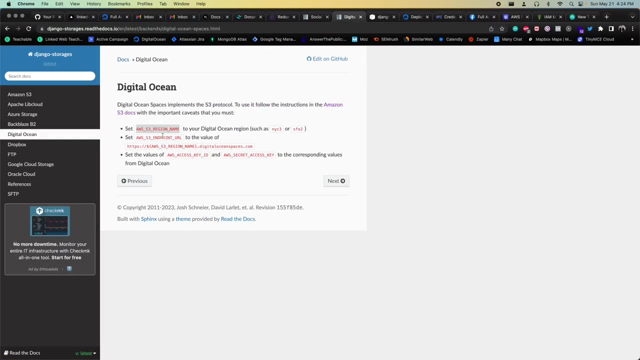 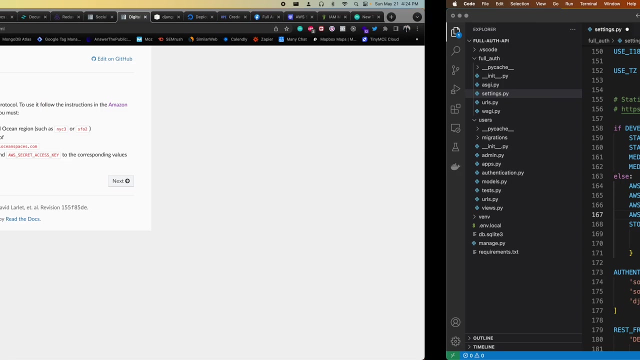 settings. we're going to need this here, So that's the region name And I'm going to get that from an environment variable which is just going to have the same name. Then I'm going to need the endpoint, And in this case it's going to be an F string. I'm 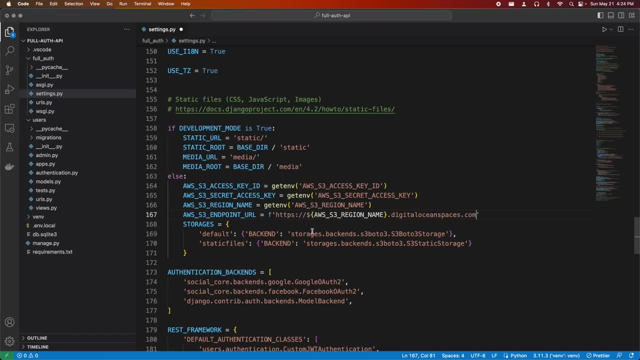 going to grab this value here. I'm going to paste it here. It's just going to be HTTPS colon, slash, slash. And then here I'm going to paste it here, And then I'm going to paste it here, And then here they also put in this dollar sign. You don't want the dollar sign. That shouldn't be. 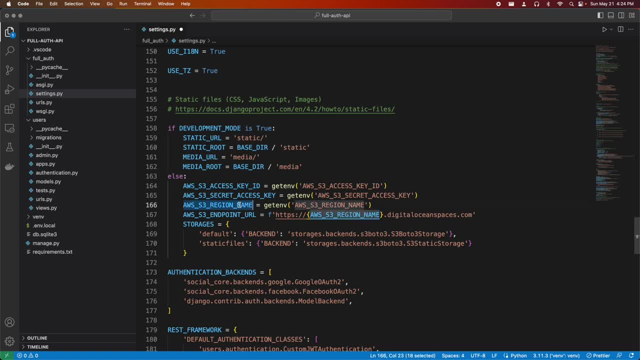 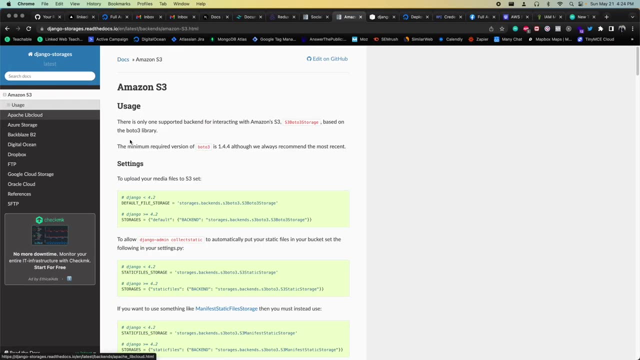 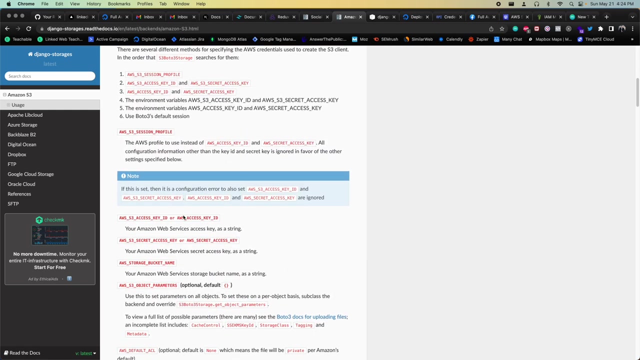 there. So we're going to have the region name which we're grabbing from here- dot digital ocean spaces dot com- And we'll go back go into the S3 settings. There's a couple other things that we need. So if we scroll down we have the storage bucket name. That's something we need. 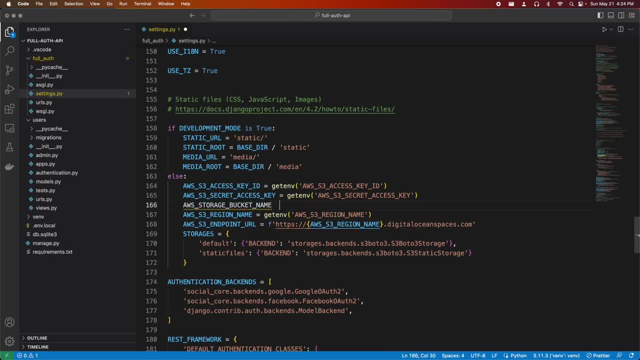 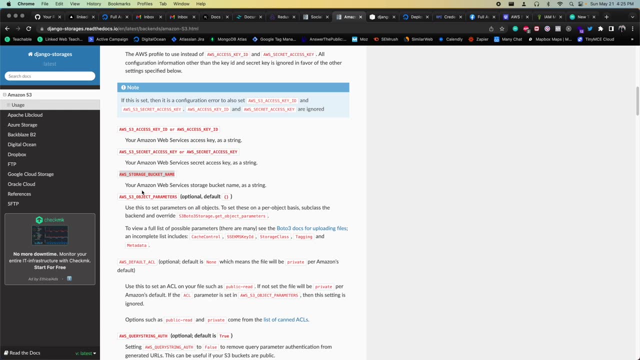 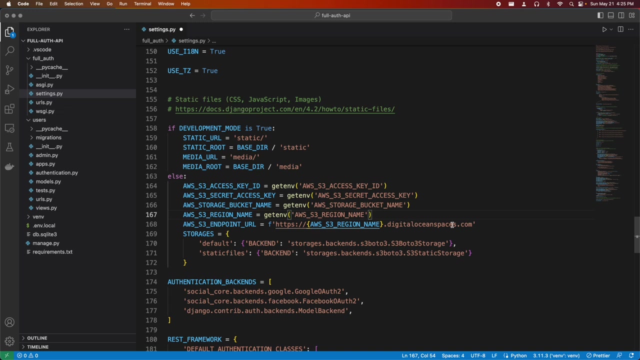 So I'll put that right below here. And then something else we're going to need is the AWS S3 object parameters. So I'll put that say below here, And that's going to be a dictionary with cache control And that's going to have max age equal to eight, six, four, zero, zero, And then 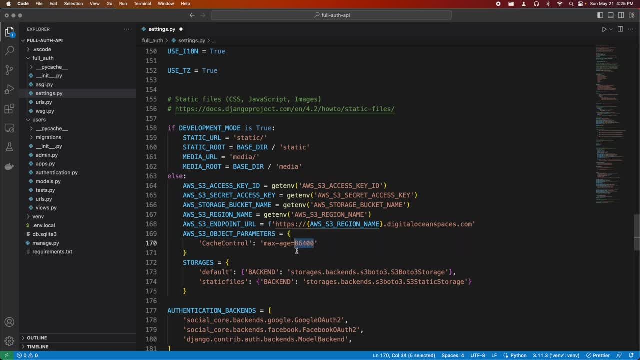 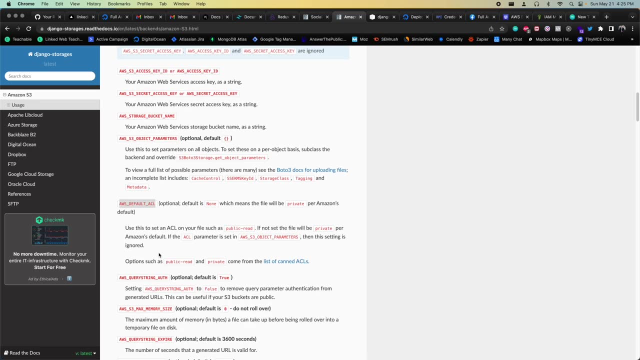 eight six four zero zero seconds is equivalent to one day. then i'm gonna go back, i'm gonna grab this aws default acl, so by default this is none, and then options such as public read and private come from here and then use this to set this to public read. if not, it'll be set to private. 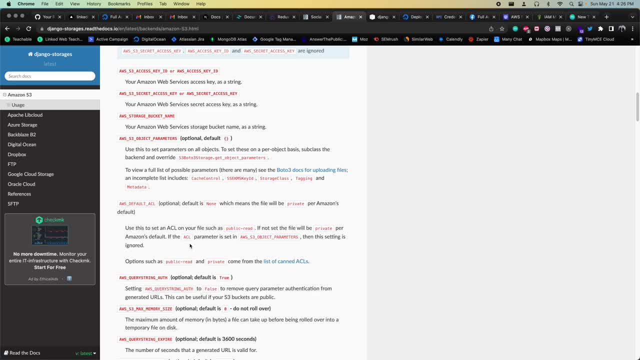 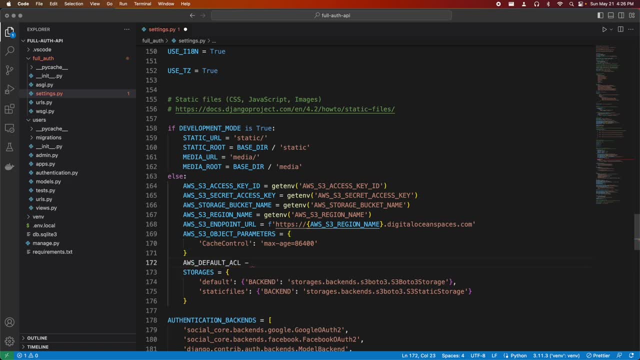 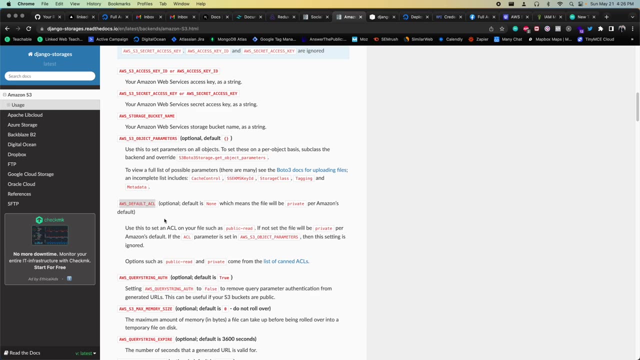 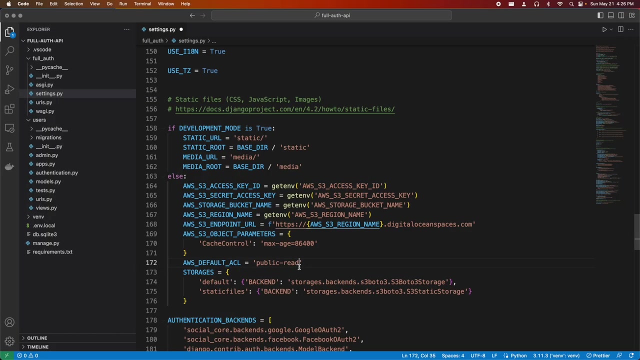 and we don't want it to be private. we want to be able to access what's in the storage, so that's going to be equal to public dash read and then, after that- i'm going to scroll down- we're going to grab the aws location and this is going to be static, so this is going to be the file. 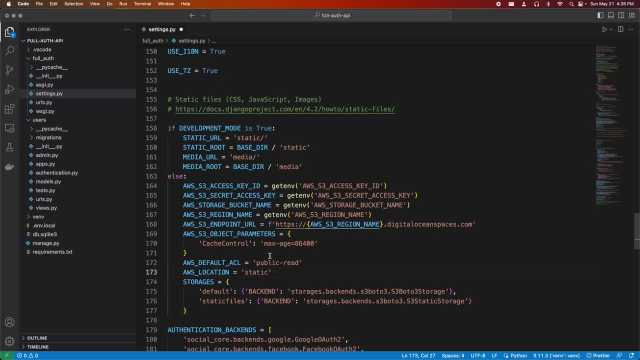 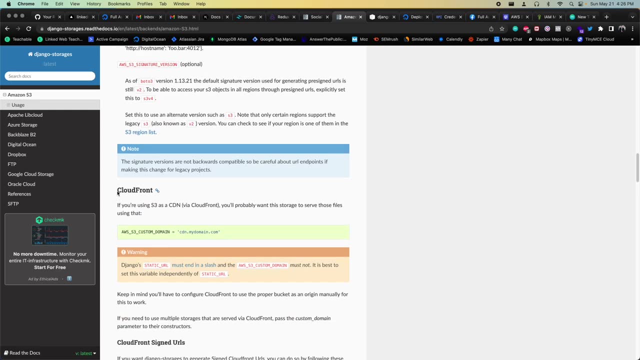 in which we have the static files inside of this bucket, and then there's only one, and then there's only one, and then there's only one more thing that we need. So if we scroll down, we have this CloudFront section where we have an AWS. 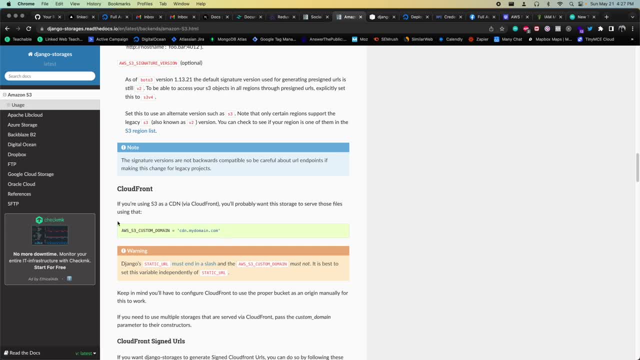 S3 custom domain that we can set up Now. CloudFront is something specific to AWS, although with DigitalOcean we can still use the same setting. So this setting is going to let us set up a custom domain for our CDN So we can configure a CDN on DigitalOcean spaces and then a CDN is a. 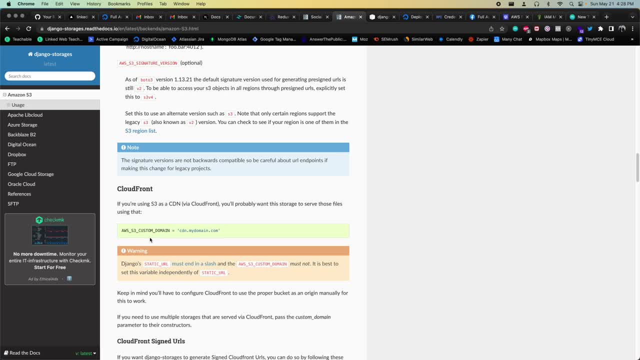 content delivery network and it's going to make fetching any data inside of our DigitalOcean spaces buckets much faster. So that's why we want to use this And we don't have to use a custom domain, but we can configure one and it'll just be much nicer to have a custom domain for that. 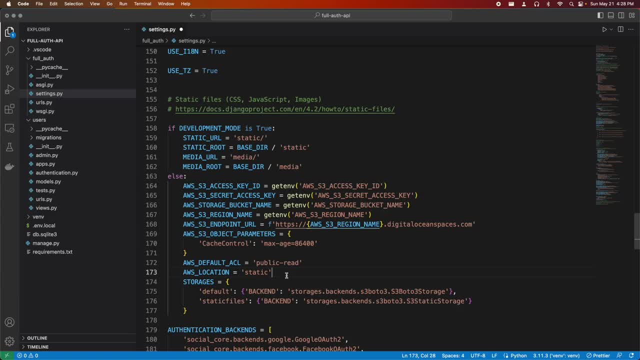 So we're going to go ahead and do that, So I'll put that setting here and that'll be get ENV And I'll have that right here. Now, all of these environment variables we configured here, we don't have to touch those inside of our ENV local because these are all only for production. 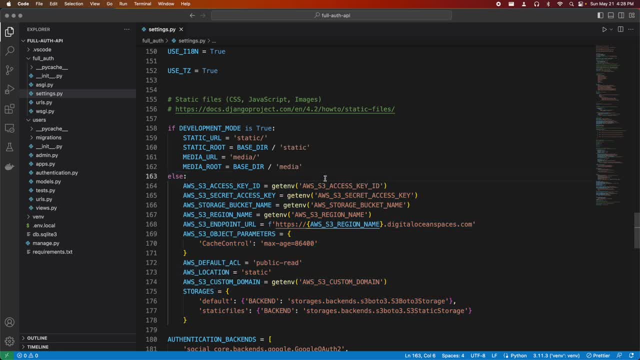 as well as the database URL settings. So all of these are production only, So we're going to have to configure those in DigitalOcean's app platform. So with that we should be officially done with writing code for this project, And now we just have to have a deployment to be successful. So 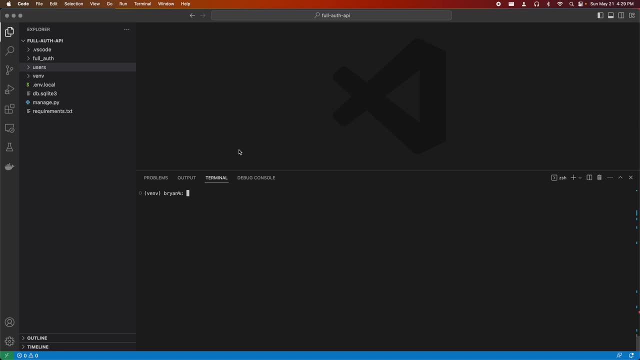 that's going to be our final step. First thing I'm going to do: I'm just going to deactivate this and I'm going to go ahead and do that. So I'm going to go ahead and do that. So I'm going to. do that. So I'm going to go ahead and do that. So I'm going to go ahead and do that. So I'm going to do that. So I'm going to go ahead and do that. So I'm going to do a git init, So I'm going to set. 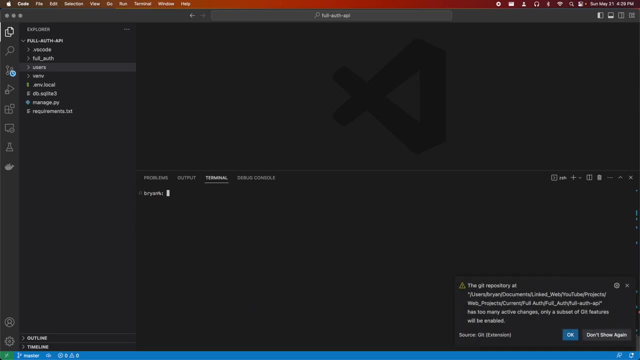 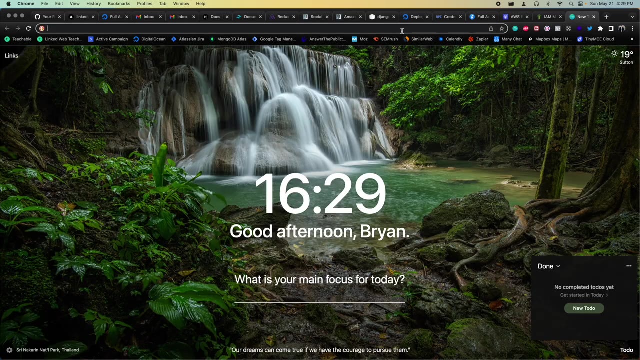 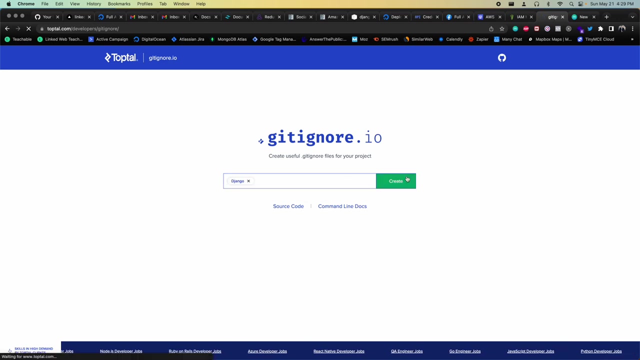 up a git repository in here, And then the next thing I'm going to do is: I'm not going to add quite yet, So I'm going to navigate to a site called gitignoreio. I'm going to type in Django. That's going to generate a gitignore for a Django project. 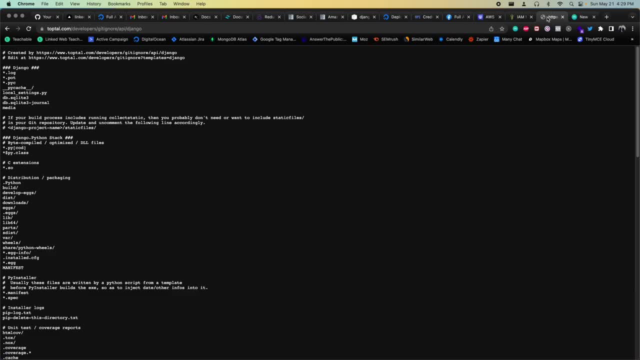 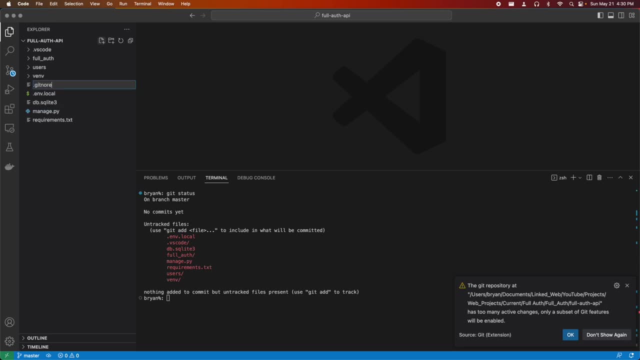 So I'm going to copy everything on there using command A and then just command C, And then back in my project I'll make a gitignore file. I'm just going to paste all of that in here and then save. 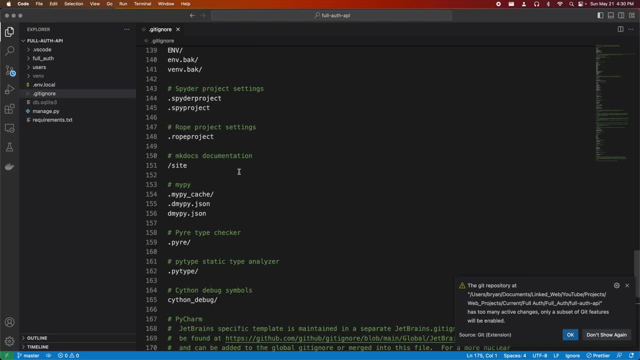 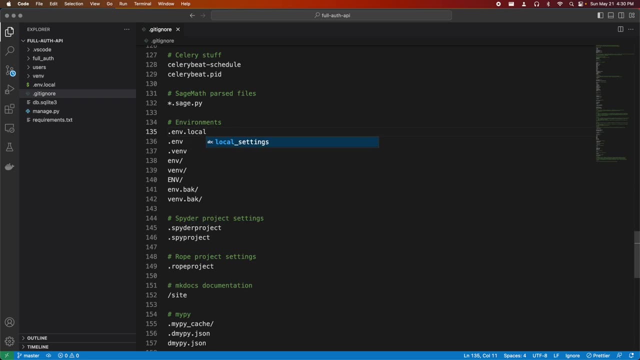 So now this envlocal, that's something I have to add in here. So under the environments that's just going to be an additional thing I add. So envlocal I'm going to save, and then that should grade that out as well. 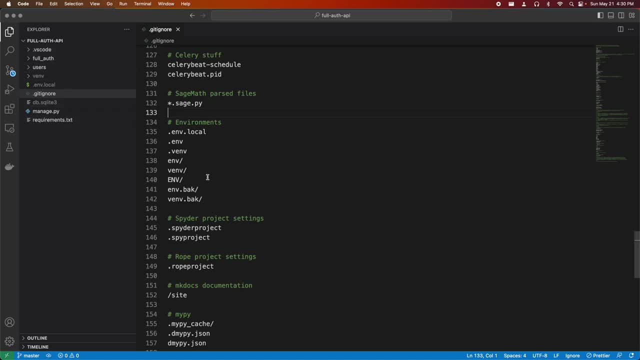 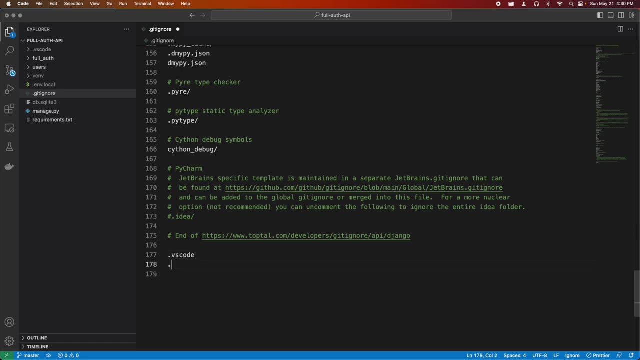 And then I also want to gray out this ds code, So I'll do that at the bottom, And then the last thing I want to do is add a ds store, which is just some file that oftentimes gets added with Mac. So I just don't want this thing to get committed, And with that we are. 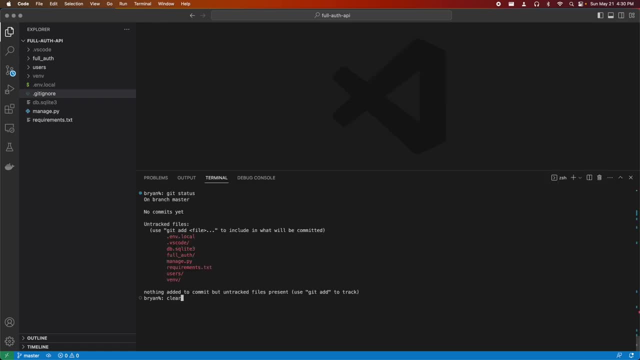 now good to make our initial commit. So I'm going to clear, do another git status. see what we have. So we have the gitignore, the project folder, managepy, requirementstxt and the user's app. So I'm going to do git add dot. 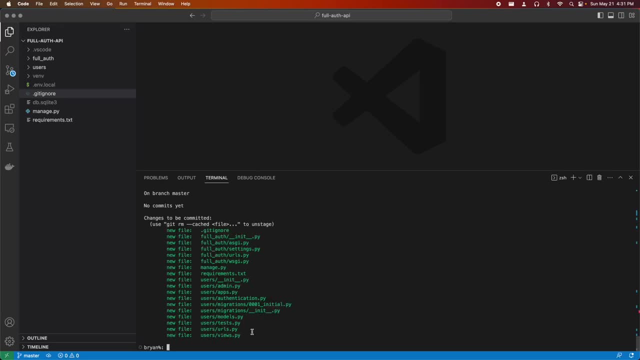 I'm going to clear, do another git status And these are going to be all the files that we add. So I'm going to clear once again: git commit dash m. Initial commit will be my message. There we are. I'm going to do a git branch dash a. So right now we have a master branch. 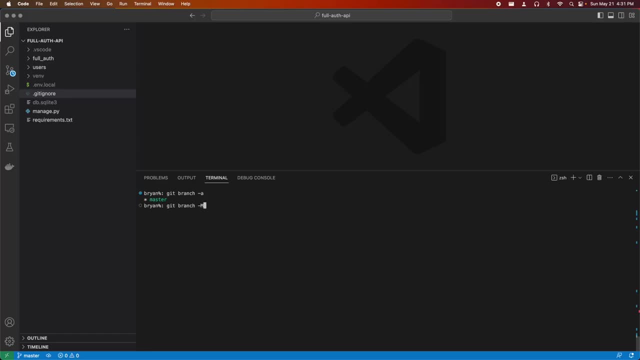 and I'm just going to rename this using git branch, And then another git branch, dash a, And then we can see that this was renamed to main. And that's just because in GitHub when you create a repository, by default it just has you set. 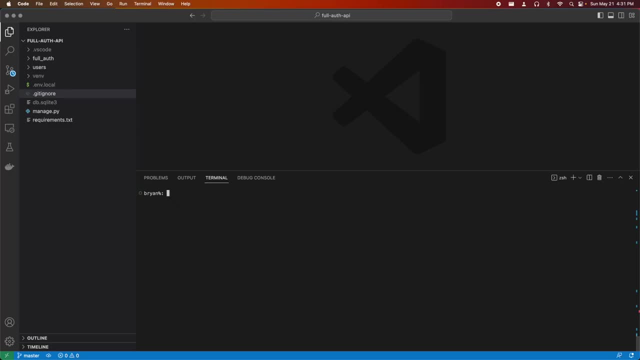 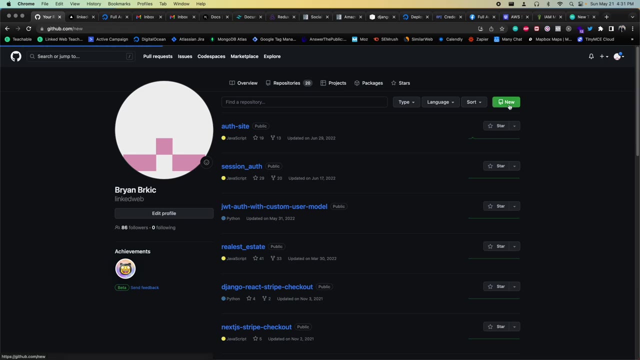 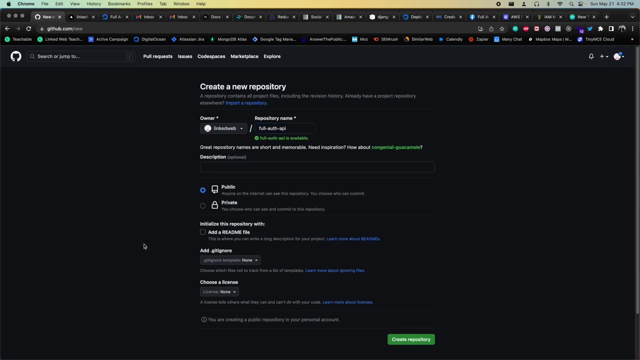 it to this. So I'll just do it that way. And then, going back, I have GitHub open And then I'm going to create a new repository. Now I'm going to call this full dash auth dash API. It's going to be public, I'm going to create it, And then here the steps: git init Also. 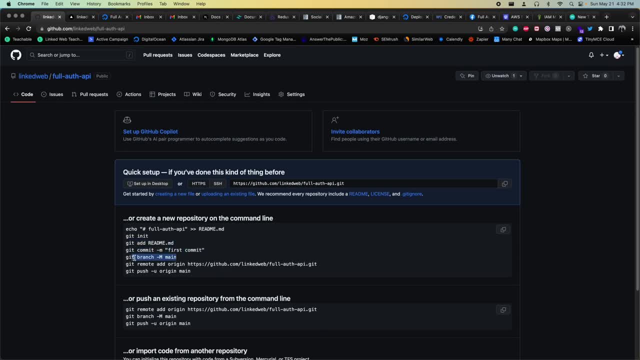 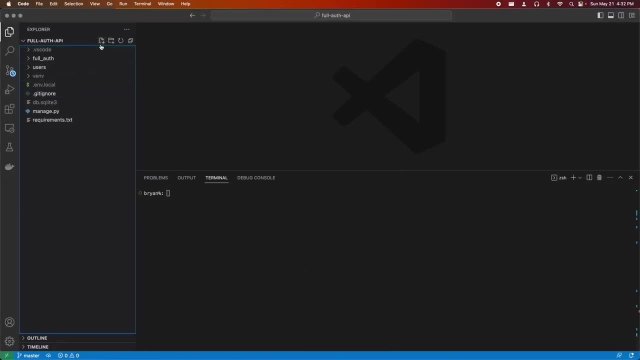 I'm going to add a readme And then we need a commit, And then- this is that step I just talked about- And then we can add the remotes. Before that, I'm just going to quickly add a readme And then I'll do full auth API. 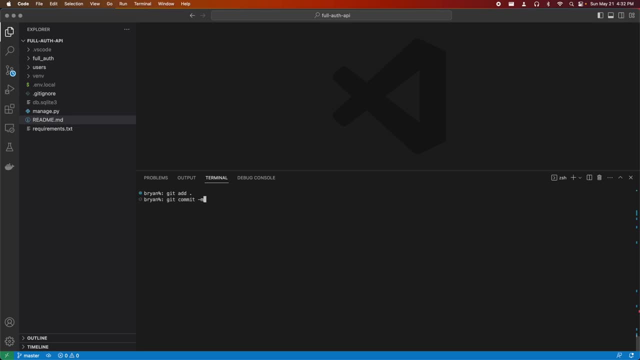 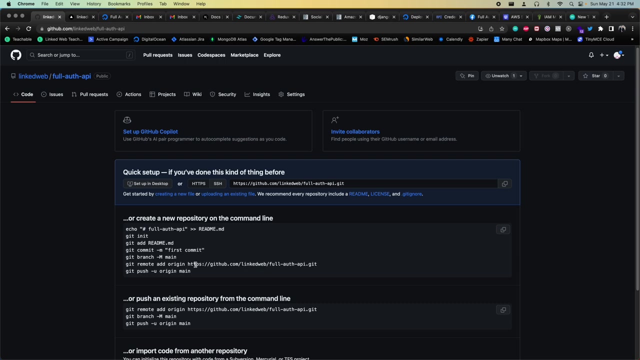 And then git add dot, git commit, And then add readme, And then I'm going to do a git remote add origin, Just like here: git remote add origin. then you're going to add your origin. Now, in your case, you're probably just going to do whatever's. 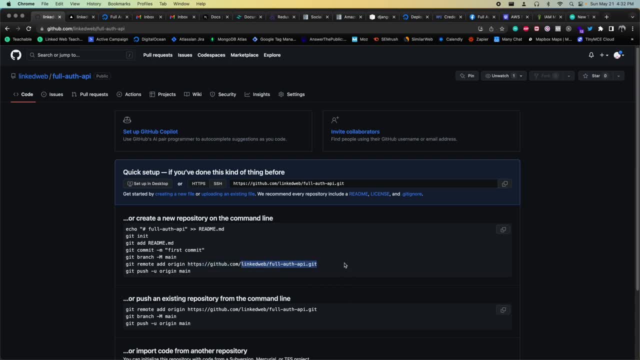 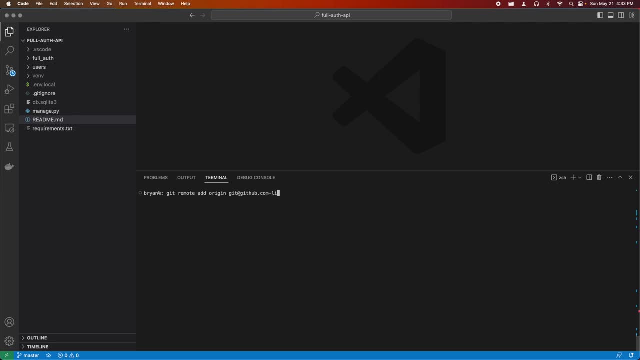 written here, But in my case it's going to be slightly different. So in my case I'm going to have git at githubcom, dash linked web colon and then this right here: So linked web: dash full auth API dot. 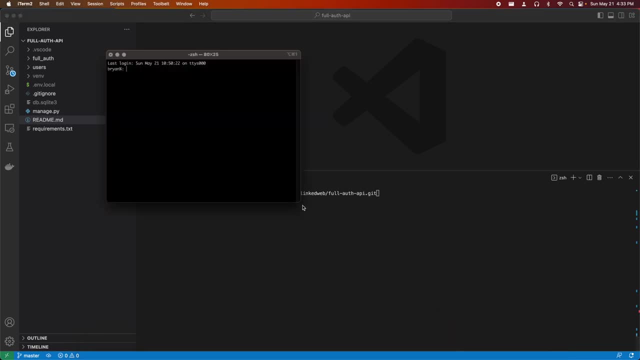 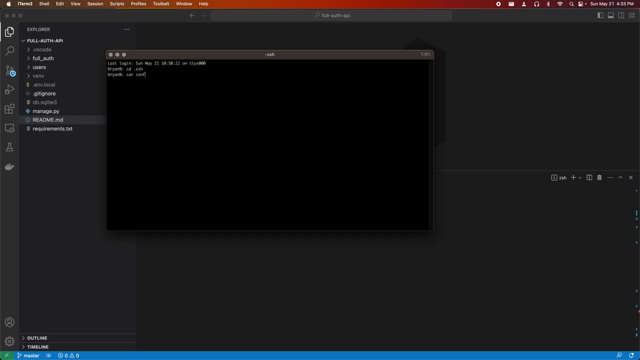 git. Now, the reason for that is because I manage multiple GitHub accounts. So inside of my home directory, if I go into my dot SSH and do a cat on config, So in particular when I do get at githubcom dash linked web, I'm going to have an SSH key that's linked to that GitHub account. 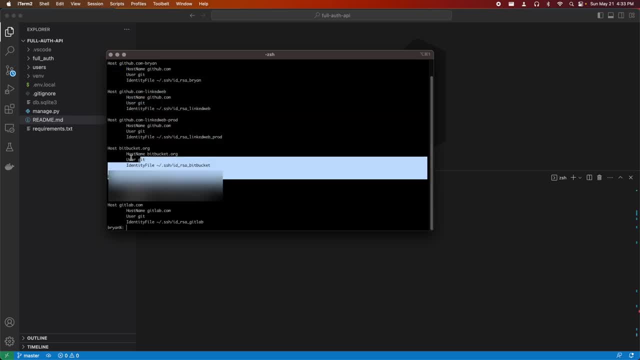 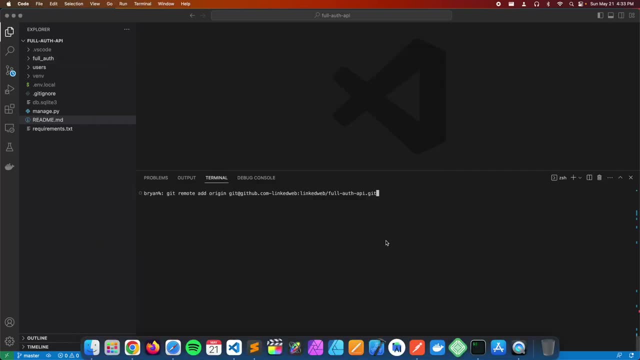 So right here you can see I have many different repositories, So in my case this is just how I manage it, So with that I can click enter. Now in your case, you're just going to do git at githubcom without. 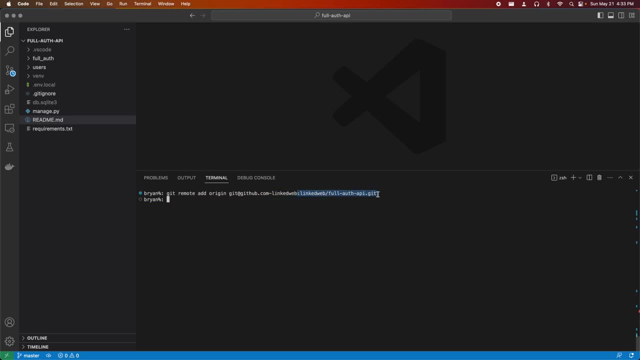 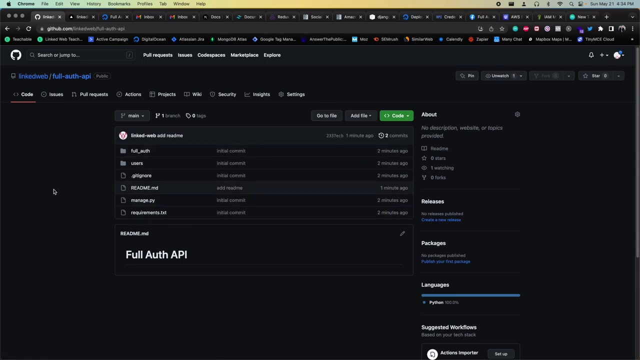 this part and then colon and then the path to your repository. Last thing I have to do is git push dash u origin main. There we go, And now I can flip back here, do a refresh And there's our code. So next I'm going. 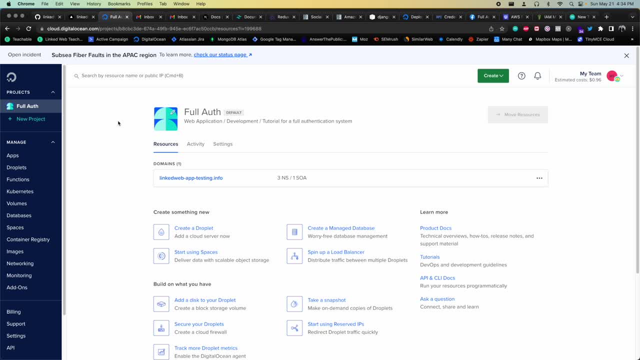 to do is go into DigitalOcean. So if you don't have a DigitalOcean account, you're going to want to create one. And then, one thing that you'll notice: I already have a project which I called full auth and I have a domain set up. Now, I set this up ahead of time, just because it takes time. 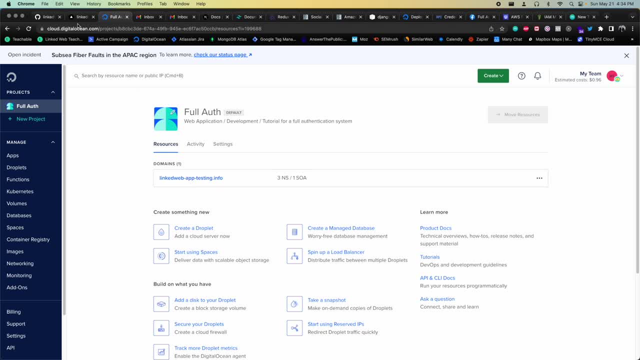 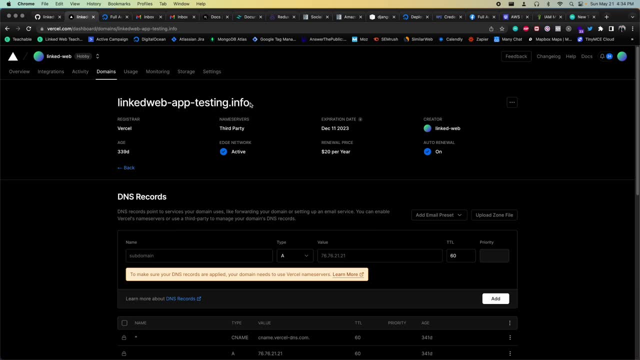 to have things propagate. So I have a domain in particular on Vercel And it's called linked web app testinginfo. It's just what I use for testing when I need a domain, And then inside of here I set the name servers to be. 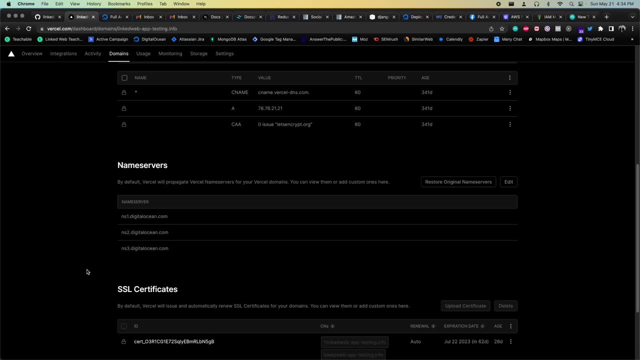 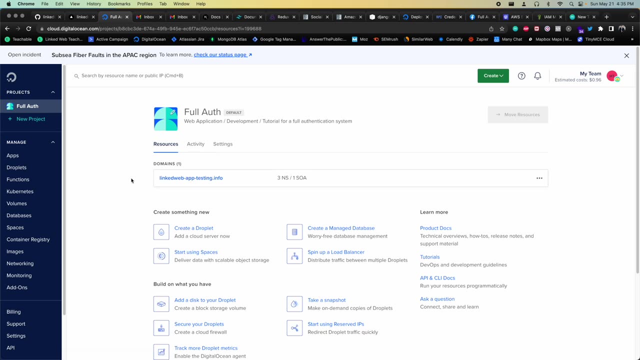 DigitalOcean name servers. So this is how you can get DigitalOcean to manage your domain. So right now Vercel is not managing this. Right now DigitalOcean is managing this because the name servers are set to DigitalOceans And then if I click into here, I don't really have anything. 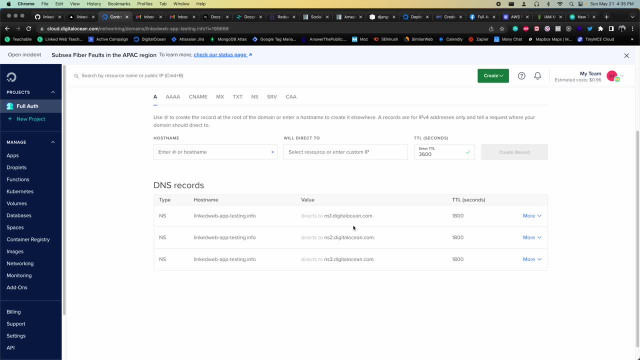 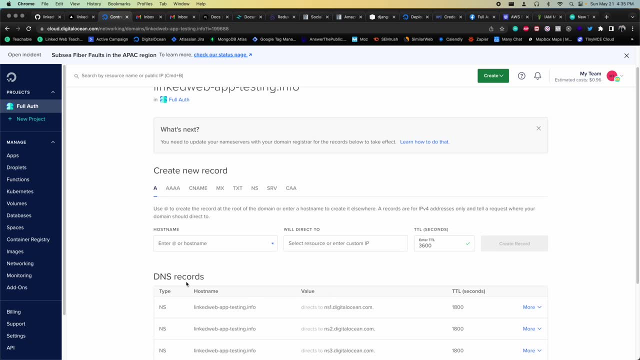 set up other than these. You can actually be using one of these NS records which just have DigitalOcean name servers. So that's where I'm at right now. So if I ended up doing this right now, I'd have to wait like 24 to 48 hours before things get propagated and I can actually use this domain here. 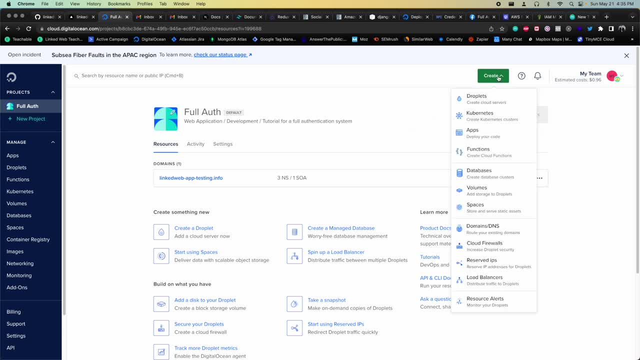 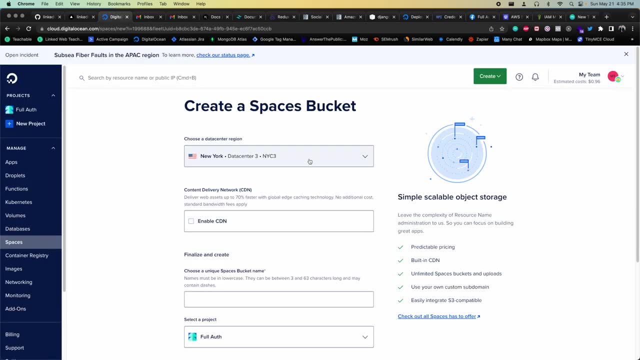 So the next thing I'm going to do is I'm going to click on this Create, and then I'm going to create first a DigitalOcean spaces, And then I'm going to set this as the damage. Just like I said, I'm going to create a new domain called DigitalOcean-services And I'm going to set this as the damage. 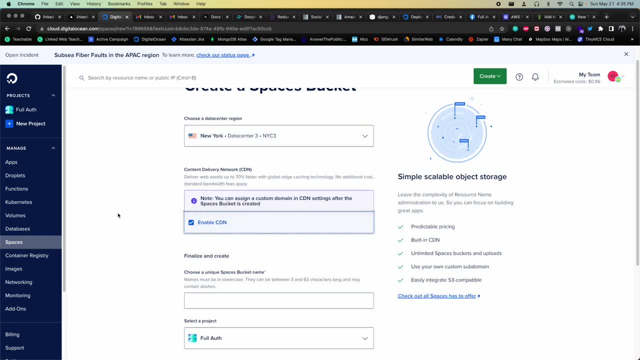 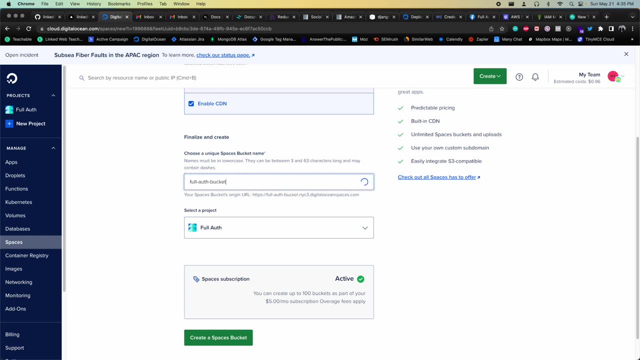 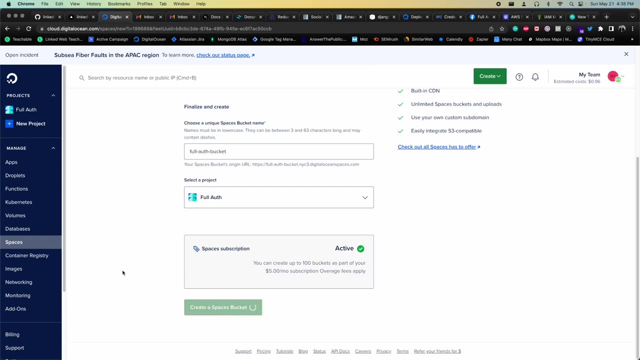 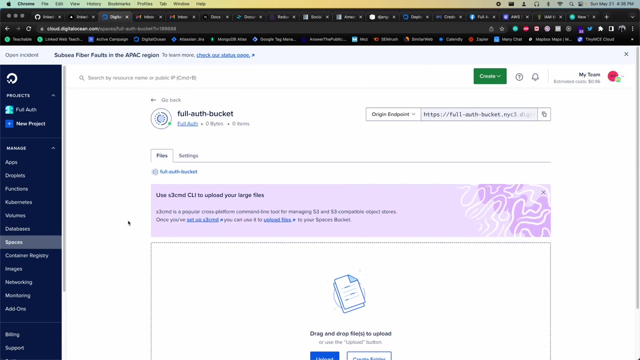 data center And then I'll enable a CDN And then I'm going to put in the bucket name. I'm going to call it full auth bucket And that's going to be in this project And I'll create this. So there we go. It's as easy as that to set this up, And then we just have to set up the CDN. 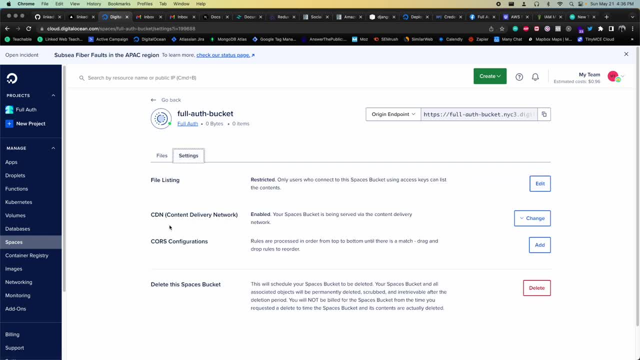 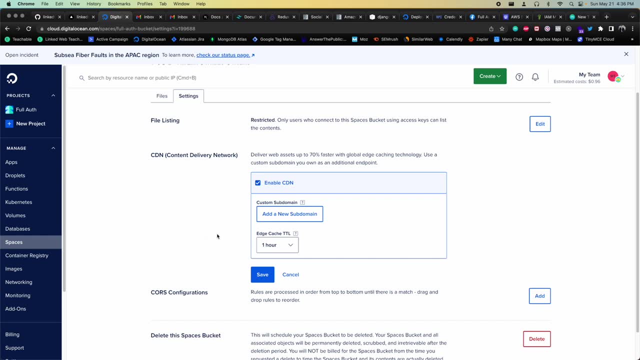 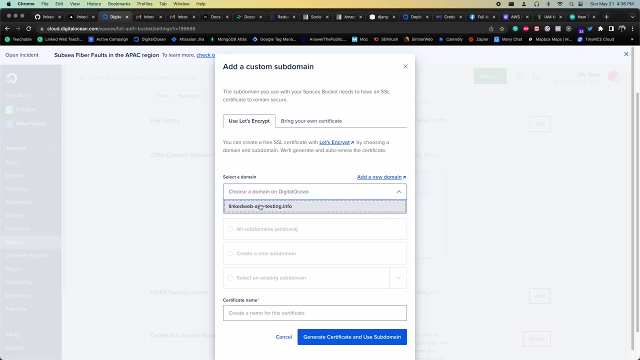 And we do have the CDN. but I guess what I mean is set up a custom domain for the CDN, because it's enabled right now, So I can click on edit CDN settings And then I can add a new subdomain. So I'm going to click on that, I'm going to select this here. 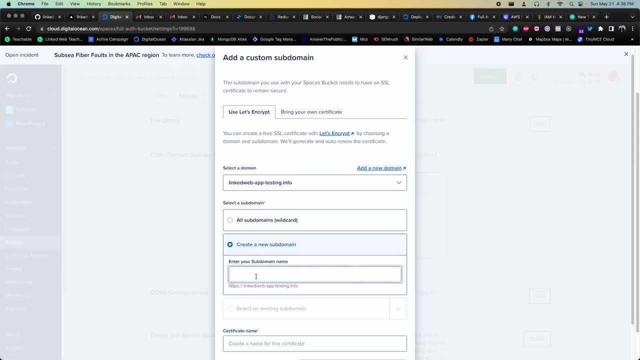 And then I'm going to create a new subdomain which is going to be spacesmydomain, So it's going to be spaceslinkedwebapptestinginfo, So that's going to be my CDN subdomain. And then I'm going to set up a certificate name. 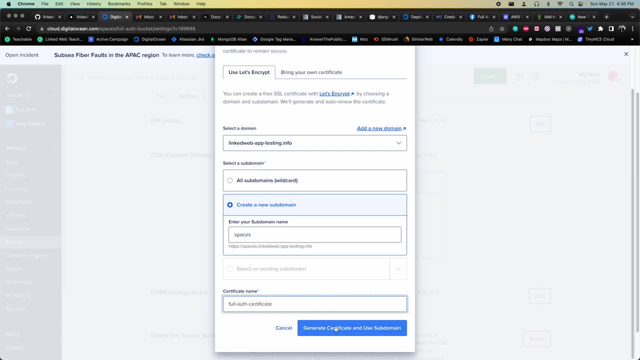 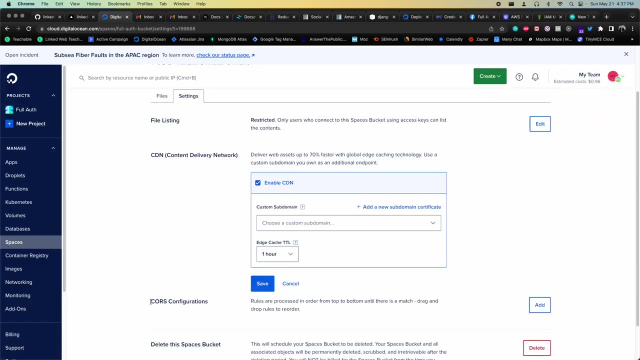 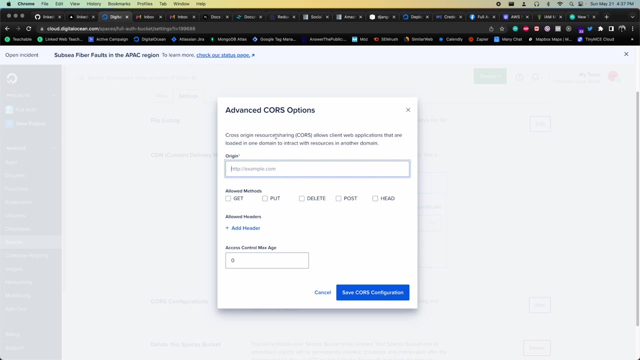 which I'm going to call full auth certificates, And then I'll generate that. So there we go, And then next we can also set up cores. So if we go here, click add, we can add an origin that we want, cross origin, resource sharing. So, in particular, 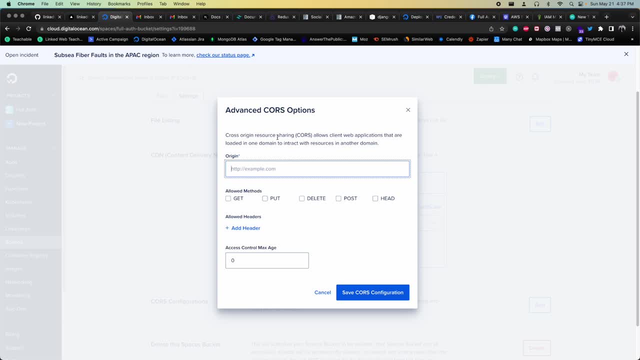 it's going to be our API subdomain Which is going to meet the cross origin resource sharing, because that's where we have the admin panel which uses the static files. So I can do HTTPS- APIlinkedwebapptestinginfo. 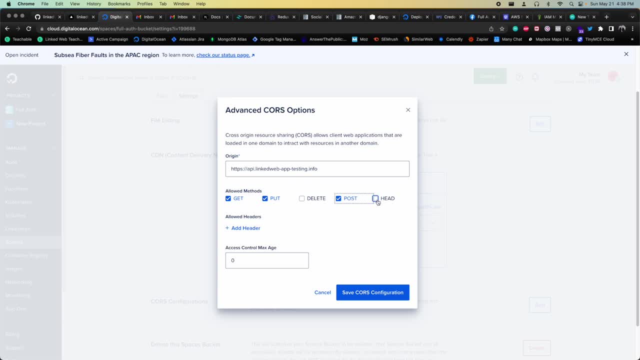 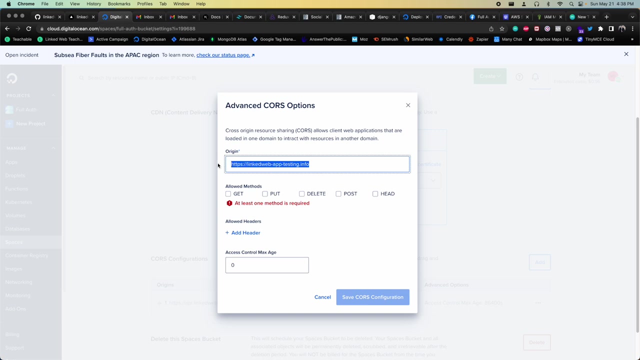 And then we can just add all of these methods And then here I'll put something like 86400 and save course configuration, And then I can also add some additional course configuration, which will be just linked. web app testinginfo. This is where the front end app is going to be. 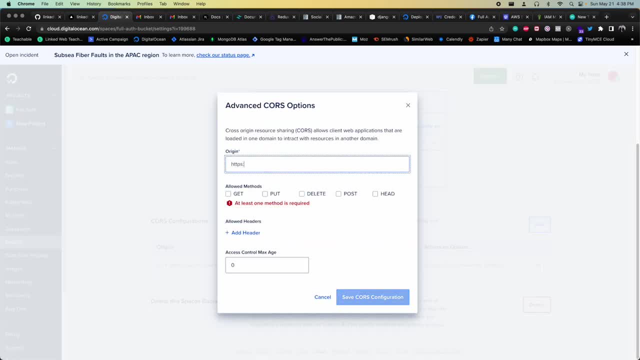 Oops, kind of clicked out of that. Let's do that again, And then for that, I'm also just going to put everything And do 86400.. Okay, Now, in particular, our front-end app isn't going to be using any static files. from what? 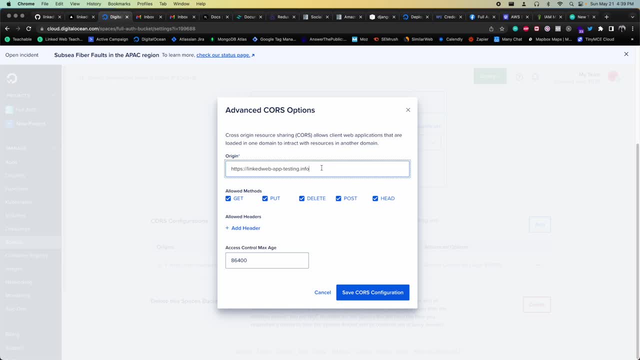 we have inside of DigitalOcean Spaces, although in some apps- most likely you will have that happening. If you have, let's say, media files that are in your DigitalOcean Spaces, then you're going to want the course configuration set up in that case. 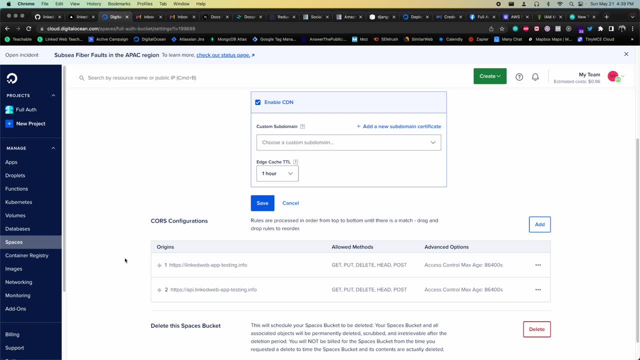 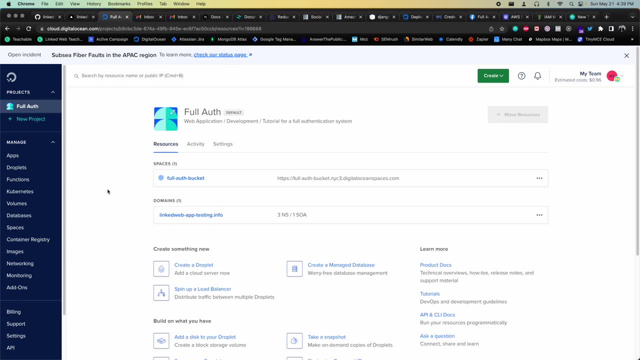 So I might as well put it there, just because it's something you'll commonly do. So with that, the next thing I'm going to do is go here And then I'm going to create and then click on apps. This is going to be the app platform. 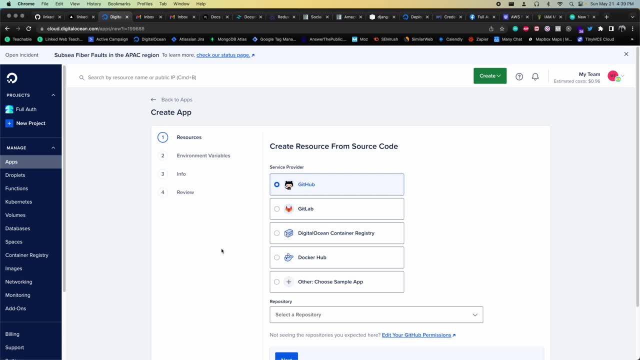 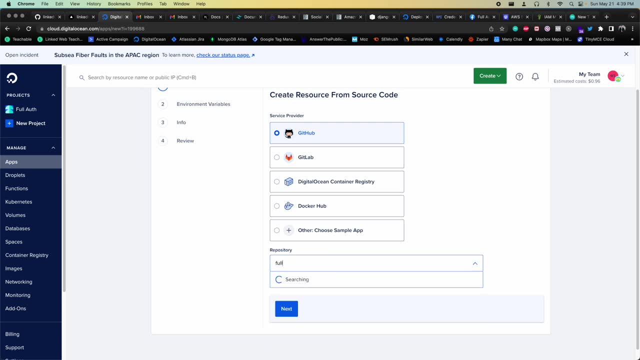 And then here we have GitHub. You're going to want to connect your GitHub to your DigitalOcean And then, once you do that, this repository. you're going to see all of your repositories here And then you can just search for the one you want. 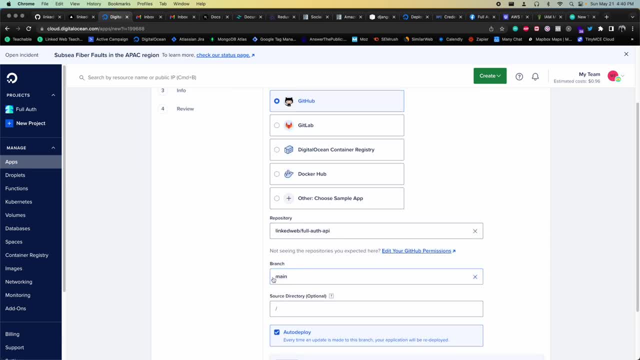 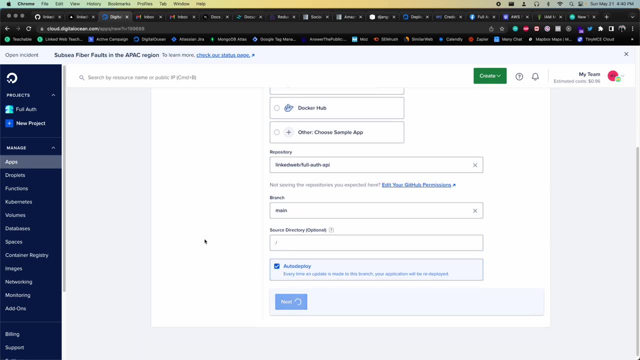 So I want full auth, API branch main, and then we're going to have this and auto-deposit, And then I'm going to click on deploy, I'm going to click next and then I'm going to add a resource which is going to be a database. 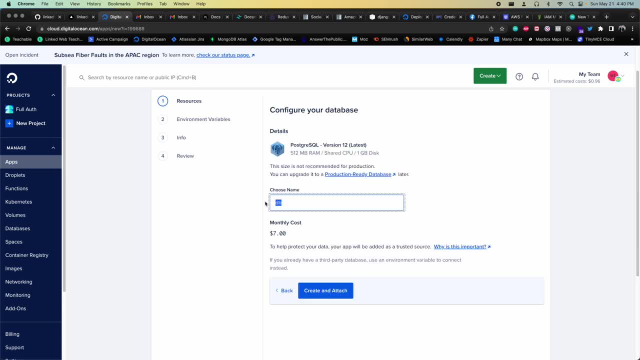 And I'm going to click add. I'm going to choose the name of DB, create and attach, click on next. And then we're going to want to set up our environment variables. So I'm going to just set up global environment variables. 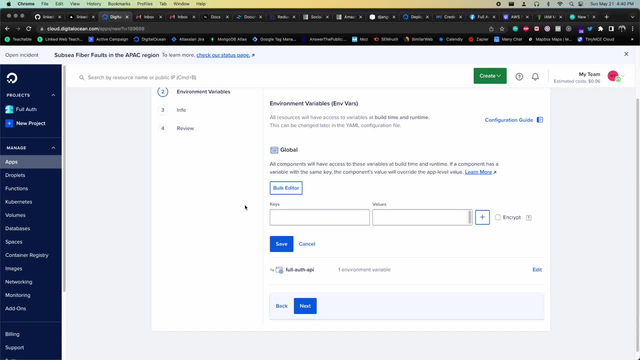 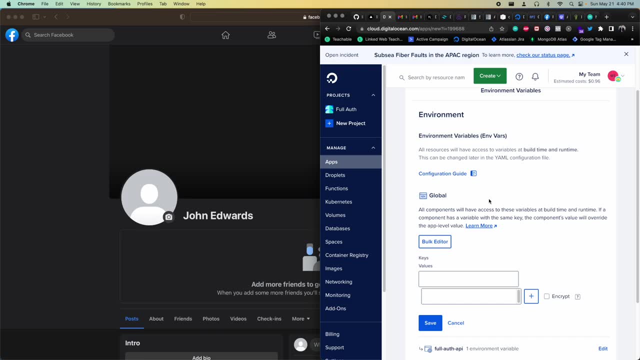 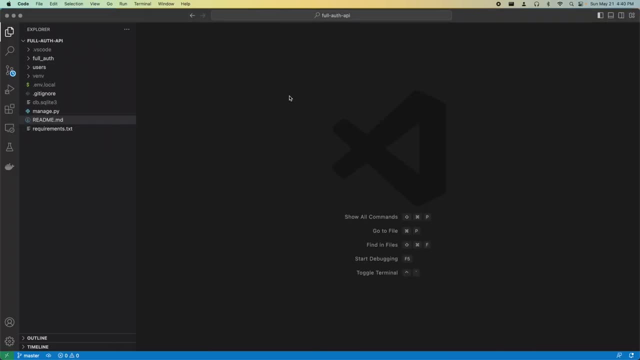 And this part is going to take a little while because we have a lot of environment variables. So what I'm going to do, I'm just going to shift this over like this: I'm going to go here, I'm going to grab this, put it in this desktop, go back and then open this up. 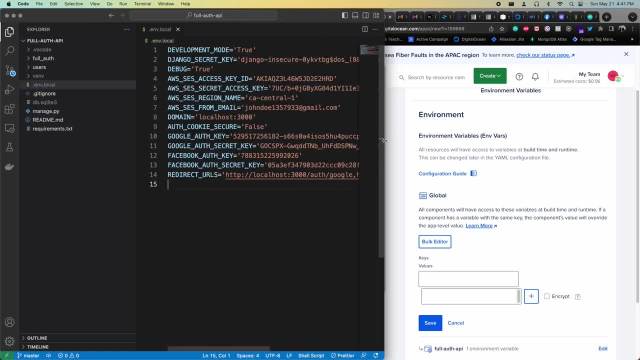 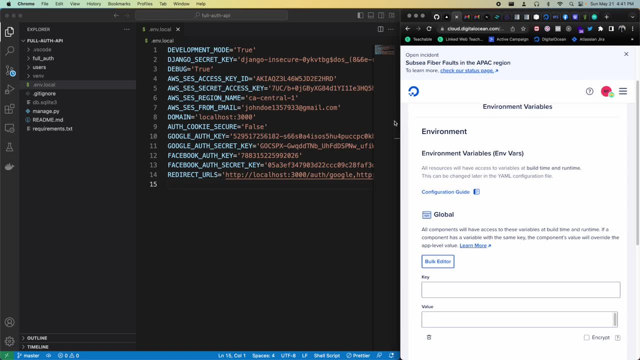 So we're going to be doing a lot of copy and pasting, So I just want to make this a little bit easier. So I'll shift this like this, something like that. So first thing I'm going to do is I'm going to go to my desktop. 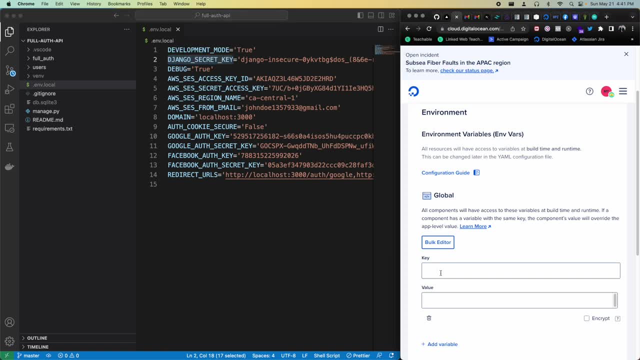 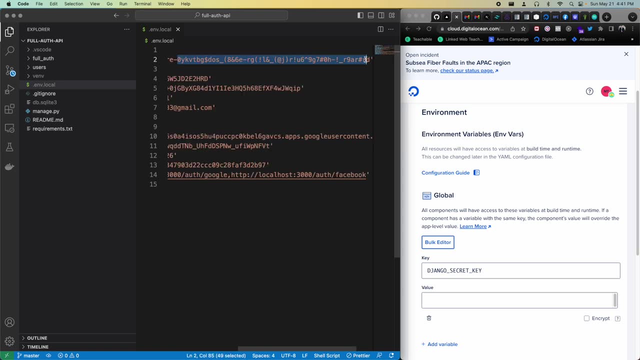 So first thing I'm going to do is I'm going to go to my desktop- So for this thing I'm going to want my Django secret key- And then, for the value, I'm just going to grab whatever's here And I'm going to add a little bit to it. 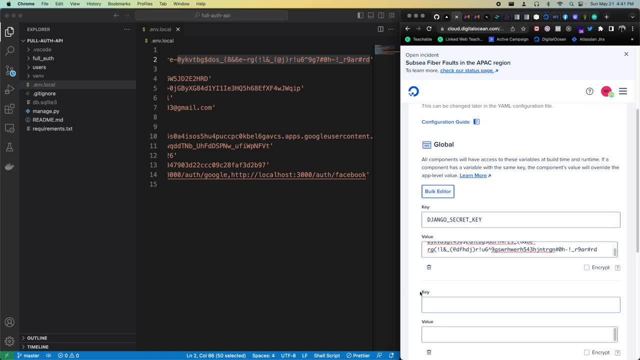 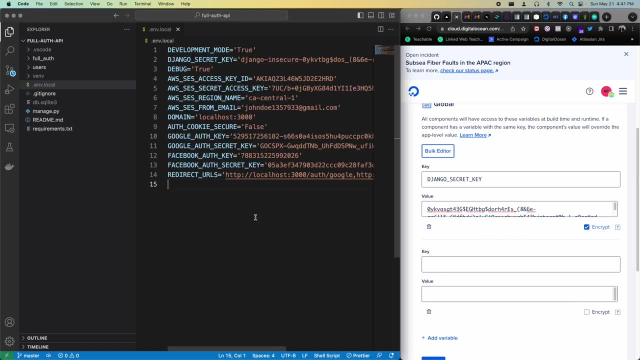 All right, I'm going to add another environment variable And then this one. I'm also going to click on this increase. So this one's called script And then debug by default is going to be false, so I'm going to have to add that. 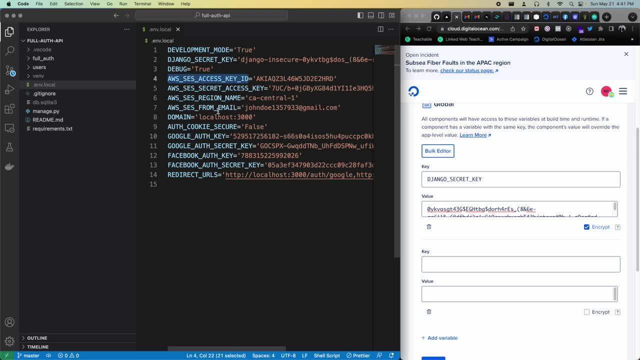 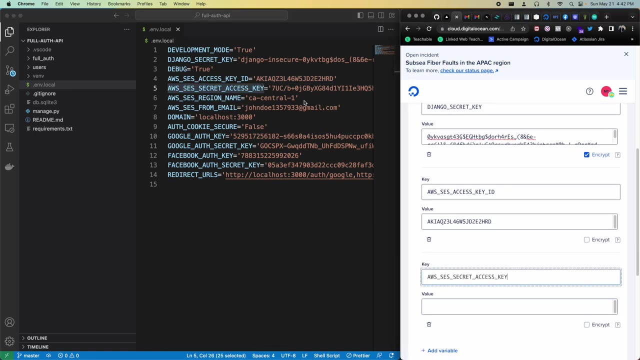 Also, development mode will be false by default, so I'm going to have to add that. But I will need this And then I'm going to need the SCS secret key. So this part's a little bit tedious, but once it's done, 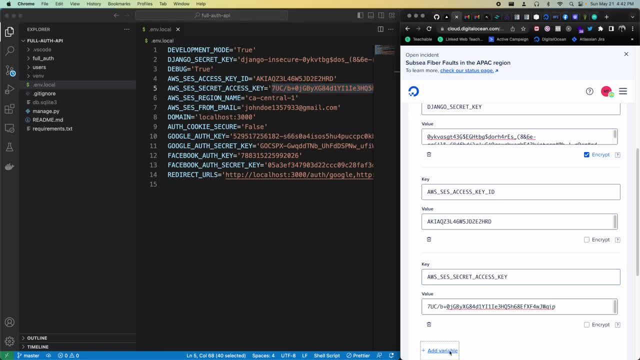 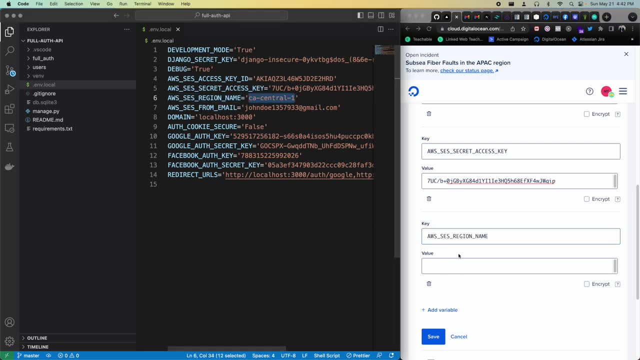 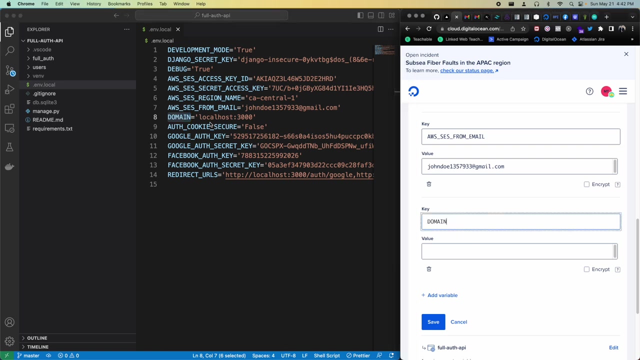 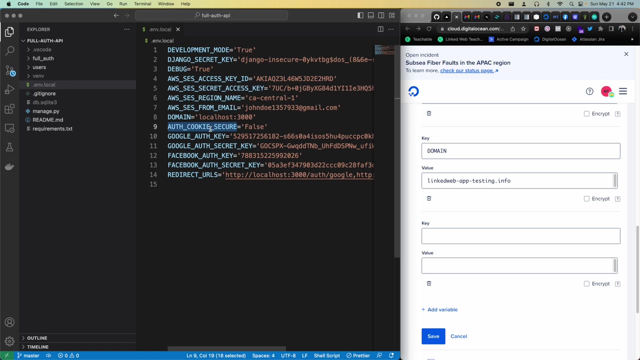 then we're good. and then the region name, and then for domain it's going to differ. this is going to be linked web app testing dot info in my case. and then auth cookie secure by default is true, so i don't have to touch this setting, but i will need the google auth key. 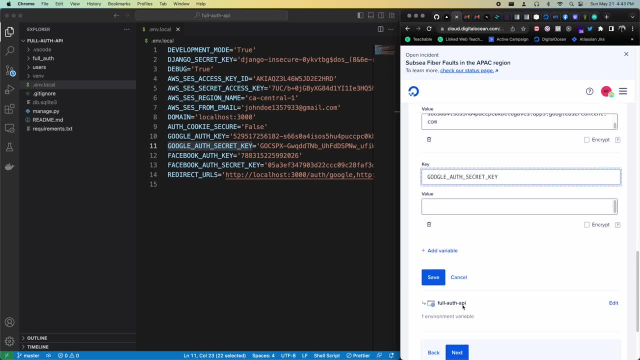 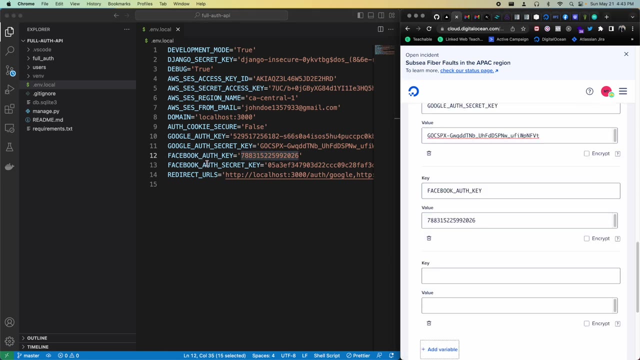 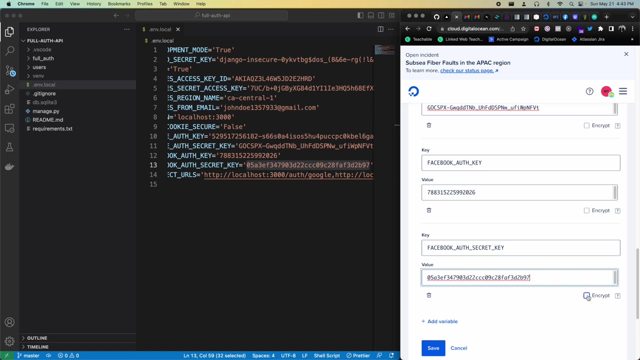 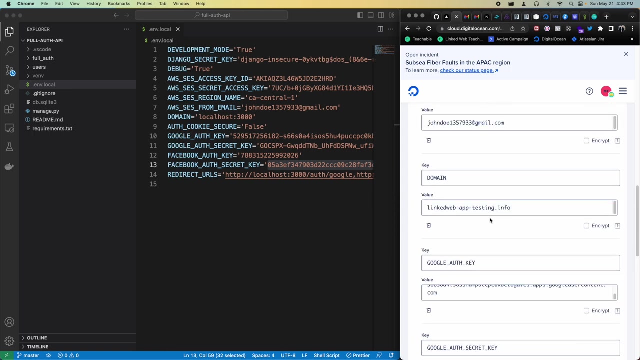 then i'll need the google auth secret key, and then the facebook auth key and finally facebook got secret key and then i'm going to encrypt this secret key. as well as this secret key, and then i think also had another secret key somewhere that was for sc. 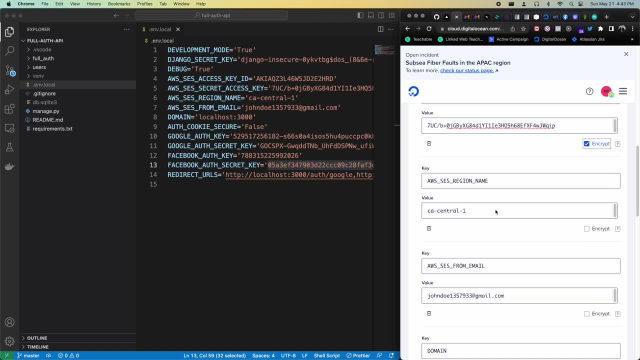 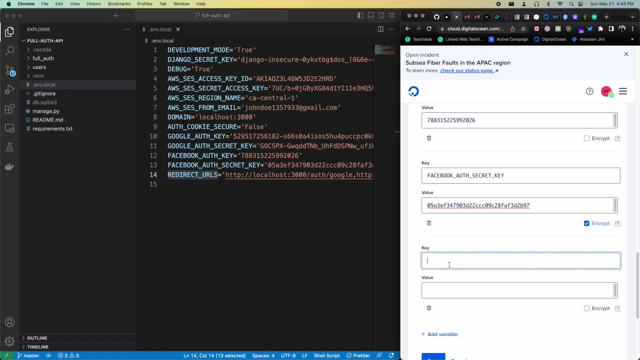 so i'm also going to encrypt this one. i'm going to go back down. next i'm going to have my redirect urls. in this case, i'm going to have https colon slash. slash. linked web app testing dot. info slash, auth, slash, google comma and then again https colon slash. 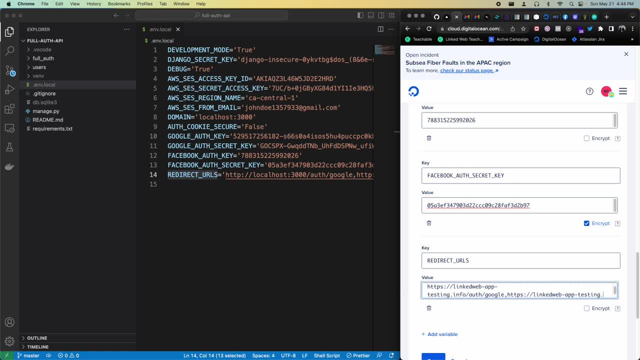 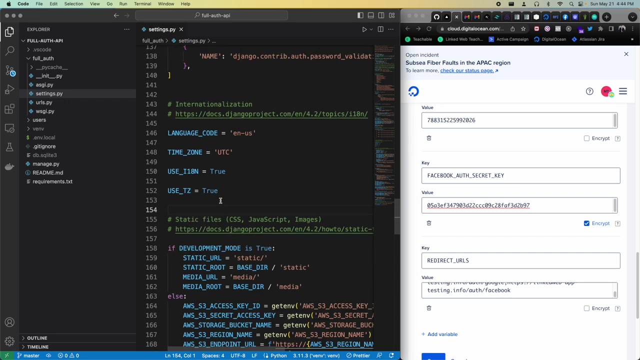 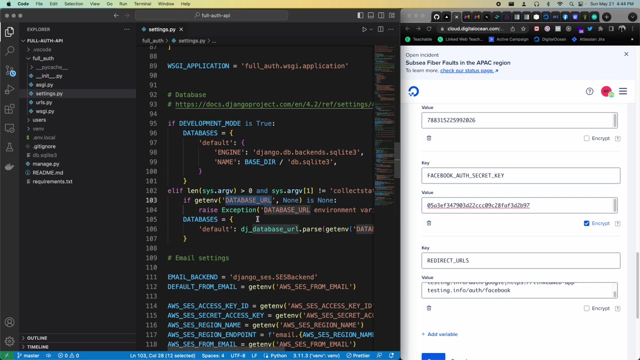 slash linked web app testing dot info. slash auth, slash facebook. so these are going to be comma separated and then we're going to have a bunch of additional environment variables we also have to set up. so we've got where's the database settings? there we are. so we're going to have database url that we have to set up. 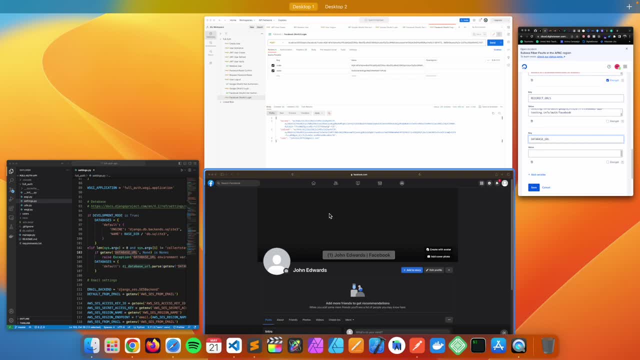 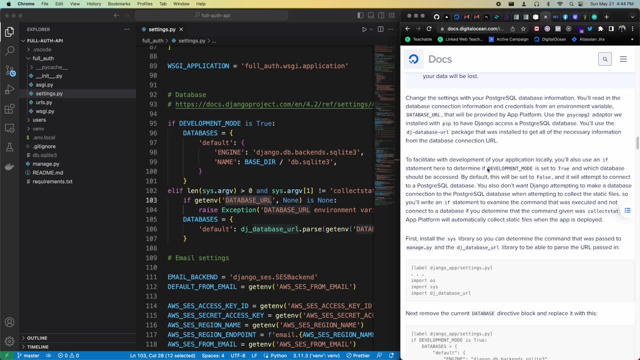 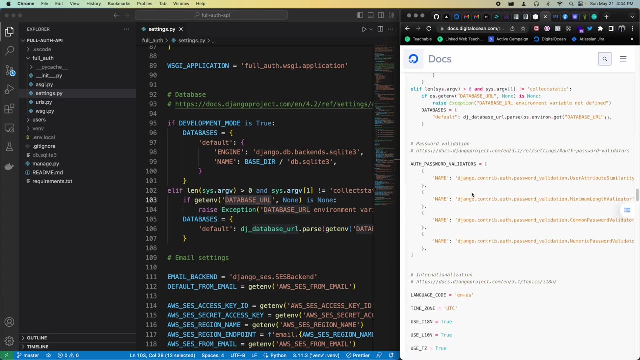 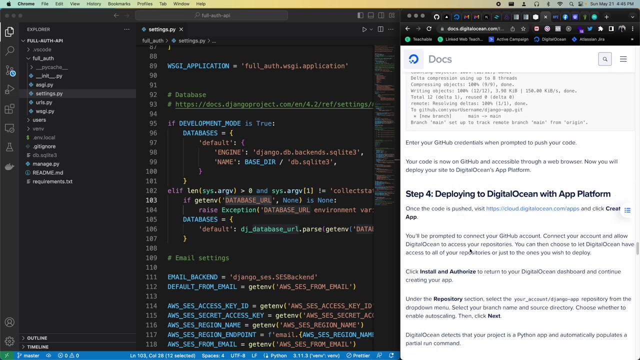 and then we are going to need a feature slash container that has early version or station authentication in it. so i'm going to use openuvdah and connect it to a provider, and then i'm using the app Savior accelerator, which is just done in the plugin, and we are going to enter when you utilize it into your resonated account. so let's, instead of using Torchroid, do thatcz, and we're going to need. the reason to use Torchroid is that we want to create a simple structure, for this would be really easy just to do this kind of a subdraft in aém. and then let me bear with me for a moment. 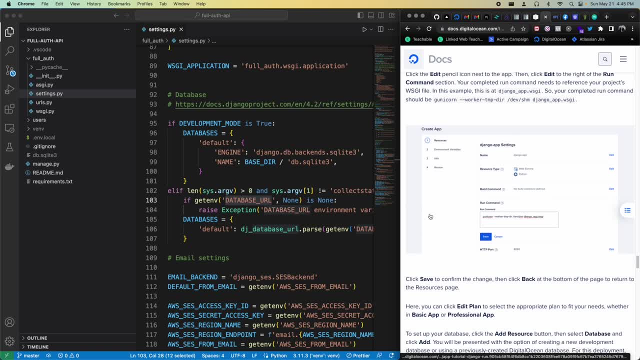 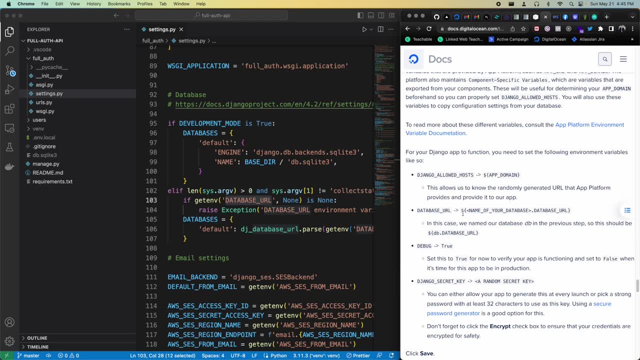 but if it is just simple, you just need to Vorschutz to create or solder necessary him protocols as good récup. we'll have to set this up, but we'll do that a little later, and then here we have database URL and this is how you set the value. so we're gonna do dollar. 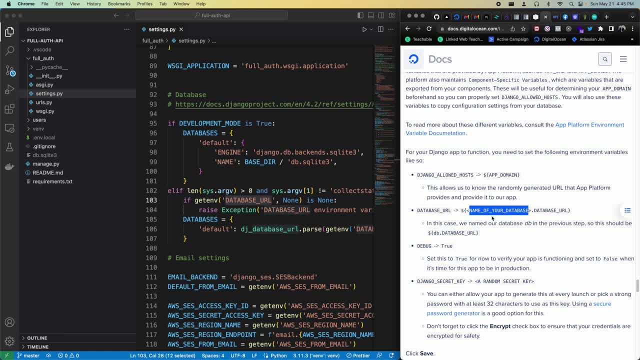 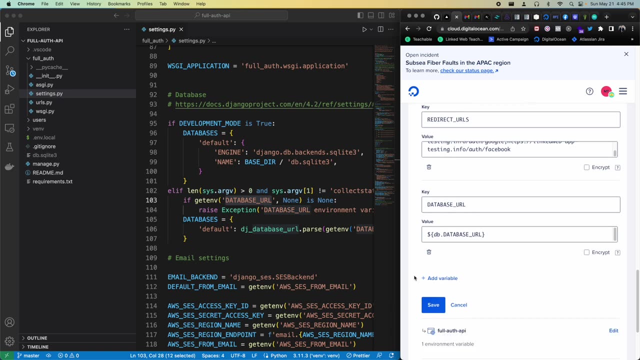 sign, curly brace, the name of our database, which is DB, then dot database URL, just like how they have here. I'm just gonna copy this. I'm gonna go back to my digital ocean settings here. I'm just gonna paste that in here, so that's gonna be the value, and create another environment variable. and then here I'm. 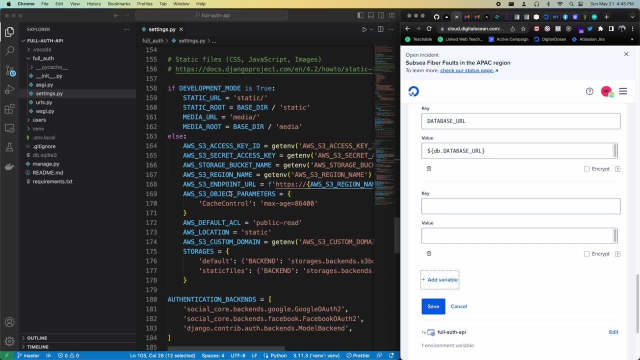 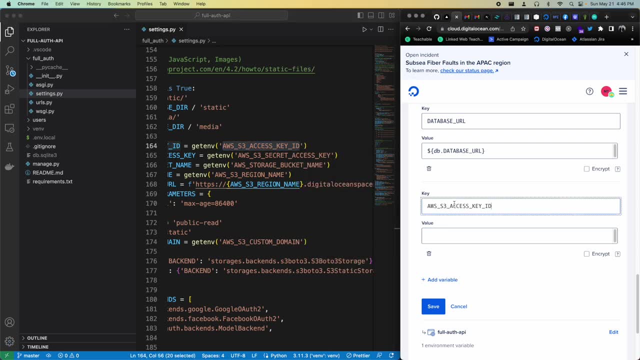 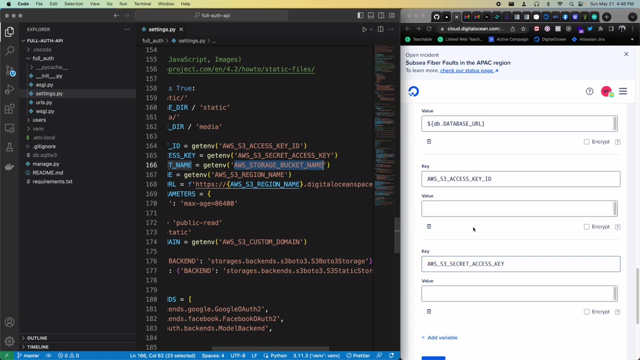 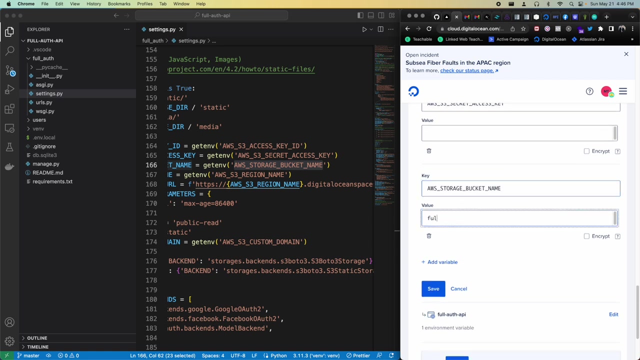 gonna have a couple, so that was in my static settings. so I have this AWS s3 access key. also have this secret key. I'm just gonna add the keys first and then I'll do the values and have the storage buckets. name you this. I can fill out right now. I called mine full auth buckets and have the. 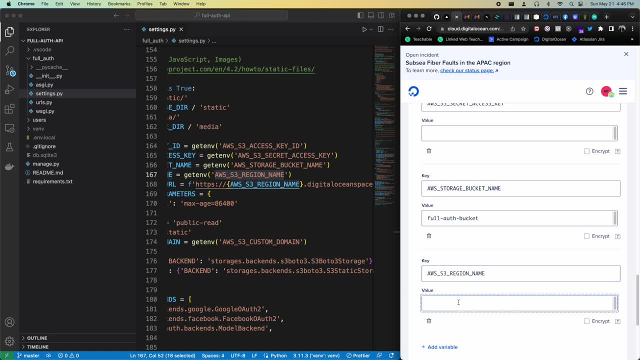 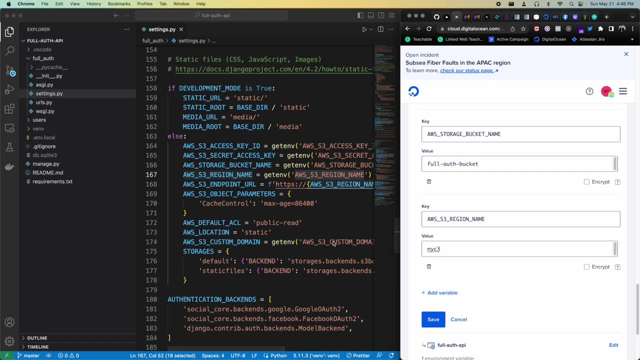 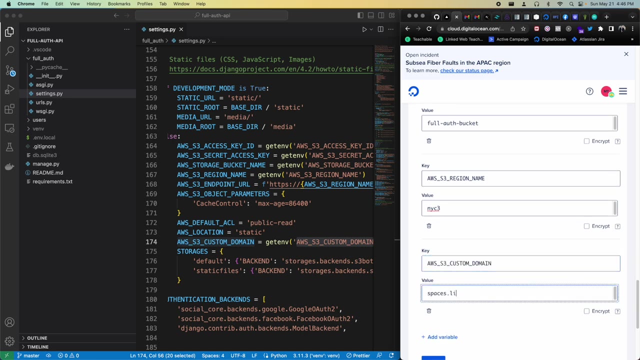 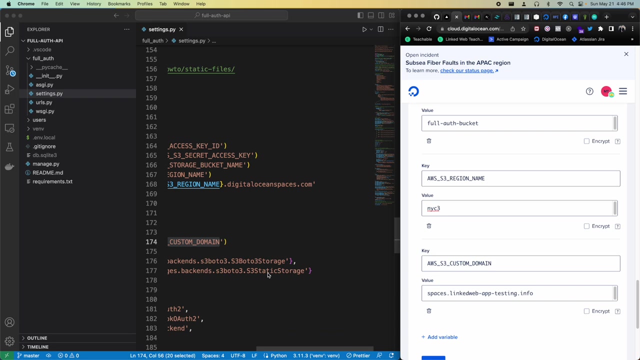 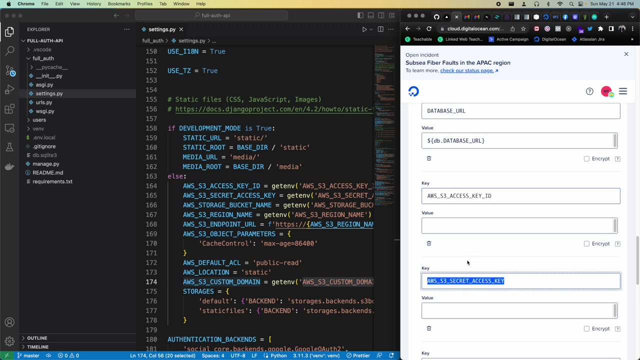 region name. this in my case is NYC 3, and let's see what else I need: custom domain, so that one's gonna be spaces dot linked web app testing dot info. that's what I set up and that should be it. so now I just have to grab the two values here. so how do we get those? so now what I'm gonna do: 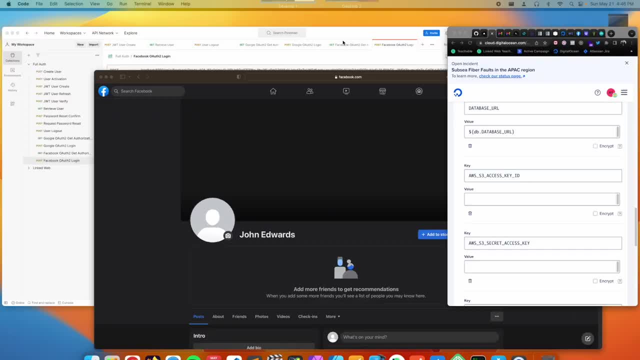 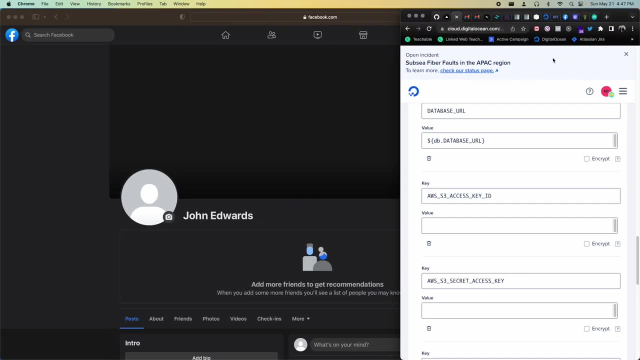 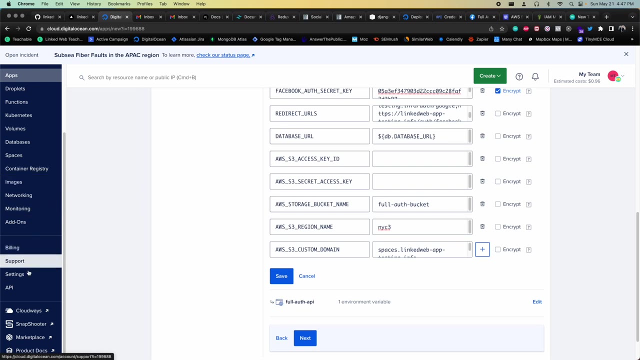 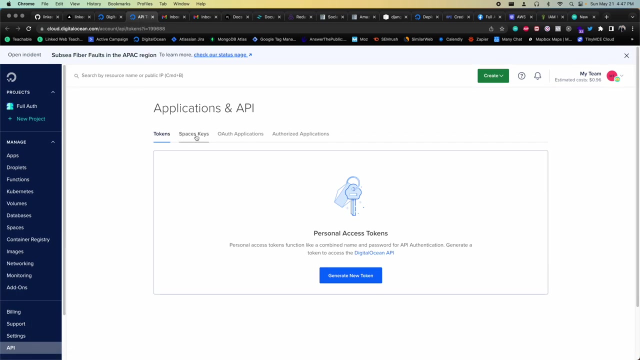 is. I'm just gonna bring this back to how it was and I'm gonna make this full screen again And then I'm going to scroll down. Then, under API, I'm going to open up a new tab to open this API, And then here we have spaces, keys. 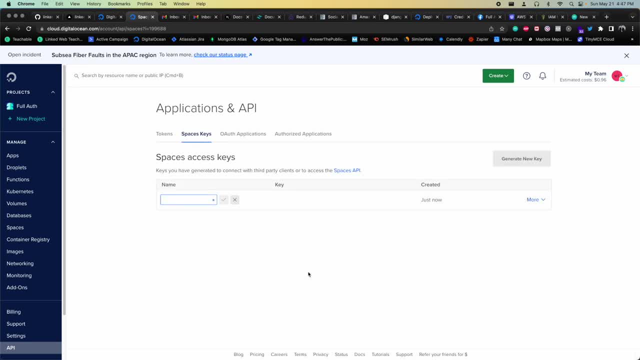 So I'm going to go here, I'm going to generate a new key, I'm going to call this full auth key. I'm going to create that And then I can copy this And that's going to be the value for the access key ID. 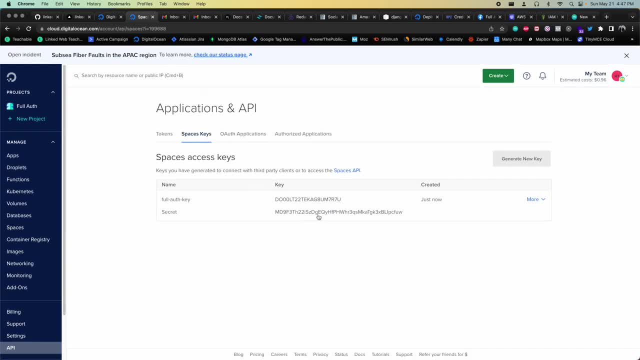 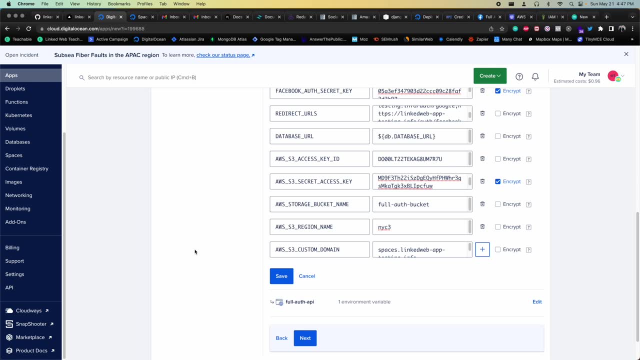 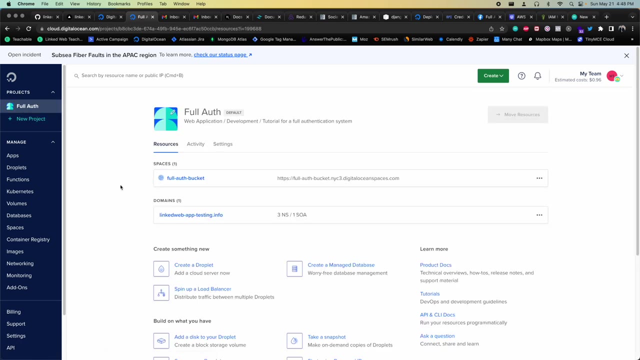 And then this will be the secret. So I'm going to paste that here And I'm also going to encrypt that. So now we should have all of our settings here, unless I missed something, which I very well might have. Oftentimes things do go wrong during deployment. 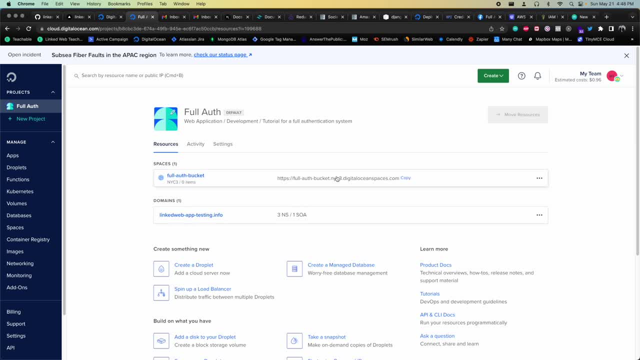 but who knows, maybe this time it won't. And then also this: right here you can see that I have a lot of things and you can see the region name and also the bucket name. So full auth bucket NYC3.. So you can get those values here. 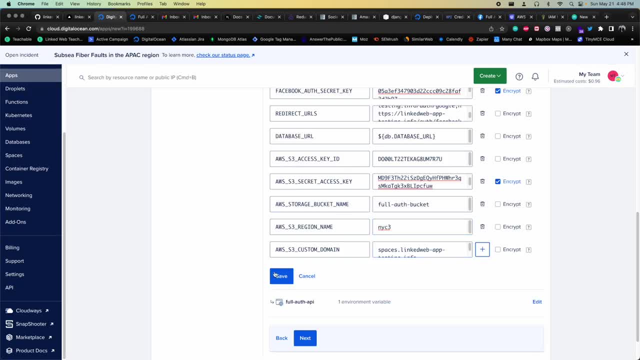 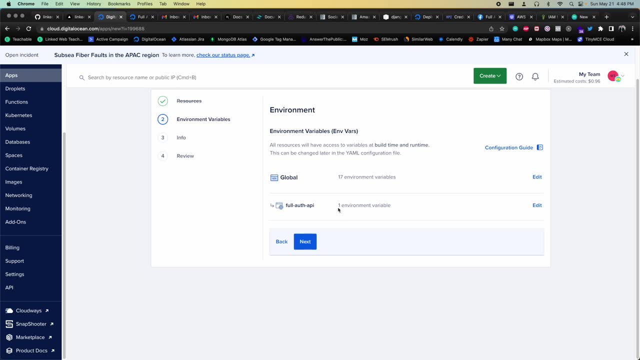 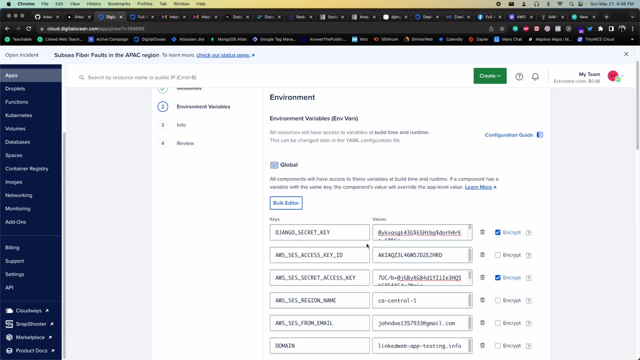 So everything should now be good to go. So I'm going to save this, I'm going to click next. And also, we have one environment variable here, And that is actually this database URL, So we don't actually have to set it up globally. 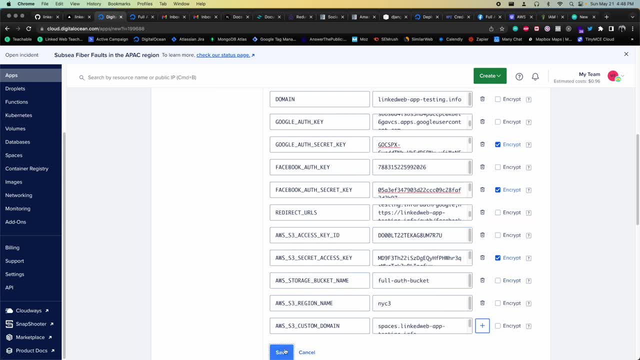 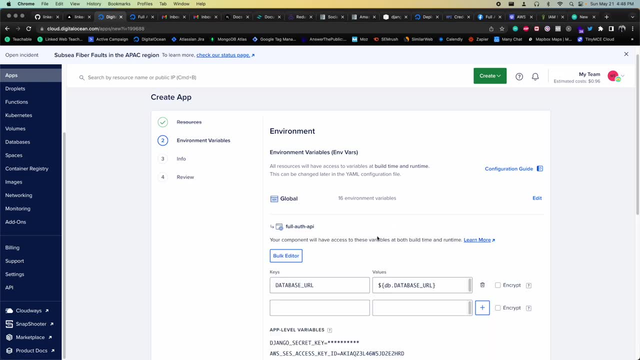 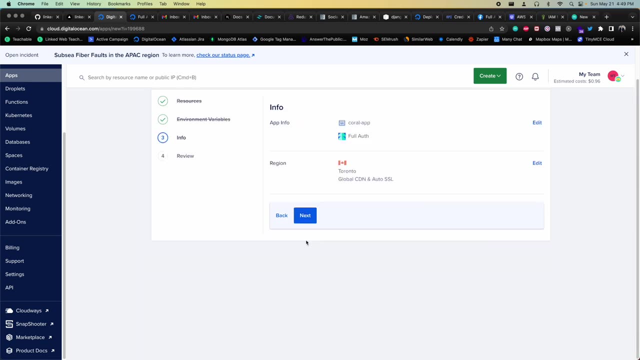 So I'll just remove that Click save. So now we have 16 environment variables And then here we have this one for the database. I'm going to click next And then let's see what else we can edit here. So we can't edit the runtime yet. 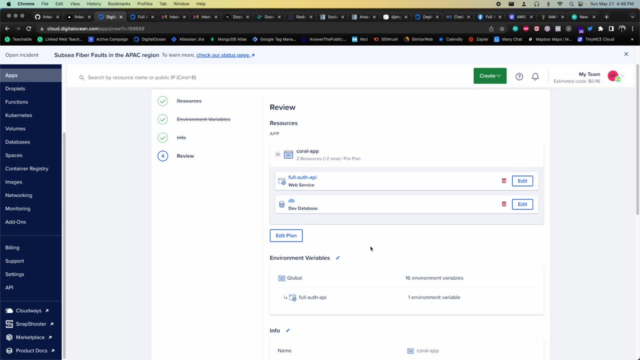 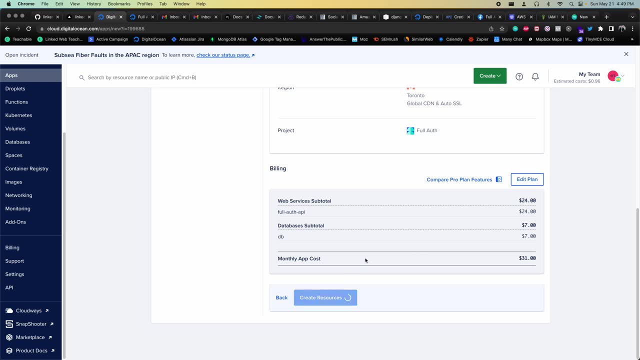 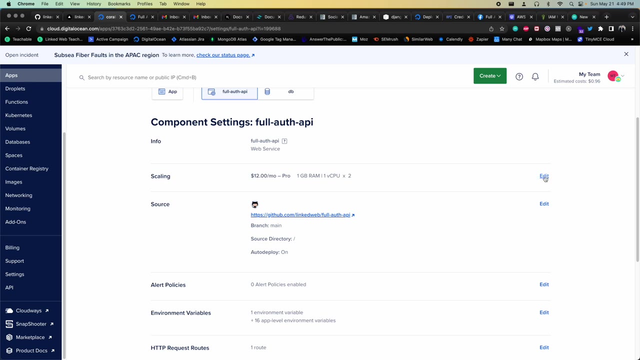 So we're going to have to do this, We're going to have to do that later. So this is what we've got for now. So I'm going to create these resources And actually I did forget to do one thing, And that was this plan. 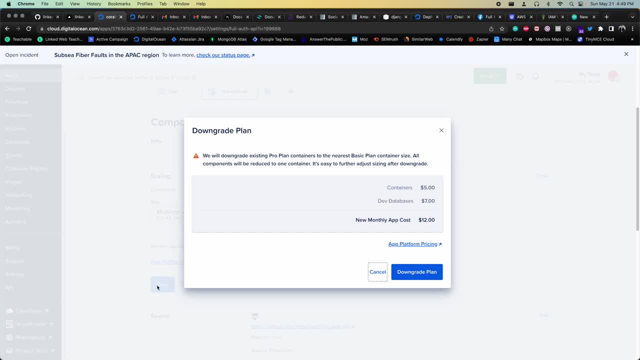 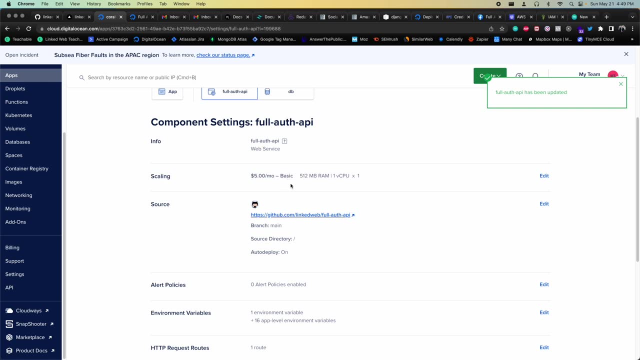 So actually what I want to do is use a basic plan. I'm going to save that and downgrade the plan, So I forgot to do that, but you can always do it later, So it's no big deal, And then we can go into commands. 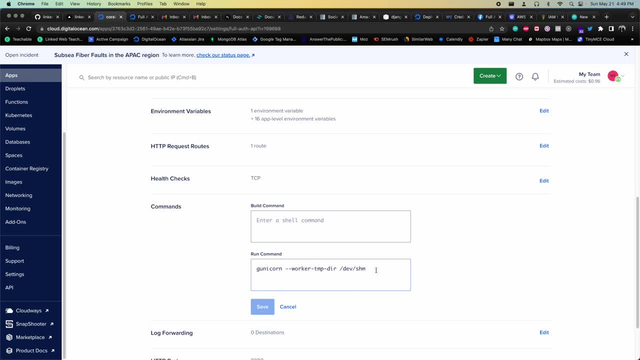 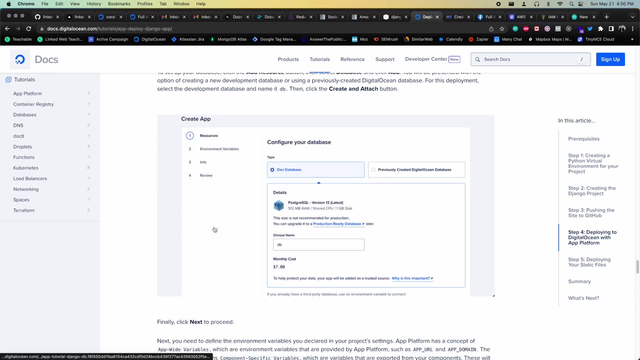 go into the run command And then you're going to put in your project name- in my case full underscore, auth, dot, W, S, G, I- And you have the same exact thing showing in here as well. I think it was just a little further up. 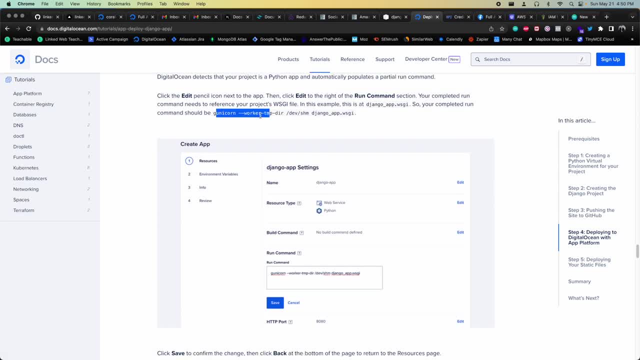 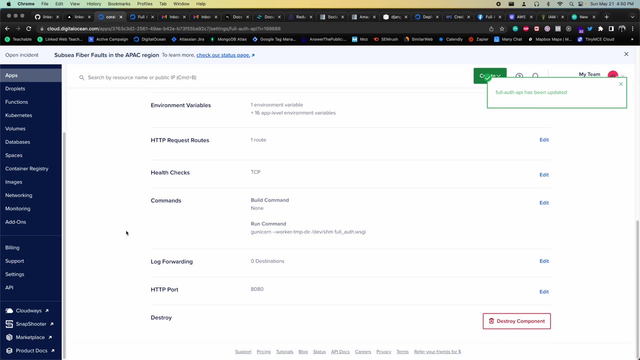 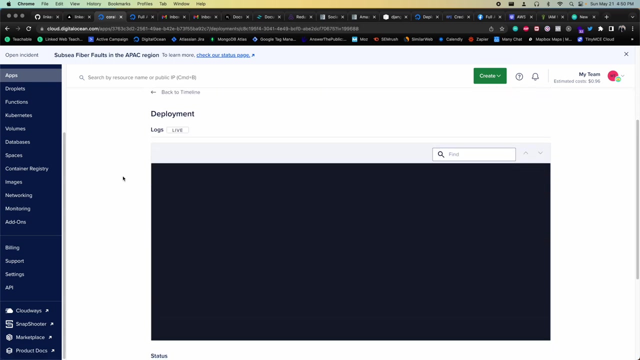 So there it is. So Gunicorn worker temp directory: dev SHM- The name of your project- dot W S G I. So that's the same thing we have here. So I'm going to save that And that should be everything. So from there I can go to the build logs and just wait for this to finish. 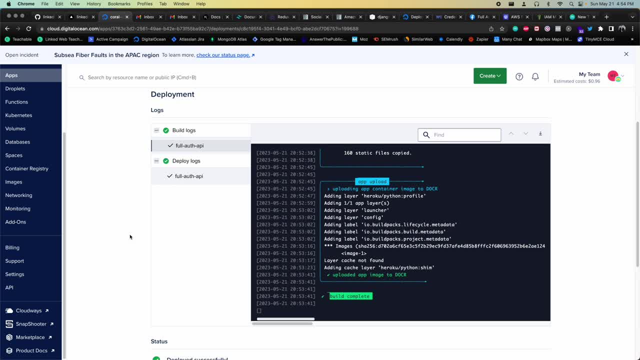 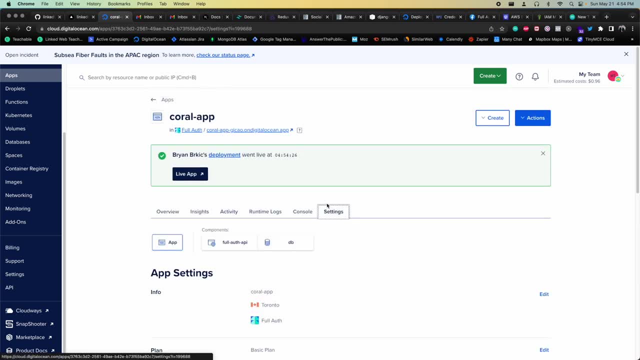 Okay, And there we go. We have our build and deployment successful. However, we're not quite done. Also, while this was going on, I did remember two environment variables that I did miss, So I'm also going to have to add those in. 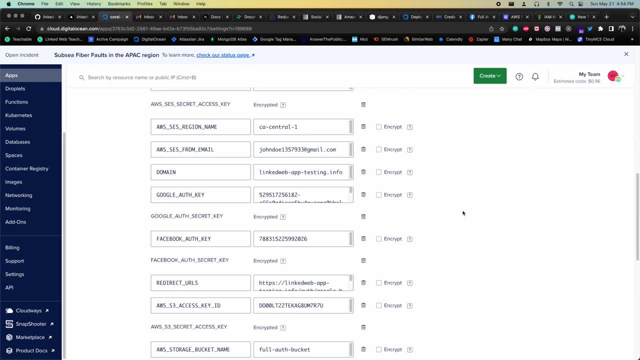 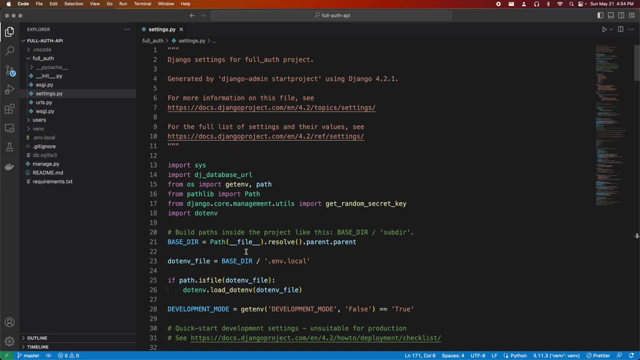 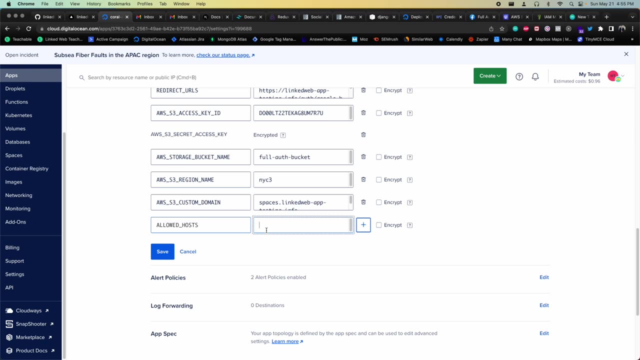 So it's pretty easy to do, thankfully. So I can just go into here and just add whatever other environment variables you need. So the ones that I missed in particular, if I scroll up, we do need our allowed hosts setting And then that one is going to be API dot linked web app testing dot. info. 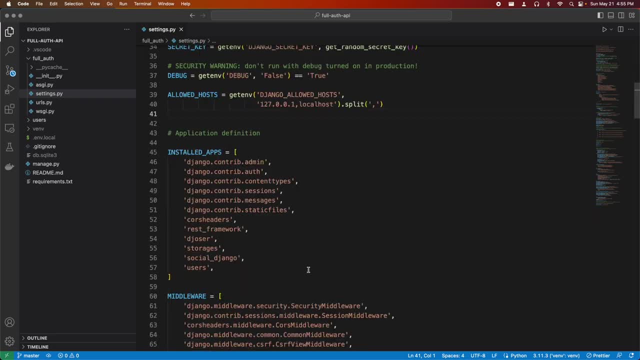 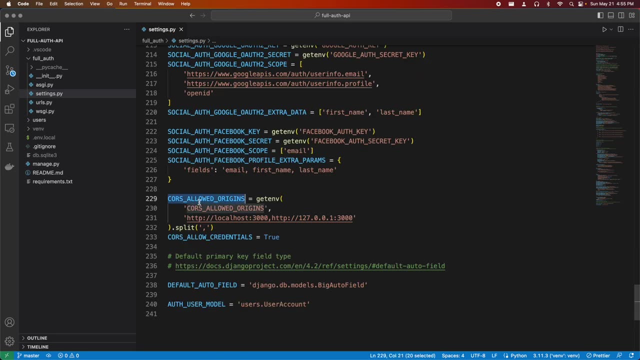 And then there's going to be One more that we need. So if we scroll down, So at the bottom we set up this course allowed origins, And here we're going to have whatever origins are allowed to make requests to this API. 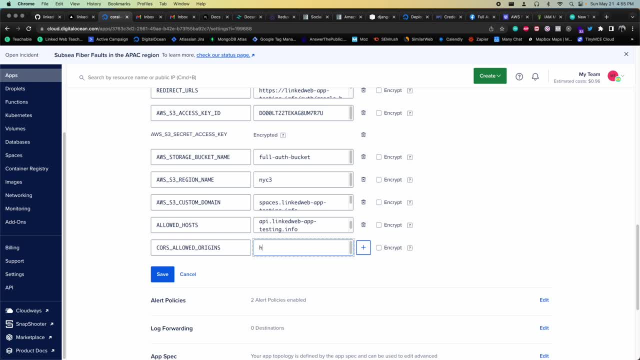 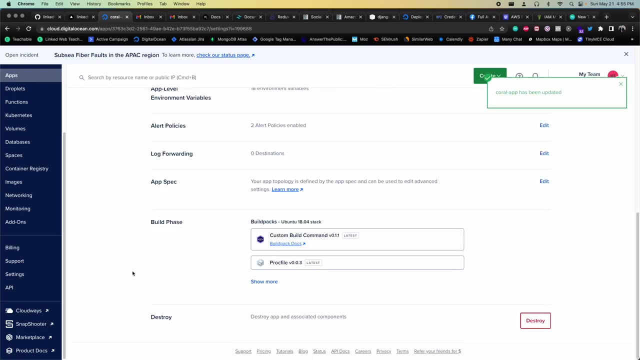 So I'm going to go back and paste this setting in and the origin we want is HTTPS, colon slash, slash, linked web app testing dot info. So that's going to be where our front end eventually gets deployed, So I can save that And then that is going to trigger another deployment. 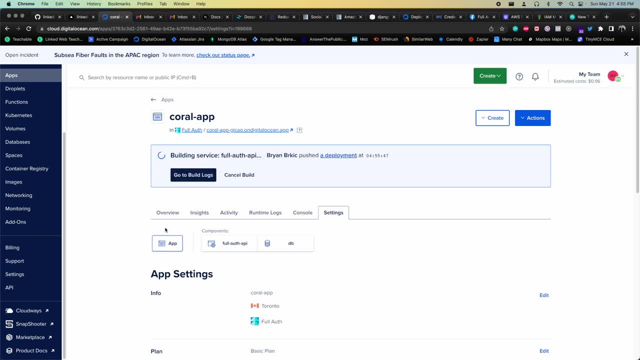 So I'm just going to wait for that to finish, And then the last thing we're gonna have to do is also set up the custom domain, because right now we added that API linked web app testing dot info, Although we didn't configure that. 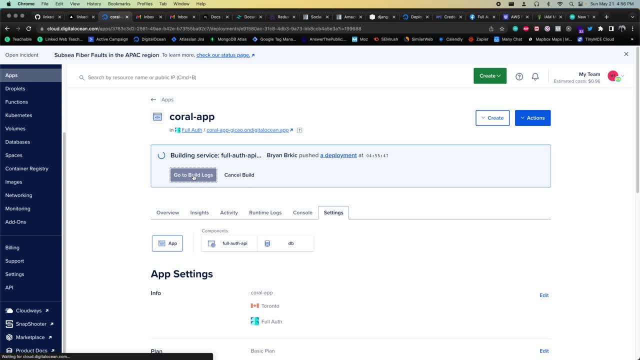 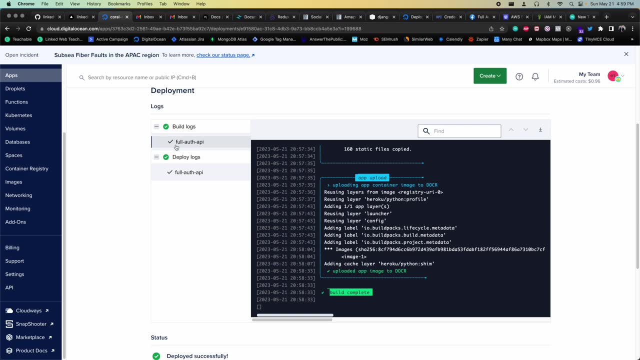 So right now things wouldn't really work, So we have to set that up as well. But first I'm just going to let this do its thing and then I'll do that after. And there we go. We ended up successfully building and deploying. 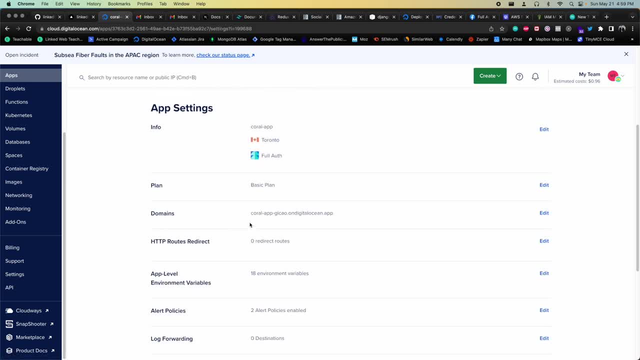 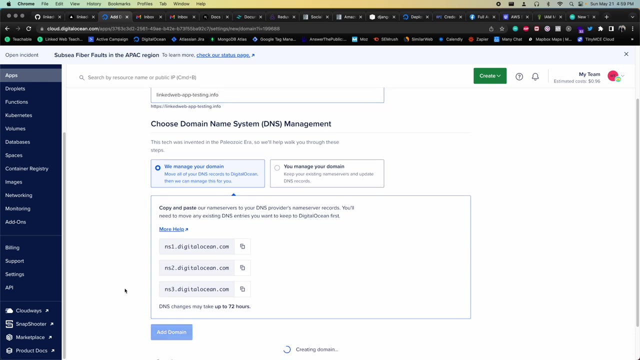 So now what I can do is I can go to my settings, I can go to domains and I can add a domain- This is going to be linked web app testing dot info- And then I'm going to say: we manage your domain, I'm going to add it and that's pretty much it. 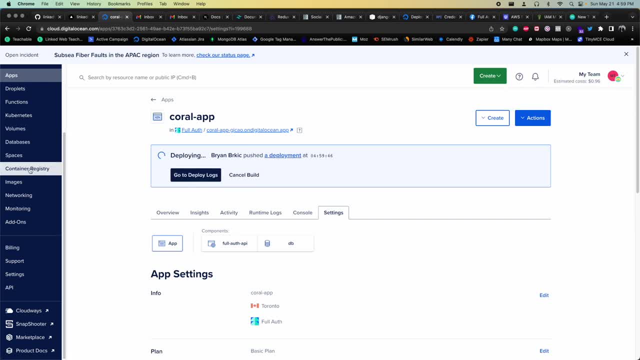 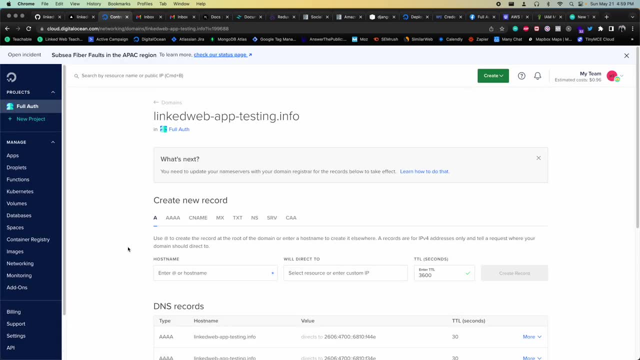 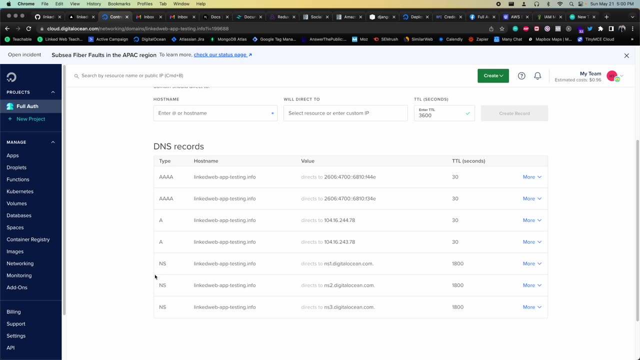 So now it's going to go through this once again, And then what I'm going to do is I'm going to quickly go into this domains just to show you something. So, right now, what we had previously was just these NS records, but we see that additional things did end up getting added here. 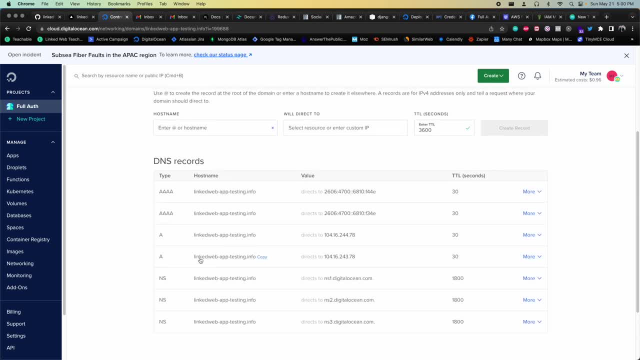 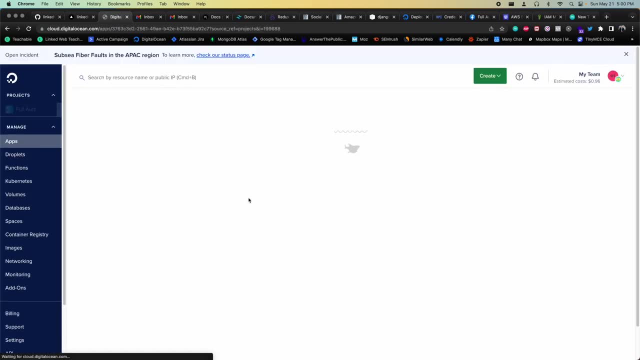 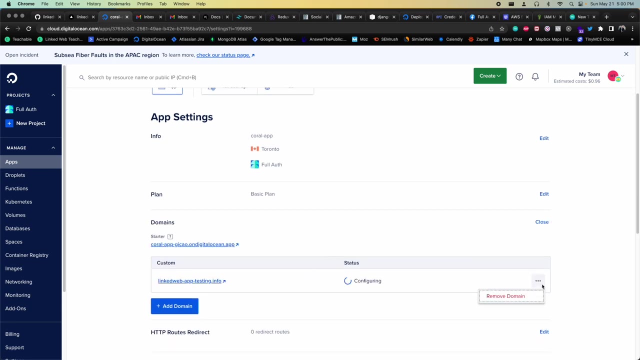 And also I did make a slight blunder. I just realized I meant to do the sub domain here, So I actually will have to go back and edit. Yeah, So let's actually do that. I'm going to go into domains and then this one I'm going to actually end up removing later. 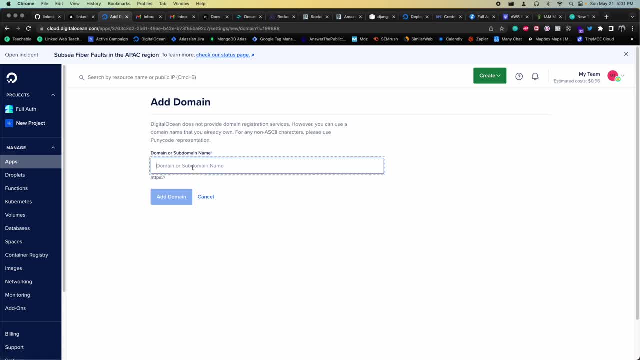 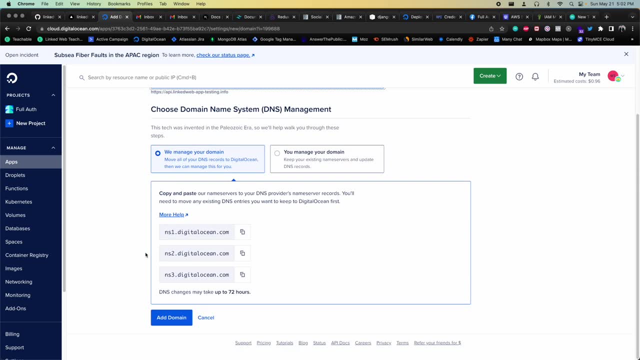 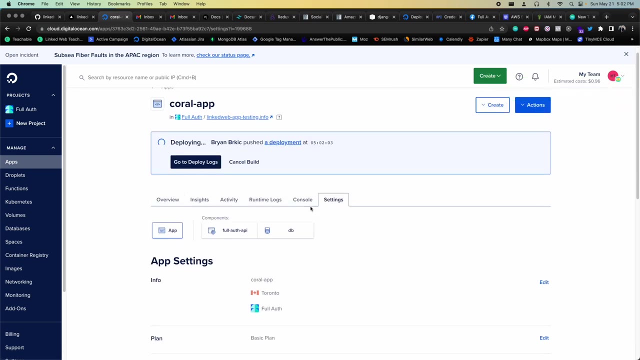 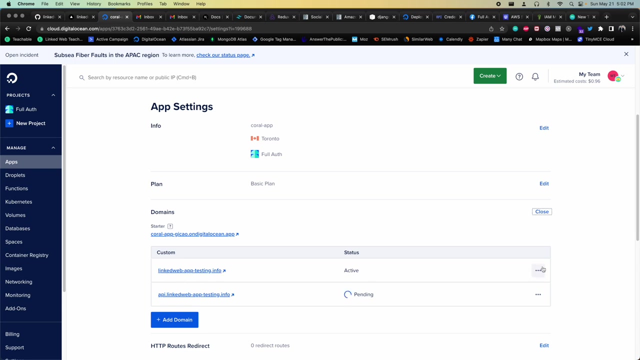 So this configuration might take quite a while. So I'm just going to add API dot linked web app testing dot info. We manage your domain and I'm going to add that That's going to run Another deployment, but then in my settings so it looks like this one finished. 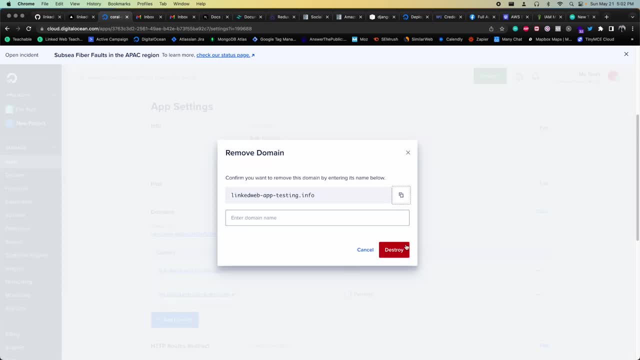 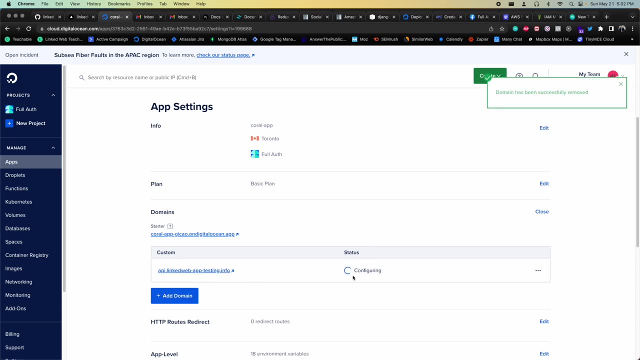 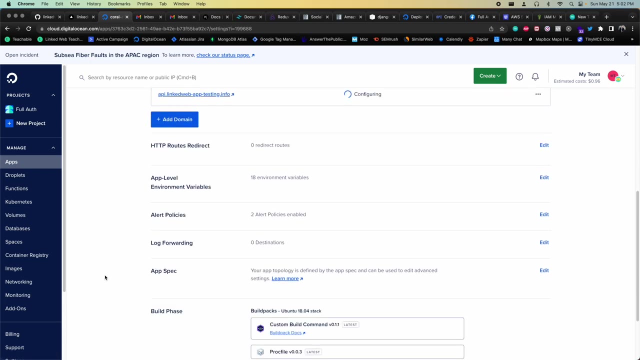 So I'm going to now remove it, since I don't want that one. That was a slight error on my end, So now we're going to configure this one instead, because we do want our API on this sub domain. So with that we should. 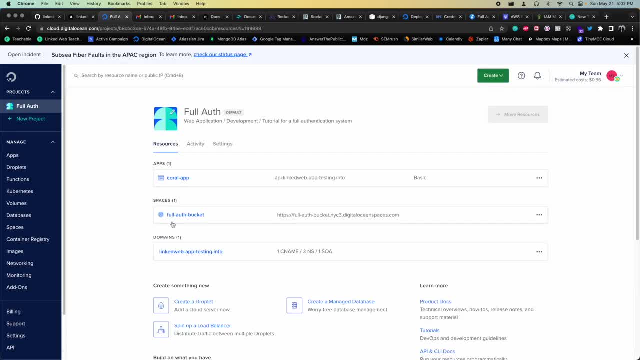 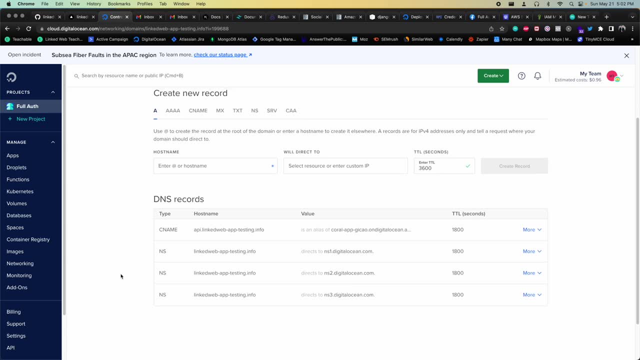 Now be able to go here, go to domains, and there we go. We have a C name. Now, one thing we don't have is our digital ocean spaces set up here. That's one thing I expected to see, but for some reason it's not here. 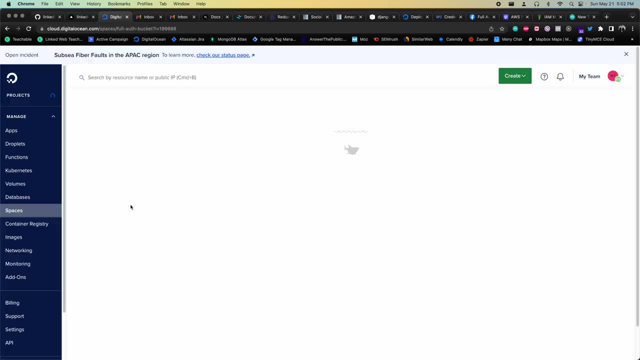 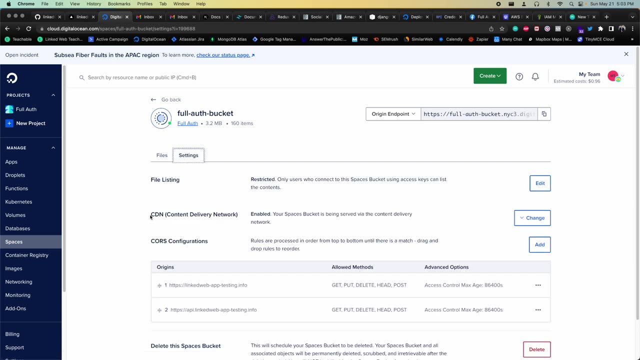 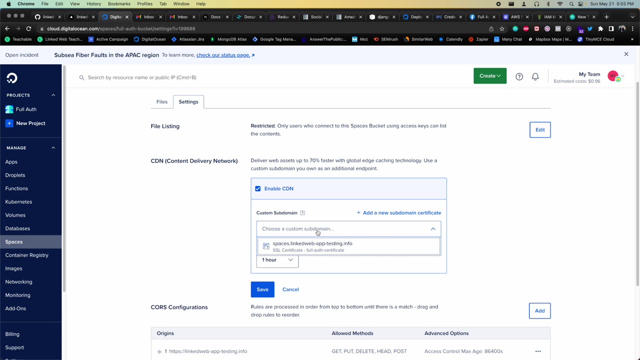 So maybe there was something I forgot to configure, So let's go back. Also, we see these static files are here, so that's good. So we set up the C, D, N And it seems that the sub domain, Oh, okay. 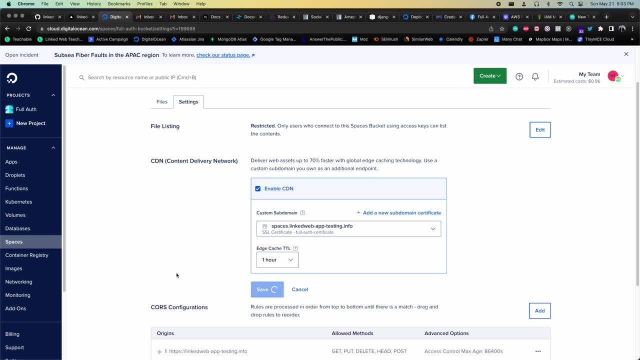 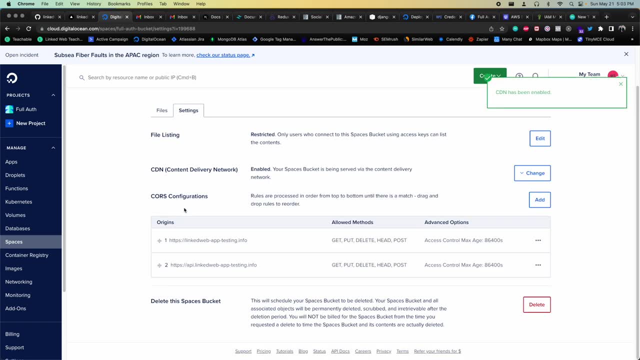 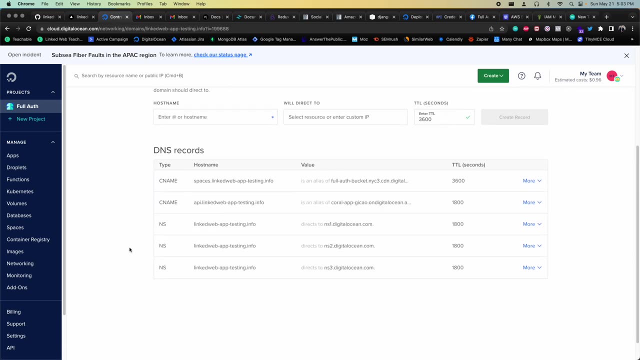 So we have to select it here and then click save. So now that should be good. So that's something I forgot to do, So with that we should now be able to go back here and then we can click on the domains, and now we have everything set up. 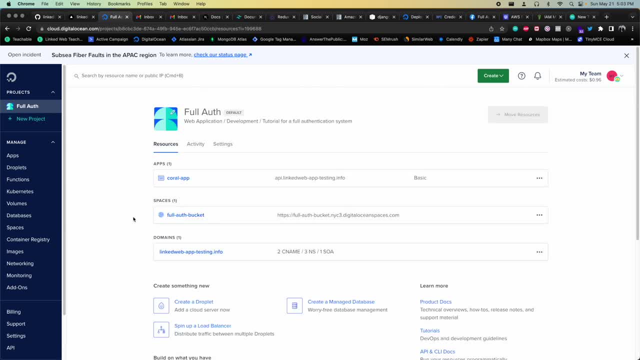 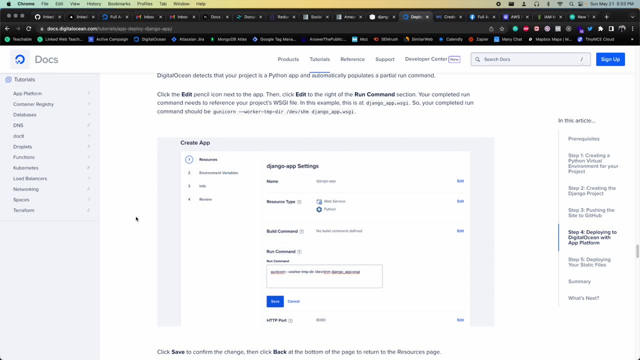 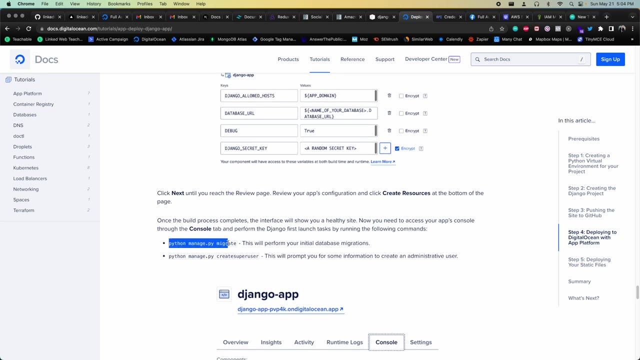 So perfect. So now everything should work, although there is one final step, and that's actually outlined in this document as well. So, once you go through everything, ah, here it is. So you're going to want to do a python, managepy, migrate and also create super user. if you want to create a super user, which in my case I do- 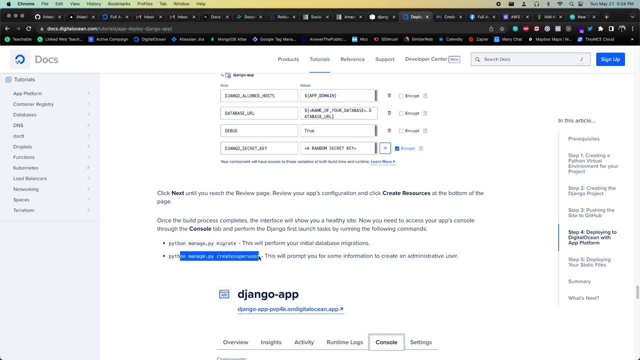 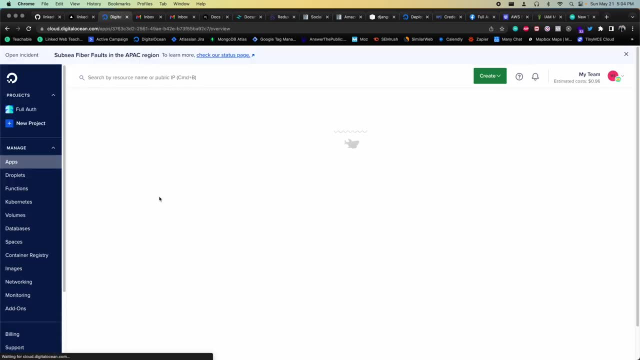 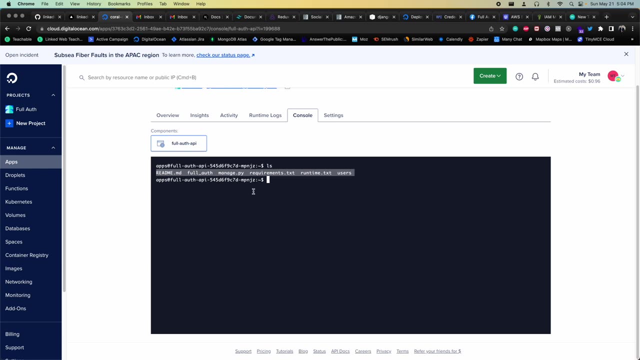 And then also, in particular, I want to do this so I can test if the static files are working in production. So now I can just go into apps, go into the console and then in here we have our project. So now I can do a python, managepy, migrate. 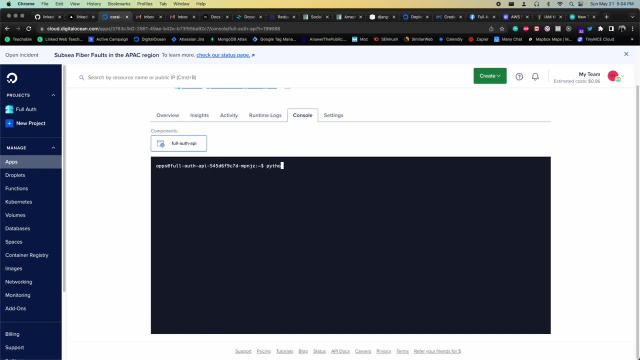 There we go. That ran all of our migrations. And finally, python managepy. create super user For this. For the email, I'll do admin at linked web app testinginfo. first name will be Brian, last name: Birkic. set my password and there we go. 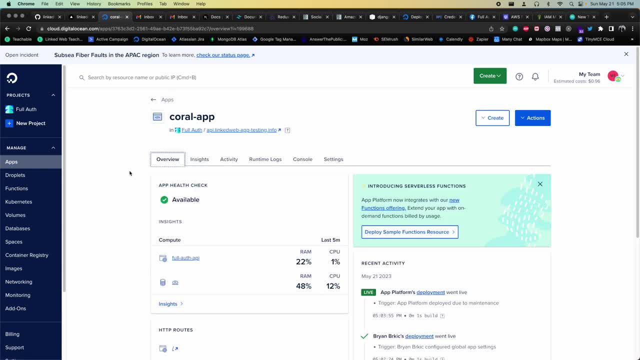 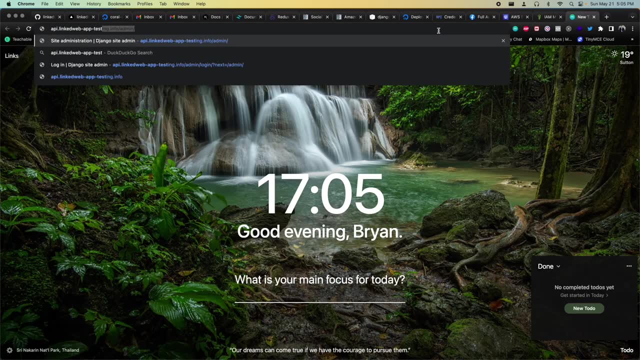 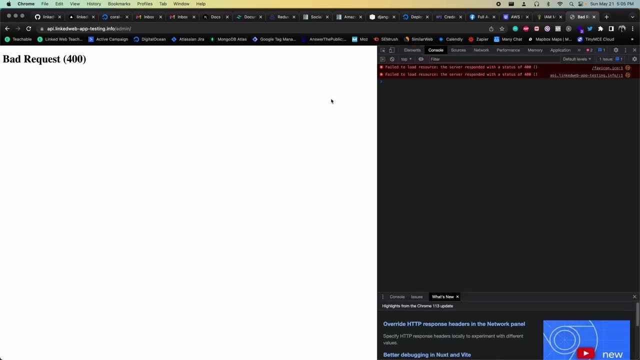 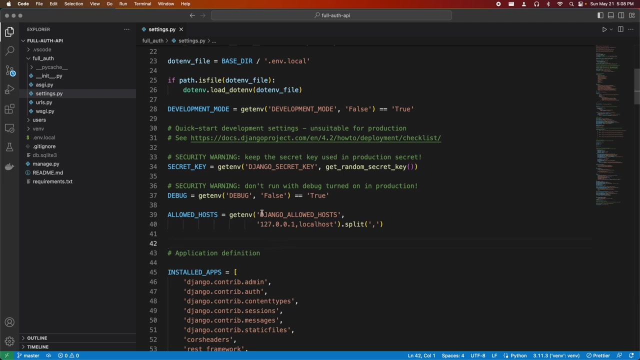 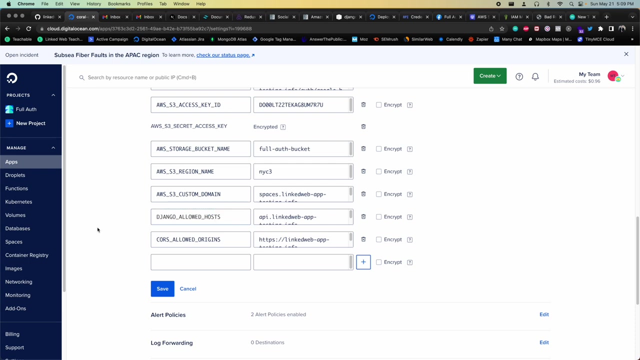 We have a super user created, so now we can test things out. so I'm going to go to apilinkedwebapptestinginfo. admin slash- admin slash- and seems something went wrong and it turns out it was actually one of the settings that I ended up configuring wrong. of course, I put an allowed hosts as my environment variable, when it should have been Django allowed hosts. I figured it might have something to do with that, so I'm going to have to edit this and change it to be Django allowed hosts and save that. 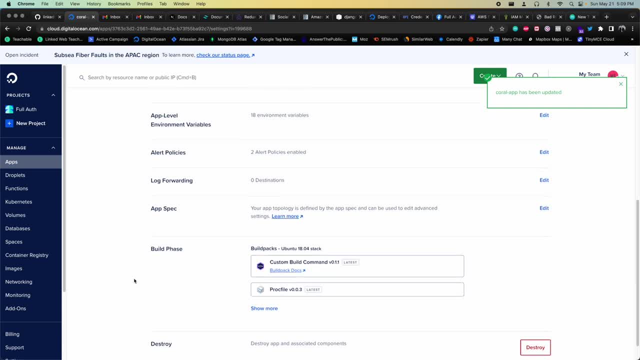 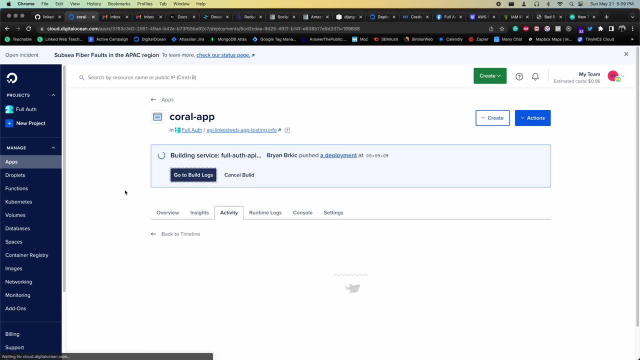 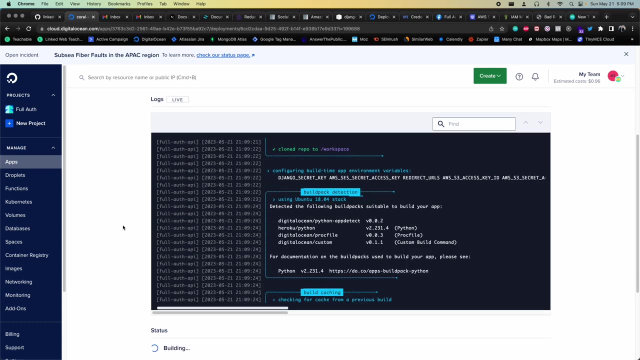 So that's going to trigger a rebuild and redeploy And after that hopefully there's no other error. Now it is very difficult to go through all this deployment process without a single issue happening, Just because there are so many steps and any little typo can just make things go wrong. 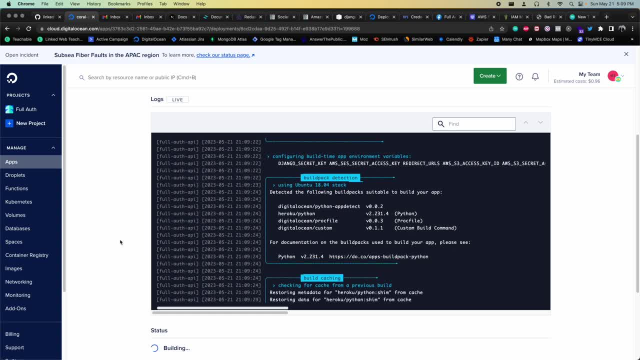 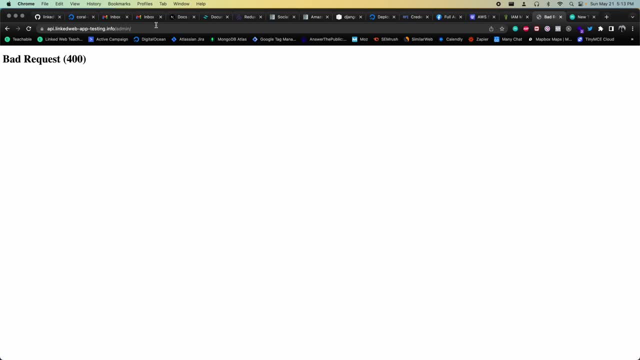 But anyway, it's going to wait for this to rebuild, redeploy, and then we'll test things out. And there we go, Our build and deployment finished up. So now the moment of truth. I'm going to refresh this page. 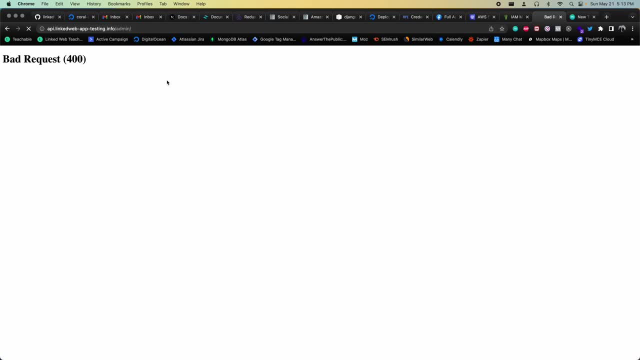 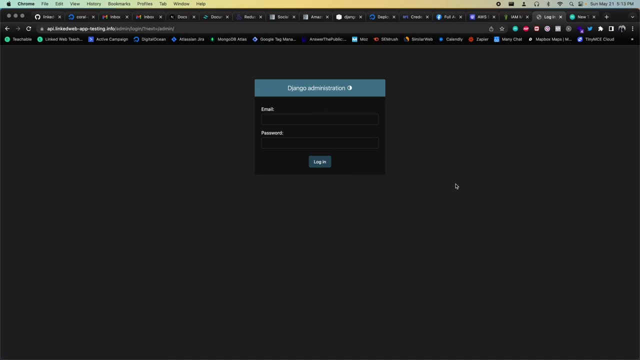 And it's loading. So let's see what happens. And there we go. We have our Django admin panel and we see CSS styling, which means our static files are working now in production. Now let's test out logging in. So admin at linked web app: testing dot info with my password. 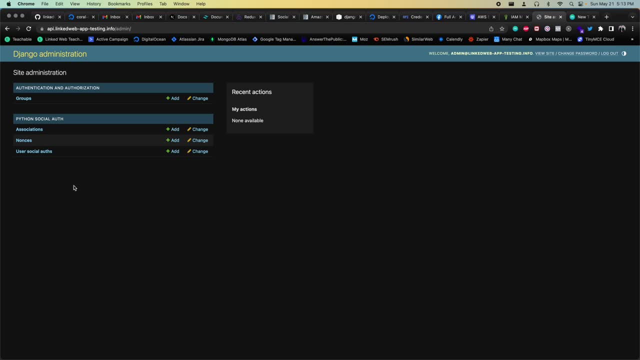 And there we go: We can log into the admin panel. Now, we didn't really configure anything inside of the Admin panel. There's nothing that we're really managing. We didn't even register the users to manage them. But all I really wanted to see was that the static files that we configured for production are working and that we can actually log in here, have all the styling working. 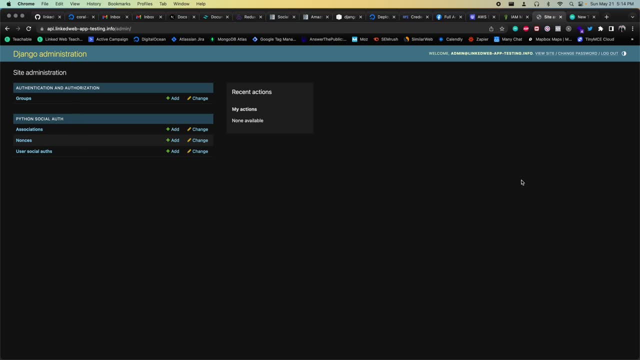 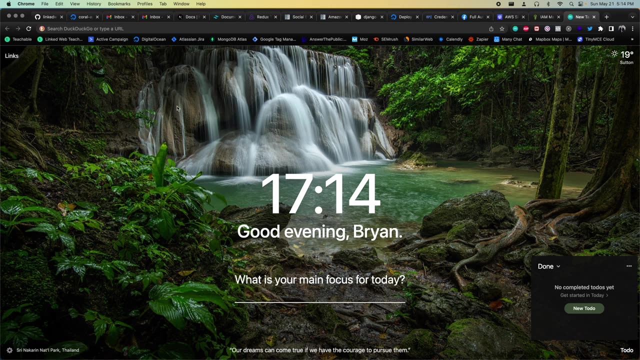 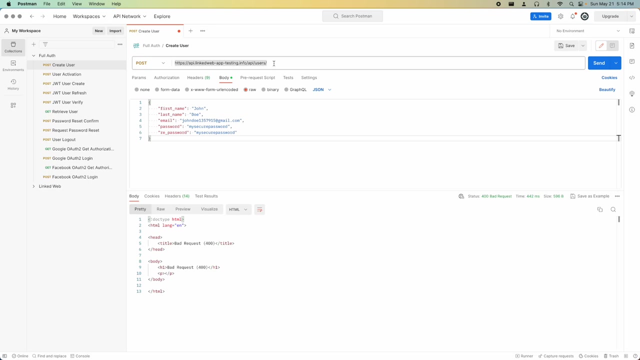 So that's really the main thing I want, Not really configuring the admin panel. So with that you can just log out. So we tested that out. So the final thing we have to do now is just test out our production endpoints. So I'm going to flip back here and now we can send this request and that's going to be for creating our user. 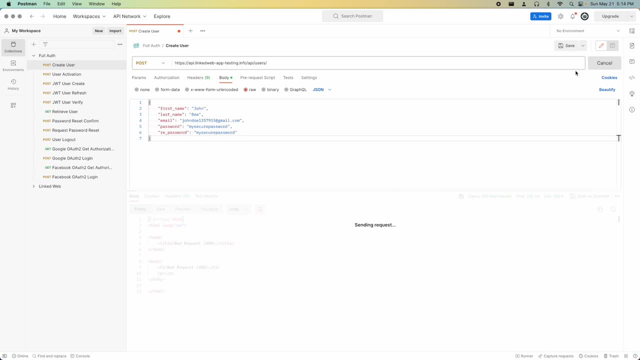 So I'm going to send this off. And there we go. Our user was created, Awesome. Now I'm just going to copy this production endpoint- because I'm going to be using that- and go to user activation and paste it in here, And then I'm just going to want to edit these values because I'm about to get a link in my email. 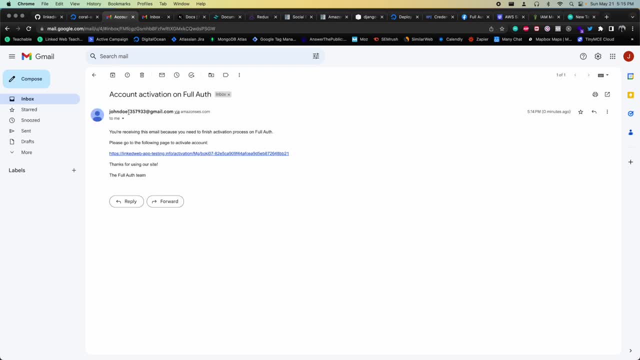 So here, if I refresh, we got an email account activation on full auth. You can also see right here, this is our production domain, So this is where, eventually, we're going to have our next JS application hosted on, And then that's going to handle this endpoint here and do the post request using the UID and token. 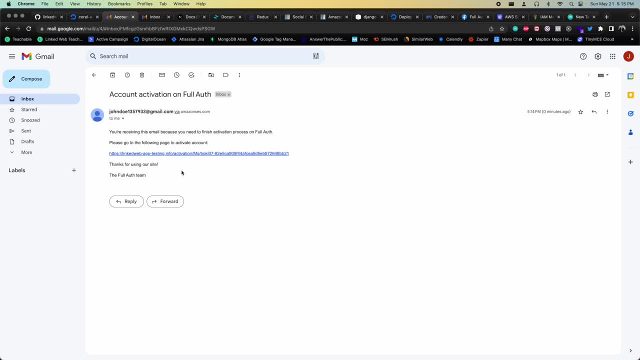 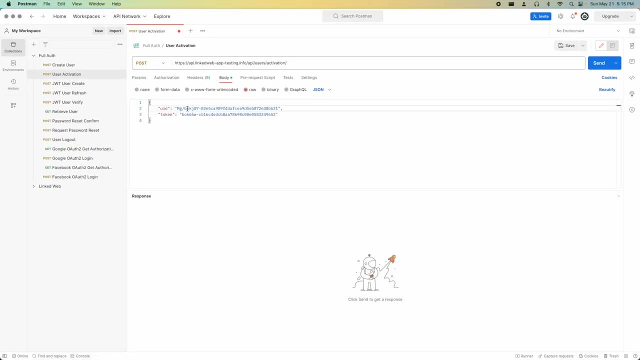 But for now we don't have that, We just have postman. So that's how we're going to hit this activation endpoint. So I'm just going to paste in here, I'm going to grab the token, I'm going to cut it, remove the slash and put the token in here. 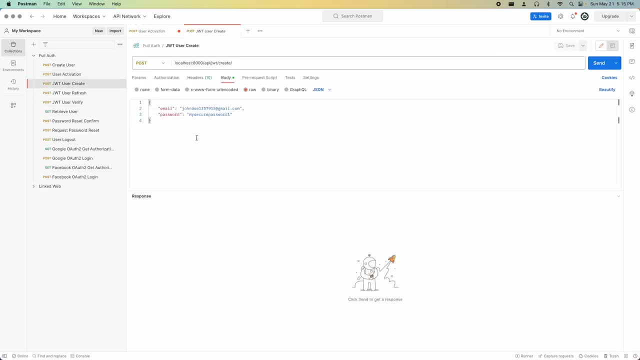 Then, before I send this off, I also want to test out the user create just to make sure that it fails. And this is also going to be with my secure password, Because inside of user create that's what we have here. And then I'm also going to grab the production domain, put that in here, save, send the request off. 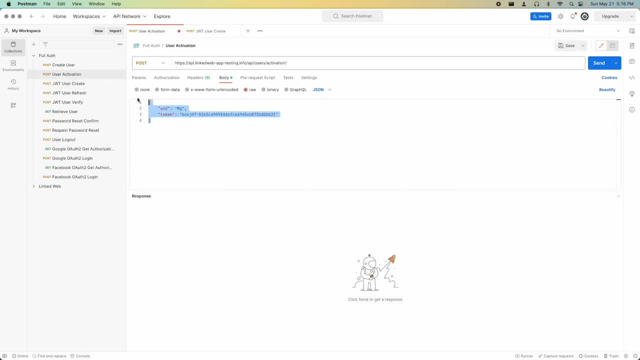 It should fail, There we go. And now if I send this off, there we go. 204, no content. So now if I remake this request, there we go. Access and refresh token. Awesome, Awesome. And then another thing is that in my cookies we're going to notice we have the cookie setup. 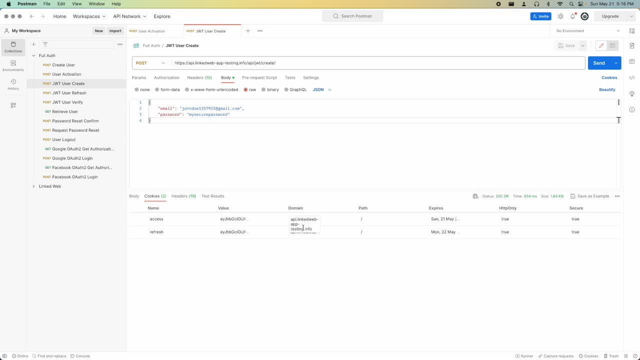 We have the domain set, which is going to be apimydomain. We have the path HTTP only and secure is true, So these are getting sent through an SSL connection. So awesome, We got that. Now we can also hit our refresh. 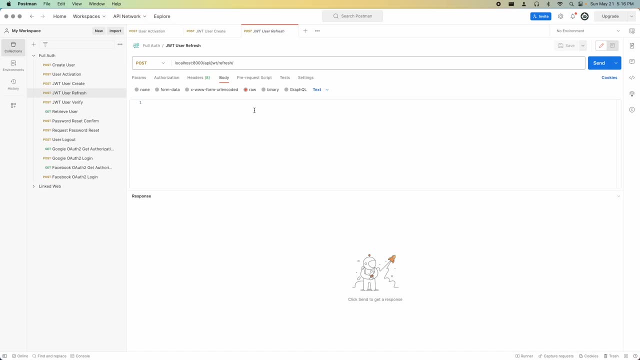 And it's also super easy now Because we don't have to go into the body and add a refresh token, We can just send the request off. And of course I forgot to adjust the production domain. I'm going to put that here and there we go. 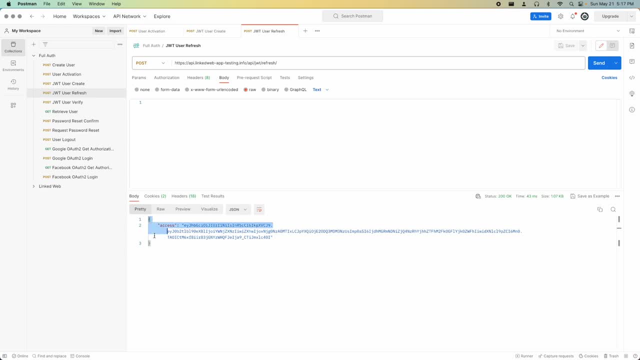 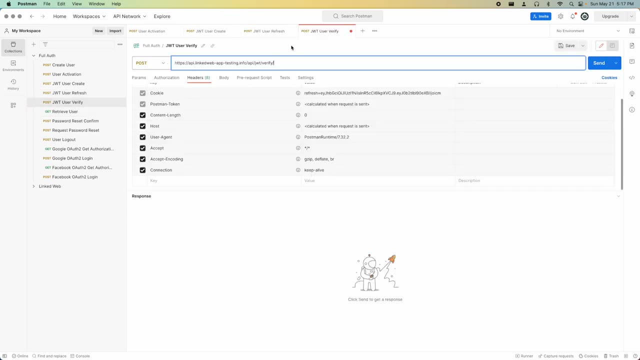 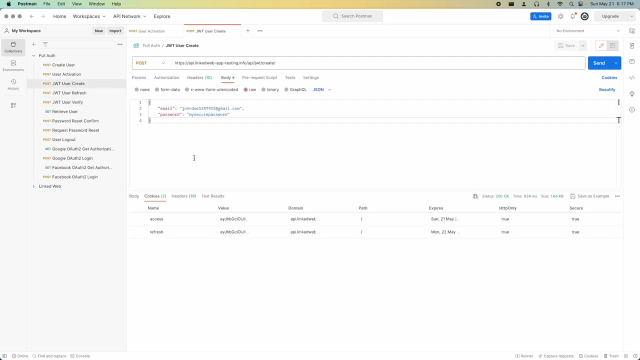 Got back a new access token which, of course, you can grab it from the data but also in our cookies. it was updated now. Then we got to verify which we can also hit. There we go 200.. Okay, And we can also hit our retrieve user endpoints. 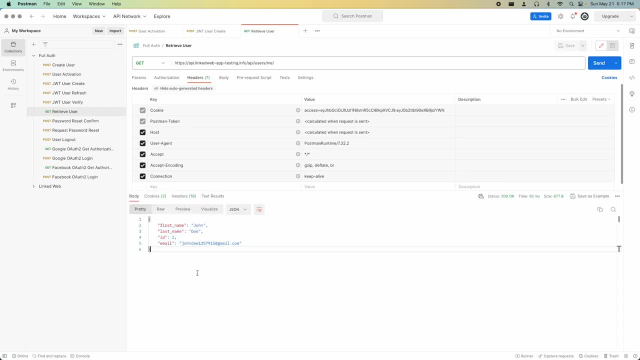 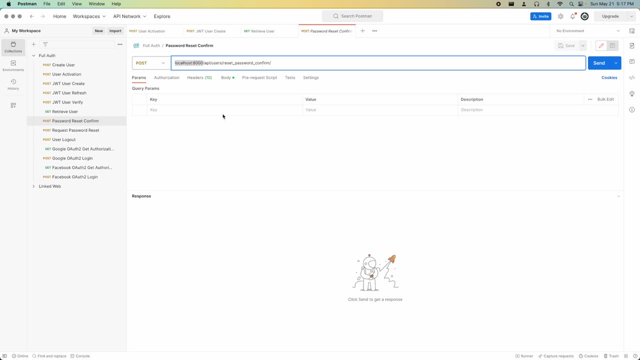 So we have to be authorized to hit this. and there we go, We get our user details. We can also test out resetting our password in production. So this is the confirm one. I want to do this one first. I'm going to send this request. 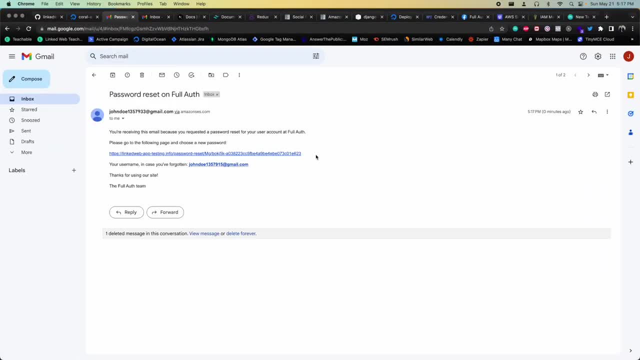 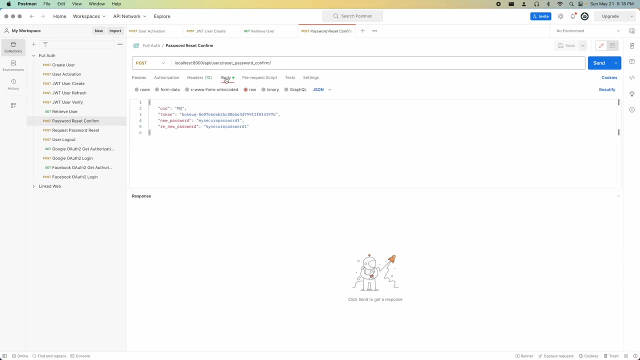 Then I should receive an email. There it is, And here we have the production URL. So what I want for now is just the UID and token, And then I'm going to go to the confirm one, go into the body, paste the contents. 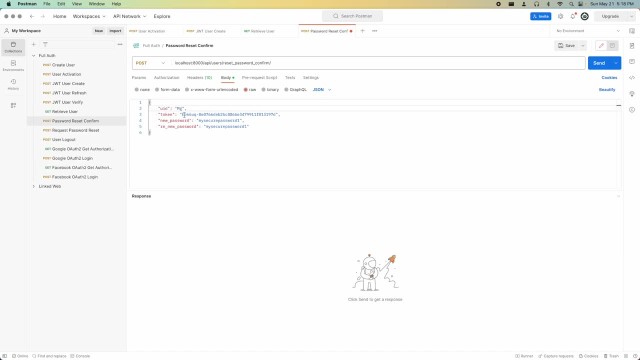 They're going to grab the token, cut that, remove the slash and put the token here. I'm going to reset the password to this right here, Just like we did during development. I'm going to send this- I forgot to update- to the production endpoint. 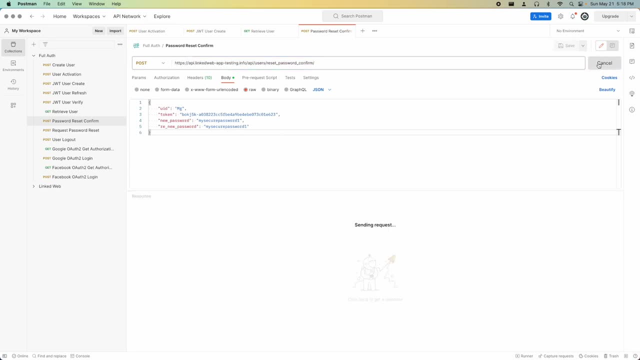 So I'm going to update that save and send There we go. 204, no content. So that should have worked, which means that right now, with my create endpoint, if I send this off, it should fail. There we go. 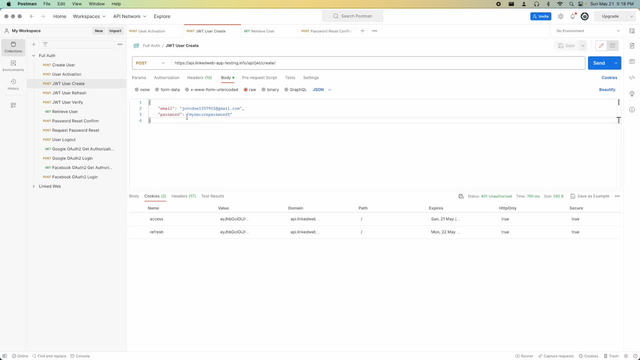 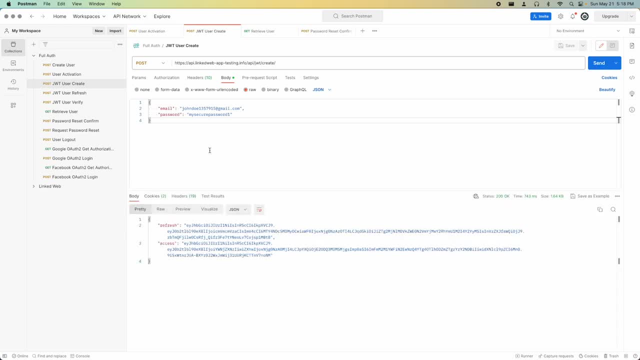 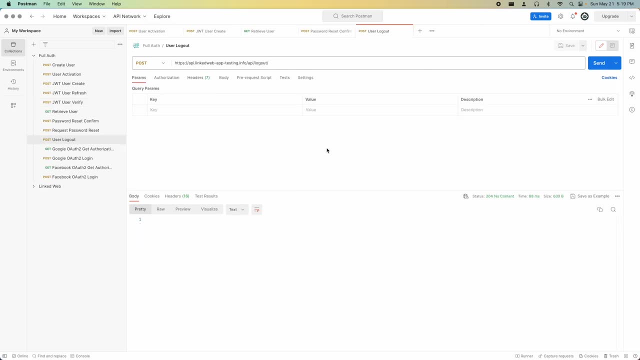 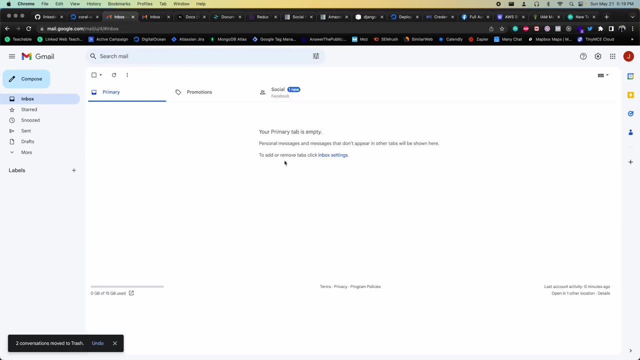 There we go, We have no token, And then that leaves us with only our OAuth endpoints left. So that's the last thing we have to test out, And then for those we are going to have to configure some things. So first I'm gonna have to go into the console. cloud googlecom. 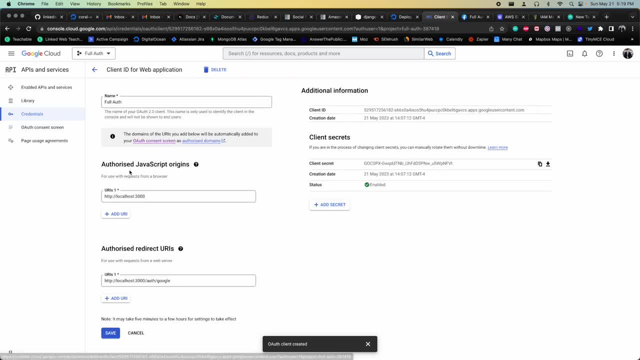 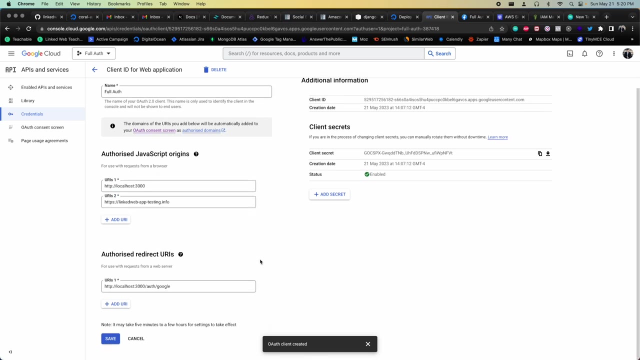 I'm gonna have to go into the OAuth 2.0 client IDs And I'm gonna have to add a URI for both of these. So for the origin I'm going to need HTTPS linked web app testing dot info And then for the 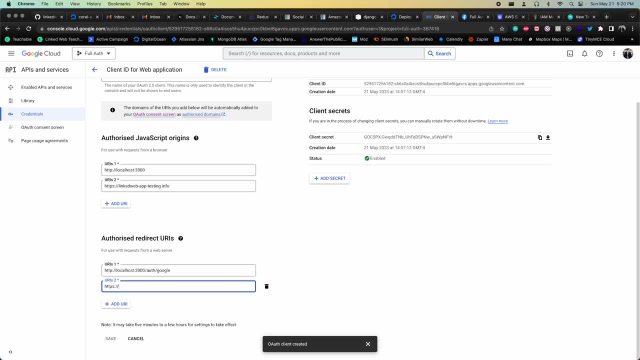 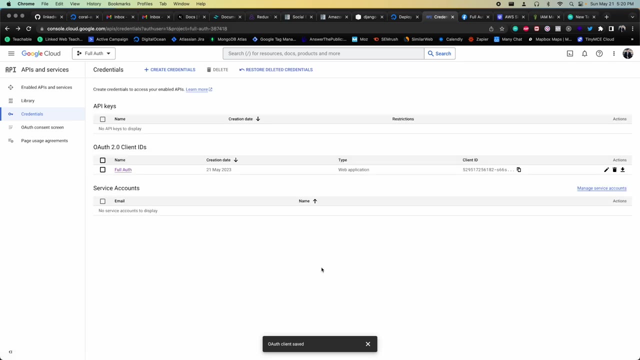 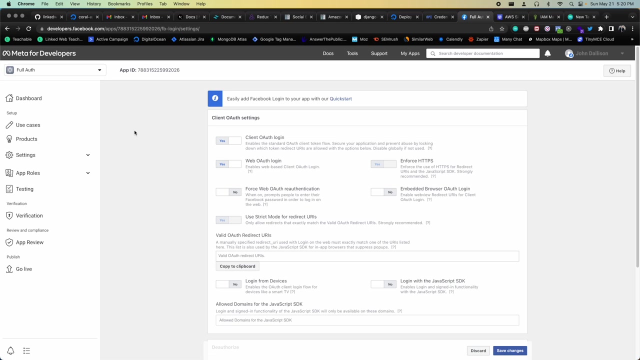 authorized redirect URIs. I'm gonna need HTTPS linked web app testing dot info slash, auth slash google. So this is going to allow this to work in production And then I'm also going to have to go into here. So this is in my developer Facebook login app. I'm gonna have to go into my valid. 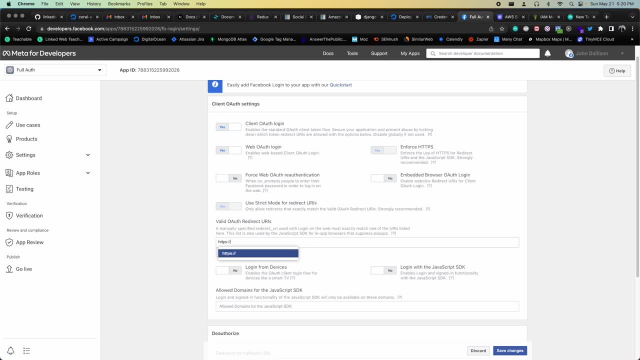 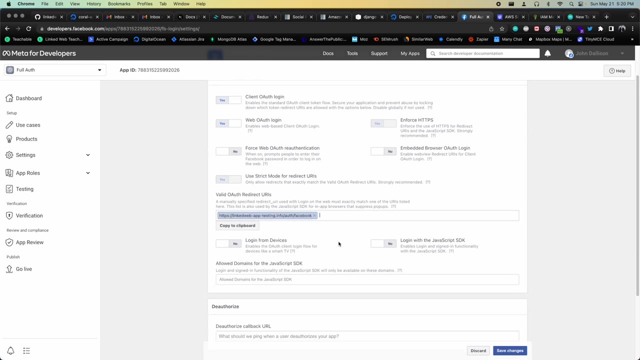 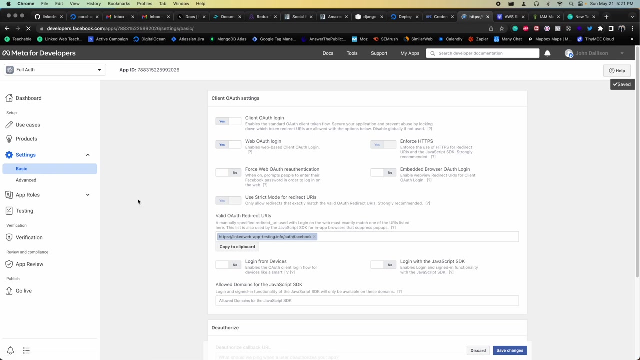 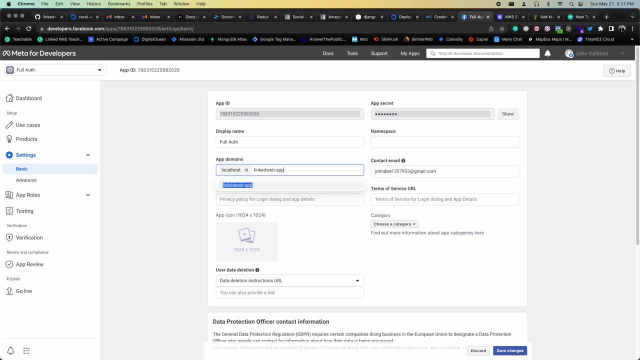 OAuth redirect URIs And then here I'm going to add HTTPS linked web app: testing dot info slash. auth slash- Facebook. That's my valid OAuth redirect URI. I'm going to save those changes And then, under basic settings, another thing I can do is under app domains, I can add linked web app. 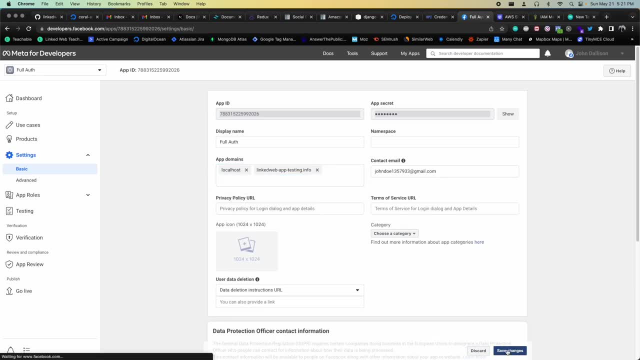 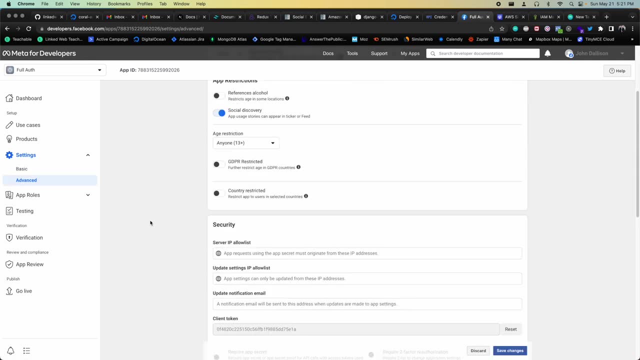 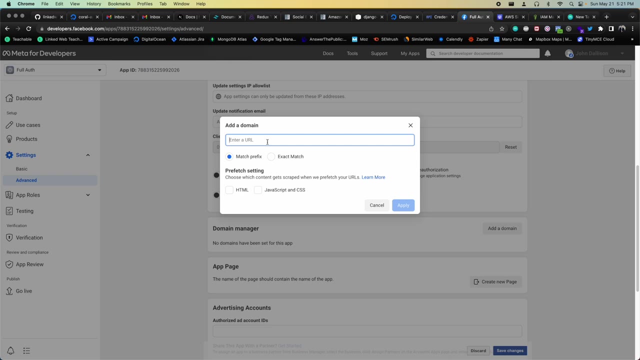 testing dot info And then also under advanced. another thing you can do is also add domain manager And you can also add here as well. So I'm going to do HTTPS linked web app testing dot info And that'll be an exact match. 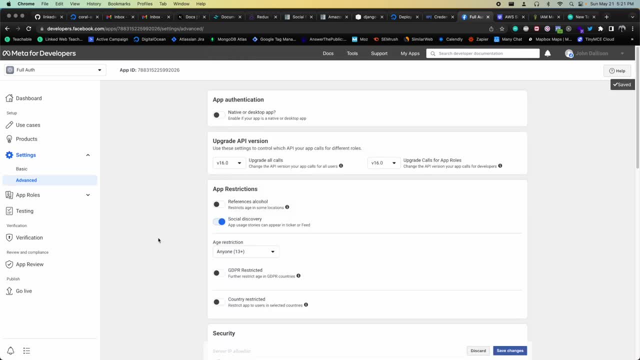 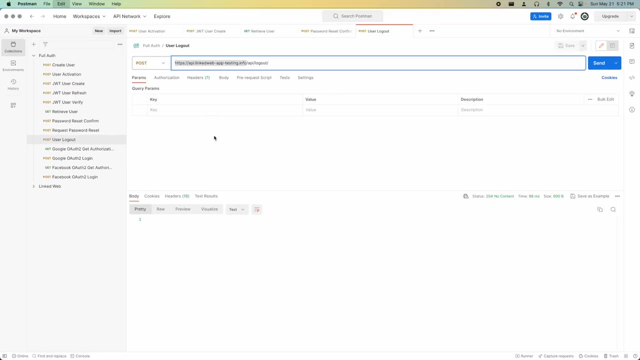 And I'll save those changes. So there we go. Right now, everything should be set up for us to test, So let's try it out. I'm going to copy the production URL. I'm going to close up some of these things. 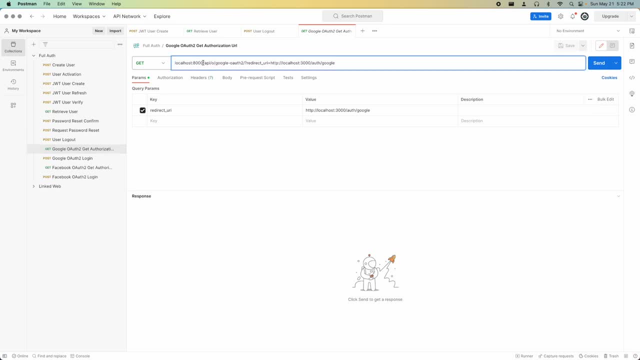 And first let's test out Google OAuth 2.. I'm going to paste this in here with the redirect Send that off And, yes, I need to actually change this here to also be the production version. So that's going to be HTTPS linked web app testing dot info slash- auth slash Google. 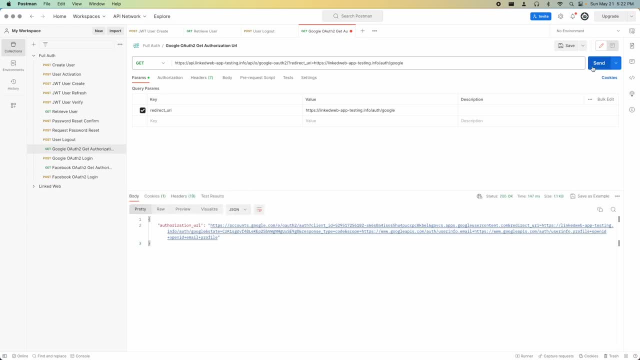 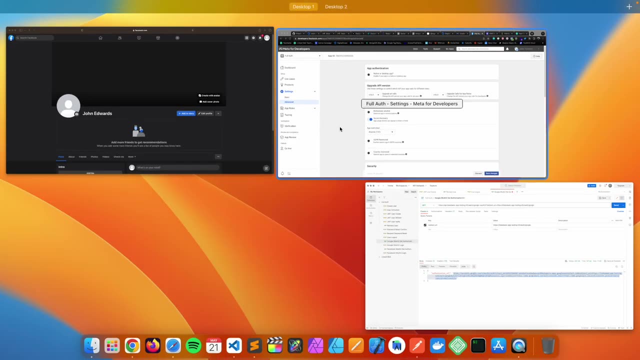 So we got to make sure we have that correct as well. I'm going to send that And there we go- Authorization URL. So now I can just copy this And then in a new tab I'm going to paste that: Click enter. 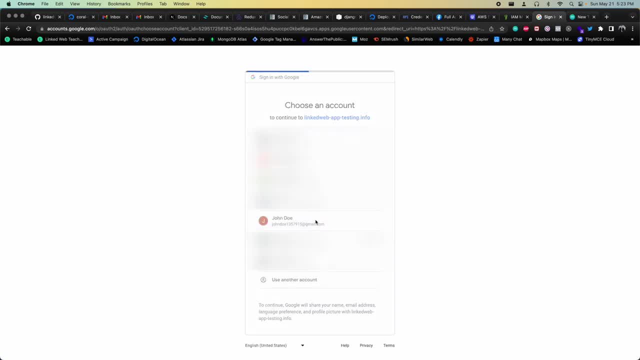 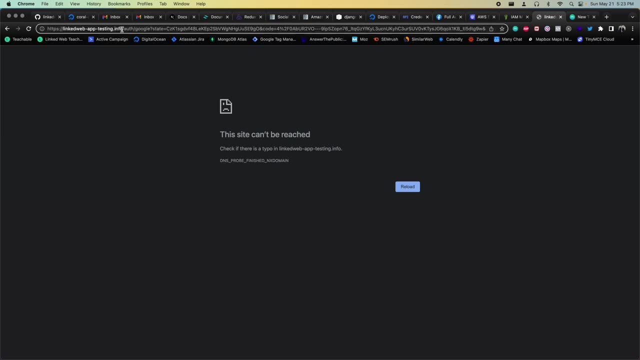 I'm going to use my John Doe one, three, five, seven, nine, one, five account, And there we go. We are now redirected to linked web app testing dot info slash, auth, slash, Google, which is perfect, Of course, we don't have our front end running here quite yet. 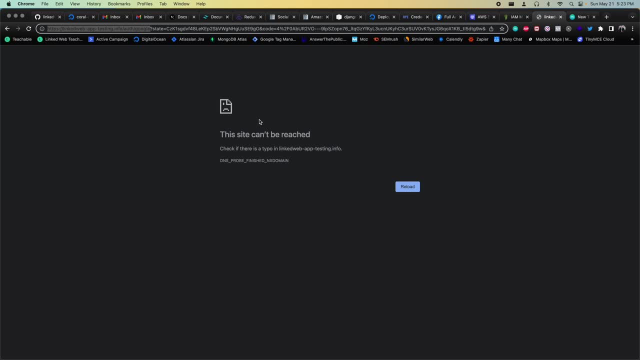 But eventually we will And this is what's going to handle that post request. But we can still test out that post request. So I'm going to grab with these query parameters the state and the code. So I'm just going to copy everything that's here. Go back to Postman. 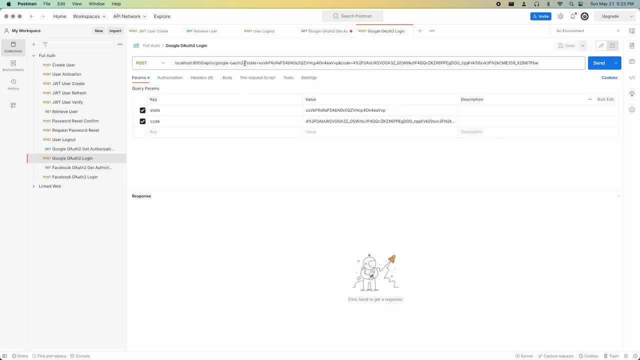 I'm going to open up the Google OAuth 2 login And then I'm just going to delete what's here. I'm going to do question mark paste, And then there's a couple of things I don't need that are here. So I think all of these. So there we go. We just have state and code now. 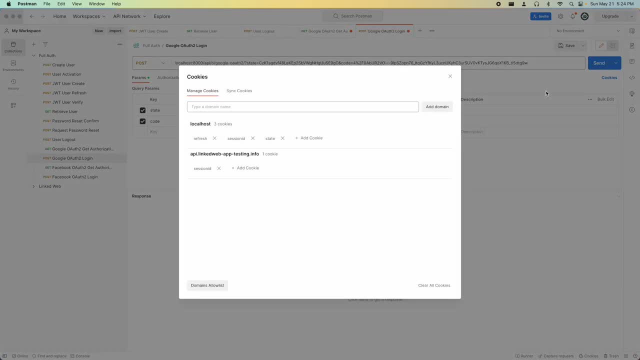 And the other thing I'm going to have to do is copy the state. Go to my cookies, remove the one that was there, Add a new one. It's going to be this state value, And then I'm going to have to update this to the production URL. 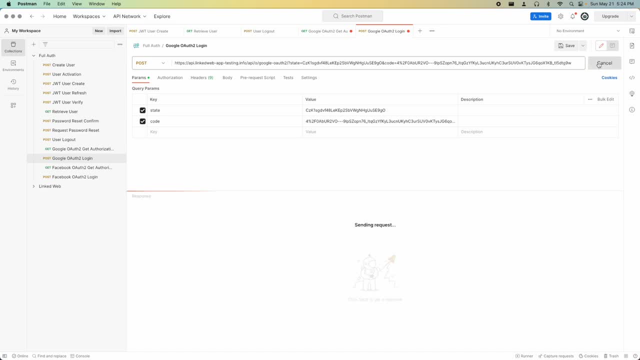 So there we go, And with that we should be good. So let's send this request. There we go. We successfully created an account using Google OAuth 2. And that was in production. So the final thing we're going to test is now Facebook OAuth 2 in production. 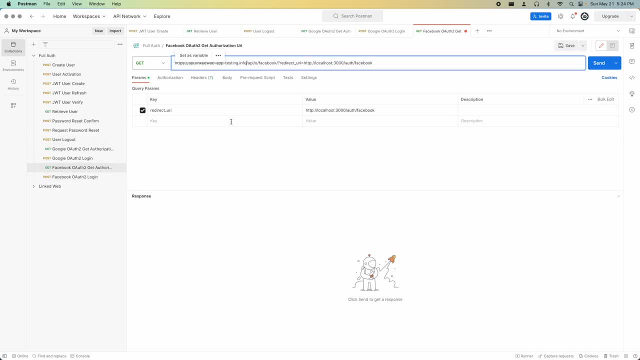 So first I'm going to go here, I'm going to paste this, And then also I'm going to update the redirect URI And actually I'm going to test it also without doing that. So there we go. We get that same error as before. 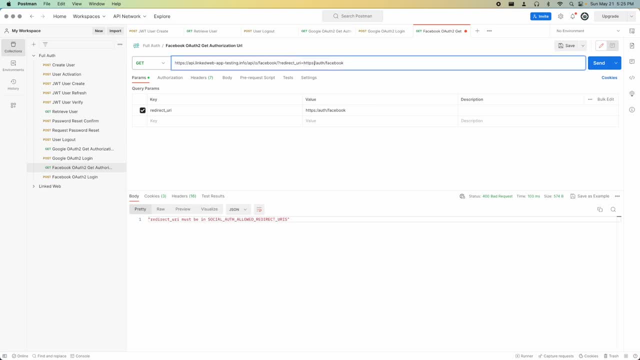 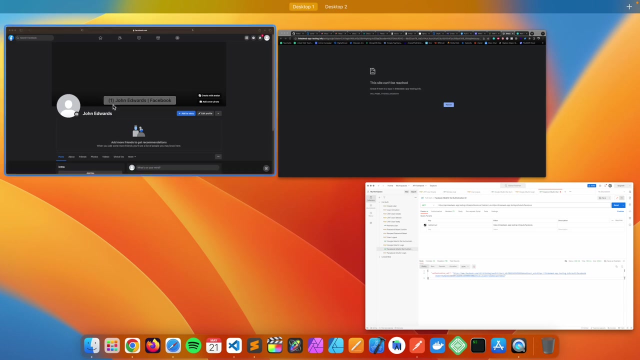 So let's update this And then we'll send this off, And now we get the authorization URL, So I'm going to copy that And then, in this case, I'm going to go into this window here where I have John Edwards. 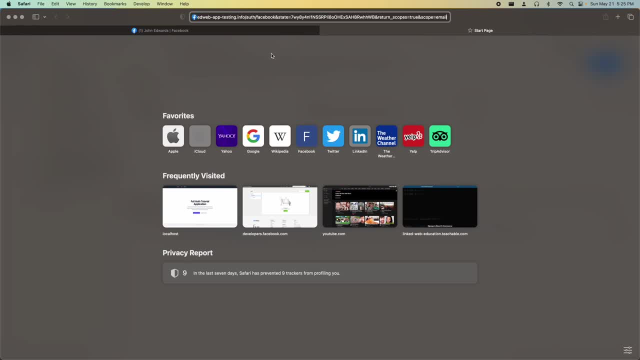 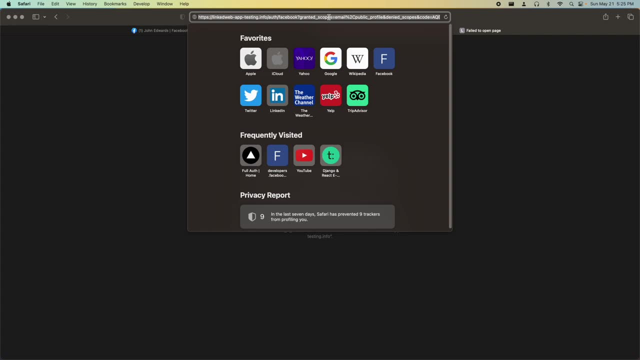 So that's my test Facebook account. Paste this in here And then if we take a look, of course we don't have anything running here, But we are brought to the correct place. Link to mbaptestinginfo- infoauthfacebook. 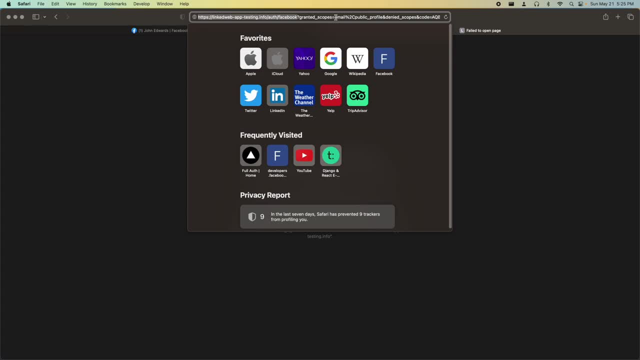 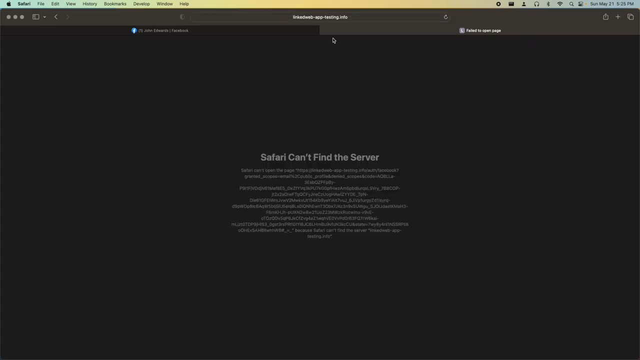 Which is where our Nextjs app will run in production and handle this post request. But what we can do right now is just grab everything in the query parameters And just copy that And then I can close this. Go back to Postman. 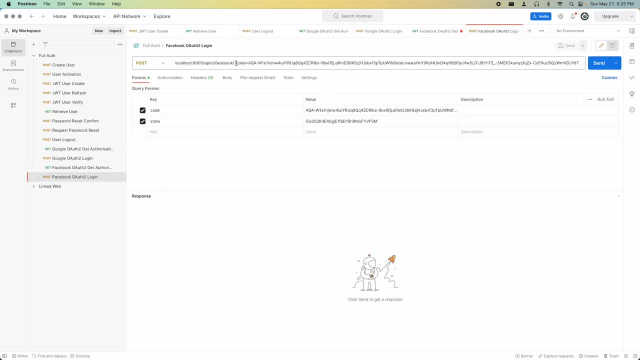 Open up Facebook OAuth 2 login And then I'm just going to delete everything here. Paste what I just copied And I'm just going to remove some of these things I don't need And only have my code and state in here. 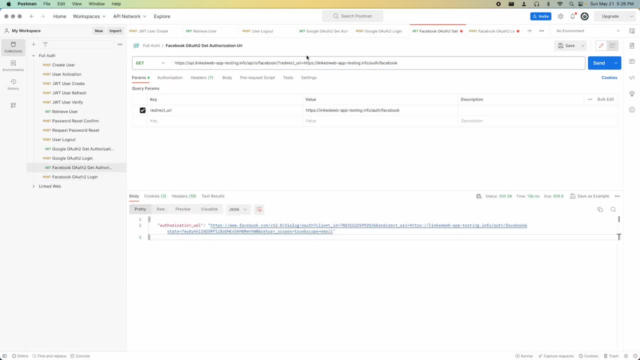 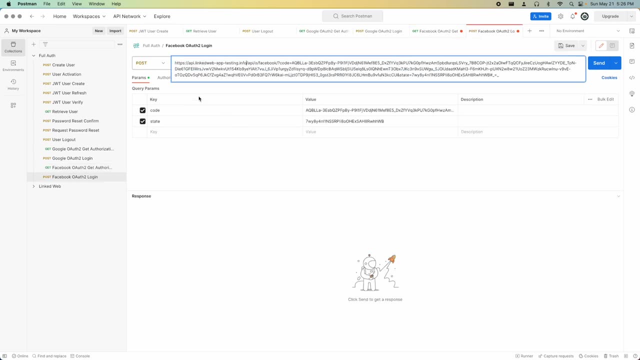 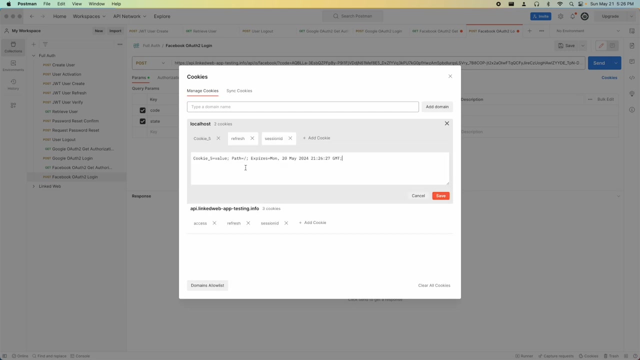 Then I'm going to have to update this to the production URL, Paste that there And the final thing I have to do is grab the state value, Go into my cookies. I'll delete the one that's there. Create a new one. 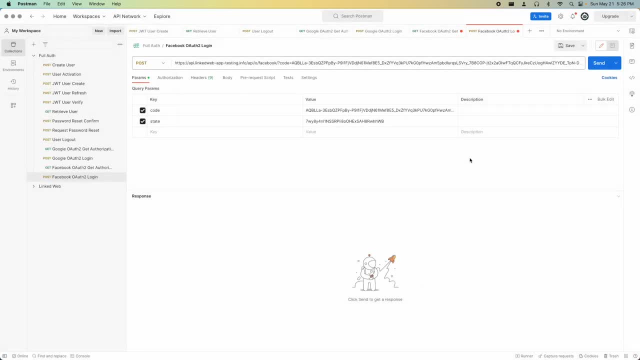 Paste, Save, And now, when we hit this, it should work And it does. Awesome. Now we also have Facebook OAuth 2 working in production, So that is super cool. So now our backend API is officially deployed and working, So with that, if you wanted this to be a little bit more production ready. 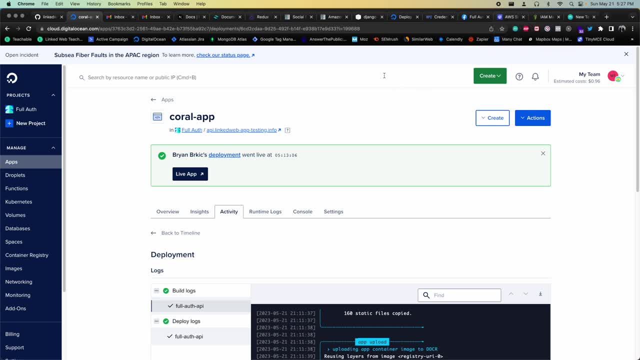 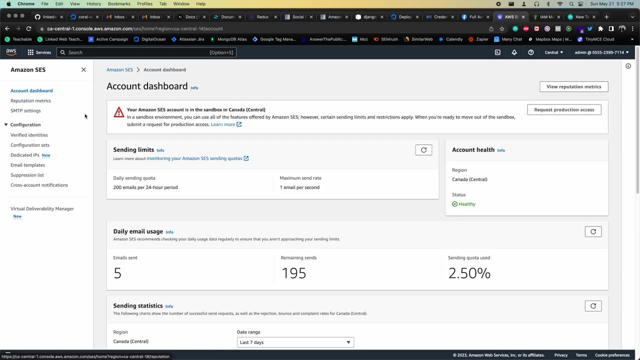 Then, of course, what you can do is with your AWS SCS, Push that to a production version, Because right now Also, I'm probably going to be logged out, Maybe not. So here we have, by default It's in the sandbox environment. 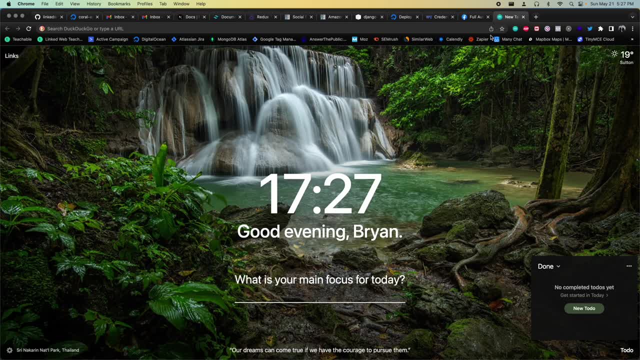 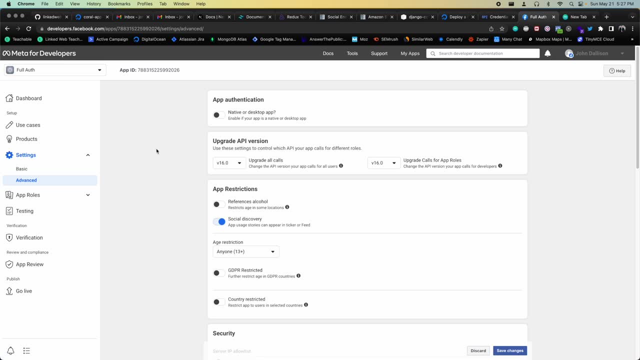 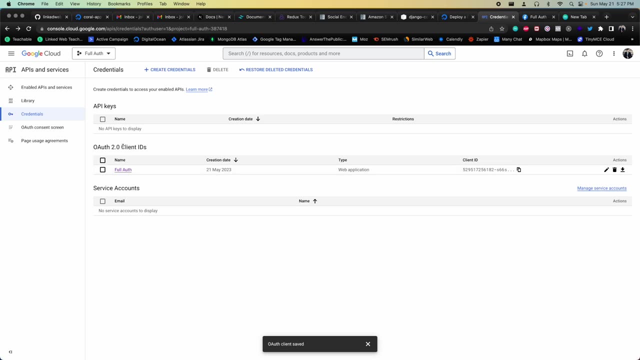 But you'd want to request production access. So that's one thing you'd want to do. Another thing is you'd want to go live with your developersfacebookcom And then with your googlecom. You'd probably just want to create a different set of OAuth 2.0 client IDs. 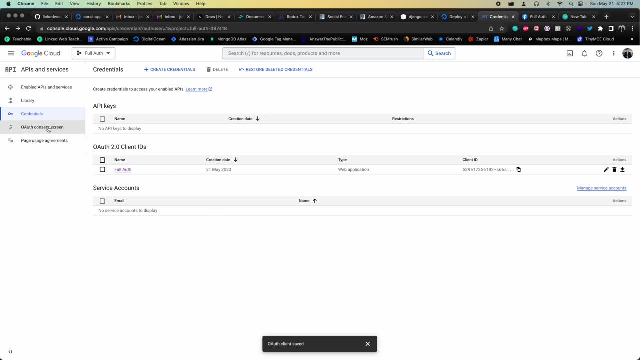 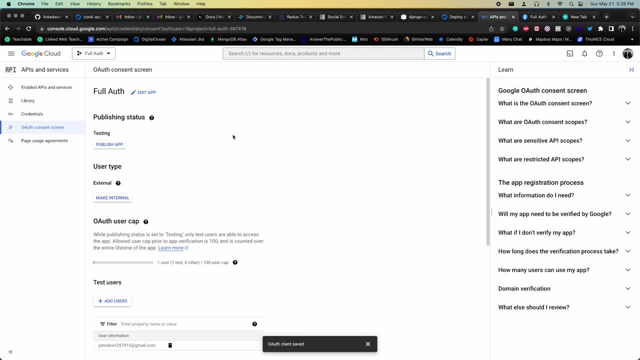 And use those for production. And then I'd say: Actually there's one more thing. You'd want to go to your OAuth consent screen And also publish your app, Because right now it's in testing, But you'd want to publish it. 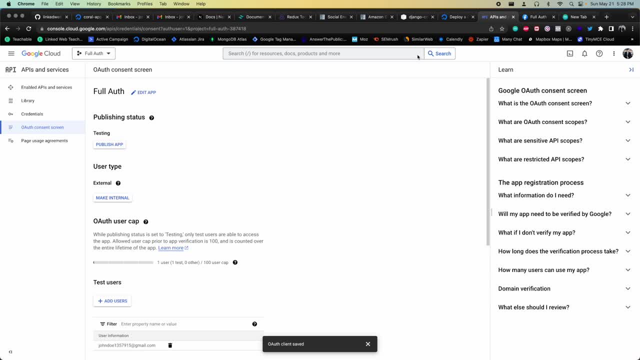 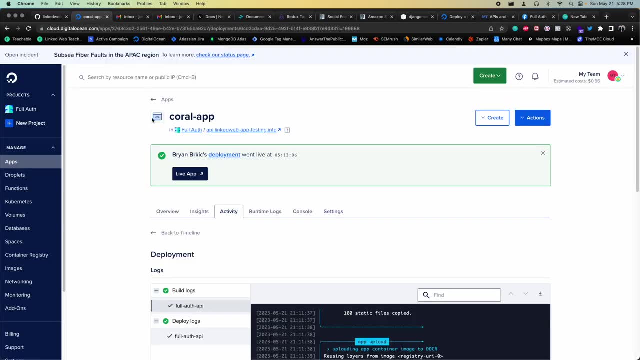 And then you would be production ready. So that's pretty much the only things you'd have to do In terms of the Google and Facebook OAuth 2.0. And then you'd be good to go. So there we go. That's literally our entire app now deployed. 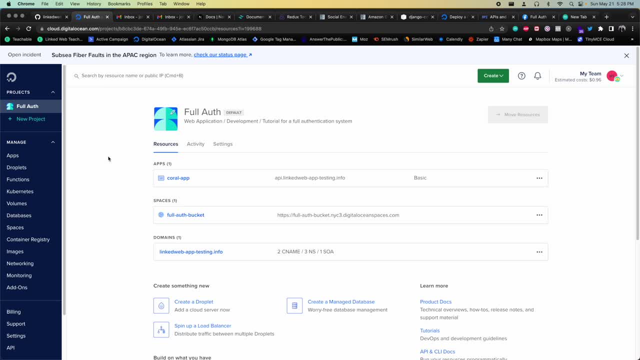 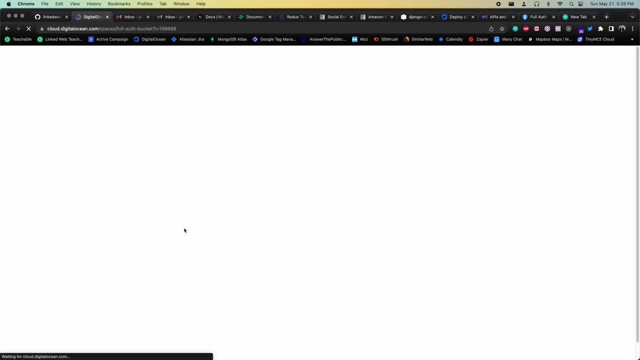 With DigitalOcean app platform And DigitalOcean spaces. So I'm just going to show one final little thing, And this is going to be with our DigitalOcean spaces, And it's not something that would come into play with our app right now. 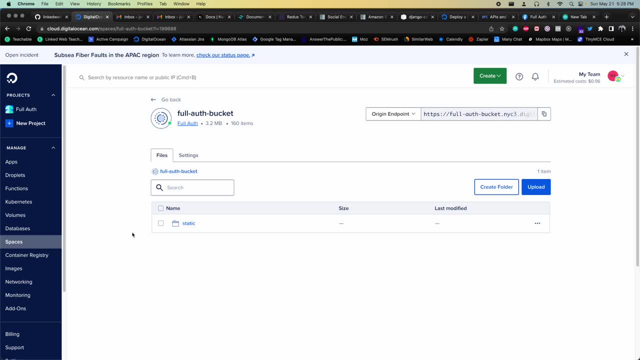 But if you had media files, They would now go inside of the static folder. So that's going to be the final thing I'm going to show. We're not going to test it because we don't really have a way to test it. 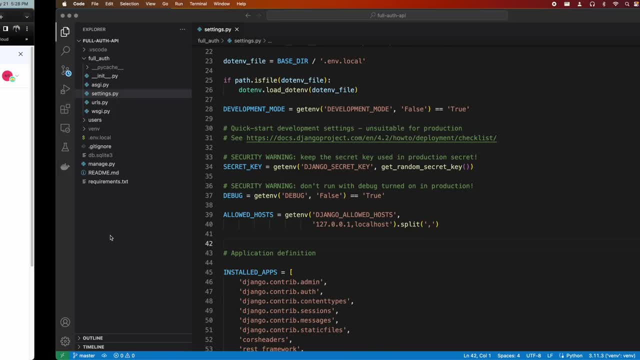 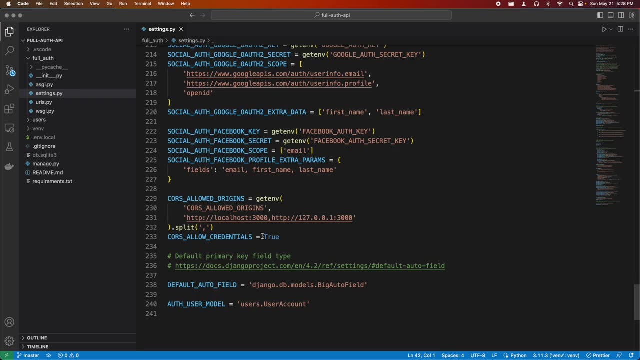 But I'm just going to show you how to do it, Just because it's a common thing you might do. So what you're going to do In order to have this behavior, So where we have our static settings, Which is right here, 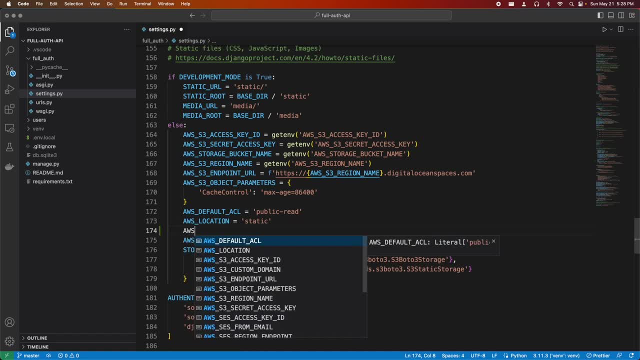 Right now we have this AWS location. We're going to add another setting, AWS media location, Which is going to be media. Now, this right here is not a setting that is part of the Django spaces package. It's just something that we have. 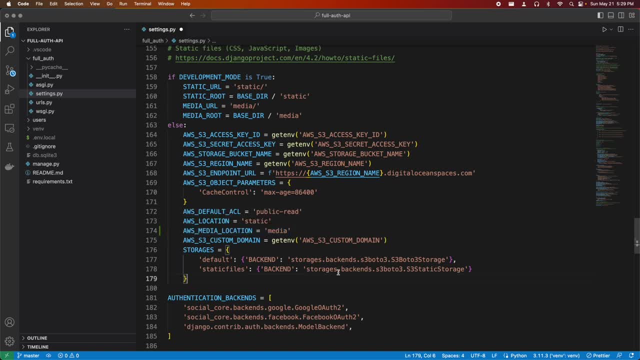 That we're going to use And we're going to set up a custom class Which is going to inherit S3Boto3 storage And then we're going to apply it here And it's going to use media Instead of static as the folder. 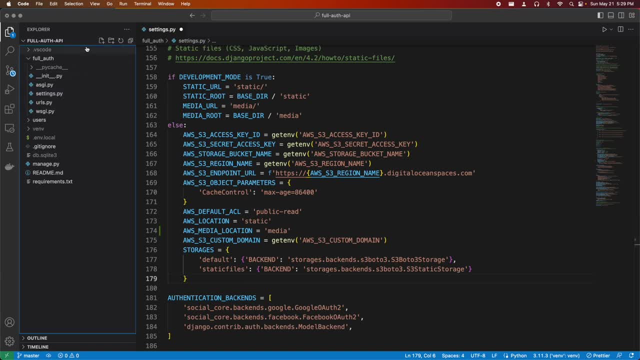 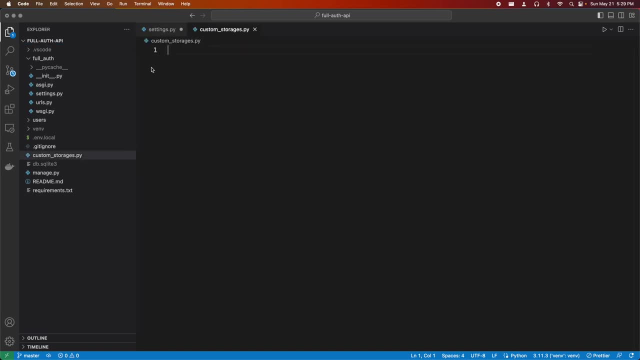 So that's going to be the final thing we do. So what I'm going to do is I'm going to create a file called custom underscore storages dot pi. Now, ideally, I would like to have this file be in, let's say, the project folder. 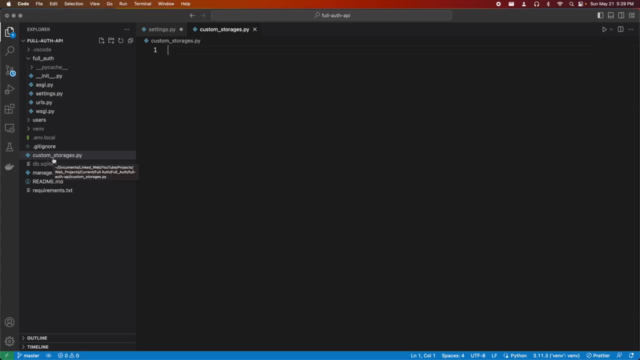 Except the only problem is that you can't create a path to it, So I think the best place is just in the root for this file, And then I'm just going to copy this, Paste it here And then from storages: backends S3Boto3. 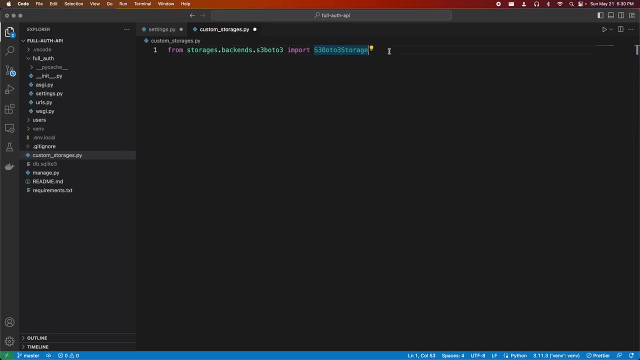 I'm going to import S3Boto3 storage. I'm going to create a class which is custom S3Boto3 storage Which is going to inherit this. It's going to set location equal to that setting we made. So I'm going to do from Django conf import settings.